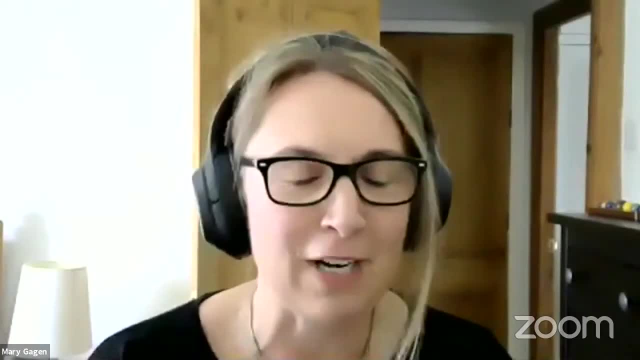 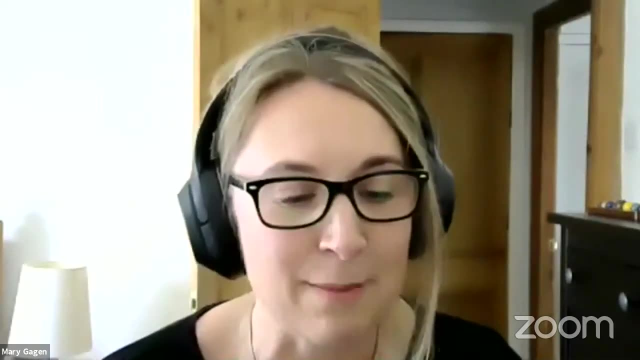 I'm just going to give a really short recap introduction for anybody who wasn't in the initial session yesterday to hear Dan's intro, Just to give a little bit of background about what this symposium is all about. back in 2010, the Geological Society produced a statement. 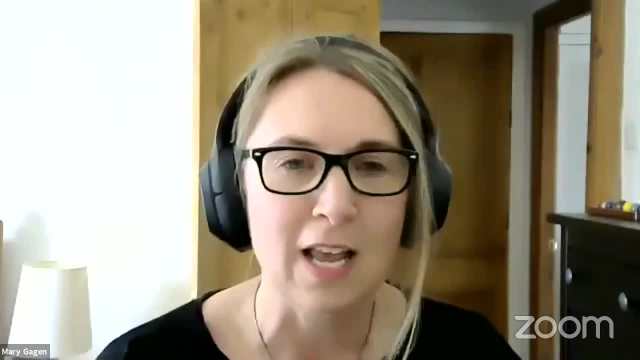 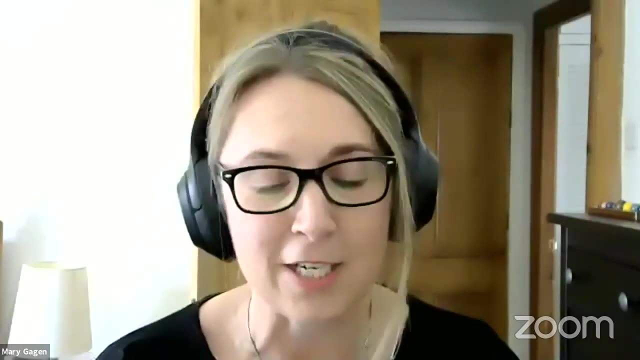 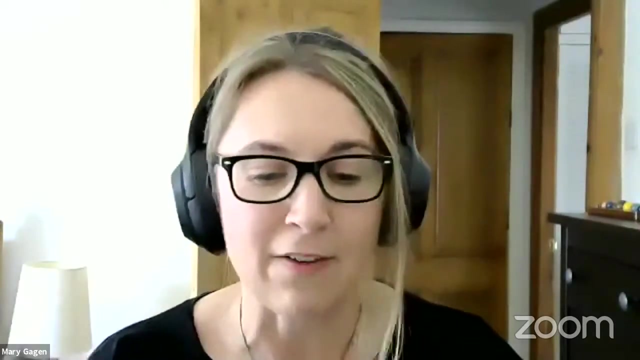 called Climate Change Evidence from the Geological Record, and that was to update the 2010 statement with our best information about the latest research, And then, in 2019, the Geological Society and the UK Paleoclimate Society jointly convened an expert working group to produce. 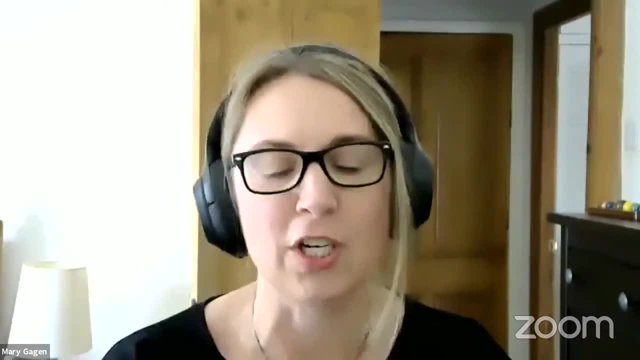 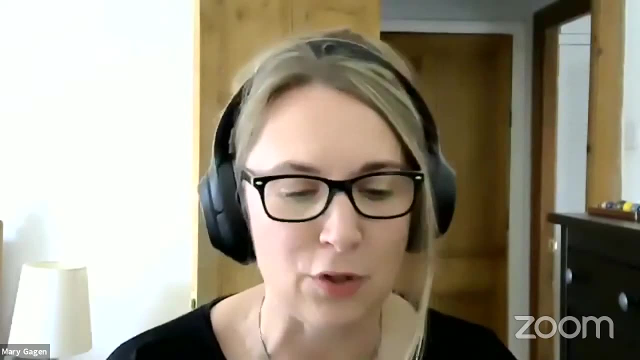 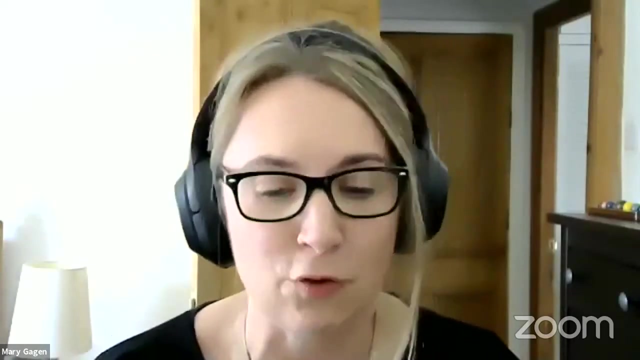 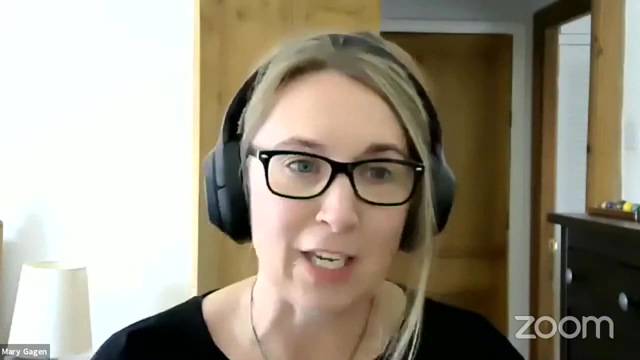 an update to that statement which was published in the Journal of the Geological Society, And that statement was structured around nine targeted questions and this symposium follows that structure, with nine invited speakers exploring those same questions and giving an opportunity to summarise our understanding in those areas. 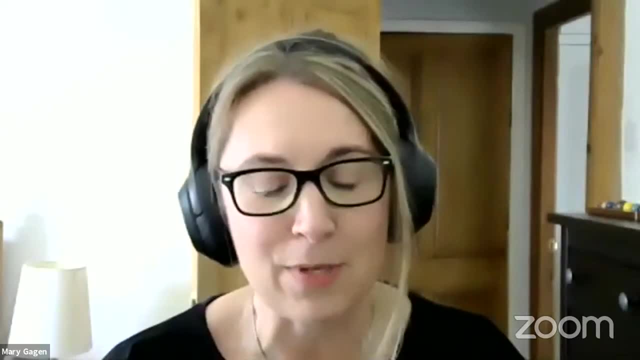 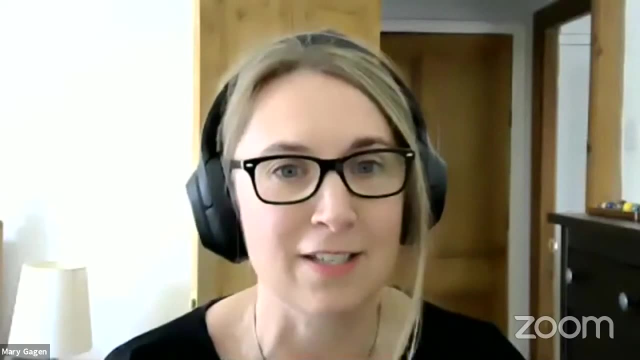 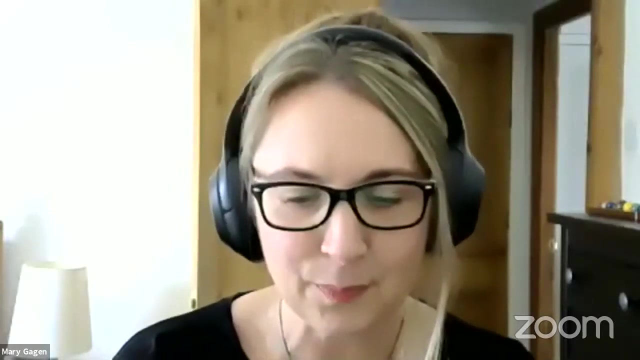 In addition to our invited speakers, the Geological Society has a commitment to supporting a new generation of early career scientists, and over these two days we'll hear from five early career scientists with shorter flash talks. We've got two of those talks this afternoon in the first part of the session. Finally, we then had an open call for abstracts, as 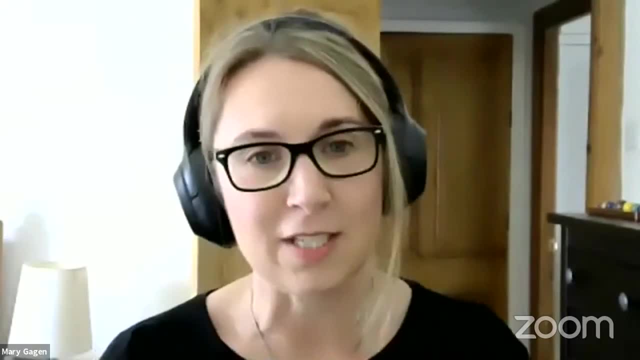 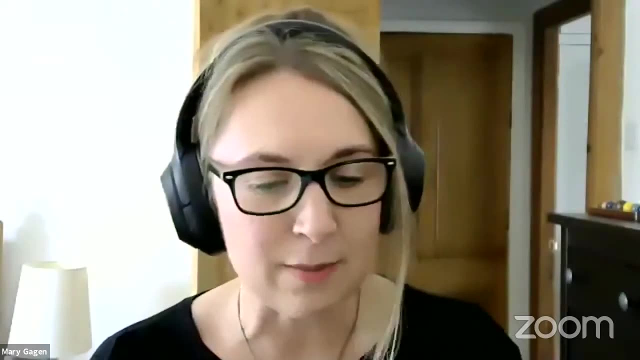 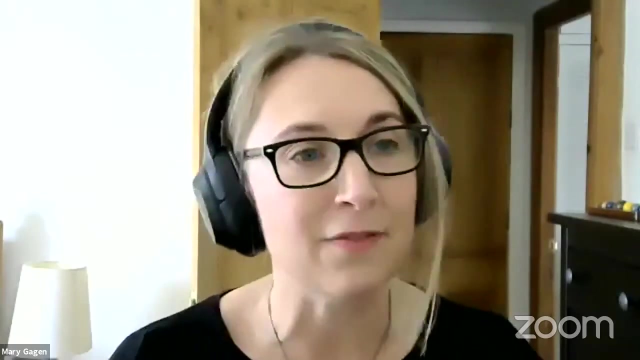 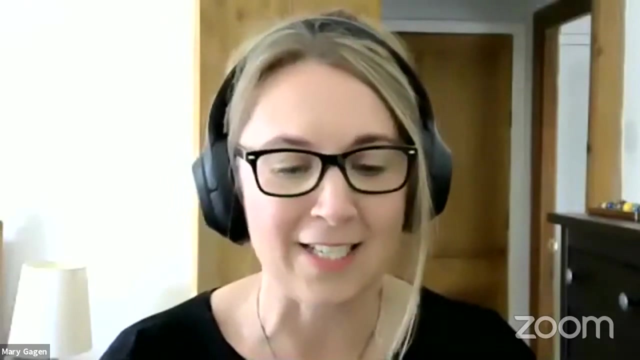 part of this symposium and had a large number of submissions, and the Society and the Committee took the view, in the interest of inclusivity, to give everybody who had submitted an abstract question, their work and their opinions in the form of one minute flash presentations and an open poster session. And that session is after the two talk sessions today and the 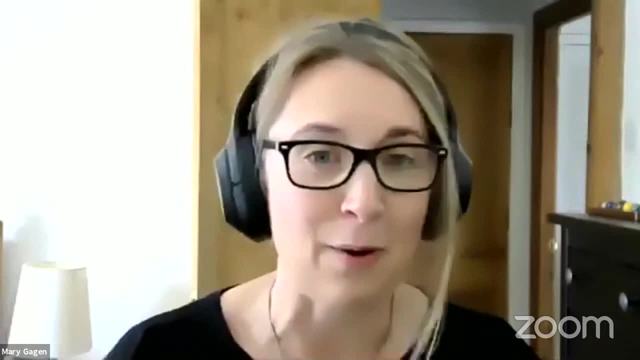 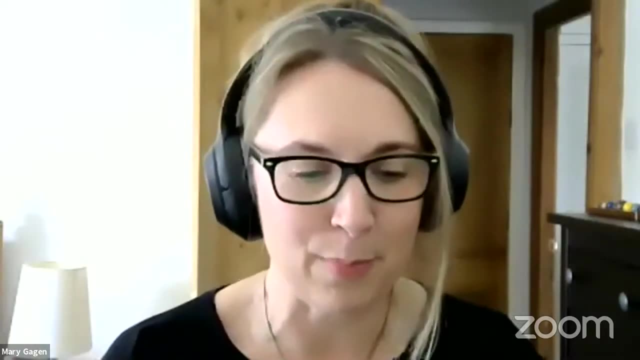 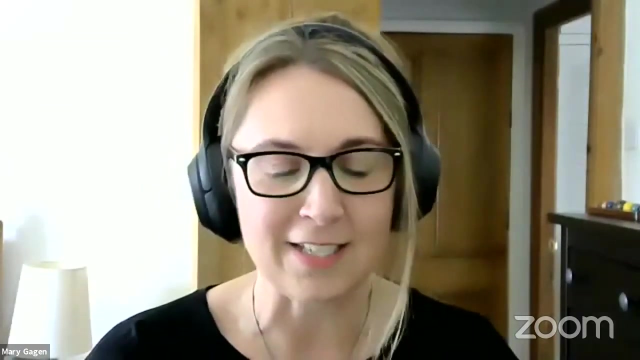 Committee would strongly encourage you all to attend those posters and chat with the presenters, and they'll run as breakout rooms for each of the poster sessions. You'll be able to move between to look at the different posters. Another reminder, as was given yesterday as well, just before we get started. 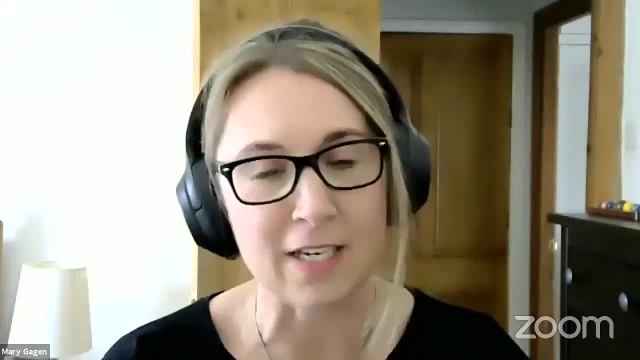 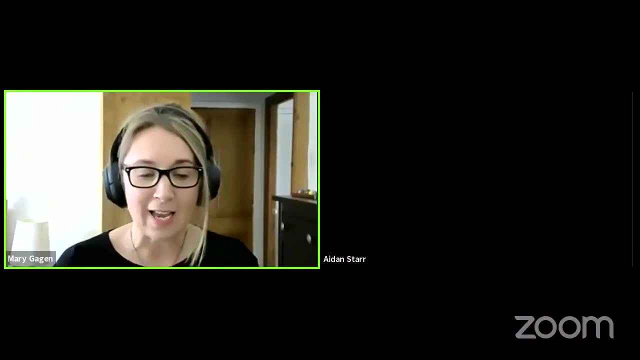 To encourage us all to remember that, participants and speakers, we're all required to abide by the Society's Meeting and Events Code of Conduct at all times, And it is important that we all understand. any of us who are violating that Code of Conduct will be removed from. 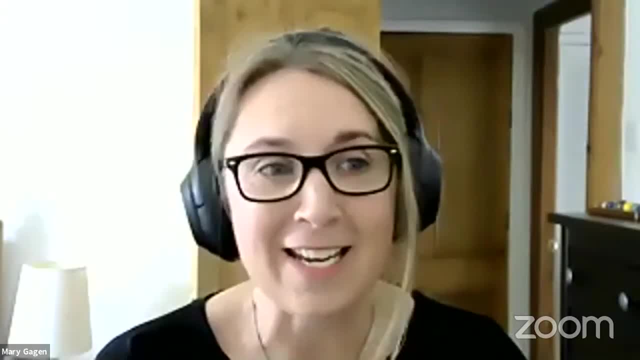 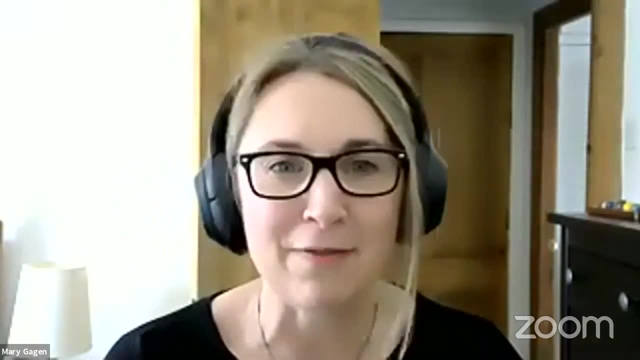 the Zoom event. And yeah, just to say to all of us, it's good for us all to keep in mind not just what questions we ask, but how we ask those questions. I think we had a really fantastic discussion yesterday. There were loads of really great questions. I think we 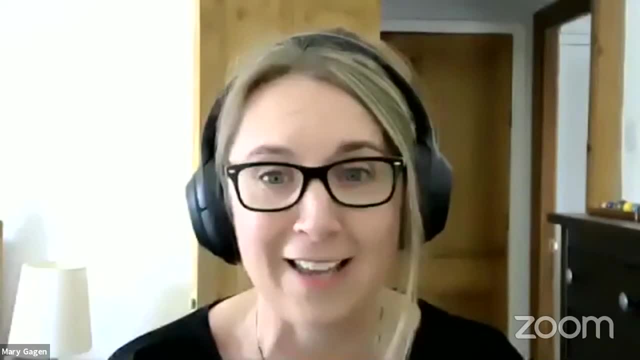 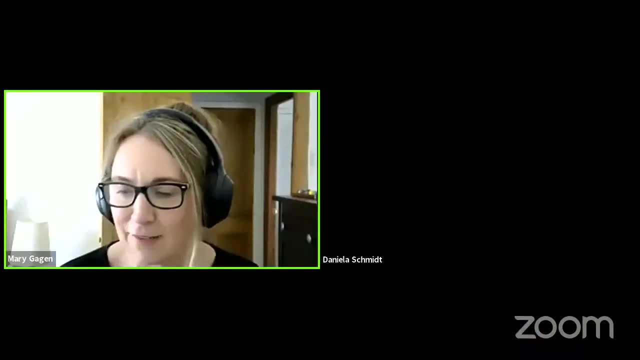 had a really fantastic discussion yesterday. There were loads of really great questions. I think we had a really fantastic discussion yesterday. There were loads of really great questions And looking forward to that again this afternoon. So, without further ado, I'm going to move on to introduce our very first speaker of. 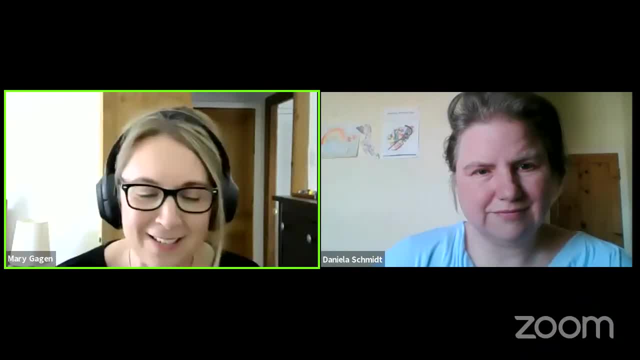 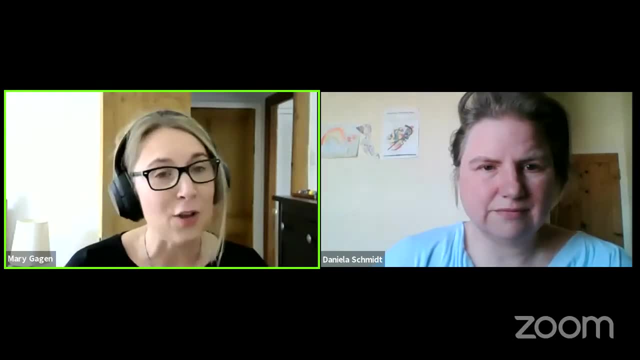 the afternoon. who is Daniella Schmidt. So Daniella Schmidt is a professor in paleobiology in the School of Earth Sciences at the University of Bristol, And she's also a member of Bristol's Cabot Institute. Daniella received a Wolfson Merit Award from the Royal Society in 2015.. 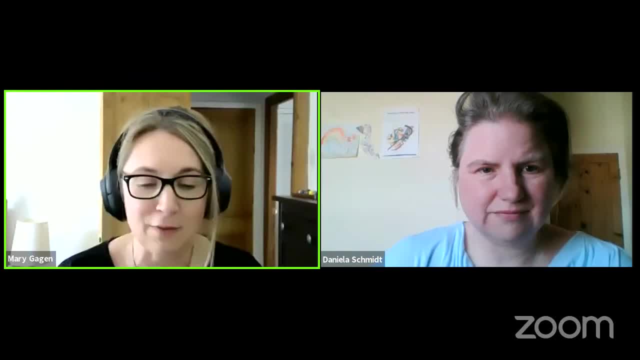 She's a Fellow of the Royal Society And she's also a member of the Young Academy of Europe and is also an IPCC Coordinating Lead Author, And several of the IPCC authors we've got on this session this afternoon deserve a medal for IPCCing through a pandemic. So we've got lots of interesting opportunities. 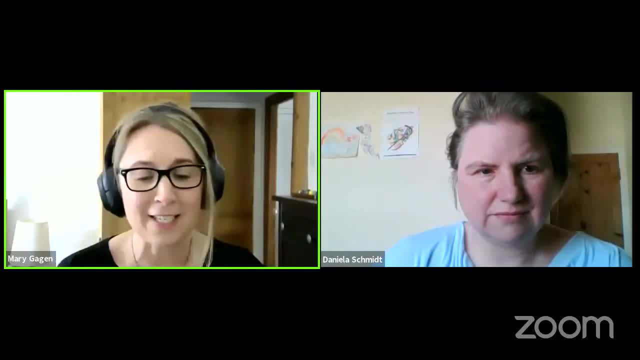 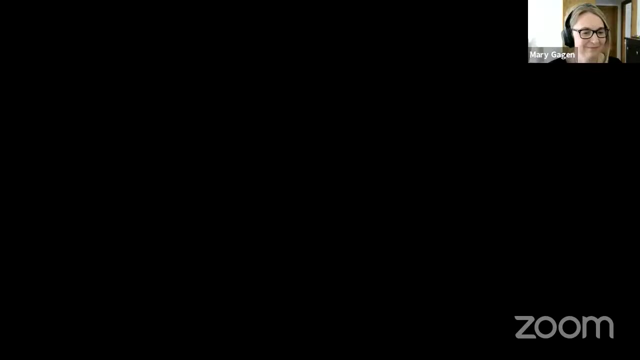 to chat with some lead authors here. Daniella defines her research, focuses on understanding the causes and effects of climate change on marine systems And she's going to be exploring for us today, Question 5.. Thank you very much for the introduction. Just to clarify, I'm a Fellow of the Royal. 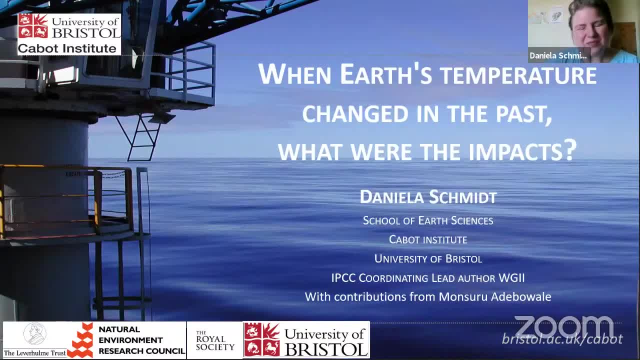 Society for Biology, not the Royal Society. So I was given the target to talk about the impacts the change in Earth's temperature had in the past. Question 5. And as we had such lovely examples yesterday, I will focus predominantly on the ecological impacts. 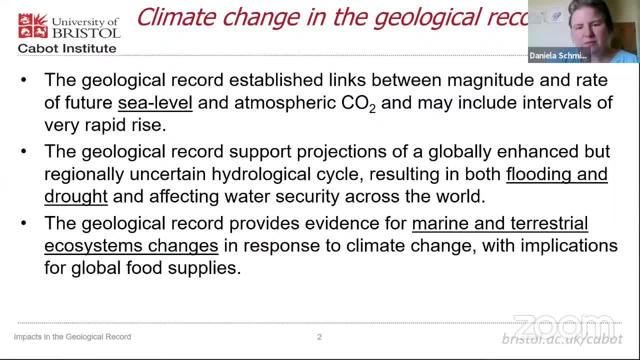 The statement said very clearly that there were links between the magnitude and rates of future sea level change in Atmospheric 2 and the geological record supports those, And we heard Mo Raymond's presentation about that yesterday, so I don't want to go into more detail here. 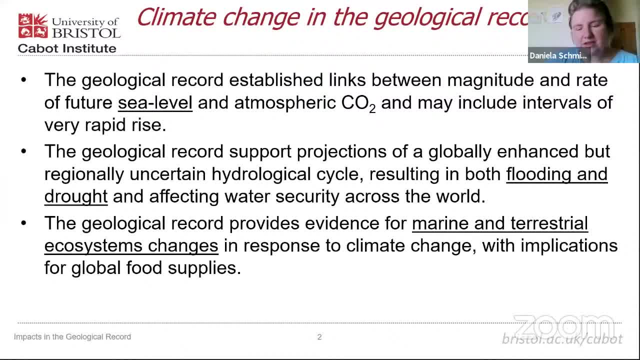 We also heard the statement, also talked about the geological record supporting evidence of changes in the hydrological cycle, and I briefly go into one of the examples, because it's also one I draw on with regards to the ecological changes. and then, lastly, that marine and terrestrial ecosystem changed in response to climate change, with implications for global food supplies. 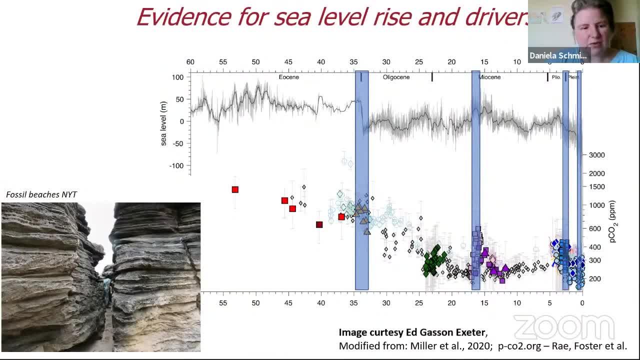 So, as I said, Mo did a lovely introduction yesterday with regards to the links between CO2 and the links between CO2 and sea level rise, so I don't want to go into much more detail there. We have beautiful sections, such as the ones she studied, which have beaches and corals and gives us indication thereof. 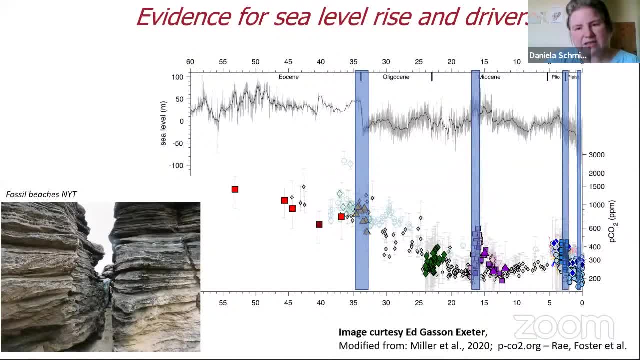 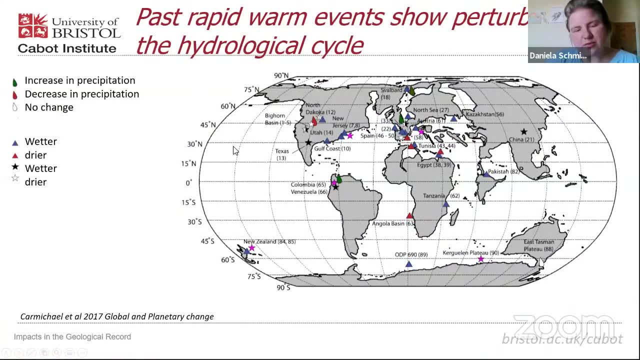 While here we have tangible relationships and we can put our hands on those changes, it is much harder if we're having a look at changes in hydrology. A range of changes have been suggested, and these go from changes in climate, neurology, changes in organic biomarkers, and all of these result into this beautiful colour pattern you can see on the graph here. 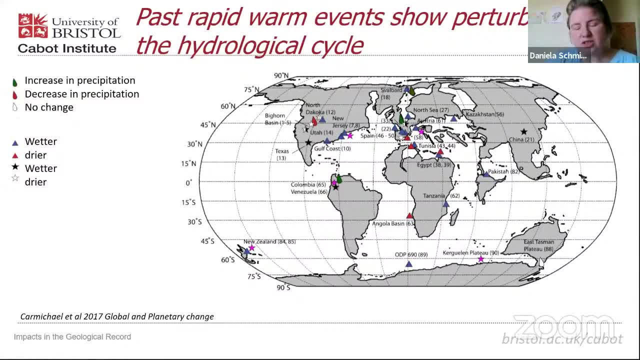 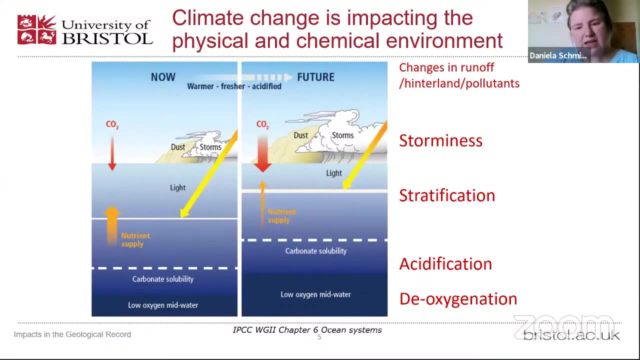 of regional differences in drying and wetting, which is very much akin to what we are starting to see in today's climate records, And also regions where we have no change at all. What happens in the ocean is more complex, because it has both the impacts of warming. 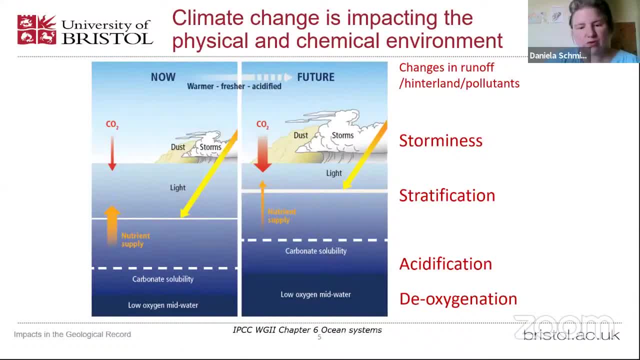 so the resulting changes in stratification, the overall warming of the ocean. but it also has changes with regards to the carbonate chemistry of the ocean. So the uptake of CO2 by the ocean results in an acidification of both the surface and the deep ocean. 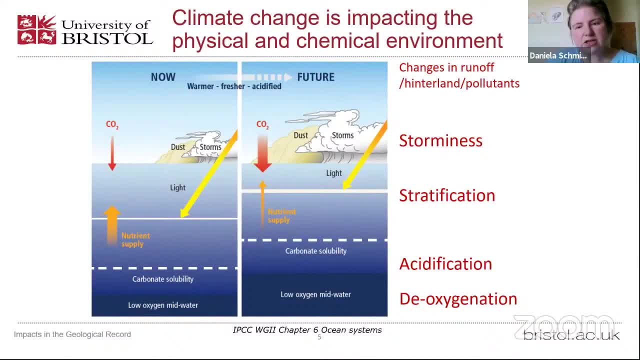 And then, on top of that, of course, the ocean itself. the ocean can't be seen in isolation and it will respond to changes in runoff in the inland, those changes in the hydrological cycle I've mentioned before, which brings a wide range of nutrients, for example, 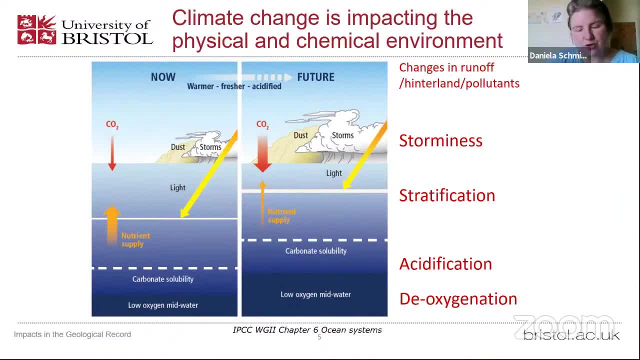 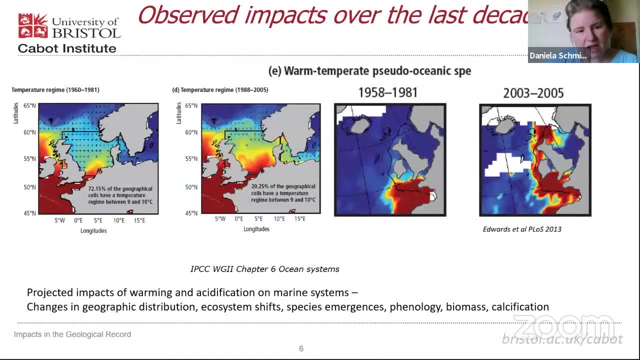 into the system, which change both the coasts as well as the open ocean. The increasing stratification limits nutrient reflux, one of the natural systems, and, at the same time, a warmer world is projected to be potentially more stormy. I think it's really important to see that climate change 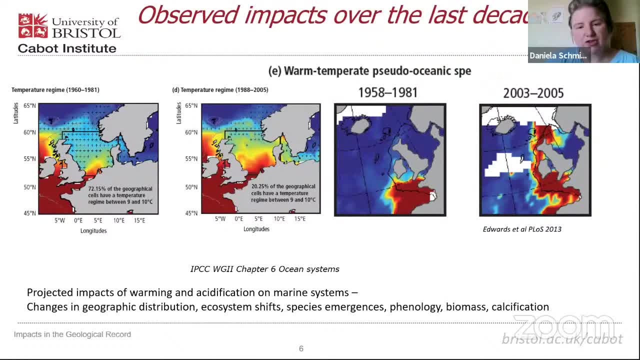 is not something which is happening in the future. We already see relationships between the warming of the surface ocean and the distribution of species today. So what you can see here on the left-hand side is a change in temperature around the British Isles and predominantly focusing here on the North Sea. 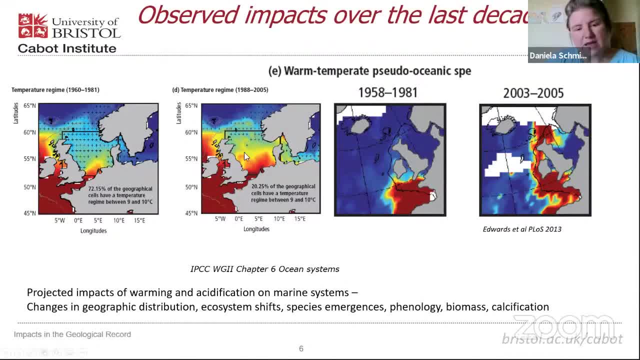 which shows you the intrusion of warm waters into the North Sea. If you then assess the changes in distribution- in this case it's a warm, temperate copper pod, so small crustacean, really important stepping stone in our food webs- You can see that a species which was predominantly 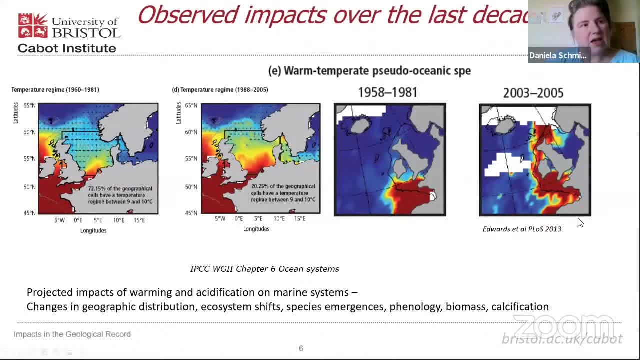 in the 60s and 70s, found in the Bay of Biscay, is now changing its entire distribution up into, along with the Gulf Stream, to Norway, And so we already have changes in the distribution of those. There's a wide range of other things projected. 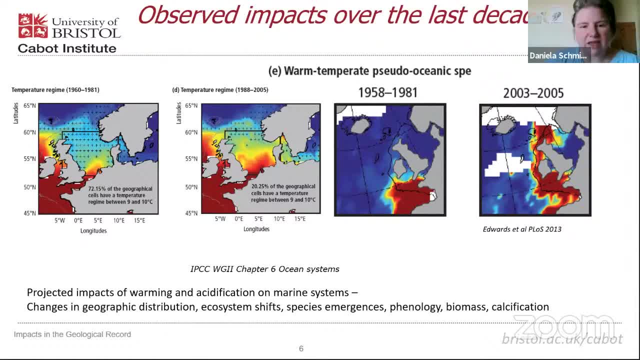 And the question is: do we find any evidence in the geological record that these are real? So do we see changes in ecosystem shifts, changes in species emergence, in phenology, in biomass and calcification. So there's a wide range of changes projected. 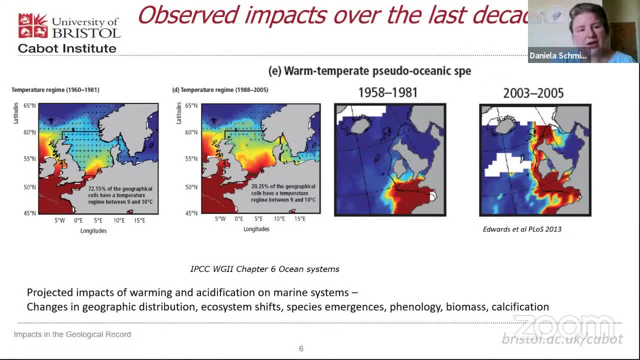 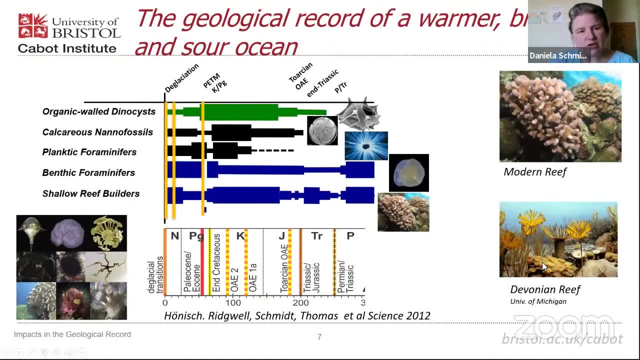 based on physiological understanding and based on modeling projections. So I'd like to take you to the geological record and I'd like to do that specifically in a few selected time intervals, because one of the main things we need to understand is that just a warmer world. 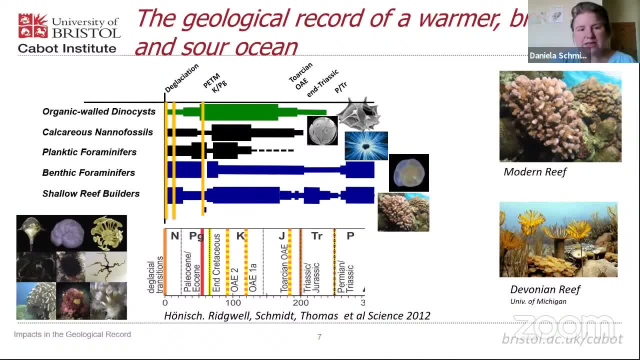 is not threatening to ecosystems. The warmth in itself is something which species over millions of years will adapt to, And therefore we can see lovely, diverse systems in the Cretaceous, which was so significantly warmer than today. We also need to see that we can't go too far back in time. 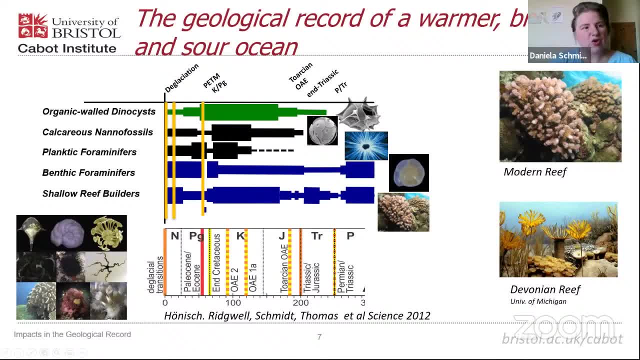 because we want to understand, you know, we want to understand our current ecosystems. And so, while here on the right-hand side, you can see an image of a modern reef and you can see a reconstruction of what we think a Devonian reef looks like, 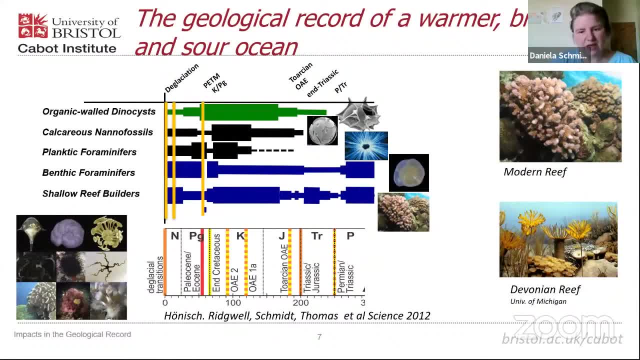 they're both reef structures, but they're clearly fundamentally different, And so I'd like to take you back to first the last eglatiation, so with the melting of the ice. Secondly, to the Pliocene, which is a time interval. 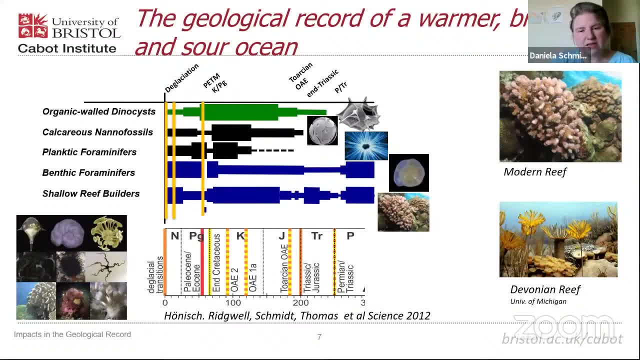 which had CO2s akin to what we are currently experiencing, and I think Ellen Haywood will go into more detail on that later. And then I'd like to take you back to the Pliocene-Eocene boundary 55 million years ago. 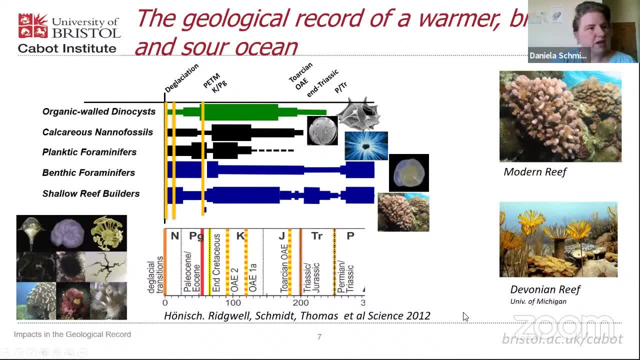 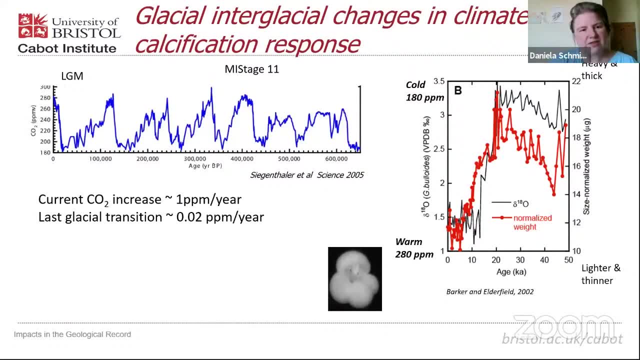 and what we can learn from that time interval. So one of the main points I'd like to reiterate here is what people have said yesterday as well- is the uniqueness of the current changes in CO2.. So what you can see here with age going in this case, 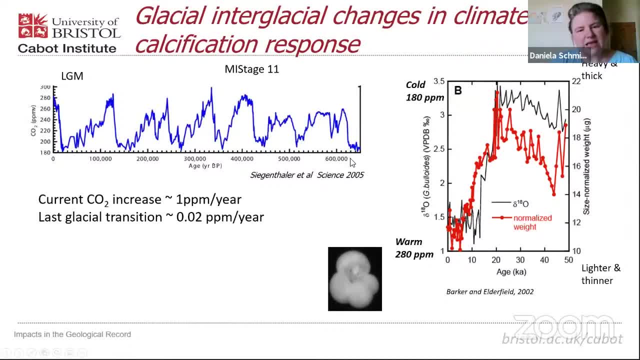 young here, older to the right. what you can see here is the glacial, interglacial and CO2 records reconstructed from the Greenland ice course. You can see higher levels in the Holocene. you can see lower values during the glacial periods. 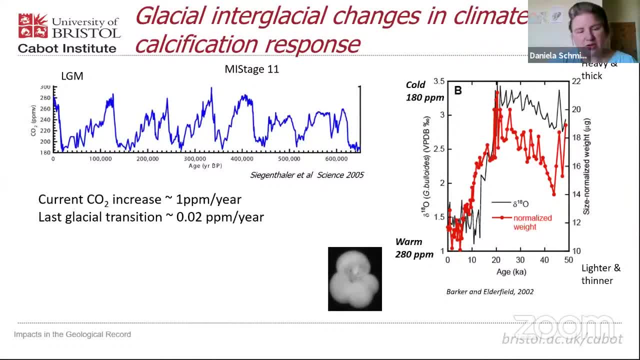 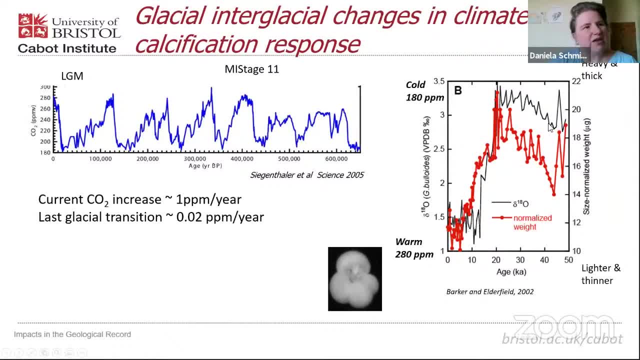 So significantly different ranges. You can see red powder in the blue CGV, the red powder shit. That's the way the blue mountain Mix system works. You can see the colors slightly off in the blue. We can only see tomorrow So significantly this product is. we just use black powder shit, so it's gonna JOHN. 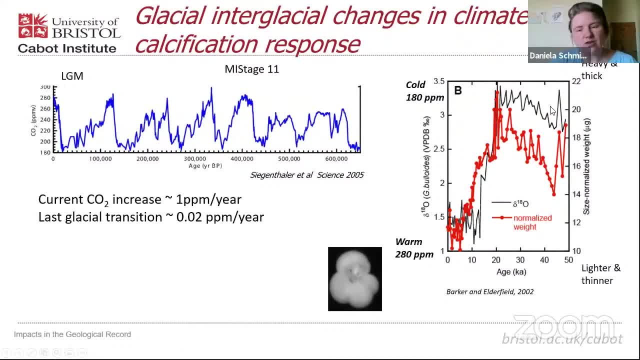 So significantly this product is. we just use black powder shit, so it's gonna JOHN some of theände the best way around. I notice that the blue сол Lö Rabbi, The based sticker: O, apex and Oexrir. That's the way the blue Female. 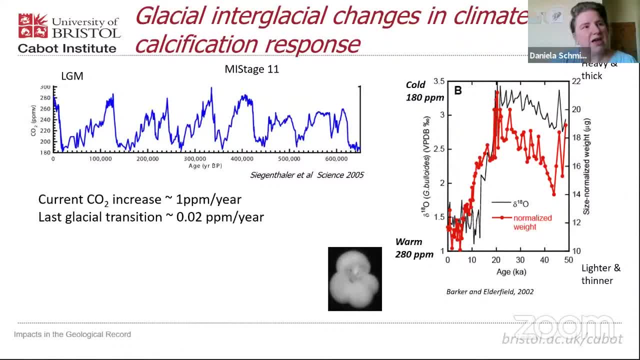 for the warming of the ice volume. so it's a combination of both, And the red gives you the weight of this species, Glorigina benoides, which is an important planktic for omnivore species. While this just looks like four pimple balls next to each other, they are ubiquitous. 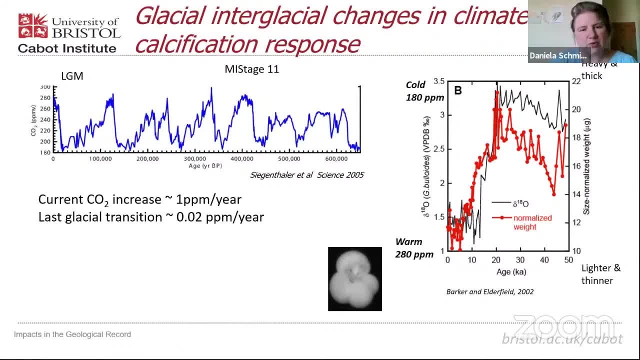 in the surface ocean and they're really important with regards to producing carbonates in the open ocean system. And what you can see here is that at times where the CO2 was lower, we had heavy, thick specimens which were weighing around 20 microns, And today, or in the pre-industrial 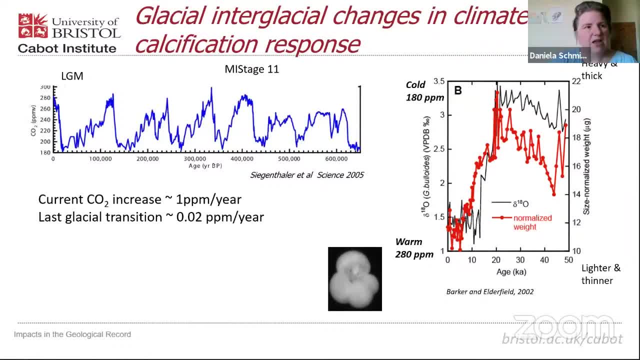 times we have lighter and thinner specimens. What it also shows you- and that's really important- is that the rate of change overall is quite similar. So what we see here is that if we have gradual changes in CO2, the calcification of this organism is changing, but it is changing. 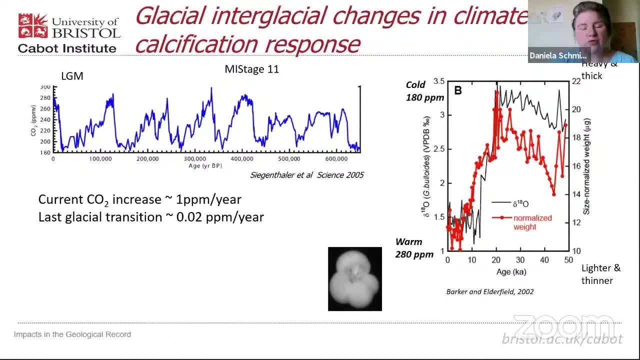 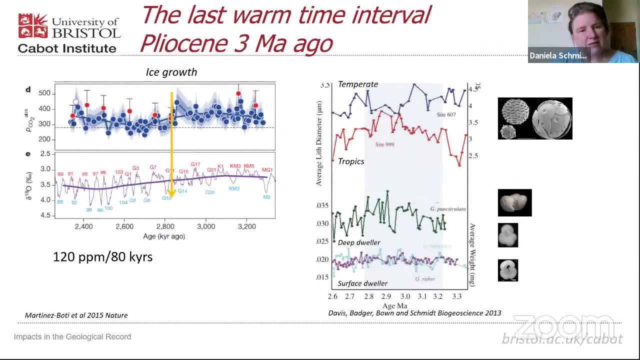 within its natural bounds. So there's no risk of concerns of losing this species. Another species will take over in other locations. So let's take me a step further back Again. let's have a look at calcification, because there's so many of the parameters we could. 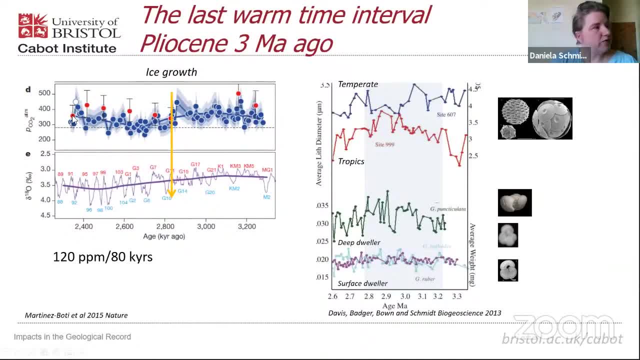 have a look at. What you can see here is a record of the pliocene CO2 at the top. This is a measuring in by the delta O18, which in this case indicates a growth of the ice volume, And what you can see here is overall values around 400 ppm, And then after this: 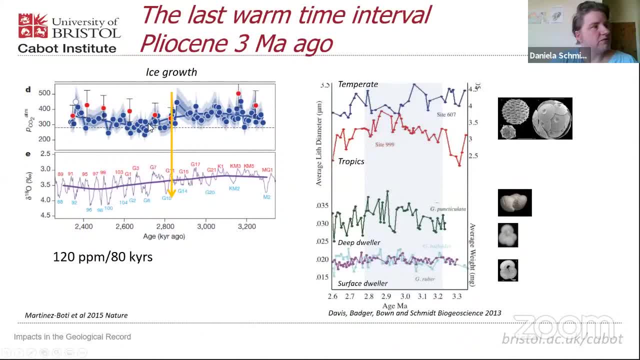 time interval. here you can see a drop towards around 300 ppm. What you can see also is that you have very low amplitudes here in the delta O18, so very small changes in the ice volume And moving over to a significantly higher amplitude. And then you can see that, as I 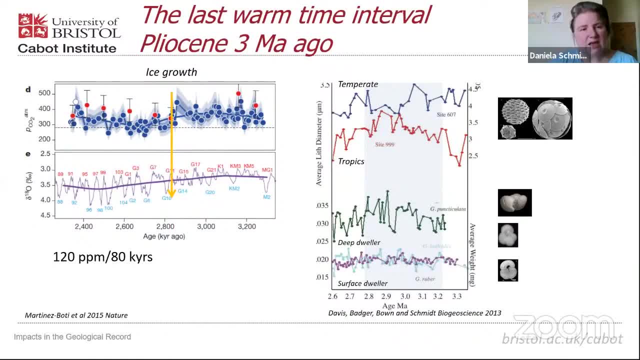 larger variations And we were interested in seeing if we have evidence for changes in the calcification as projected for the future, across this change in CO2.. The assumption would: be higher CO2 would produce less carbonate, lower CO2 would produce the specimen would the species would. 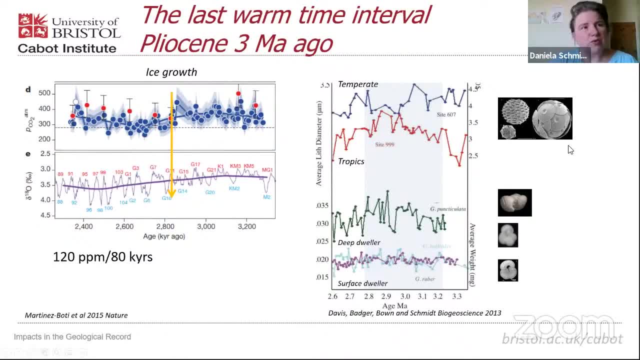 produce more carbonate. We've looked at two different groups, and these are haptified algae, these are coccolithophores. So if you go to the White Cliffs of Dover, you can see that they are rock forming organisms. so every time you use chalk you have millions of those. And again in 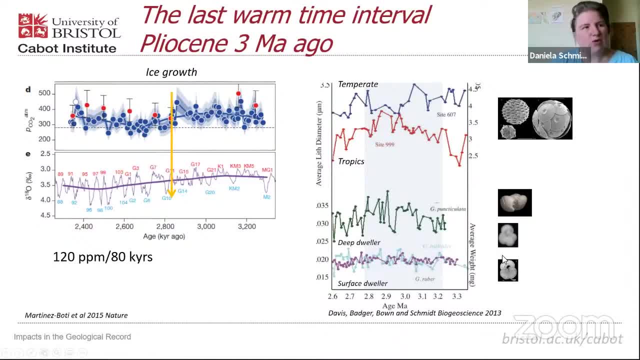 this case, three different species of plankton pylori. We looked at two different locations because we wanted to see if the tropics, where temperature might become high so that the species might be threatened by it, versus a mid-latitude, which is much more a dynamic environment. 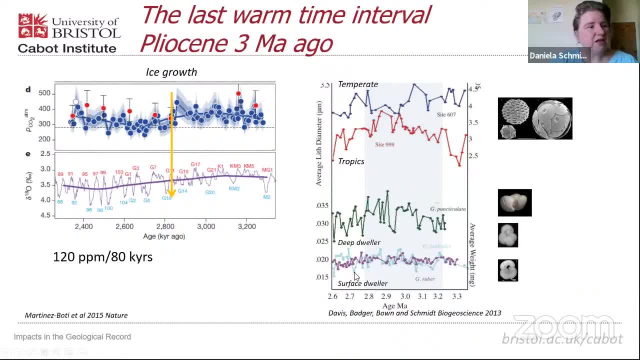 And what we can see is that there's different variability between, you know, tropical side and the cold water side, that there's different absolute values between a temperate species and a tropical species. There is no change over time. So again this relatively 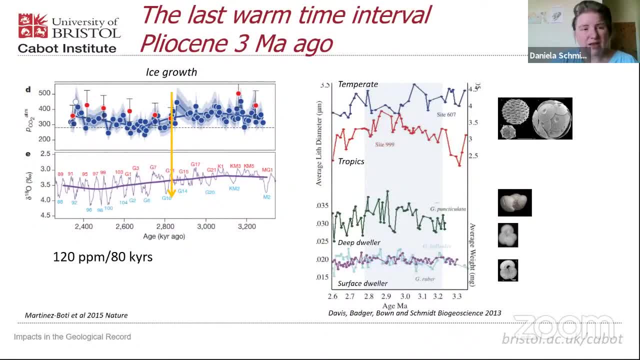 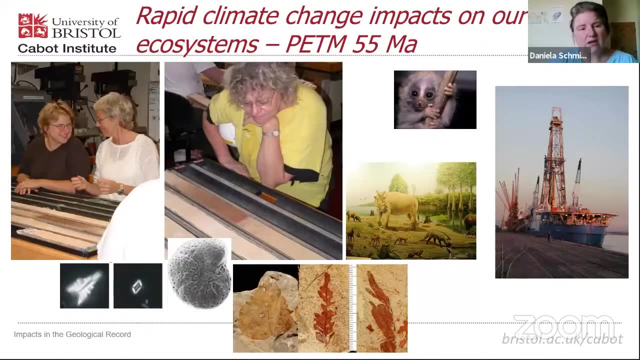 low change in CO2, a roughly 120 ppm over again roughly 80 000 years, did not impact the calcification of the species negatively. So what then causes the concerns we have with regards to the changes in warming in the fossil record? 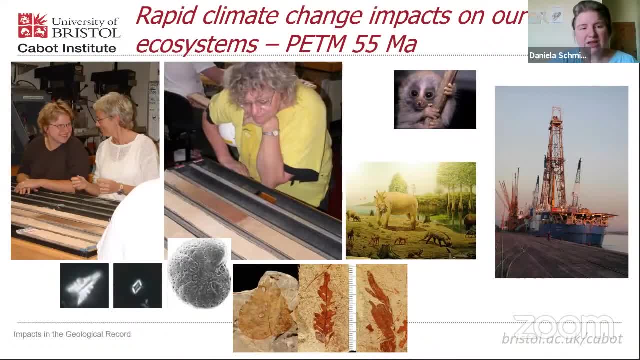 So I need to take you significantly further back in time, which gives you an indication of quite how unique the current experiment is, And I'm taking you to the Paleocene-Eocene Thermomaximum, or the PETM. It's the difference to the two intervals I described before. 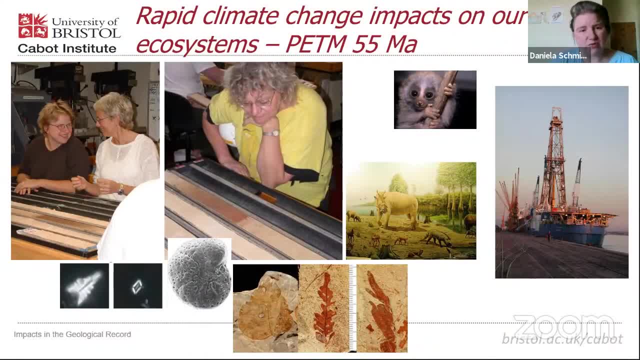 is the rapidity with which the changes happened and the amplitudes with which these happened. You can see, associated with this event, changes on land, so we can see changes in vegetation. you can see changes on amongst the animals. it's just by chance. it's the base of the mammals. 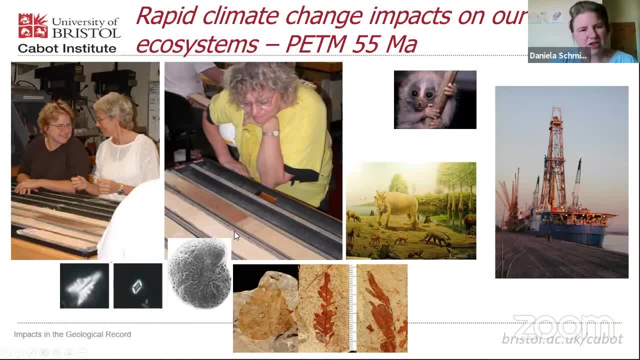 But you can see very clearly in the geological record that something changed rather dramatically. What you can see in those pictures on the left-hand side are two photographs of a core which records this interval. You can see in white the time before the event and then you see a very sharp boundary turn into what's red. 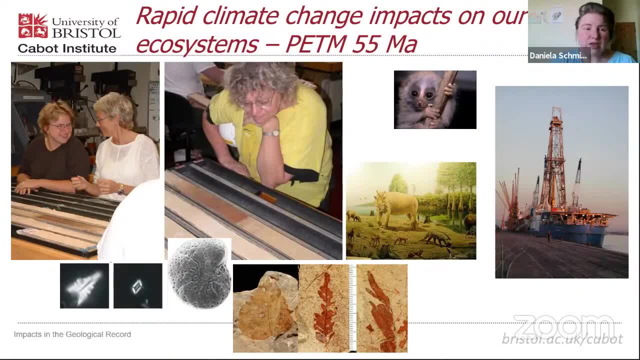 which indicates this change. If we are losing the colour changes because of a change in the carbonate in the sediment. And there are two ways how we can use the carbonate in the sediment. We can reduce the carbonate formed at a specific space or we can dissolve it after it has been. 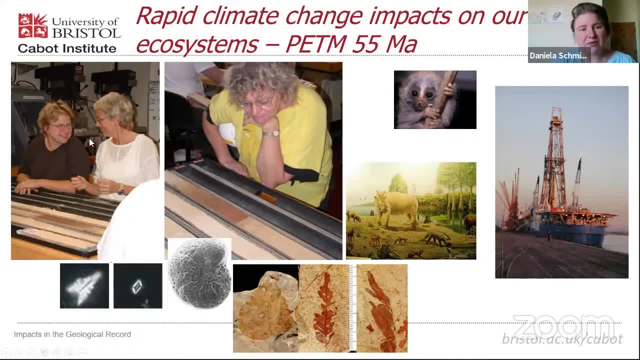 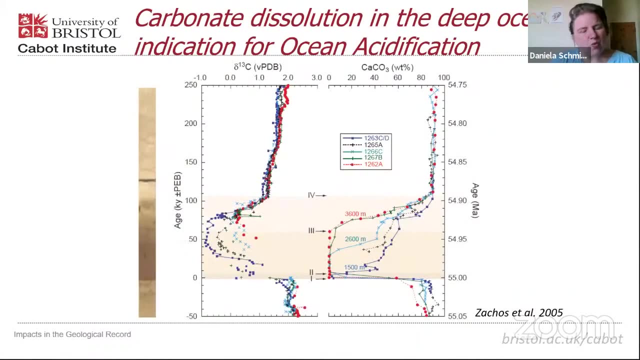 deposited And you can see the excitement in a much younger me here which is very much a result of finding such a glorious record Again. that was my colleagues on board of the JOIDES Resolution, which is one of the workhorses for marine climate research. 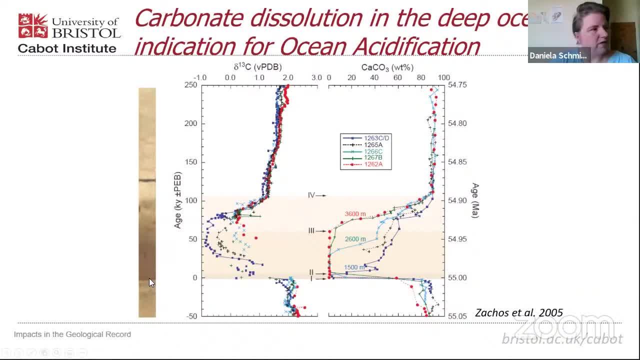 What can we see in the record? What you can see here again is now a core picture. So again, you have the whiter, you have the browner. you can see it's less brown towards the top. the dark line here is a core break. Our cores are 1.50m long. 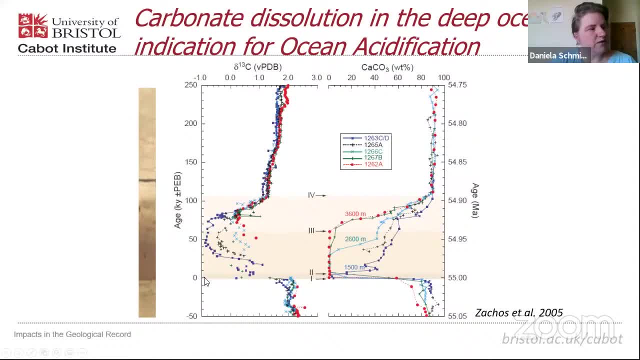 can see here is change as time relative to the onset of the event, and you can see two different panels, one of which is carbon isotopes and the other one is calcium carbonate in the sediment. the different colors represent different cores which we have taken a different water depth. 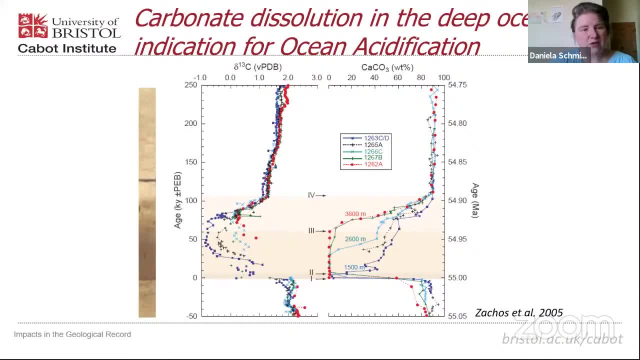 between um, at that point of deposition, one and a half thousand meter water depth and three and a half thousand meter water depth, and i hope what you can see is that um, these record a very strong change in carbon isotopes which we interpret as a large injection of of carbon into the, into the. 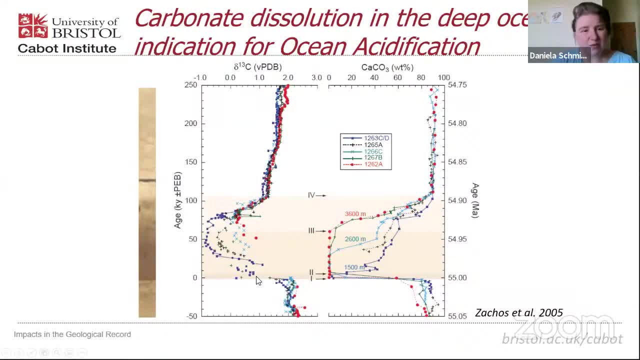 ocean atmosphere system. there's a gap right at the boundary, and that's because the material is completely resolved at this site and but we have others where we can look at the transition in much more detail. what you can then see also is that the perturbation in terms of no carbonate is very 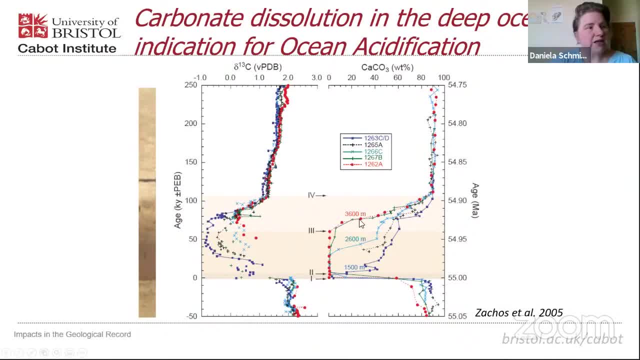 short-lived in the very shallow waters and much longer lived in the deep waters, showing that the carbonate compensation depth- the depth at which carbonate is preserved. shoals became shallower due with the injection of the carbon and then um recovered into into um, first in the shallow sides and then later in the deeper sides. 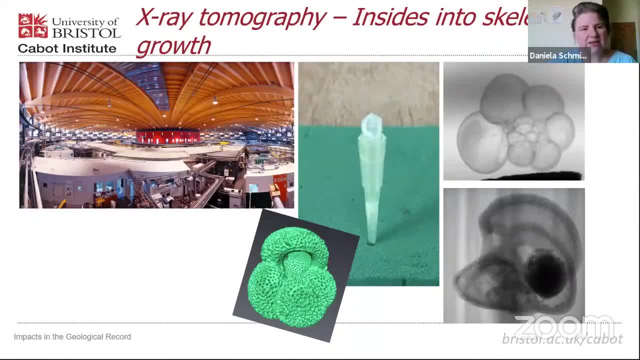 so how do i look in such old material, where we've had um strong ecological perturbations but also strong preservation biases, into what the classification record is? and what we do is we take our specimen and they're so small- this is a pipette, tip um and you can't see the specimen easily on it. but what we do is we're bringing 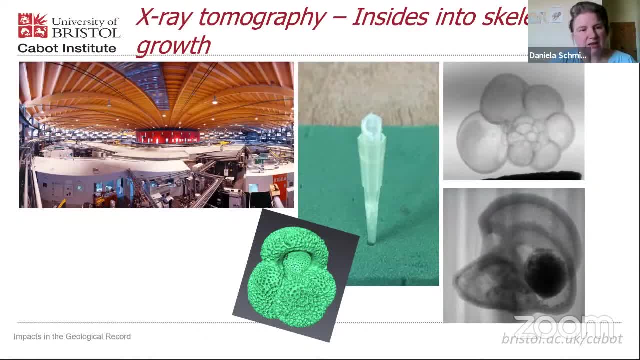 it to either, um a benchtop ct scanner, a computer tomography akin to what you might experience in a memory scan, and our smallest specimen here, to the synchrotron, um to the particle accelerator. and what it does is it generates those lovely images for us which allow us to reconstruct. 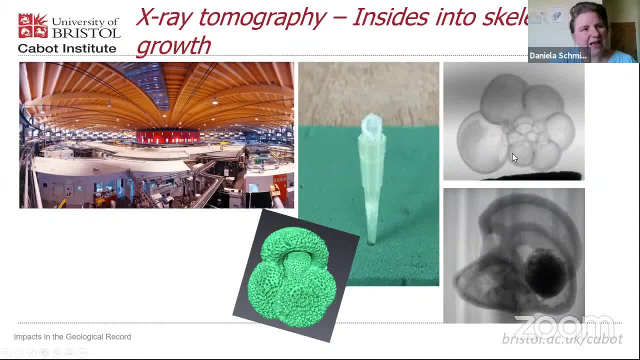 the development of those species. so they start by growing the first chamber and then adding those as well as its wall thickness, and making those reconstructions you can see here in green. we can then go back and um, look at the developmental history, but that's not what. 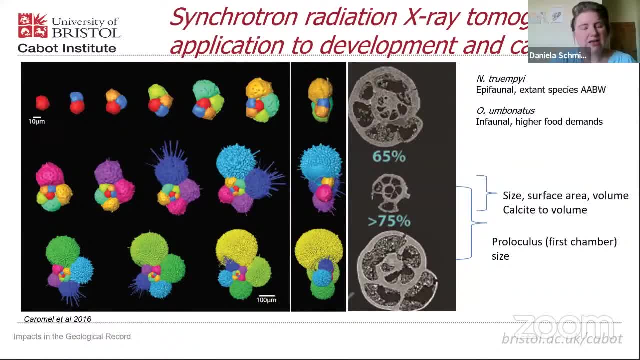 i'm trying to focus on here, but it would allow us to have a look at, um, you know, changes to that. what i will be presenting here is data which we gather if we take cross sections through the specimen and we calculate its volume and we calculate the amount of calcite. the beauty of that. 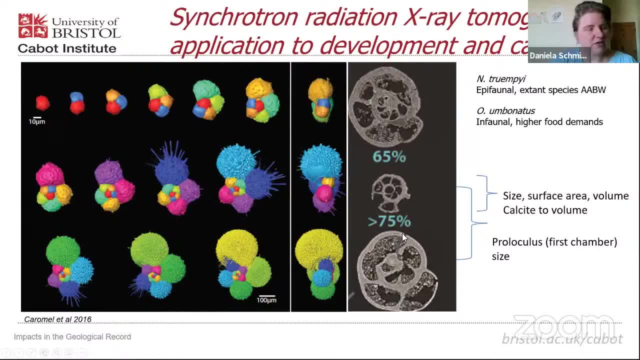 that we can work with material which has some indications of dissolution but also some infilling, because um, painfully, monsoro adobo, whose phd i'm presenting here, um is cleaning up those images to to make those reconstructions, and we then calculate its overall size, the surface area, the volume and the ratio of calcite to volume. 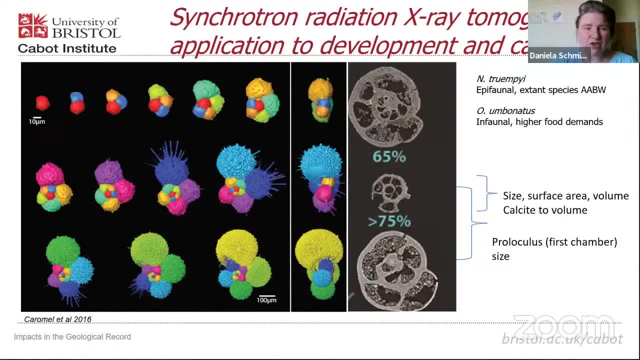 to have a look at. you know, is the surface area increasing, which is the area over which the species can forage? um, is the volume decreasing because it doesn't get enough food to sustain itself, or maybe not enough carbonate to calcify? we're looking at the calcification to volume, the 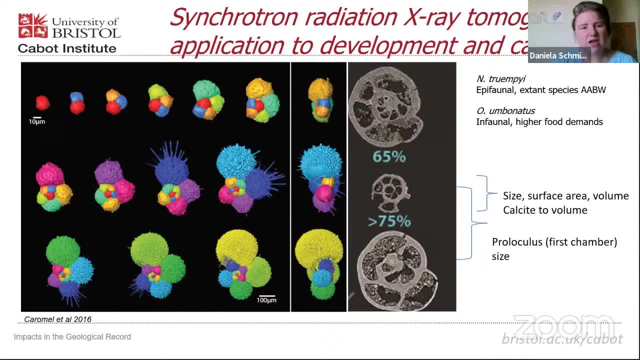 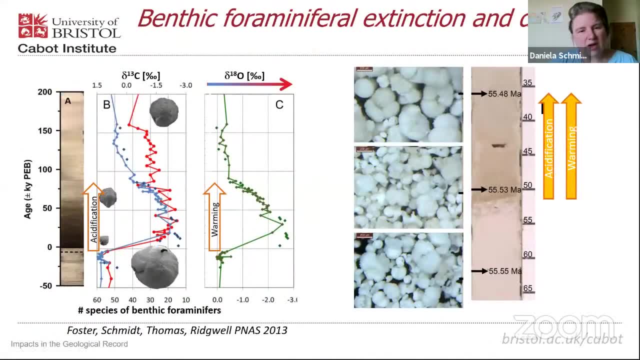 calcite to volume, to then understand if there has been a negative impact of this event on the ability of the species to calcify. what is quite important about this event is that it's a really important extinction event amongst this group, the benthic foraminifera. 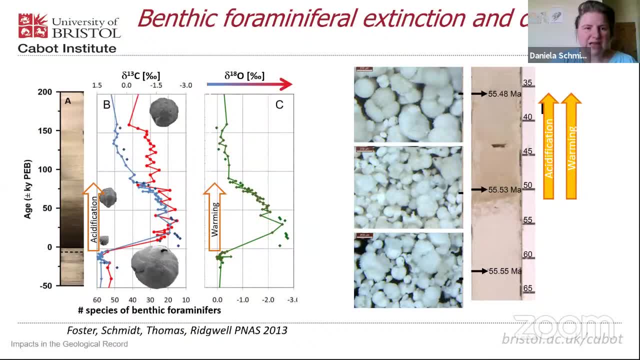 this is a very, very sturdy group. through the cretaceous paleogene boundary, when the dinosaurs went extinct, there's hardly any perturbation in their diversities, of the number of species, but here at this event, we're losing around 40 percent of the species. the other thing you can see again. you have the core image here at the left hand side. 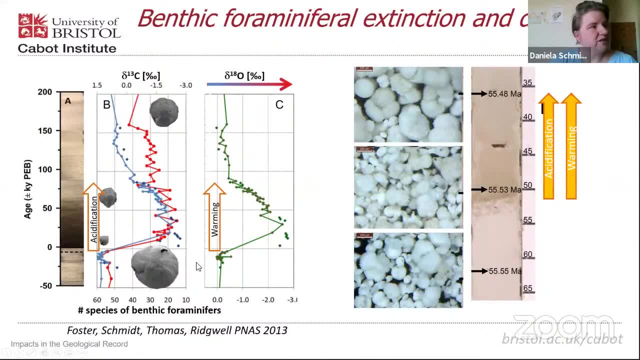 um, you have carbon isotopes indicating where the event is. you have oxygen isotopes which give you a first indication of temperature, um, and you have a few images here of those specimens from a side, from the same side. i showed you earlier, walkers, which these are all at the same scale. so the most dramatic change you can see here is that we're 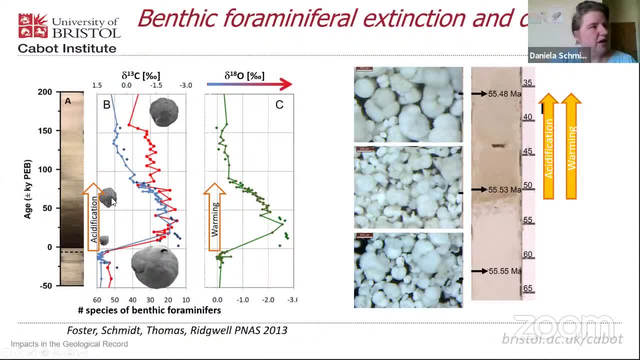 going from a really, really large specimen to something which is so tiny and still small when we're going to the recovery um of the event. a similar pattern of dwarfism is also something which we can see in planktic form, um, but i'm trying to concentrate on one group here, um, because 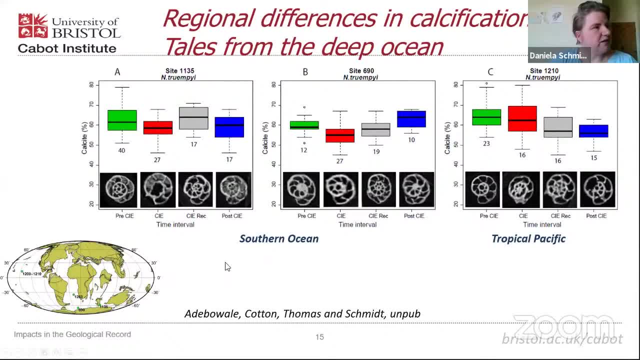 of the time. so we're looking at three sites. so we have one side here, 690, which is off antarctica, which is a relatively deep um in the ocean. um, that's the middle panel. we have another side, side, 1135, which again is off antarctica but very shallow, and food availability for species in the 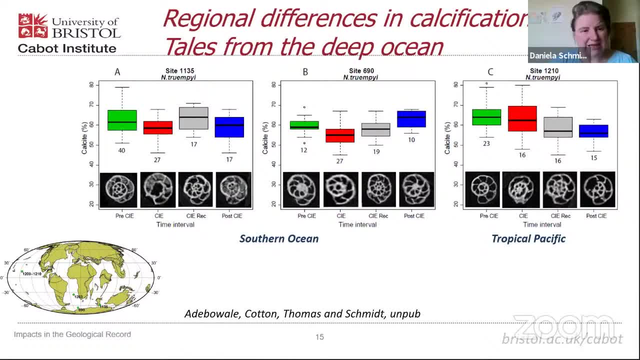 deep ocean changes, with more in the shallow water and less in the deeper part. and then we have a third side, here in the middle of the pacific, a highly stratified part of the ocean where food is. so we've focussed on those very small annoyances with food from the ocean and therefore 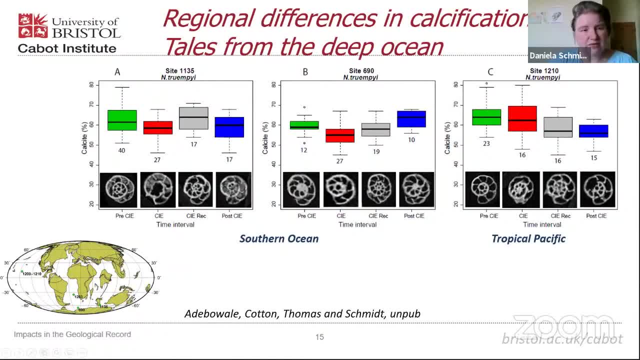 and we'll talk about them in what don't we believe there are currently at the moment called cancer complication. calcification as percent calcite, as I explained earlier, while the difference here with a neighbouring site in the Southern Ocean but deeper has a reduction in calcite production by the species during the event. 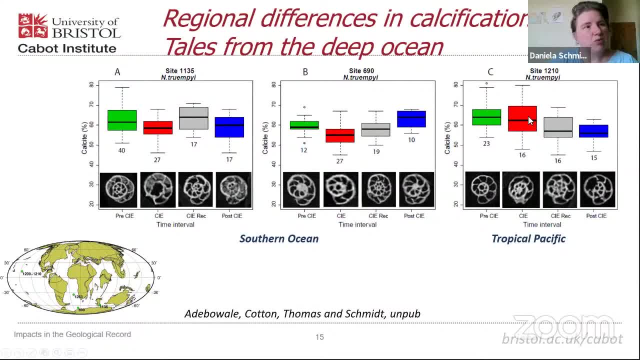 and then a recovery towards the values before. What we can see at the site in the Pacific is that we have really high variability, but overall, again, no significant change, And so this suggests that there are other factors then warming which influence the carbonate production by this species. It also suggests that the water depth is really important, because with 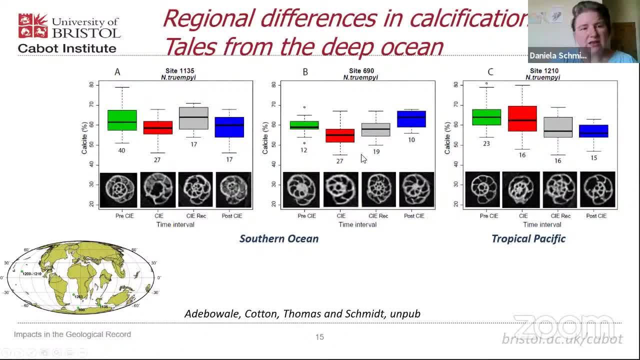 two sites which had a similar latitude, we see that the deeper side has a reduction in calcite production and the shallow one does not. So the next thing we did, then with those specimens is to have a look if we can see changes in its form. So are they becoming smaller? Are they changing its? 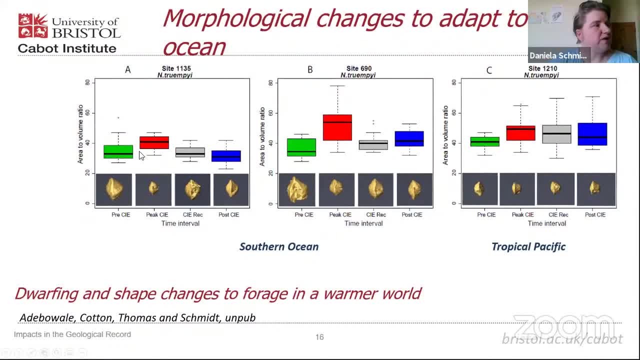 form. So, again, this is something that we can look at. It's the same arrangement, the same course, in the same order, this time showing you the surface area to volume ratios and images, again at the bottom, trying to highlight that These images are all at the same scale. so I 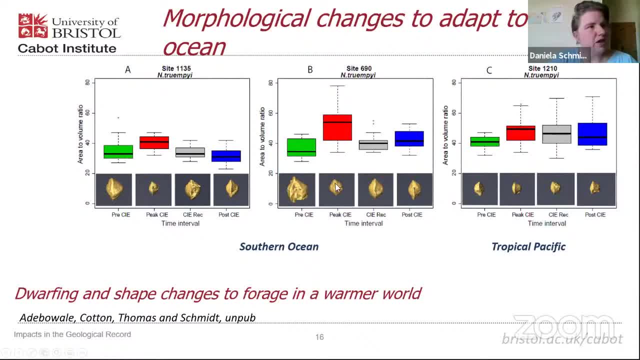 hope that you can see very clearly at both site 1135, so the both Southern Ocean site and site 690, that the specimens which have grown during the peak of the carbon isotope excursion are much smaller where in the tropical Pacific. they were small from the beginning, So they must have already been. 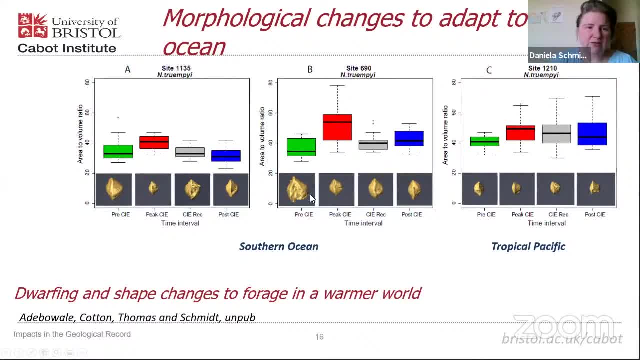 limited in their growth and they've never reached sizes as you would have at this other location. If we then look at those three sites again, we don't have dramatic changes in the surface area to volume, so the ability to forage over the amount of 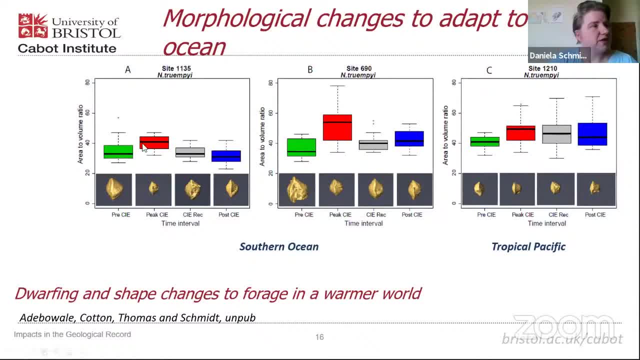 biomass it needs to support at size 1135.. There is some increase but it's not statistically significant. In contrast, at 690 we see a dramatic increase of that. so it changes its shape and if you interpret the importance of surface area in terms of foraging or in terms of oxygen uptake, 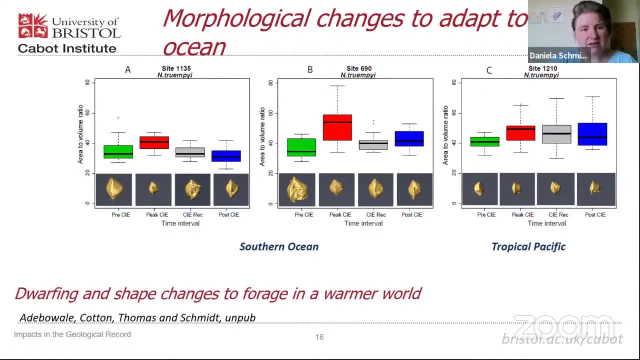 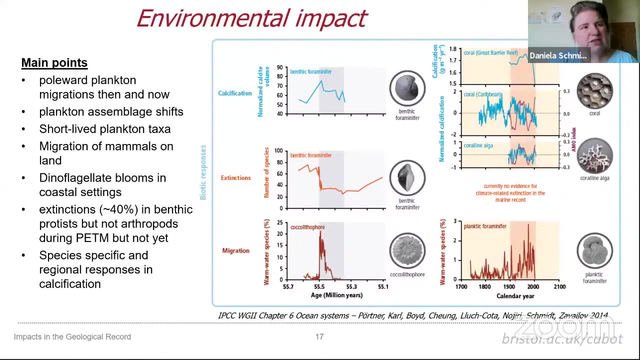 you would. you could interpret this as a need to have more food to sustain calcification and to sustain its metabolism, so its ability to function. So we have see both dwarfism and shape changes in this species. We tried for the last IPCC assessment to summarise some of those events and to compare between the PETM and the current. 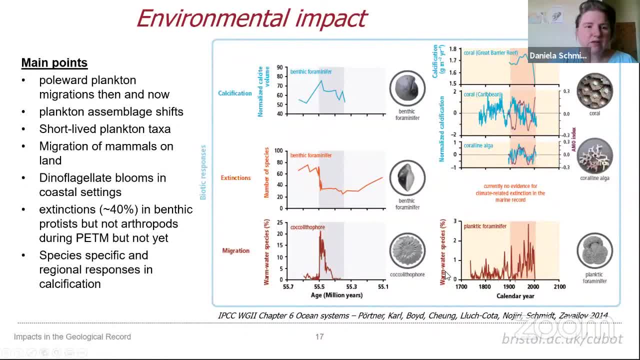 There's some things which give us confidence that we understand those patterns very well. So what you see here, for example, is a warm water species migrating into the Southern Ocean. This is the increase of a warm water species in a cold setting today. 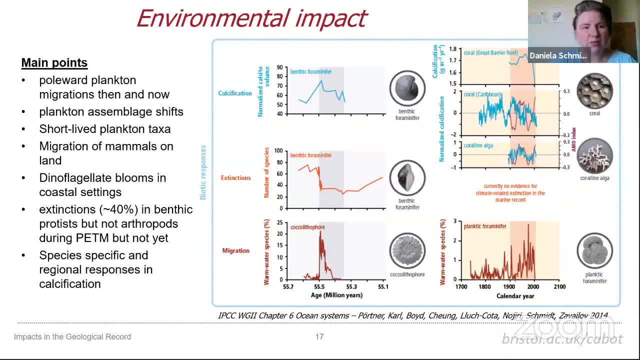 Different taxa, but ultimately what they both do is species in the open ocean follow the temperature optimum, So they just change their biography. They've done it then, they're doing it now, And it relates back to the example I showed you at the beginning. 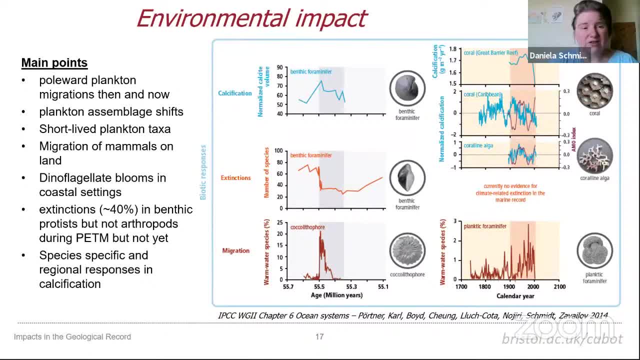 In the geological record we've had extinction and currently there's no evidence yet for extinction in the ocean. There are clearly extinctions on land, but they are predominantly driven by land use changes up to this point and not by climate change And then calcification. I showed you lots of different responses at different locations. 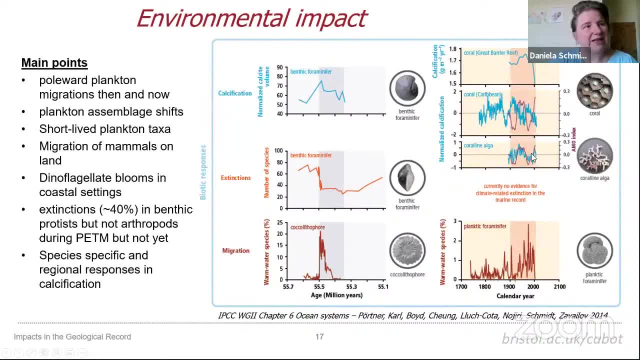 And the same is something you can see today. These are coral and algae at two different locations and they do different things. And these are tropical corals, And again they do different things. So calcification seems to be something which is much more dependent on its species and its own metabolism. 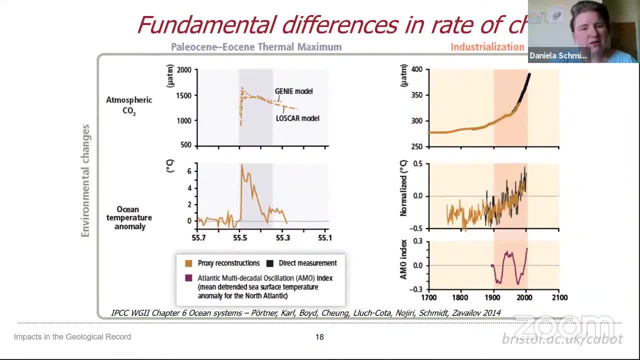 What is most important, though, is what I was trying to get to you early on- is the difference in time. So the CO2 rise we've had since the beginning of the industrialization happened over 120 years, And therefore the changes here in warming and in atmospheric CO2 are incredibly quick compared to an event. 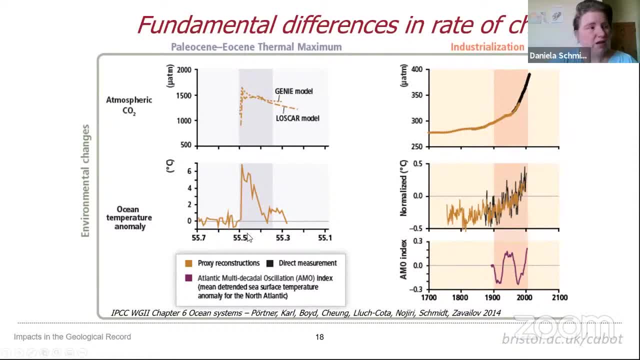 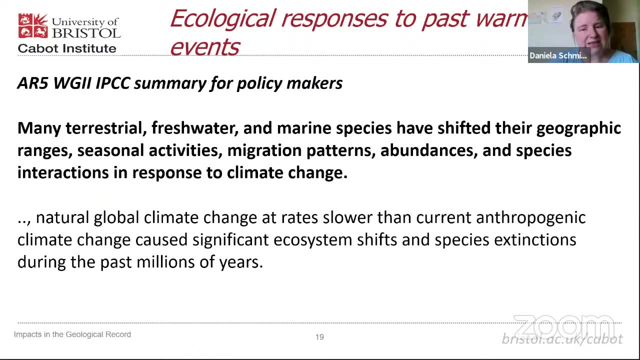 In this case, this time is in millions of years, And so we've had an onset, over several thousands of years, of a similar amount of carbon than what's projected to be emitted because of fossil fuels And land use changes, And so what's absolutely clear is that we can see changes in the geological record of species shifts. 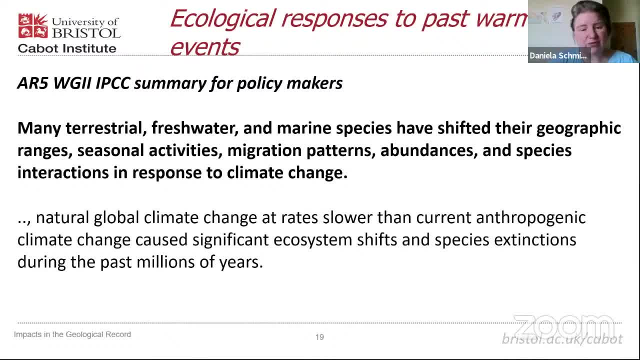 And that this has happened at rates which were significantly lower than what we are currently seeing. We know that rate of change determines an organism's ability to acclimatize or to evolve if needed, And therefore you know there's severe concerns of the impacts this might have on the environment. 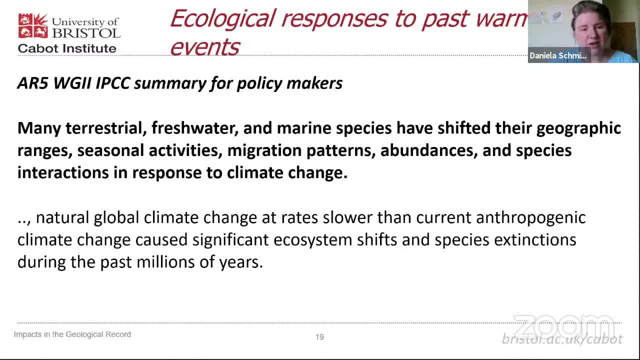 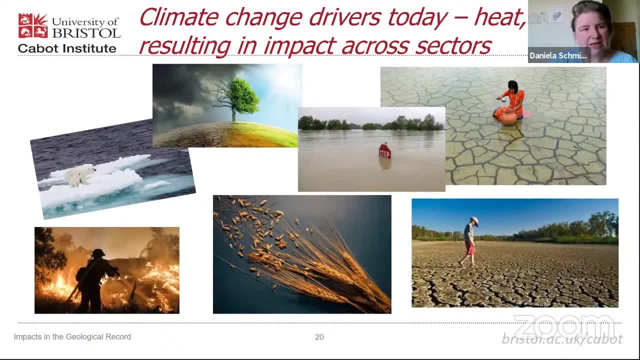 And so we can see changes. We can see concerns of the impacts this will have. with this incredibly rapid change, There's a large number of climate change impacts which are already detected. There are changes in the hydrological cycle, There are changes in fire regimes. 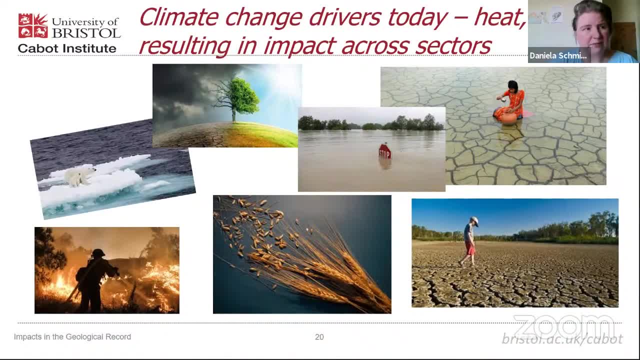 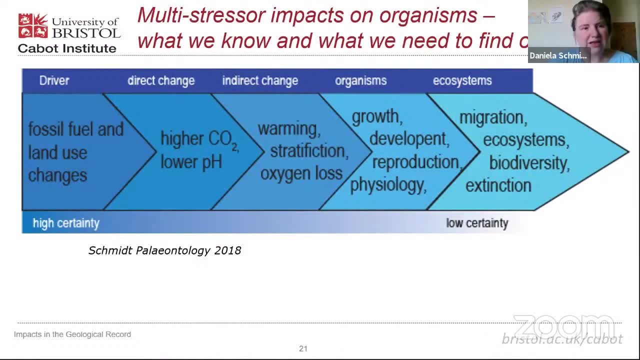 There are changes in where species are growing and how they're migrating. The question is, and what we are supposed to do with regards to future projections, of how do we upscale from the knowledge we have at individual places and on an individual taxa? 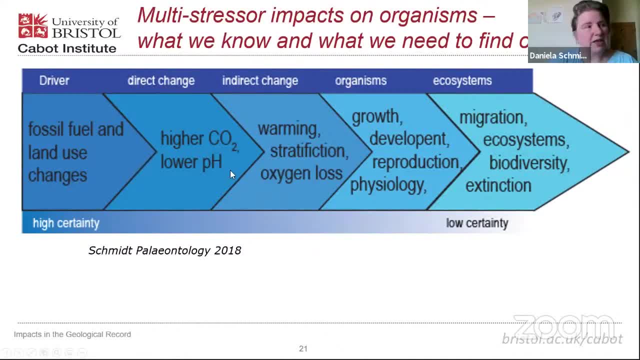 We know that burning fossil fuel increases CO2.. If it increases CO2, we also know it lowers the pH, because that's a simple equilibrium equation. Indirectly it changes. It makes the planet warmer, It changes stratification and oxygen loss. 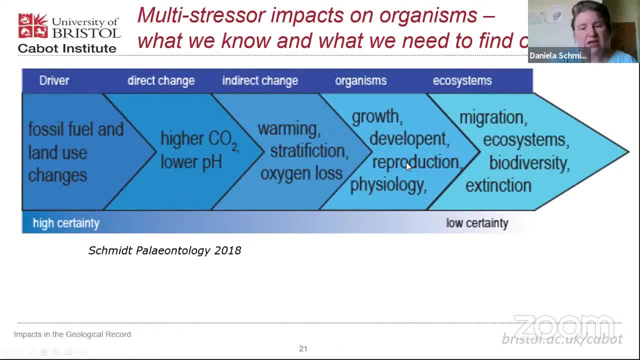 We have experiments which show us changes in growth and development and reproduction of individual species, But ultimately what we're interested in is ecosystem services, Such ability to produce food, ability to regulate CO2, and the loss of species for us, And we have increasing uncertainty when it comes to those projections. 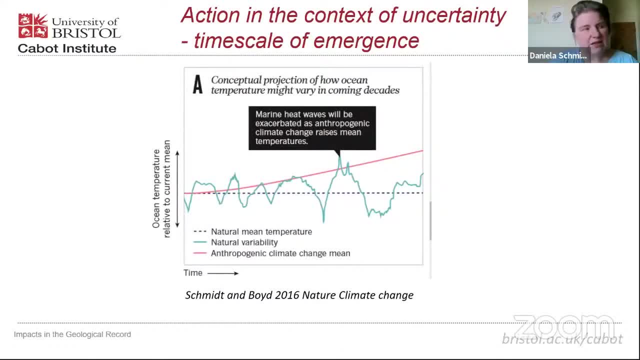 The other thing which is still very unclear is: a lot of people are saying that the impacts aren't visible. yet across many of those systems We have a lot of natural variability- And this is just a hypothetical Decay- variability which we see in many parts of the world. 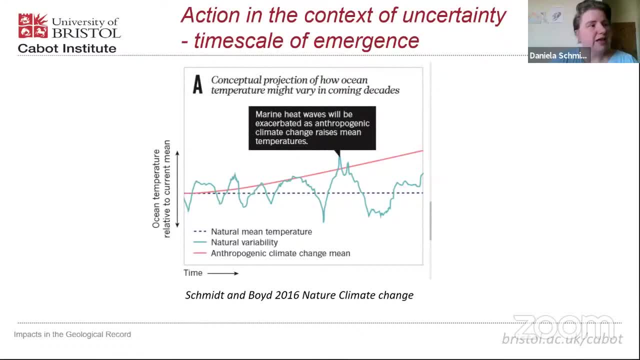 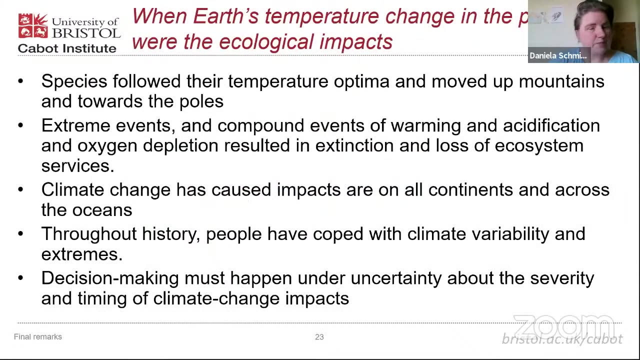 Interconnected, teleconnected with each other. So the question is: can we wait until the anthropogenic climate change has left this envelope Or are we significantly concerned about the projections that action is happening now? Ultimately, we know that species followed and will do so in the future. 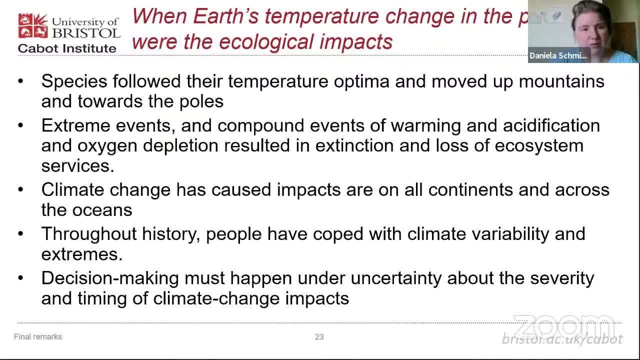 They're temperature optimal And they move towards the pole And they're moving towards the sun And they move up the mountains And mountains end eventually And the poles get warmer, That we have extreme events and compounds of warming and acidification and oxygen depletion. 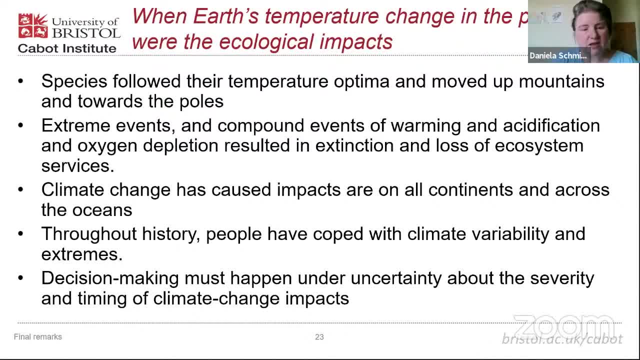 And that in the past, these resulted in extinction and loss of ecosystem services. We know- we have evidence for this across all continents and across all oceans. We know that in history, people have always coped with climate variability and extremes, But it has never been as fast as it is currently. 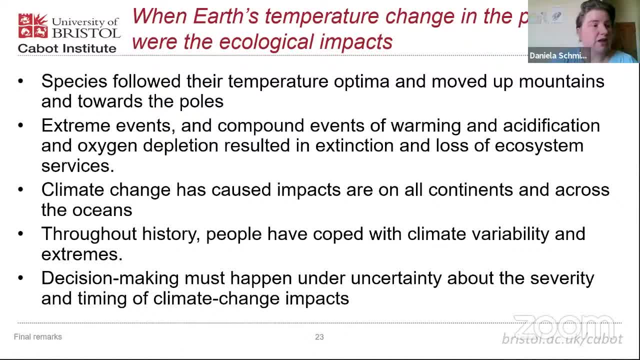 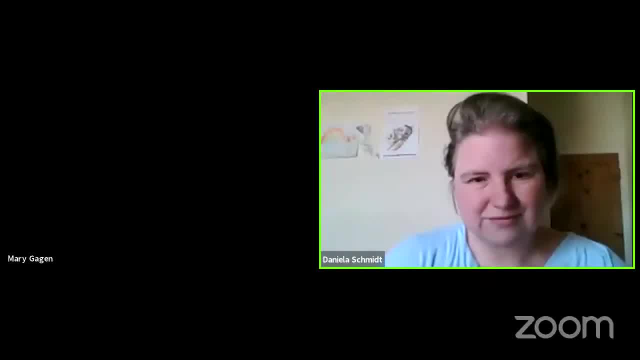 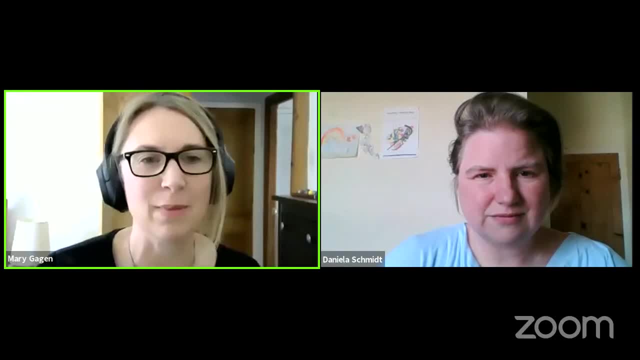 So we need to have a discussion if we want to have action, despite uncertainty about the severity and the timing of those impacts. Thank you very much. Thanks so much, Dani. Really fascinating, And it's always amazing to see those timelines next to each other. 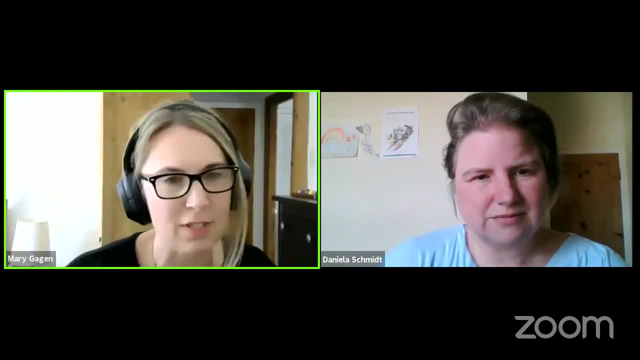 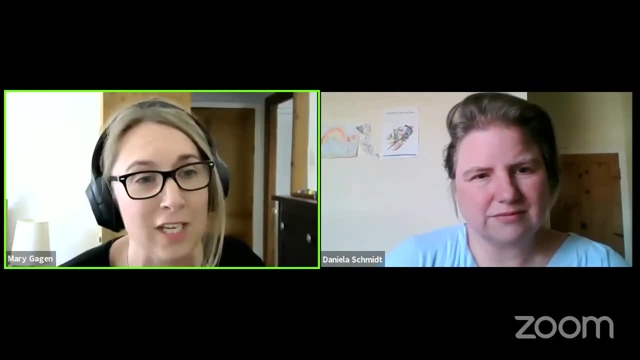 We've got some great questions And I would encourage you all to keep posting your questions And just to say to early career researchers who are on the webinar: please don't be shy. We're very keen to hear from you, Dani. I'm going to start with some of the more general questions that have been posted, if that's okay. 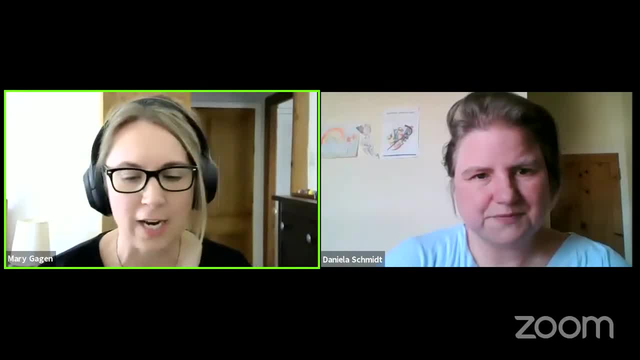 We've got a few questions around ocean acidification And whether future predictions take into account elements of ocean chemistry such as buffering effects. I wonder if you could talk to that for a moment. Yeah, I mean, the buffering effect is beautifully visible in the paleo example. Because what happened there is that the deep ocean sediments dissolved and therefore buffered The impacts. That process takes around the time of the turnover time of the ocean, So we're talking about a thousand years. So it's a question if we have that time. 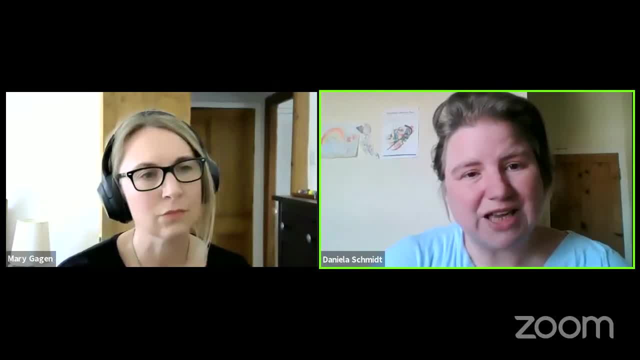 I've also seen another question which talks about the term ocean acidification in itself And asks: you know if the ocean will ever become acidic? And it's like no, it won't. We're still talking about global warming and Britain will nearly never be hot. 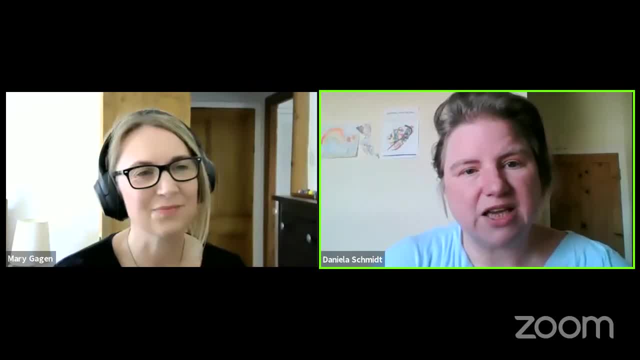 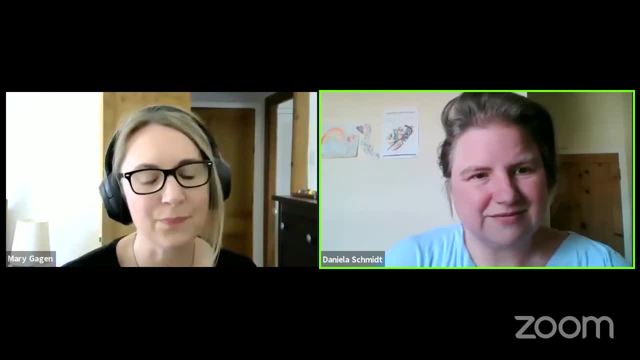 And still we're talking about the change, the relative change, And so acidification just talks about the change. It just talks about the move away from the basic 8.1 which we've had pre-industrial. Great, thank you. Thanks so much. 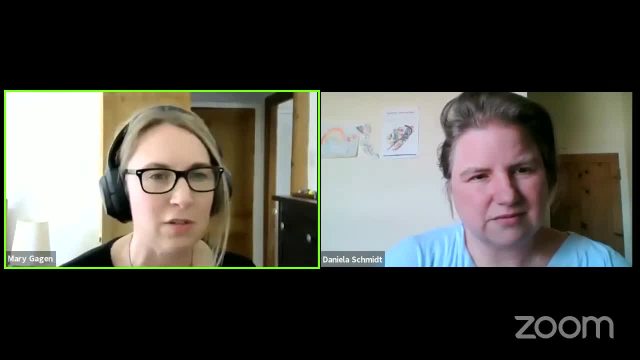 There's a question as well about how long some of the species that are in the oceans have been around, But I guess I would summarise as: if a species has remained largely unchanged for hundreds of millions of years, Does that mean it's immune to changes that happen over timescales of decades or a hundred years? So That's hard to say. In general, what we see is that species which are very specialised, so which live in a narrow geographic area, are those who are more vulnerable. So those which have long time ranges and those which have long geographic, wide geographic averages, tend to be more stable. 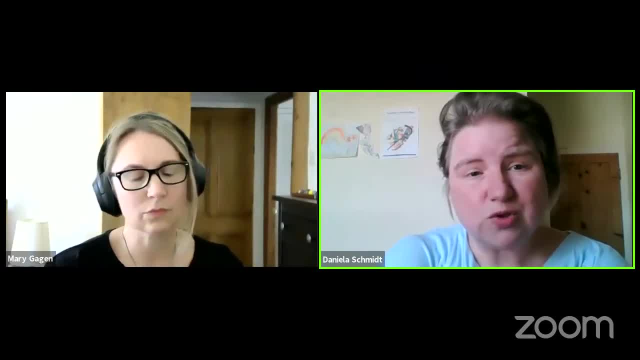 Because if they find environments at one location which aren't suitable for them anymore, they can move to another, While if you're highly specialised to one place, That next space doesn't exist, And so we tend to describe it more in terms of the specialisation of an organism. 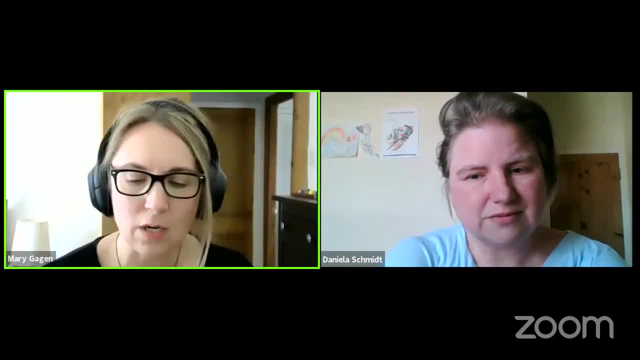 Thanks so much. There's a few people asking as well about the different, the variety of impacts that are on oceans at the moment- Things like overfishing and all the kind of ecological and human effects as well- versus climate change. So would you say that in our modern oceans, the current changes that we're seeing are mainly driven by climate change? 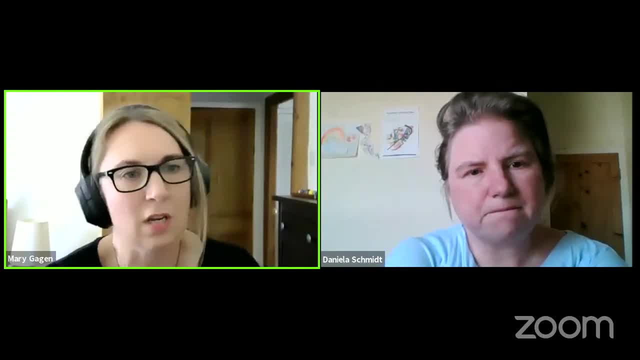 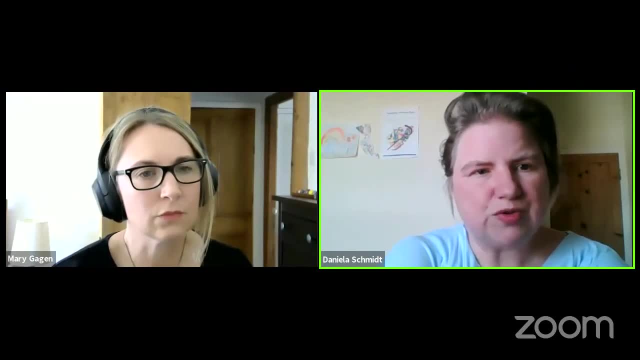 Or those other human effects, Overfishing and those sorts of things. So if we're looking at a coastal system like the UK, we can see that, you know, changes in land use change, the runoff into our coastal systems brings in more nutrients, brings in more sediments and therefore is impacting there strongly. 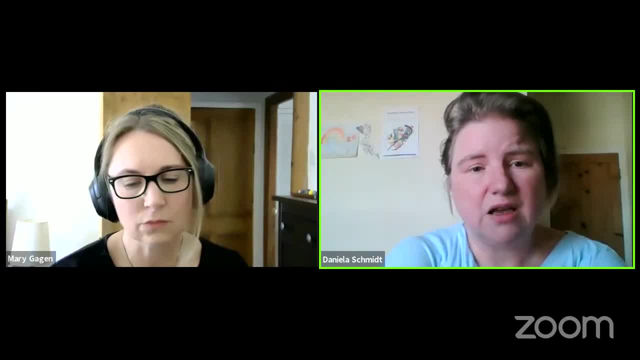 If people talk about fishing, that system is very clearly threatened because of the overfishing and not because of climate change. But going to the open ocean those pressures become smaller and therefore the impacts of climate change are significantly easier Because those other secondary drivers are less important. 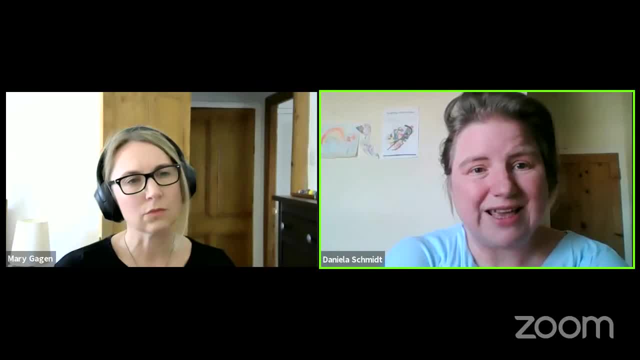 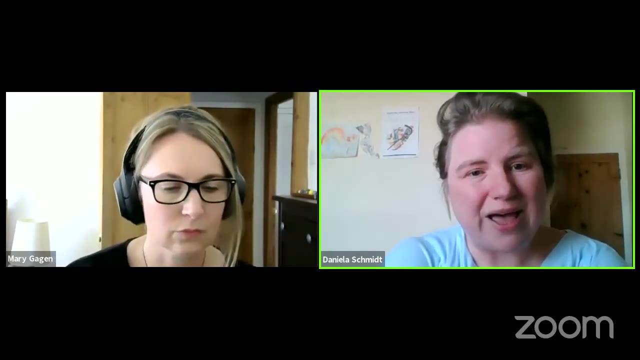 But in a coastal system, you can also turn this around and say: you know, we have the power to change things and reduce some of the stresses which, additional to climate change, impact those systems, Because land use changes, pollution, you know, of nutrients, of plastics, is in our hands. 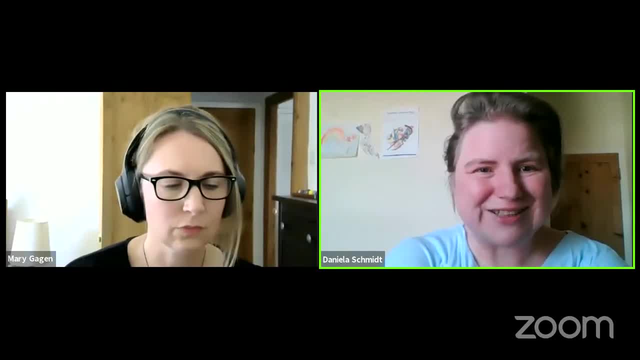 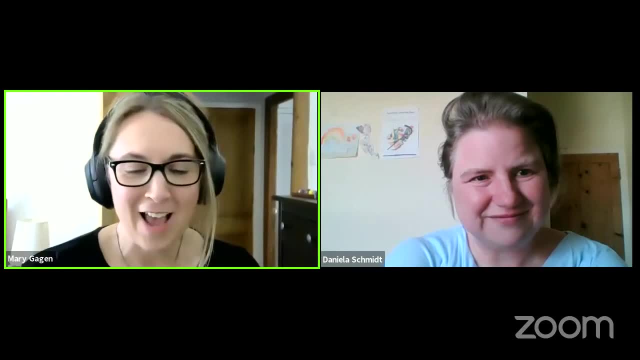 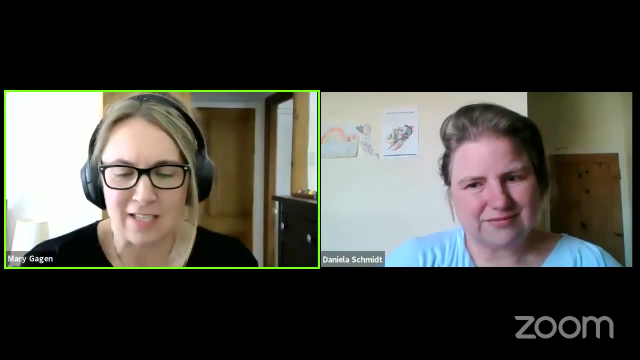 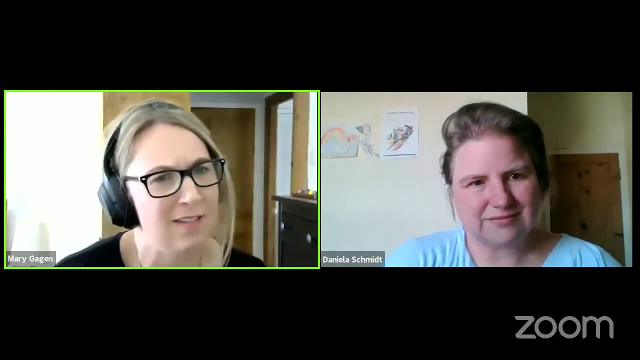 And so it gives us ability to take charge and change things and not wait for global decisions- Good, The all important decisions- being with us. So there's a question around the warmest seas and that there's a sense someone's saying they've read that the world's warmest sea, the Coral Sea, is actually the healthiest. 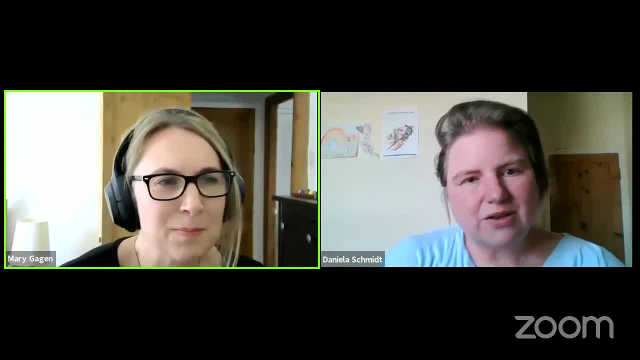 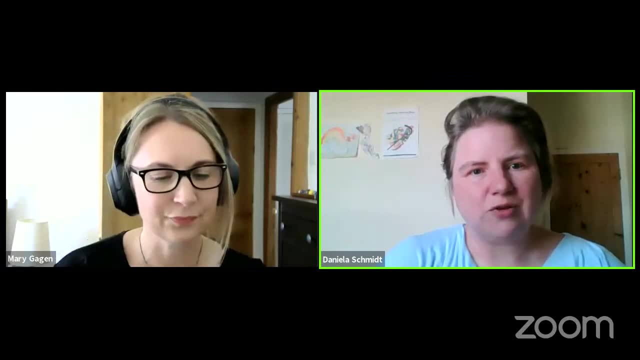 Could you talk about that? So it's a biodiversity hotspot. So it is a place where a lot of species live. So it's a place where a lot of species live. So it's a place where a lot of species live. So because of the humidity, it becomes quite a very cold place. So it's not very warm, But a lot of those different species have been living for a long time And because it is relatively warm today and there's species reaching the temperature range, it is a much more vulnerable place. So you can have a very healthy place if there's very little human interaction, which is now very vulnerable because the species are at the upper-end of their temperature ranges. 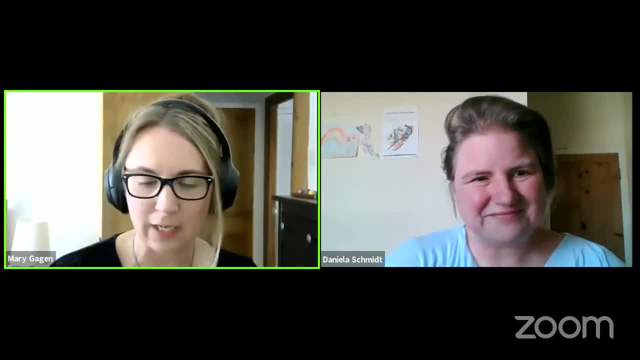 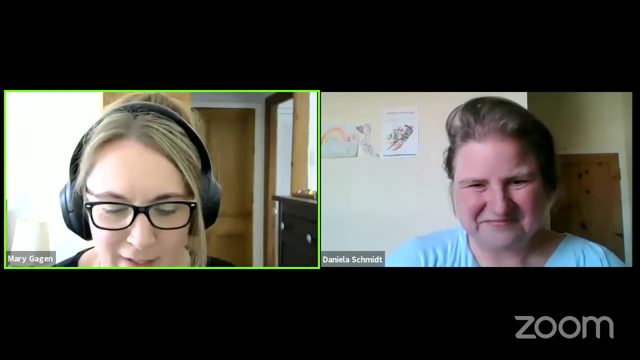 i'm keeping my eye on on the clock and we are- we are- shockingly on time, so i'm i'm going to just wrap up with one, one question, if that's okay, and then we'll stay on time. um and sorry, just let me. i'm just scrolling through questions here to try and make sure i'm i'm, uh, spotting. 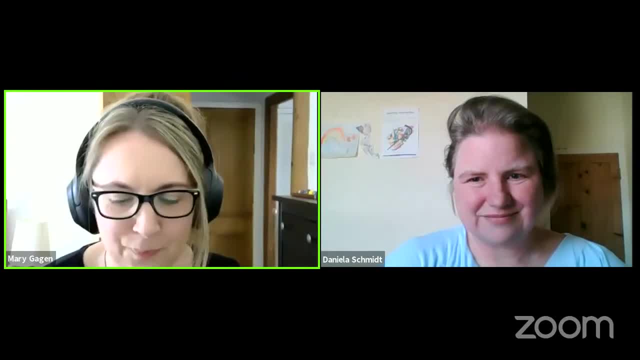 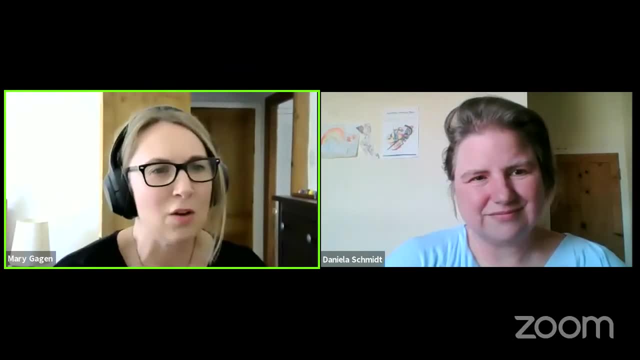 everything okay. i think we've covered some of those. um. i wanted to ask you, danielle, actually, if i could, about um connectivity in the ocean. so when i talk to marine ngos, this is a really hot topic for them: the idea of how source areas and connectivity is really important for species. 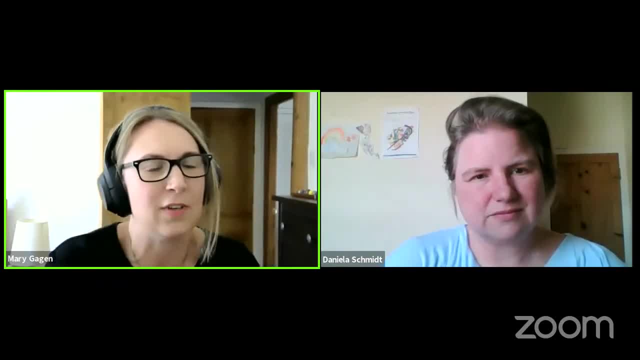 health. so a herring spawning ground is essential for the survival of that species. and, um, i always think it's really interesting to think about how climate science can kind of address those questions that are vital for the ngos that are trying to manage environments. now, and is that? 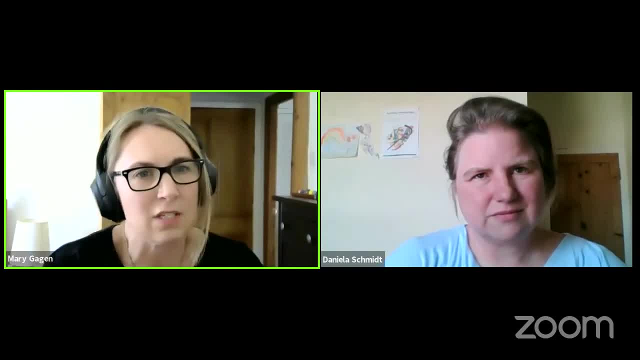 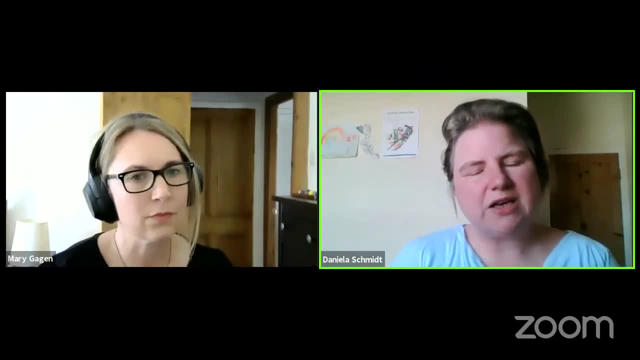 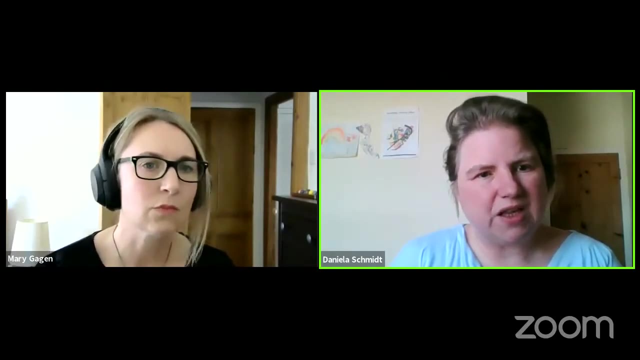 is there anything that the geological record? can you see evidence of changes in connectivity in the past from the geological record? so if we take the example again of the paleocene, you've seen thermal maximum. we saw species which have never been seen in high latitude suddenly moving into those regions. so if we have such dramatic changes, 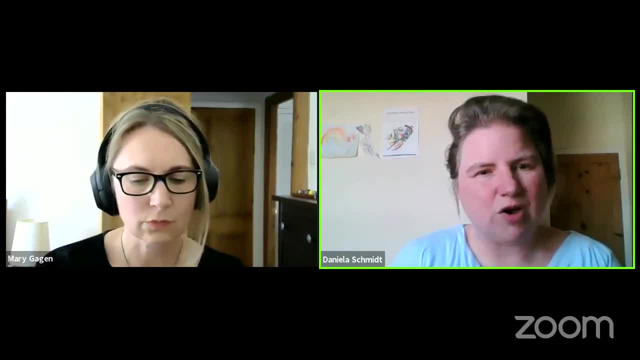 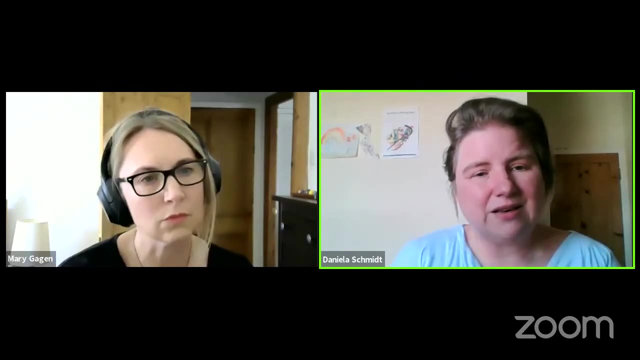 in the distribution. we also need to think about that today. our approach of those ngos and is to protect marine protected areas. if marine protected areas that were static and are not changing with the distribution of those species changing- so that's the connectivity they talked about- then they become not fit for purpose when we already see relocation of species over the last. 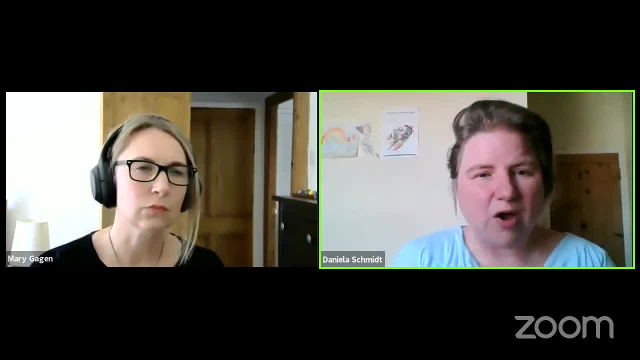 you know, decades, and so that's something which, again, is really powerful for for us to think about. you know how we could um improve some of of the threats, to reduce some of the threats to species is by having protected areas which allow those stepping stones where you know the brood, the 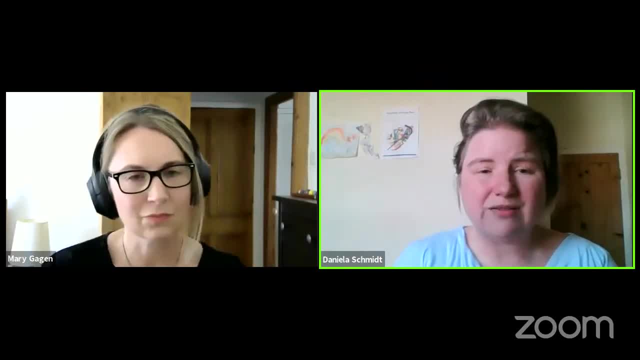 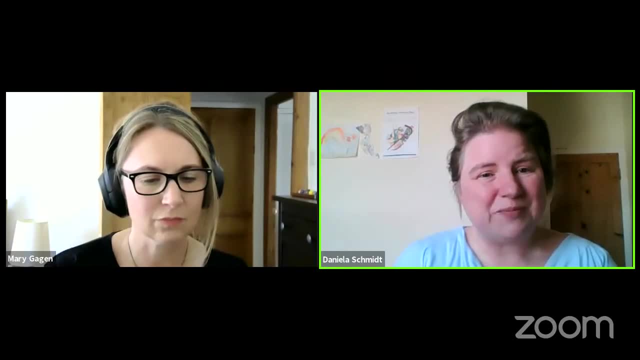 breeding grounds, the adult species, the- or in a relocation of species further to the north in the uk. we are in the transitional zone between two climate zones and so you can see those changes along our coast really rapidly. but it also allows us to provide those stepping stones for species. 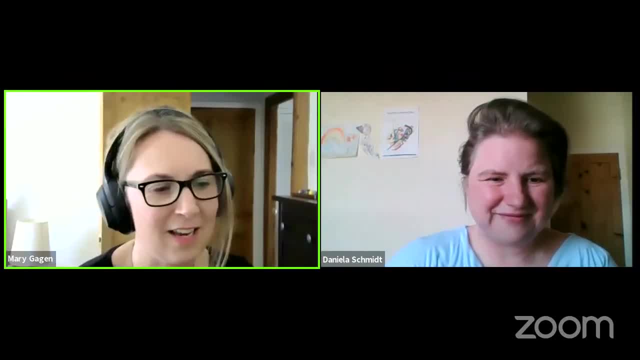 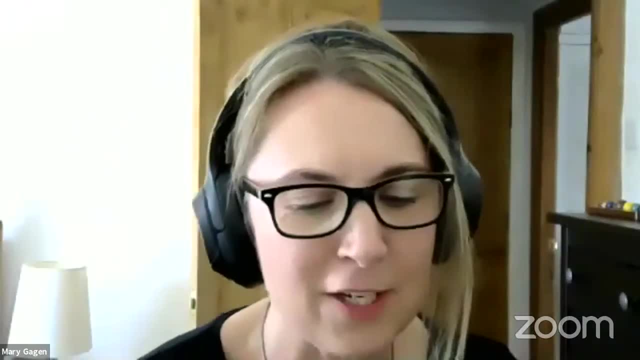 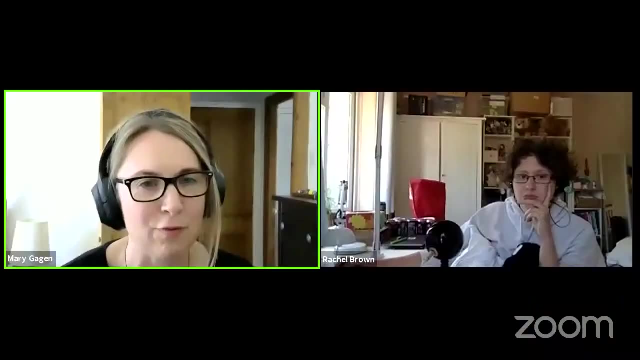 thanks so much, danny. um, really really fascinating start to this session. um many thanks. um, i'm going to stay nicely on time and move on to the first of our flash talks from um, the first of our early career researchers for this afternoon, and it's my pleasure to introduce. 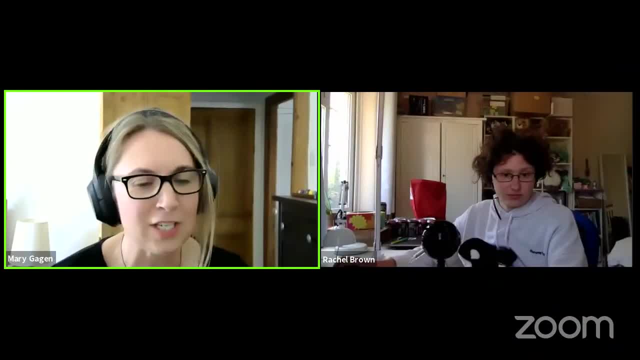 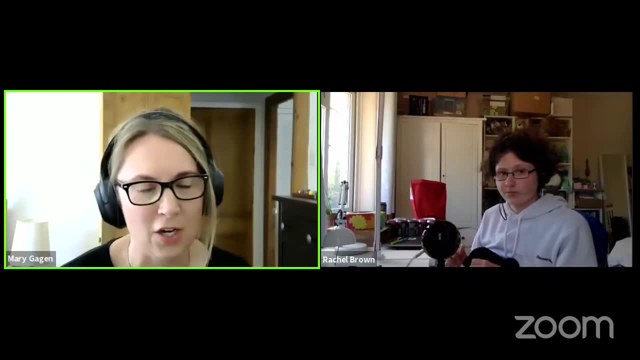 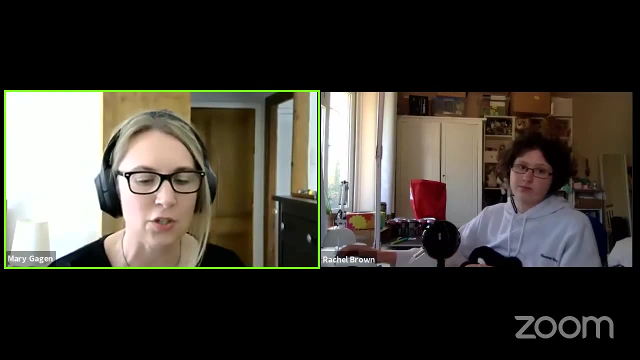 rachel brown to you. rachel is a third year phd student with gavin foster at the university of southampton and her work looks at boron isotopes and using them to reconstruct past co2. i look at investigating the role of co2 in relation to the major climate transitions. 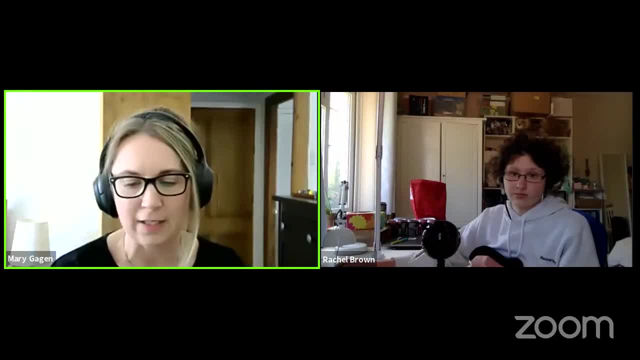 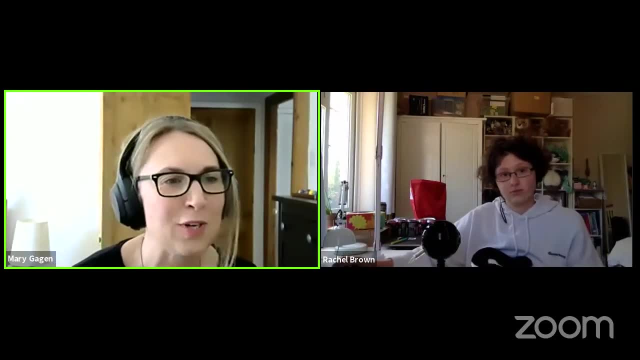 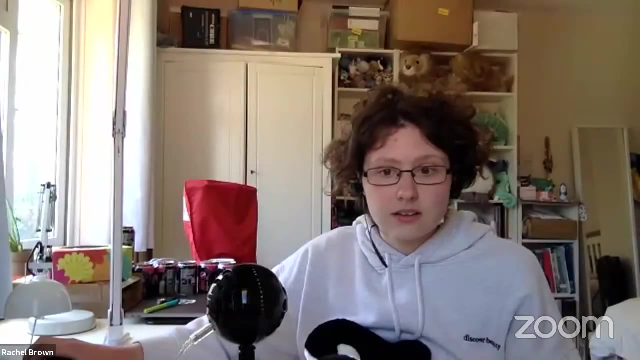 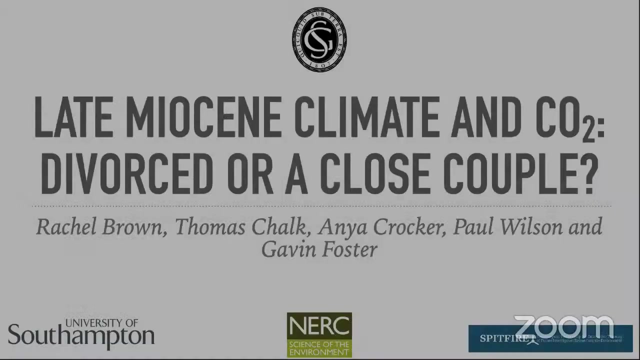 such as the intensification of northern hemisphere glaciation and late summer myosin cooling, and she's going to be talking about myosin co2 in her talk now. so i'll hand over to you, rachel. thank you okay. you can see it, we're good. yeah, go for it, rachel. thank you okay, okay, hi, uh, yeah, so today i'm going to be talking. 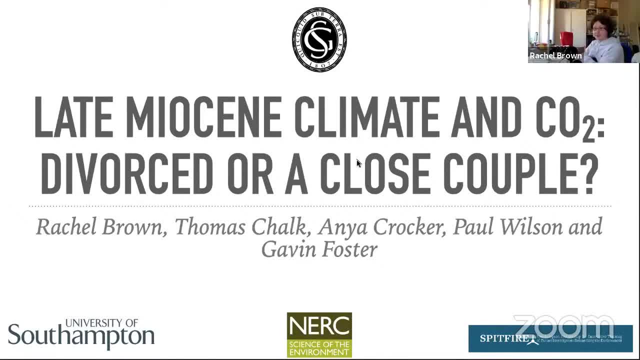 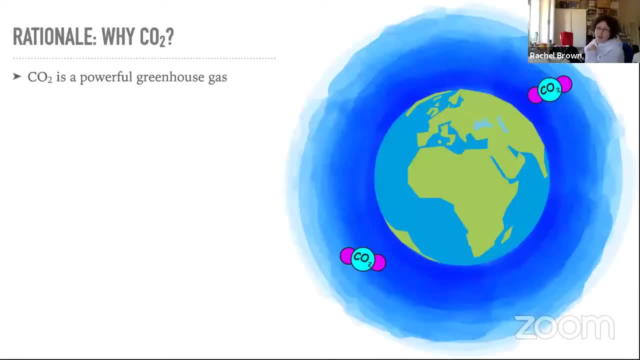 to you about, uh, late myosin climate and the role of, and its relationship with co2. uh, thank you to all those people for helping me with all this and, uh, these people for paying my rent. so, first things first. why do we care so much about co2? uh, well, it's a really powerful greenhouse gas. that is. 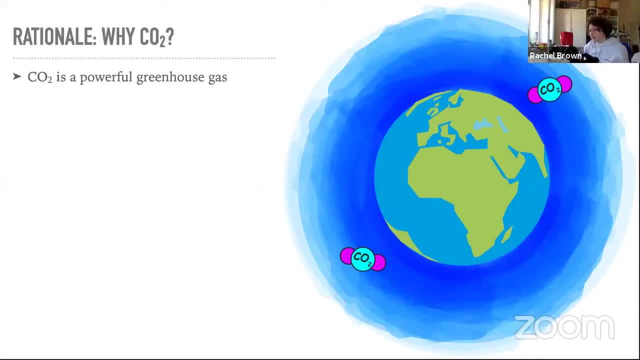 able to generate a lot of greenhouse gas and it's able to generate a lot of greenhouse gas and it's able to generate a lot of greenhouse gas and it's able to generate a lot of greenhouse gas. heat in the atmosphere. you increase the amount of co2 in the atmosphere. you increase the amount. 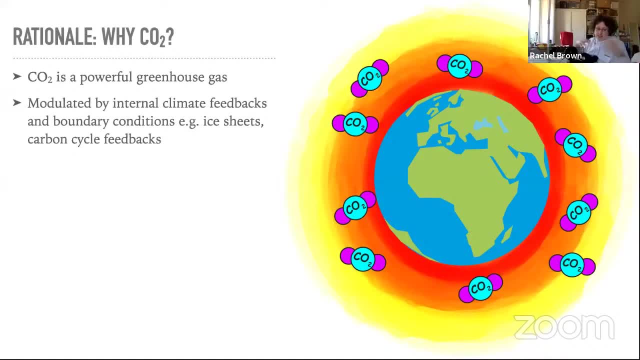 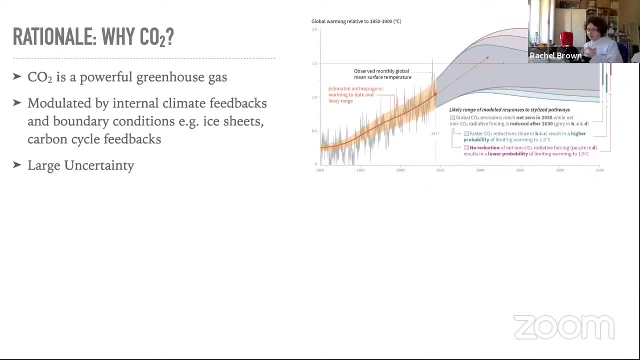 of heat trapped and that results in warming. however, however, this relationship is modulated by internal climate feedbacks and boundary conditions. as a result, the uncertainty in regards to what the expected temperature changes for any given change in co2 as a. therefore, one way to reduce this uncertainty is to look at the relationship between co2. 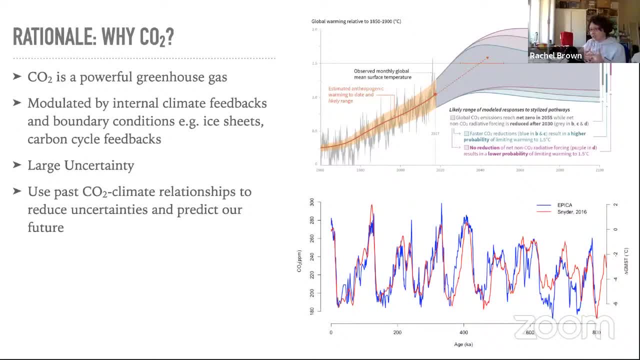 and climate in the past. the majority of studies that have done this previously have focused on periods that are um much colder, and primarily the late pleistocene like. the problem with these in regards to like constraining future warming is that they're one colder and also they have really 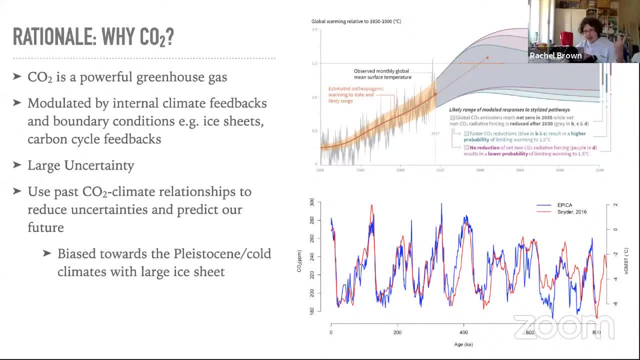 large ice sheets, which we're going to be both warmer and and have no ice sheets in the future. so, given that there's potential for state dependency of climate sensitivity, we should probably also try to look at the relationships between co2 and climate sensitivity in the future. 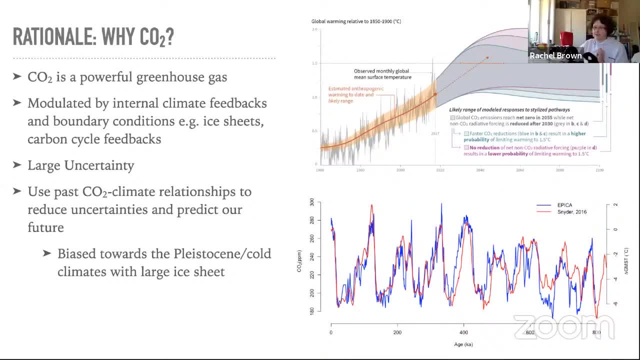 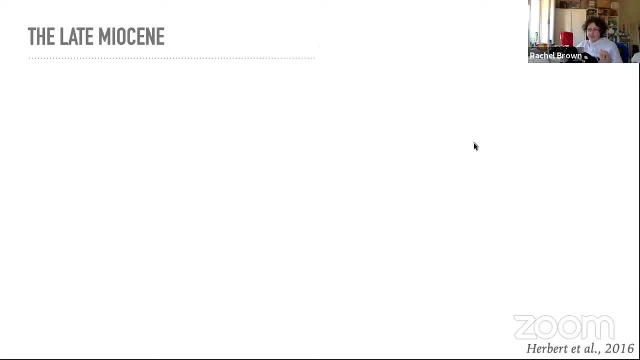 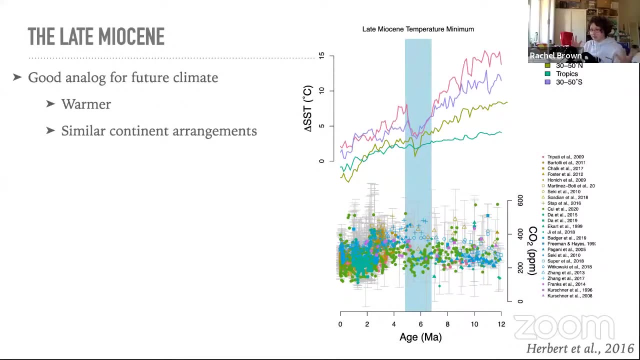 and climate in warmer than present climate, past climates enter the late myocene. the late myocene is a really good time period to target for these kinds of studies, mainly because it is, one warmer than present and, two, the arrangement of the continents is similar to that of today, so it 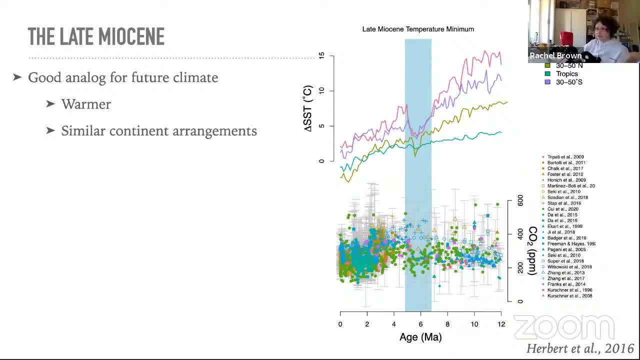 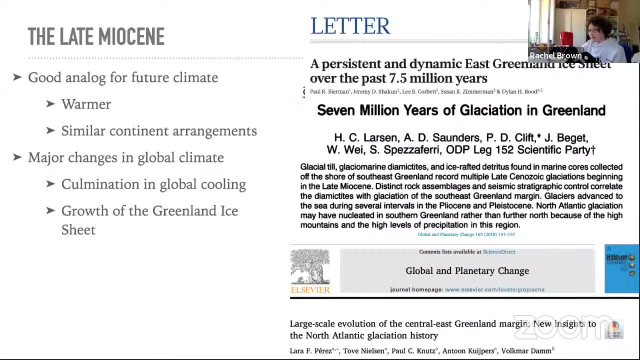 has similar boundary conditions. it's also a period of intense climate change, given that it there was substantial global cooling, there was likely the beginnings of the builds up of ice sheets in the northern hemisphere and there was likely the beginning of the builds up of ice sheets in the 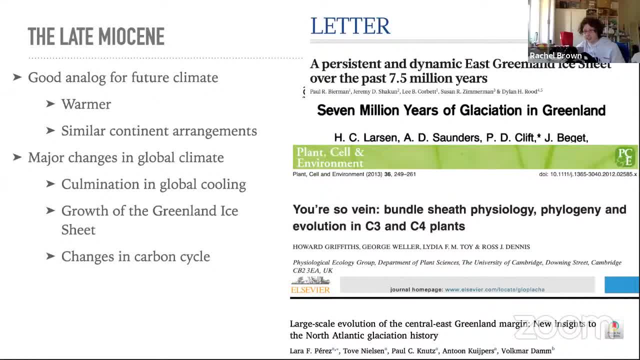 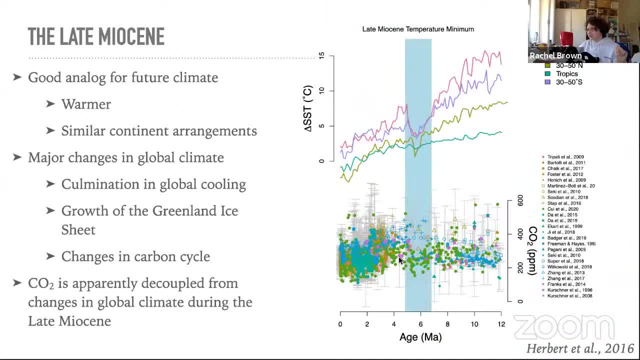 northern hemisphere. there were substantial changes in the carbon cycle and global vegetation, to name but a few. however, in spite of all these changes in global climates, the co2 record is rather ambiguous, showing not a lot of change in co2. this has led to the suggestion that co changes in co2. 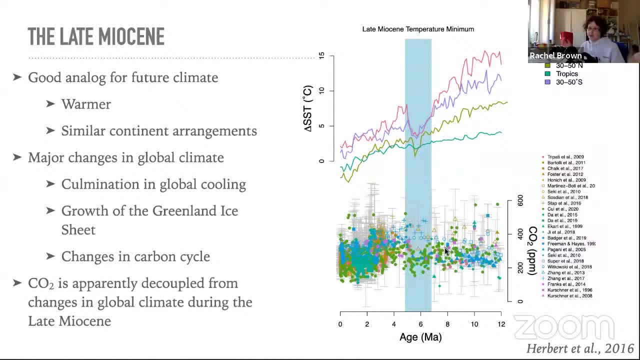 were actually decoupled from changes in global climate during the late myocene. however, a lot of these records are one associated with some pretty large errors that make it difficult to resolve these changes in co2, and the other is that the climate changes in the global climate are not 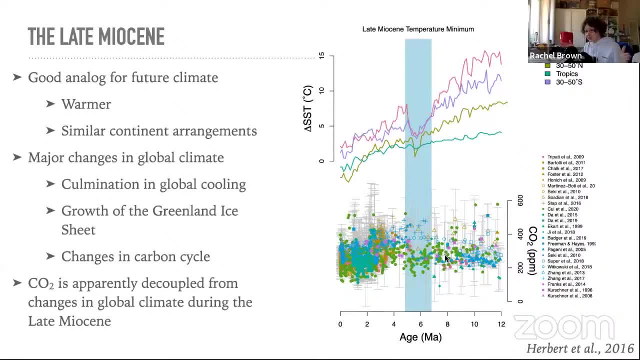 in co2 and also a lot of these records are really low resolution, meaning that we may be aliasing any of these changes in co2. as such, we decided we wanted to create a high resolution record to resolve these changes in co2 during the late myosin, particularly during this period. 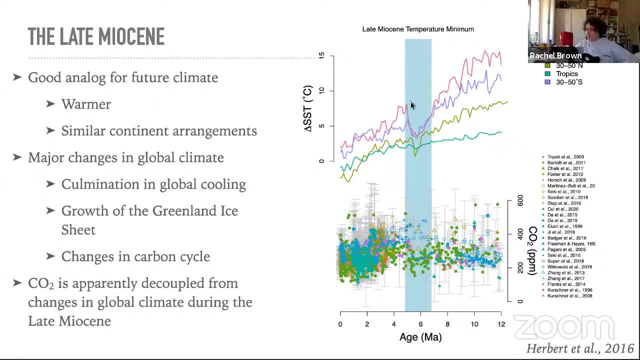 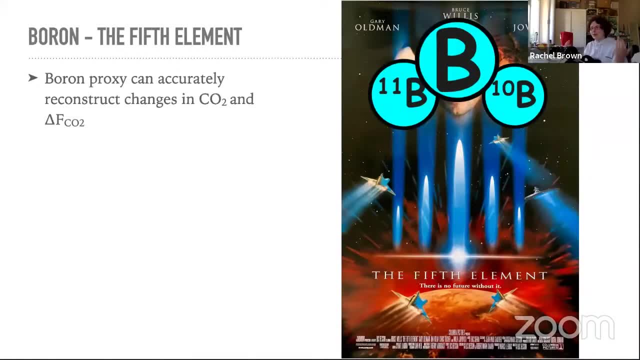 sent. when the um during the temperature minimum of the late myosin from five to seven million years ago, we were able to do this using foreign isotopes. now foreign isotopes are able to really accurately reconstruct changes in co2 and the radiative forcing associated with it. 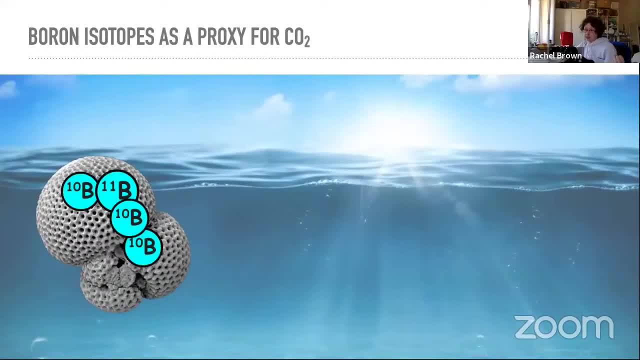 we're able to do this by first looking at the ratio of the stable isotopes in little surface dwelling plankton called form nephro. now, the change in the boron isotopes of these little forums is directly is strongly core, is directly related to changes in surface ocean ph. now, because 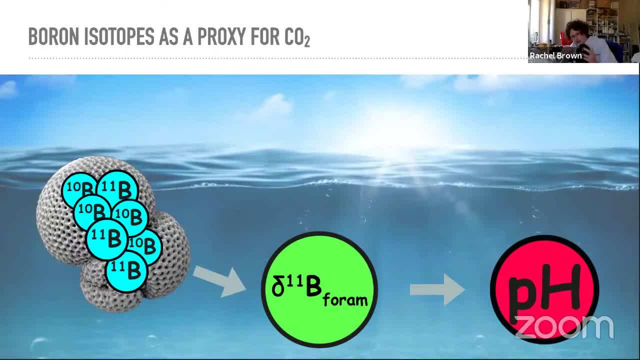 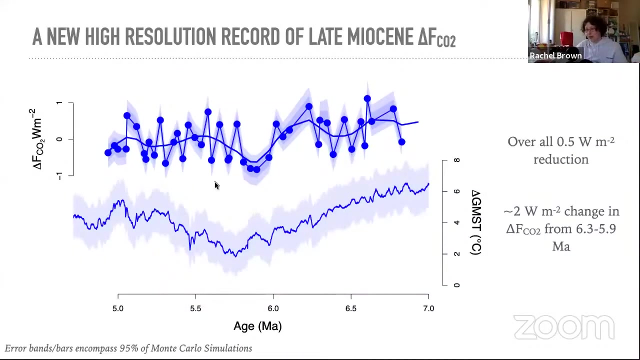 social changes in. still hear me, because, because changes in surface ocean ph are directly correlated with changes in atmospheric co2, we can use the relative changes in boron isotopes recorded in these forums to reconstruct changes in co2. so what did we find for the miocene? well, in regards to, we found that there. 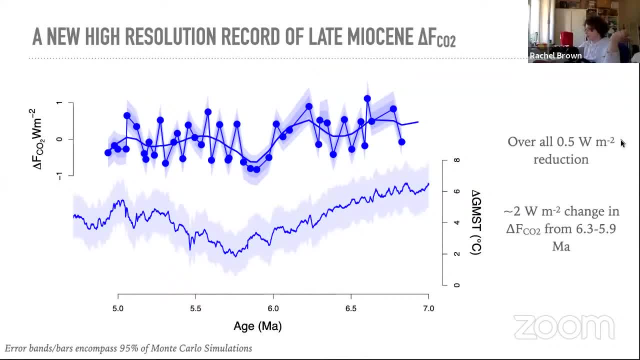 was about a 0.5 watts per meter squared reduction in forcing associated with co2 during the late miocene, but we also- probably more notably- observe of two watts per meter squared reduction in radiative forcing associated with co2 from about 6.3 to 5.9 million years ago. 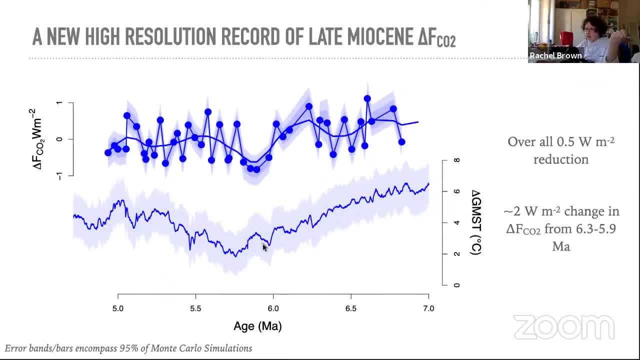 this corresponds with all the previously mentioned change: changes in global climate observed during the late miocene, the global cooling minimum, the growth, the um expansion of ice sheets in the northern hemisphere, carbon changes in vegetation- all of them. as a result, our record strongly implies that, contrary to previous suggestions, co2 and climate were coupled during. 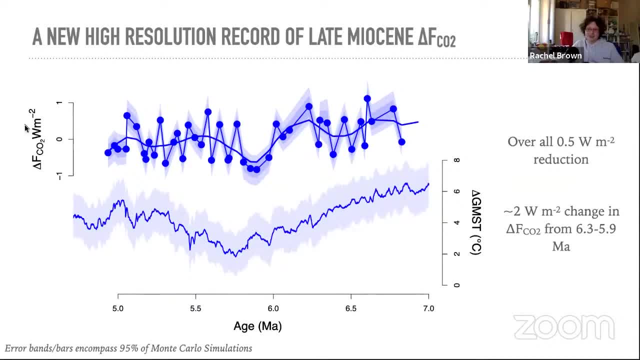 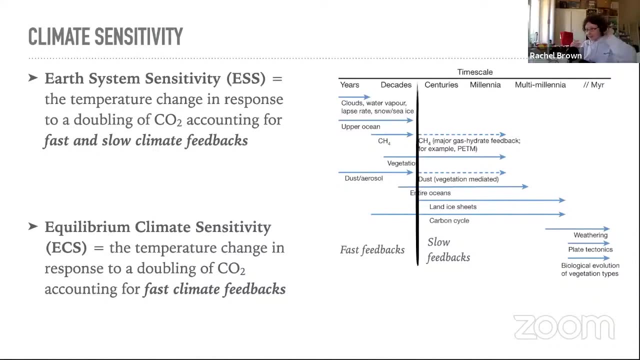 the late miocene. so we have a record of the radiative forcing from co2 and global mean surface temperature change. next stop is to calculate climate sensitivity. so a quick reminder about all the different climate sensitivity definitions that von der heide talked about really nicely yesterday. um first Earth system sensitivity is the temperature change. 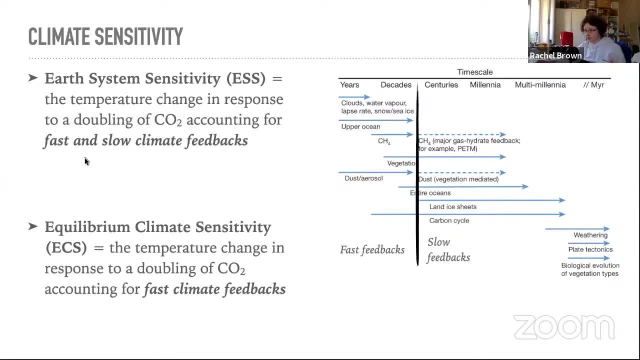 in response to a doubling of co2, accounting for fast and slow behavior, if you will, these skydiving Representations of power in a open universe range human and anylica reach. climate feedbacks, Equilibrium, climate sensitivity only accounts for fast climate, fast climate. 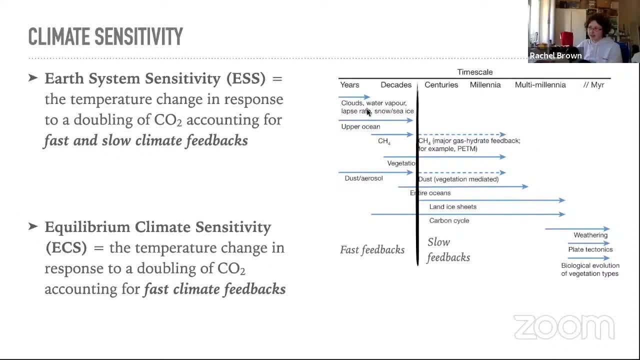 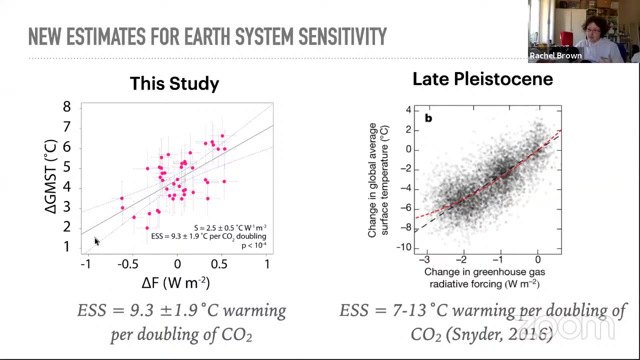 feedbacks, ie climate, ie changes in clouds, while Earth system sensitivity will also account for changes in land, ice sheets and carbon cycle changes. So we estimate that equilibrium climate sensitivity or Earth system sensitivity for the late Miocene to be between, to be about 9.3 to. 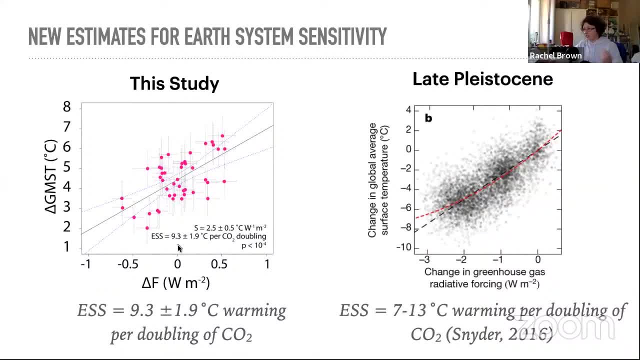 9.3 degrees warming per doubling of CO2.. This is really similar to that observed during the late Pleistocene, which is generally, which is between 7 and 13 degrees warming per doubling of CO2.. This strongly implies that very strong, that strong slow climate feedbacks were operating. 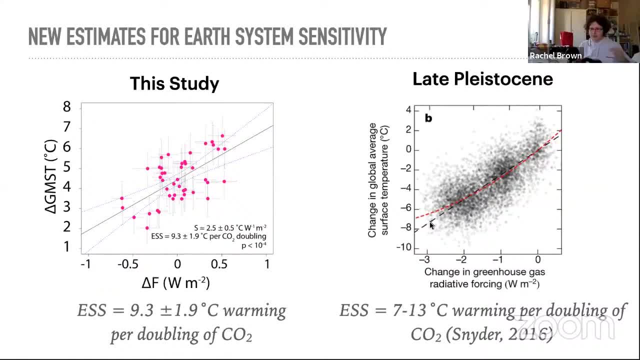 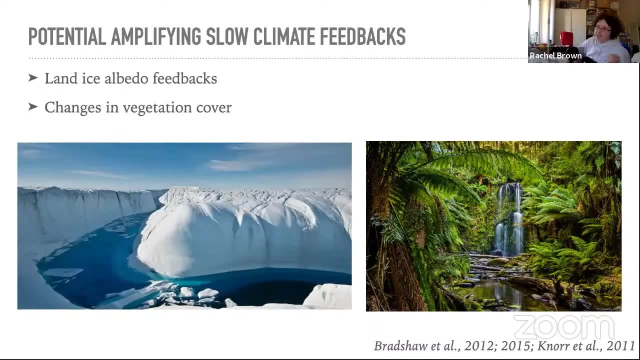 during the late Miocene. similar to how, similar to what was off, similar to the late Pleistocene. Indeed of various model simulations for the late Miocene climate. suggests that suggests that a high sensitivity was due to some land ice albedo effects. and 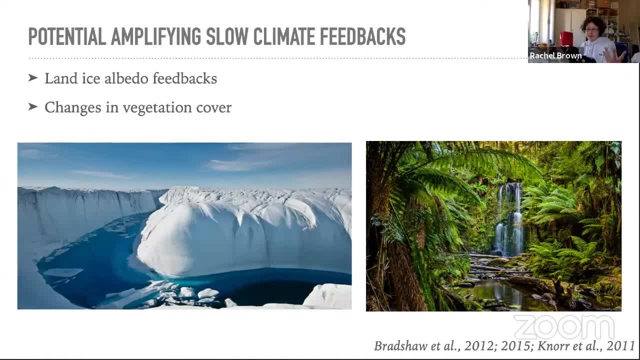 differences in global vegetation cover. To calculate equilibrium climate sensitivity from this, given that we don't actually have, like direct proxy measurements for the radiative forcing associated with albedo feedbacks from vegetation or ice sheets, we we look at the we look at the ratio between equilibrium climate sensitivity. 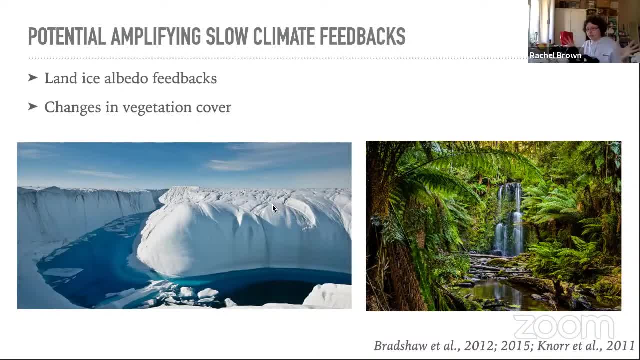 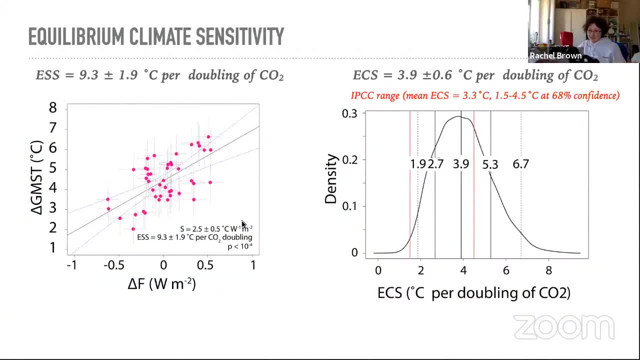 and Earth system sensitivity a suite of various models, and use that to parameterize slow climate feedbacks. Using this method, we're able to estimate equilibrium climate sensitivity for the late Miocene to be about 3.9 degrees plus or minus 0.6 per doubling of CO2.. This is well within the range. 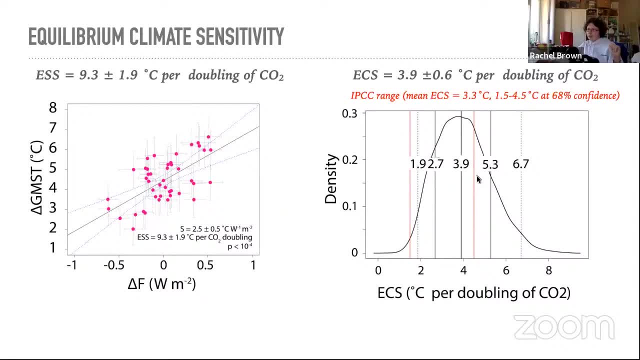 given by the IPCC of 1.5 to 4.5 degrees and strongly suggests that we don't actually see any state dependency in regards to warm climates with equilibrium climate sensitivity. This is not to say that there isn't any state dependency, just that we currently don't see any in our data, as 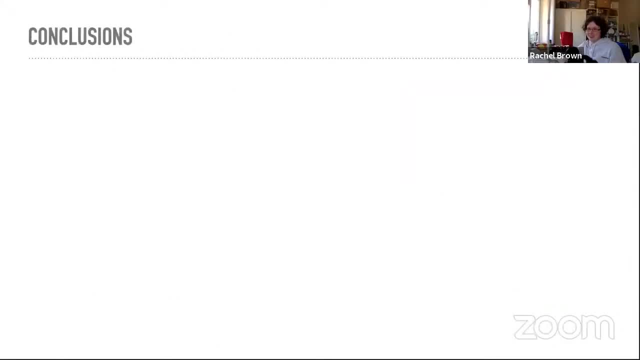 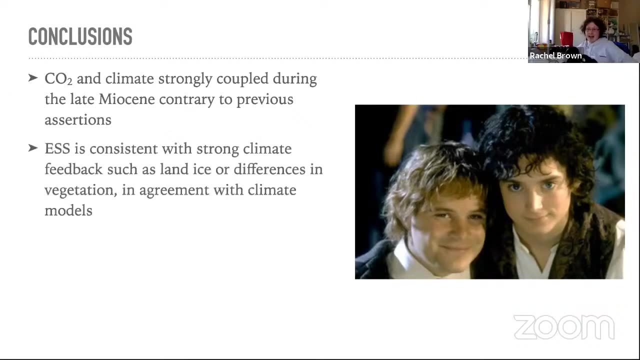 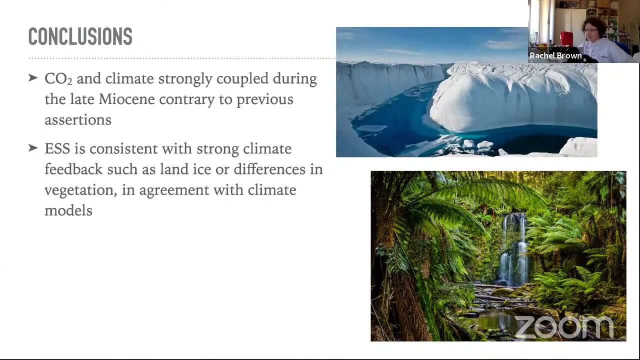 currently is So. to conclude, CO2 and climate were strongly coupled during the late Miocene, contrary to previous assertions, And the higher system sensitivity observed is likely due to strong slow climate feedbacks such as ice sheet and different coverage and vegetation albedo feedbacks. And when we take 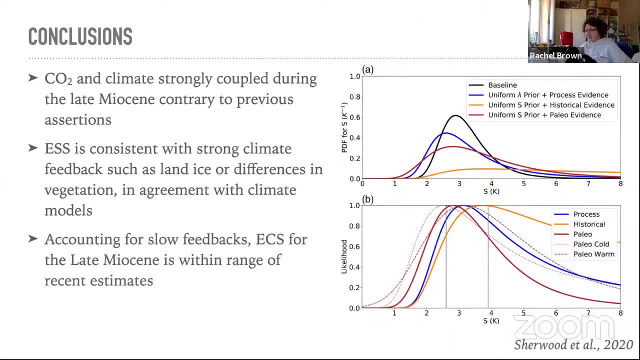 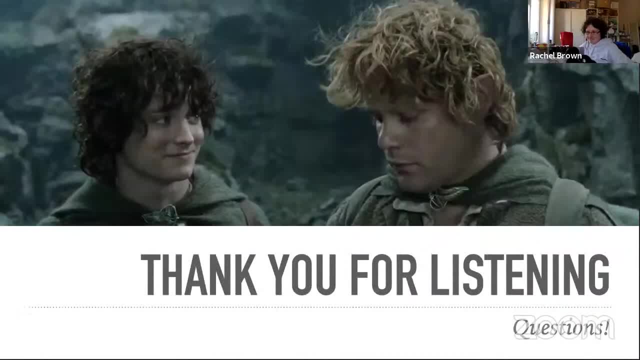 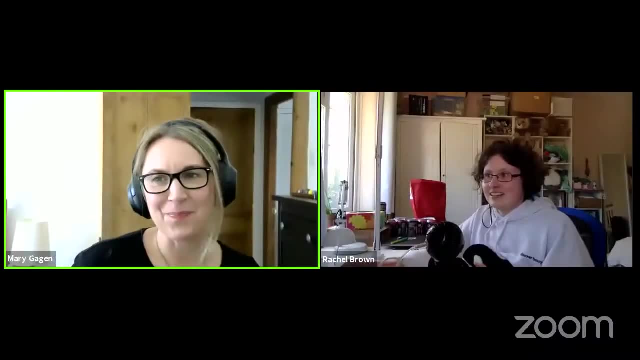 into account these slow feedbacks, we get an equilibrium climate sensitivity. that is for the late Miocene, that is, within range of recent estimates, Thank you, Thanks so much. Rachel Whistle stopped all through the Miocene there Just to keep us on track. I'm just going to ask one or possibly two very quick questions. 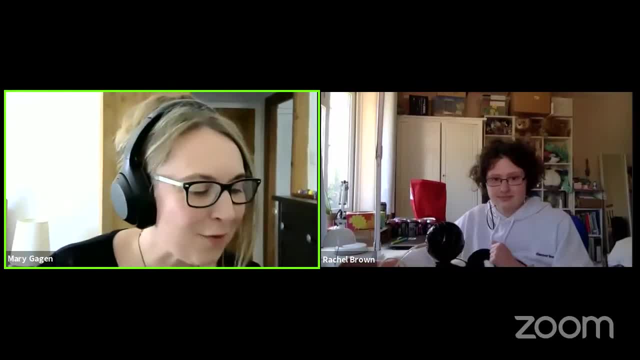 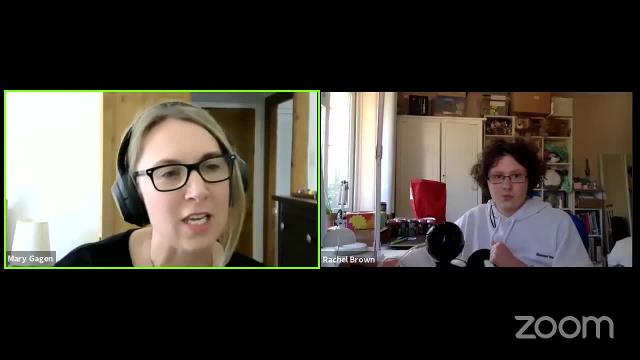 if that's okay. So first of all, can I ask you to talk a little bit about what we think has caused these changes in Miocene CO2?? Do we think they were weathering changes that dominated, or volcanic, or a combination of the two? 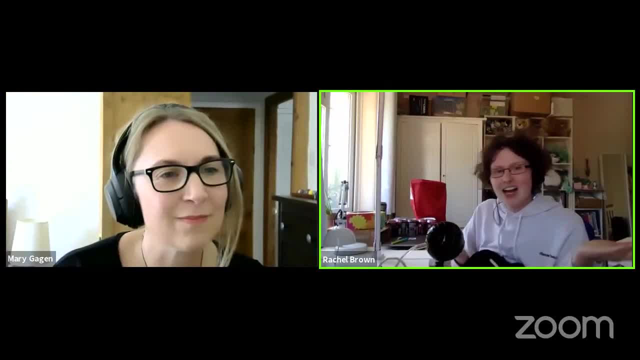 No one really knows. There were a lot of changes in the carbon cycle during this period, particularly with, with in regards to like there was a carbonate crash, where a lot of carbonates just started dissolving for a bit, And there's the shift in, there's a drastic shift in the 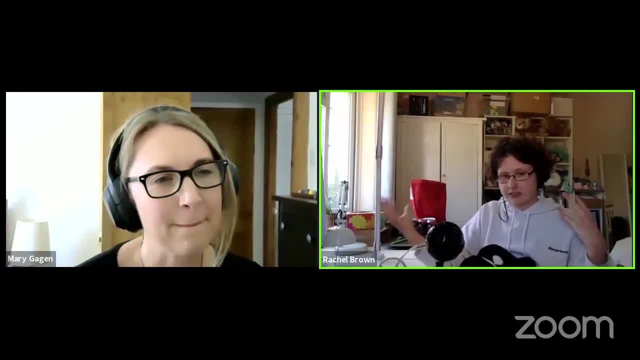 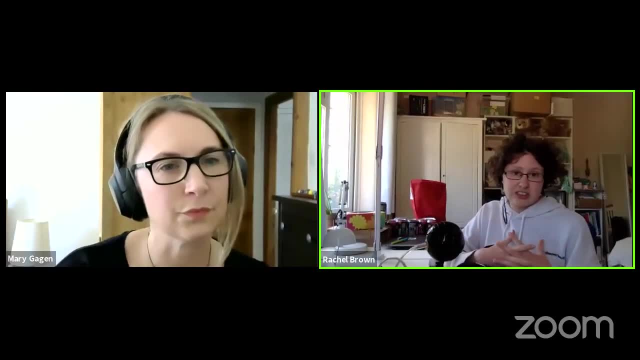 vegetation In like in vegetation on terrestrial, in the terrestrial realm. So there is suggestion that potentially there was a shift in where the carbon was stored into the deep oceans. So that might be it, But we don't really have good enough records at the moment to resolve. 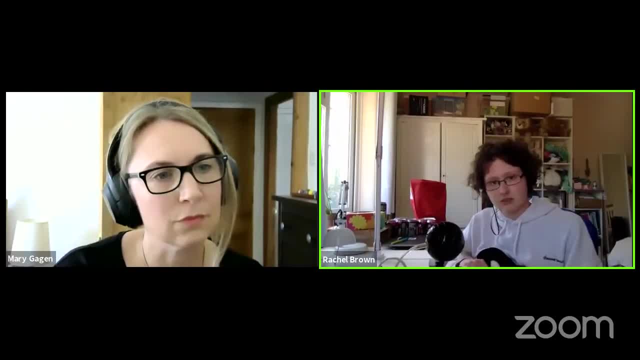 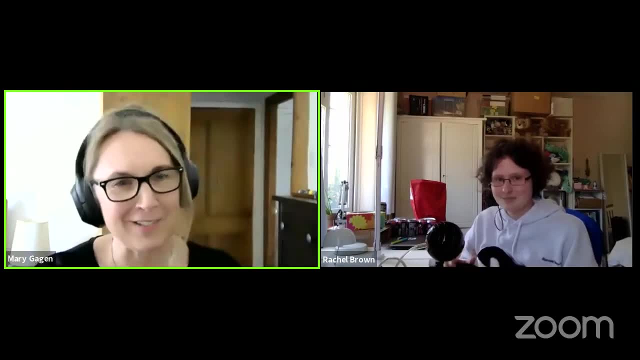 what might have been the mechanism for the CO2 reduction. That's always a good one, And if you're, if you're starting out on your work, you've got something for the future. Unanswered question. Um, one other question. 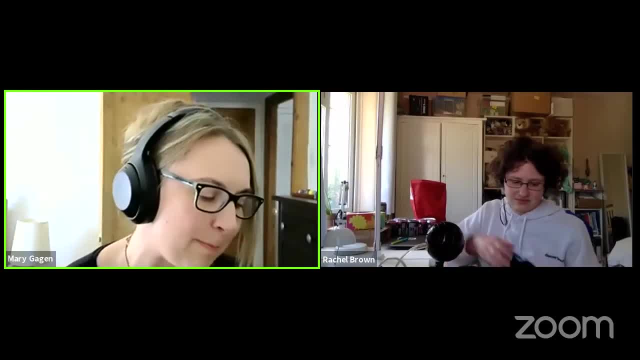 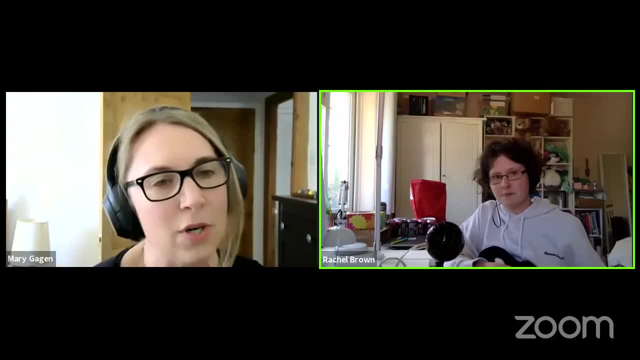 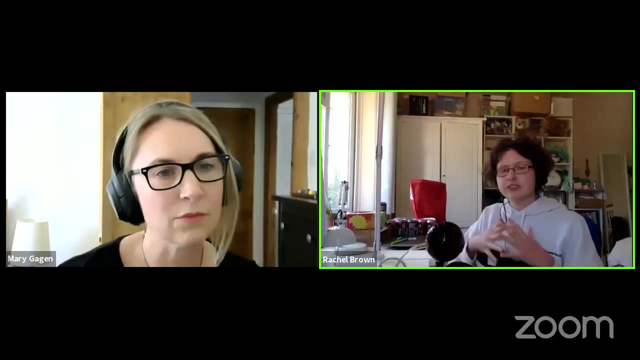 Someone's asked with regards to Miocene ice feedbacks, were they mostly related to Northern Hemisphere or Southern Hemisphere ice sheets? Or again, is that, is that something that's in progress? Uh, that is something that we don't know. There was like there was growth in both the 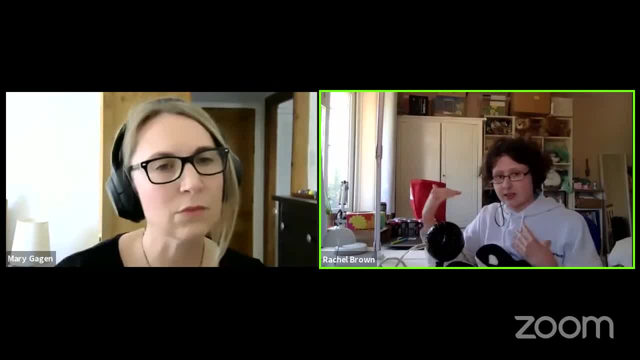 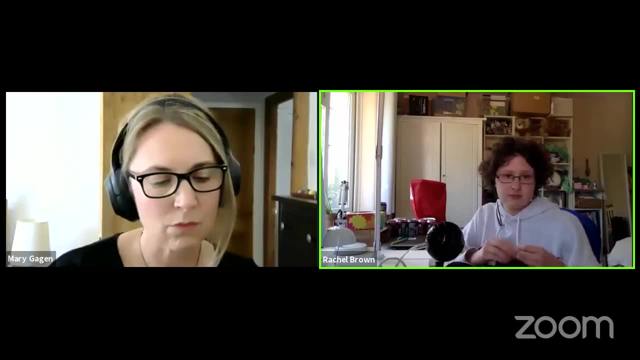 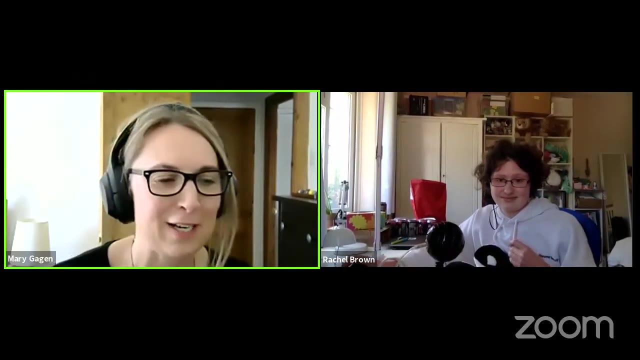 Antarctica at this time was also growing as well, as there was an increase in sea ice and ice in like the Northern Hemisphere, So both probably contributed most likely. Thanks so much, Rachel. Um, really, really fascinating talk there. Thank you for for one of our flash talks And we're gonna move on Now, more or less. 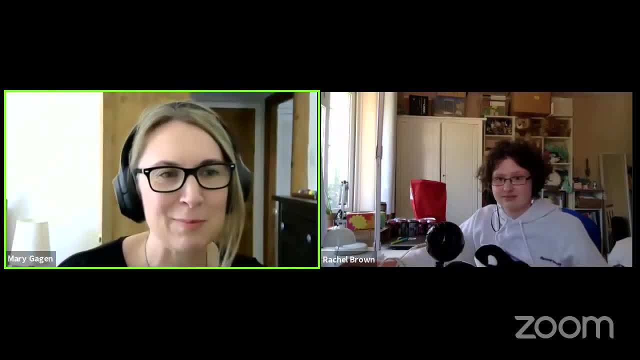 exactly on time. I'd say thank you so much to our speakers so far for sticking to time. Um so our next invited speaker is Alan Hayward. Alan is professor of paleo climate modeling in Leeds in the School of Earth and Environment. Alan Hayward is professor of paleoclimate modelling in Leeds in the School of Earth and Environment. Um Alan was Creative Director of the Singapore Skyline and Water Science programme and he's a professor in the School of Earth and Environment And so, on the survey, he has been working with Professor Kurt Becker, Professor of Analytics and Climateale Oloughby, and Professor David Oyel and Professor Dominique Nott. 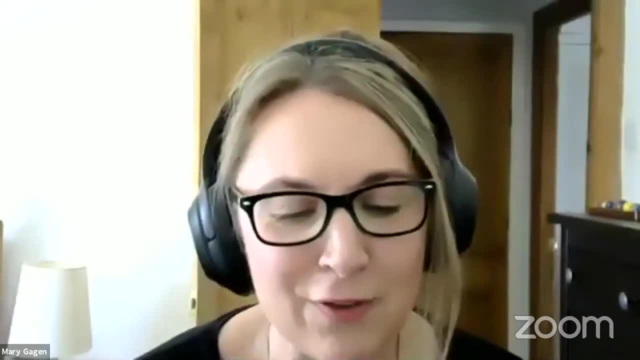 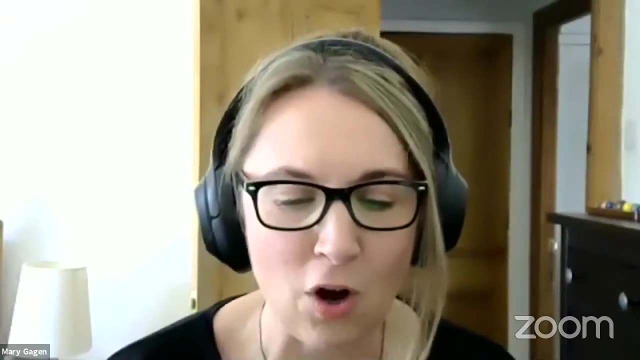 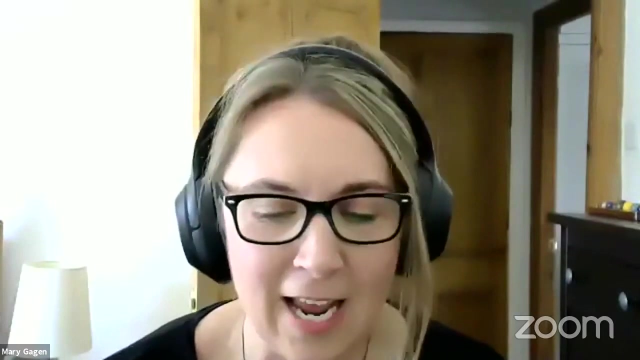 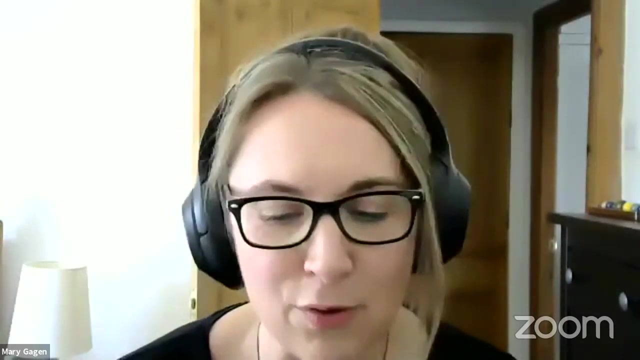 Alan was PDRA within Meteorology at University of Reading and then moved to BASC, the British Antarctic Survey, where he directed a five year research programme on the greenhouse to ice house transition within Antarctica. Since joining Leeds, Alan has helped to lead the International Pliocene Model Intercomparison Project and he contributed to both the fifth and the sixth assessment reports. 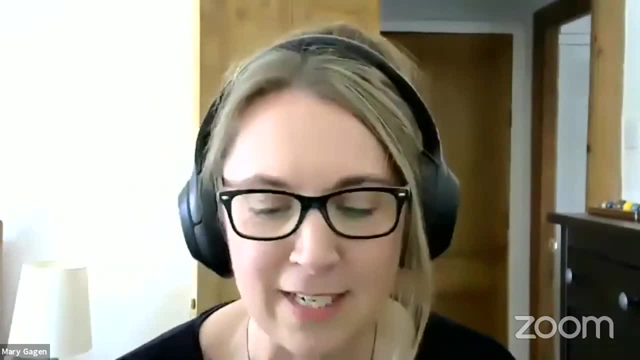 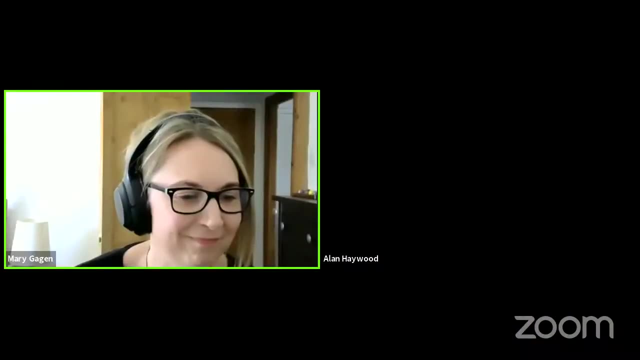 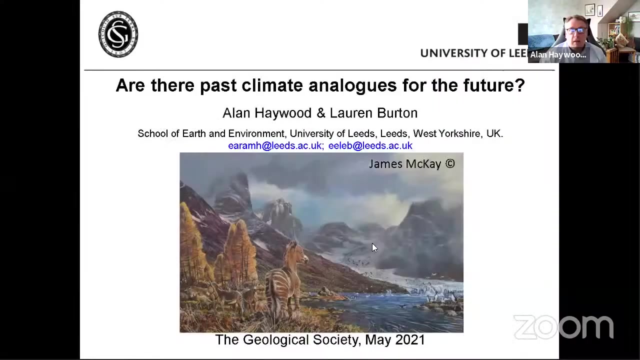 Alan's going to talk to the seventh question in the climate statement, which is: are there past climate analogues for the future? So I'll hand over to you, Alan. Okay, thank you. Thank you, Mary. Okay, can you see that okay? 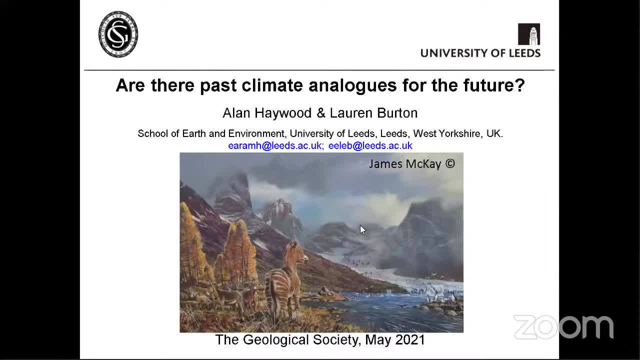 Yeah, that's great, Alan. Thanks, Okay, thanks very much. So let me start by saying thank you for the invitation to contribute To this event. I was fortunate enough to be involved in helping put together the first position statement on climate change, which was done by the Geological Society some years ago, So it's great feedback to contribute again to this active area, an important area of science. 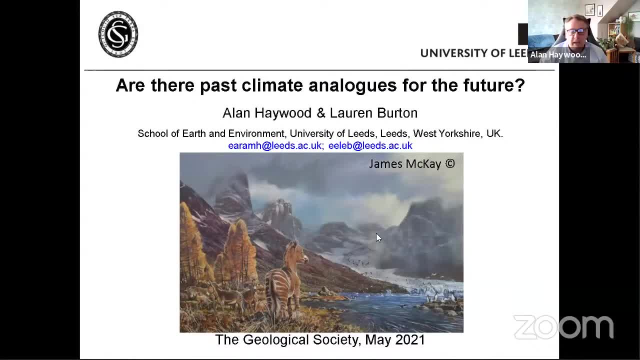 And so I have a particular question that I'm addressing today, which is: are there past climate analogues for the future? And before I go into it, I would just like to point out the contribution of my PhD student to this talk, Lauren Burton. 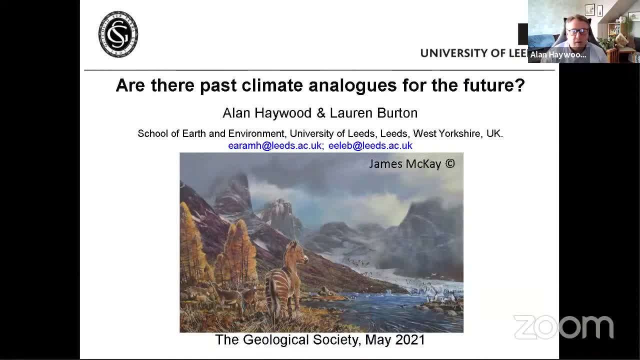 Lauren is a first year PhD student who's already really doing very well and producing a lot of great science, And as I was putting this talk together, it became more obvious that I needed more of her input, So I'm sure you'll be hearing more from Lauren in the future. 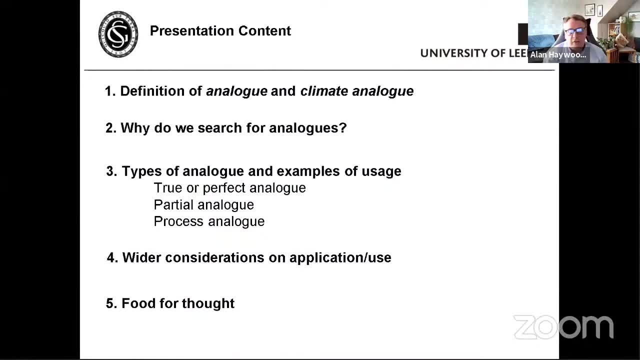 So I'm sure you'll be hearing more from Lauren in the future, So I think it's going to cover what I'm going to be presenting today. So I want to start from the basics and talk about the definition of analog and what we mean by climate analog. 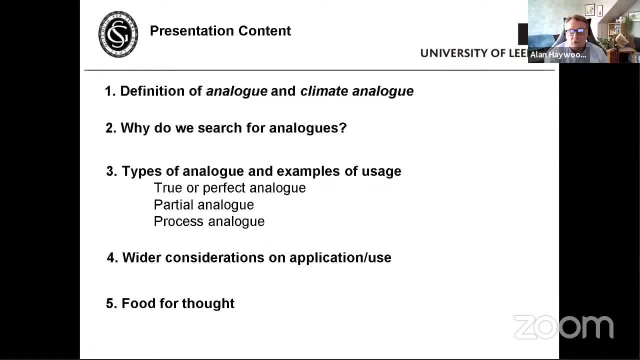 Then I'd like to go on and talk about why do we search for analogs, as scientists, as geologists, as paleoclimatologists. Then go on and talk about the types of analog that we can find and provide some examples of their usage. and specifically in this context, i want to touch upon 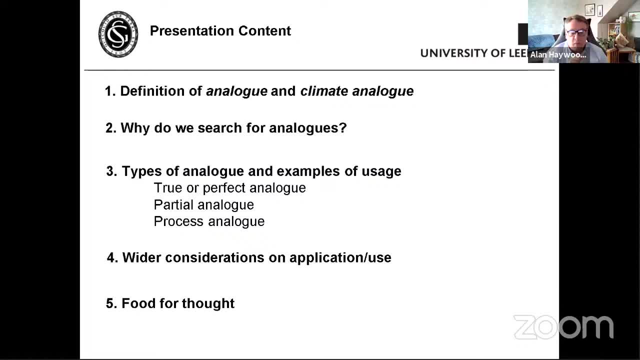 three different types of analog and the question about whether or not there is a true or perfect analog in the geological record for what's going on right now. um, the partial analog or the process analog. so we're going to take each one of those in turn with with some examples, and then i'd like 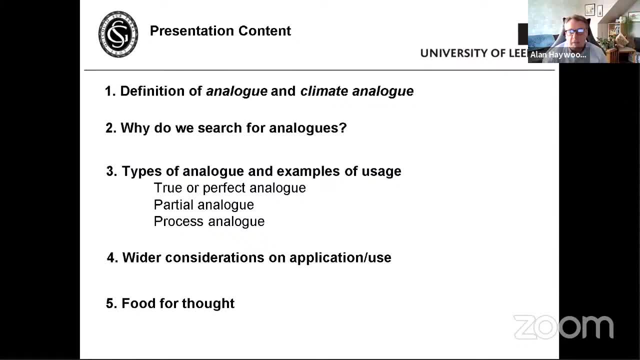 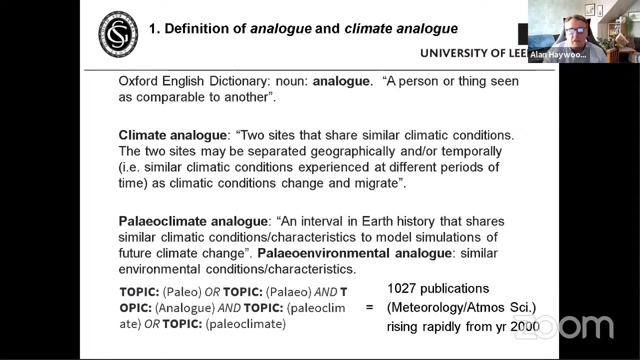 to go on and talk about some wider considerations on application and use of analogs and then kind of try to tie things up at the end with some comments and some things which i will hope will provide some food for for further thought. so let's start off with the definition of analog and climate. 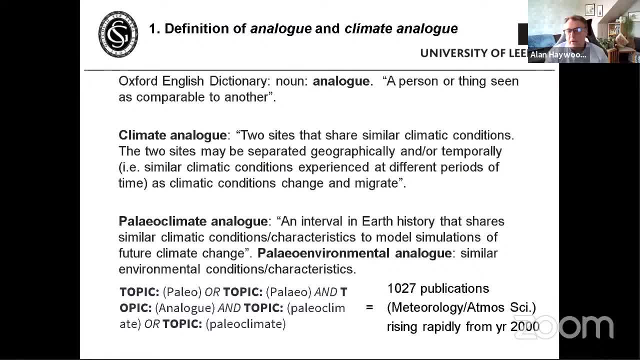 analog. so the oxford english dictionary, the mount analog is a personal thing seen as comparable to another climate analog and has been described in the literature something along the lines of this: two sites that share a similar climatic conditions. the two sites may be separated geographically and or temporarily. 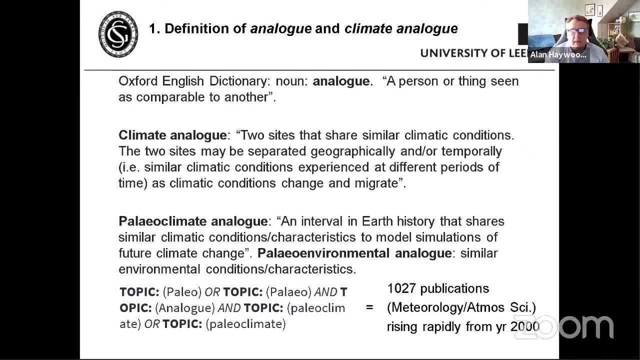 ie similar, similar climatic conditions experience at different periods of time as climate conditions change and migrate. so how do we transfer that in the context of paleoclimate- and i'm doing, i'm trying to do that here- essentially an interval in earth history that shares similar climatic conditions and migrates to different climatic conditions and migrates to? 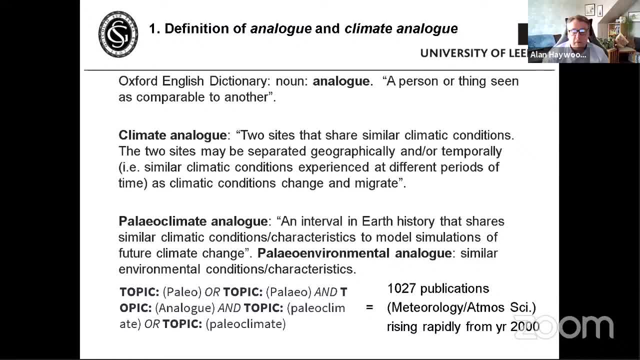 similar climate conditions and characteristics to model simulations of future climate change and, of course, we can extend that also to a paleo environmental outlook. similar environmental conditions and characteristics, i mean- and this is obviously a a key area, a very active area of research. one of the things i like to do to try to demonstrate this is go and have a look at the 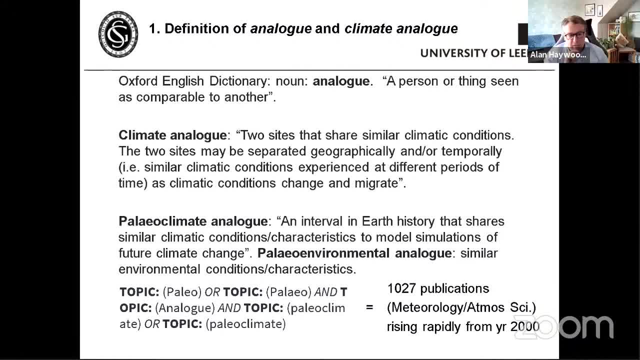 published articles that are out there and do a kind of a meta analysis of how much is coming out over time. so i did quite a conservative search here, looking at the different topics- paleo, analog or paleoclimate- and restricting that just to looking at in the areas of meteorology and atmospheric science, and i found over a thousand. 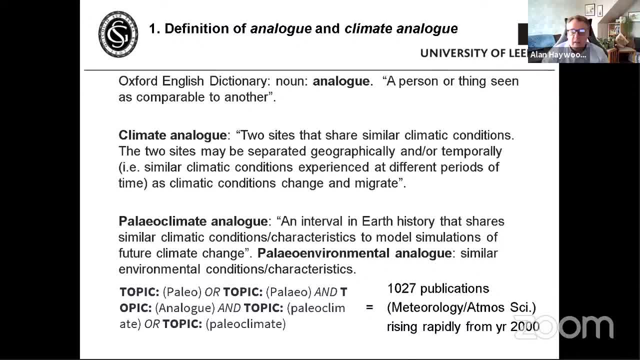 publications which have those keywords, which from the year 2000, and it's been rising rapidly every year since the year 2000.. if i, if i, then extend that to the geosciences, then we end up with something like 20, 23 000 articles. so clearly this is a very active and ongoing. 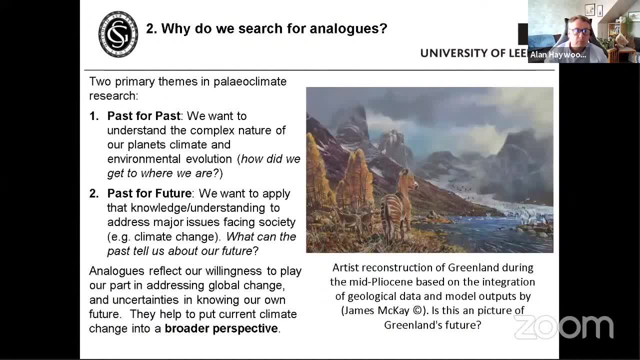 question and area of research. so why do we search for analogs? well, i think the best way to try to answer that is to touch base and reflect upon probably the two primary themes that we have in paleoclimate research, the first being the kind of past for past approach. so we want to understand the complex nature of 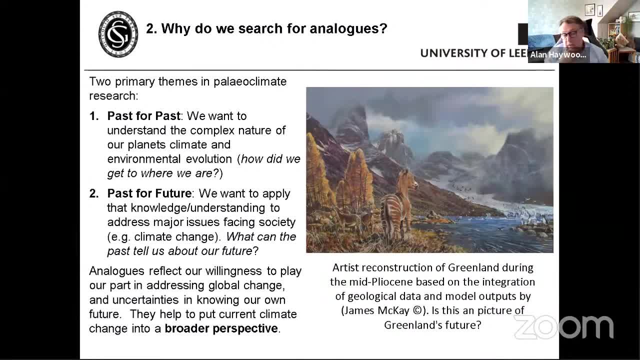 our planet's climate and environment, environmental evolution. so how did we get to where we are, where we are today? there's a another primary theme- uh, past for future, and this really focuses around the fact that we want to apply the knowledge about the understanding of the past climate system to try to address major science issues facing society. so climate change. 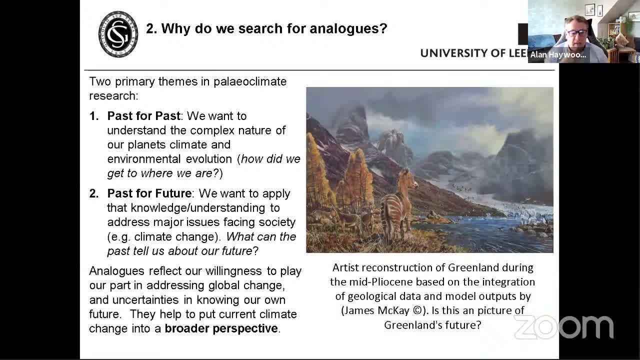 so what can the past tell us about our future? so analogs really reflect our willingness to play our part in addressing global change and the uncertainties of knowing our future. but, critically, they also help put the current climate change into a broader geological perspective, and i think that's something. 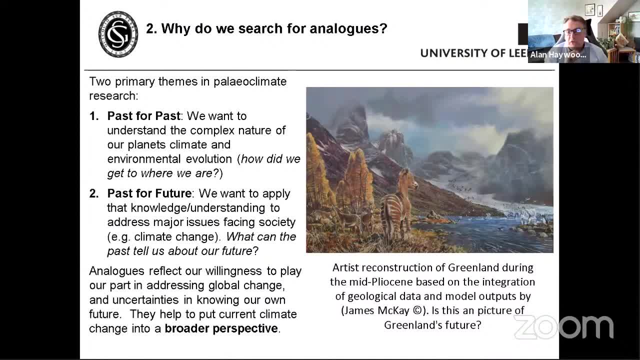 which is incredibly useful. so on the right here i'm showing you a an outcome of a collaboration that we had at leeds with an artist, james mckay, and we at the leeds group we do a lot of work on pliocene research- and we decided: wouldn't it be great if we could try to kind of synthesize all? 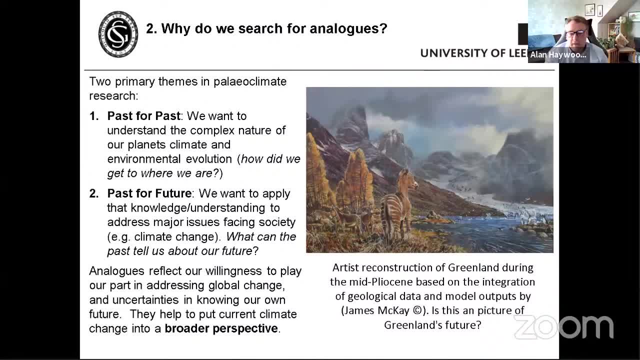 of the information that we had from the paleontological record and from the geological record, from climate models and from eye sheet modeling that's been done for the pliocene, to try to come up with a composite picture of what we thought the environment was like. 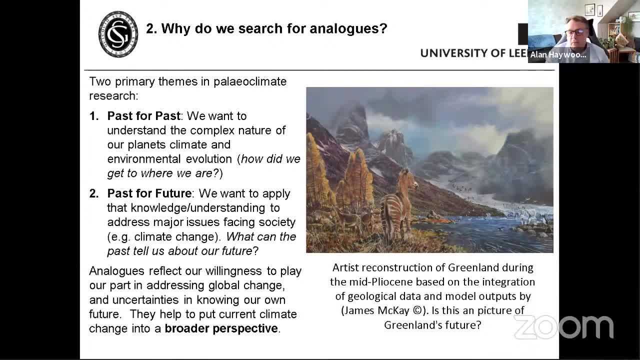 on greenland during the mid-pliocene, so around about three million million years ago. there's a way of looking at climate change and the environment and the environment in general to try to convey that information about how much the environment and climate was has changed, how. 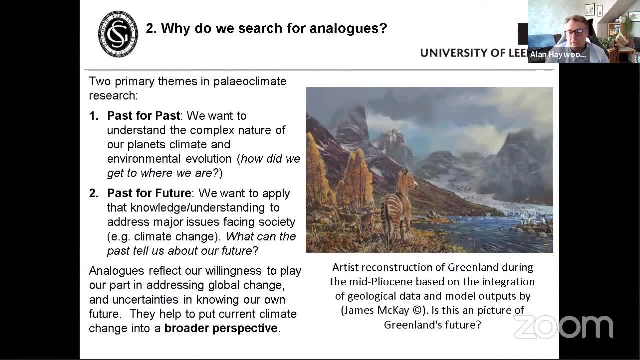 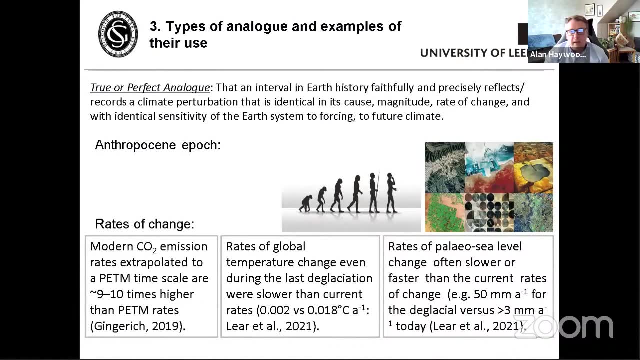 much. it was different back then to a broader audience of people, and so the obvious question that comes out when you look at something like this is: is this a picture which looks something like greenland's future? so let's talk about the types of analog and talk about some examples of 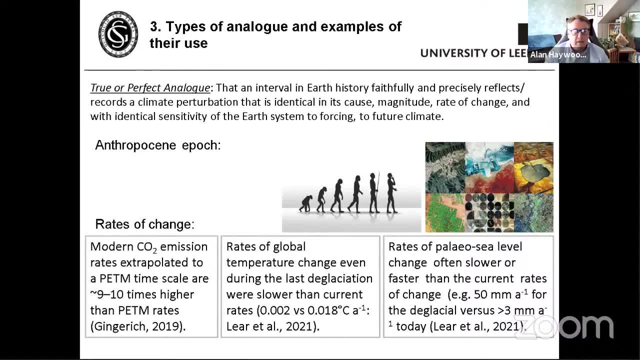 their use. so let's touch upon the first one, the concept of a true or perfect analog. so what i mean there really is that there's an interval in earth, earth history, which faithfully and precisely reflects, records, a climate perturbation that's identical in its cause, magnitude, rate of change. 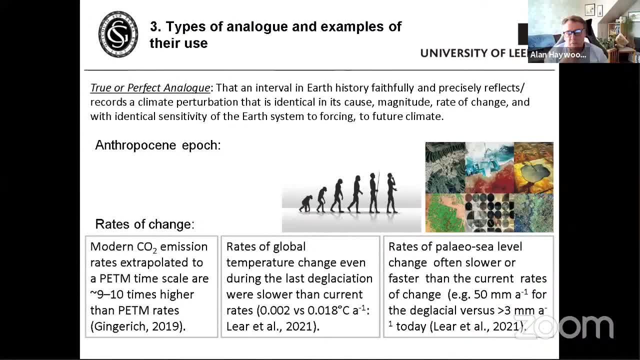 and with identical at a time where there's identical sensitivity of the earth system to forcing to a future climate state, and i think one of the things that we can do is that we can understand that that's an extremely difficult question and an extremely unlikely outcome, and there are a number of reasons. 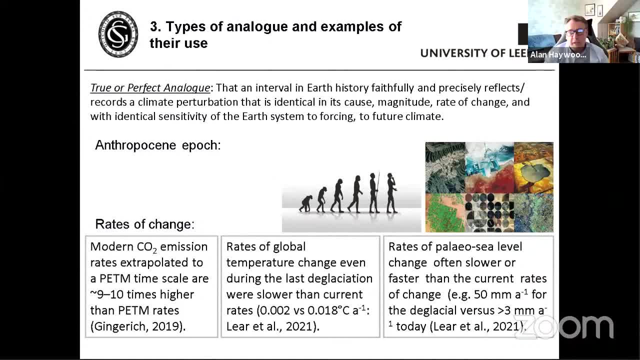 for that. so the first thing is that we are living, as some say, we are living in the anthropocene epoch. so, in terms of the climate changes that have occurred in the past, of course they they occurred in the absence of us, in our species. now we have an absolutely fundamental 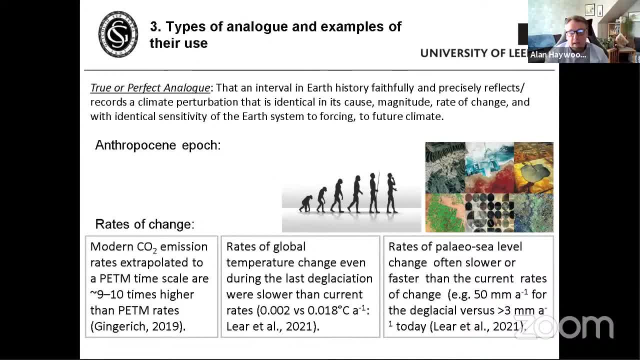 role in the changes which are going on right now in our climate system across across the world. but i think the key thing is that it's not just the climate that we're forcing directly through greenhouse gas emissions. we're having a fundamental effect on our planet as a whole, which the whole concept of the anthropocene tries to. 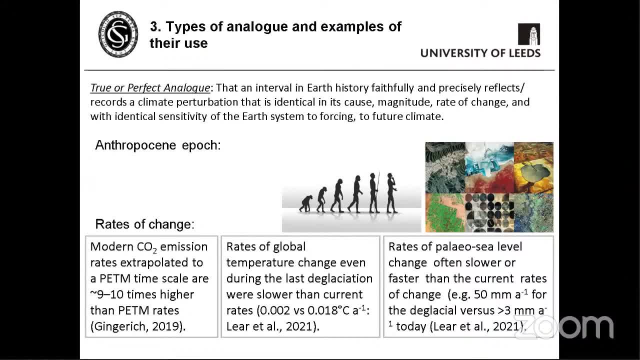 highlight or codify, exemplify, if you like, and i think, the thing that we also have to appreciate as the time goes on into the future, we are hardly going to be passive bystanders in what the outcome finally is. so, merely from that point, the fact that we are here and we have had a role in this, 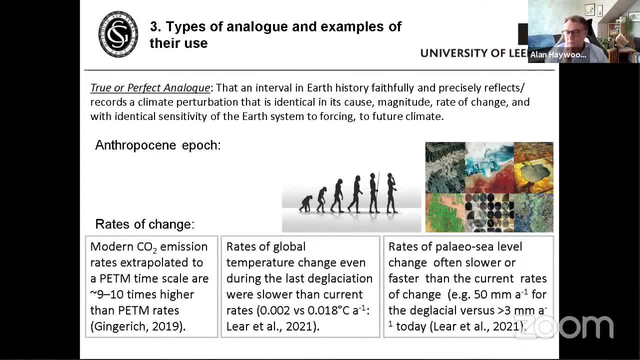 makes it very unlikely to be able to find something which is exactly equivalent- uh, which will be exactly equivalent- in the context of the past. even so, if we just go beyond that just a moment to think about some of the other reasons- and it's kind of nicely laid out in the, in the 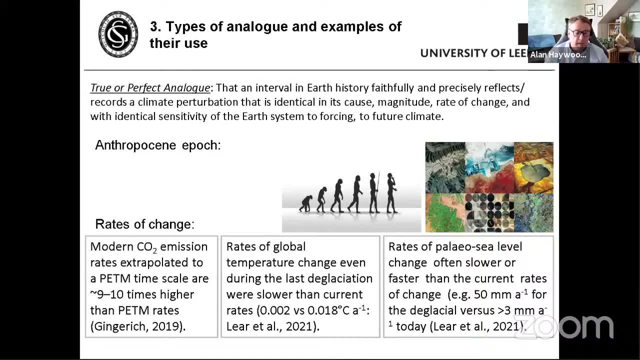 journal's um uh publication in the lee rat, information publication here. but if we think, think about some of the rates of change. so modern co2 emission rates extrapolated to a ptm time scale are something like nine to ten times higher than the p10 rates. so it's actually 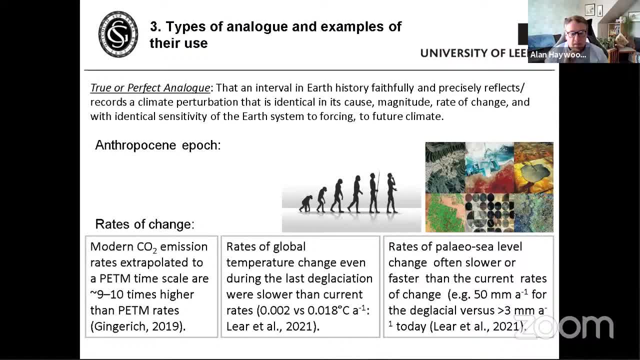 requires some considerable thought to relate the time scales of which things have happened into the past, to compare them to the rates in which things are happening now. so we know that there's a difference in the rate of co2 emission, even for something like the ptm, which was pretty. 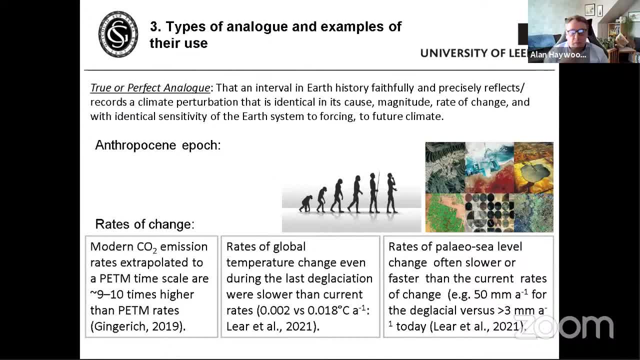 rapid by geological standards. um, if we think about the rate of global temperature change, even for something like the last deglaciation- and we saw very rapid uh changes- they're slower. they were slower than the current rates of change by some considerable margin. but then we can look. 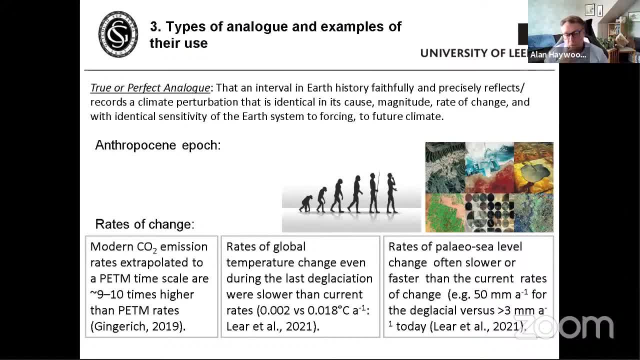 at other aspects of the earth system- response to forcing into greenhouse gas, forcing like, like sea level- and we can actually find other examples in the geological past where the rates of change may well be considerably faster than we're currently observing. so there is an issue associated with the rates of change and, of course, as other speakers have highlighted in their talks, 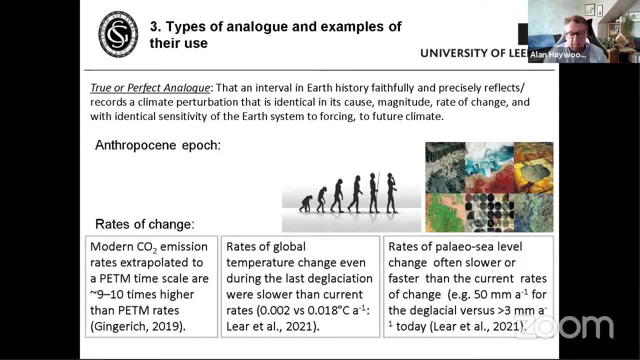 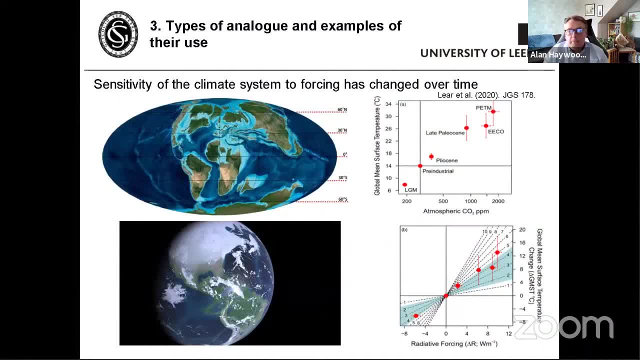 the rate of change is critical in correctly assessing the impact and the ability of our planet to deal with what's happening. and the other thing is obviously a lot has changed over geological time and the further that you go back into the past, the higher the potential is. 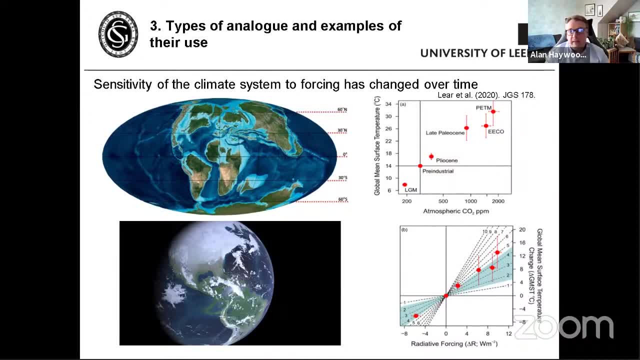 for those changes to become larger and larger, and this has an impact even on thinking about the degree to which the state, the basic state of the climate system and the sensitivity of the climate system to forcing and to greenhouse gas. forcing has, um has evolved over time. so i'm showing you a picture here of a cretaceous- uh paleo geography- animal and 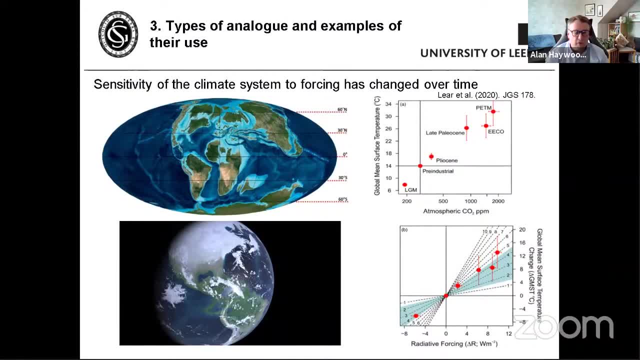 underneath that, showing you a a reconstruction of north of the northern hemisphere, north america, during the last glaciation, and so clearly you know these differences that we that we've had in the past in the environmental conditions. the base state the environmental condition is is rather large, and anna did a great job yesterday of articulating how the, the point at which you 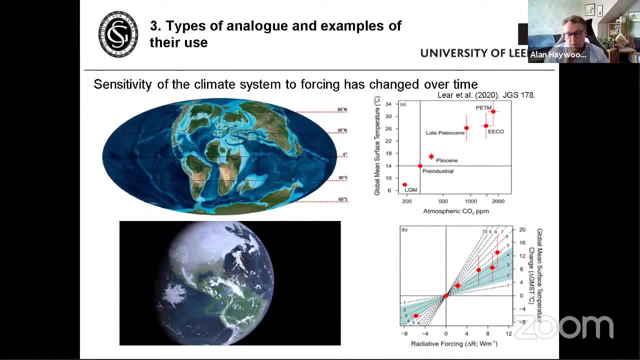 start from can have an impact on how the climate responds to a uh, to a greenhouse gas, changing a radiated uh forcing. so the fact that the earth has changed its probably sensitivity over time is is important in the context of considering the idea of there being a perfect analog in the geological past. so if we just put that aside for 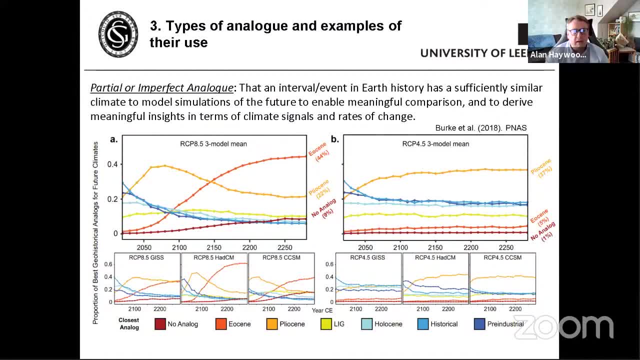 a moment and think: well, we, we, we can't find a perfect analog, um are there a partial or imperfect analogs that we can look at? and so i'm defining that here as an interval or event in earth history that has a sufficiently similar climate to model simulations of the future to enable a 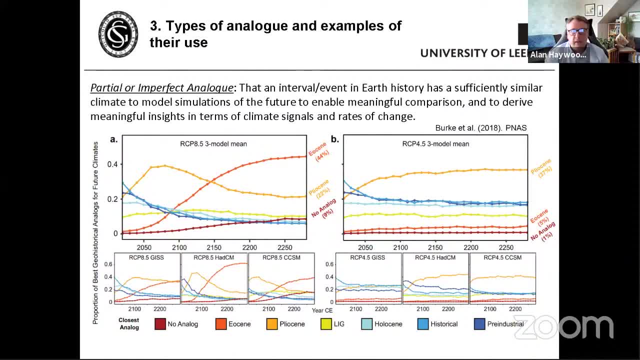 meaningful comparison and to derive meaningful insights in terms of climate signals as well as rates of change. and there has been some work, um, there's been a lot of work which which has looked at that, and i'm showing you one particular example here, by burke et al in 2018, published in proceedings. 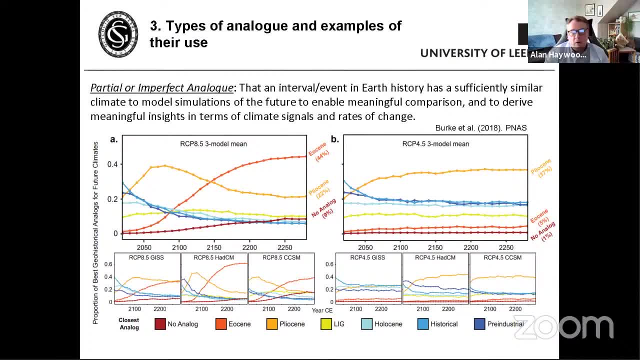 of the national academy of sciences. so what happened here was um the. the authors took different simulations produced by three different climate models: the gist model, the hadley center model, version three, and and the ncar model, ccsm, um for a different, um, geohistorical potential, geohistorical analogs. so 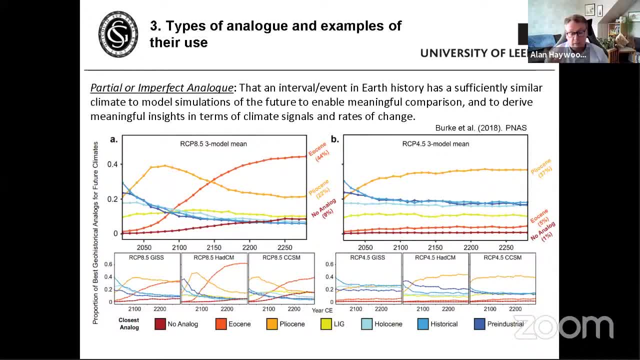 that would include the, the eocene, the pliocene, the last interglacial or the league, the holocene, the historical period as well as a pre-industrial baseline, and then actually performed a statistical comparison, looking at the similarity between, uh, those model simulations for those different geohistorical analogs, um compared to different scenarios for future, for future. 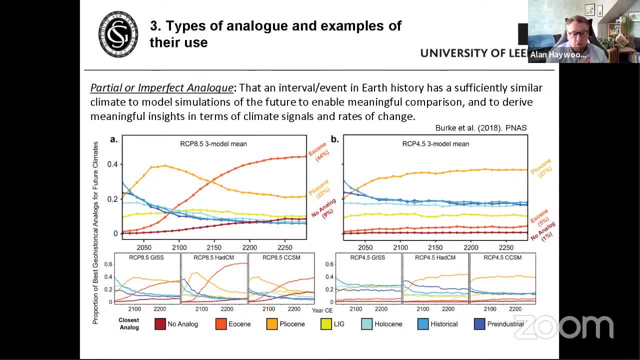 climate change and i'm showing you here to here two of those examples. so the concentration pathway: 8.5 as well as 4.5, and so this is essentially showing you the top figures are showing you the kind of three multi-model mean outcomes for that and the degree of similarity that we see between 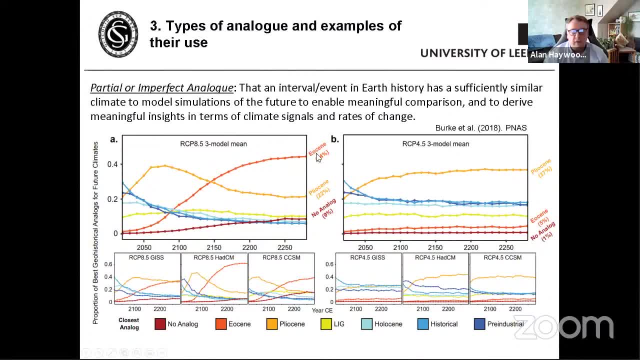 the future climate scenarios 8.5 and 4.5 and the different geohistorical- uh potential analogs that we're looking at here, and so we can see that actually, the degree of fit is partly dependent upon which rcp scenario we're actually going to follow by the time you get out to 20 to 22. 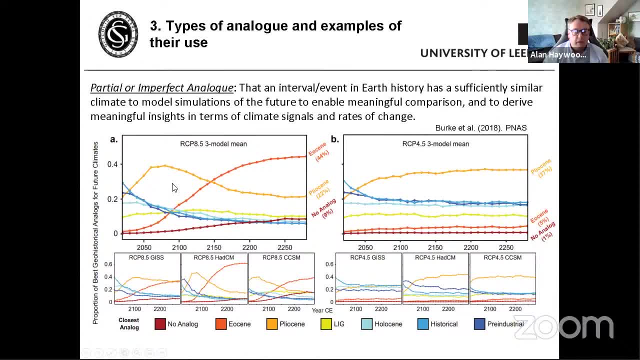 250, 2300 um, but you can see so, for example, for icp, rcp 4.5. but in terms of the degree of fit, then the pliocene, rapidly, into the near future, becomes the one which has the greatest similarity. if we follow rcp, something more like rcp 8.5, then the pliocene starts off by being the most analogous. 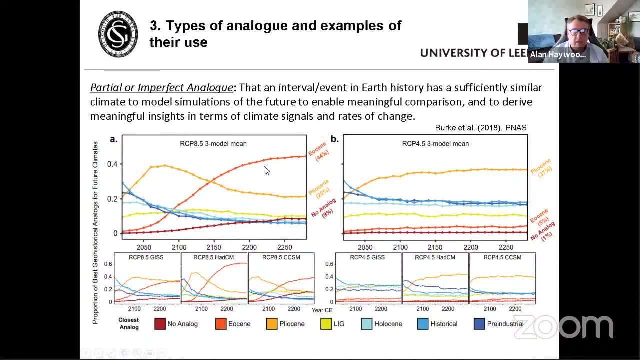 but then by around 2150 or so, gets overtaken by the ear scene. now, obviously, um, there are uh differences from model to model to model in that, but overall the patterns are actually quite, actually quite quite similar. so we can kind of see that we can actually relate patterns of change that we're able to simulate or reconstruct into the past. 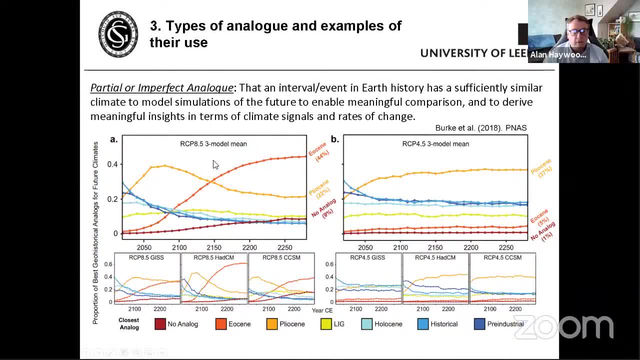 into things which we anticipate as possibilities, uh, for the, for the future. but i mean, one thing i suppose i would note is, even in the context of rcp 4.5 and the pliocene, we're getting up to about seven percent, uh, similar similarity. perhaps that is sufficient to say there's a partial out, a good. 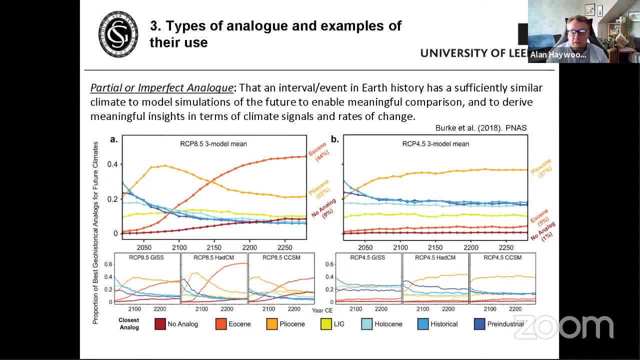 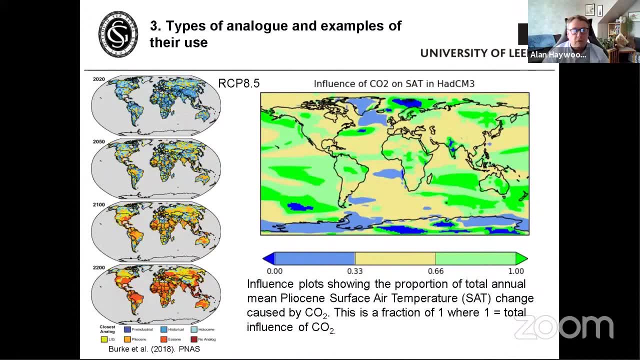 partial analog, um, but um, no one's actually defined the threshold at which we can actually say that. i'm going to come back to that in a little while- um, so you can look at this in another way if you like. so this figure that i showed you here previously is now being represented. uh, here. 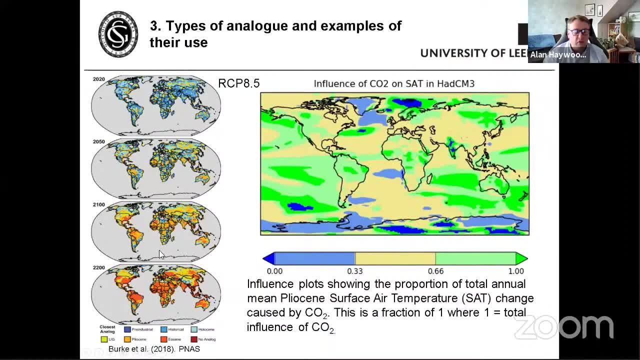 on the left for rcp 8.5, but it's showing you the spatial evolution of that similarity over over the world. so we start off at 2020 to 2050 and go down to uh 20, 2000, uh 2200, so you. 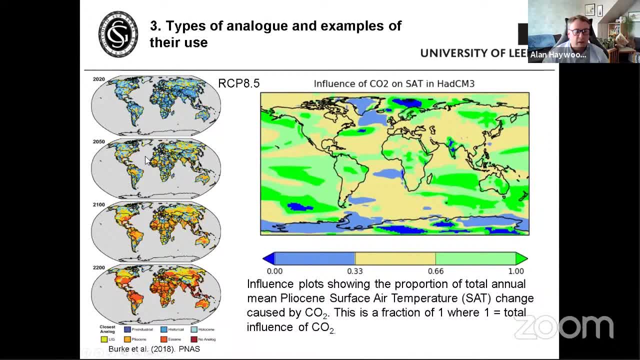 can see lots of blue. as we continue to go forward in time then we start to see that the more and more parts of the world become more pliocene-like and more eocene-like. but i think one of the other things we also see here is that we move into scenarios into the future where we get an 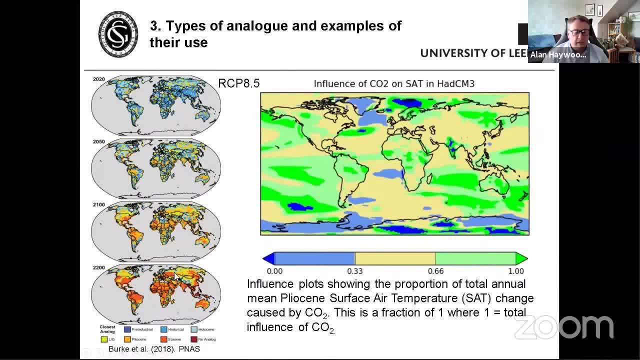 increasing, um, increasing number of increasing area of the world which is really doesn't have a, doesn't have a geo geological, at least in terms of the different ones that we sample here, which is quite, uh, breathtaking in that sense. but, as i said before, there are different things which contribute to climate changes of the past, and i think one of 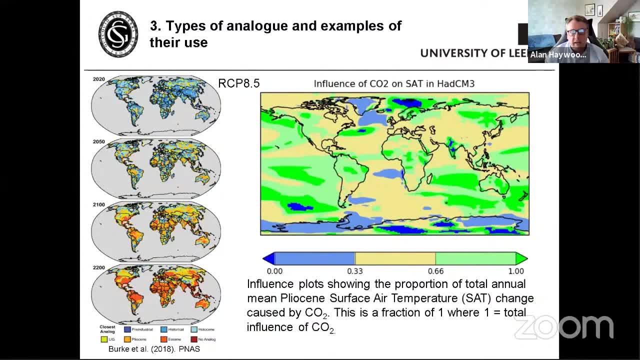 the things which is quite useful for us to try to understand is the is the overall influence of carbon dioxide on patterns of climate change that we have seen in the past, and this is certainly one of the things that we're trying to address. uh, using climate models which use, which do a whole. 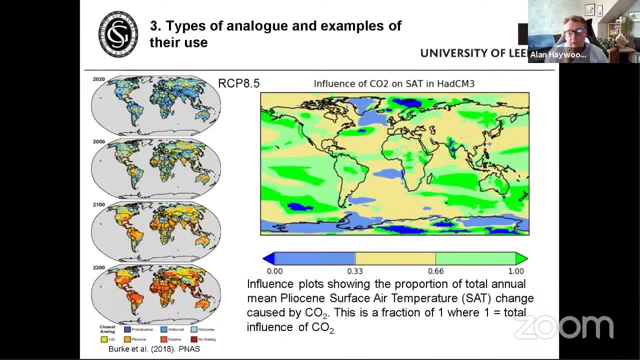 series of different experiments making incremental changes in the boundary conditions within those models, so that you can actually identify the contribution from individual changes that you make to the model. and i'm showing you here an example: uh, for the, for the pliocene, this is an influence map and showing you, for our own model, had cm3 how important, what sort of level of. 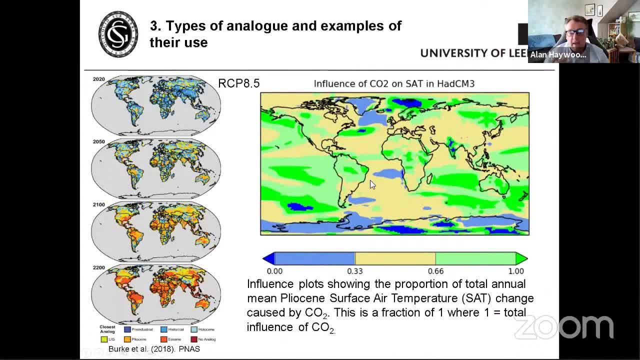 the forcing of carbon dioxide had on the the amount of temperature change that the model simulates for this period. so the pliocene minus the pre, minus the pre-industrial, and i think one of the things you can see uh is that over wide swathes of the world, then uh, co2 um is how the 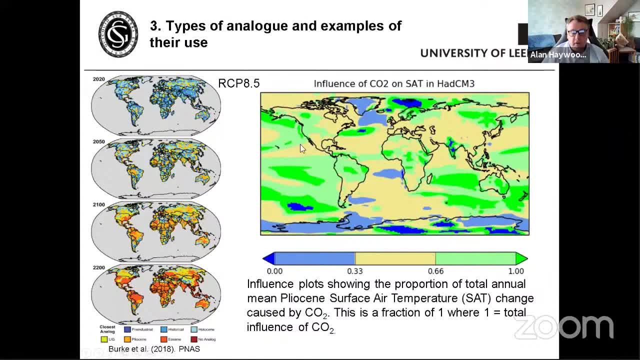 co2 forcing is having a considerable to dominant effect on the pattern of change that we see at this particular time and that really backs up, i think, one of the things that um paul valdez was showing in his presentation yesterday, when he was showing that for multiple 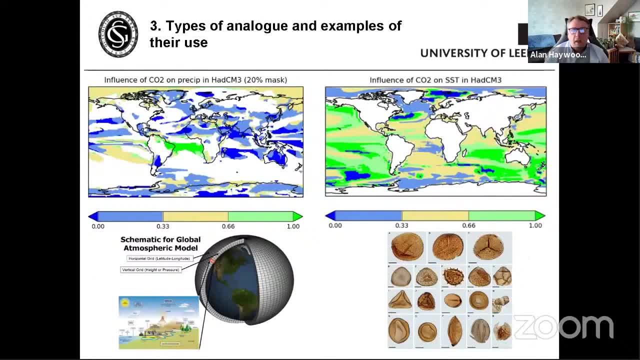 for multiple time series, and but one of the things which is clear to and important to remember is that climate is not just temperature. we, we, we talk about temperature a lot in the context of the paleo, because it's one of the key things that we can try to reconstruct geologically. 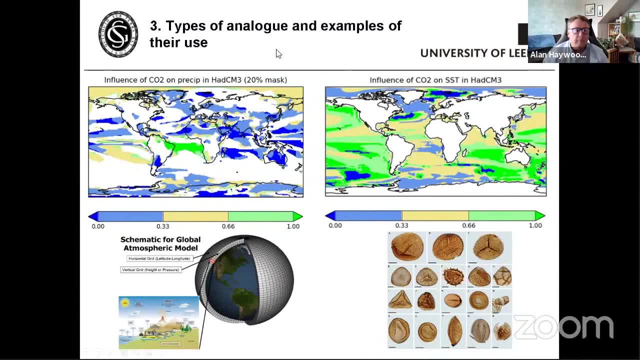 um, but but temperature is only one aspect of climate, and so i'm showing you here, on the top left, another example of the figure i just showed you, but this time for precipitation- uh, not for, not for temperature change, and here we have quite a different uh, here we have quite a different outcome. so again there, 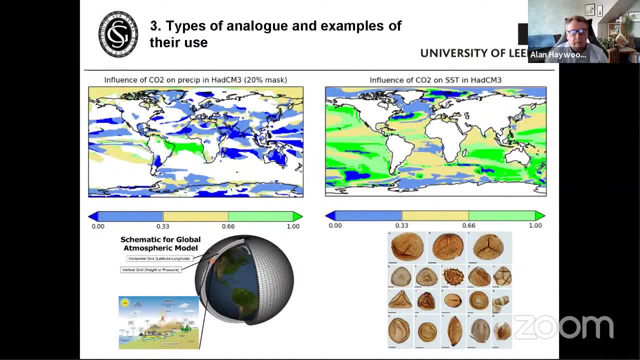 are areas of the world in the context of the pliocene, where the where the co2 forcing is very important in determining the pattern and the magnitude of precipitation change, and but actually there are large areas of the world where where the response of co2 in terms of 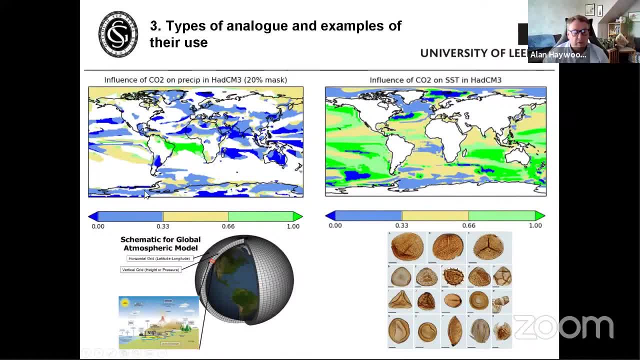 the precipitation change we see at this point in earth's history is relatively small, and so what that's actually suggesting here is that the other boundary condition changes that we've made in the model- principally changes to orography and to ice sheets into vegetation- is having more of a more of a dominant effect in in determining what happens. 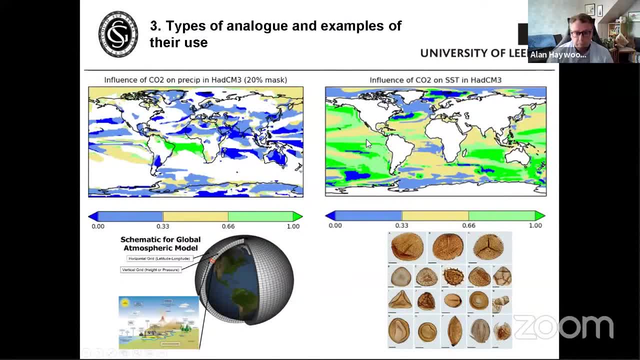 to precipitation uh than the co2 forcing. i'm showing you something here which is similar in the context of sea surface temperatures, and here this is more of a similar pattern to the, to the pattern and the influence of pliocene. so we're able to do this using models and, of course, we have access to different. 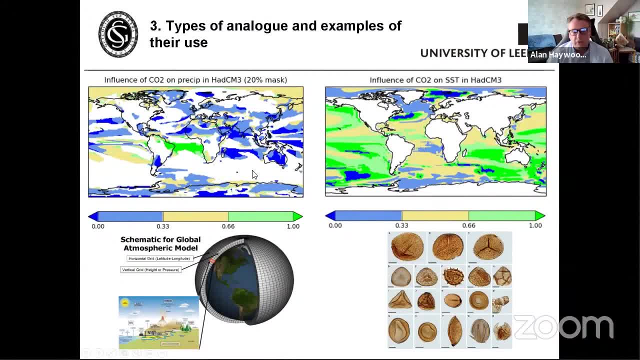 model simulations which have performed the same experiments, so we can also assess how dependent these kind of results are based on the model that you use. and more challenging is to try to do this sort of analysis from the point of view of proxy data alone, although if there's one thing that i've learned is you should never 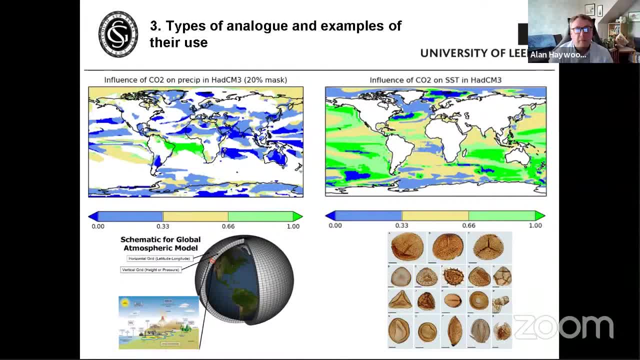 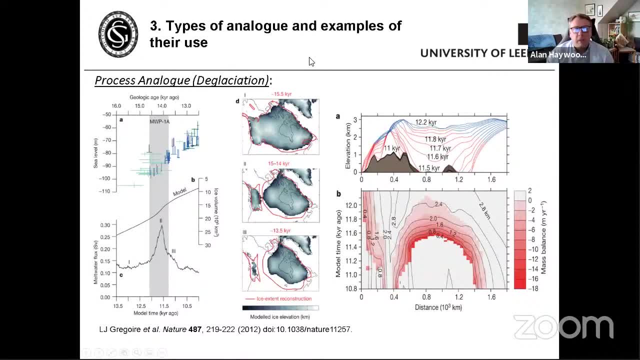 underestimate the innovative capacity of geologists and paleo environmental scientists. so let's, let's move on and think um about um other types of analog examples. so, um, i want to just talk about here, uh, the deglaciation, and i'm moving away from the partial analog and really moving now into the kind of process, uh, analog space. so we're not 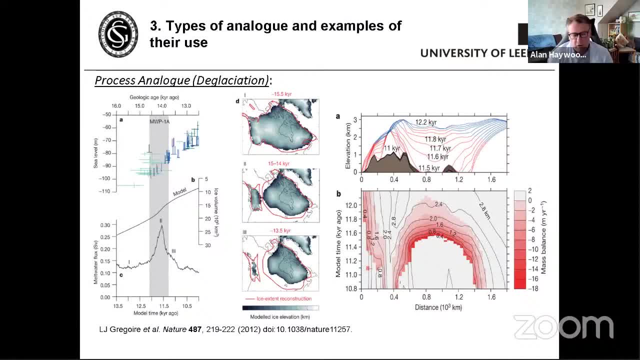 trying here to sort of directly relate patterns of temperature and environmental changes past, in the future. we're trying to actually understand, uh, the fundamental processes which are operating in the future, which may be, uh, which were key and may be relevant in the context of the future, uh. so we're going to take three examples here, going progressively further back. 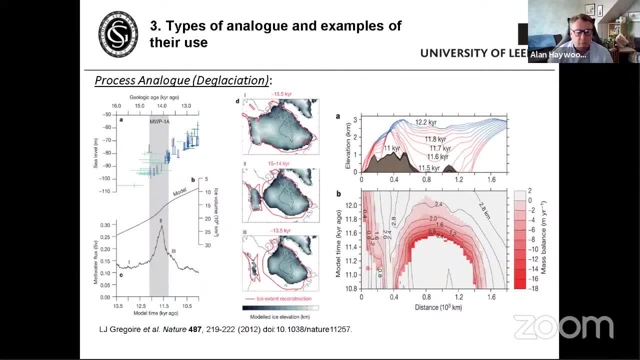 in time. so this is the first one, uh, the deglacial period. so we're now talking about a time where, uh, insulation, changes in insulation forcing and co2 forcing over time had really an absolutely profound effect uh on um, on the global climate and on the amount on the. 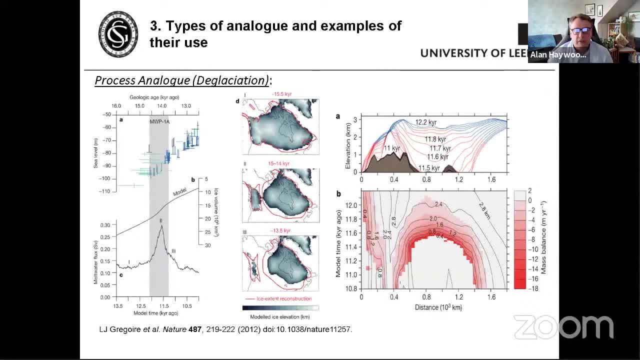 amount of ice which was in the system at this time, particularly in the northern hemisphere, and the growth and decay of the major ice sheets, including north america. i'm showing you here a study by lauren bragoire et al which was published back in in 2012. but essentially what this study, one of the 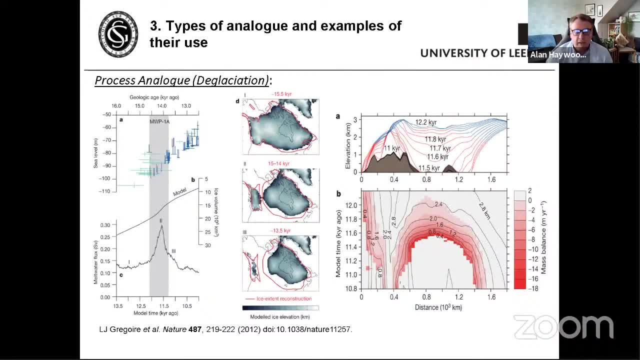 key outcomes of this study was was the fact that we can kind of understand the, the patterns that we change, that we see going through the, the deep, the deglaciation, by understanding the complexity associated with um, with ice sheet morphology, geomorphology, the underlying, the underlying topography at that time, the interrelationship between that and the. 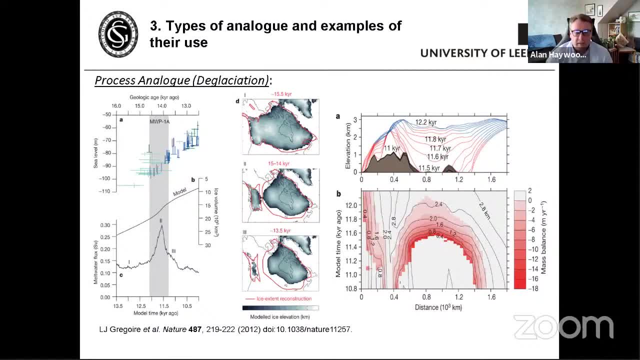 four things that were going on at that time and how we can see sudden accelerations in ice sheet loss and also then sea level rise because of surface mass balance feedbacks and mechanisms called something like, which were referred to as the saddle collapse. so suddenly, the fact that you had an ice sheet which was made up of multiple ice caps which then decayed, and 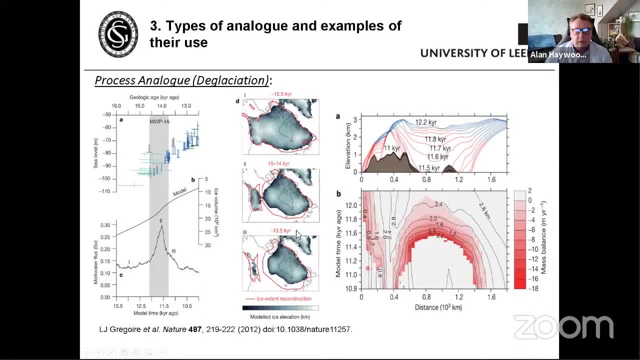 separated, with the resulting acceleration of ice loss and therefore sea level rise, and so we were able to then think about the context of which mechanisms like that may relate and may be relevant in the context of the future. similarly, if we go back and talk about the pliocene, one of 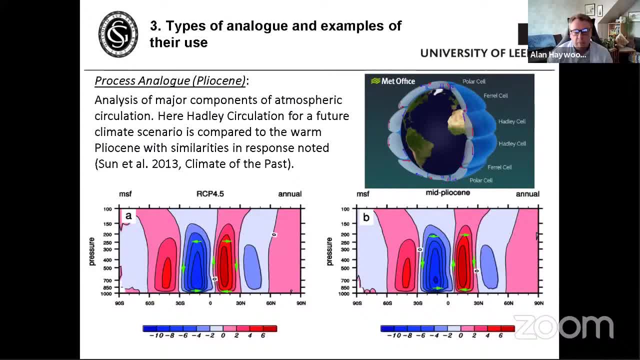 the key things we want to know and are focused on is actually what happens to atmospheric circulation at this time. so i'm showing you here a study by sanitel 2013, which did an analysis of the major components of atmospheric circulation, and the thing that they were pointing out was that they were comparing the pliocene simulations of 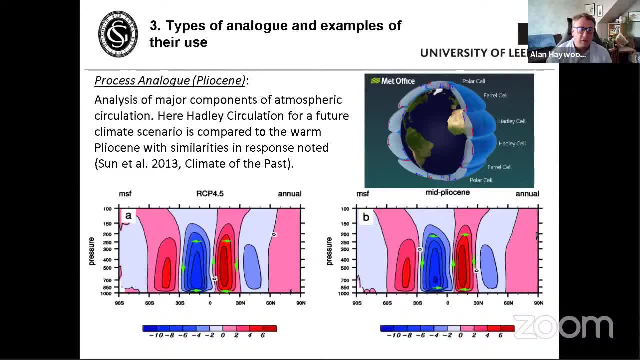 the hadley circulation to also a specific scenario for climate change into into the future. and you don't have to be an expert in analyzing atmospheric circulation plots to be able to see the strong similarity between these two plots down here at the bottom of this figure. so so clearly there are. there are some fundamental things. 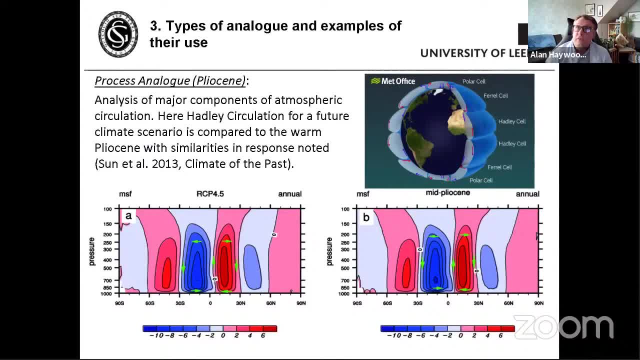 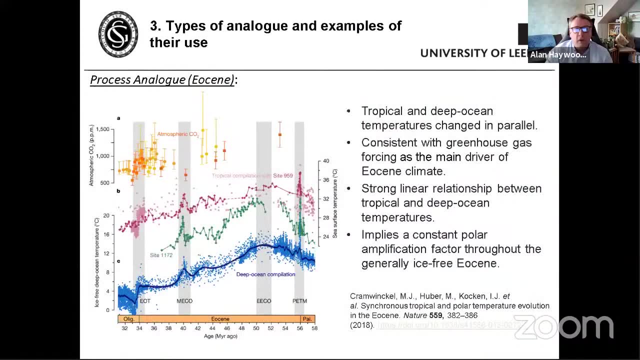 that we can learn about the nature in which first order effects, like changes in tropical to high latitude temperature gradients, the way that influences large-scale atmospheric circulation in the past and also into the future. the last one i want to talk about is in the context of the ear scene, and this was a paper that came out back in 2018.. 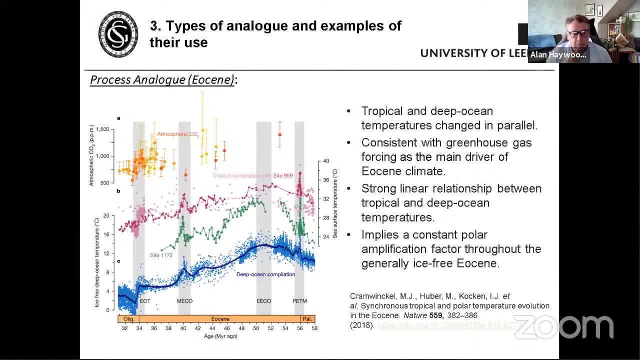 which did, i think, a really interesting job of compiling different atmospheric co2 records for this particular time and coming up with a compilation of tropical sea surface temperatures as well as deep ocean temperatures, and one of the things that they found from this was that tropical and deep ocean temperatures appeared to change in parallel. they made the argument here that this 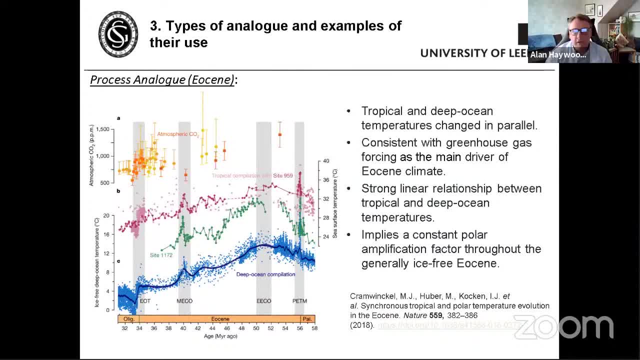 is consistent with greenhouse gas forcing being a primary driver for eoc climate change. but there was a strong linear relationship between the tropical and deep ocean temperatures and the interesting thing about this was that it sort of implied a constant polar amplification factor throughout a generally ice-free ear scene. so certainly, even though things in back in the year seemed, 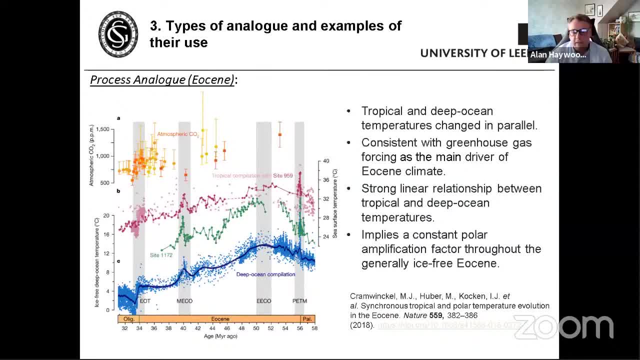 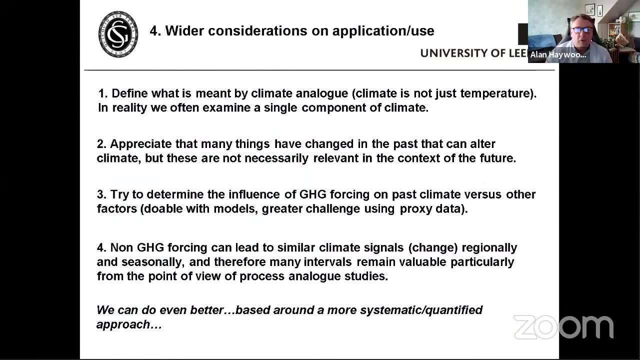 substantially different compared to they are today and that we would expect in the near future, there may be still fundamental. there are still fundamental things about the way that the system operates which can be translatable from the geological past into the future. so let's just move on in terms of thinking about some of the wider consider considerations on. 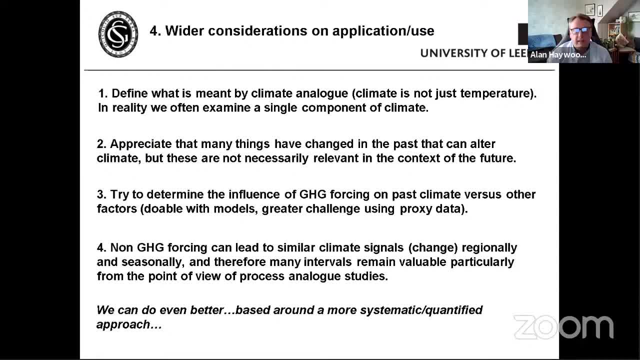 application and use, and i think the the key thing. some of the key things that we need to consider are outlined here. so i think, when we talk about, this is important what that we, what that we define, what we mean by climate analog, if we're going, if we're going to do. 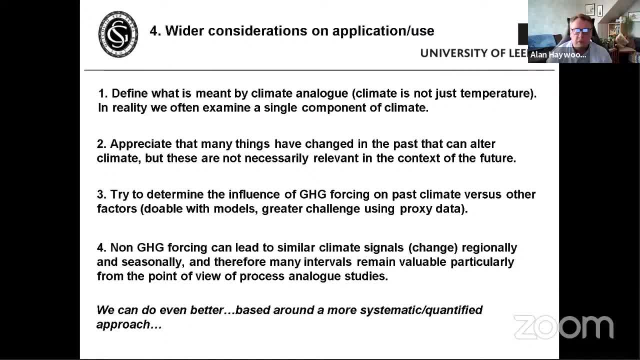 more of this, and i'm sure we will. it's important for us to be explicit in those things that we want to understand in this, and we're going to be much more explicit about what we actually mean, and i think the key thing is that climate is not just temperature. so 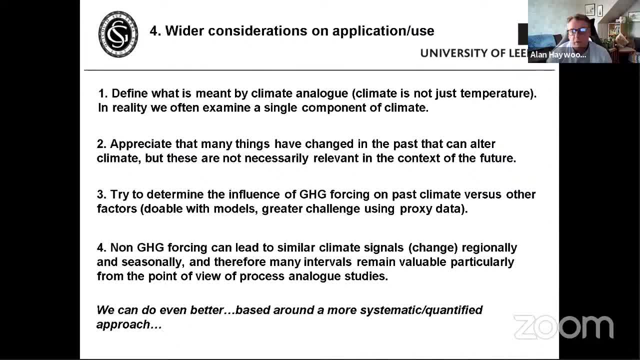 we have to be more, more specific in how we refer to these things. so, in reality, we often examine a single component of climate. are we talking about analog of temperature and analog of precipitation on our climate? and if it's climate, it reply, it requires us to think a bit more broadly. 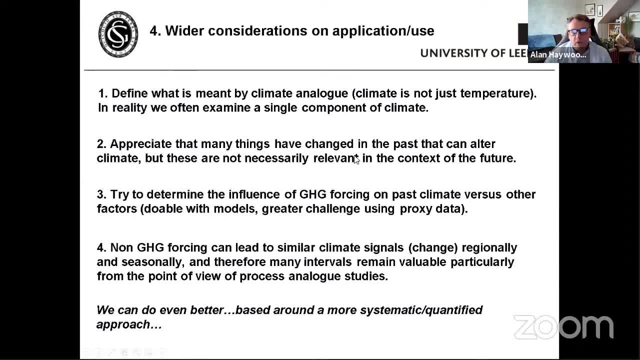 and we certainly appreciate that many things have changed in the past that can alter climate. but these context of the future and we can do the kind of studies that i've showed you to try to get an idea about the degree to which greenhouse gas forcing is influencing specific and critical regional 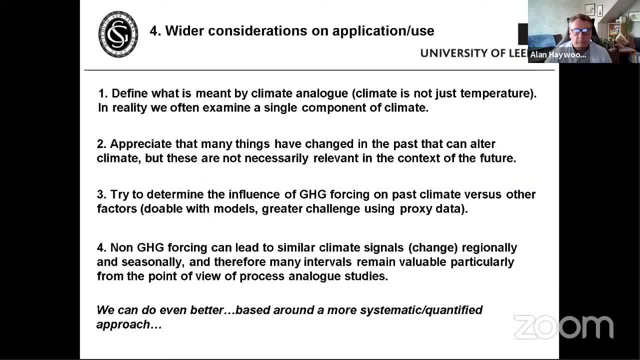 changes in climate, any violence in the past, so, and we can do that with models and, of course, but it's a greater challenge using proxy data. it's a mistake just to focus on intervals of the past that had greenhouse gas forcing related as being uh linked to the changes that were going. 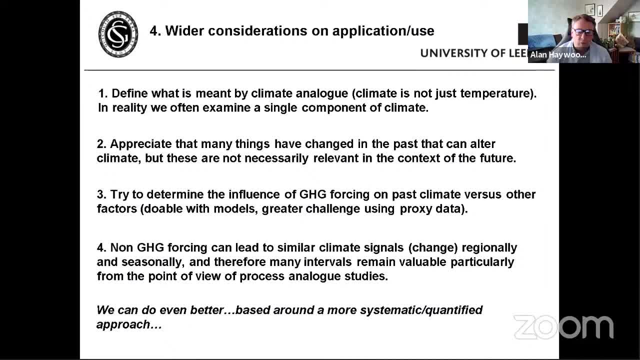 on at the time. there are other periods of time which are, which were forced by different types of changes, so insulation, for example, um, which was still- uh, we're still led to regional and seasonal changes which might be similar to what we expect for the future, so that we can still learn. 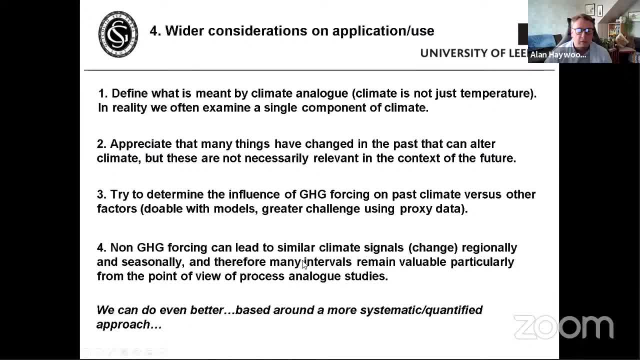 from these many intervals and they remain, uh, valuable, particularly from the point of view, i think, of process animal studies. so we can, we've done a lot, we can do better and i i think what we can do, moving forward, is to continue the pattern of development that we're already doing around more systematic. 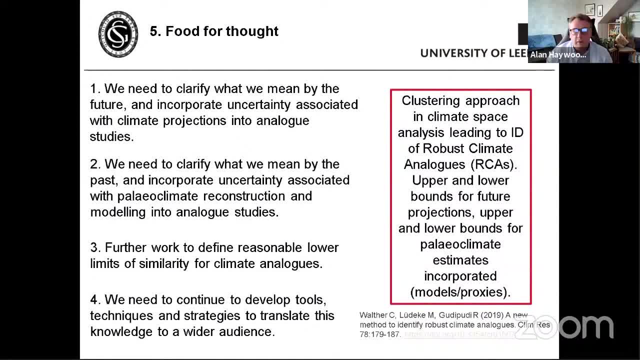 and quantified approach. so i'm just going to finish off now by talking by talking a little bit about food, food before. so one thing i say in the context of formalized analog studies, i think that one thing we need to do is to clarify what we mean by the future. so, as you can see, 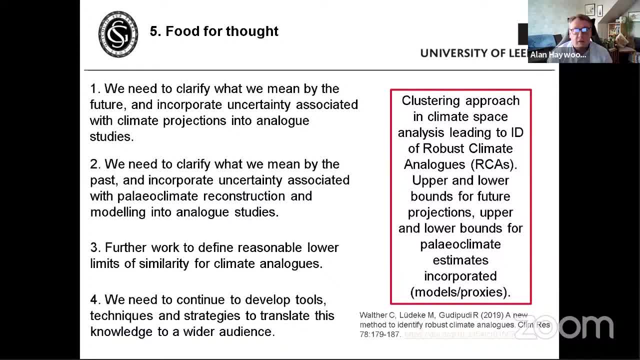 that was done in in the context of the burka fell study, using different scenarios. so when we say future climate, what do we actually mean? do we mean 20200? do we mean 23, 2, 300? what scenarios forcing are we going to use um along those different pathways? so that needs to be considered. 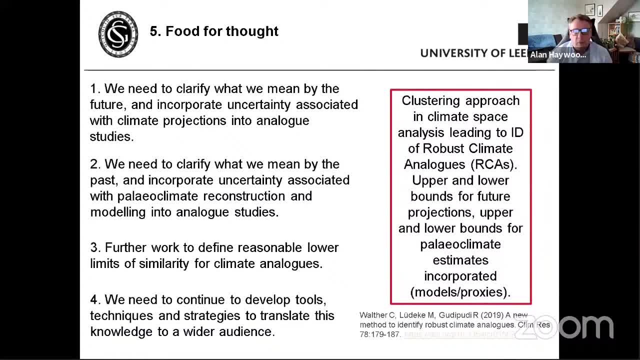 quite carefully. um, we also need to clarify what we mean by the past um and and incorporate uncertainty associated with palehguru or model Isa fox response and response later. that requires our, our analysis of the material effects that we call opportunities to stretch between such contexts opolitically and the converse. diversifying, healthier way of thinking about a range all and so what? children don't Adapted to music in evidence, not for courses. warmляagh was a large cause to think about a number of these users, but i'm tired so we have to. 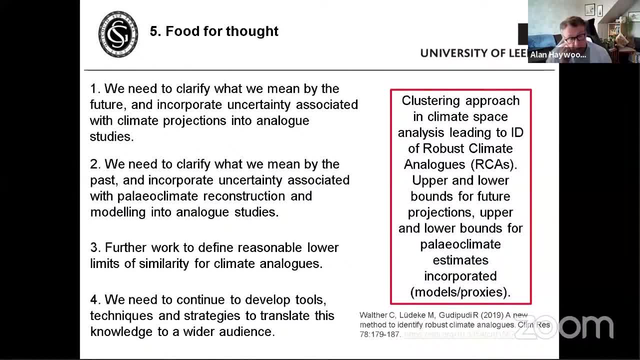 climate reconstructions and modeling into analog studies. So for us, if you say something like, the Pliocene is an analog for the future, I actually know that. we know that the Pliocene actually represents a whole load of different climate states, So one of the things that we could also do- 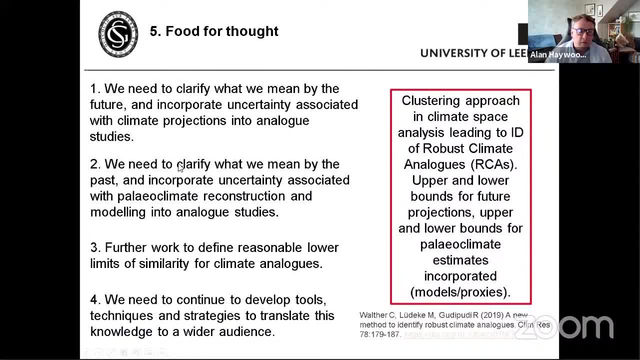 to try to firm this up and put a more structured framework into the future is to be more precise in terms of what we mean about the past. I think there's some further work to do to define reasonable lower limits of similarity for climate analogs. 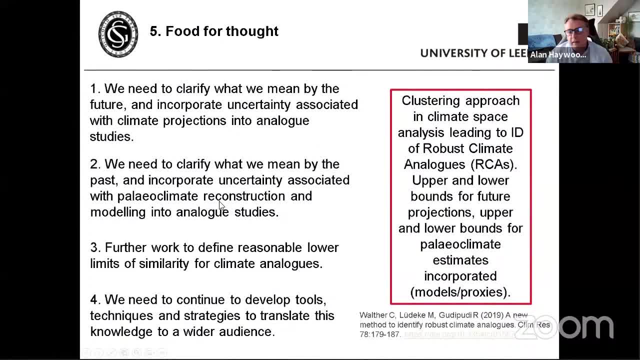 And I'm not trying to suggest that this work isn't going on. I think that this work is already absolutely going on And I picked up a paper here by Walther et al in 2019, which was presenting a new method to identify robust 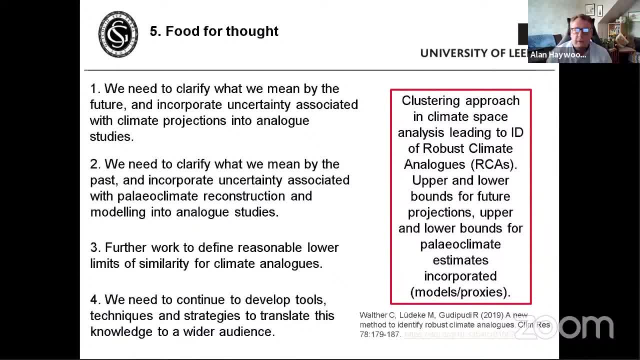 what they refer to as robust climate analogs in climate research. So you know I think there's some further work to do to identify robust climate analogs in climate research. There they were using a clustering approach in climate space analysis, leading to the identification of what they referred to. 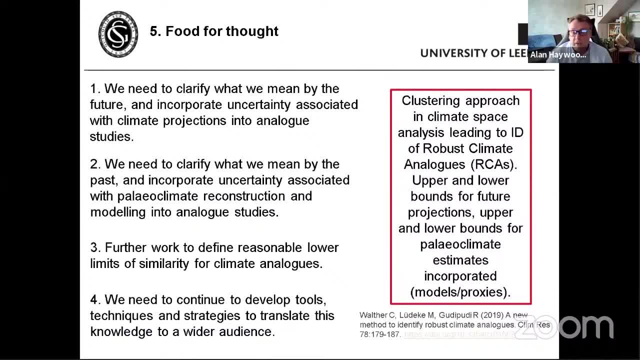 as robust climate analogs using upper and lower bounds of future projections, But we can also, in the context of our work, also start to think about how we include the upper and lower bounds of paleoclimate estimates, both from models and proxies, as well. 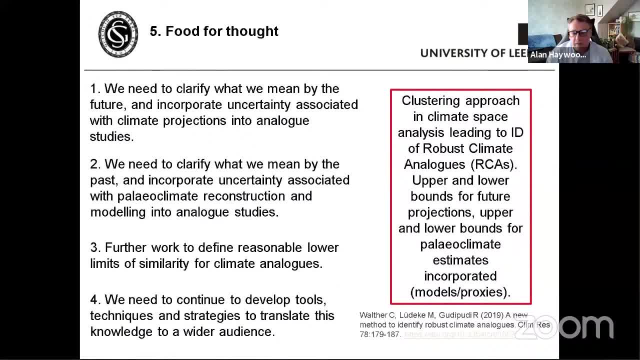 And finally, I think, the last thing I want to say, which will hopefully lead on nicely to Rachel's talk a little bit later on, I think what Mo Rameau said yesterday about the importance of co-production and the absolute requirement to continue to develop. 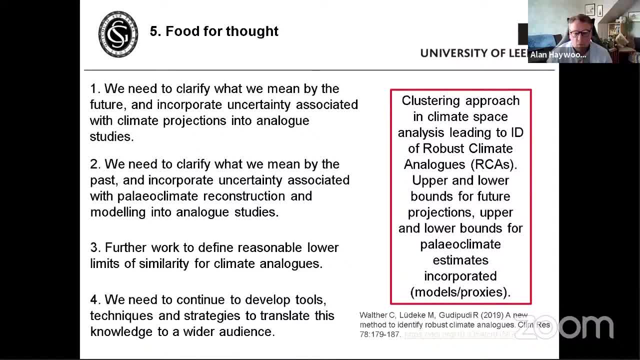 the tools and techniques to get our work out to the widest possible audience if it's going to have the biggest possible impact. So I think we need to continue to develop tools and techniques and strategies that help us translate this knowledge from the paleo to a wider audience. 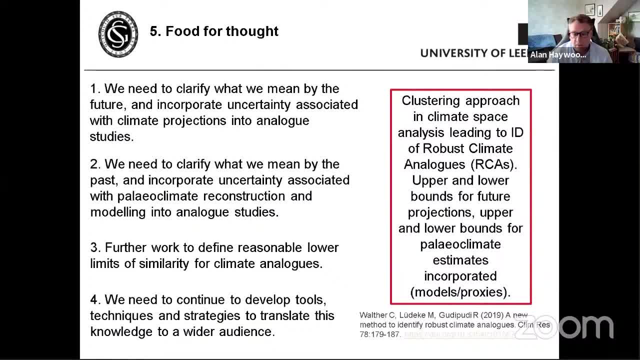 and maximize the potential it can have in helping society deal with this huge challenge that we're currently facing. And I think with that I'll end. Thank you very much. Thanks so much, Alan. We've got a few questions and I've got my eye on the time slightly. 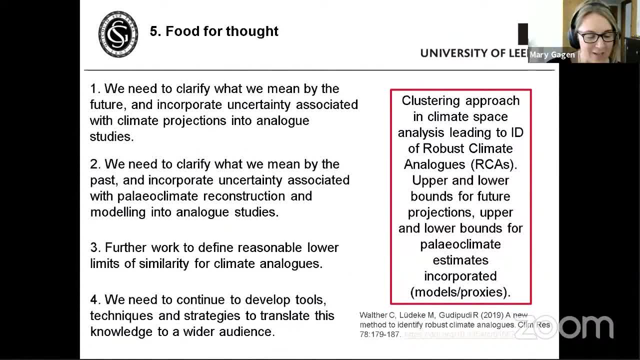 but I'm certainly going to ask a couple. So we've got a question from Babette first of all, Alan, So under a business as usual scenario, Babette's saying we are looking at similar rates of changes during the EO scene and asking what could this mean for our 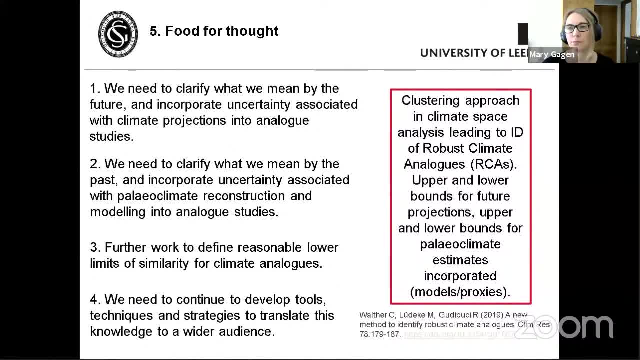 future climate. Sorry, the question was: what does that mean in the context of that? So what would that mean If we were looking at similar rates of change as experienced during the EO scene? what would that future climate look like? Well, I think I don't really quite understand the question. 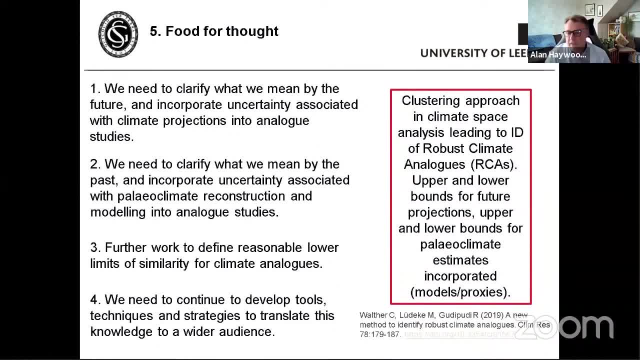 because the rate of change that we have right now is not the same as we've seen. It's not the same as the future climate. It's not the same as we've seen. It's not the same as the future climate. in the in the in the ear scene, i, i think it partly comes down to um addressing the: the unknown nature. 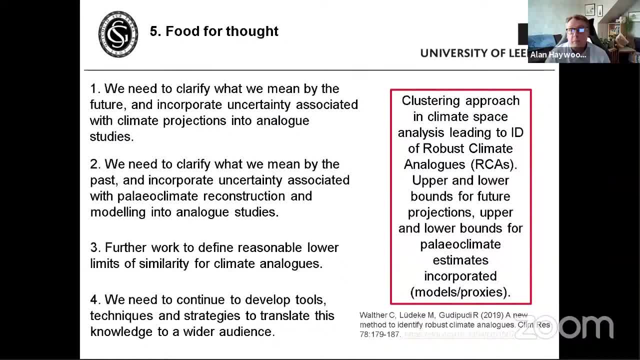 of what some of these impacts are going to be, and it partly comes back to the kind of um work that um that danny was presenting earlier is the fact that we we can get an idea from the geological record about what some of the impacts will be when we've had kind of geologically normal. 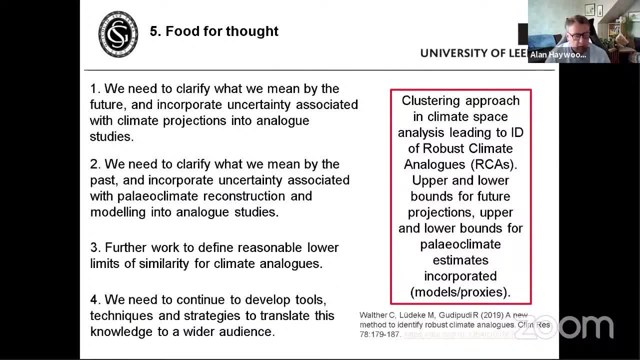 rates of change. but the question then has to be and the danger becomes: what happens if you, if you make those sorts of changes under time periods which are substantially contracted? and i think that's where a lot of the danger and a lot of the the risk in terms of how we're going to be able to. 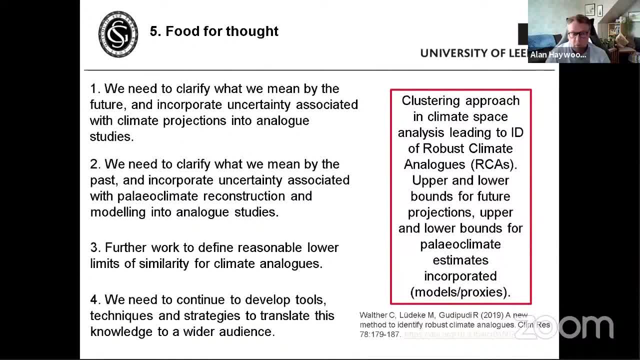 cope in the future actually comes from, and so we we need to be precautionary, we need to be careful, we need to try to get the situation under control as quickly as we can. um a question from from gavin: with increasing computational power, will we see more modeling efforts focusing on transient 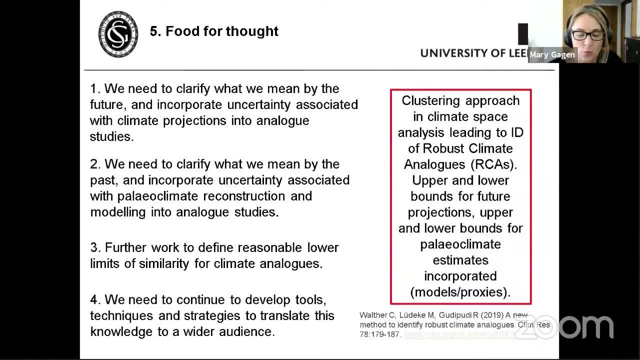 signals in a geological record and, if so, how useful would these be versus the current focusing on equilibrium states? yeah, that's a that's a really good question, i mean. i mean, i i think one thing we are already seeing is we are seeing more and more transient climate studies. 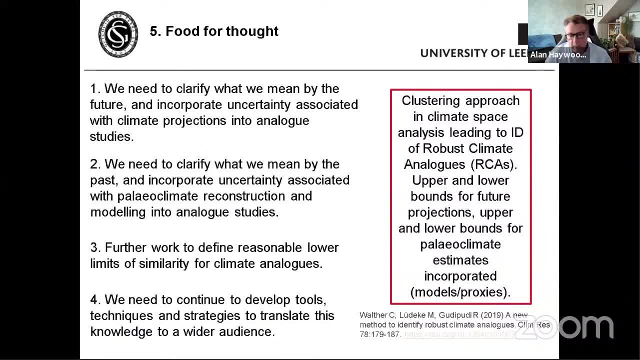 which are coming out in the context of paleo, climate modeling and and the, the improvements in our energy and the energy production and the energy and the energy production. That's, in this context, and i think, the one of the key things which remains a limitation, uh, into the future in that context, particularly when we start thinking about applying those sorts. 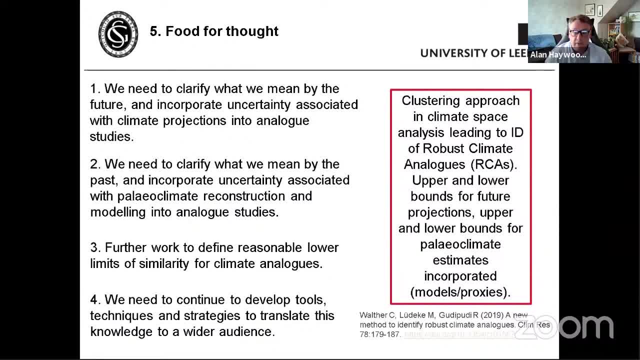 of transient climate modeling techniques to intervals of time further in the past is being able to come up with really robust and sensible um transient forcings for those particular models. so it isn't actually just the technology that's going to be important in the future. we do see a lot more. 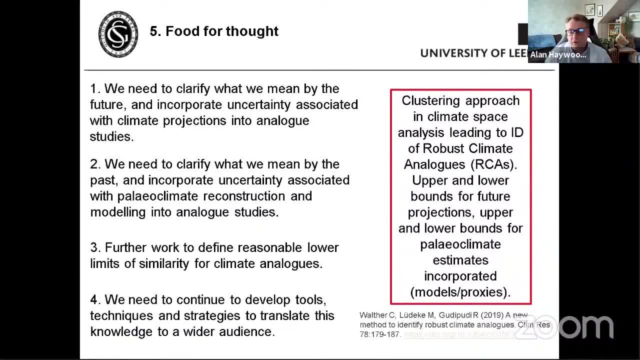 if you like. there's going to be some work to do in figuring out what would be sensible in the context of initial forcings and transient forcings, for a modelling framework like that for different intervals of time, And I think that's an interesting challenge and it's certainly a 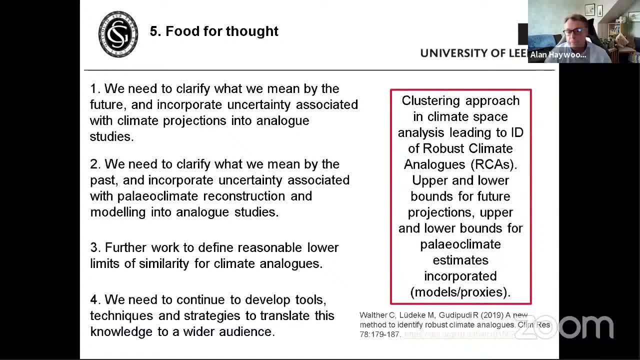 challenge which is well worth taking up. We are running slightly over, but I just want to ask one last question, which is a really nice question from Pallavi. We have a tendency to become slightly temperature obsessed, and Pallavi is asking: please can you say 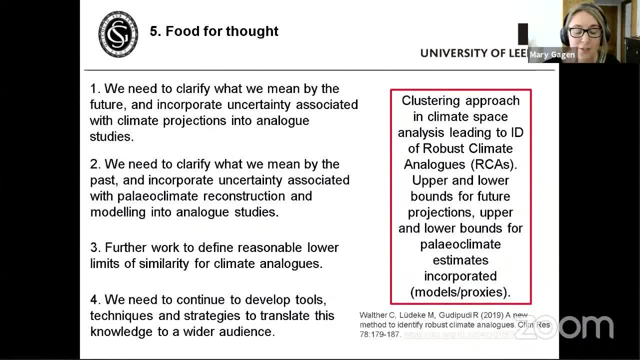 something about how paleoclimate records, on hydroclimate, can help us moving forward. Oh, yeah, sure, I think that this is absolutely critical and the reality is there are more limited array of topics and techniques that we have in terms of getting exact precipitation estimates into the past. 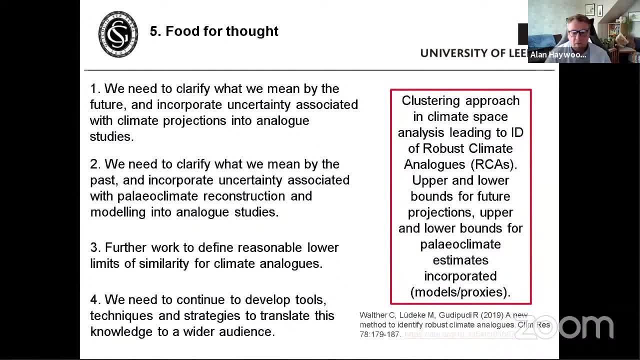 but it's still possible And we certainly need to be able to carry on that work. But I think one of the key things that we can also do is look at that a little bit more holistically. So I think some of the older techniques in the context of actually working out the hydroclimate conditions. 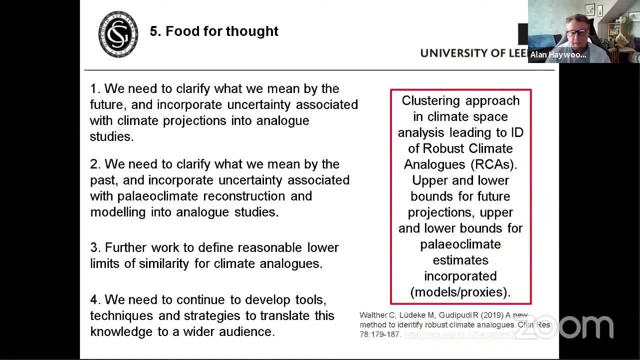 into the past. some of the lithological indicators, some of the climate sensitive Fasci's work that was done in this sort of space can really complement and enhance the number of data points that we have available which can inform about hydroclimate variability into the 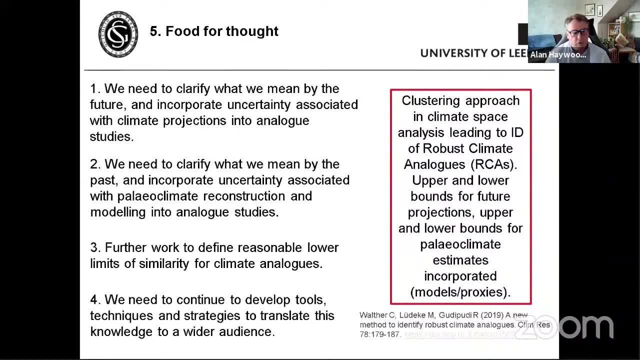 past. So I think part and parcel is it's about trying to use all of the tools and techniques that we've got available to us, not necessarily just the ones that might give us an absolute estimate of precipitation change in the past, with also its associated uncertainties. 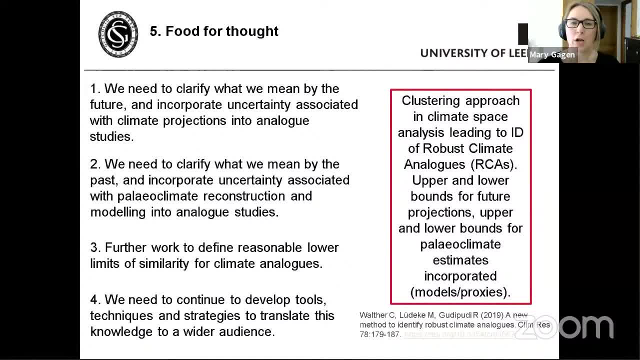 Thanks so much, Alan. I'm going to wrap up there and move on, But just a little reminder as well to all our speakers: please do jump onto the Q&A after your talk or at any point actually in the session, because there are additional questions that we're not able to get to, And don't forget as well. 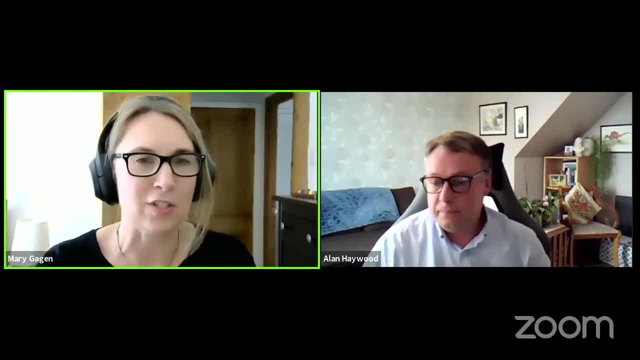 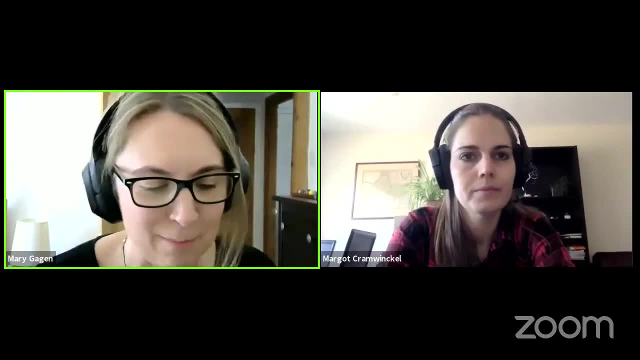 have a quick look in the answered questions, because there's lots of questions in there that are relevant to more than one speaker and you might have something to contribute as well. So thanks very much, Alan, And I'm going to move on to our second. 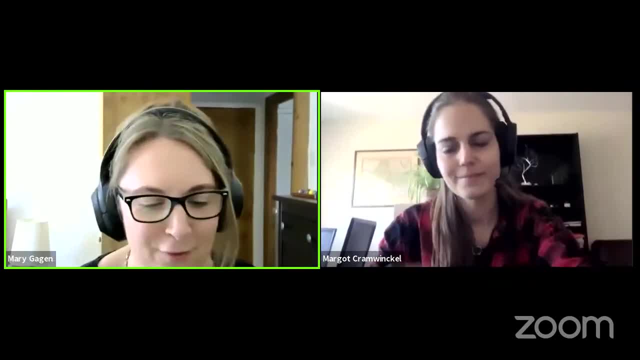 flash talk of the day. So I'm going to move on to our second flash talk of the day. So I'm going to move on to our second flash talk of the afternoon, which is from Dr Margot Kramenkel. Margot is a research fellow within ocean and air science. 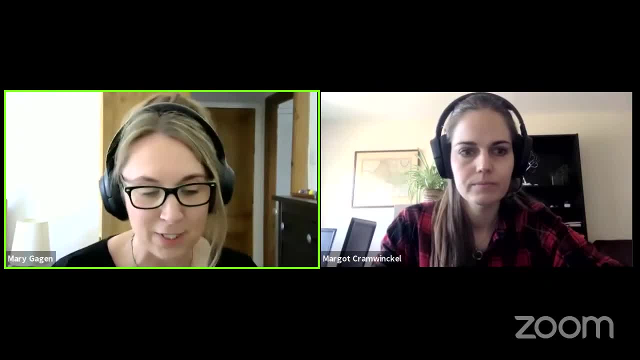 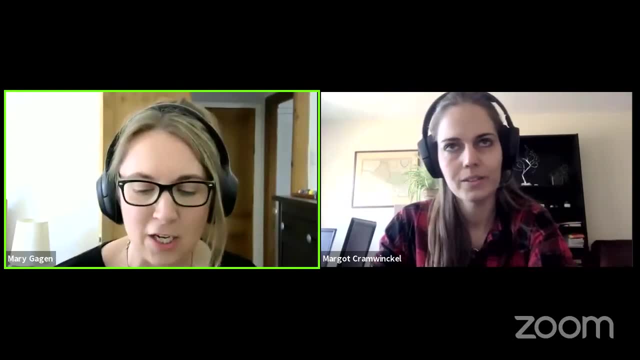 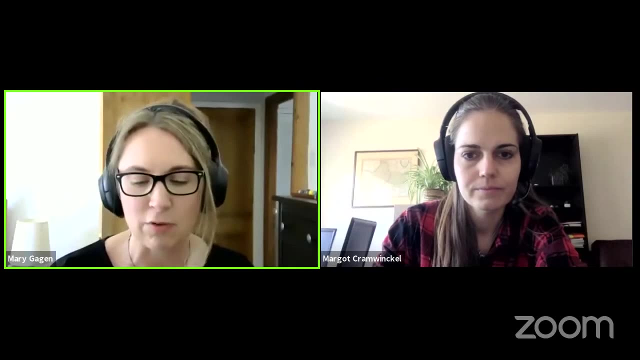 at the National Oceanographic Center in Southampton And her research is on Eocene warm climates to explore our air system states under higher CO2.. She uses both proxies and model simulations to explore not only the climate but the critical carbon cycling and that broader. 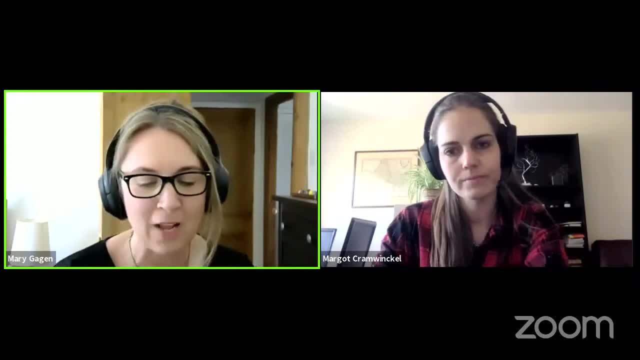 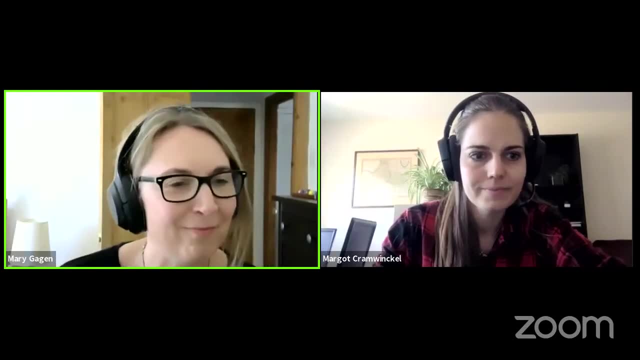 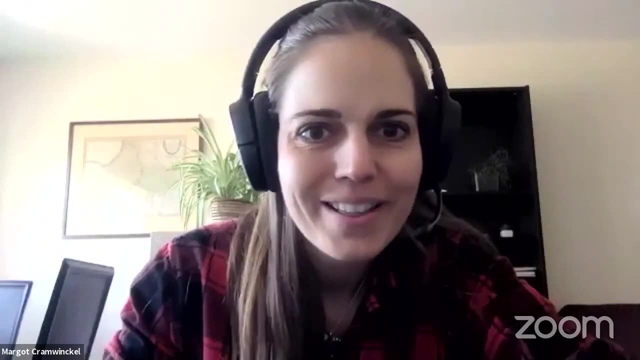 environmental response to past high CO2. And Margot is going to talk today about the early Eocene hothouse climate, so I'll hand over to you, Margot. Thank you very much for the introduction. I have to say I've really been enjoying all of the talk so far, so thanks to all the presenters. 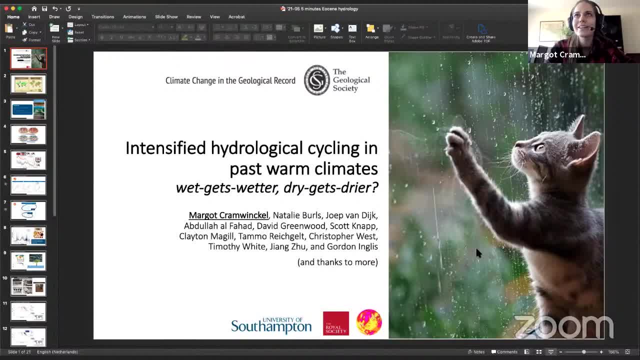 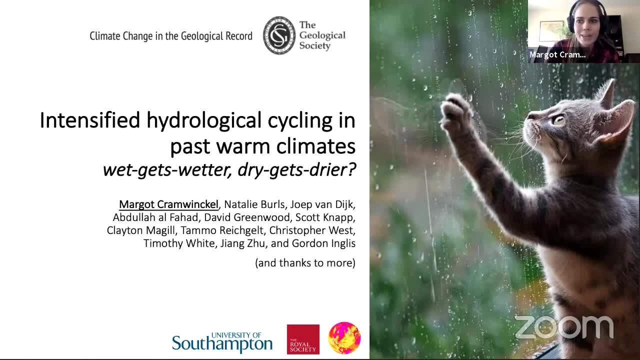 All right, there is my presentation. All right, and thanks of course, also for the opportunity to let me talk a little bit about my past year of pandemic post-talking in sunny Southampton, And I'm going to use these five minutes to show a little bit of my in-progress results on. 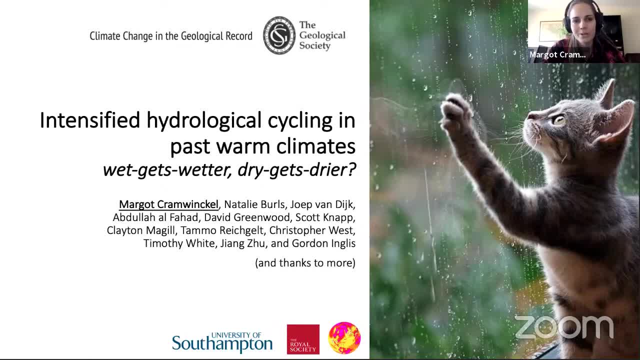 hydrological cycling in the warm Eocene. so that actually ties in pretty well to the last question we were just discussing, And the cat picture is just to help you stay awake and keep an eye out for some more. All right, I think that these two pictures clearly illustrate the importance of the 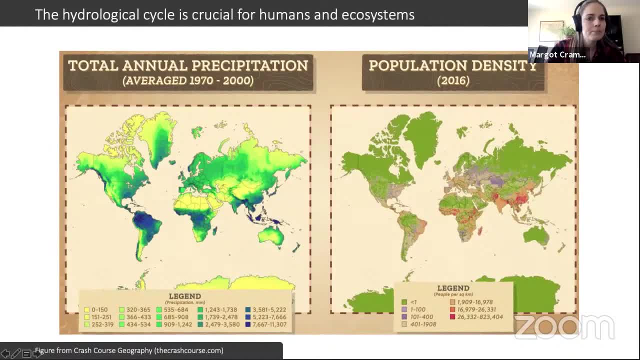 water, And I think that these two pictures clearly illustrate the importance of the water. All right, I think that these two pictures clearly illustrate the importance of the water cycle, as annual mean annual precipitation on the left really shows the same patterns as population density, So greater density in areas with the most rainfall per year, as our food production, of course. 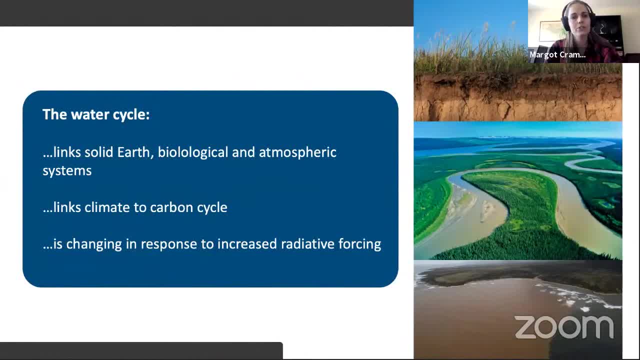 depends on this, But, moreover, the water cycle is also really important in linking the climate and carbon cycle together through runoff. So, all in all, it's very important to be able to predict how hydrology will change in the future under future warming. And while we're pretty sure that the hydro 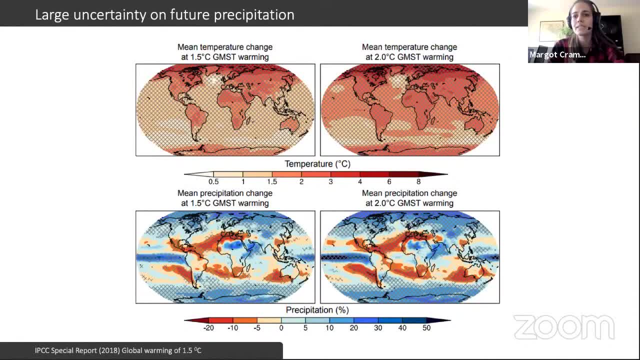 logical cycle will intensify as global temperatures rise. the specifics of this remain very unconstrained, as illustrated here. So these panels show future IPCC projections for scenarios of one and a half and two degrees of warming under high emission scenarios, And in these panels, 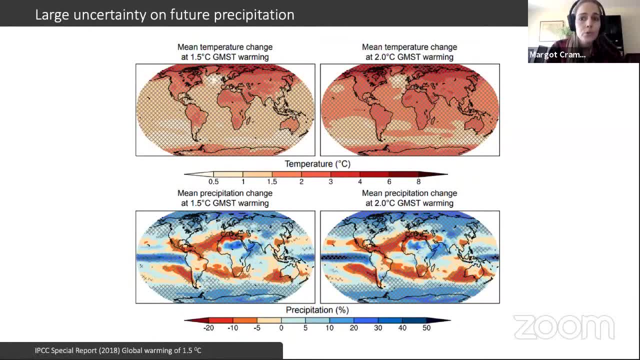 the cross hatching represents areas where more than two thirds of the used models agree on the sign of change. So the upper panels show good agreement. So all regions will basically warm under these scenarios, which makes sense. But in the lower panels you can see: 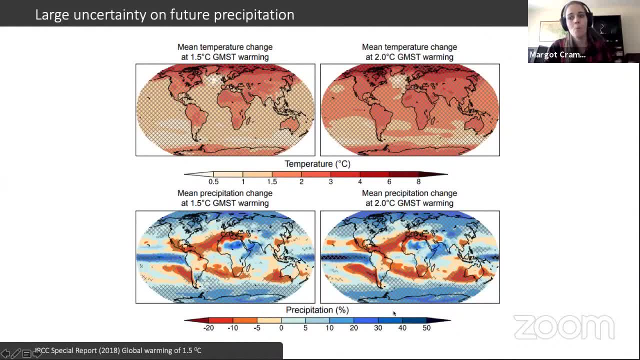 that most model projections agree on more precipitation in the high latitudes and the equator. So there's cross hatched areas. but there are also large regions where the models do not even agree on the sign of change. So whether regions will get wetter or drier under future warming. 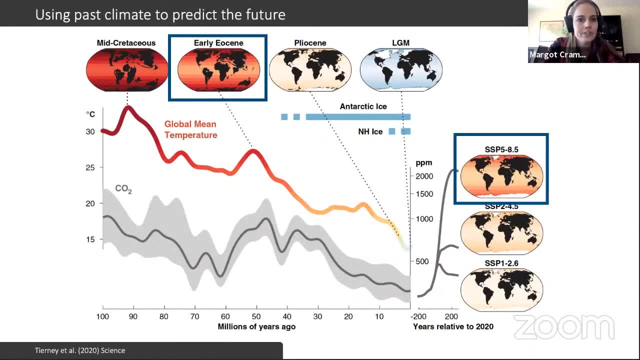 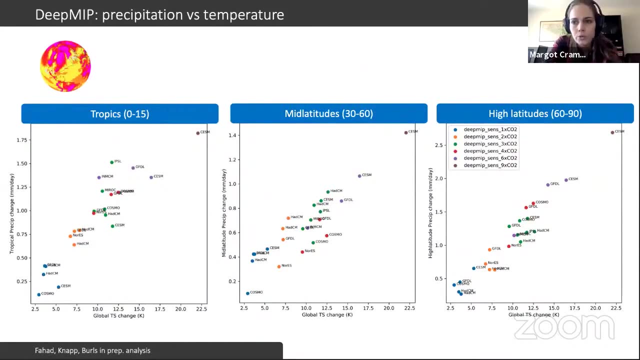 So let's try and constrain this future response a bit by looking at the early Eocene, which can be used, as we just heard in Allan Mit sport talk, as a partial analogue to next century climate under high emission scenarios. Here are some scatterplots showing the model values from a set of early Eocene model simulations. 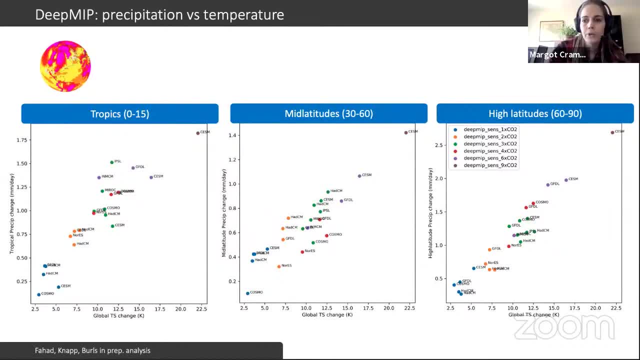 as generated within the deep MIP project, the Deep Time Model Intercomparison project. All of these plots have temperature change compared to pre-industrial in the horizontal axis and they all have change compared to the pre-industrial on the vertical axis. So what we clearly see here is: 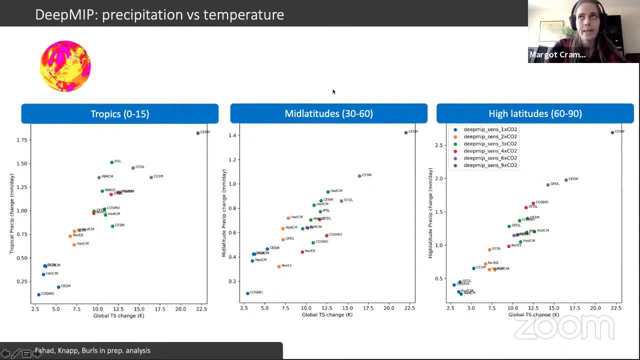 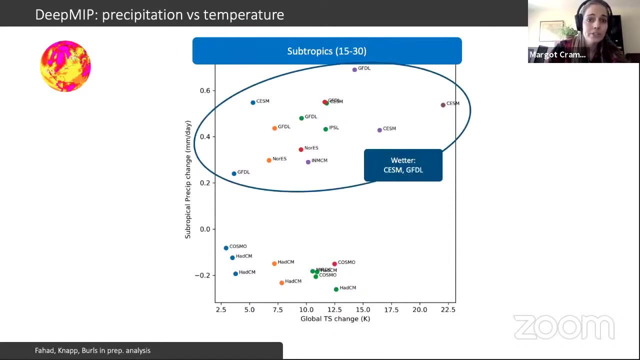 that for these latitudinal bands- so the tropics, the mid-latitudes and the high latitudes- all models simulate increasing precip with increasing global temperatures. But looking at the subtropical band, some models actually predict wetter conditions, whereas other models predict drier subtropics. So that's a bit of an uncertainty there. 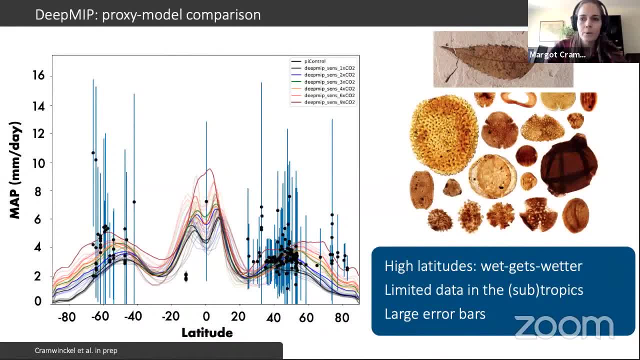 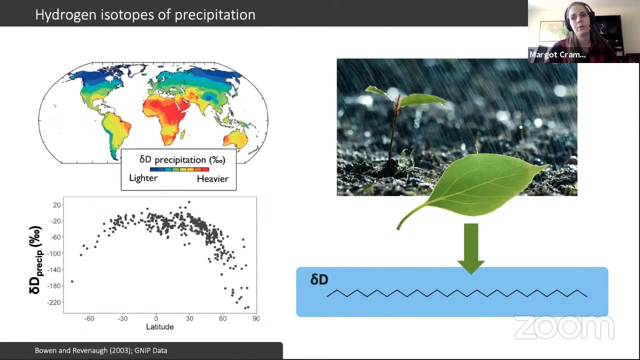 Now based on the comparison to the available paleobotanical proxies that are actually able to give you absolute estimates of precipitation for past climate. unfortunately, we really cannot say anything very meaningful about this difference, as there's very limited data availability in the tropics and subtropics. Also, the error bars are fairly large here. Now an alternative approach. 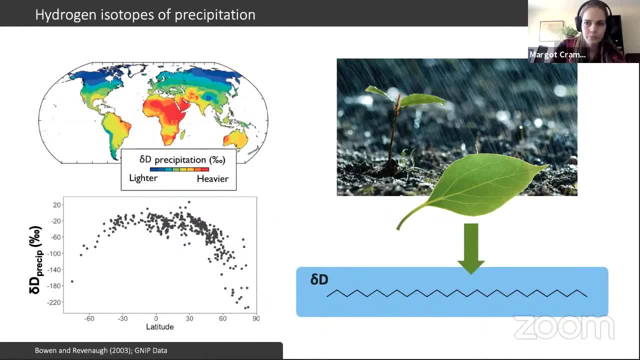 to reconstruct past hydrology is to look at the isotopic composition of precipitation in terms of hydrogen and oxygen isotopes of water, And, globally, the most clear pattern in this is this latitudinal gradient. Two major factors play a role here, and those are temperature and water vapor. 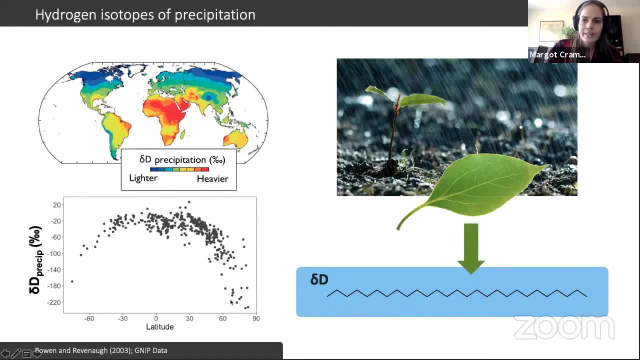 transport. So we have more depleted values at high latitudes due to increased rainout of the heavy isotopes during transport, as well as greater fractionation at cooler temperatures, And this isotopic signal of the rain can actually be recorded by plants in their leaf molecules. 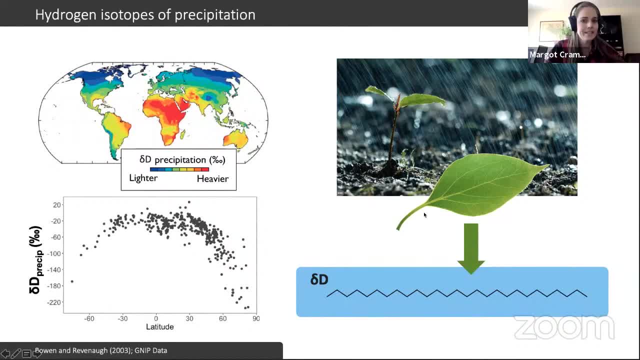 and plants take up water from the environment And, as these leaf waxes or long chain anal canes preserve very well in sediments, they have been widely employed as proxies for past hydrology and they've also come by a couple of times in the talks we heard yesterday. 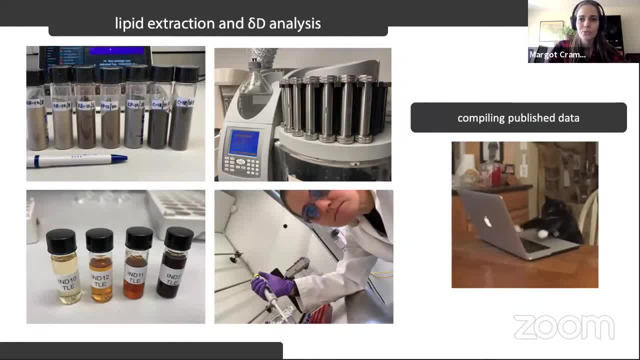 So I've been extracting and measuring lots of leaf waxes from early Eocene sites from different parts of the globe, as well as compiling all the data I could find in the literature, And here I've plotted these results. I've plotted them together with the modern gradient. 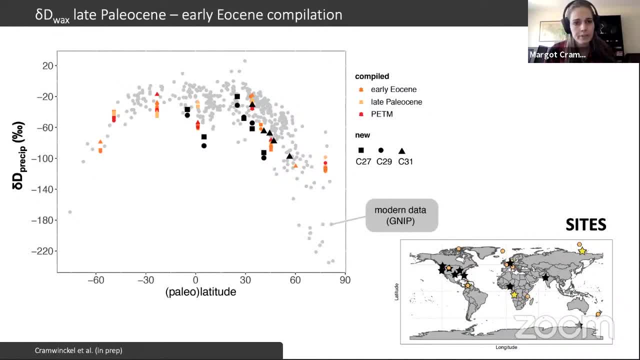 A note here is that I've just assumed a constant fractionation factor between my measured leaf waxes and precipitation, which is likely not realistic, But still for now it allows us to at least compare the shape of the gradient to the modern gradient, And in terms of this shape there's some 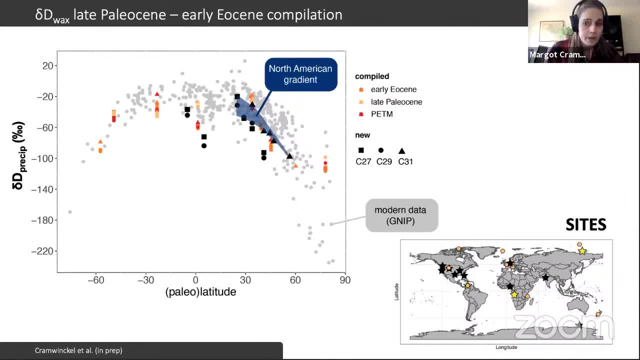 preliminary observations. So first, we have quite some new data from North America and based on this data, those data nicely line up And also pretty similarly to the modern gradient. Second, values in the tropics seem fairly depleted, which might be due to extensive rain-out, which is known as the Amount effect. 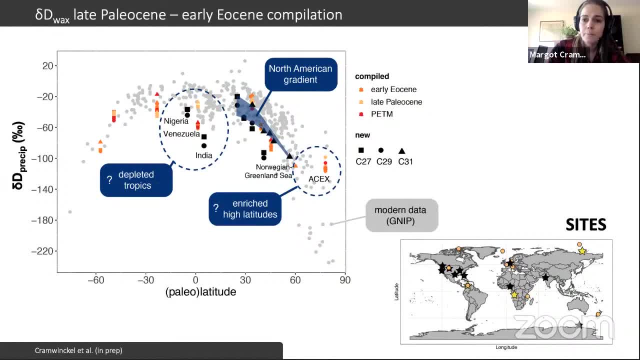 On the other hand, values in the high latitude seem relatively enriched, which has been related in earlier work to warmer temperatures and increased moisture delivery to the Arctic, And these observations seem to work together toward towards a strongly reduced gradient in isotopes in precipitation isotopes in the early Eocene. 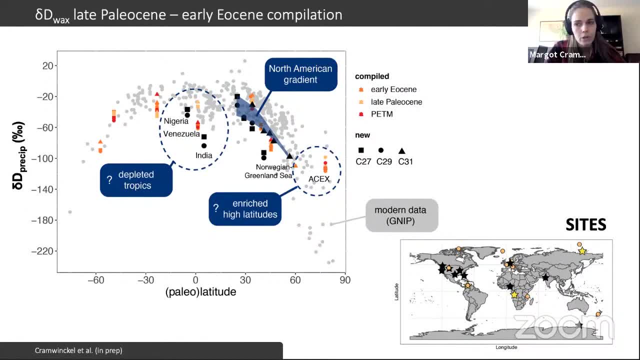 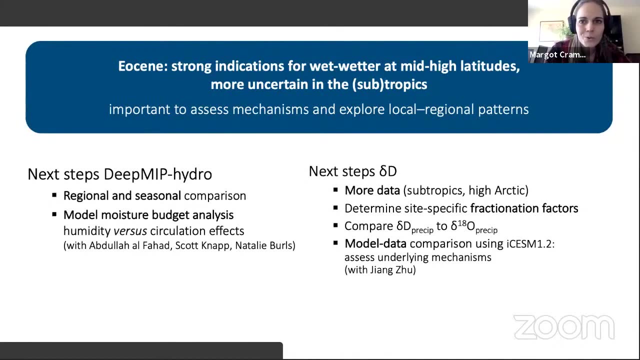 Although keeping in mind that the data is still fairly sparse in the lower and the higher latitudes, which is why I'm going to try and generate some more data there. And these are the yellow stars on this map. So, seeing as I've managed to talk myself past the five minute mark already, 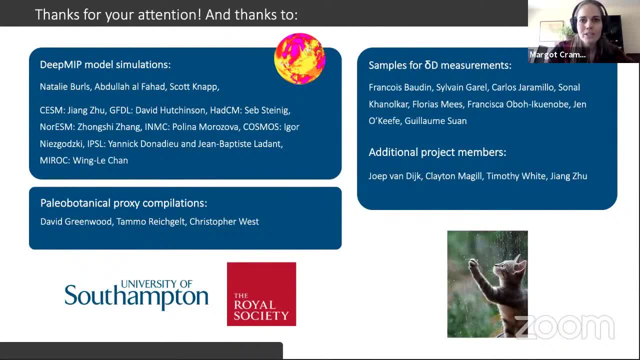 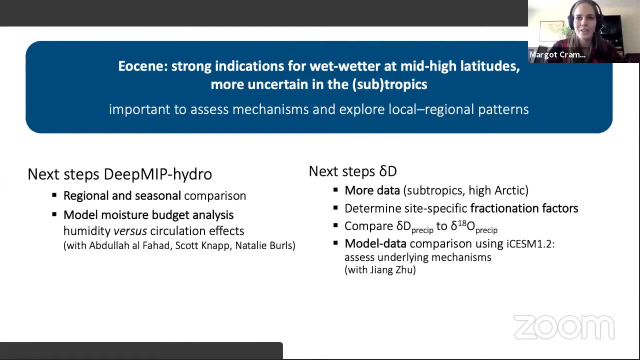 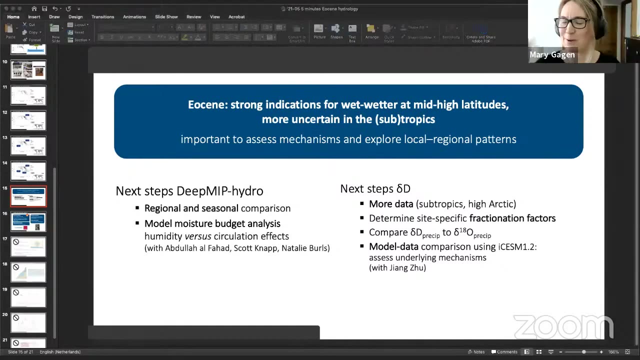 I would just like to thank a lot of collaborators because, of course, this incorporates a lot of proxy data and model simulation, So a lot of people worked on that, And I'll just leave these, these next, next steps, open for your thoughts And thank you. Thanks so much, Margot. 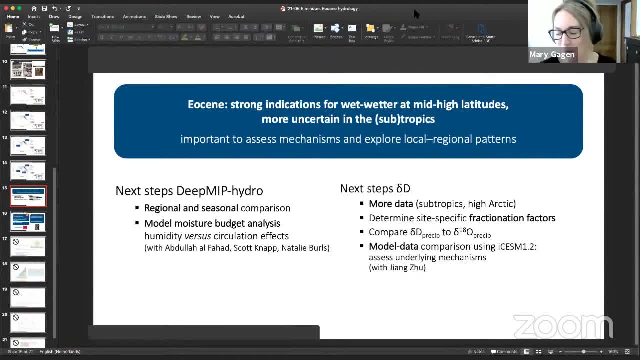 Really nice to hear some isotope plant work. So we've got a question actually from from the panel, because I'm just keeping an eye on checking I'm not overlooking any questions that are open. So, Margot, a question for you: Do we need to take into account the evolution of plants when interpreting leaf waxes as a proxy? 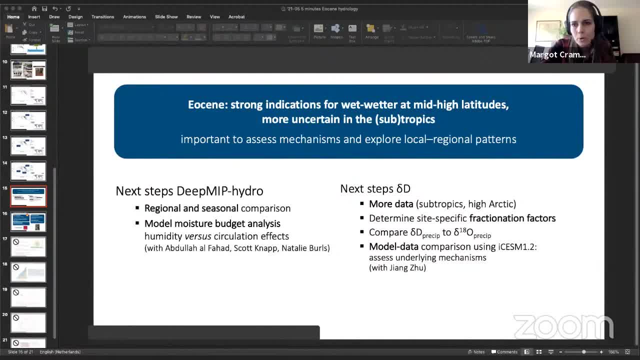 Yeah, good question. I think it's. it's probably important that we keep in mind the the large plant groups that these molecules like They're likely derived from. So that's why I was also mentioning my constant fractionation factor that I'm using. 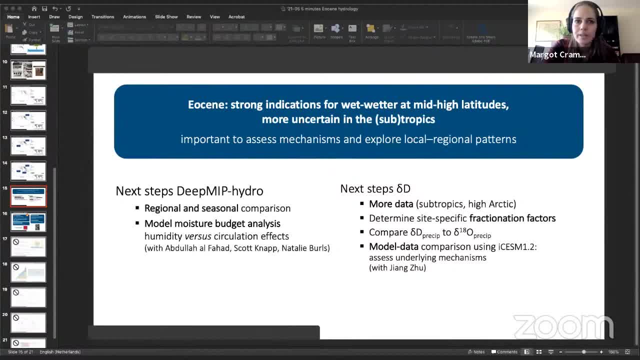 So we might be able to use the plant assemblages to correct for for the effect of different plant groups contributing to the to the NLK signal, And so, yeah, this isn't meant to be an unfair question at all, but I can ask you. 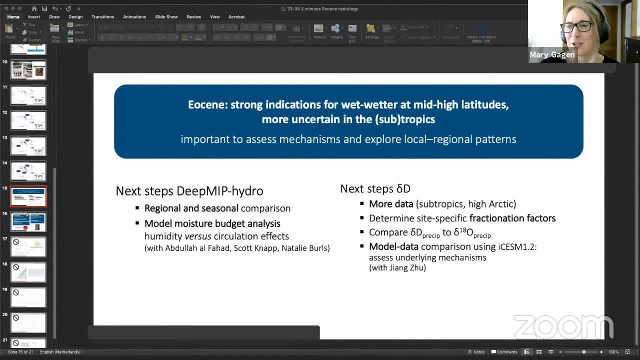 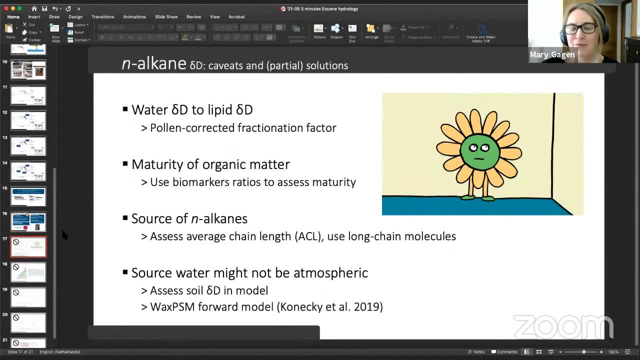 So I know there's so much more to say about the fractionation assumptions that I wanted to just give you an opportunity to say that. So, how, what assumptions might we think are problematic in assuming constant fractionation like that, particularly with hydrogen, Because it's it's such a tricky one, Yeah, So am I still sharing this slide? 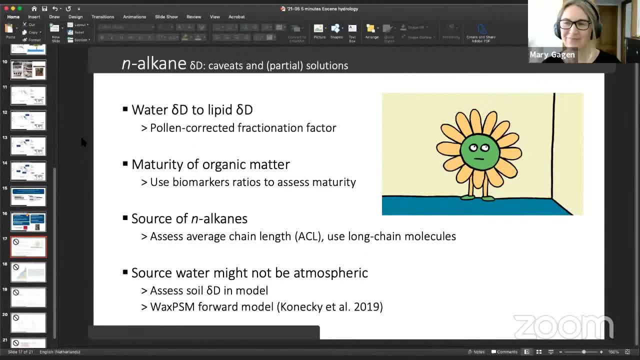 Yeah, Yeah, Yeah, OK, Yeah, So there there's. of course, those plants are not taking up the precipitation directly from the area. They are actually taking up water from the soil. So that's one of the factors. Yeah, And you can. you can target that by potentially looking at- actually looking at- soil isotopes derived from models. 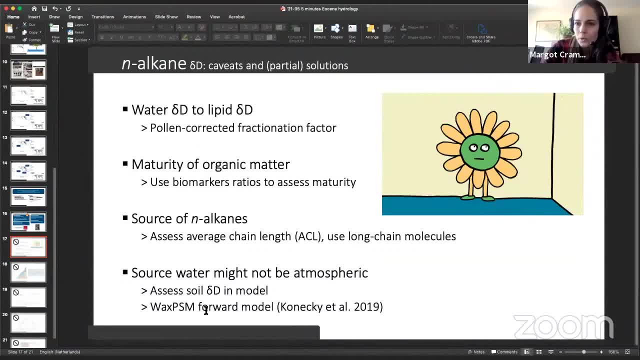 Or there's also been some work on this forward modeling, which I'm going to look into if you, if that might be a possibility to apply this. Yeah, Other things to take into account are maturity of biomarkers And this and the actual source of the NLK. 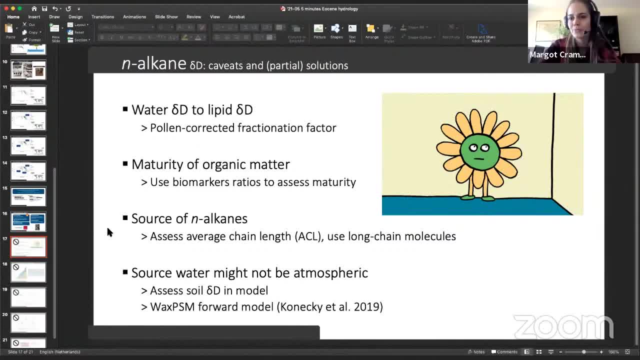 So what kind of plants they are deriving from? Are they actually deriving from? from higher plants, Yeah, But those are all things that we are. we are trying to take into account as much as possible And we'll be also taking into account more in the future steps of the project. 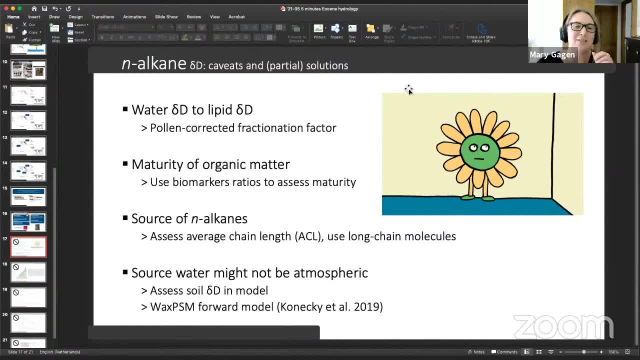 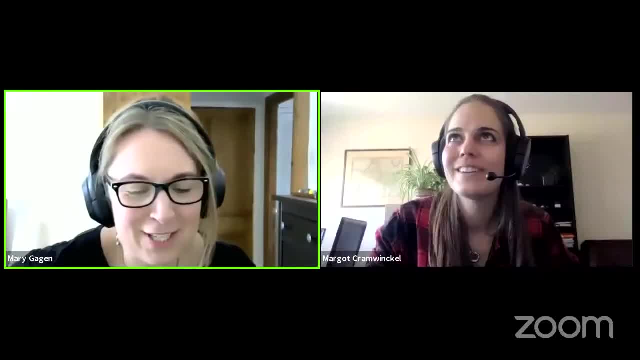 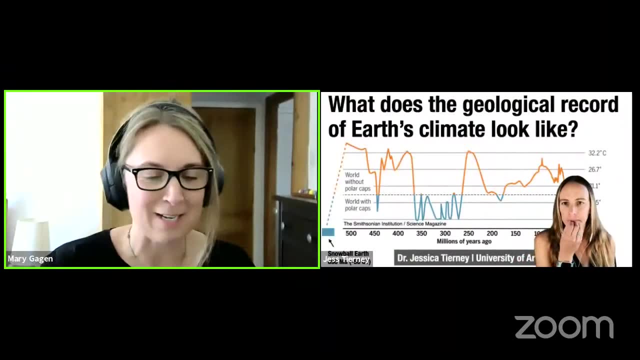 Thanks so much, Margot. Really lovely talk And thanks for thanks for waking us all up with cats- Always good, right, Thanks. So I'm delighted to move on to our last speaker of this session and to welcome Jess Tierney to talk about the first question in the statement. 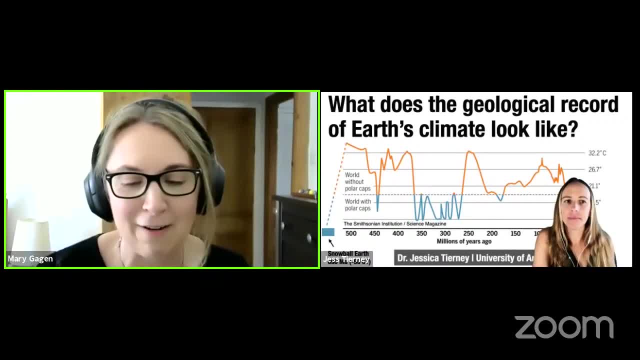 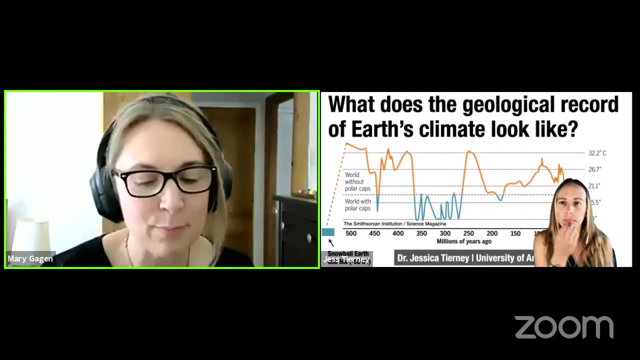 So Jess is an associate professor at the University of Arizona, and her research focuses on the study of past climates over a variety of timescales, particularly using organic geochemical techniques and statistical climate reconstruction. Jess's post-grad and postdoc work was looking at defining East African climate over the last 60,000 years and also established her as a world authority on biomarkers in paleoclimatology. 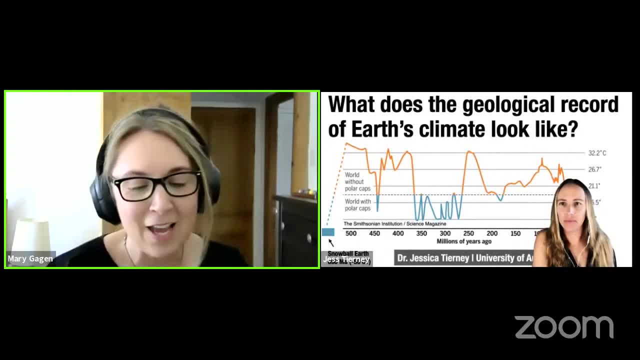 And it's how a lot of us know Jess's work. Jess is a Packard Foundation fellow and a fellow of the American Geophysical Union, and is also an AGU medal winner in 2014.. And she's also another of our lead authors on climate change. 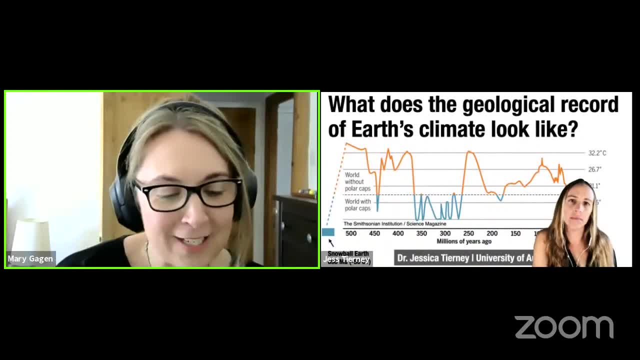 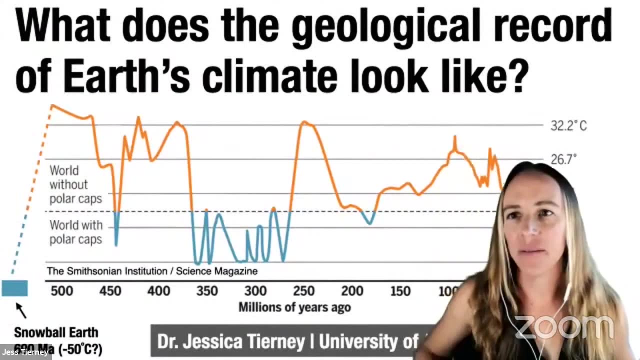 So Jess has been invited to discuss and come full circle to the very first question in the climate statement, which is: what does the geological record of climate change look like? So I'm going to hand over to you Jess. Yeah, Hi Mary, Thank you so much for that kind introduction. 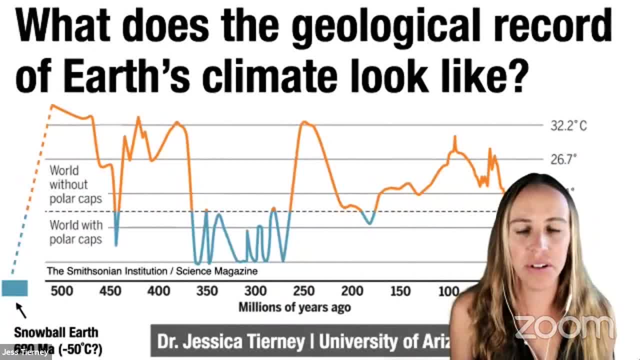 And thank you to everybody for tuning in today, this afternoon, this morning. Just a quick tech issue, So I am not sharing my screen, I'm just going to be in front of my slides, like that. So if you want for me to be kind of front and center, go ahead and click on the three dots in the upper right hand corner of my talking screen and click pin. 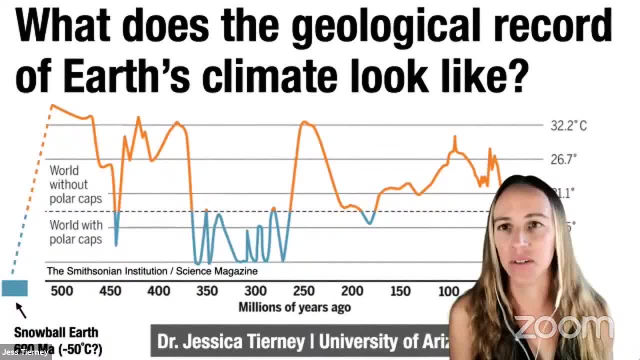 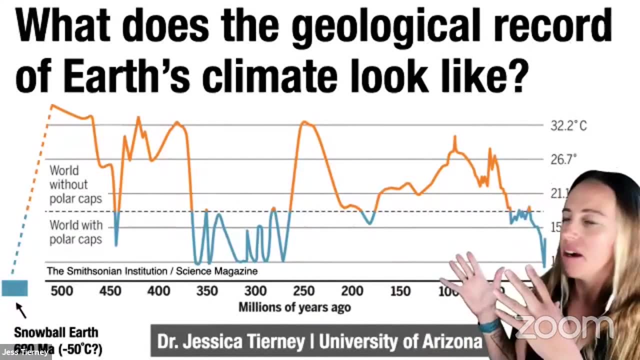 And then I won't flip in and out if someone else makes a noise. So just a little tech hit there. So the question that I was asked to address today is: what does the geological record of Earth's climate look like? And what you see behind me is sort of an informed 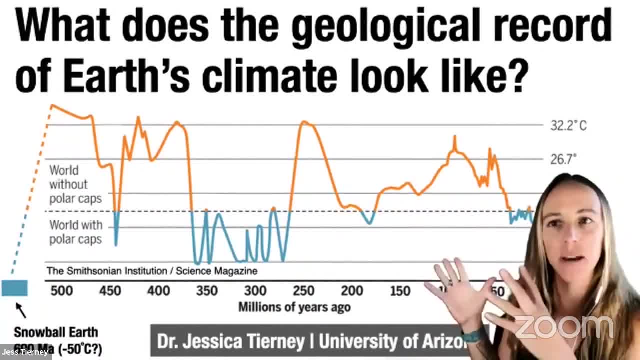 Reconstruction, I would say, and sometimes it's a best guess. Sometimes it's more quantitative than that of global surface temperature for the past 500 million years, And this is actually a curve that's on display in the Smithsonian Museum in Washington DC. 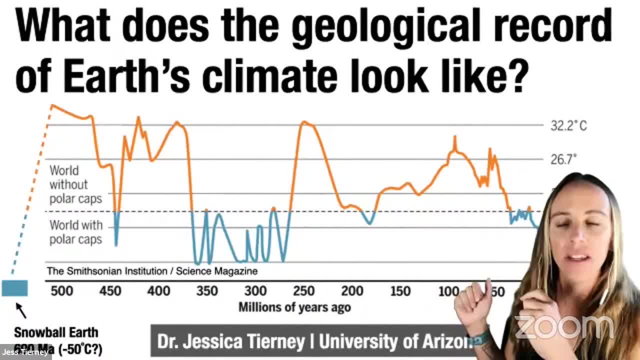 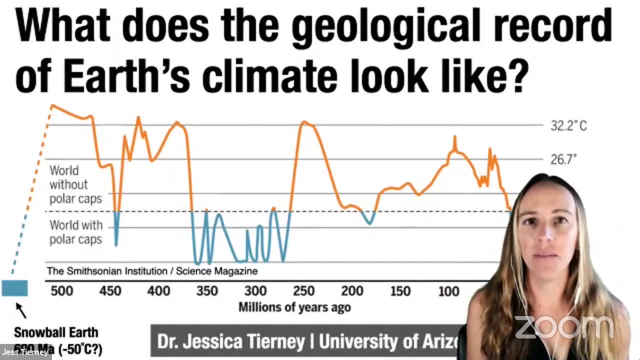 and here in the United States- And incidentally, we're working very hard to improve this curve. But what it does show, just broadly speaking, is that Earth's climate has experienced some dramatic changes In the past. there's a lot of drama going on. 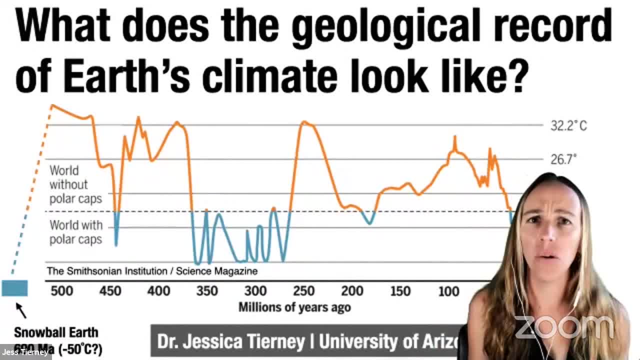 There are times when the Earth has been extraordinarily cold, for example during snow. all Earth, which we'll talk about in a second Estimates- place at temperatures at maybe as low as minus 50 C global temperature, So super cold. And then there are times that are super warm. 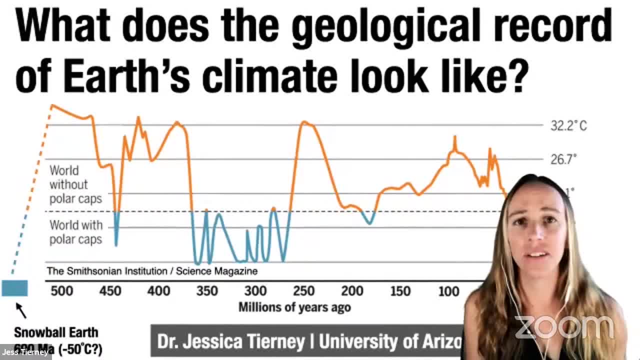 And we've already heard about a couple of those times, already this morning And just now, with Margo's talk about the early Eocene as being one of those times, The Eocene as being one of those greenhouse climates where there are no large ice sheets. 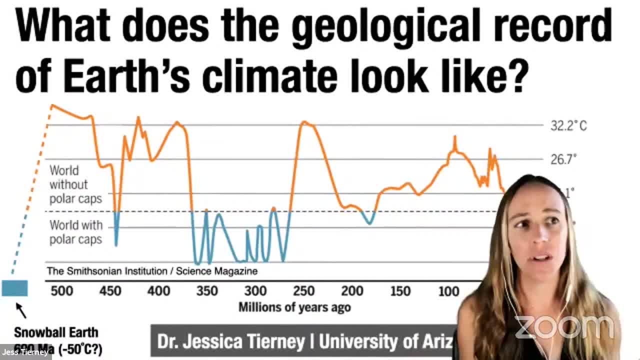 The planet is quite warm, So I don't have time in 20 minutes to actually talk about all of these swings and temperature and so on, But. but so I'll just feature some extremes. Right, We'll talk about extreme cold and extreme warm. 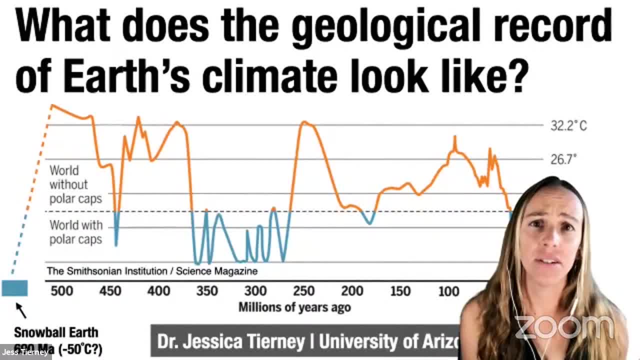 And the bottom line is that we can learn a ton about how the Earth's climate system responds to external forcings. So let's start by studying these extreme swings in climate in the past, And they are directly relevant for our understanding of future climate change as well. 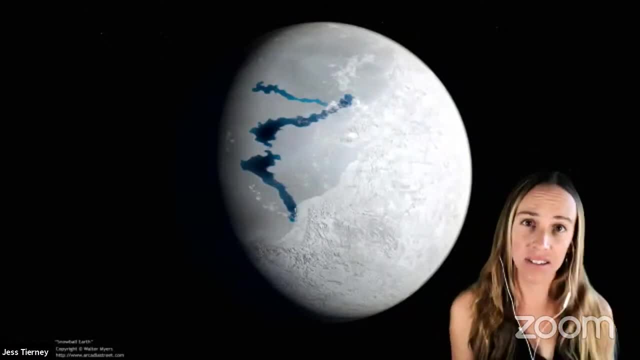 So let's go way back, probably farthest back that we've been in this session so far, to the snowball Earth time 700 million years ago, when the Earth may have been completely covered in ice: land ice over all the continents, sea ice over most of the oceans and maybe a few openings here and there. 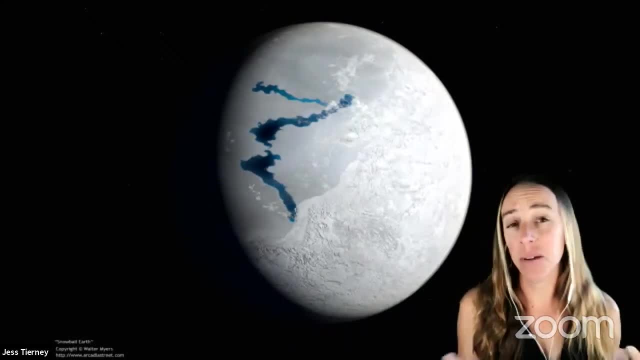 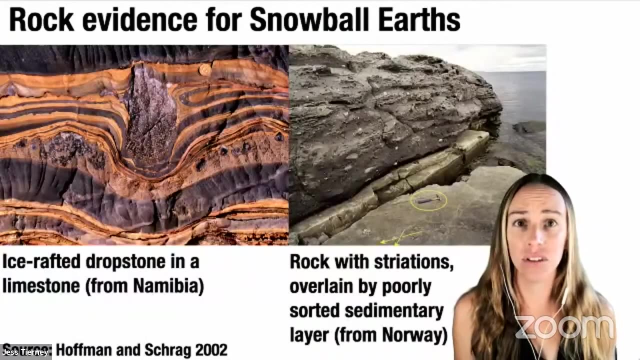 So this is a pretty extreme climate change And, first of all, you're probably wondering: how do we even know that this actually happened? Well, we have some incredible geological evidence of snowball Earth conditions that is found all over the world, And so when you're looking in the rock record for evidence of large ice sheets on land, 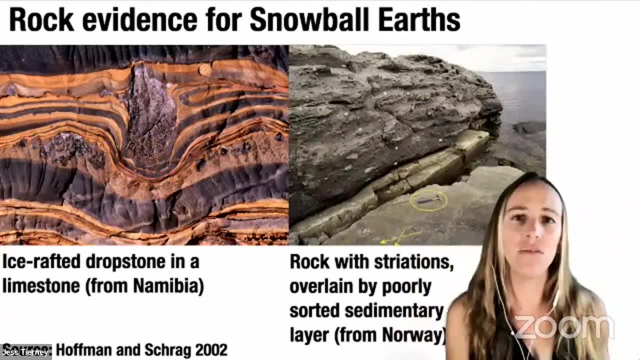 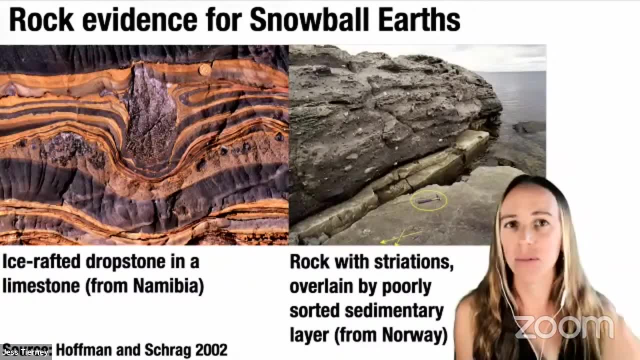 you're looking for things like, right up here, glacial tillite, poorly sorted facies striations left on the rock As large ice sheets are grinding away And messing up the rocks on land In the ocean sediments. you look for things like glacial drop stones on the far left here. 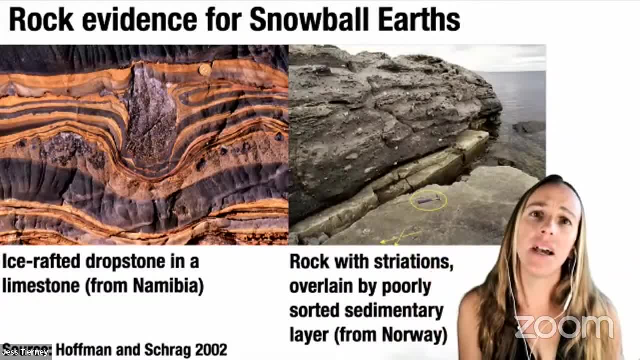 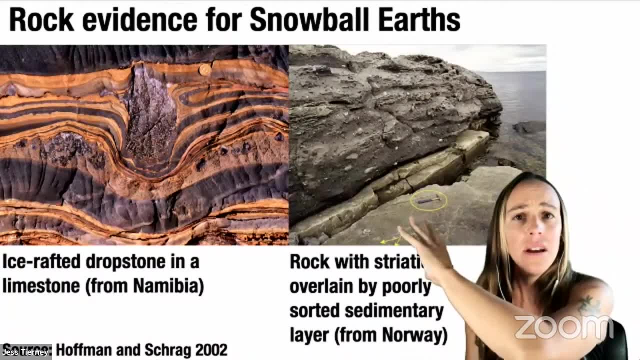 boulders that are rafted out by icebergs and then plop down and into the fine ocean sediments. You can see there a nice drop stone set in what is a banded ion formation: A drop stone dropped into a low oxygen ocean. 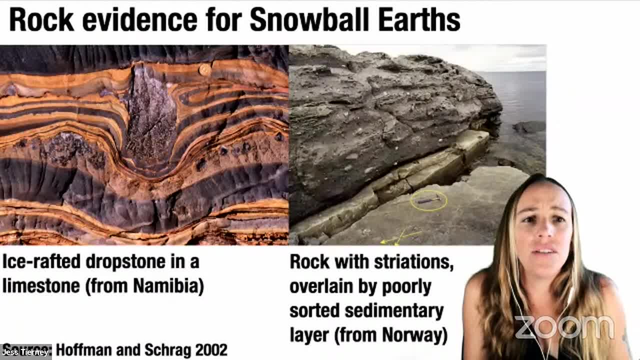 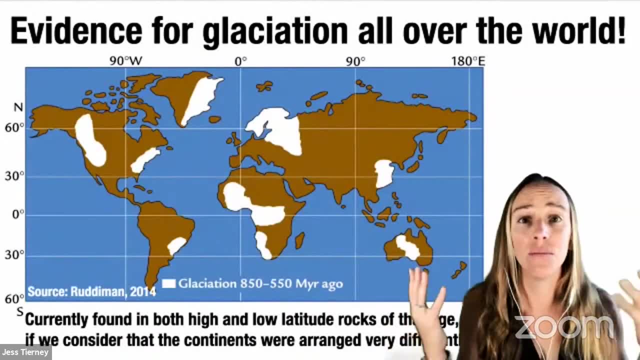 And so, in fact, geologists have found these, these glacial rocks, all over the world, all dating back to the time of snowball Earth, around 700 million years ago or so, And they're finding high and low latitude rocks, But if we consider that the continents, of course, 700 million years ago were in a completely different place, 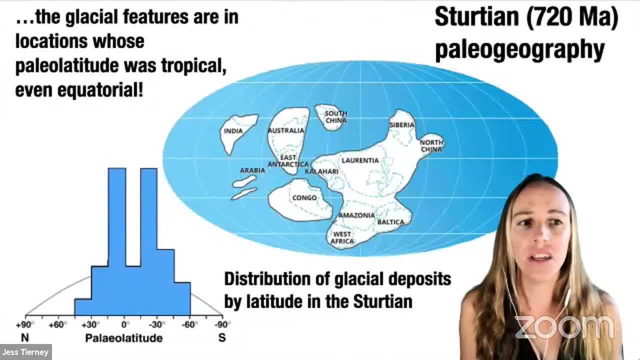 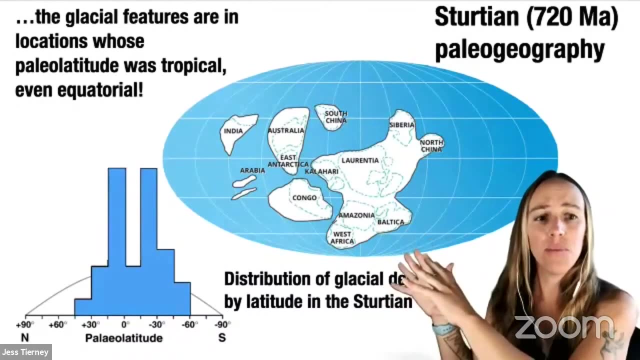 It turns out that the evidence for glaciation is actually coming all the way down from the tropics. So we are seeing glacial tillites, We're seeing drop stones at the equator, which is extraordinary, right. So here is a distribution plot of the glacial deposits during the Sturtium, which is one of the snowball Earth times. 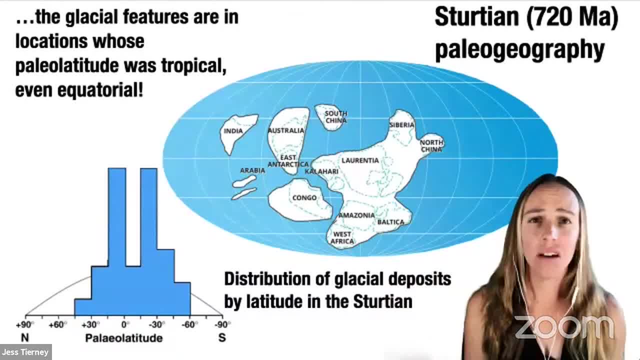 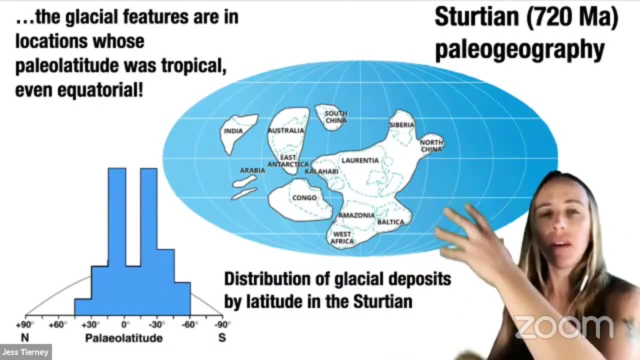 And you can see that it's bounded between 60 south and 60 north, because in fact, there were no polar continents at the time. This is what the world roughly looked like, But we find glacial deposits all the way to the equator. 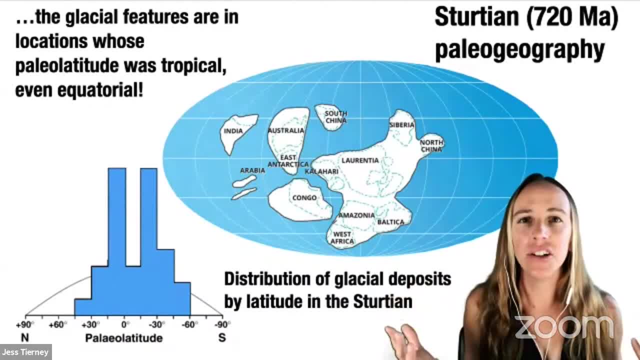 Right, So hence the snowball Earth idea. How do you get large ice sheets that are grinding away at rocks all the way down into the warm tropics, And so you can imagine that we're really pushing your system hard across some important thresholds. 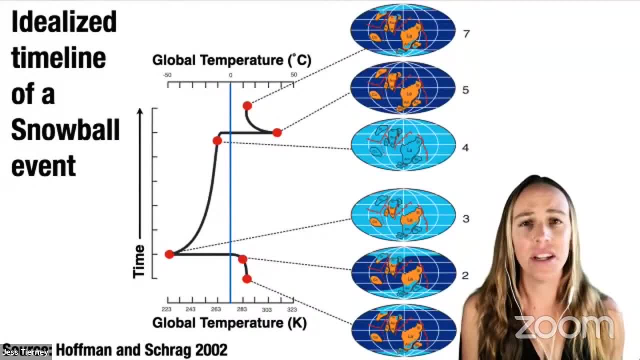 And one of the reasons I like to talk about snowball Earth is that it is actually a type case for tipping points in the Earth system and nonlinear behavior, if you will. So both getting into the snowball Earth and out of the snowball Earth involve pushing the Earth from one stable state. 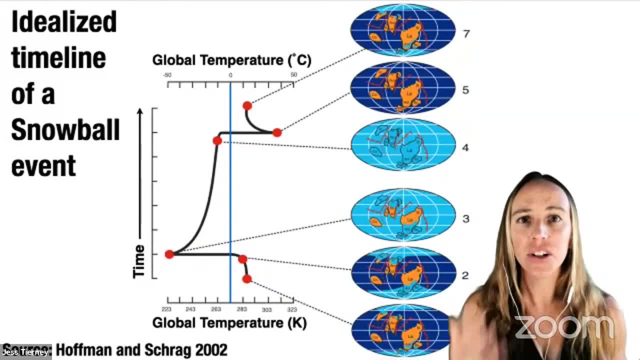 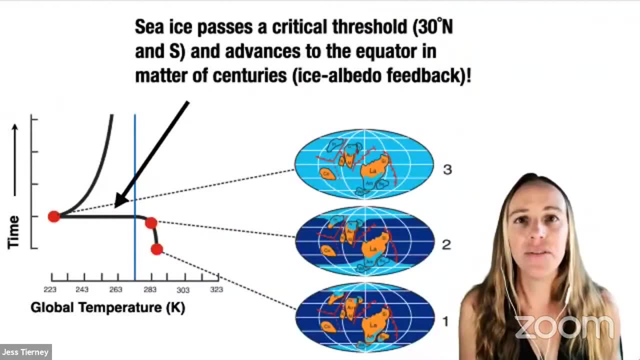 into another, across a sort of threshold where it can't really exist anymore. It can't really exist in between. So when we talk about getting into the snowball Earth, right, we have to cool the climate down sufficiently to grow ice sheets on the continents which are largely equatorial. 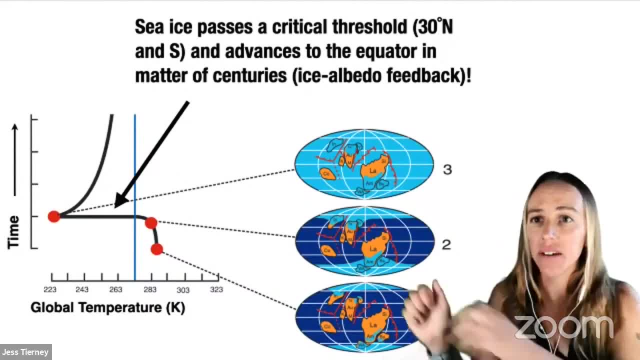 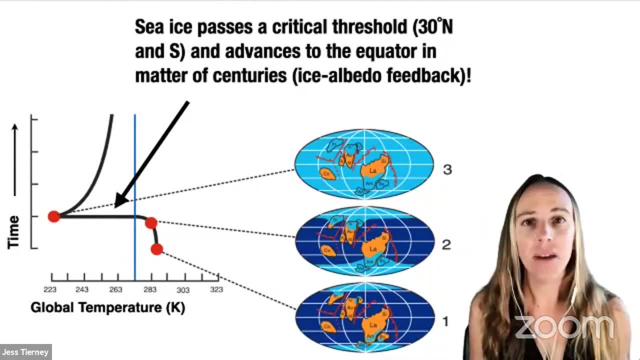 but also to extend sea ice from the poles down and closer and closer to the equator. And what we can do is we can actually simulate this process in a climate model And what we see is that once the ice passes, about 30 north and 30 south. 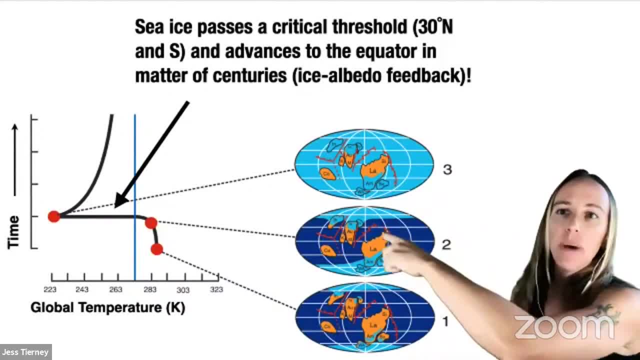 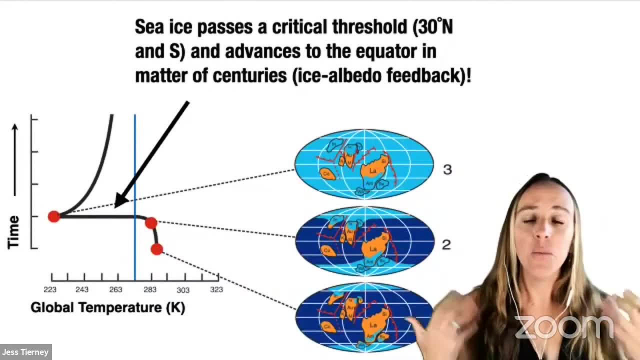 the system rapidly cools down To about minus 50 C global temperature and snowballs completely glaciate over. So there's a threshold behavior. And why is that? It's because once the ice becomes extensive enough, the ice albedo feedback- a positive feedback in the Earth system- takes over. 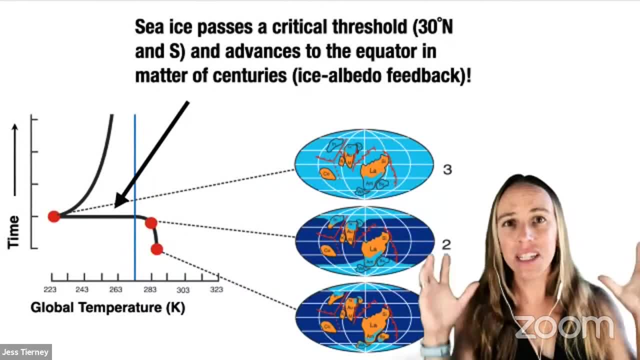 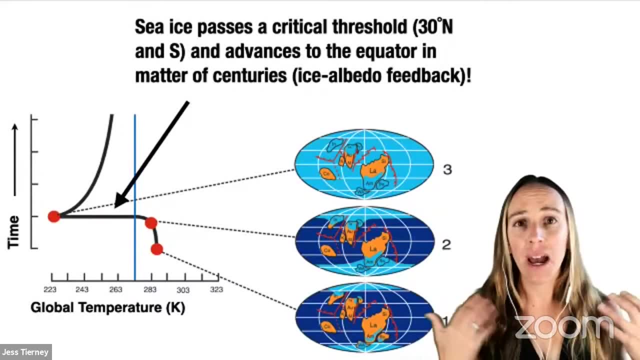 There's so much bright white ice on planet Earth, It's reflecting sunlight back to space, And so, as you have more and more ice, the albedo of the planet increases to a dramatic level, And then, ultimately, you pass that threshold and go into the snowball Earth. 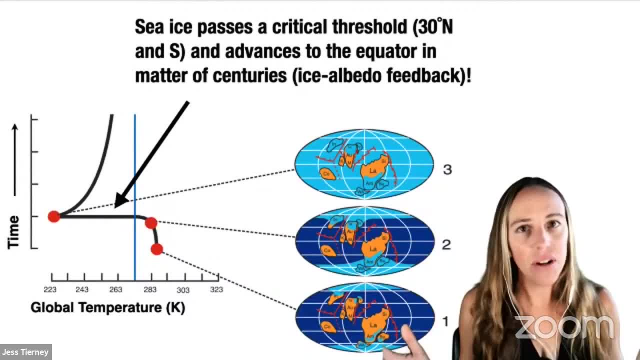 And that's what we call a snowball state, Extremely cold state. Again, we don't know exact temperatures here, but minus 50 C has been thrown out there as the temperature of a snowball Earth Now going out of the snowball. same issue, right. 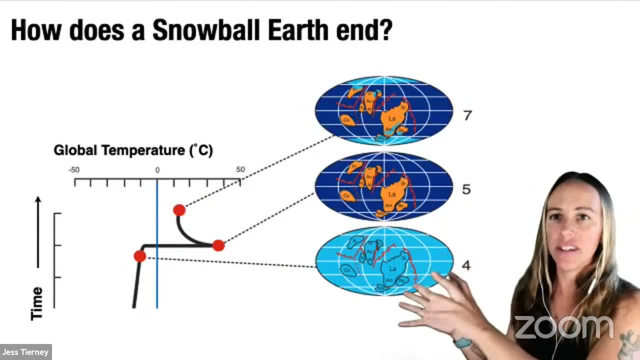 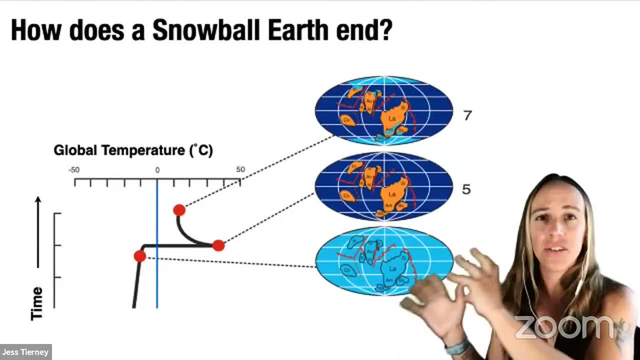 Now we have to warm the planet sufficiently to kick it out of the state. This is a stable state. The ice, you know, the iced over state. You need to warm the planet sufficiently to start to melt the ice. Once you melt the ice past a certain threshold, though, 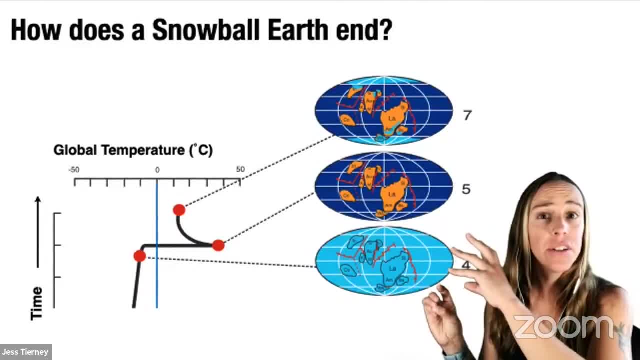 then you have the ice albedo feedback in in reverse. So the ice melts, You have less bright, white, you know surfaces reflecting sunlight into this, into space, and you have a positive feedback. Right, So how do you kick yourself out of the snowball Earth? 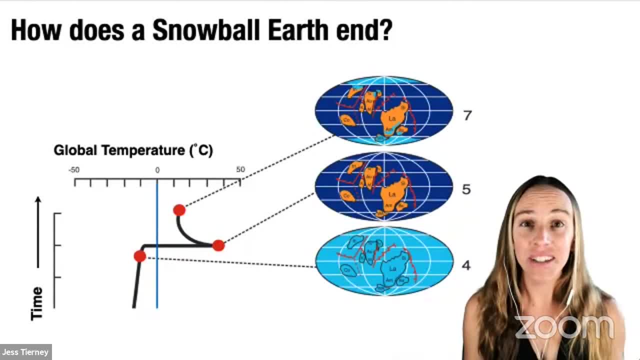 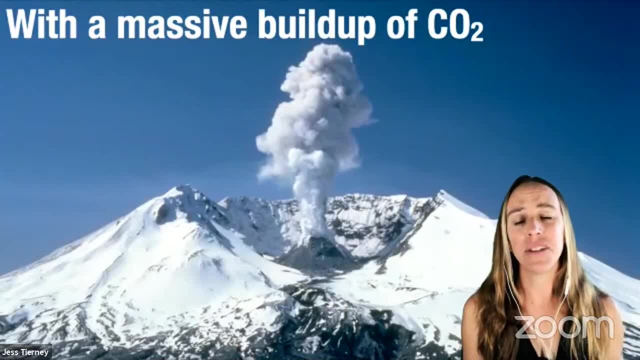 How do you escape? Well, the answer is: you bet Greenhouse gas is a ton of CO2.. So our best estimate is that we must have needed like percent level of CO2 in the Earth's atmosphere To kick it out of the snowball. Where is it coming from? 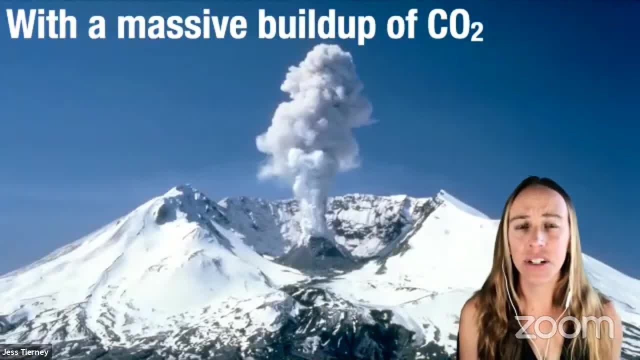 Volcanoes. So even though the planet is iced over, tectonics are still active, And so you do have a buildup of volcanic CO2 over time And slowly, slowly, that's going to build up in the atmosphere. 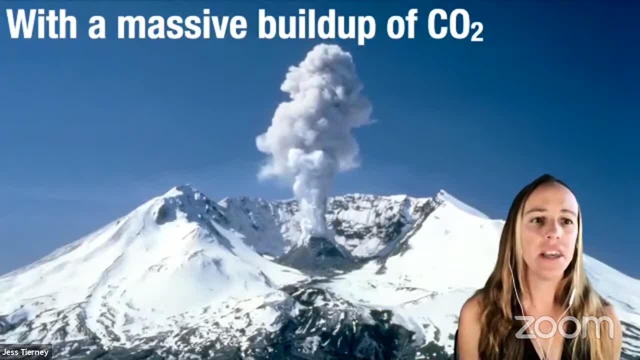 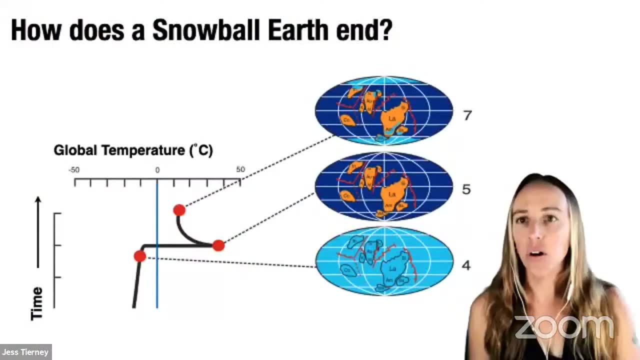 There really isn't a sink for it, because everything's covered up with ice. Eventually, the climate is warm enough to bust out of the snowball state And you might have noticed there's actually an overshoot situation here, where the Earth's temperature pops up to an extreme warm. 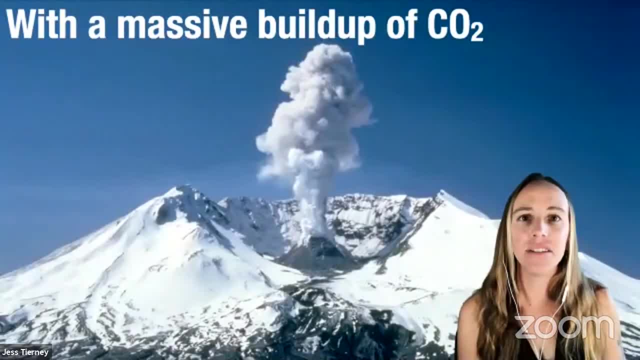 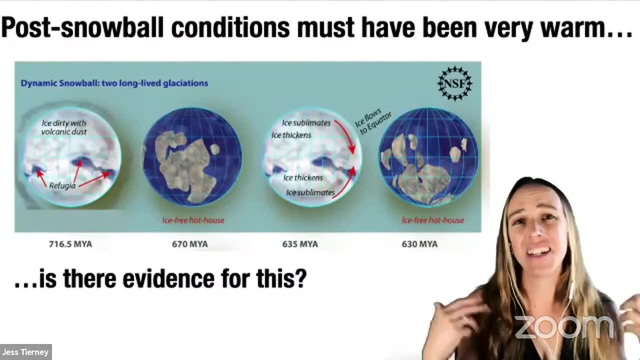 Climate because of the intense amount of CO2 that's in the Earth's atmosphere, And so it follows from this theory that the post snowball conditions must have been extremely warm, And so you actually have this crazy movement of the Earth's climate between ice state. 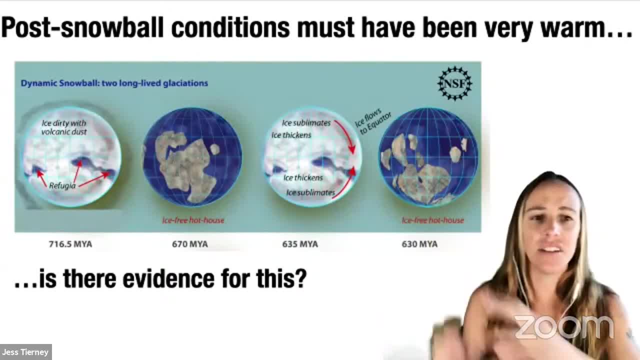 you know, sauna state, ice state, sauna state, back and forth, And through these snowball Earth events, because in order to get out you have to put an enormous amount of CO2 in the atmosphere And then the climate becomes very, very hot. 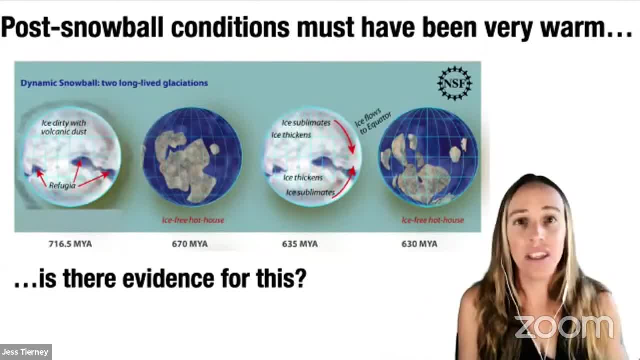 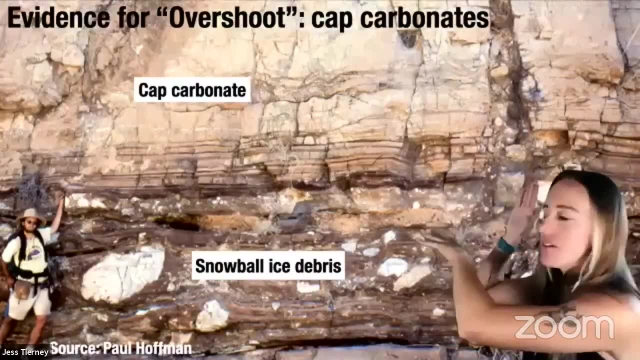 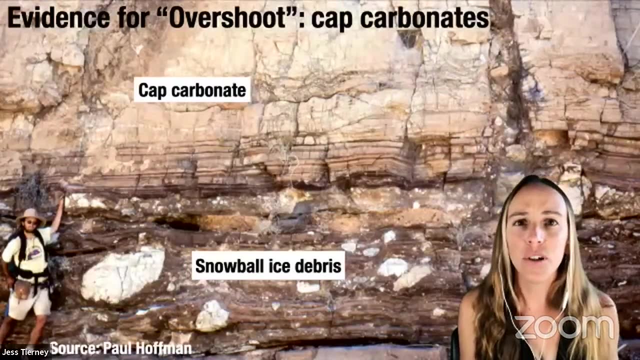 Is there rock evidence for these hot conditions? The answer is yes. We have these spectacular cap carbonate deposits that are sitting right on top of the snowball. Earth debris, Cap carbonates, these bright white limestones, And this is a telltale signature that the climate was warm, because once we really warm up the climate and amp up the hydrological cycle, 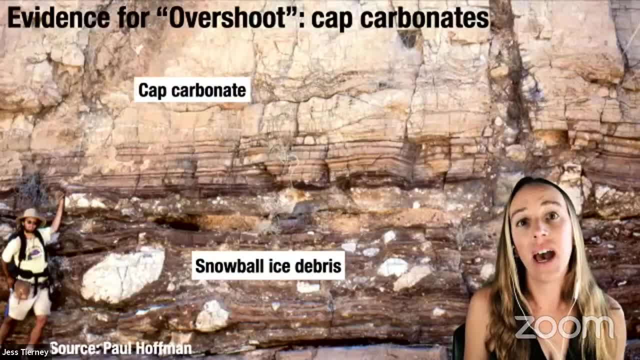 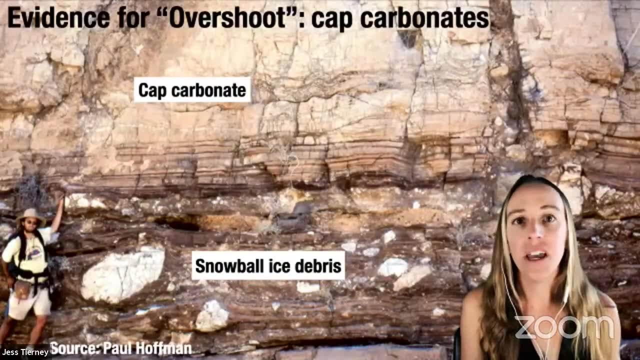 we start to dump a ton of alkalinity from land into the atmosphere And it builds up in calcium carbonate. So this is like telltale signature that this theory is working, that we, that we must be going from a very cold state to a very warm state. 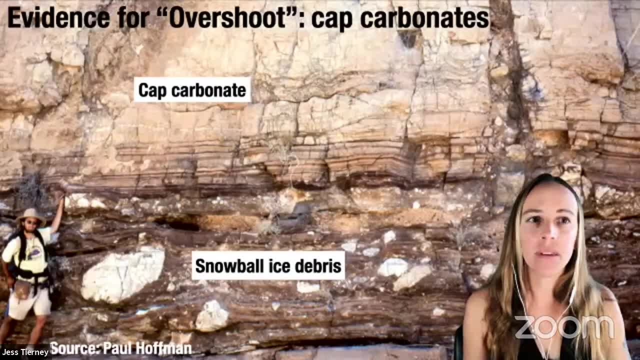 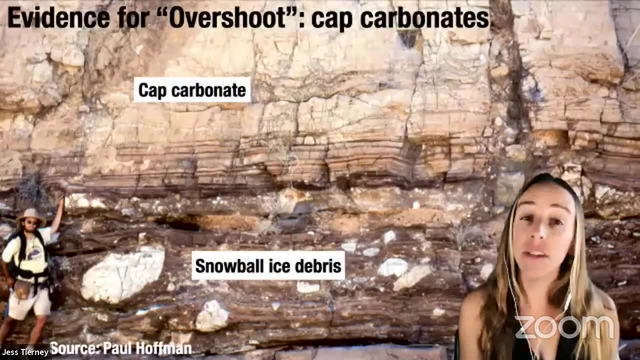 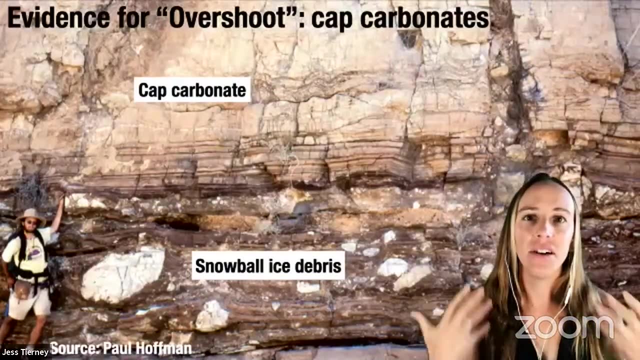 And the culprit is CO2.. All right, So what have we learned from snowballers? We can learn something about the importance of the ice albedo feedback- which is something that is happening today as we are ultimately melting ice sheets Right- And the importance of that non linearity. 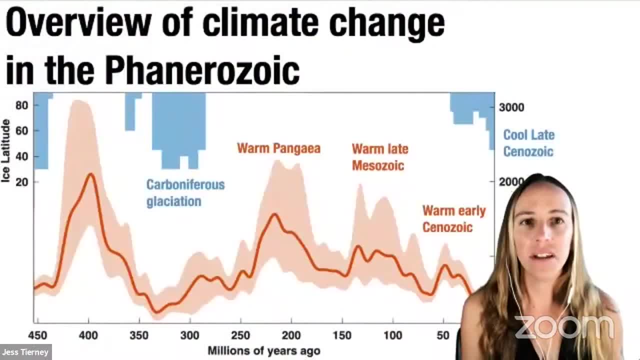 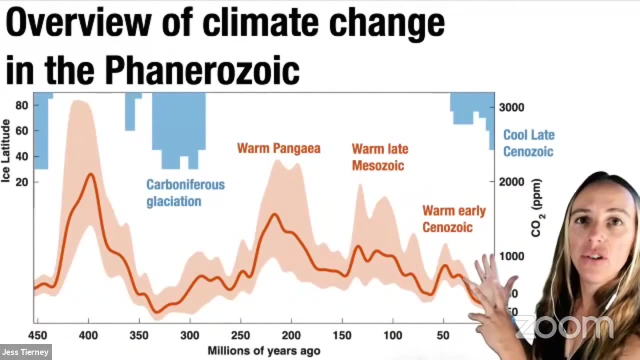 And the importance of CO2, obviously in warming the climate. Now, when we move forward into the phanerozoic, we have more quantitative estimates of what temperature change was like and also what CO2 change was like. So what you're looking at here is a reconstruction of atmospheric CO2 going back 450 million years. 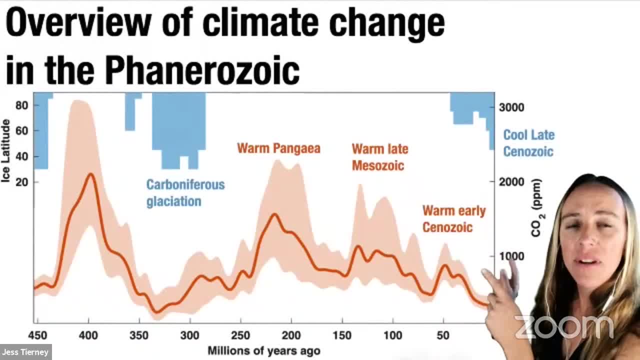 And I don't have time to talk about how scientists do this, but it's an amazing process. We have lots of really cool tricks: using paleo botanical instruments, Paleo botanical indicators, using isotope systems to actually get at CO2. And so we now have a picture- a rough picture still, with a lot of error bars- of how CO2 has changed. 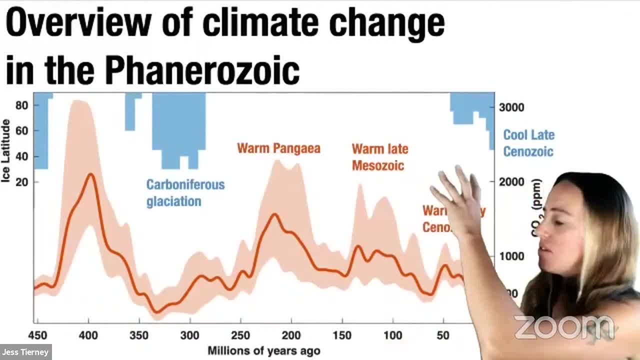 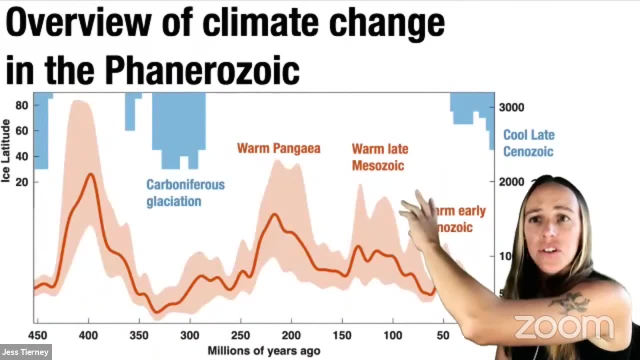 And what do we see writ large? So on top I'm showing the times in blue when there's extensive ice sheets on land. So, going back all the way to the left, we have the Ordovician glaciation and the Carboniferous glaciation, and then the Late Pleistocene glaciation. 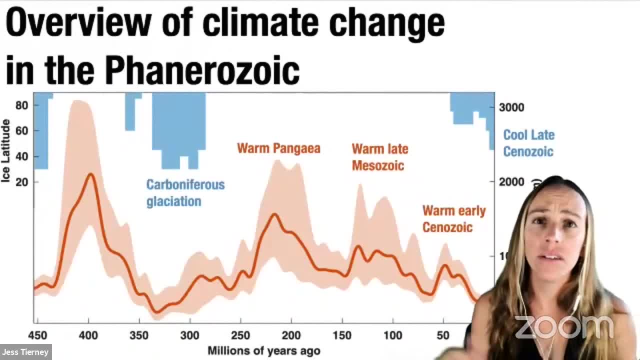 What you can see is, every time that there's a lot of ice on planet Earth, CO2 is low, And then, when there's no evidence for land ice, CO2 is high. So, very simply put, CO2 is in the driver's seat. 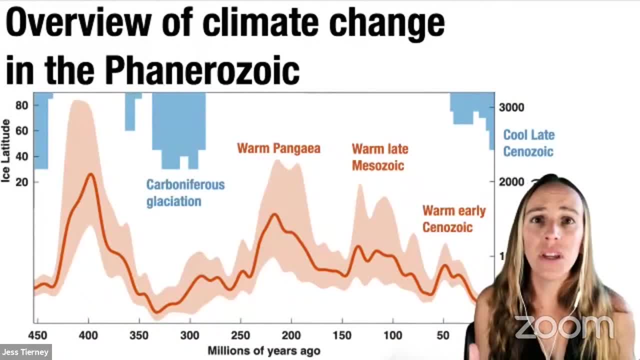 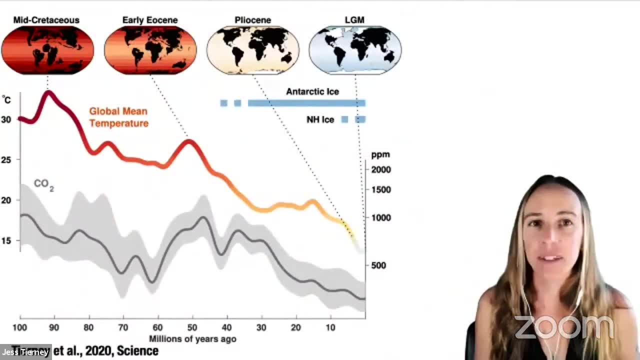 It's ultimately pushing the Earth's system between ice house climates and greenhouse climates. So now let's focus in a little bit on the shorter timescale, the last 100 million years, And actually Margo just showed this picture. So in talking about the Eocene, 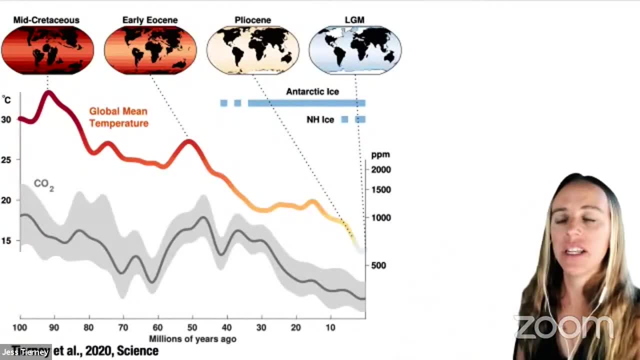 So, but I'll just show you a picture, I'll just go over what's what you're looking at here. So we're looking at a reconstruction of global mean temperature, than that colored line on top, And then CO2 curve, same one that I just showed you. 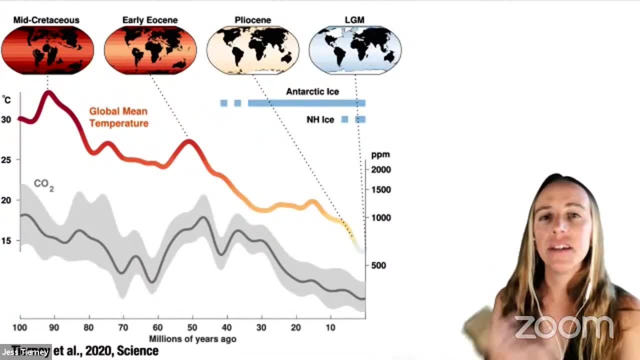 But now we're zoomed in on the last 100 million years, And so what we can see is, over this time school, the Earth's climate has been slowly cooling from an extreme hot house climate in the mid-Cretaceous down into an ice house climate of the Pleistocene global mean temperatures possibly peaking above 30 degrees Celsius. 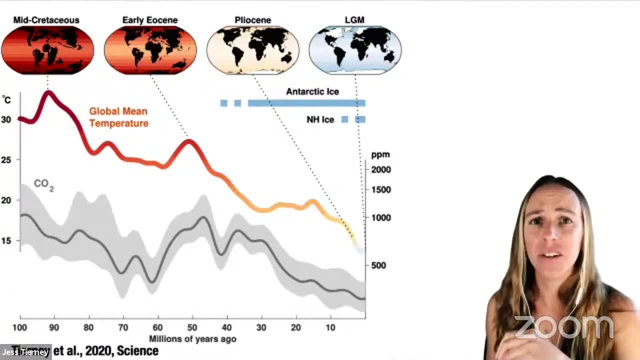 in the mid-Cretaceous. Compare that to present day global mean temperatures of about 14 C. Right, So that's a different climate And CO2 generally measuring temperature, although not perfect, But we can see that CO2 has been declining. And then we see, you know that. 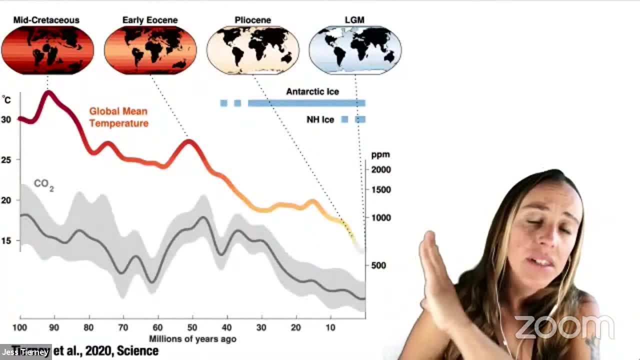 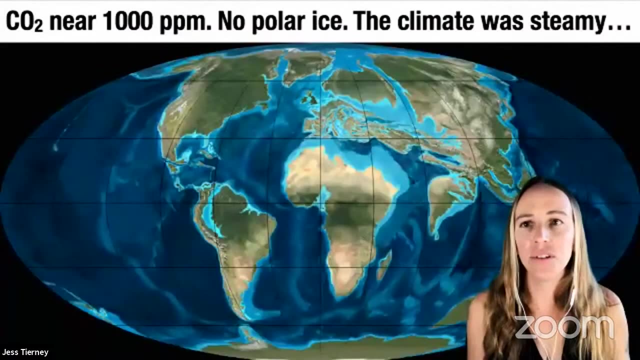 But for a long time before the recent ice house, CO2 was much higher levels. So I want to talk about warm climates now And I am going to focus on the early Eocene, which Margo already introduced to us This time period around 50 million years ago, when CO2 was around about a thousand ppm, maybe higher. 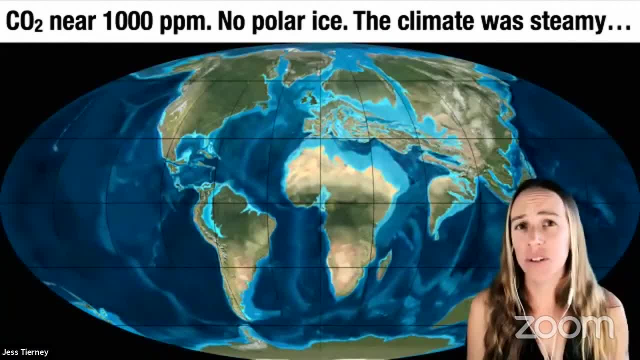 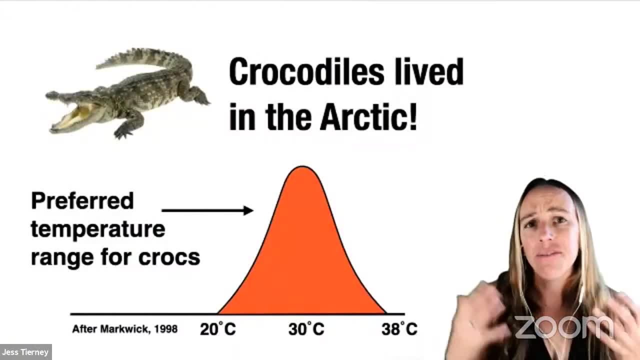 There was no polar ice and the climate was super steamy. We have lots of indicators for how warm the climate was, But we can start with the most basic of ones, like the fact that crocodiles were living and thriving in the Arctic. 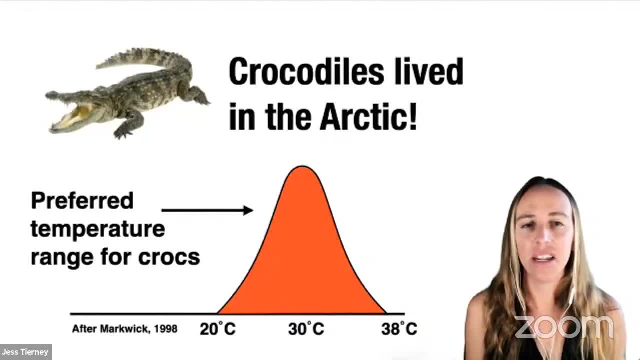 So we find crocodile fossils in the high Arctic dating back to the Eocene, And that's like a first order piece of evidence That it must have been really hot, because these guys are cold blooded, Right, So they don't really do so well below about 20 degrees Celsius. 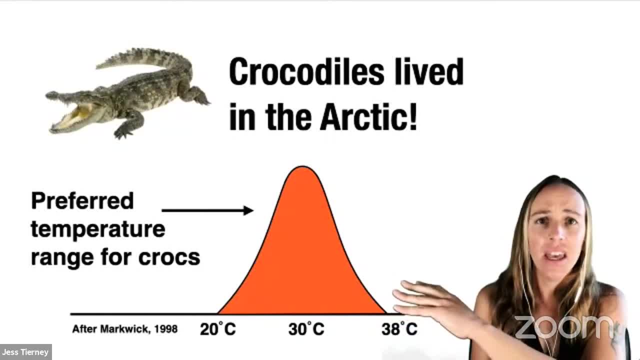 So the fact that they're hanging out in the Arctic and doing OK, it kind of gives us a minimum bound on land temperatures there, that they must have been at least about 20 C on a mean annual level. We also see evidence of palm trees and baobab trees. 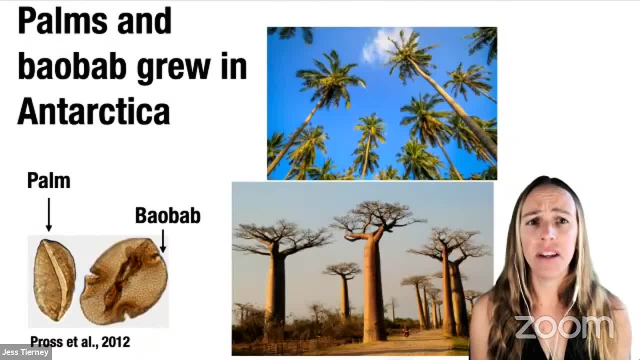 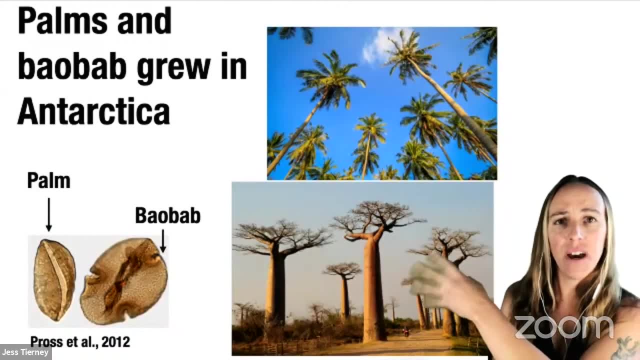 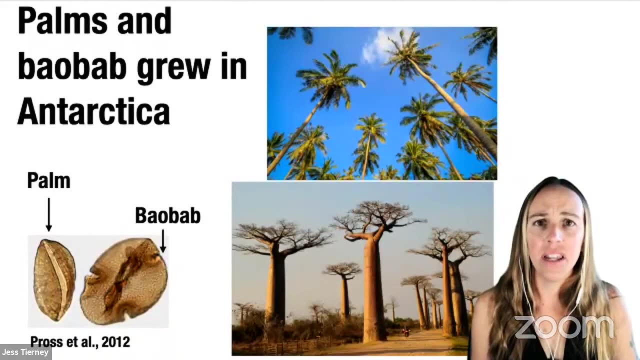 So subtropical trees growing and thriving on the coast of Antarctica. These are some on the far left of phytoliths that are preserved from these trees, and we find them right off the Antarctic coast. So again, a really good sign that the high latitudes were a lot warmer than today. 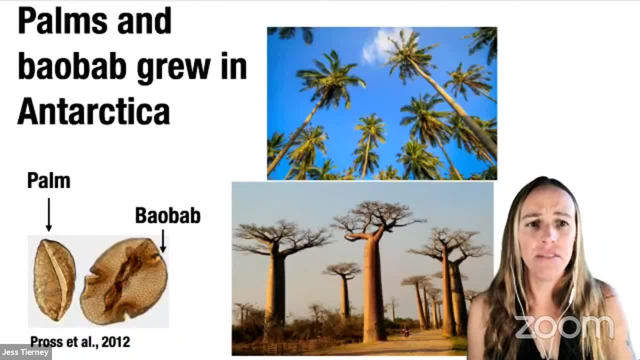 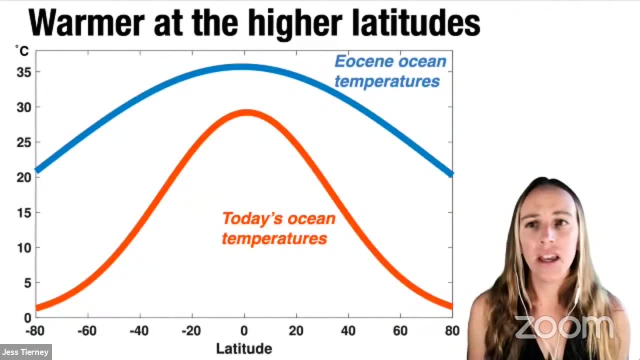 And this, this sort of floral and faunal evidence, actually fits really well with some geochemical evidence that we have concerning what the temperatures of the ocean were like, And so the blue line is our best estimate of Eocene ocean temperatures compared to today's ocean temperature. 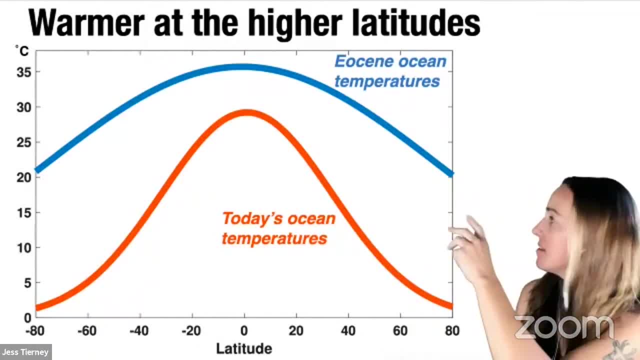 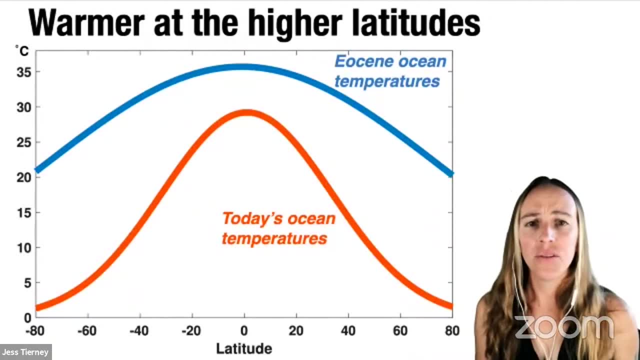 And what you can see is in agreement with the crocodiles and so on. The high latitudes are around 20 Celsius, and then the tropics are warmer as well- sort of around 35 degrees Celsius or so. But you can see that there's enhanced warming at the higher latitudes and that is a feature of warm climates. 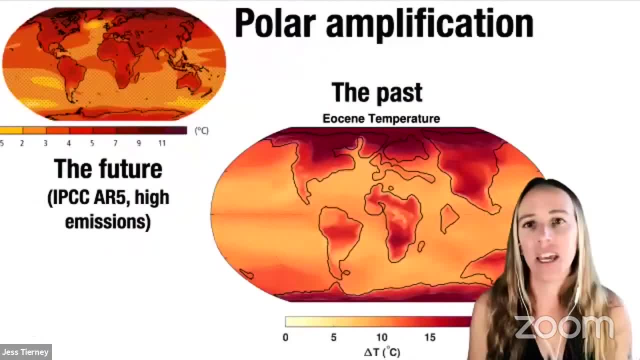 And we call that feature polar amplification. polar amplification: more warming occurring at high latitudes, And this is a very typical response To elevated CO2.. And so here, what I'm showing you is a model simulation of the Eocene. 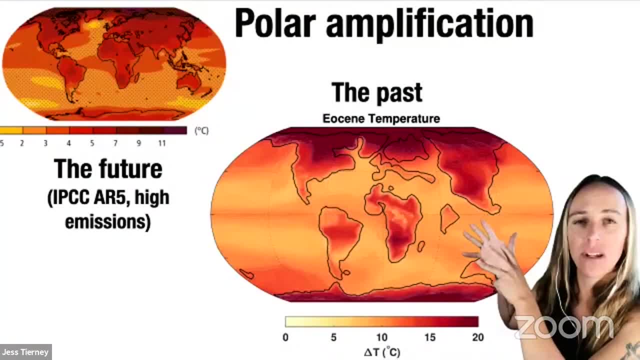 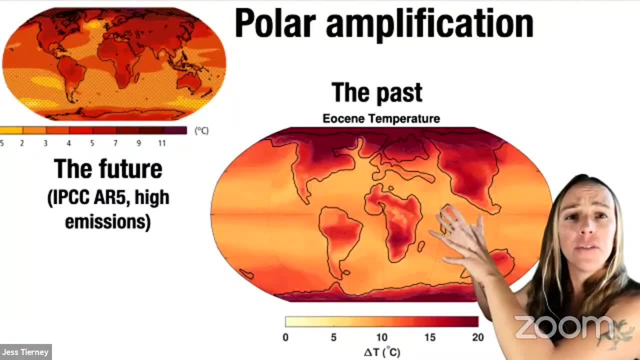 This is the change in temperature relative to the pre-industrial And then comparing in the corner to the prediction from the last IPCC report for what temperatures look like under a high emission scenario, the RCP85 scenario, And what you can see is, even though the continents have moved around, the basic pattern is the same. 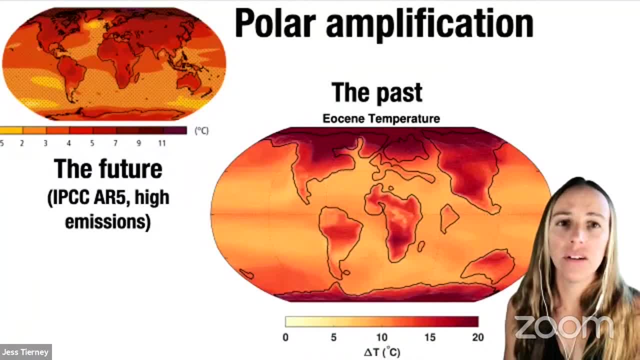 The high emissions, The high latitudes warm more than the low latitudes. The land warms more than the ocean And Paul Veldez tested on this yesterday that, basically, you know well, paleogeography is important for regional climatology. 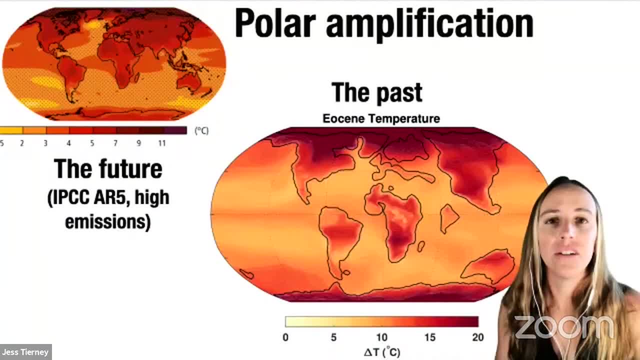 Moving the continents around doesn't really change global metrics like the global latitudinal pattern of polar amplification or global mean temperature changes, And for that reason we can use the past, We can use paleoclimates, to really learn about these physical processes. 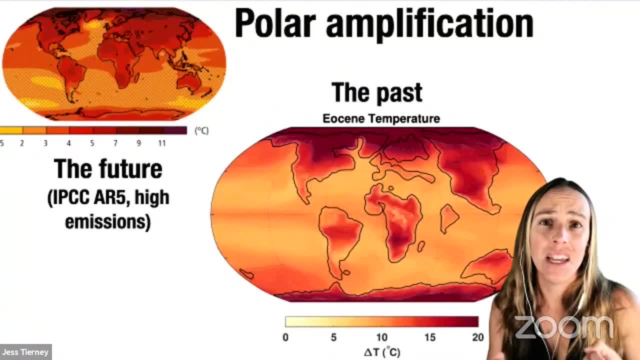 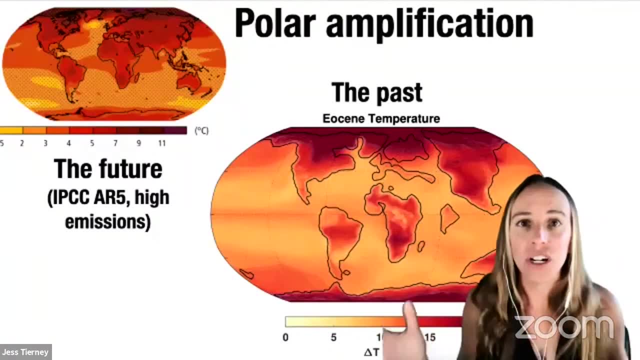 The physics of the climate system stay the same, And so you can see the remarkable similarity between these patterns, which indicates you know what's the shared forcing here? It's CO2.. So you know why is polar amplification happening. 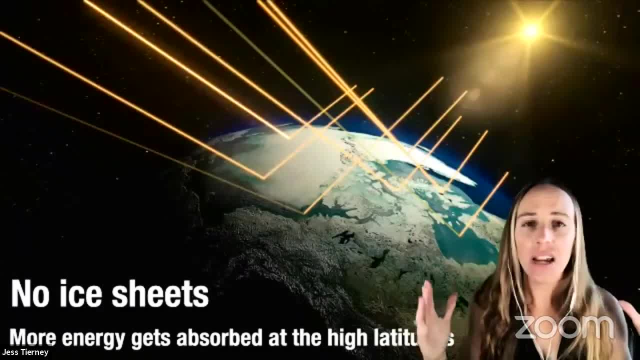 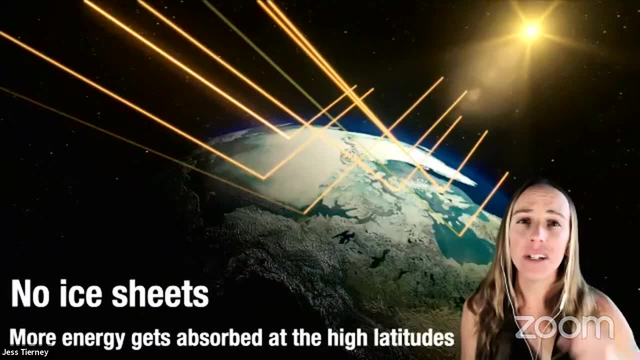 So first order, right you have, if you get rid of the ice sheets at high latitudes, right, you warm them up by a lot because those ice sheets- again ice albedo feedback- are reflecting sunlight back to space. So once you take them away, more energy is absorbed. 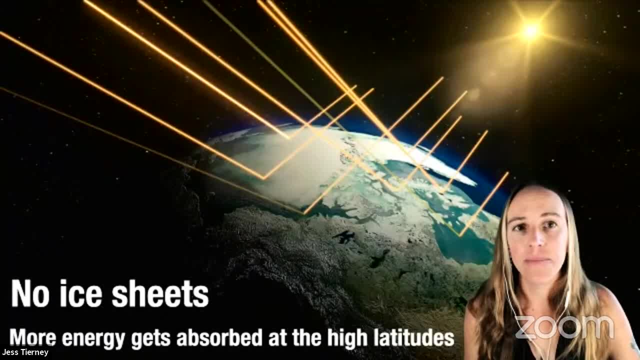 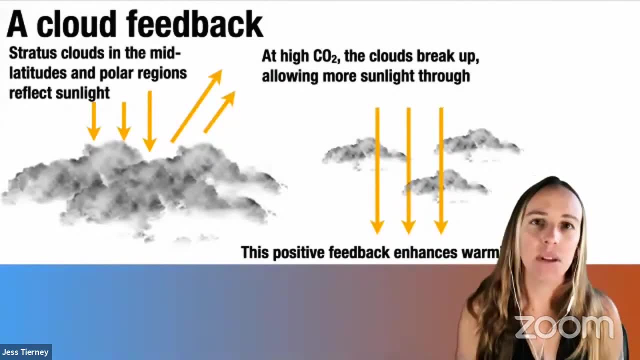 And this is one of the reasons why we see polar amplification. But another reason that we're increasingly appreciating actually has to do with clouds. In the last few years there's been a lot of research looking into the role of clouds, and particularly the low stratus clouds, the stratus decks that hang out in the subtropics and in the polar latitudes, and the role they might play on the energy balance of planet Earth. 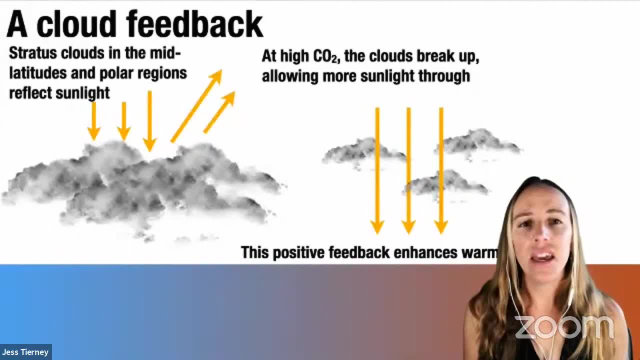 So these particular kinds of clouds, stratus clouds- they reflect sunlight, They're bright and white and they're low. So sunlight comes in, it bounces off and goes back to space. So their general role in the climate system is to cool the planet down. 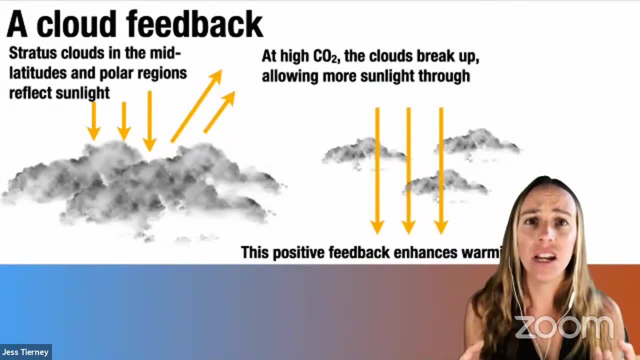 But at high CO2.. What happens is these stratus decks start to disintegrate, They break up, They essentially rain out, rain away And more sunlight can then come through, which means that this is a positive feedback. At high CO2, you break the clouds up and then you allow more sunlight through and you warm even more. 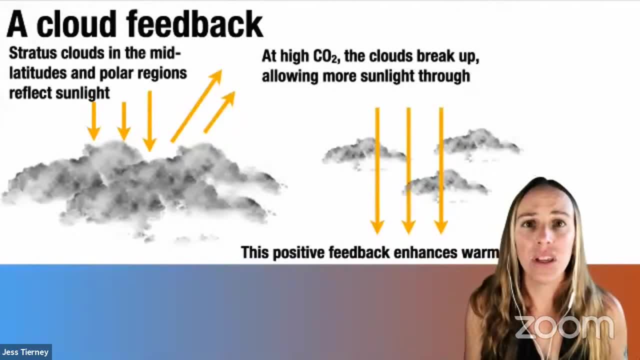 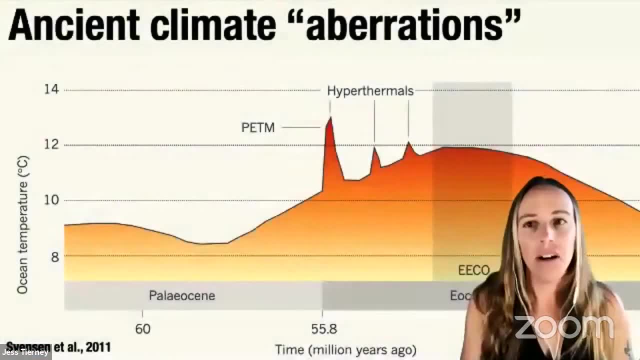 And we're now learning that this is a key element of explaining polar amplification and warm climates like the Eocene, as well as in our future. All right, So now I want to focus in on what we call astrophysics, And I want to talk about some of the collaborations for rapid climate change events that represent this sort of extreme but temporary excursion of the climate system. 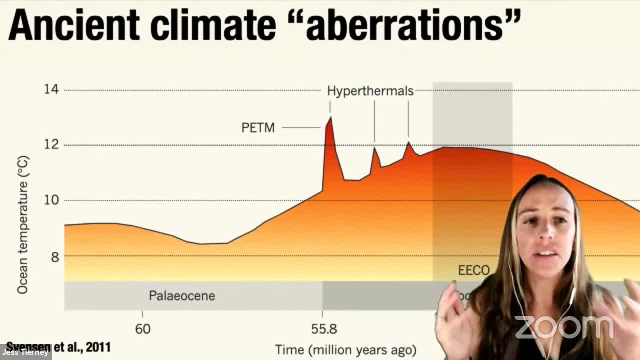 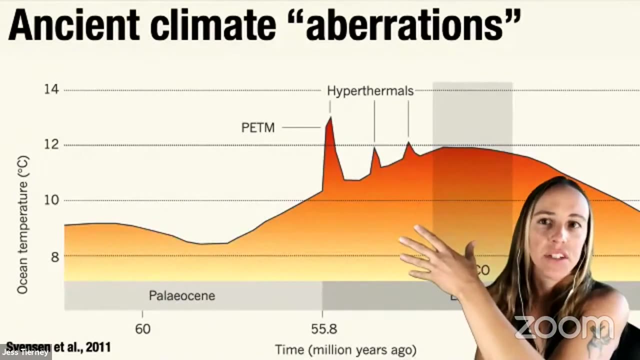 And I want to talk about the Paleocene-Eocene Thermal Maximum. So Danielle this morning already introduced some of the effects that the PETM had on ocean ecosystems as it was a major acidification event. So PETM and its sort of sister, hyperthermals as we call them, and that's sort of self-explanatory. 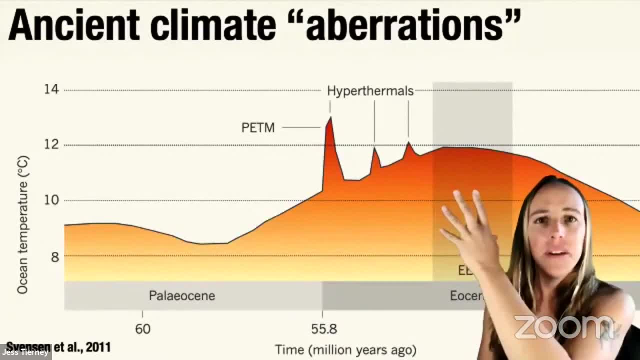 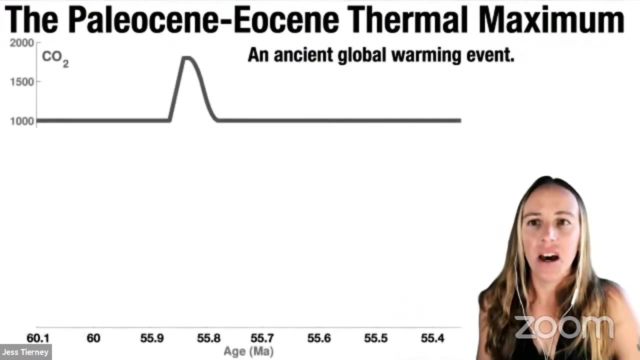 are happening right before us. They're happening right before the peak warmth in the early Eocene climatic optimum, And so about 55.8 years ago, a million years ago, we have the PETM event And just as a review of what's happening during this event, basically, first of all, CO2 bumps up temporarily. 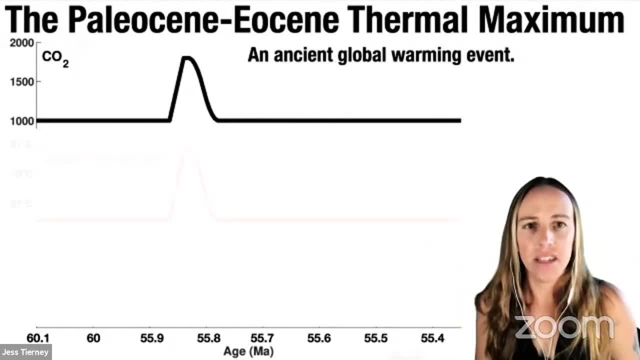 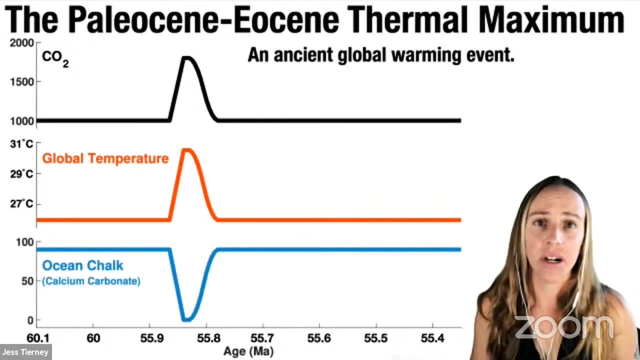 We think this is due to volcanism in the North Atlantic, And then, at the same time, we see a bump up in global temperature And we also see a decline in ocean chalk. We see a sharp drop in oxygen carbonate, which Daniella talked about this morning. 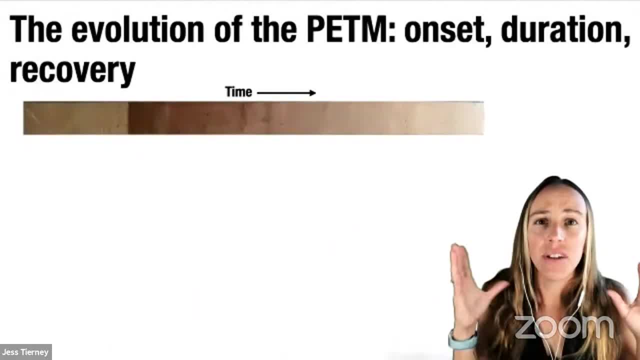 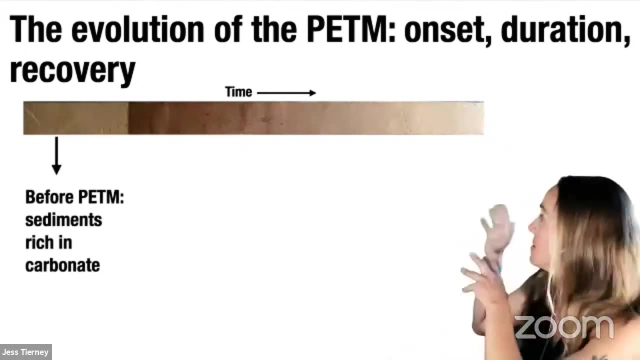 And in fact, as she pointed out, you can see the PETM straight up in the sediment cores that are collected to capture the event. You can literally see it in the color of the mud, which is spectacular. So before the event, on the far left here we have sediments that are rich in calcium carbonate. 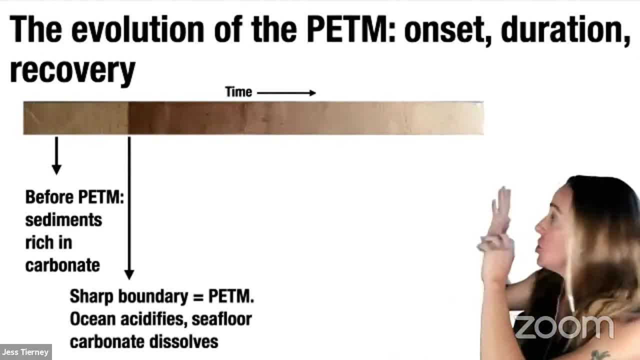 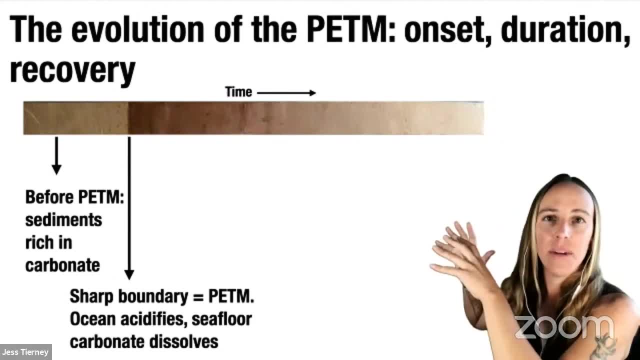 Everything's fine. And then boom, we hit the event. There's a sharp boundary, The PETM is starting to come, TM is starting and the ocean acidifies, And so all that bright white carbonate that's in this sediment core has been dissolved away because the pH has dropped. And then we see that this 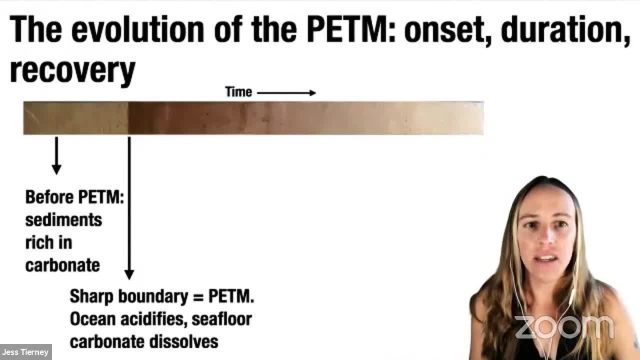 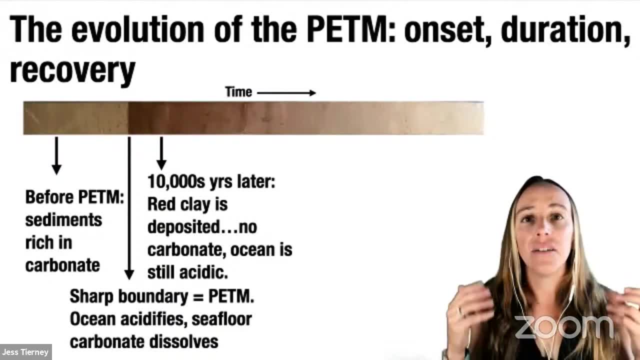 red clay kind of take over. That's what's left, And the red clay hangs out for a while. 10,000s of years later, we're still not recovered. So it does take a while for the earth system to buffer carbon dioxide, And that was a topic that came up earlier today. It's really on geological. 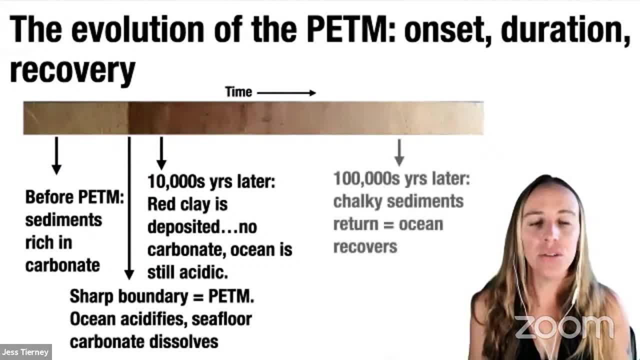 timescales right Now. finally, you see the return to the chalky sediments 100,000 years later. So the total recovery time, which we can directly learn about from the PETM right, is, on that order of time, 100,000 years. And that's when all of the earth's mechanisms for 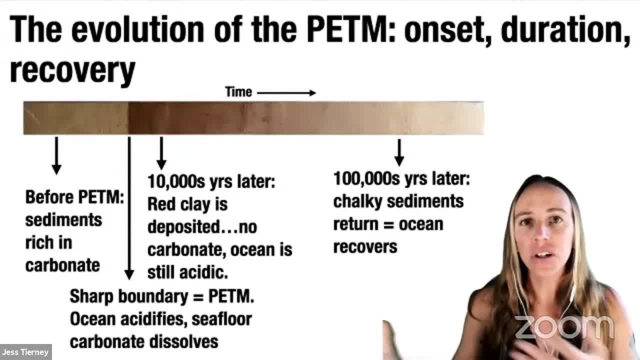 buffering CO2 come into play and can return the system back to normal. So from that we're going to talk a little bit about how we can return the system back to normal. So from that we're going to talk a little bit about how we can return the system back to normal. 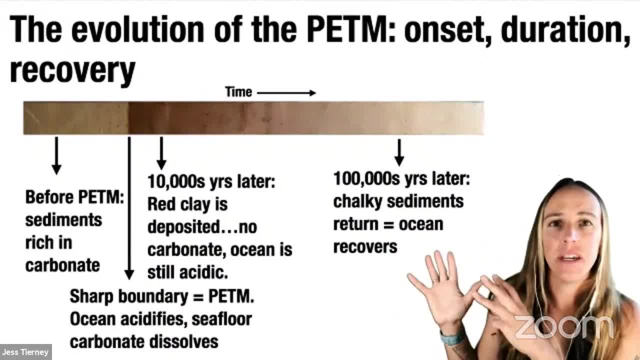 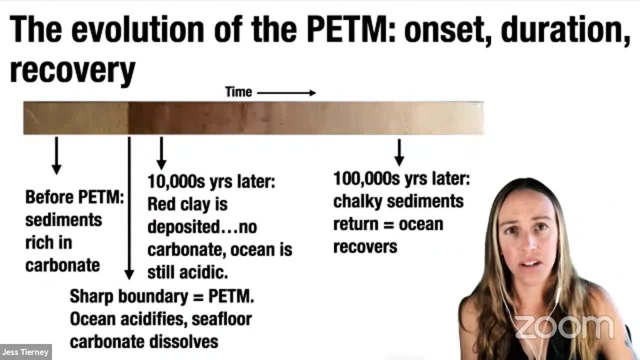 So from these you know beautiful sediment cores and study the PETM. we can learn a lot about how the earth system processes a sudden increase in carbon dioxide, which is obviously relevant for where we're headed. I just want to put the context of the PETM you know directly. 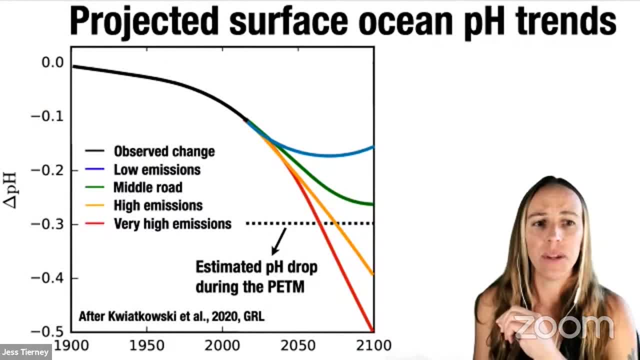 next to some of the future predictions for surface ocean pH. So this is this is a sort of a new prediction of of of possible trajectories of ocean pH by 2100, um, with the colors corresponding to the amount of CO2 we emit. So the blue would be the lowest emissions. 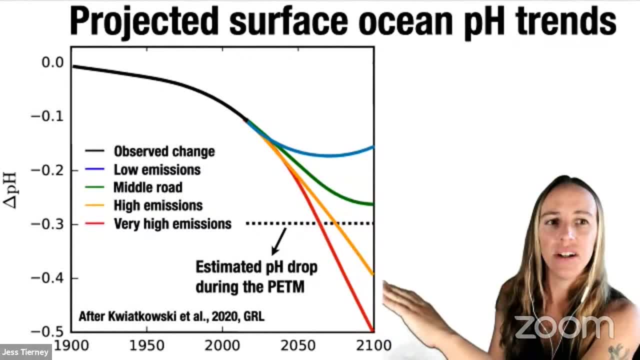 scenario And the red is the highest emission scenario And we estimate that the drop in pH during the PETM was about 0.3 pH units. Now it doesn't seem like very much, but remember that pH is a logarithmic scale and that is a ton more acidity in the ocean and organisms are. 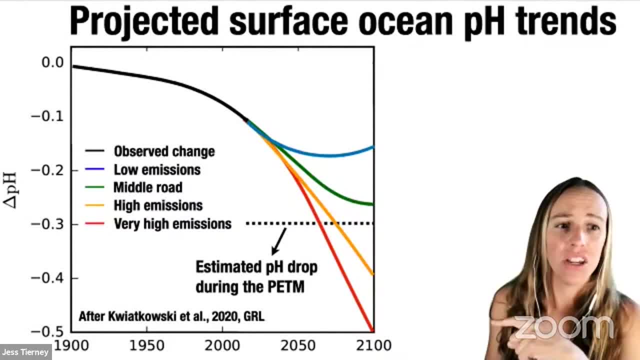 are definitely not adapted to deal with that big of change in acidity. And so we can see- which is shocking to me- that if we continue on a high emissions scenario, we will actually meet, if not exceed, the PETM level acidification before 2100.. So this is something that your children will. 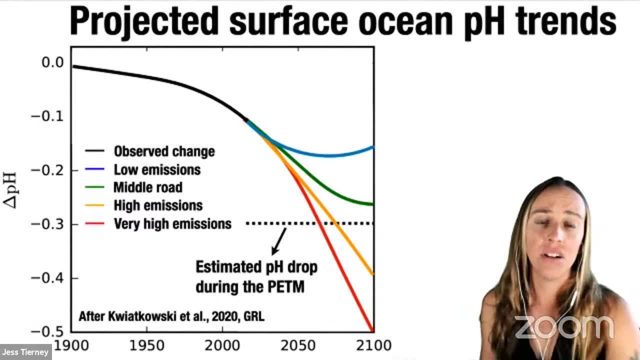 see in their lifetime. We could see the complete destruction of our coral reefs of calcifiers in the ocean on a human timescale. So pretty scary, So we don't want to do that, Right, All right. So one thing I'm really interested in: 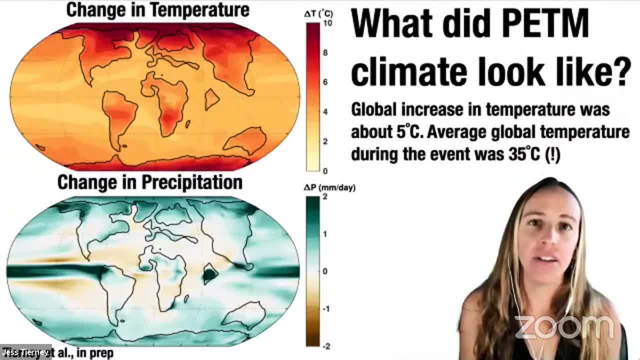 is: what did you do? What did PETM climate look like? You know, what I'd love to do is get in a time machine and go back and be like whoa, what's going on, Right? But of course we can't do that, So we have. 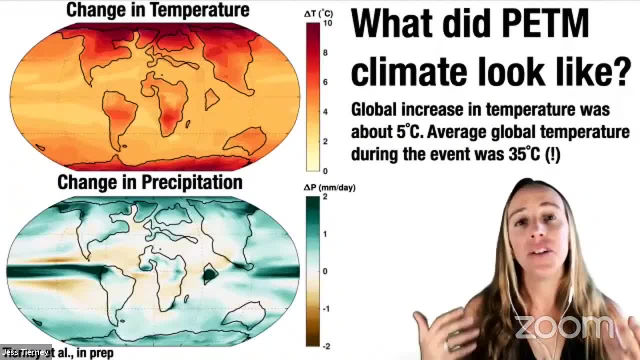 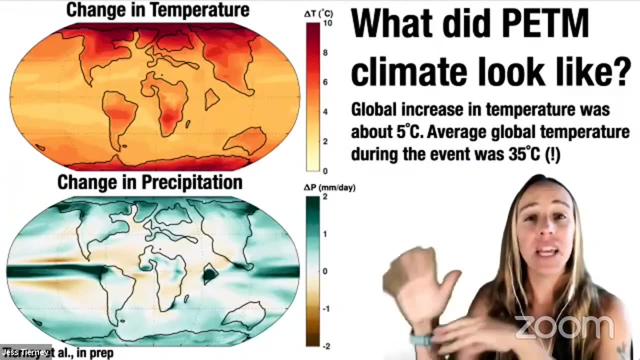 to reconstruct what the PETM looked like from geological information and from climate model simulations. So what you're looking at here on the left is a blend. So Dr Eddie Otto-Blesner yesterday mentioned that we're now using this technique, where we're actually blending proxy. 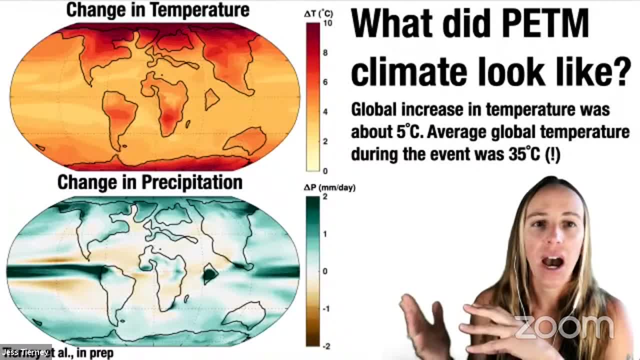 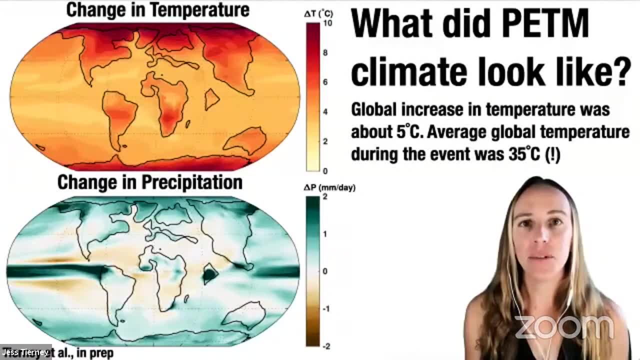 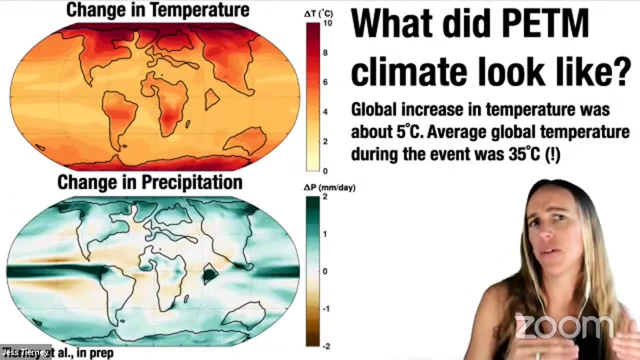 climate information So we can get a full field picture of what the PETM looked like. So the panel on the top shows you the blended estimate of the change in surface air temperature between the PETM and, right before the event, what we call the pre-PETM. So what you can see from that plot is polar amplification. 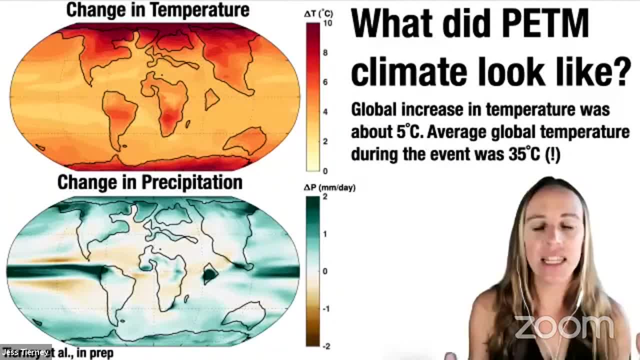 right. So we see a much bigger change in temperature in the high latitudes up to 9 or 10 degrees C or so than the low latitudes up to 9 or 10 degrees C. So we can get a full field picture of what's happening in the high latitudes. The global increase in temperature is somewhere around. 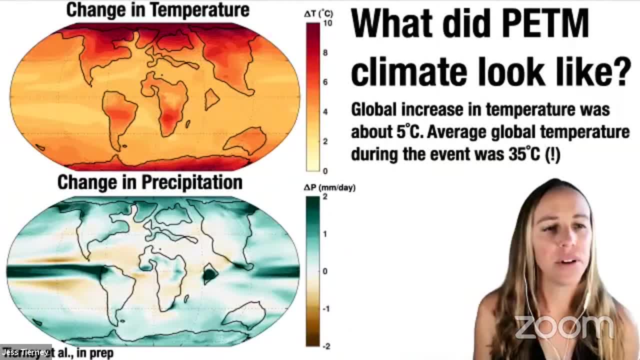 5 degrees Celsius. This actually agrees pretty well with previous work, But something that's a little bit scary to me is that our best estimate right now is coming out as an average global temperature of about 35 C in the absolute, which is really really freaking hot. So we'll see if 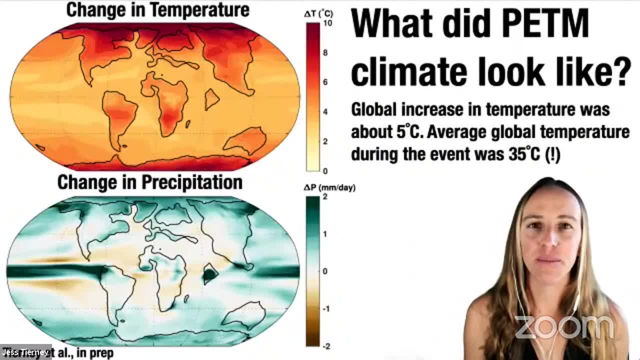 that pans out. This is work in progress. I just wanted to show you something hot off the presses, but that is super toasty, So that's a bit of a surprise. and it's a little bit of a surprise, but it's a little hotter than previous estimates have put it up. Now we talk a little bit about. 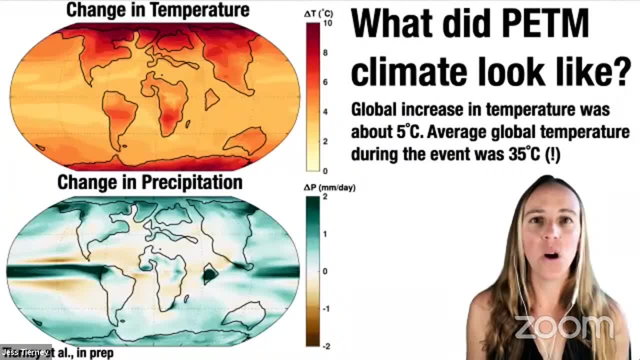 hydrological cycle. I'm glad that it has come up, because water is so important in thinking about climate change, And so with this technique, we can also get a blended estimate of the change in precipitation in the PETM, And what you can see is that there's a lot of that sort of blue. 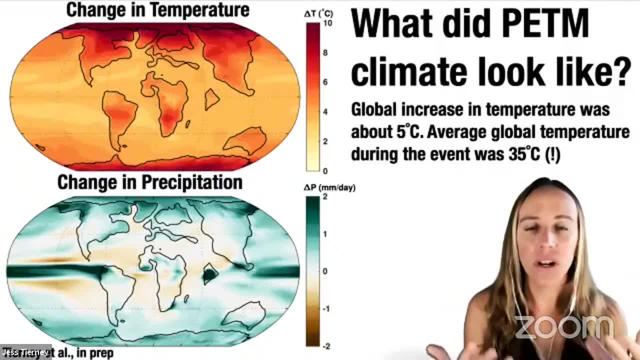 green color. Basically, most places are getting wetter, which makes sense because we're warming the climate and overall warm air holds more water And overall you expect things to get wetter, But in fact it's a little bit different, So we can see a little bit of a change in precipitation. 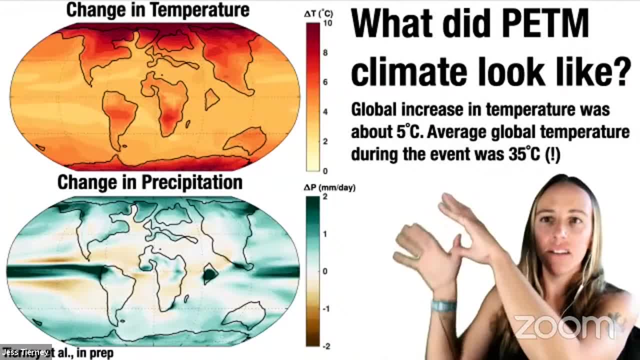 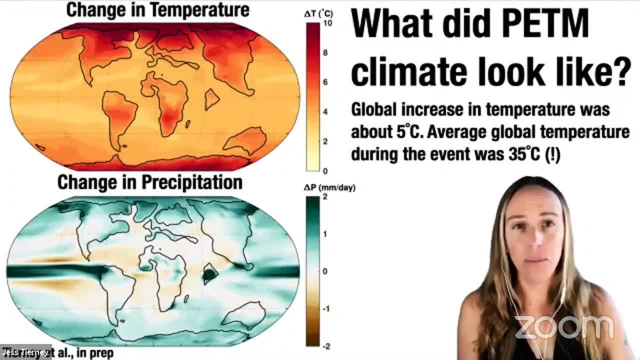 in particular, the tropics are much wetter and the high latitudes are much wetter And there's a little bit of drying in the off equatorial regions, And that actually fits again with what we think happens under high CO2 worlds And it also looks a lot like some of our future. 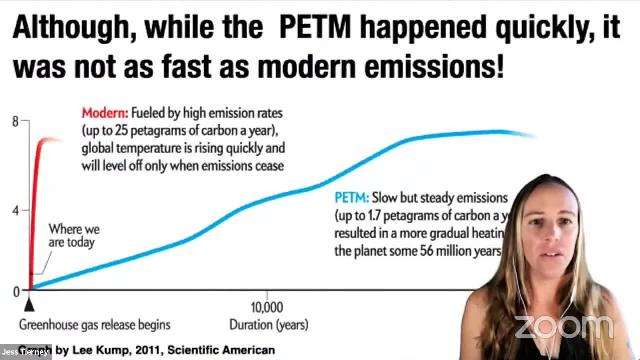 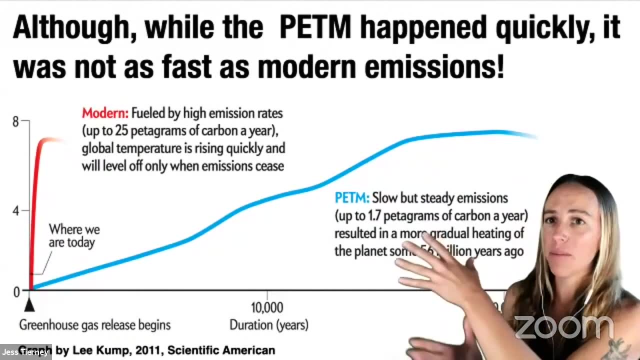 projections of precipitation change. So this point was made earlier by Alan and Diana and Daniela, which is that although the PETM was extreme, it's important to remember that it was still not as fast as what we're doing right now. So the blue line represents the rate of warming during the PETM And the red line represents the 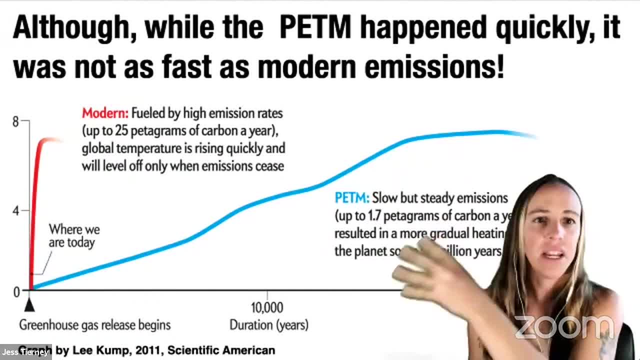 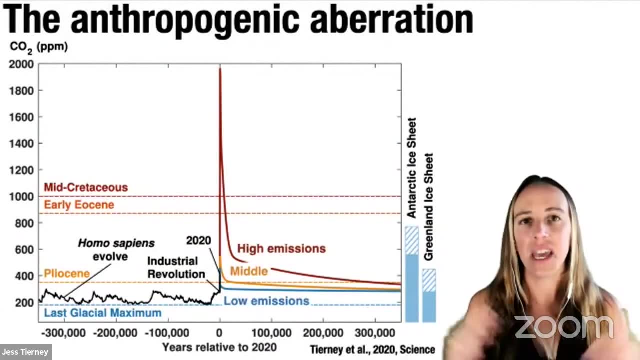 rate of warming that we're doing right now. So the current rate of emissions of CO2, emissions of warming- is an order of magnitude faster than the PETM, which is pretty extraordinary. So it is a really extreme thing we're doing to the climate system right now. We can call it the anthropogenic. 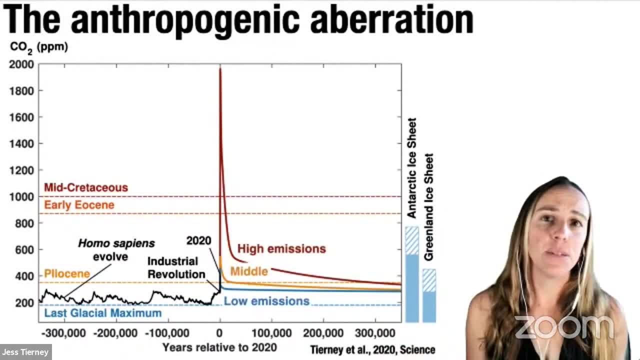 aberration And it's a really extreme thing we're doing to the climate system right now And we can call that an anthropogenic aberration And and it's sort of a fun thought experiment. One thing we wanted to do is visualize what the anthropogenic aberration looks like on the geological timescale. 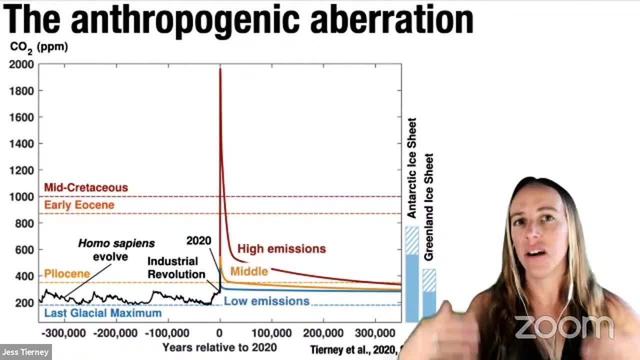 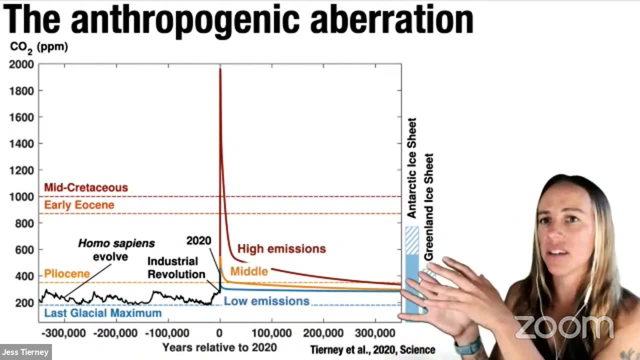 Right. So if you were to zoom out and and meet- you were geologist million years in the future and we're looking back on the anthropogenic aberration, what would it look like? So, to give some context to that, what we did in this plot is we actually ran out the the emissions trajectories. 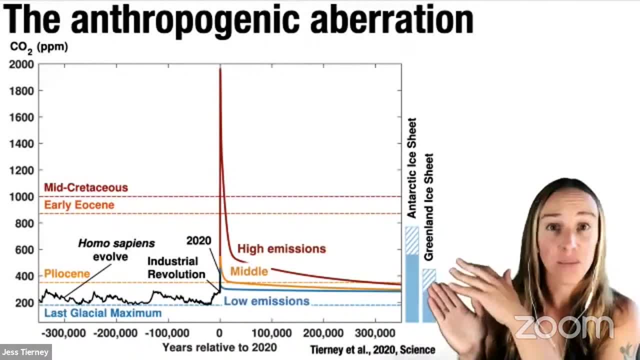 low, medium and high to 400,000 years. plus. It's antonym particularlywal tabloid weather forecast. So we thought we did this first, and then you ran out. So there's these initial videos showing that the CHAN queens Transformers seem to hold you know theDAY category that's going to rise. and then you sayja TrueChat. 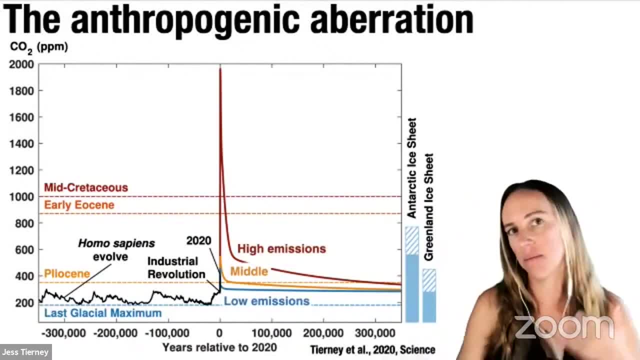 to see what happens to co2 as your system starts to process it. you know, ultimately the earth system will recover, right, we have, there's these natural processes that buffer co2. the problem is, if you look at the x-axis, the time scale right. so the time scale is relative to 2020 and you can see. 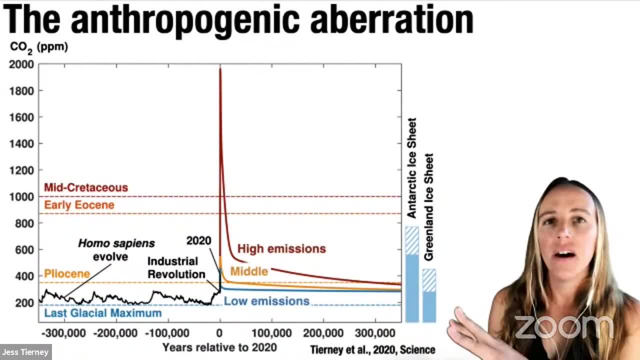 that our species evolves around 300 000 years ago and we have spent our entire existence on planet earth between co2 levels of 180 and 300 ppm. that's it. we're an ice age species. we know nothing about these warm climates, we've never even felt it, and so, all of a sudden, now you see industrial. 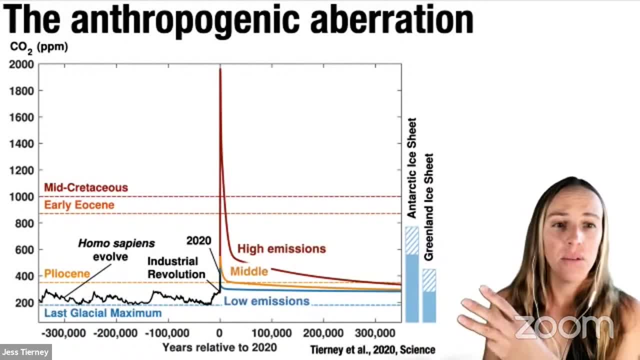 evolution 2020, uh, 2021. now we're already outside of the envelope of co2 levels, uh, that we've seen in the last 300 000 years. and then, of course, we have these three very different trajectories. low emissions- you know, we pop up, but then we get. 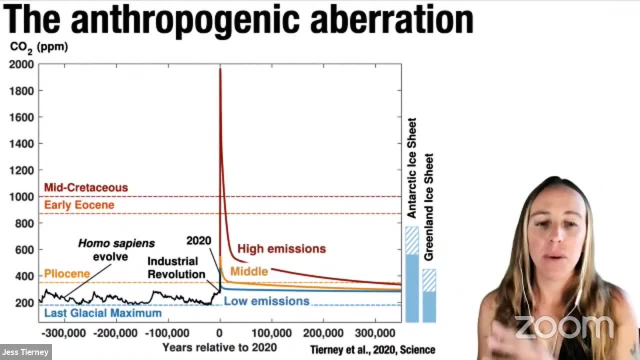 things under control. control Middle emissions, we pop up to levels that are above the Pliocene three million years ago And you can see that there's sort of a long tail of recovery. And then the high emissions scenario is pretty terrifying. right, That would put us at CO2 levels that possibly exceed things. 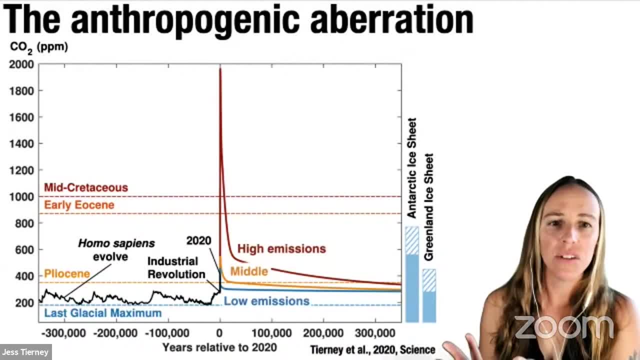 that we've seen in the hothouse climates or are comparable to them, like the early Eocene or mid Cretaceous, And it takes tens of thousands of years to even come down on that steep slope and then all the way out to multiple hundred thousands of years to completely. 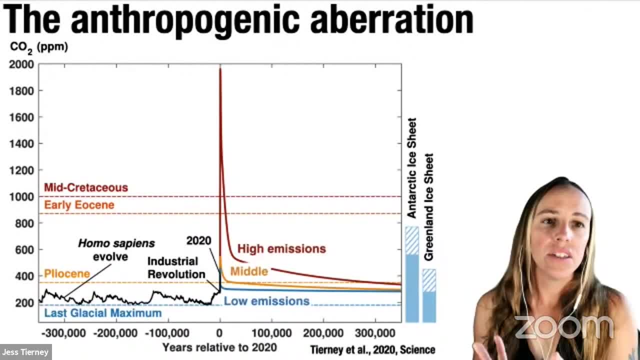 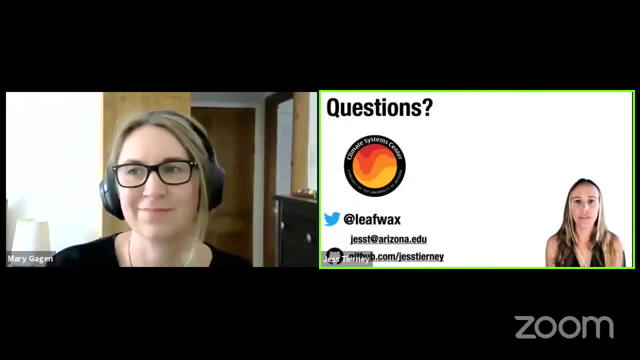 go back to normal. So on the Earth system timescale, this looks like a blip, But for us and the other species that we share this world with, it is actually a state change. All right, so with that I will end, and I'd be happy to take some questions if there's time. 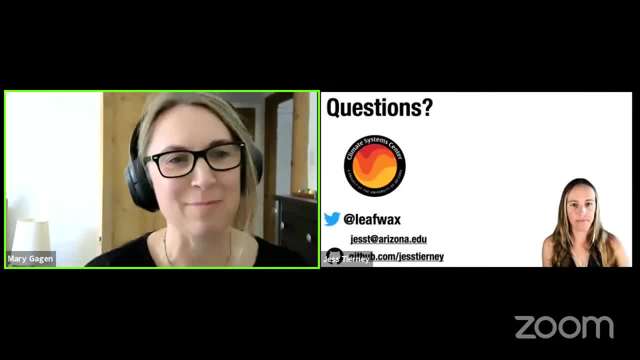 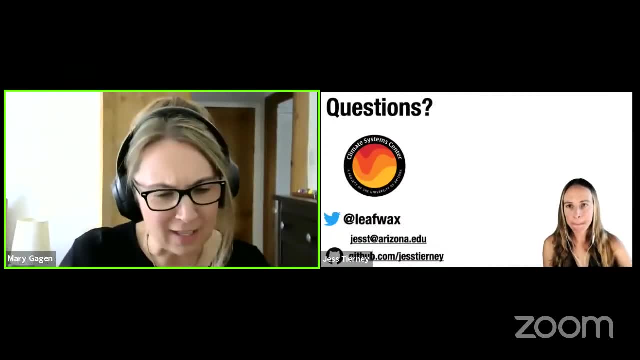 Thanks so much, Jess. Yeah, definitely gonna keep us here for a couple of questions, if that's okay. I'm gonna start with a couple of more general questions, Jess, that are sort of bringing together a few different points both from the panel and from the chat. I don't know if I could. 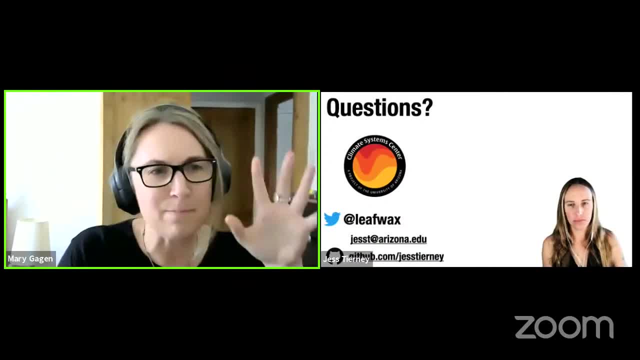 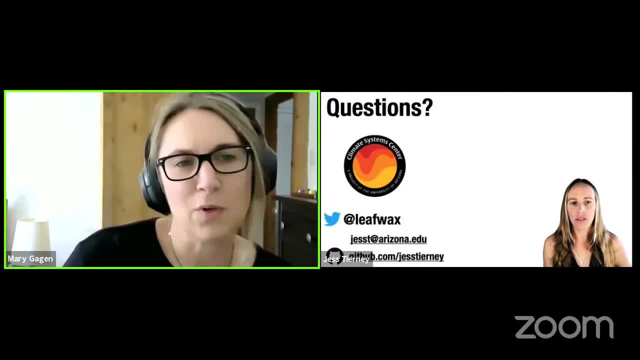 ask you to go back to your lovely kind of Phanerozoic summary plot that you showed a few times with the kind of evolution, temperature evolution through the Phanerozoic. Don't worry if not The one at the beginning, Yeah, the one right at the beginning. and then you showed it. 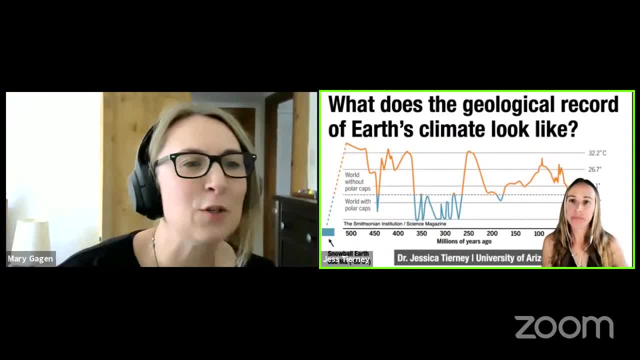 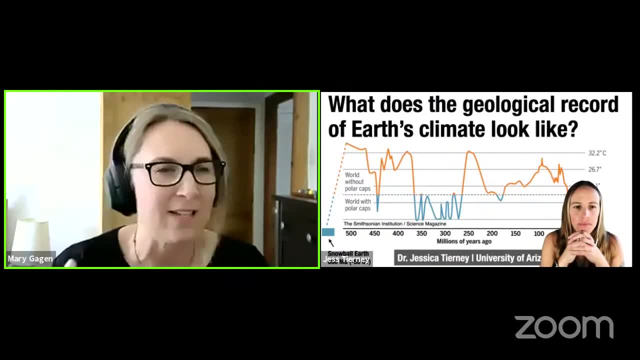 again at the start. Go back, There we go. I just wanted to give you a chance, um to talk a little bit about what are the greatest sources of uncertainty in this. which axes hold the uncertainty, and where does that uncertainty come from? 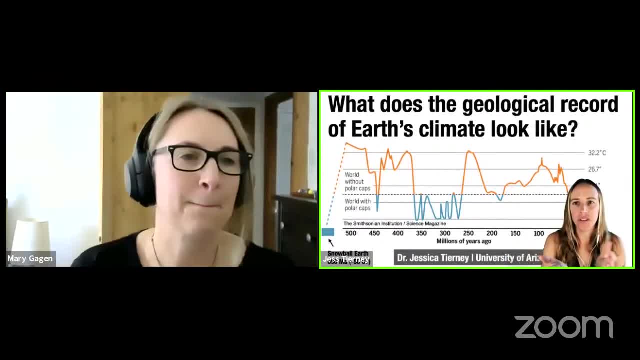 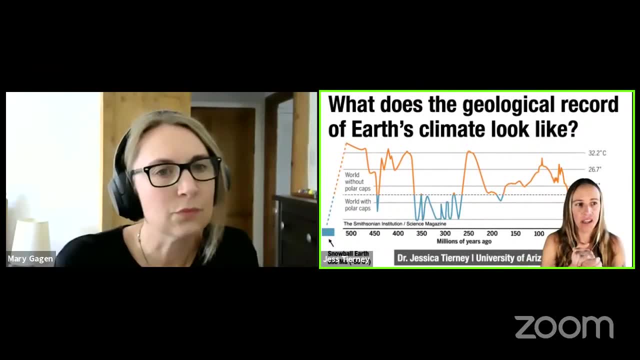 Yeah, sure, So, um, there certainly is age uncertainty in our understanding of this, but it's going to be the x-axis uncertainty on these timescales is going to be smaller than the y-axis uncertainty. And, yeah, so we don't have thermometers right, So we can't just like. 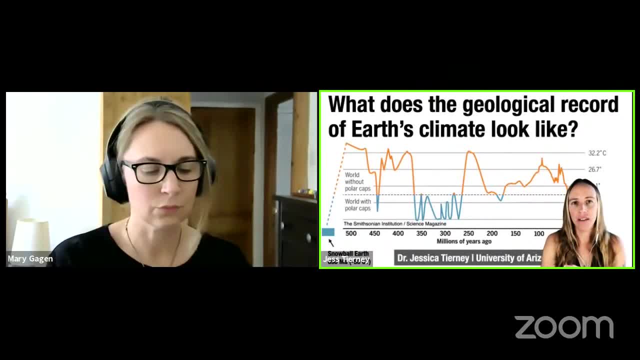 go back and know what the temperature was. We have to rely on our entire arsenal of both uh- geochemical indicators for temperature and also- uh, you know, uh- floral indicators for temperature or crop crocodile indicators for temperature. Um and so, to create a curve like 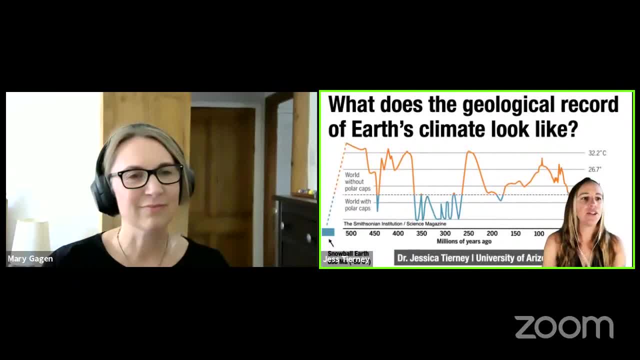 this you know you really need to bring together, like all the information that you possibly can um compile it. And then you know, of course, the, the proxies- we call them proxies because they're standing in for temperature- that they're not necessarily. they're sensing temperature. 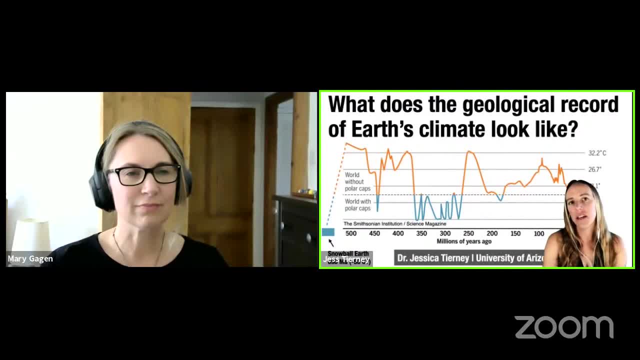 but they're usually recorded in a unit. That's not. that's not temperature, And so you need to translate that into temperature units, which requires some statistical modeling. Um and so it's. it's actually non-trivial right. 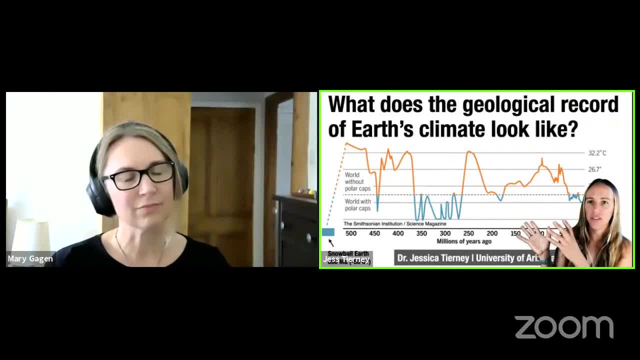 So while I think the general trajectory of this curve is is going to stay the same, because we know some very basic things, like we know that, you know, during the carboniferous there were really large ice sheets, So it's probably cold. Um, the details will evolve as we get more and 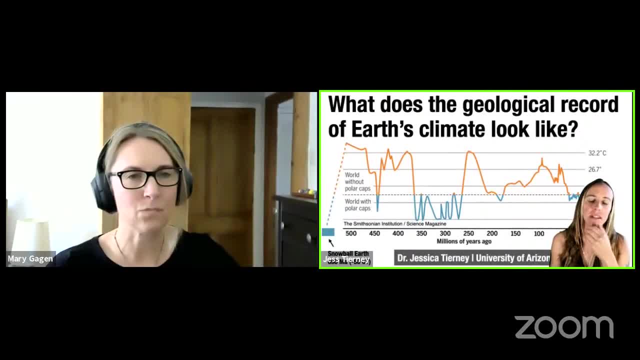 more um, heat, freeze, all kinds of things. Um, but so it's, it's, it's, it's, it's, it's, it's ages that we need to. that's the argument for it. So, um, yeah, definitely it'll be. 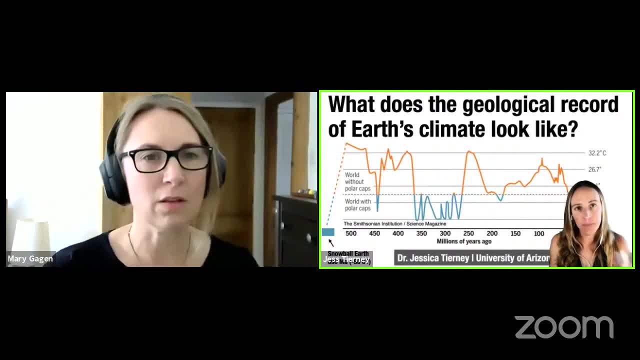 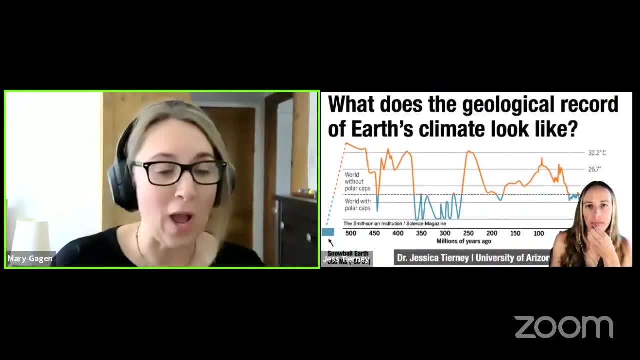 exciting to see how this curve evolves and how it improves in the next few years. Thanks so much. Um question from from Matthew in the in the chat. um, who's asking? uh, in a hopeful way, um, if we're looking at the PTM as an analog for RCP 8.5, if we you? 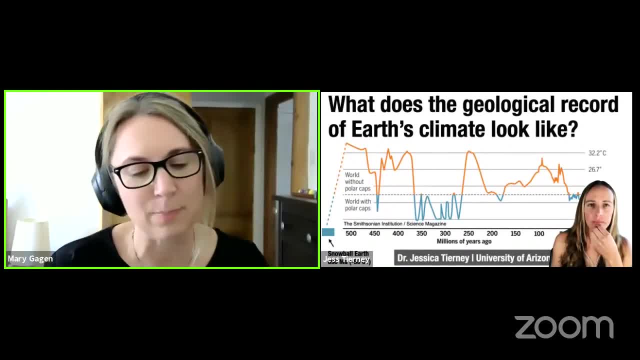 know, with our, with our hopeful view on- uh think about perhaps undercurrent temperature, you know that can change. you know the temperature, the, the temperature, the temperature, the temperature. you know can, can, can, can, can, can change. you know the temperature, the temperature, the temperature. 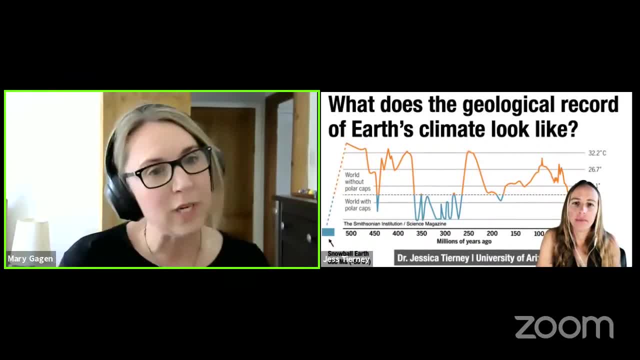 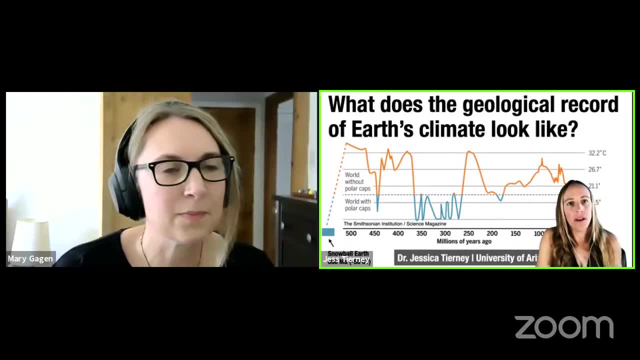 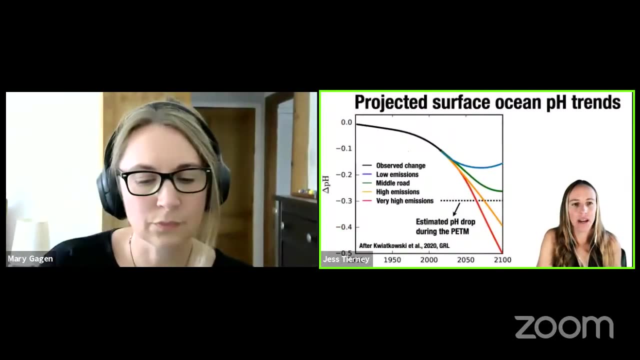 climate pledges. that being a more distant prospect, where would we look for analogs for rcp7 or 6 instead? well, it depends on what your baseline is for analogs, because if we're talking about ph change, i'll just go back to that um so high emissions. here is rc, is a ssp7 um, and so, in fact. 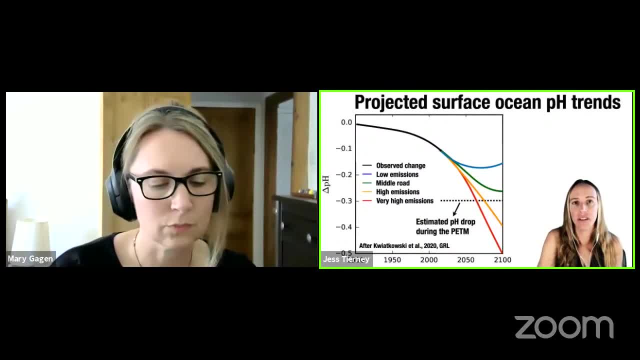 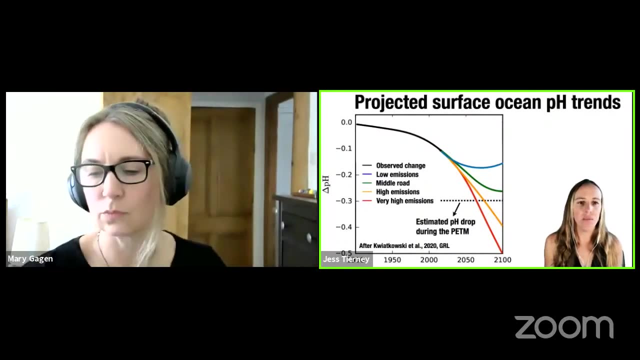 the ptm is still an analog for ssp7 in ph terms. um. so i would say that you know just a, you know basic analog. i mean, as alan discussed, the term analog is sort of loaded and you can sort of take that to be very literal or or or not, um, but i actually think that ptm is pretty relevant for 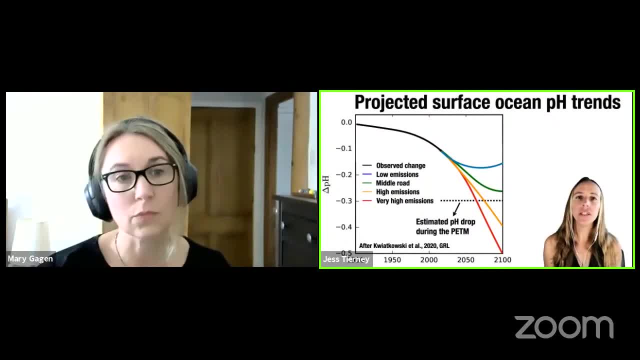 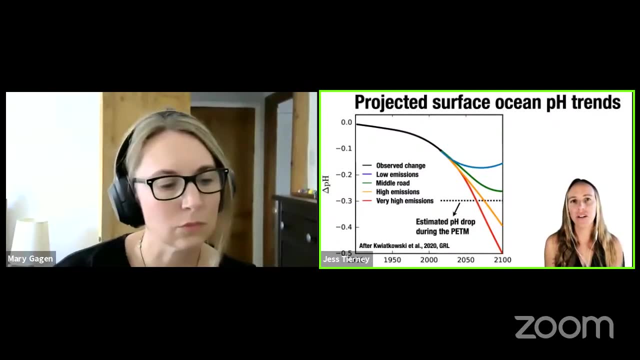 understanding even middle to somewhat high trajectories, uh, because we are getting very close to the level of acidification that we've seen on this level, um. so so yeah, still still an analog, i would say, for those middle emissions. now the lower emission scenarios, middle road, you know, as alan discussed maybe the climates that are not so extreme, like 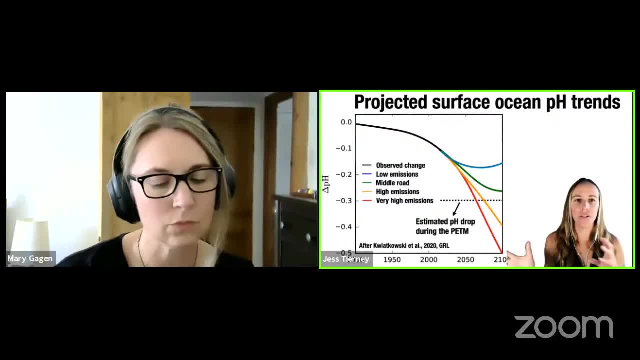 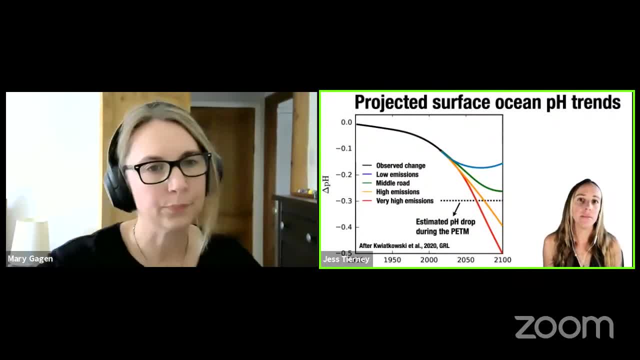 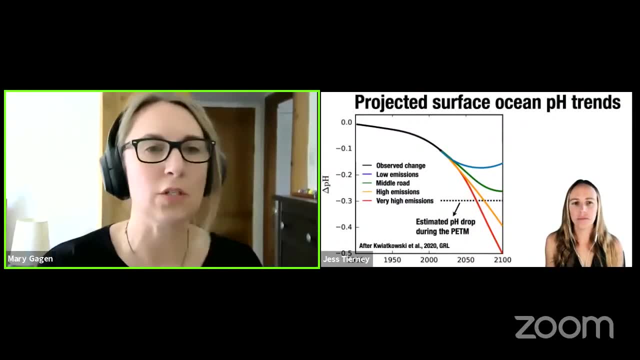 which is actually what we need to understand, right, because we're not going to see equilibrium right in human time scales, right? thanks? thanks for that, jess. um, i'm going to try and summarize a few. there's lots of questions in the chat around what, what else you know, orbital forcing and these. 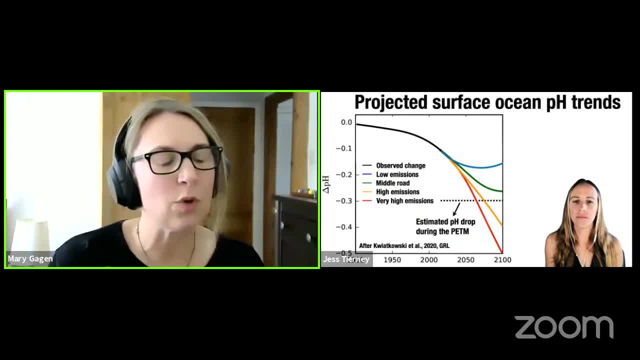 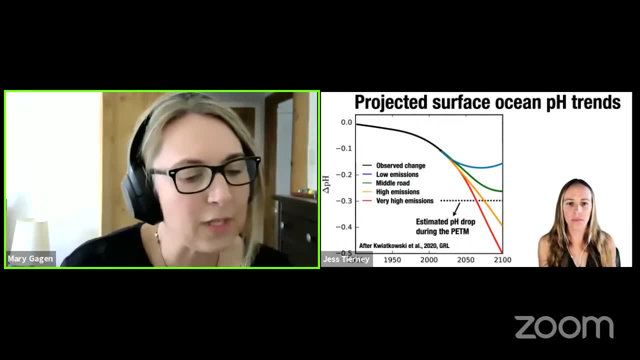 sorts of things and um and questions around. you know, you know, clearly there isn't a perfect, simple relationship between co2 and temperature. obviously, because it's the planet. and why would there be? um, so the plot that you showed during the oligocene, um, and i guess i, i 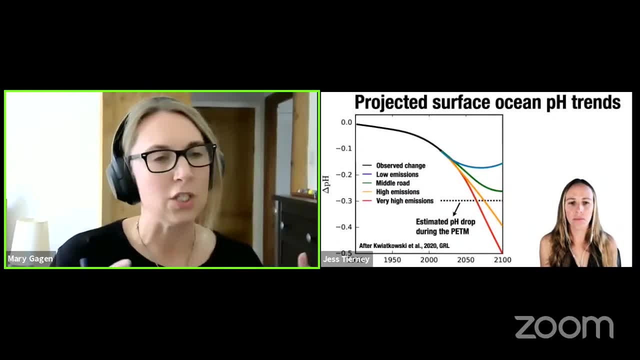 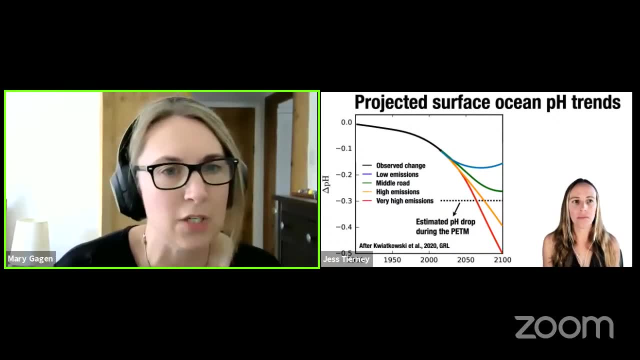 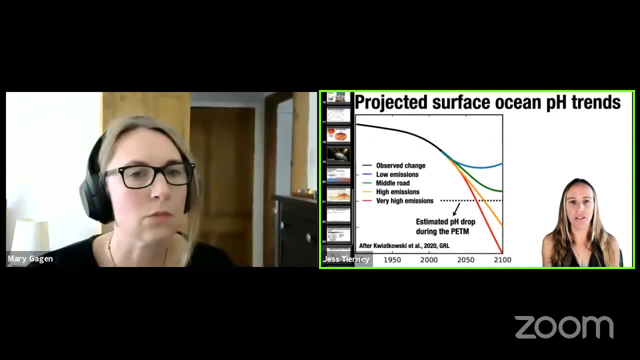 guess i would say: could you talk a little bit about whether that's around uncertainties in the records or or an actual decoupling at time periods of the co2 temperature relationship? yeah, absolutely, um it. i really think that those times, when you know, i'll go back to the plot. you 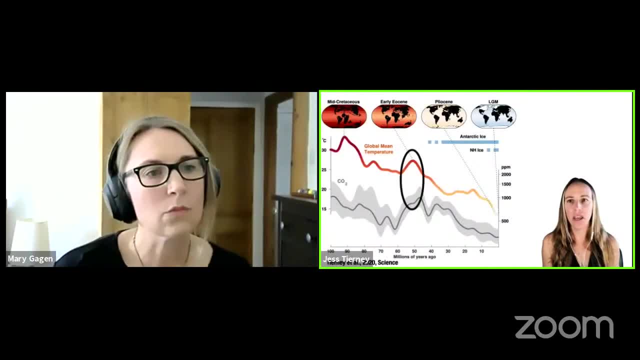 know that co2 and temperature don't follow one for one. i, i'm, absolutely, i would, i would, i would bet money that it's, that it's going to, that they're going to match that. they're going to match that. mostly, this reflects uncertainties in our ability to estimate co2, so i'll give you some. 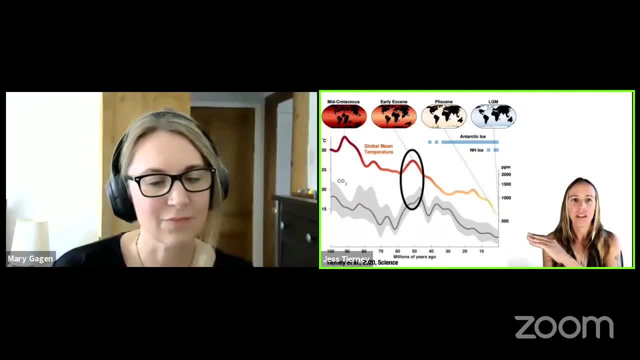 examples. so for one thing, you can see that that timing of that eocene oligocene transition is a little bit off and- and that is actually coming from a couple proxies that seem to be sort of shifted in time in the co2 compilation. but if you actually look, for example, at specifically the boron, 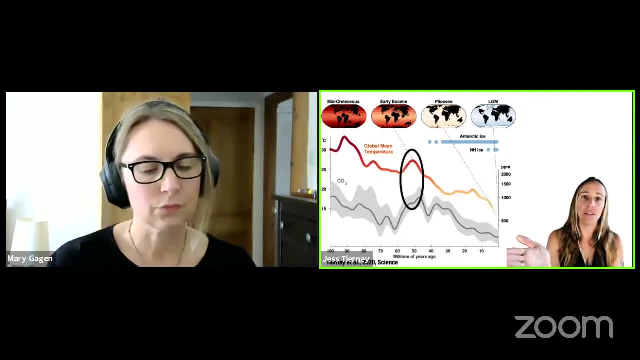 data. they actually, you know, match the, the mean temperature record, pretty much precisely. so i think as we get more data over that time period, we're going to be able to see that there's a lot of that transition. they're going to start to come in alignment. another example is between 60 and 70. 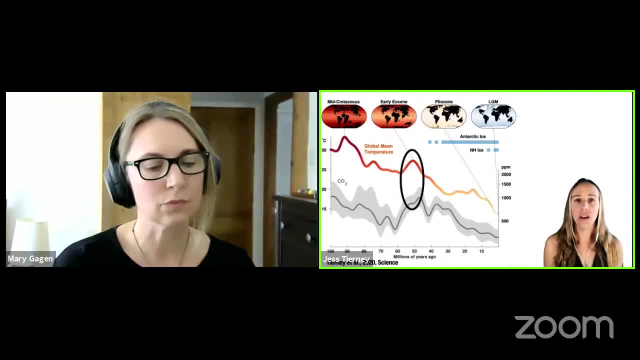 million years ago. the co2 estimates seem a little bit low, um, and the problem is we have a real drop off of data in um, in the late cretaceous, in the paleocene, um, and so, like you know, there's a lot of data in the eocene and then the paleocene is, like you know, a little more boring, so maybe we 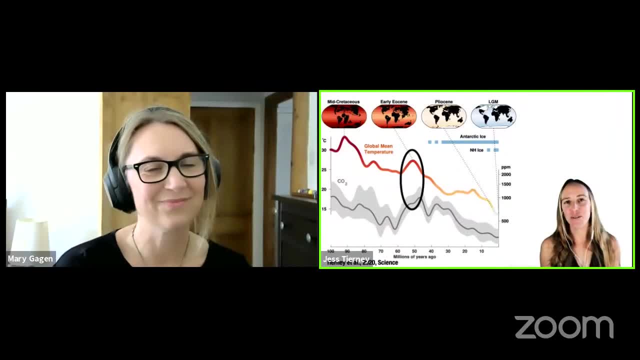 you know we don't measure it as much, but i am absolutely confident that once we, that we extend the data into the, this curve is going to be a little bit more boring, and then we're going to reshape um, because you know, ultimately on these time scales it co2 is in the driver's sheet. so 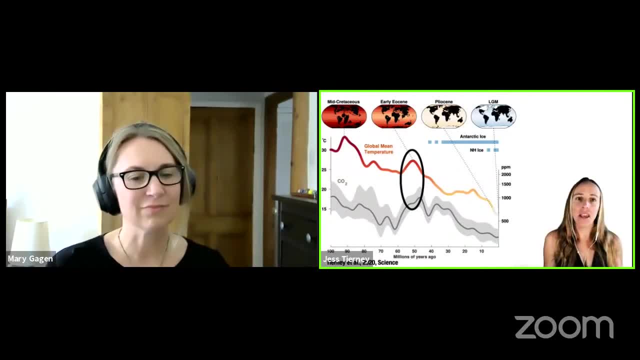 orbital stuff. that's important on smaller time scales and it changes, as we heard, uh, the other day, the seasonal balance of energy, right, and so it's really important for things like regional climates, for monsoon systems, but on these long geological time scales, um, you know, it's, it's. 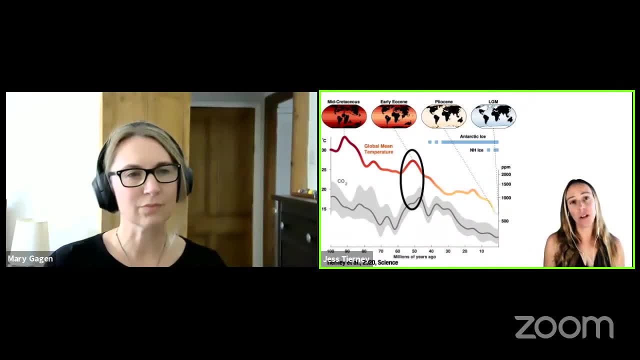 basically, uh, what's controlling the climate? solar luminosity. so it's really important for things like the um and the uh, the solar systems, and this is the thing that's so important in the global climate and that's what paul valdez said, right, the sun is. 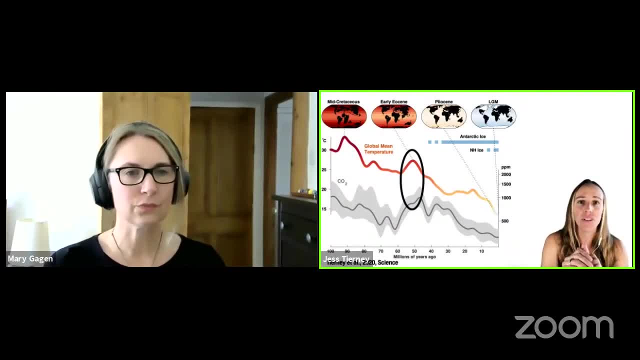 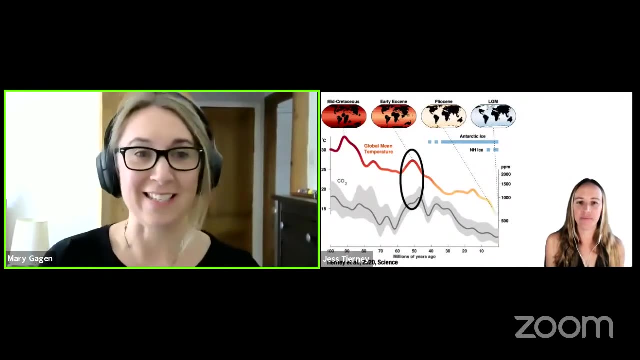 changing its output very, very slowly. um, and then paleogeography- less important, right. and then it's co2. it's greenhouse gas, it's co2, right. so that's it. um. so i'm pretty sure that this mostly reflects uncertainties in the in our ability reconstruct co2. it's not easy, as many people in the audience. 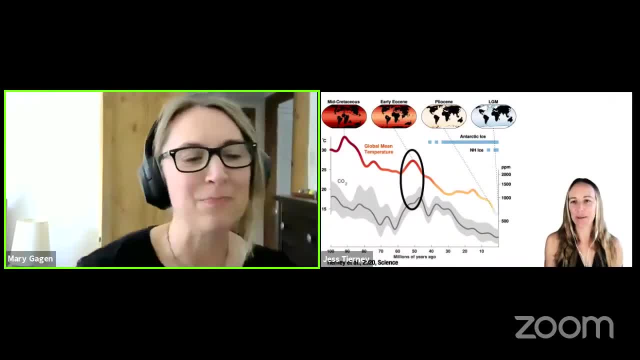 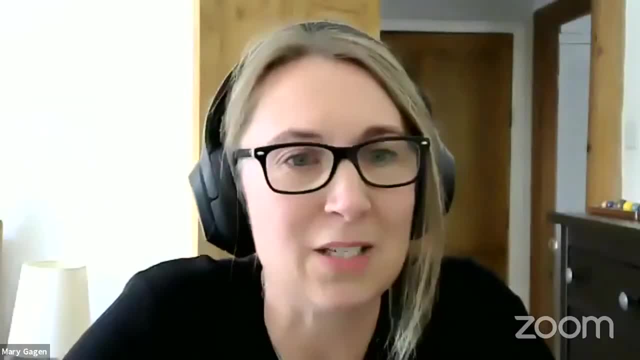 really appreciate. thank you so much, jess. um, i'm gonna say a huge thank you from from me, um, to everybody who's who's been speaking today, to all of our speakers and to everybody who's participated in the q a as well. thank you so much. a reminder again to our speakers that there there probably are a few. 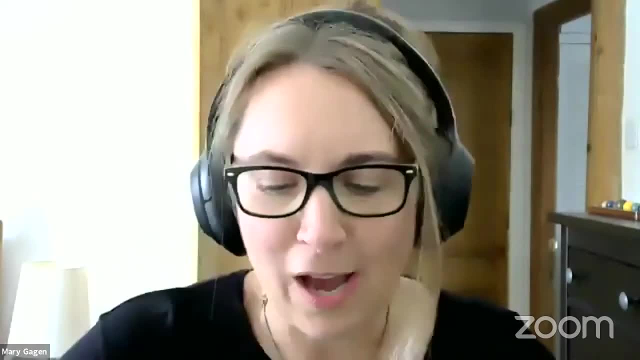 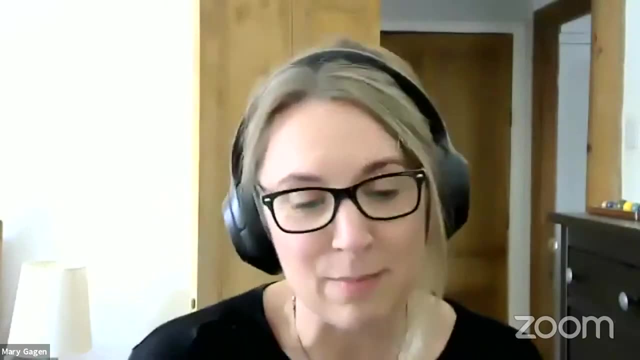 questions. uh, left in there and do feel free to engage with those um. i'm sure everybody's desperate to grab a cup of tea, run up and down the stairs a couple of times, so we are taking what is now, sorry to say, a 15 minute break. we're back here at 4: 45 um for invited talks from rachel and cow. 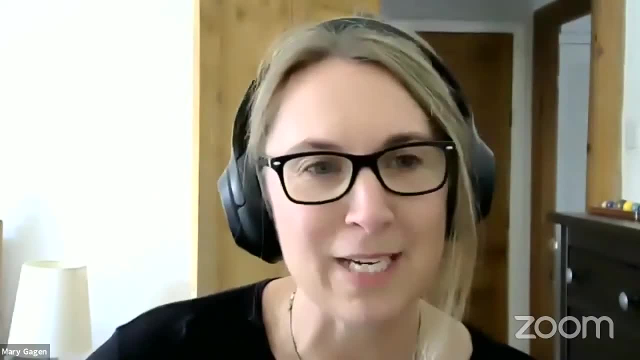 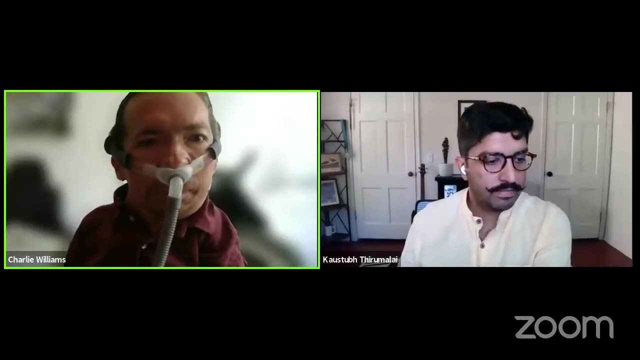 and then they'll post a session. so so huge thanks for me and we will. we will see you all soon, okay, everybody? uh, let's get started for the last session. so my name is charlie williams. i'm a research fellow in climate science at the university of 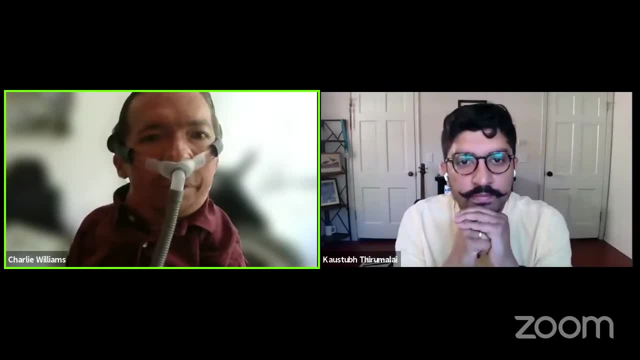 bristol, and i'm delighted to be your chair for the last session. so we have two final speakers, cow and rachel, and in between these we're going to have the flash talks, where, for those of you who submitted a poster, you had the opportunity to pre-record a one-minute presentation on your work. 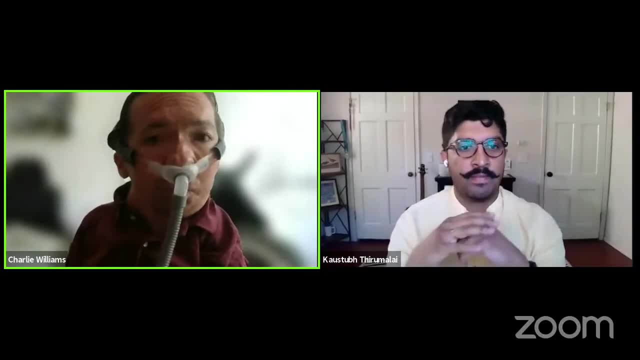 um. after that, at the end of the session, we're going to go into breakout rooms where those of you with posters will have the opportunity to um present your poster and people can ask questions. so before that, i'd like to introduce our first invited speaker, carl serum and i. how is a assistant professor at the university of arizona? 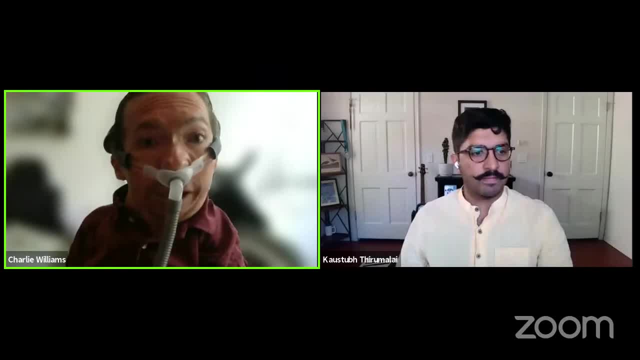 in the us. his interests are wide. they include climate variability, paleo, oceanography, as well as extreme events and how the geological record can inform us about future projections. today he'll be talking about question four of the statements. what does the record indicate about global versus regional change? 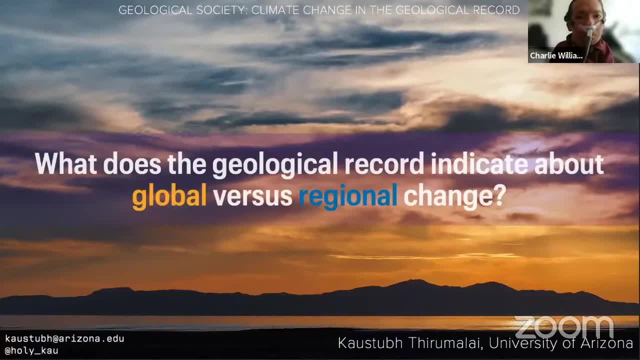 so, as you now, i will turn my camera back on at your two minute, uh, two minute warning over to you, carl. i will turn my camera back on at your two minute, uh, two minute warning decided, Okay. thank you very much, Charlie, And thanks to all the organizers for giving me an opportunity to. 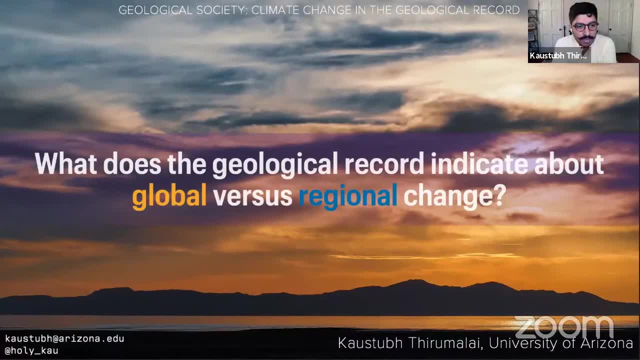 share some of my research here And the topic that was assigned to me. the question is: what does the geological record indicate about global versus regional change? And naturally, as others have talked about you know, it's tough to cover all the different topics of. 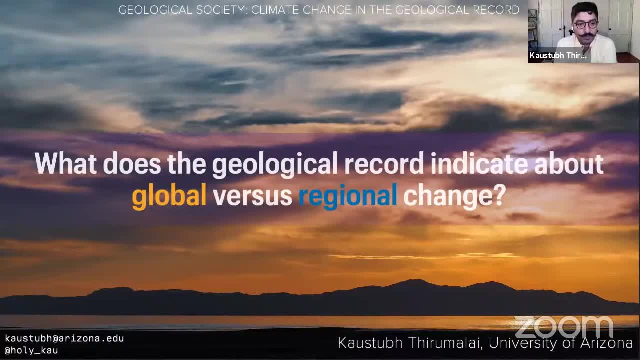 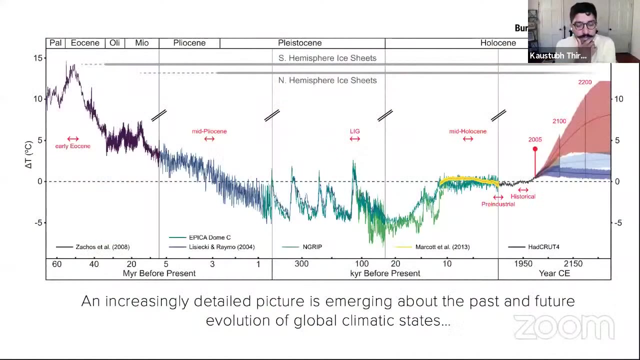 regional change throughout the entire history of the Earth's geological record. So I'm going to apologize straight up and basically focus on a couple of aspects that I'm working on, And so let me start off by showing you a graph that many of you have already seen and many speakers have. 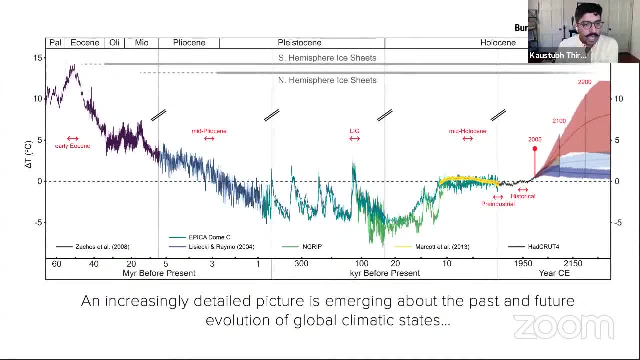 already talked about in this workshop And in particular. so this is a graph that's spliced together by Burke and others in PNAS And you can kind of see this is sort of the evolution of global climate temperature Over time, over geological time, from 60 million years ago all the way into the future, with future. 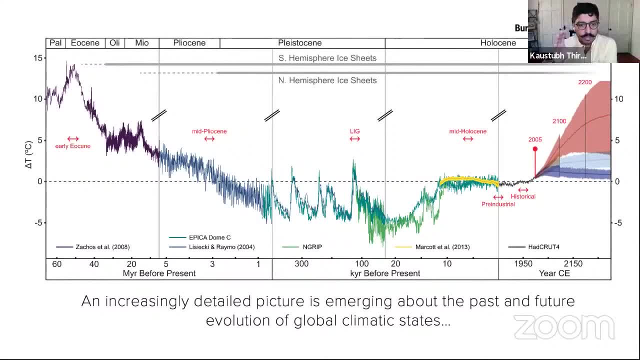 projections as well, And what I wanted to kind of sort of indicate here is that we're really getting an increasingly detailed picture about past and future evolution of global climatic states, And it was fortunate that I'm following Jess Tierney, because Jess really nicely gave an overview about 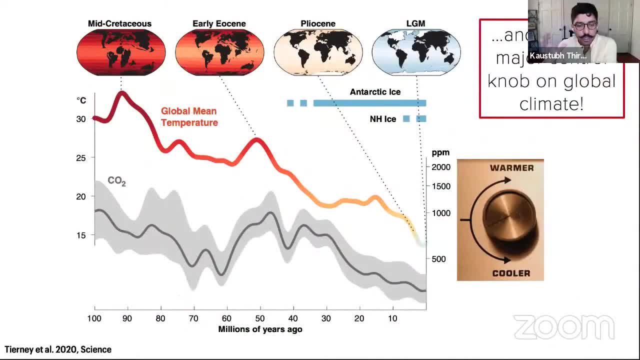 how, particularly in the Cenozoic, the major control knob on global climate- on global climate as well as global climate, global temperature evolution- is really carbon dioxide. So CO2 is a major control knob on global climate, including moving from a greenhouse world into an ice house world, And we have to be really cognizant. 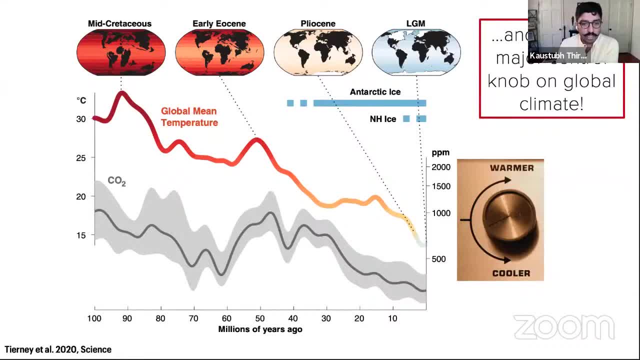 about which world we want to move into in the future. Undoubtedly it's getting warmer, But, depending on the different trajectories of CO2 emissions, we're going to see a lot of change And we're going to end up in different worlds, And so the trajectories that really we have in line for 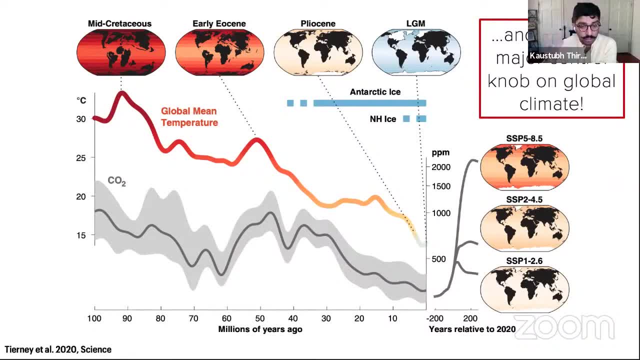 the future they're going to hold really strong implications for global climatic evolution, but also, in particular, future regional climate variability and extremes. So when we take a look at these sort of disparate states that the future might hold for us, the way that these states 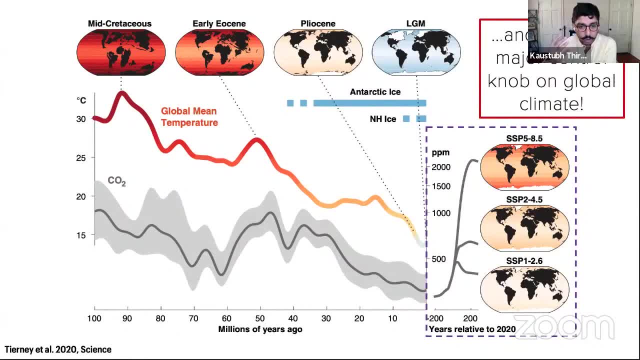 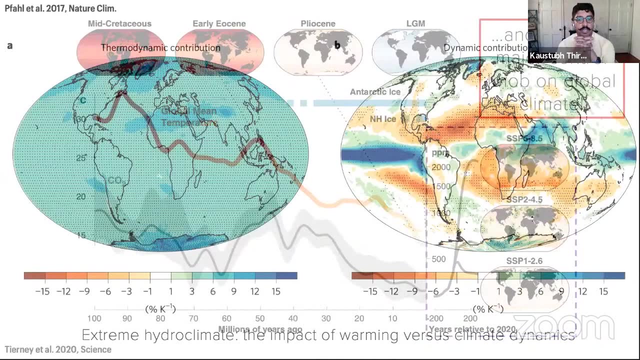 trickle down into sort of regional hydroclimate evolution and regional extremes is still uncertain. Now we know for a fact that CO2 is increasing and that's going to induce warming across the planet, And so some researchers- there's been a lot of work on trying 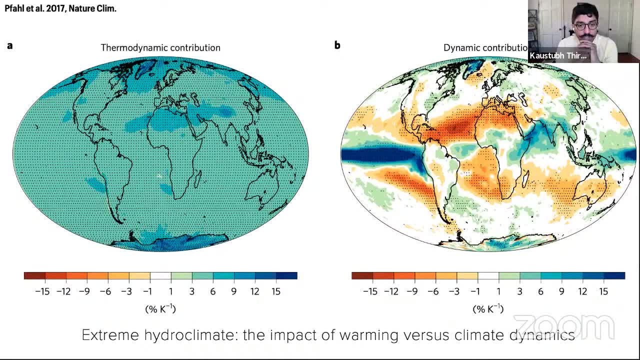 to figure out how warming is actually going to impose changes in extreme hydroclimates, so extreme precipitation. So here's a figure from Fall and others in nature climate change from a couple of years ago where they sort of disentangled the impact of the 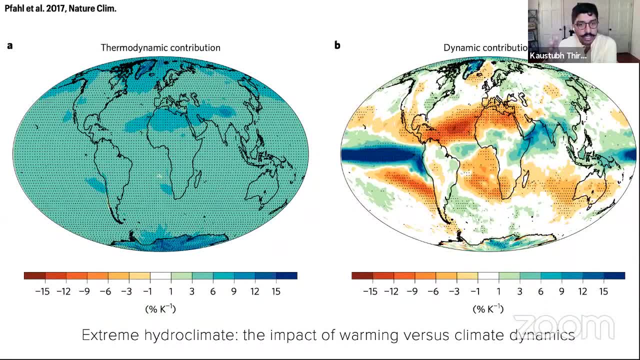 thermodynamic contribution and the dynamic contribution of changes in future extreme precipitation. So on the left hand side, what you can see here is basically an entire globe. that's kind of about three to 9%, maybe a little bit more in certain areas, And what this is talking about. 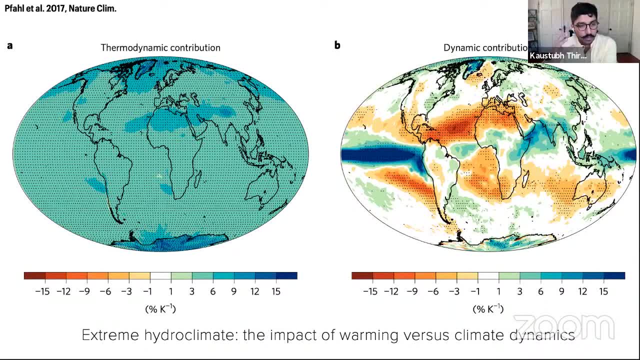 is the fact that the thermodynamic contribution, the fact that we're going to increase CO2 in the atmosphere, is going to essentially supercharge the hydrological cycle and allows the atmosphere to hold more water vapor. And the graph, the sort of the scale right here, is the percentage change. 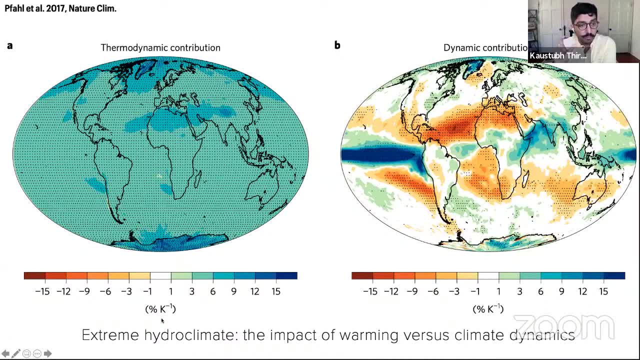 in the hydroclimate extremes per degree of warming. So when you disentangle the thermodynamic contribution, we know that the increased warming is certainly going to impose a larger change in the hydrological cycle that leads to larger extremes. Now I also would like to point out: 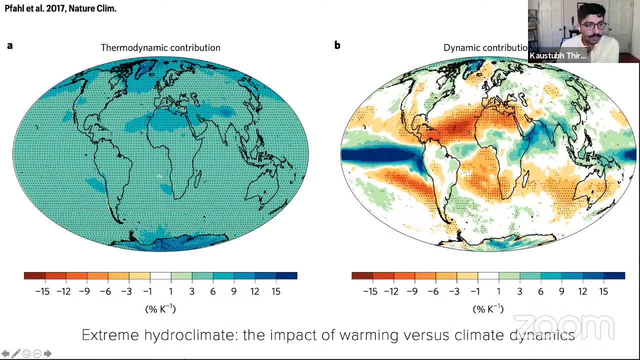 that this is a multi-model ensemble composed of over 20 models, And these dots that you see here indicate that over 80% of the models agree on the sign of change. So all of the models across the globe are in agreement that the 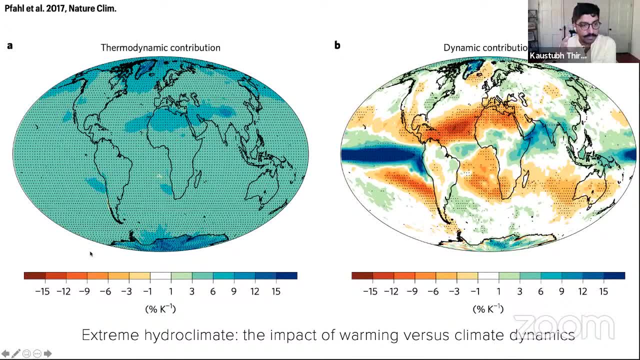 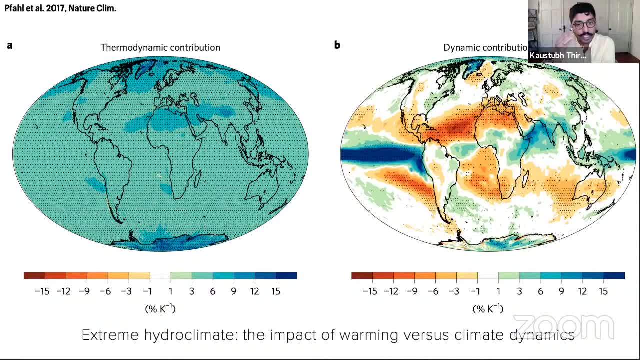 here is a plot that shows the dynamic contribution to these changes in hydroclimate And, as you can see, there's a lot more nuance here and large changes that go from more negative changes to positive changes as well, And really, critically, many of the models are not in agreement, even on 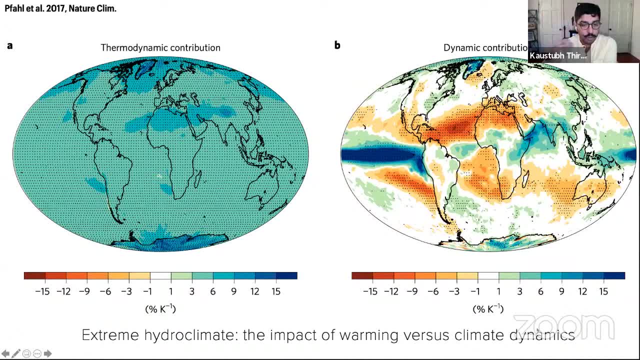 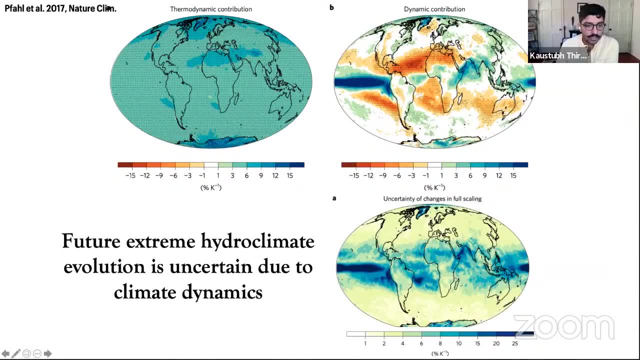 the sign of change in the in the in future extremes, And so, in particular, these authors actually also looked at the uncertainty of changes in the full scaling model and they looked at the uncertainty of changes in the full scaling model and they looked at the uncertainty of changes in the. 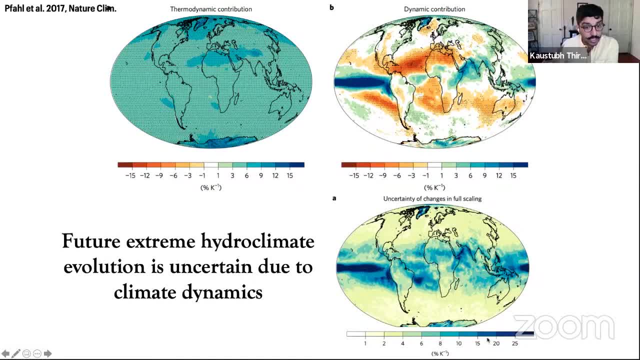 full scaling model and they looked at the uncertainty of changes in the full scaling model. So this plot right. so this plot right here at the bottom, shows you the uncertainty that is the sort of the spread between the models that that contribute to this dynamic contribution, And you can see here that. 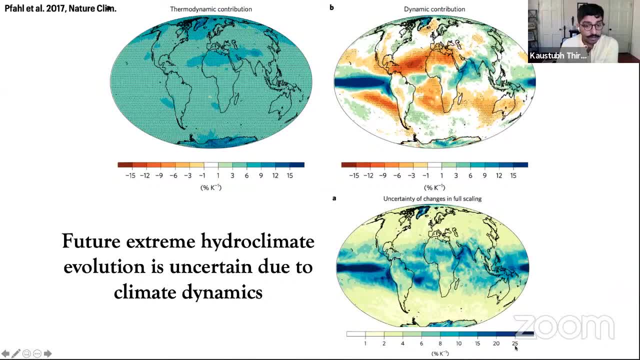 these changes are large, these uncertainty is large on the order of 25% per Kelvin, where the signal in itself is on the order of 30% per Kelvin, And so the bottom line is that the future of hydroclimate extreme evolution is really uncertain, largely owing to how climate 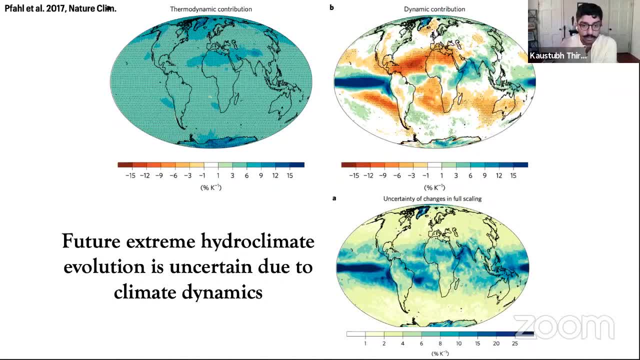 dynamics are going to change as we move into a warmer world, regardless of how warmer that world might be. you're basically going to have extremely substantial implications for regional climate evolution, And one thing that I'd like to point your eyes towards is looking at 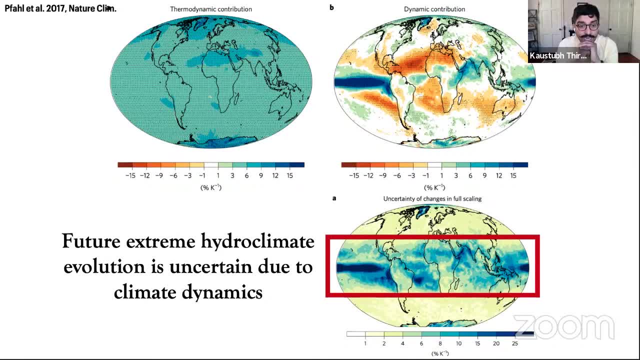 where we have the largest uncertainty, and that uncertainty arises in the tropics. So you can see the tropical uncertainty in hydroclimate extremes that we're looking at And the tropical uncertainty in the tropical climatic impacts is exceptionally large. And this is kind of one of the major motivations for my own research is that the tropics are where 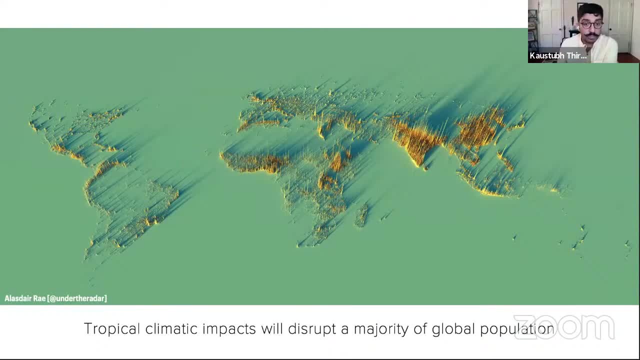 we have the largest number of people, So tropical climatic impacts are going to disrupt a majority of global population. In particular, this is a kind of a- some of you may have seen this before, but it's kind of a staggering statistic is that more people live inside that circle than outside of it. 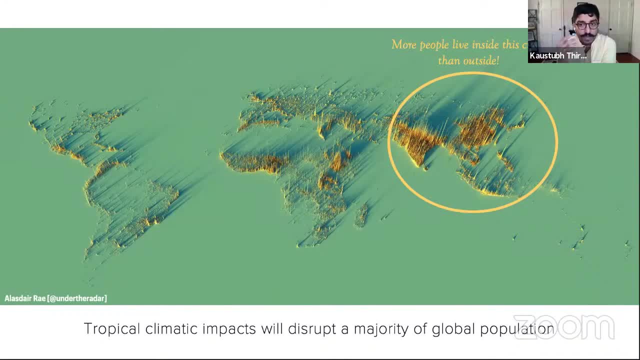 And, moreover, we know that the amount of people that live in tropical climates, including things like drought, wildfires and extreme flooding events, are increasing in these countries that are particularly vulnerable and hold a majority of the Earth's population, And so here are just some. 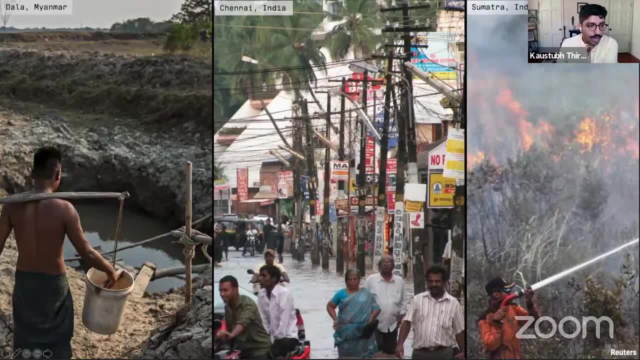 examples of pictures showing you some of the extremes that are happening. So here's a picture of drought in Myanmar in 2016.. This is extreme winter monsoon flooding in Chennai in 2017.. And then there were wild wildfires across Sumatra and Java in Indonesia in 2017 as well. 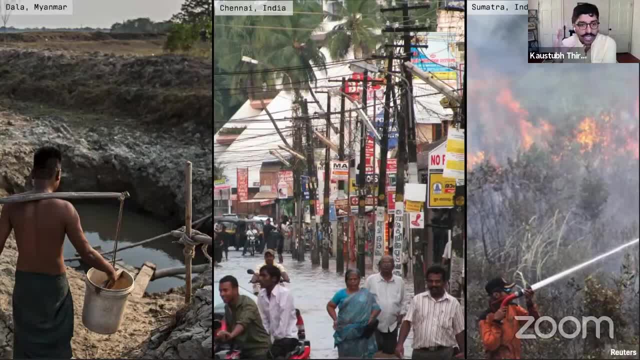 And so, in particular, the sort of the socioeconomic currency of regional climate change is hydroclimate extremes. So we want to really be able to anticipate the different types of extremes that are important for different regions and how that's going to evolve as we move into the future, And the bottom line is that the sort of the transfer of global change into 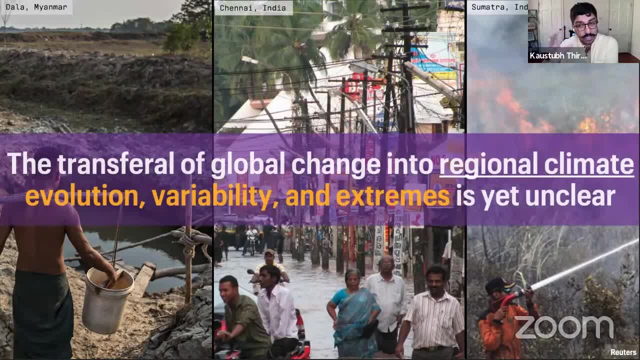 climate evolution, variability and extremes is still unclear. So what does this look like? What does future climate variability in the tropical oceans look like? And, largely, mind you, many of these events have been attributed to changes in the sea surface temperature domain in the 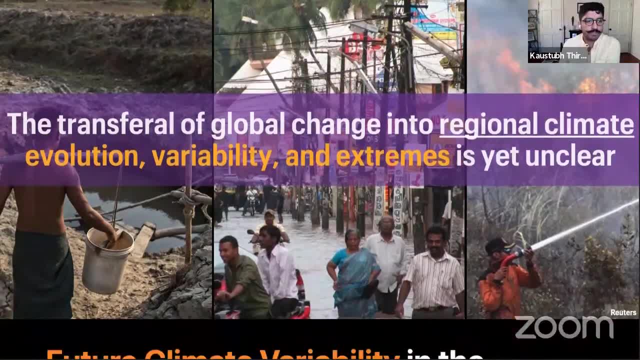 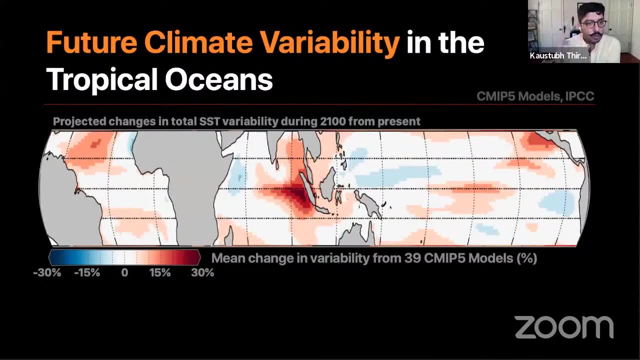 tropical oceans. So what does that look like when we look into the future? Well, so here is a plot of the multi-model ensemble mean of future changes, of projected changes in sea surface temperature variability during 2100, subtracted from the present day simulations. And so this is the mean change in 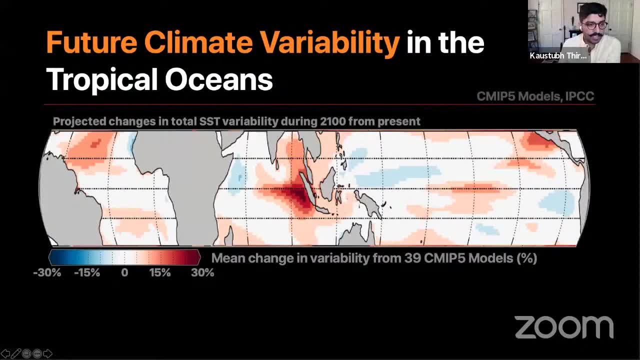 variability across 39 different models and going from a scale of minus 30% to plus 30% relative to today's variability, And the bottom line here is that a large part of this graph is white, at 0%. Now does that mean that models suggest that there's going to be no change in variability? 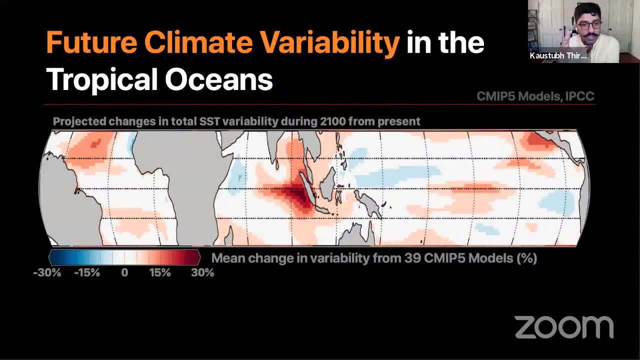 That's not true. What this actually says is that there's a lot of models, some suggesting increases, some suggesting decreases, such that the average ends up being zero, close to zero. So they disagree on what's going to happen to the future of climate. 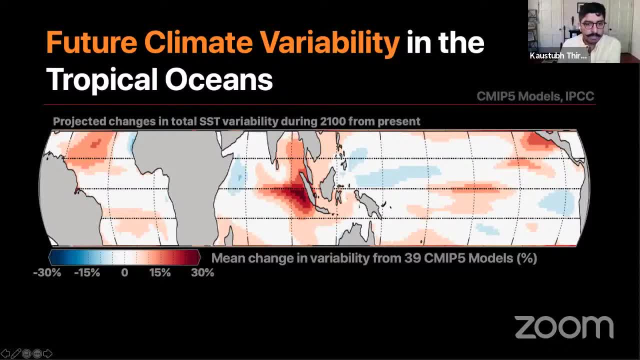 variability in the tropics And largely this arises from uncertainty in the evolution of the El Niño-Southern Oscillation. But another thing that emerges out of this picture is that models seem to converge- at least some of them do, in order to sort of overcome the noise amongst them that there is a stark 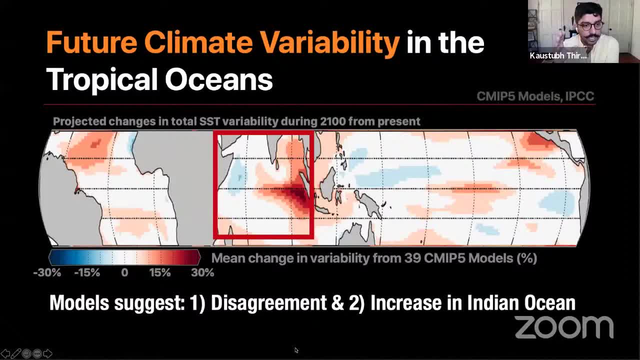 increase projected in Indian Ocean SST variability And, as I showed you before, the Indian Ocean and the Indian Ocean Rim harbors countries that are really critically dependent on a sort of steady rainfall as a direct impact on their socioeconomic stability, And so we really want to try and 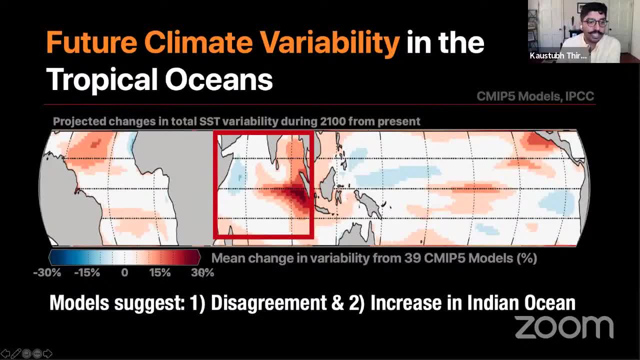 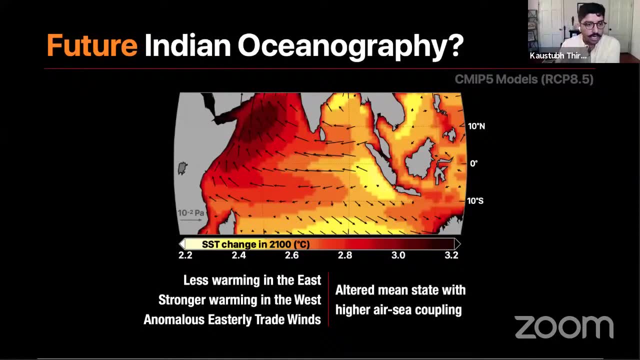 understand what's going on in the Indian Ocean and whether such incredibly large changes of 30% in sea surface temperature variability are even plausible or not. So, zooming into the Indian Ocean realm, here is the sort of the projected future Indian Oceanography. So what I'm showing you here are the 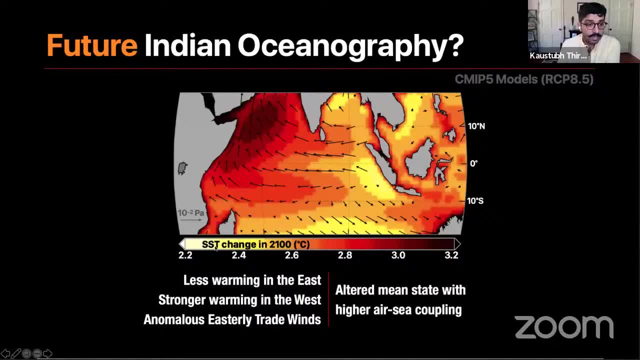 projected changes at 2100 relative to today in anomaly space. So all models agree that the Indian Ocean is going to warm. There's no question about that. But very interestingly, the models are suggesting that the Eastern Indian Ocean is actually going to warm a little bit less than the. 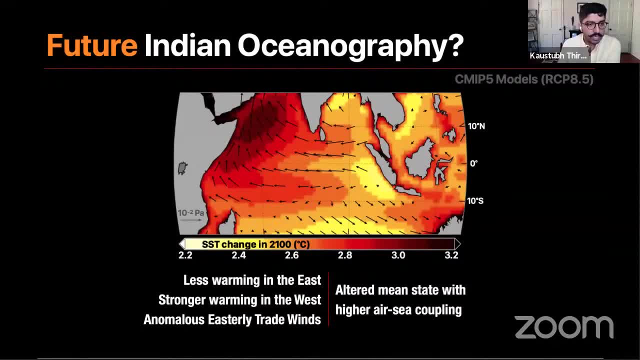 Western Indian Ocean And, in particular you can see that, the Arabian Sea. here it warms a lot. That's already happening. Many people have focused their research on this aspect, But again, this is the future projection: that there's less warming in the East, stronger warming in the West And this asymmetry in the 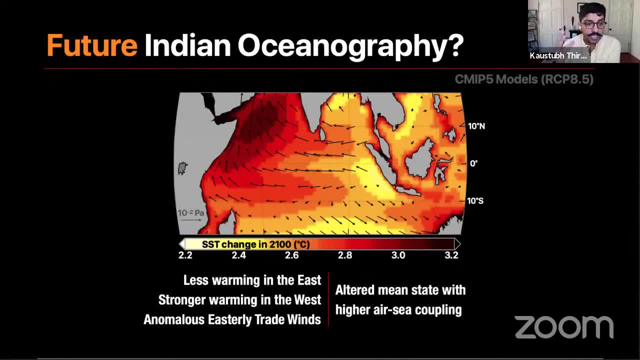 zonal gradient basically triggers anomalous easterly trade winds that do not exist today in the permanent mean state of the Indian Ocean, And so if I could direct your sort of focus on the equatorial Indian Ocean, you can see here that there is this stark contrast in the zonal SST gradient. 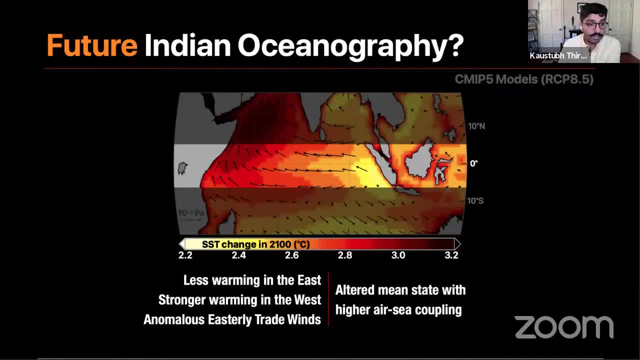 where the west warms more than the east And basically you have the onset of these anomalous easterlies And essentially the models are suggesting that this altered mean state is going to elicit higher air-sea coupling or stronger ocean atmosphere interactions that are going to give rise to 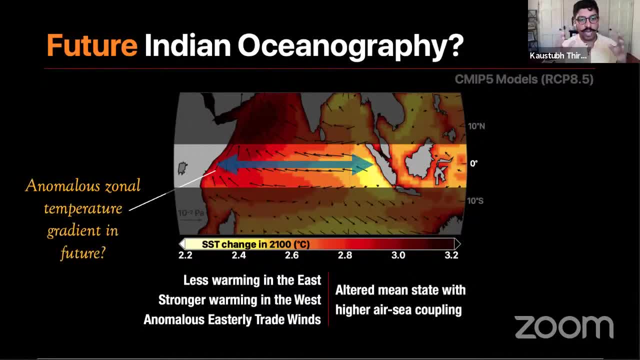 larger climate variability. So the anomalous zonal temperature gradient in the future is a tenet that models are suggesting And we want to try and understand what that can actually mean For climate variability and regional climate change across this densely populated region. So the sort of the thrust of my talk today is basically trying to establish that the 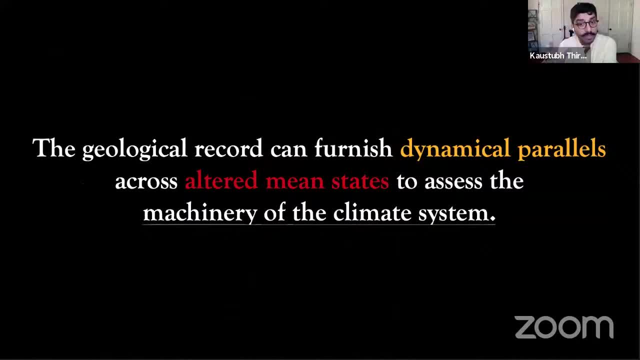 geological record can absolutely furnish dynamical parallels across altered mean states to really really try and assess the machinery of the climate system. So, in other words, the question is: you know, can we go back in time to try and look at whether the Indian Ocean ever had? 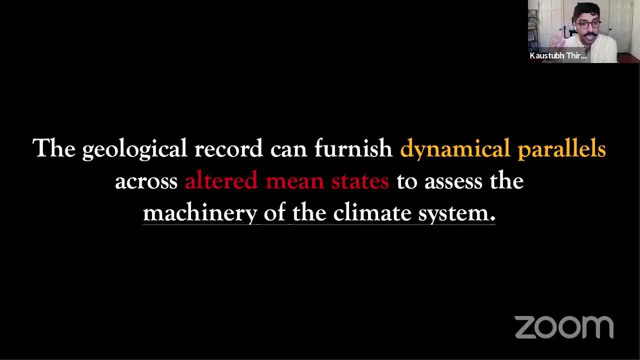 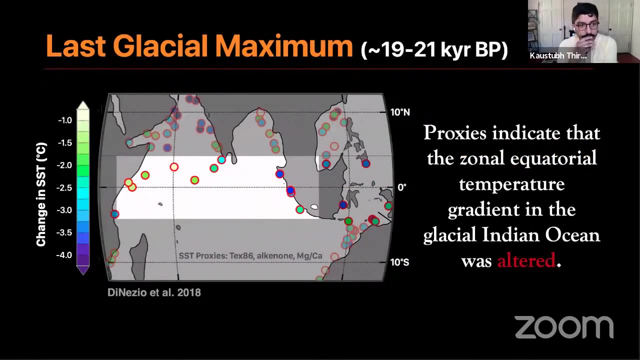 such a scenario that existed, where the zonal SST gradient was much, much different and altered completely relative to today, And I'm not going to go into too much details into the background climate state but, as several of you have already witnessed with some of the speakers, 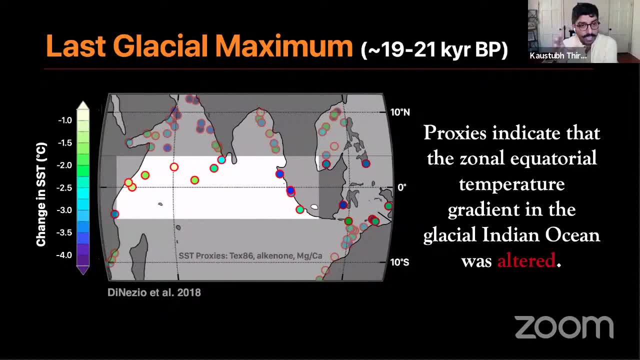 in the workshop before. I'm going to be focusing on the last glacial maximum. that happened about 19 to 21,000 years ago And we've identified the state as a potential dynamical parallel to the global warming scenario And I'm going to explain how. But this plot right here is taken. 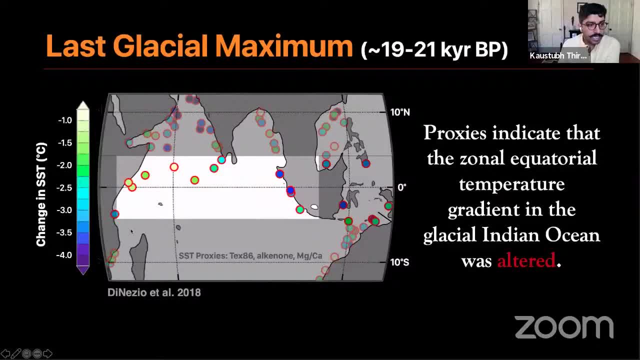 from my collaborators paper in 2018.. Each one of these circles right here basically represents a sea surface temperature proxy reconstruction, And the color inside it tells you the degree of cooling during the last glacial maximum, And so essentially what I'd like to point out right here. 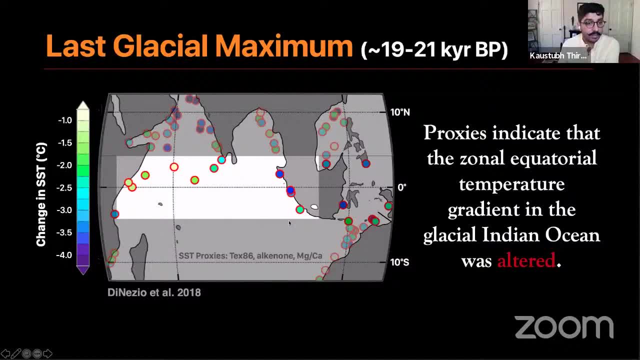 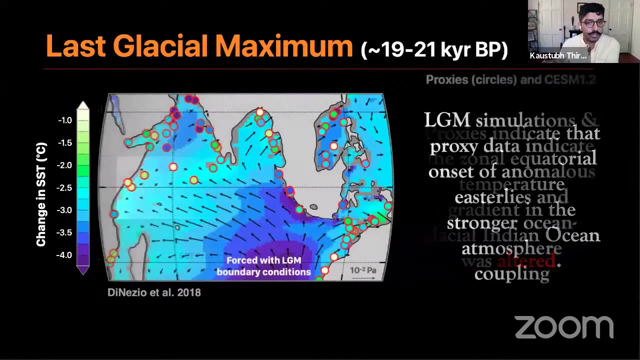 in the equatorial Indian Ocean is that the proxies are indicating that the zonal equatorial temperature gradient is much, much lower, And so what we're going to do is we're going to look at the the climate models. I'm going to show you a figure with a simulation from CESM 1.2.. 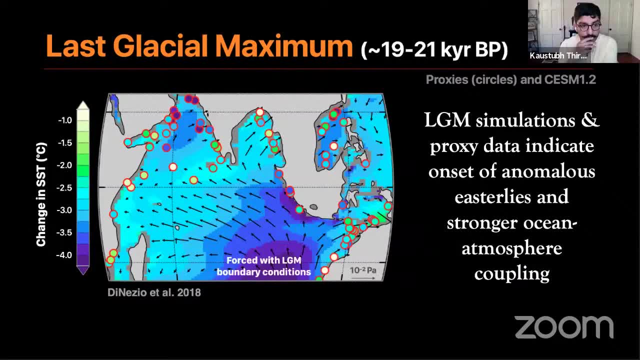 look at what the climate model has to say about the changes in the wind stress regime as well. so the lgm simulations and the proxy data: they both indicate that you know, the eastern indian ocean was a lot cooler than the western indian ocean, and this and the simulations tell us that. 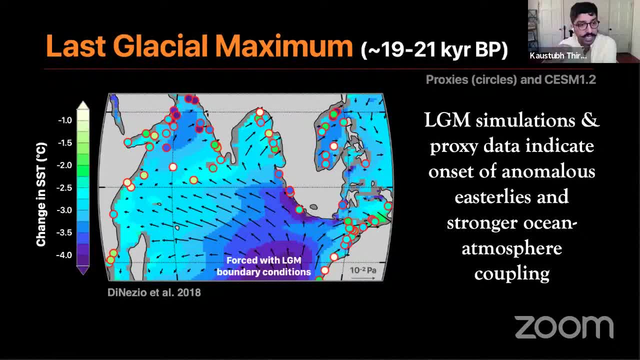 there was this onset of these anomalous easterlies in the equatorial indian ocean 20 000 years ago. okay, very intriguing. when you force a model with these lgm boundary conditions, they agree with these proxies and they also suggest this onset of these anomalous easterlies. 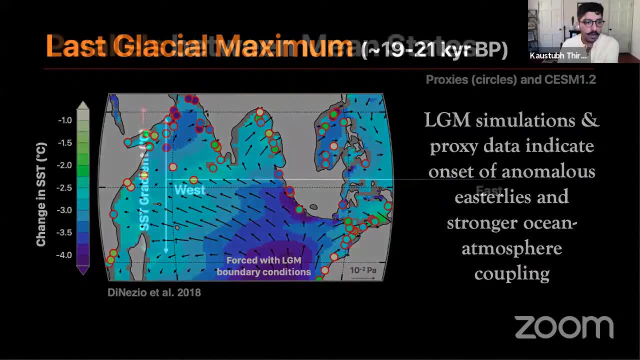 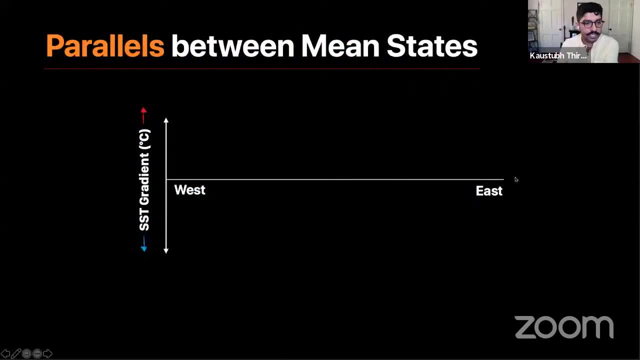 that we're looking at in the future, that we want to try and assess now. um, to kind of simplify this and and to uh really draw out this dynamical parallel, let's assume that this is the modern uh gradient in the indian ocean. so this is the western, it's the eastern. the lgm case is basically: 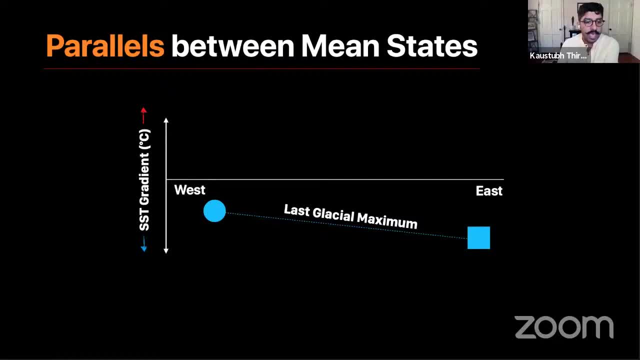 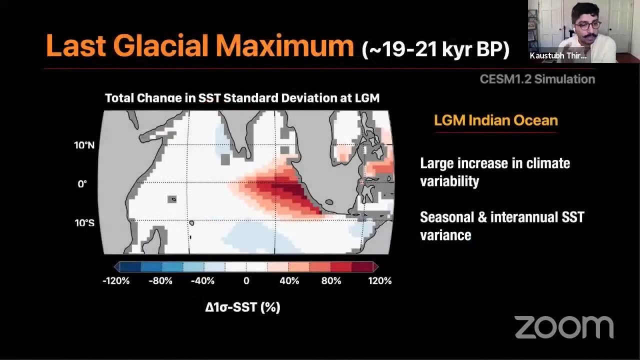 telling us that the east cooled a lot more than the west and the global warming paradigm is such that the west is going to warm up more than the east, but the zonal contrast is similar. so the question really is: how do we take advantage of the zonal contrast? okay, so, uh, and here is what the model actually simulates for. 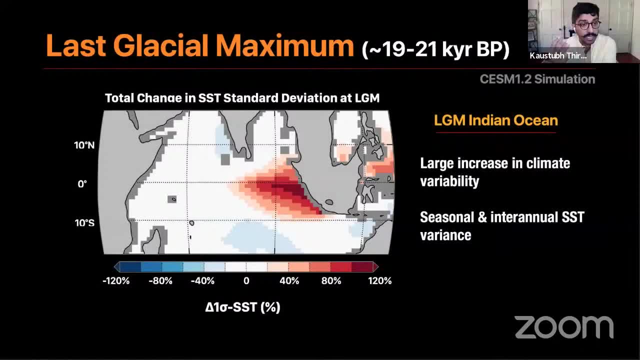 the change in the sst standard deviation. so the variability of sea surface temperatures in the lgm according to the simulation and the model suggests that there's a really really large increase in the sst variability, uh, during this time period. so really, again we want to take a. 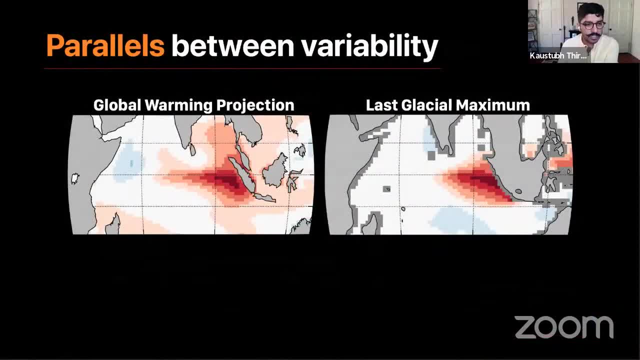 look at how can we take advantage of this scenario. so here's just a schematic showing you the sort of the parallels in the global warming scenario and the last spatial maximum scenario, and i i want to really be key here. i want to point out that we are not headed into a colder state in the future. 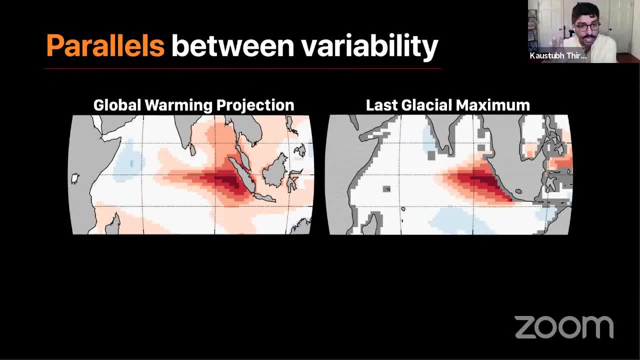 there are different dynamical drivers for why these patterns arise, but the fact is, the similarity in these dynamics should be able to tell us something, and we ought to be able to learn whether such dynamics can actually operate in the indian ocean or not, in spite of the fact that we're in the northern states. okay, so again, we're not going into a last glacial maximum. 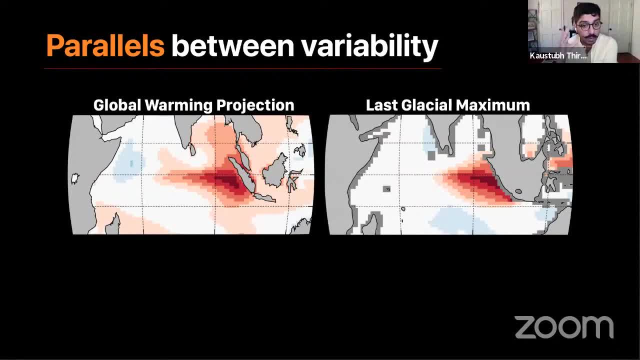 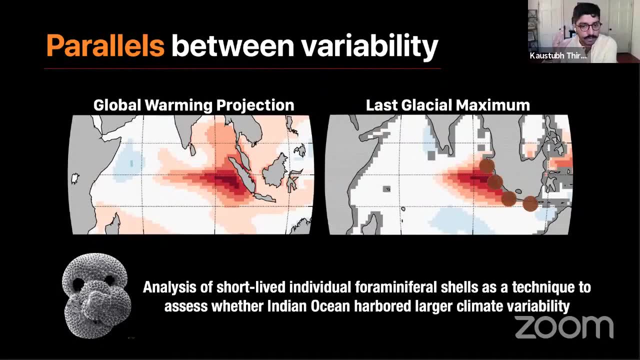 that's totally out of the question. there are different drivers for these patterns, uh. but we want to learn from these dynamical parallels, and so the question really became: you know, how can we reconstruct sst variability during the last glacial maximum? and i'm going to skip on a lot. 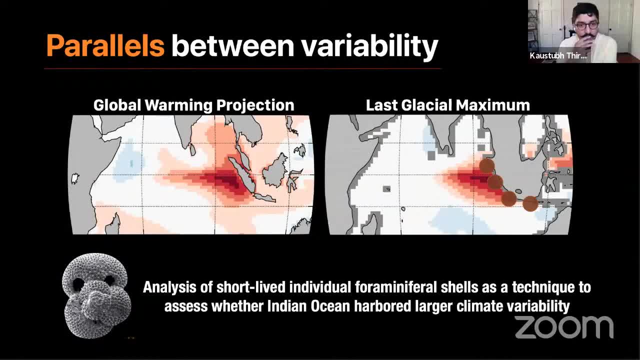 of the nuances and the details. i'm happy to answer them in the chat, uh, but for this particular project, we looked into um uh, calcareous protists known as unknown, as foraminifera uh, that others, of course, have talked about in this workshop. but the analysis of short-lived, individual foraminiferal 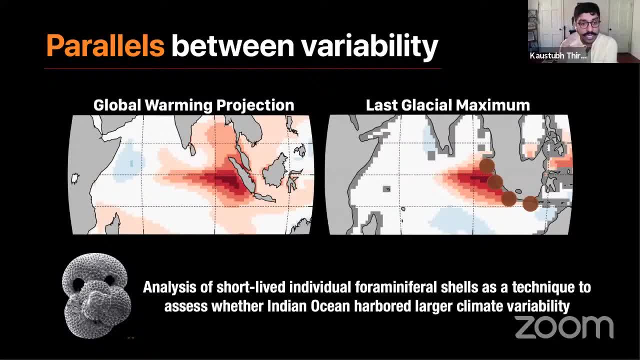 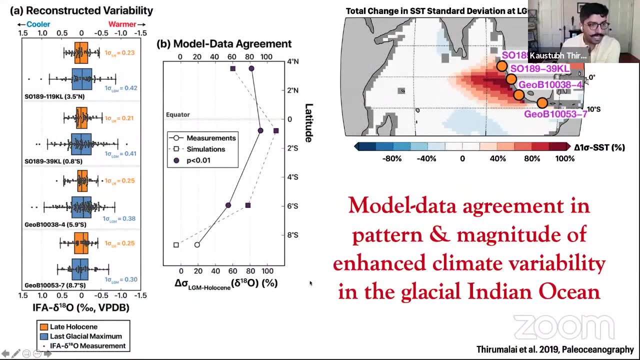 shells. uh, we use that as a technique to assess whether the indian ocean actually harbored larger assignment variability in the past. uh, so i'm going to cut to the chase here and show you some of these results. uh, there's a lot going on here, so let me walk you through with from the left-hand. 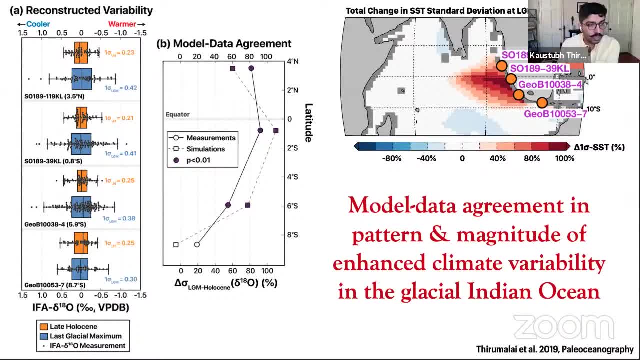 side to the right-hand side. so we chose these four different sediment cores, and each one of these right here represents an individual foraminiferal measurement. the orange represents modern sediments and the uh, basically the blue represents last glacial maximum sediments, and so the point. 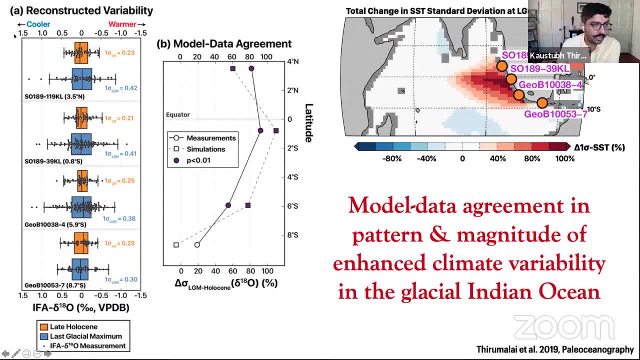 here is that these are auctionized stove measurements. uh, and suffice to say that on the left-hand side is cooler and on the right-hand side is warmer. i have, of course, removed the mean cooling between the two states. i've put everything, aligned it on zero, just to look at the variability. 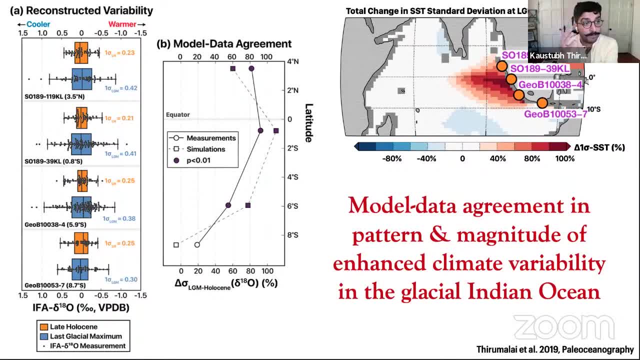 so, of course, the last glacier maximum is cooler, but we're trying to compare the variance between the modern state and the last facial maximum and, uh, essentially what emerged out of this analysis is that, uh, pretty much across these three different cores, uh, where the model actually simulates increased variability, we actually see that the data, these, 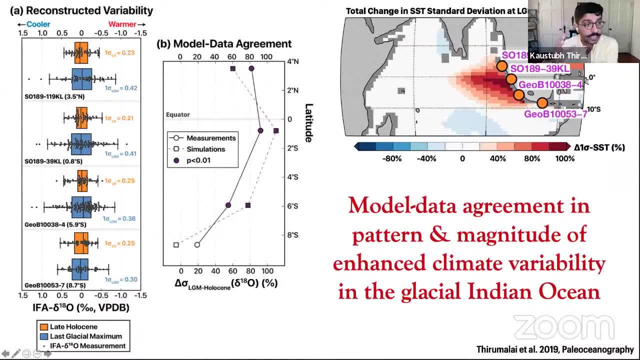 foraminifera are indicating much larger variance both in the cold state, in the cold tails as well as in the warm tails during the last glacial maximum. so you can see here how these variants increases. right here, uh, and in the in our southernmost site, we actually did not see a statistically significant 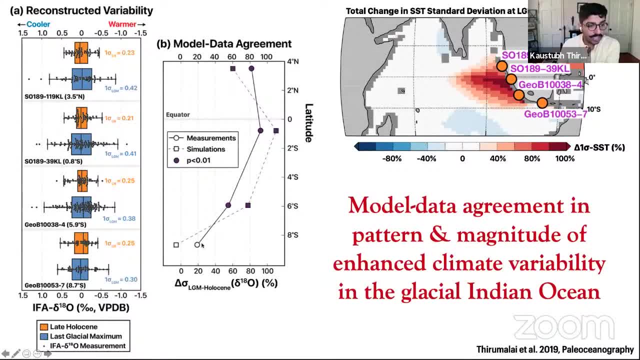 uh change in variance. however, that is also what the model simulates as well. so right here is the translation of these individual foraminiferal results into the standard deviation, the magnitude of standard deviation between uh, the change between the modern and last glacial maximum and. 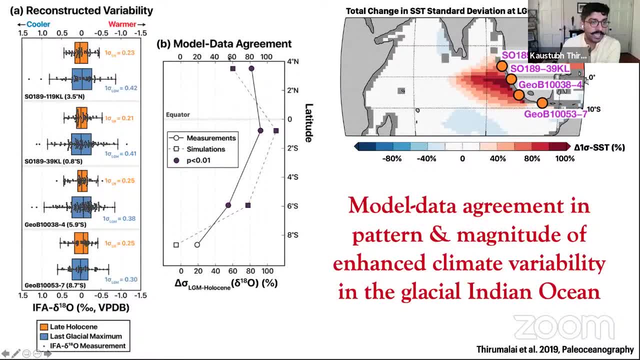 the circles are telling you about what the actual data say, and the squares here are from those particular grid points in the actual model. so there's model data agreement here, in both the pattern as well as the magnitude of enhanced climate variability in the glacial indian ocean. so both these completely disparate 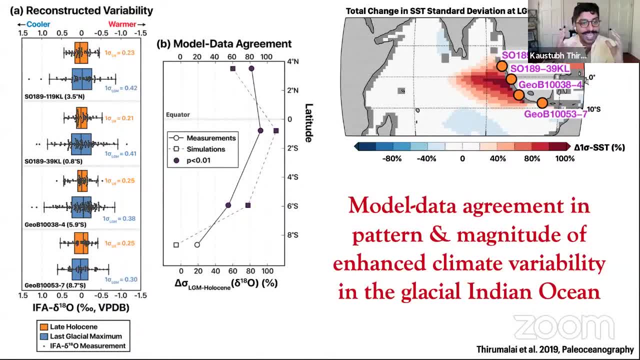 lines of evidence are telling us that the indian ocean is capable of harboring a lot larger climate variability than we see today. so the sst variability that actually gives rise to a lot of these hydroclimatic extremes, uh was was a lot larger in the last glacial maximum. 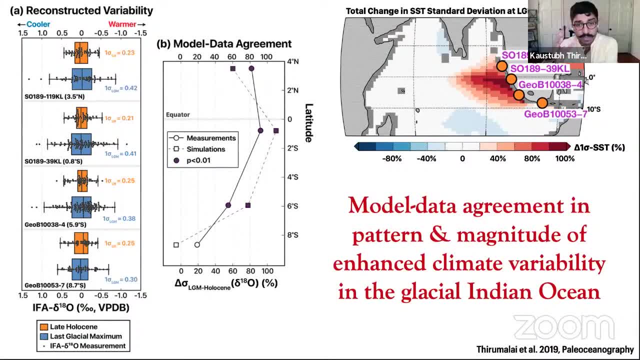 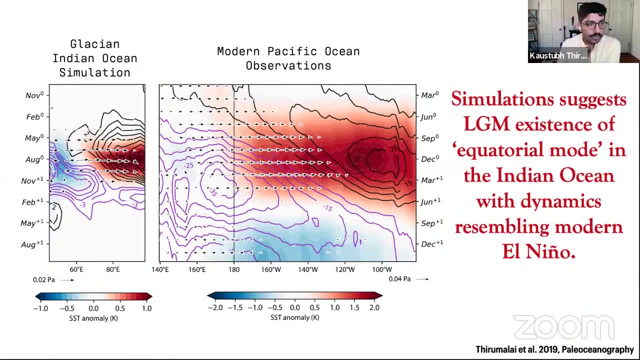 and so this agreement between the model and the data actually gave us, uh, some confidence in investigating the model and to try to see what nuances the model's dynamics actually can tell us about. so, uh, this is a huffmuller diagram. i'll walk you through what this exactly means. 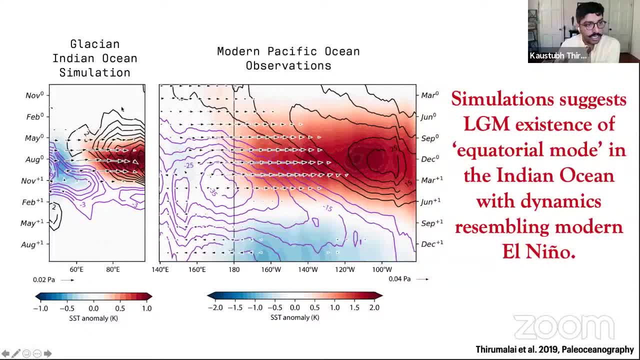 but on the left hand side is the simulation for the glacial indian ocean and on the right hand side is uh, observations from the modern pacific ocean. so essentially, what we're going to do is we're going to start by reading the whole theory of interstellar temperature. so this is a composite of all el nino events and la nina events that happen on record in terms of instrumental observations in the pacific ocean. 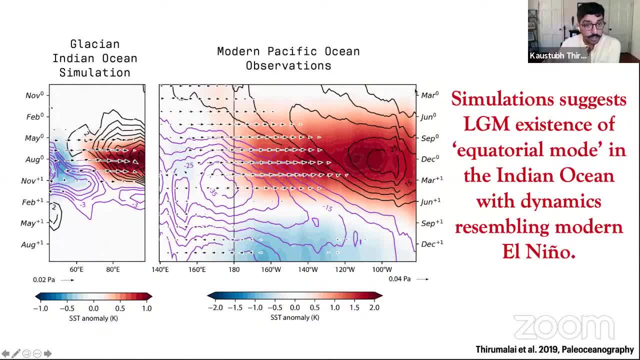 and the way to read this is: you start from the march of year 0 all the way up, so you're going forward in time. as you move down in this plot to december of the next year, the colors are telling you about the intensity of sea surface temperature warming or cooling. 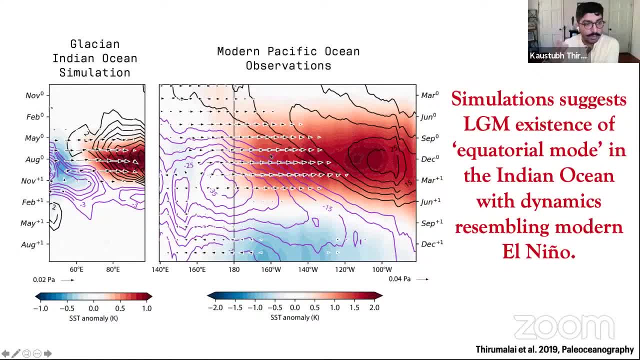 the arrows are telling you about the direction of wind stress anomaly, And these contours are telling you about changes in the subsurface depth of the thermocline or the subsurface structure of the ocean. And so, essentially, what happens during an average El Nino event is that the central and the eastern Pacific basically warm, and this warming peaks during December. 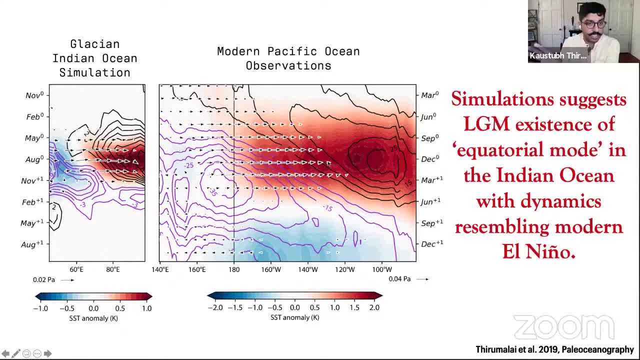 And this warming occurs with the onset of these anomalous westerlies in the Pacific Ocean and a deepening of the thermocline in the eastern Pacific. Now we see very, very similar dynamics that are occurring in the Indian Ocean, according to the simulation as well. 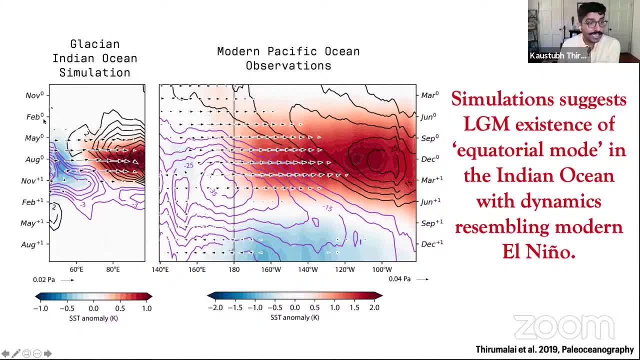 There are some differences that you can clearly see here, but I would like to highlight the similarities in terms of this sort of dipolar nature in the equator. So these are both averaged across five north to five south. So these are equatorial processes that we're looking at. 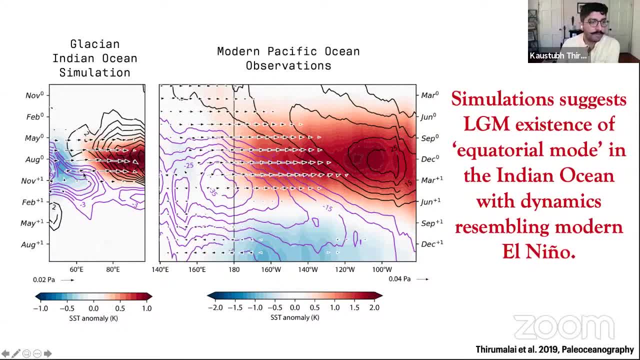 And you see, this onset of these anomalous westerlies that give rise to warming here, That that are accompanied by a halting of upwelling as well. Some of the key differences: that this tends to peak during August, during the summer monsoon months, whereas the El Nino, of course, as we all know, peaks during the December, January, February time. 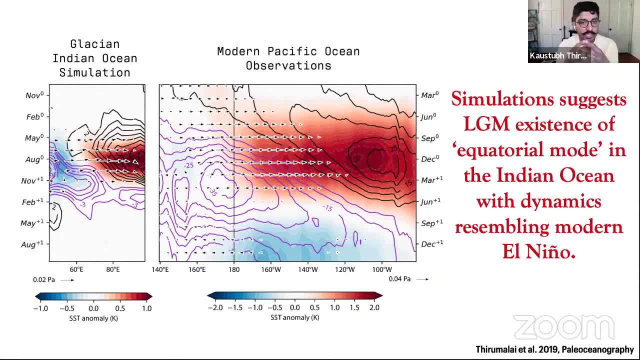 OK, so the simulations. when we dive deeper into them, they suggest that the Indian Ocean harbored this equatorial mode, or we're calling it the Indian Ocean El Nino, colloquially. But this Equatorial mode is unobserved today. 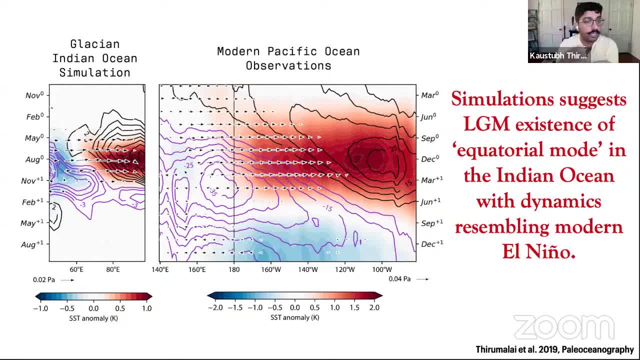 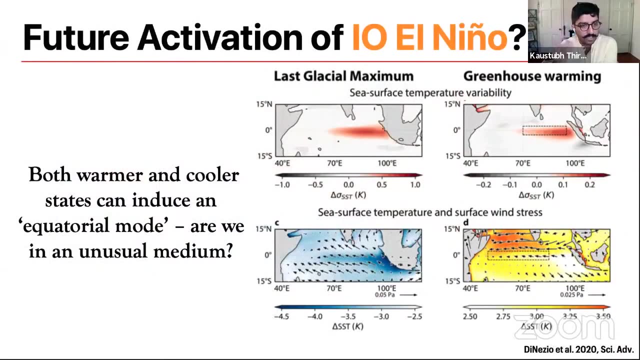 We do not see this mode in the permanent mean state of the Indian Ocean over observations, But during the last glacial maximum this mode seems to have existed And the data, the form nifl data, seem to confirm that. Now, very interestingly, we have to ask the question about the future activation of this Indian Ocean, El Nino and model simulations from a paper from that we put out last year from my collaborator Pedro D'Anezio. 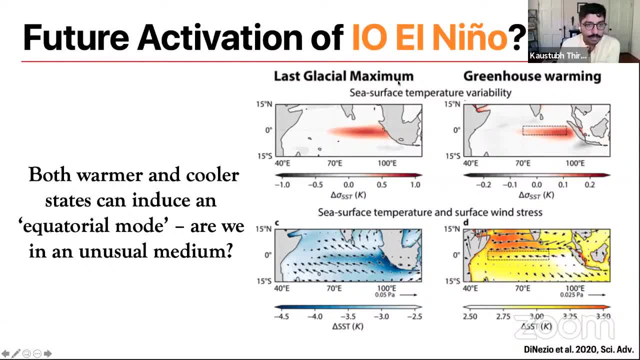 And you can see the sort of the parallels between the last glacial maximum in terms of sea surface temperature variability and when it comes to greenhouse warming. So this is really unusual that you have to think about it. that are we currently in an unusual state? 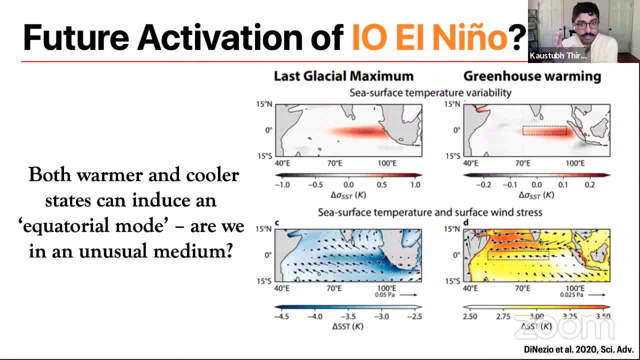 So did the entirety of human civilization and the sort of the rapid flourishment of populations in this densely populated region. did that happen under sort of a precarious balance, such that today we're in neither extreme state, Neither a cold state, nor a warm state? 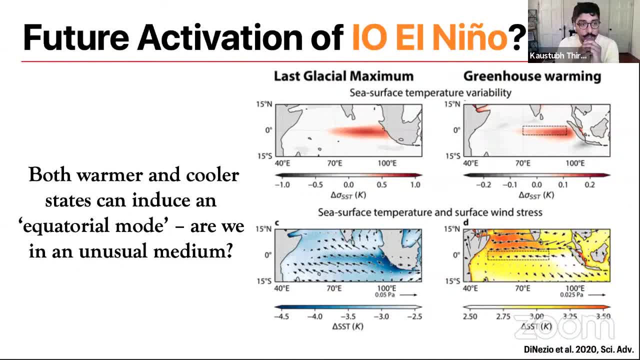 And we don't have this sort of equatorial mode that exists in the Indian Ocean. But simulations in concert with paleoclimate data indicate that the Indian Ocean can harbor this larger variability. So both warmer and cooler states can potentially induce this equatorial mode. 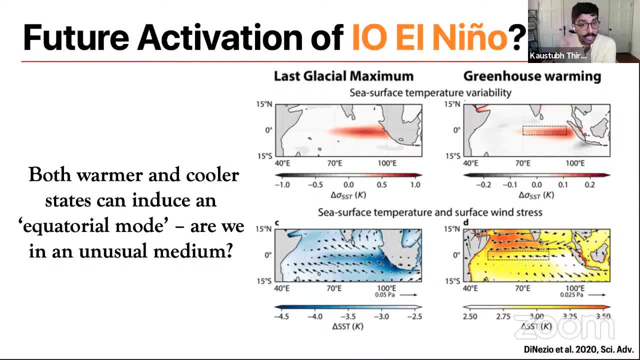 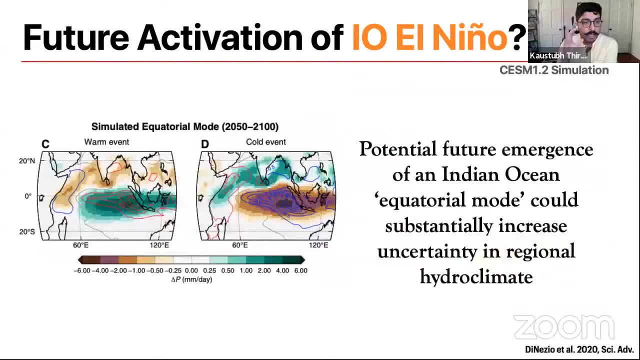 So are we at kind of the precipice where this mode can actually be triggered and be activated? So some of our research we actually looked into what might happen If this mode was activated in the future, and I'm going to spare you the details. but the bottom line is that if this mode were to get activated, we're going to have a lot more uncertainty in anticipating hydroclimate changes across this region. 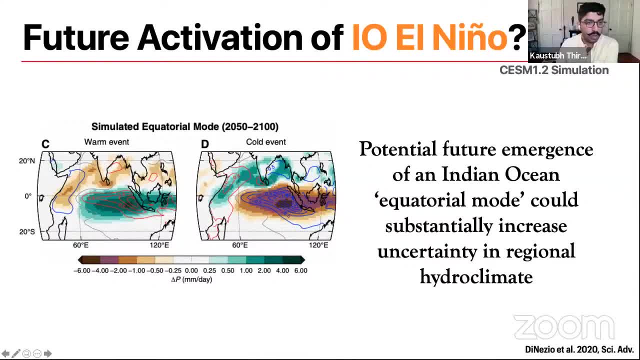 So you can kind of see here that during the warm events of this mode and the cold events of this mode, there are characteristic hydroclimatic signatures here that are basically going to impose a lot of variability and that are going to contribute to extremities in these densely populated regions. 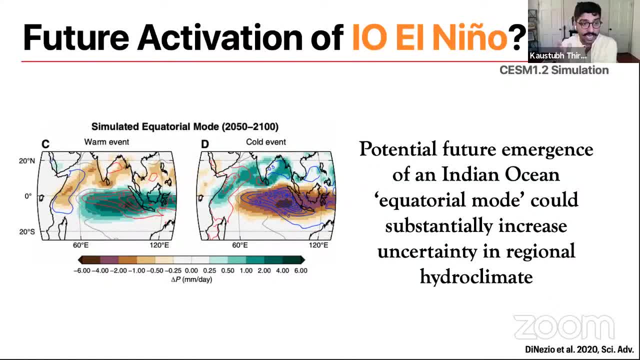 And so this is alongside the impact of El Nino, for example, on this region, as well as the Indian Ocean dipole on this region, And they're going to have substantial interactions with the Indian monsoon and the Asian monsoons that are going to further increase the uncertainty in future regional climate evolution in this particular region. 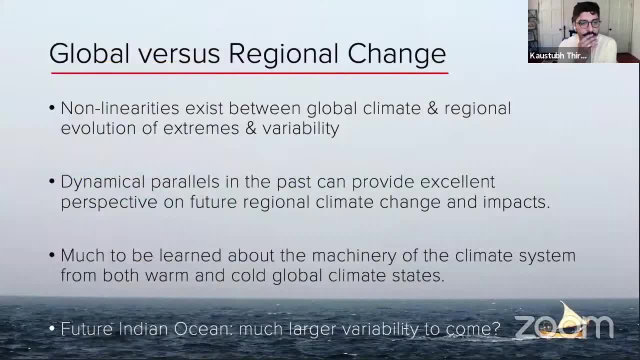 So I'm going to stop right here and just quickly summarize what I've just presented on global versus regional change- admittedly just for one region, So I apologize for that- not necessarily showcasing some of the other regions, but given that this is where I focus on and where I think a lot of vulnerable populations are going to be dependent on sort of how well we anticipate the future trajectory of regional climate change, 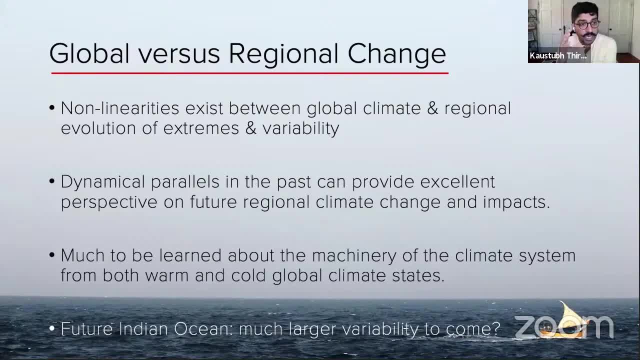 So the four key points that I'd like for you all to take home with you is that there are nonlinearities that exist between global climate and regional climate evolution, And so just because the world is going into a warmer state doesn't necessarily imply That you know there's going to be a sort of concurrent increases or changes in the extremes across the board in many of these regions, and each region is going to have 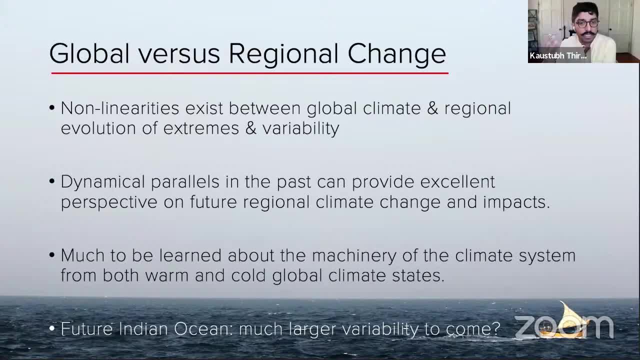 sort of its own sensitivity, both socio economically, but also dynamically, with different types of extremes, And so these dynamical parallels in the past can provide really excellent perspective on future regional climate change. And there's much to be learned about the machinery of the climate system when we look back into both warm and cold global 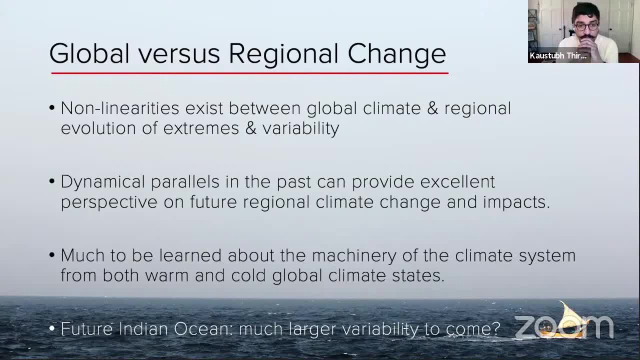 Climate states, as just here, and he kind of showed with the extreme states in her previous talk. and so the bottom line for the future Indian Ocean is that you know there's a question of: is there much larger variability Yet to come? so i'll stop right here and i'm happy to take any questions. so thank you very much for your time and for the opportunity to present here again, thanks. 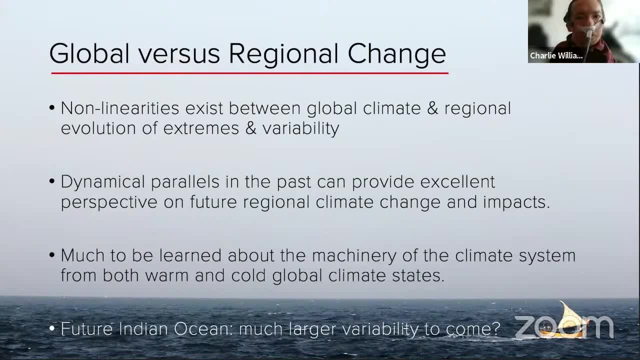 Okay, thank you very much, Really, really interesting. So we have a number of questions, and firstly from one of the panelists: are there any proxies that can tell us about daily or weekly scale variability? Excellent question. so the question is: are there proxies that can tell us about daily or weekly temperature change? 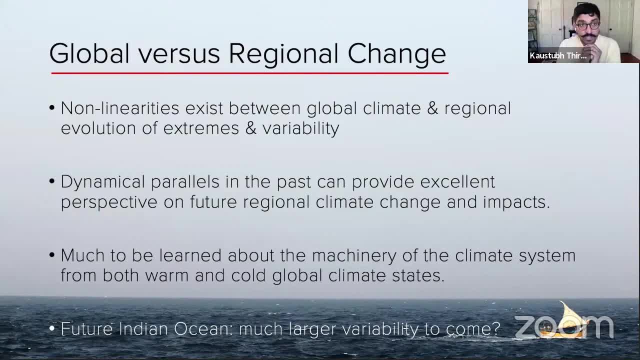 One. let me just say that when you look at these time periods going further back in time, it's extremely difficult to get well resolved proxies. But that said, New techniques, reinvestigating, sort of well developed proxy methodologies, are really beginning to show us some really high resolution daily and weekly. 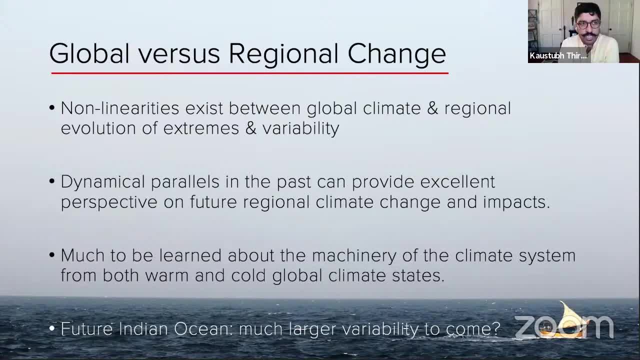 reconstructions. now it's still. admittedly, there's a lot of uncertainty, but I can give you an example: in a study that I was involved with a couple years ago, There are some really, really fast growing gastropod shells, for example, so snails, and, in particular, things like, you know, the giant axe. 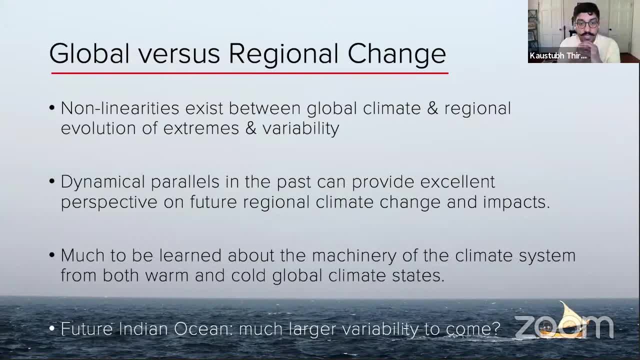 African snail, for example, that grow really fast and and we've shown that they actually incorporate into their skeleton geochemical fingerprints of weekly to sub seasonal rainfall variability. And we can find these shells, for example, across outcrops, and we can actually query them as to what they might tell us about, for example, active periods or great periods in the monsoon domain. 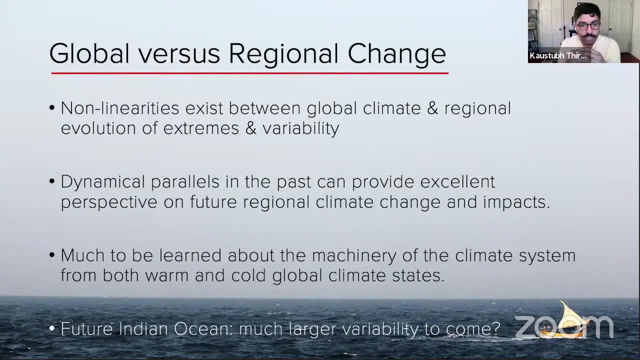 Other ways that people can actually look into these super high resolution, Ultra high resolution variability is you can you can really scan sediments, for example, that are accumulating at a very, very fast sedimentation rate, and try to understand things about weekly to sub seasonal climate variability. 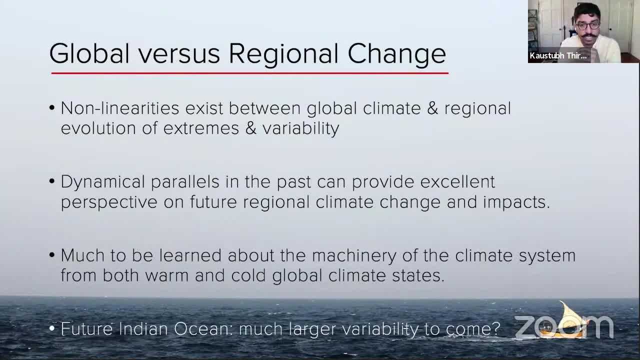 And then, finally, i'll just make a pitch for ostracods. these are basically crustaceans that that live in both lacustrine as well as marine environments, and They actually molt, and when they molt, they basically deposit their entire calcium carbonate shell In a matter of hours. 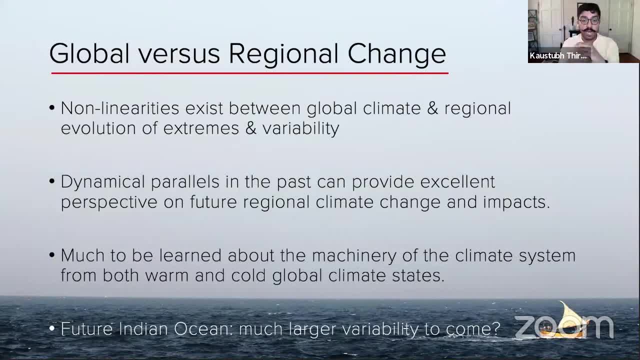 Today, And so they're going to lock in whatever the environment, those those geochemical signatures of the environment at that particular time. so there are ways forward. it's fraught with uncertainty right now but I think with More records and improve nuances in the technologies we can really try and get a handle on what that might actually hold for us in terms of our understanding of future changes on those really ultra high resolution timeskills. 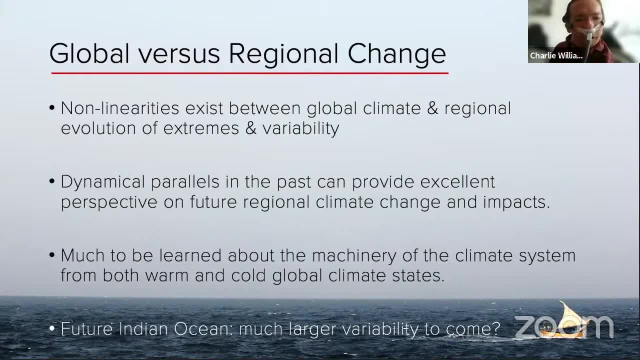 Okay, thank you. so we have another question. Can you speculate on what the role of the Indian Ocean El Nino might have had during previous greenhouse climates? Yeah, this is a really good question. Short answer is that we have a hunch, but we are yet to test this. 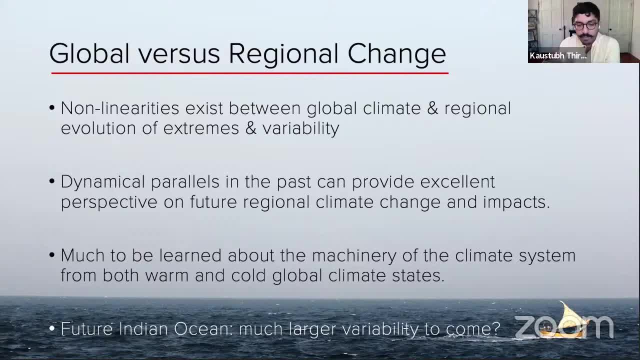 So we can look into, for example, many of the warmer analogs that multiple people here in this workshop have described. for example, you know, the marine ice stove, stage five, or the Plants, Plants, Plants, Or the Pt M, and we can try to think about you know what. 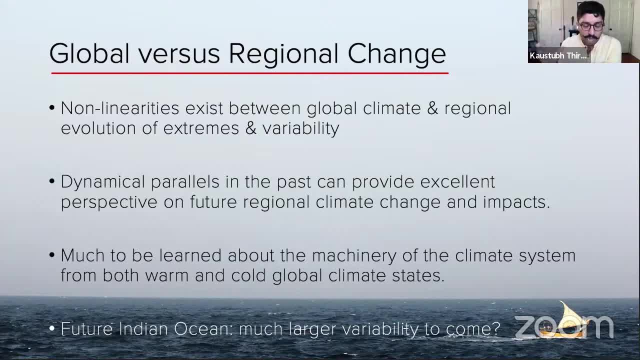 The Indian Ocean, as you know, with the, with the modern paleo, with the modern geography, what that might hold for this onset of the Indian Ocean, El Nino, during these greenhouse periods, and so this is a work in progress, but we do have some simulations for the last interglacial as well as for the mid Holocene. 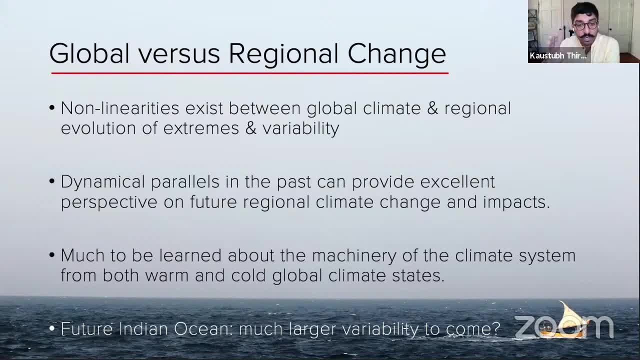 That seemed to suggest that Perhaps a weaker but still a consistent form of this Indian Ocean, El Nino, existed during both both of these time periods as well. we don't necessarily have the data yet- that's a work in progress- but that's an excellent question and something that we're trying to focus on. 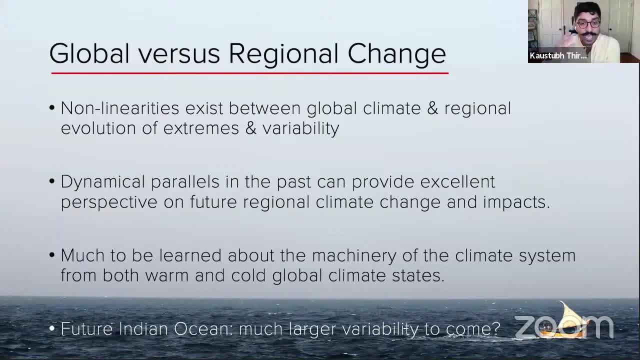 whether we can look into the geological past for greenhouse periods and try to see whether the indian ocean, el nino or this equatorial mode existed. okay, and then we have, i think, time for one more question from the audience. so the question is: how does the indian ocean 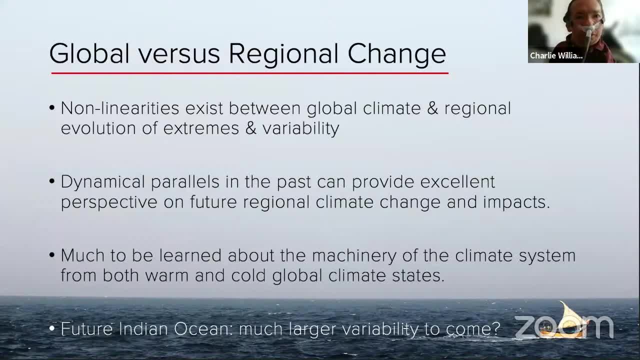 interact with the pacific enzo and are there any patterns for intensifying and stabilizing impacts? again, that's a very excellent question because, uh, we know that today many of those extremes, uh, including the ones that i showed you, are really triggered by changes in the pacific el nino. 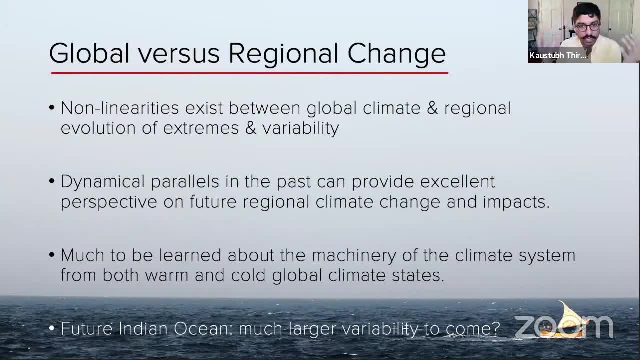 and so the pacific el nino has a strong hold on the indian ocean realm, and the short answer is that when you look at the last glacial maximum, according to some simulations and some data, it's a little more uncertain. in the pacific, we have evidence that the el nino and the enzo system was actually weaker during. 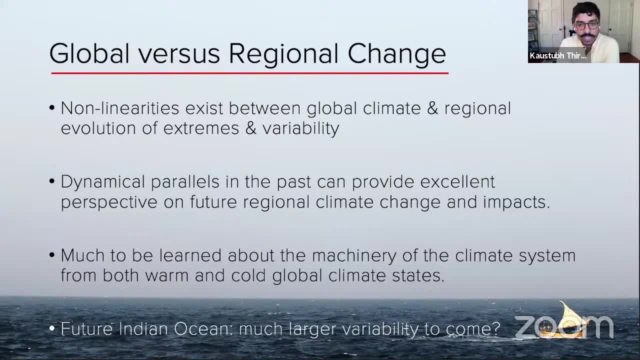 the last glacial maximum and because it weakens the simulations actually indicate that the uh sort of the hold of el nino on the indian ocean realm also weakens and so that allows the indian ocean dipole and this equatorial mode to emerge in the indian ocean and really 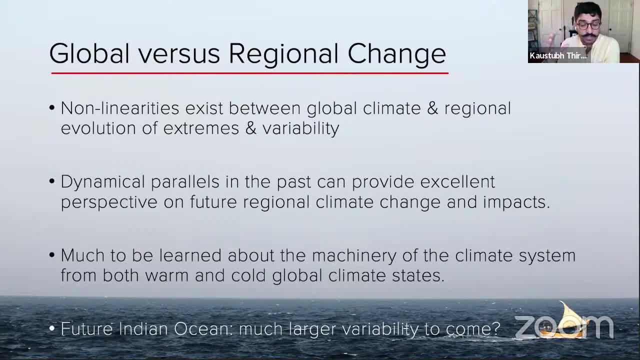 dominate the sst variability and which is much more increased relative to today. uh, in the future, we all we we're uncertain about what enso is going to do, and so it's really a key sort of a thing that we need to pin down for regional climate evolution. 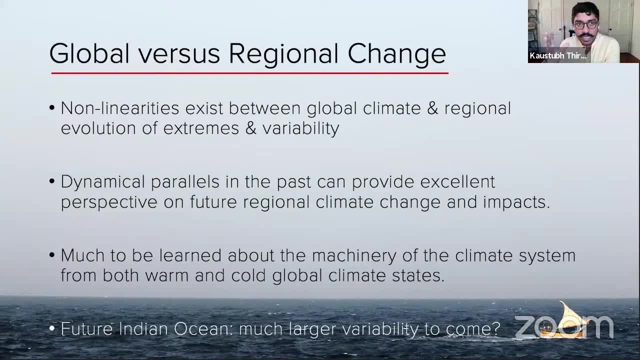 but what we can really say in terms of stability or not, is that enso serves to sort of, uh, impact the monsoons in the forthcoming year and, uh, this mode seems to impact the monsoon during that particular year itself. so, whatever it's going to be, we're going to, we need to further. 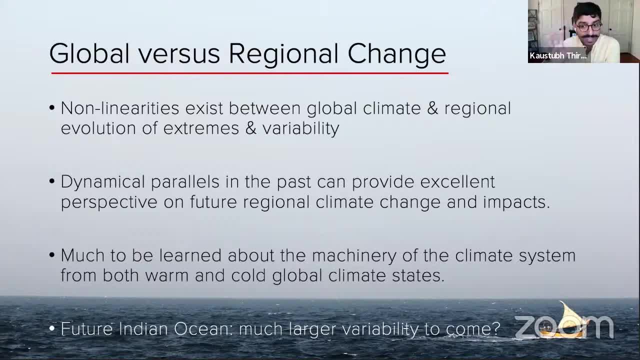 investigate the exact sort of relationship between the two, but, that said, we know that they're going to. both of them together are going to impose more uncertainty in their evolution and, furthermore, on their impacts- uh for hydroclimate across uh the indian ocean realm as well as asia. 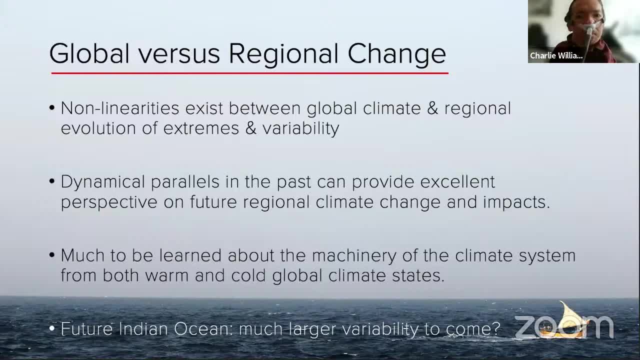 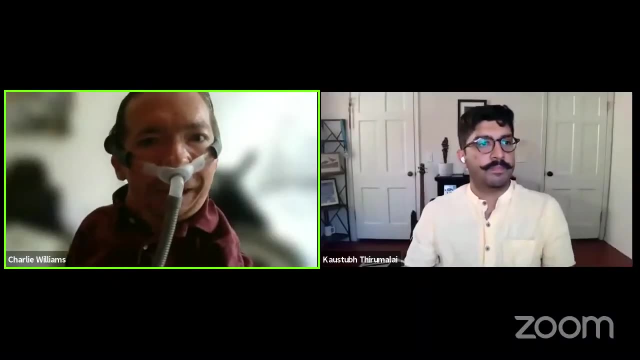 okay, well, thank you very much again, kyle. i think that's probably all we have time for, and there are a couple more questions questions in the q a, so please do check that out, um, as we as we go through the next talk. so i think now we have the- uh, one minute pre-recorded talk. so, alicia, are you able to press? 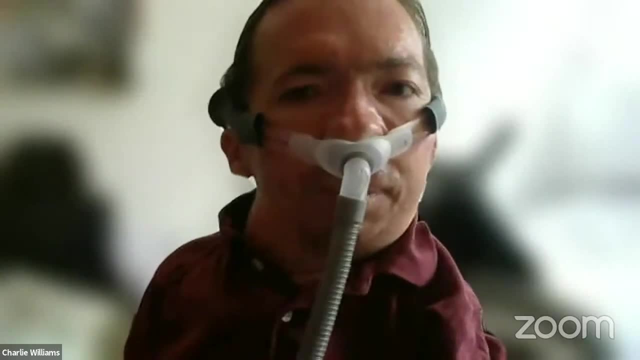 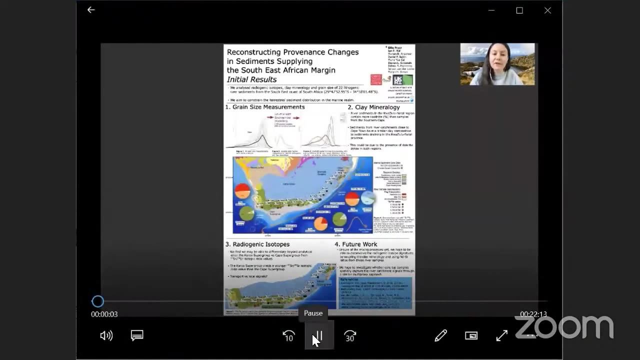 play on those. we sampled south african rivers and isolated the finest green size fraction. this clay fraction has the highest potential to integrate the river catchments into the marine realm, as this fraction is more easily transported than coarser fractions. we find three m. members explain 89 percent of the variance in the grain size data. 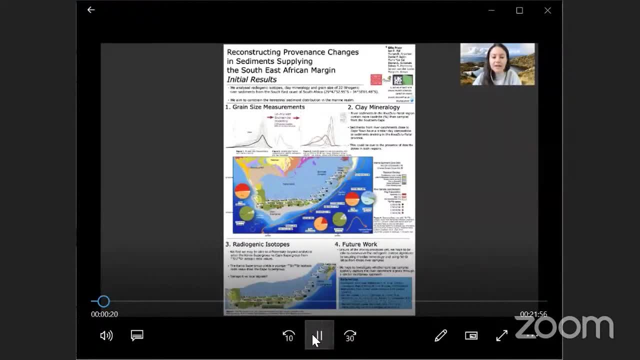 and additional m members added are in the coarse fraction when compared with typical marine m members from the southeast african continental margin. m number three from the river data fits better with m number two from the marine data. we analyzed clay minerals and radogenic isotopes from this isolated clay fraction to minimize the strontium grain size offset. we 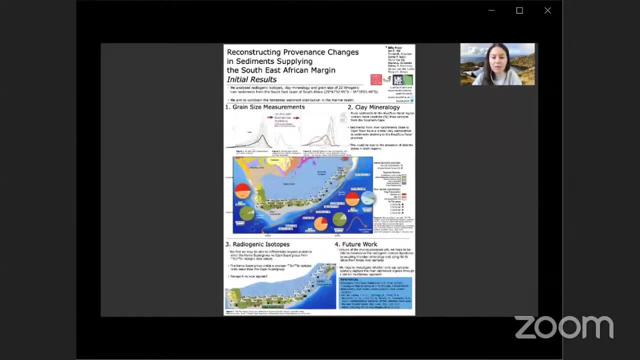 identified that karoo supergroup samples have a younger strontium fingerprint than the cape supergroup, beyond analytical error and we hope to constrain the provenance of these river sediments by coupling the clay mineralogy and using neodymium strontium ratios, as neodymium is. 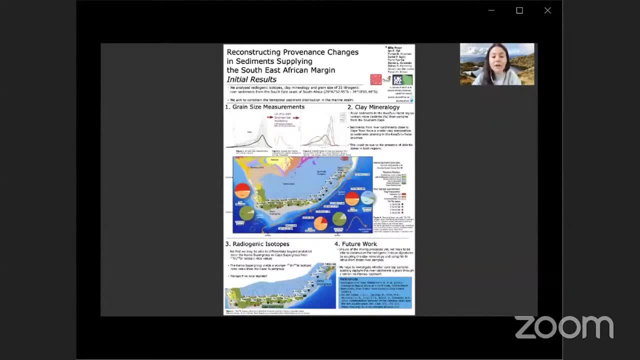 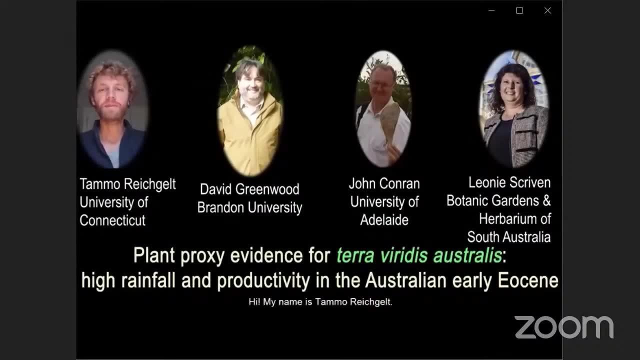 less sensitive to grain size. if you have any questions, please come to my breakout room. thank you, hi. my name is thomas reichel. let me tell you about our poster on easing plant fossils from australia and what they can tell us about climate and primary productivity in the ancient land down. 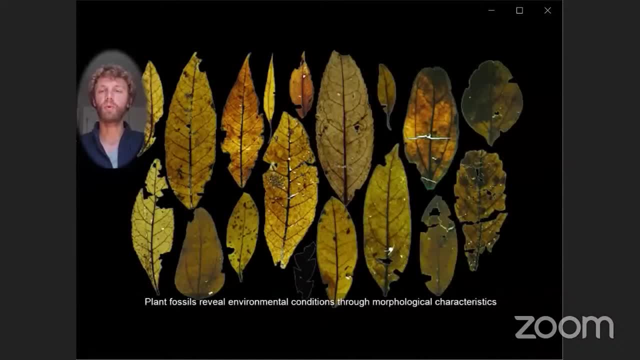 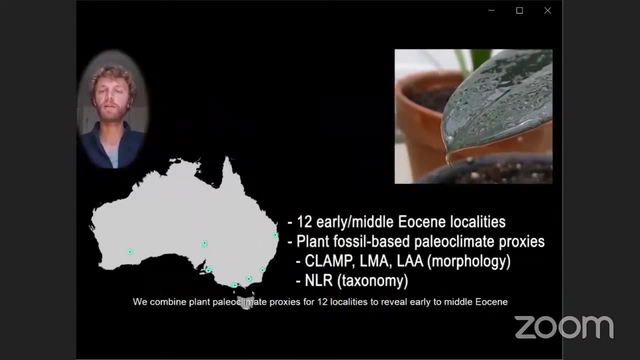 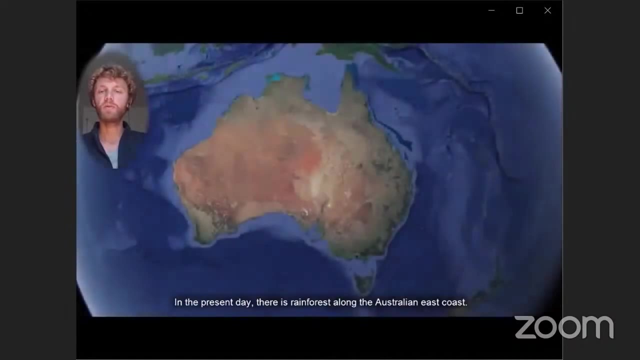 under plant fossils reveal environmental conditions through morphological characteristics as well as taxonomic affinities. we combine plant paleoclimate proxies for 12 localities to reveal early to middle eocene temperature, rainfall and net primary productivity. in the present day, there is rainforest along the australian east coast. these forests have high rainfall and primary productivity. 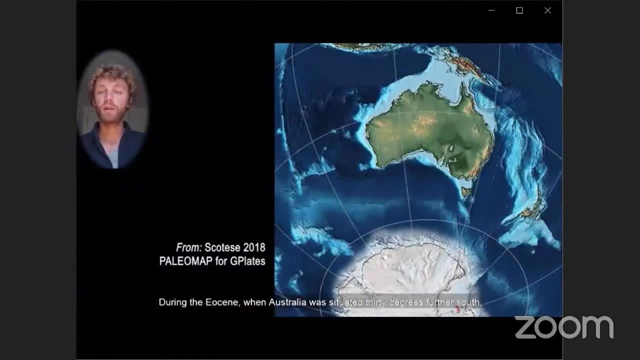 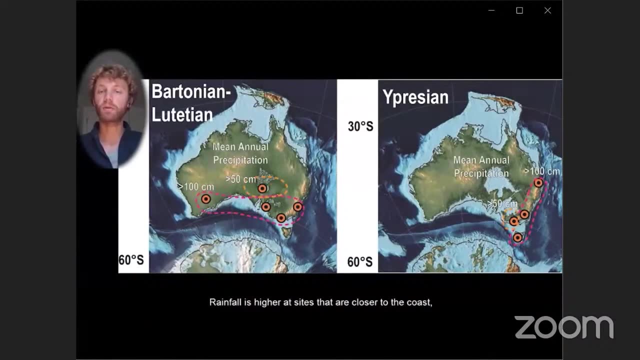 especially in the tropics. during the australian east coast there is high rainfall and primary productivity, especially in the tropics, the eocene. when australia was situated 30 degrees further south, temperatures were uniformly subtropical. rainfall is higher at sites that are closer to the coast, but inland sites experience 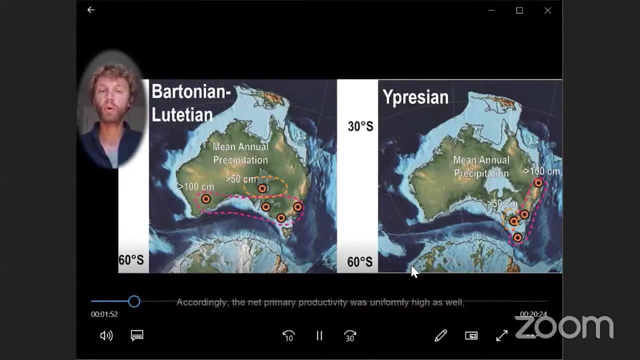 at least four to five times as much rainfall as they would today. accordingly, the net primary productivity was uniformly high as well. similar to subtropical forests today, this is in stark contrast with the large areas of grassland and deserts on the australian continent, where net primary 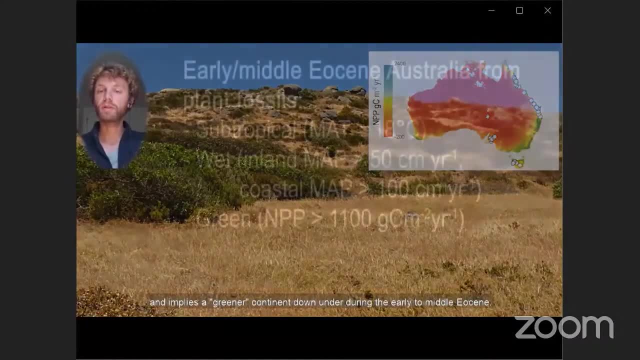 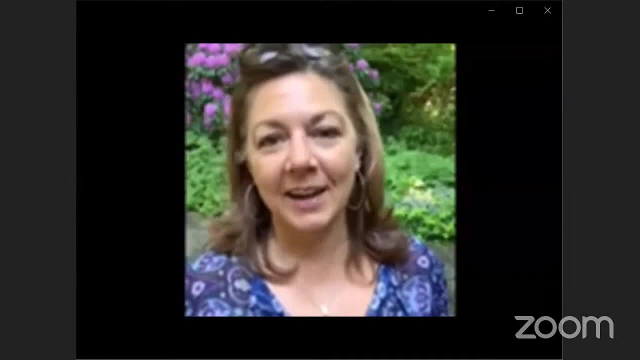 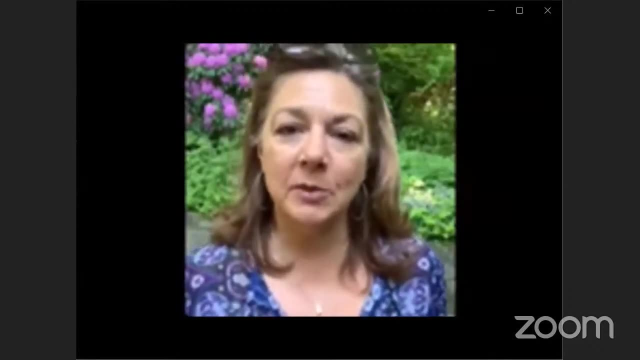 hi, i'm marcy robinson in my backyard in fairfax, virginia, and i'd like you to come take a look at my poster on paleoclimate signals in the coastal plain sediments. um, we've looked at coastal plain sediment cores and outcrops from the eastern parts of virginia and maryland along the mid. 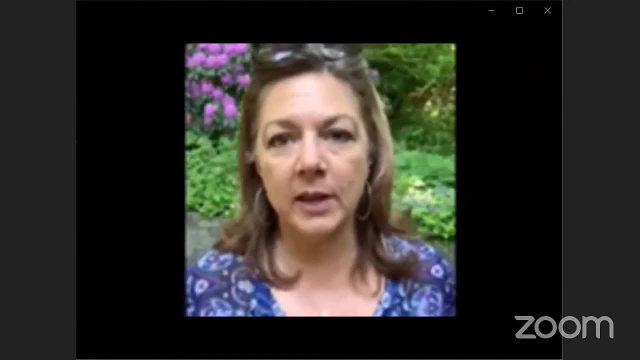 leading coastal plain of the united states and we've looked for sediments from three warm periods. and we've looked for sediments from three warm periods when sea level was high compared to today, when sea level was high compared to today and marine sediments were deposited on today's 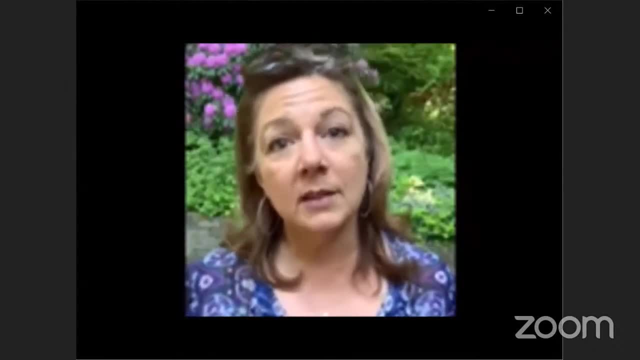 and marine sediments were deposited on today's coastal plain: the paleocene eocene thermal maximum coastal plain, the paleocene eocene thermal maximum, the miocene climate optimum and the mid-peach the miocene climate optimum and the mid-peach indian warm period. in short, we found that these 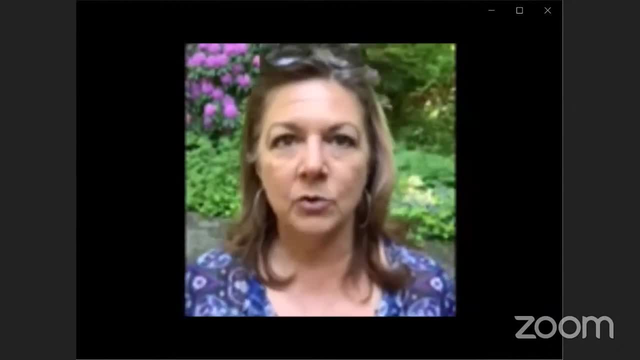 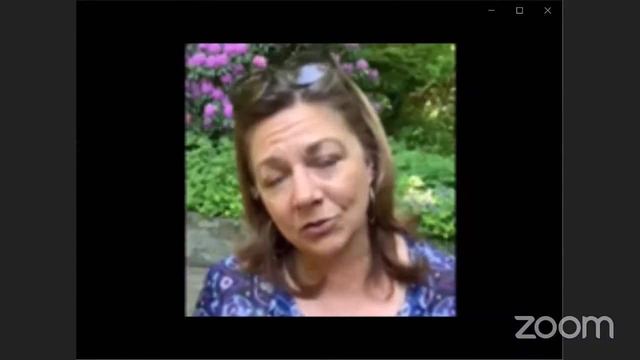 indian warm period. in short, we found that these sediments contain excellent snapshots of extreme sediments, contain excellent snapshots of extreme climate states and record valuable quantitative climate states and record valuable quantitative paleoecological data um. this work is important. paleoecological data um this work is important because these records capture the nature of 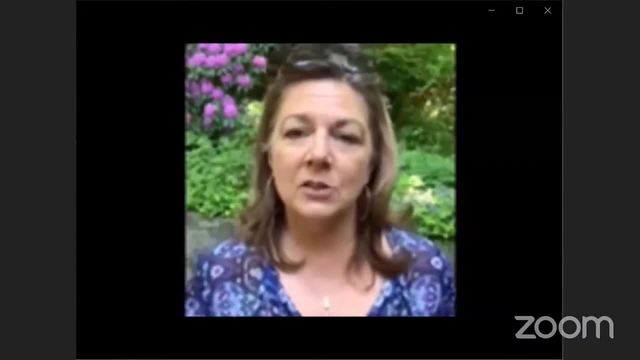 because these records capture the nature of climate-induced changes in this area where a lot climate-induced changes in this area where a lot of people live and it highlights the differences of people live and it highlights the differences within a single warm interval that might have. within a single warm interval that might have multiple pulses of sea level and all of this leads. 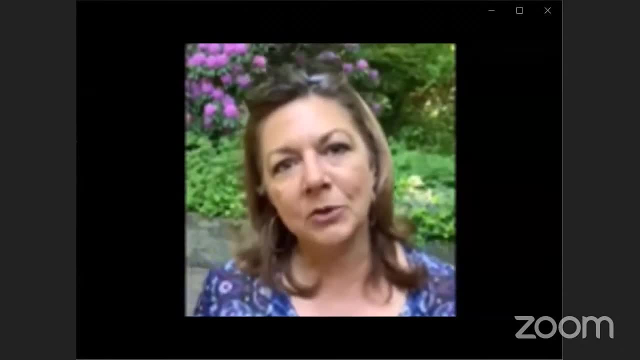 multiple pulses of sea level, and all of this leads to a better understanding of potential future, to a better understanding of potential future impacts. so come, take a look at my poster and feel impacts. so come take a look at my poster and feel free to ask me questions. thank you, hi, everyone. 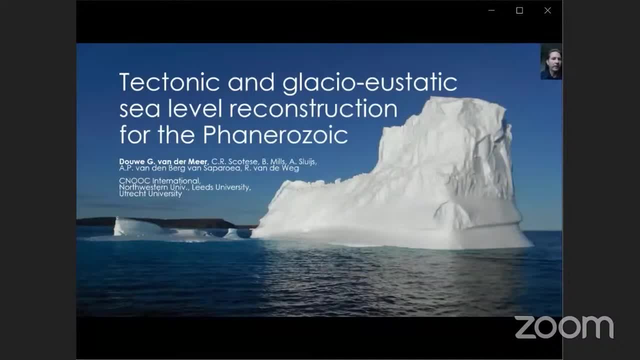 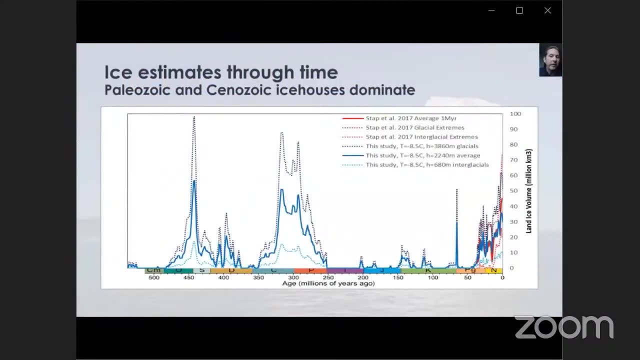 free to ask me questions. thank you, hi. everyone. welcome to our talk on the tectonic and glacier. welcome to our talk on the tectonic and glacier. eustatic sea level, reconstruction for the entire eustatic sea level. reconstruction for the entire phanerozoic. these are our ice estimates through. 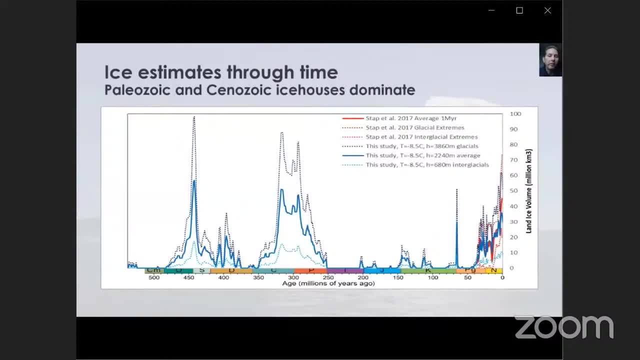 these are our ice estimates through time in solid blue. we have our one million time in solid blue. we have our one million time in solid blue. we have our one million year steps. reconstruction of a land- ice year steps. reconstruction of a land- ice year steps. reconstruction of a land- ice volume. 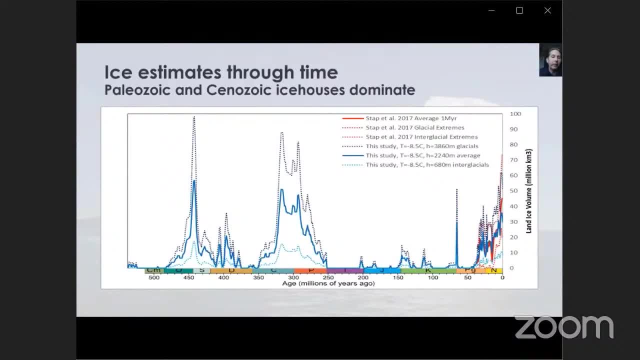 volume, volume, and in the dotted lines we have our ice and in the dotted lines we have our ice and in the dotted lines we have our ice. volumes, volumes, volumes both for glacials and interglacials, so both for glacials and interglacials, so 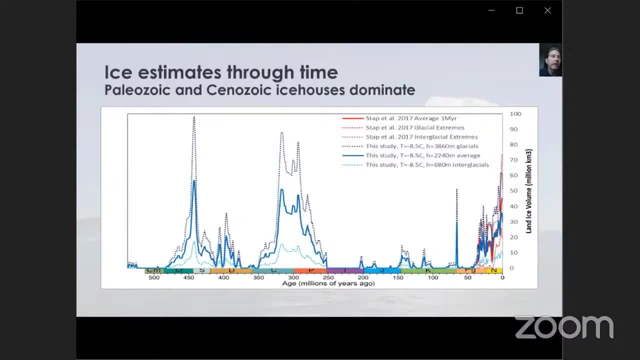 both for glacials and interglacials. so these are the peaks of ice variation. these are the peaks of ice variation. these are the peaks of ice variation that we, that we that we estimate that could have happened within estimate, that could have happened within estimate, that could have happened within, or less than, one million years. so you 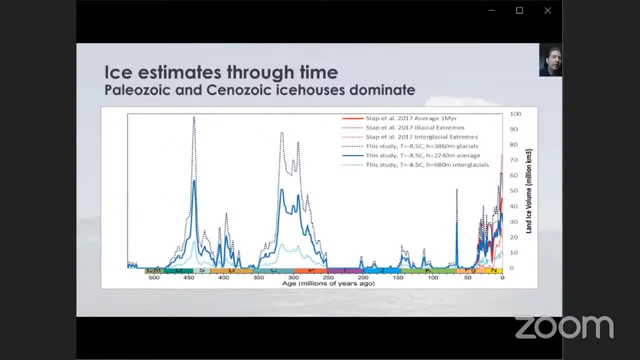 or less than one million years. so you or less than one million years. so you can see, for example, in the late, can see, for example, in the late, can see, for example, in the late paleozoic ice house there was a lot of paleozoic ice house, there was a lot of. 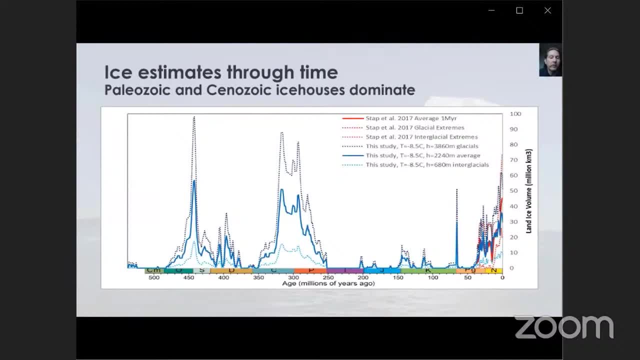 paleozoic ice house, there was a lot of variation in land ice volume, variation in land ice volume, variation in land ice volume and, as a consequence, this leads to a and, as a consequence, this leads to a and, as a consequence, this leads to a large variation in sea level 2.. 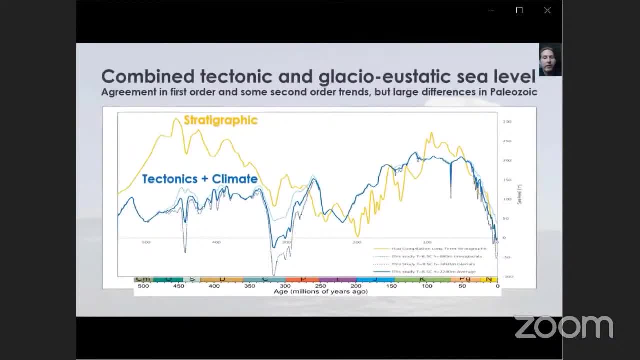 large variation in sea level 2.. large variation in sea level 2: when we combine our sea level curves, when we combine our sea level curves, when we combine our sea level curves with a stratigraphic estimate from a with a stratigraphic estimate from a. 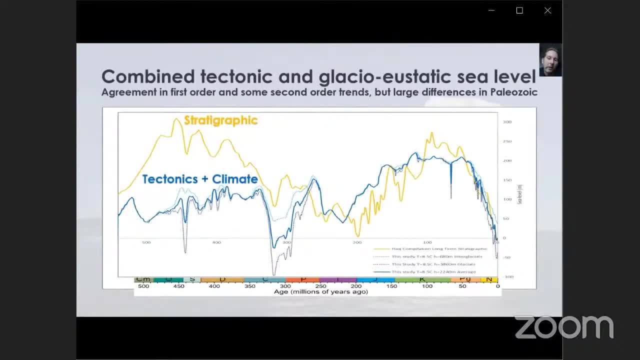 with a stratigraphic estimate from a compilation of studies of haq. compilation of studies of haq. compilation of studies of haq. you can see there's a lot of similarities. you can see there's a lot of similarities. you can see there's a lot of similarities at first order level in the mesozoic and 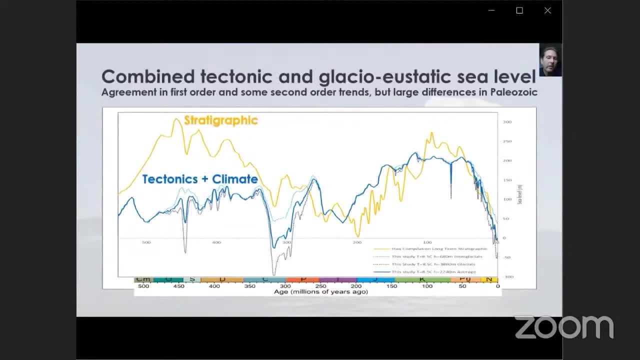 at first order level in the mesozoic and at first order level in the mesozoic and cenozoic- cenozoic, cenozoic, but to a lesser extent. we're in a lesser but to a lesser extent we're in a lesser but to a lesser extent we're in a lesser agreement for the paleozoic. 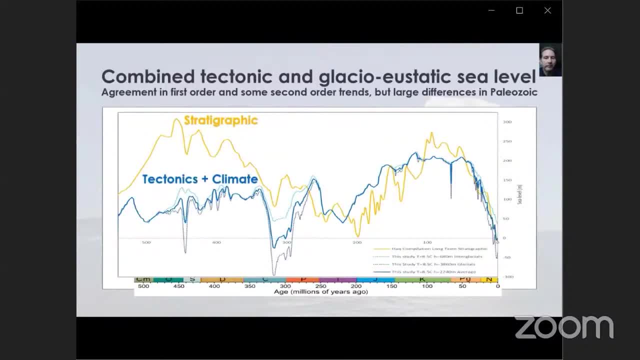 agreement for the paleozoic, agreement for the paleozoic, which we need to research further, which we need to research further, which we need to research further. hi, i'm tom gurnan and i want to talk. hi, i'm tom gurnan and i want to talk. 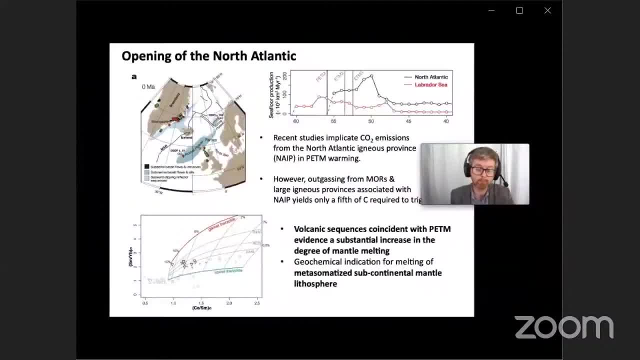 hi, i'm tom gurnan and i want to talk to you about mobilization of mantle carbon, to you about mobilization of mantle carbon, to you about mobilization of mantle carbon during the ptm, during the ptm, during the ptm. so some recent studies have implicated: 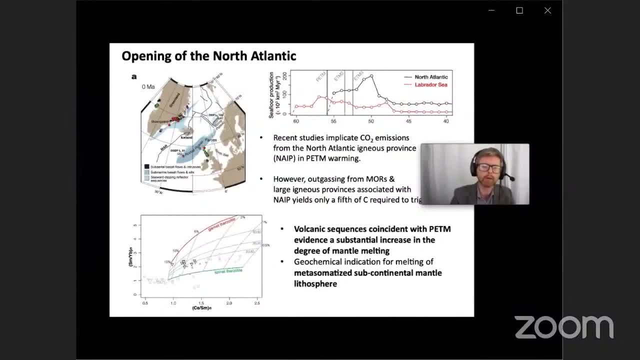 so some recent studies have implicated. so some recent studies have implicated the north atlantic igneous province, the north atlantic igneous province, the north atlantic igneous province, in driving ptm warming. however, using in driving ptm warming, however, using in driving ptm warming, however, using plate simulations, we calculate that 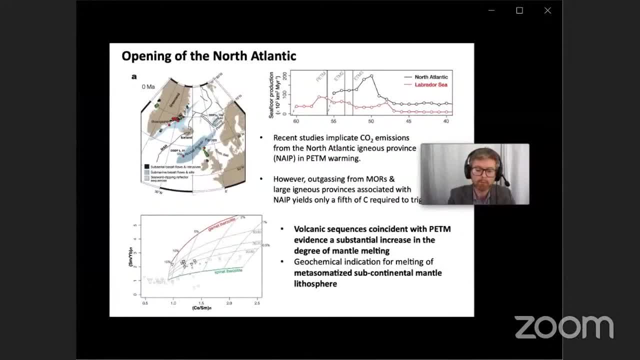 plate simulations. we calculate that plate simulations. we calculate that ocean ridges and large igneous provinces, ocean ridges and large igneous provinces, ocean ridges and large igneous provinces at this time, at this time, at this time, yield only about a fifth of the carbon. 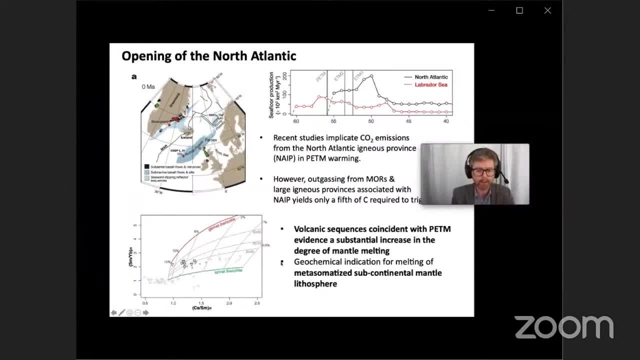 yield only about a fifth of the carbon, yield only about a fifth of the carbon required to drive that warming, required to drive that warming, required to drive that warming. instead, we identified volcanic. instead, we identified volcanic. instead, we identified volcanic sequences spanning the ptm that showed. sequences spanning the ptm that showed. 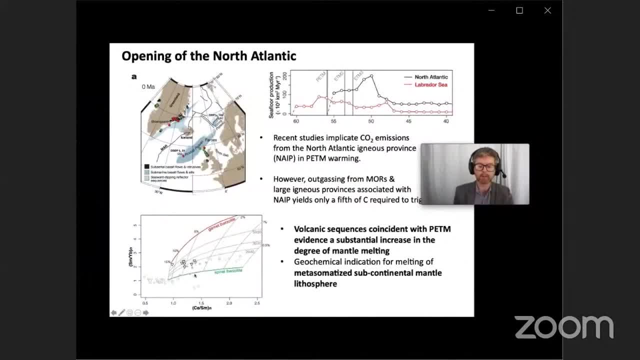 sequences spanning the ptm that showed geochemical evidence for substantial geochemical evidence for substantial geochemical evidence for substantial increases in mantle melting at this time. increases in mantle melting at this time. increases in mantle melting at this time which involved metasomatized lithosphere. 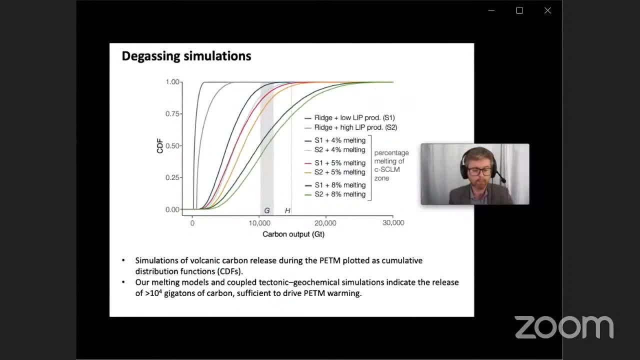 which involved metasomatized lithosphere, which involved metasomatized lithosphere, which is a key reservoir of carbonate, which is a key reservoir of carbonate, which is a key reservoir of carbonate. using coupled tectonic geochemical: using coupled tectonic geochemical. 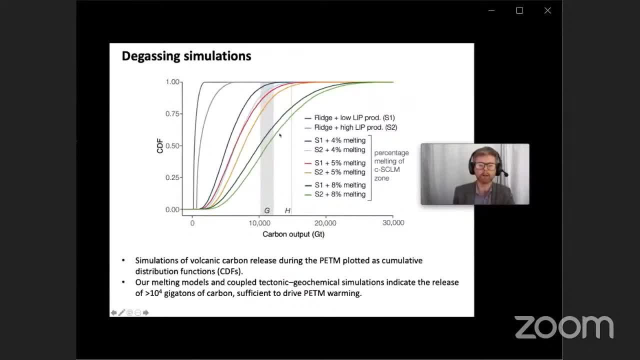 using coupled tectonic geochemical models, models, models. we show that this process is melting. we show that this process is melting. we show that this process is melting can. can drive over 10 000 gigatons of. can can drive over 10 000 gigatons of. 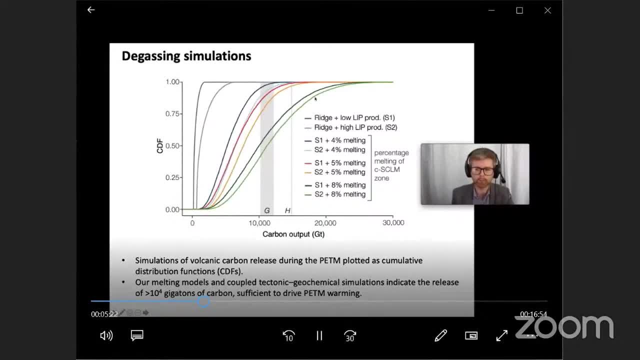 can, can drive over 10 000 gigatons of carbon, carbon, carbon being released which is sufficient to being released, which is sufficient to being released, which is sufficient to promote ptm warming, promote ptm warming, promote ptm warming. we propose to enhance melting of the. 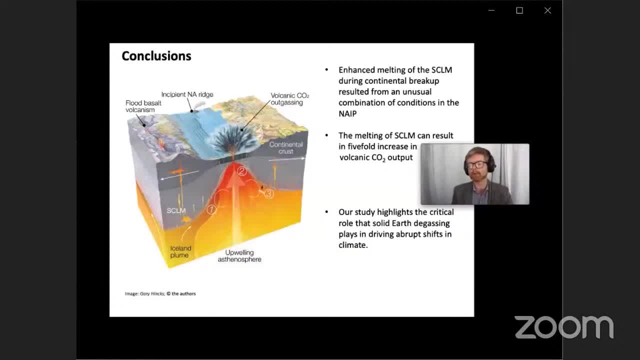 we propose to enhance melting of the. we propose to enhance melting of the cretonic lithosphere during stretching. cretonic lithosphere during stretching. cretonic lithosphere during stretching causes a five-fold increase. causes a five-fold increase. causes a five-fold increase in volcanic carbon release, driving the. 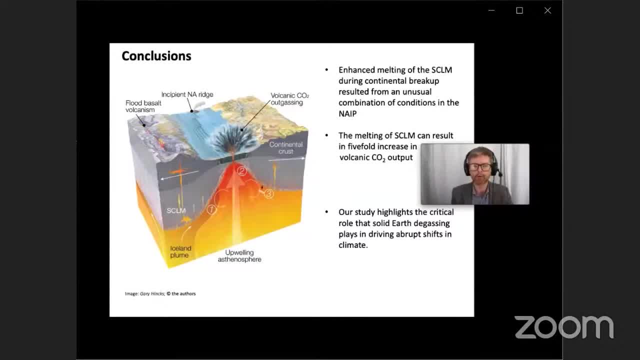 in volcanic carbon release: driving the in volcanic carbon release, driving the ptm and reconciling ptm and reconciling ptm and reconciling the deficit of carbon from background ridge, the deficit of carbon from background ridge, the deficit of carbon from background ridge and lip magnetism. 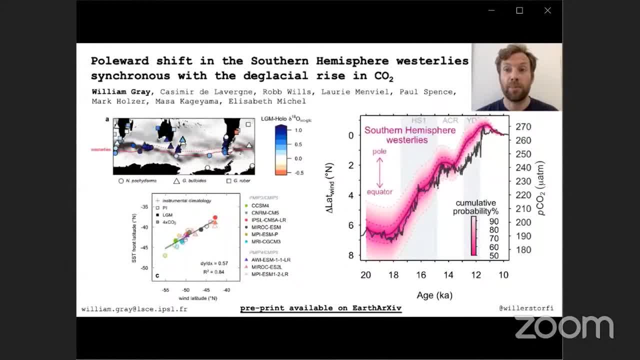 hello the southern hemisphere. westerly hello the southern hemisphere. westerly hello the southern hemisphere. westerly winds have long been hypothesized to winds, have long been hypothesized to winds have long been hypothesized to help regulate atmospheric co2. help regulate atmospheric co2. 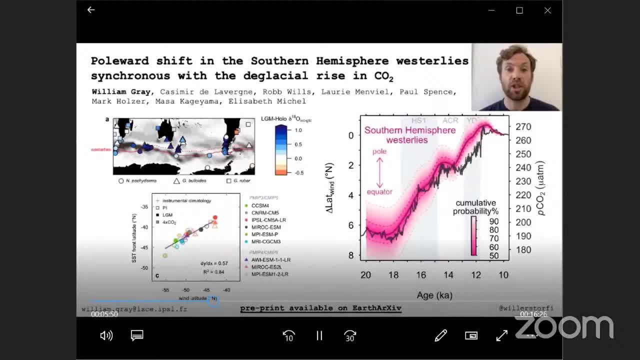 help regulate atmospheric co2 over glacial interglacial cycles, however, over glacial interglacial cycles, however, over glacial interglacial cycles, however, constraints on past changes in the constraints on past changes, in the constraints on past changes in the winds are lacking. winds are lacking. 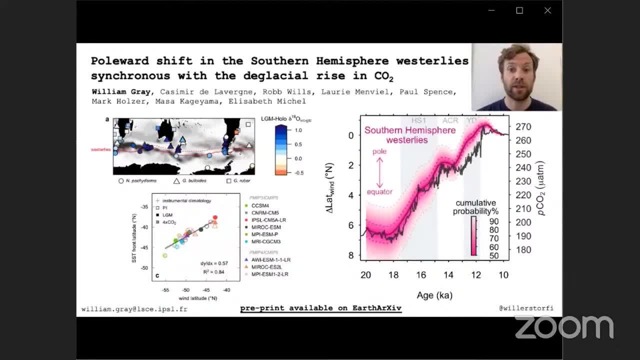 winds are lacking. here we exploit the link between the. here we exploit the link between the. here we exploit the link between the position of the sea surface temperature, position of the sea surface temperature, position of the sea surface temperature front in the southern ocean and the front in the southern ocean and the. 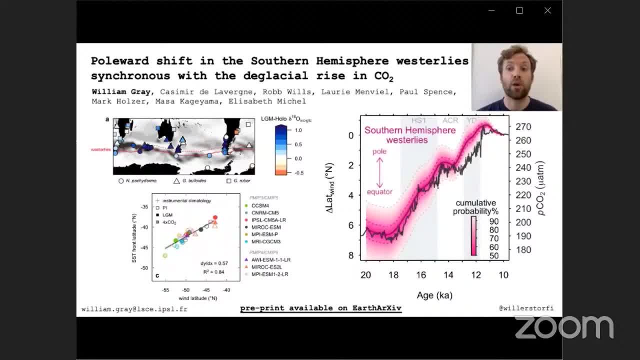 front in the southern ocean and the position of the westerlies. and using a position of the westerlies, and using a position of the westerlies. and using a compilation of planktic: four-miniferal compilation of planktic: four-miniferal compilation of planktic four-miniferal delta-18-0: an ensemble of climate models. 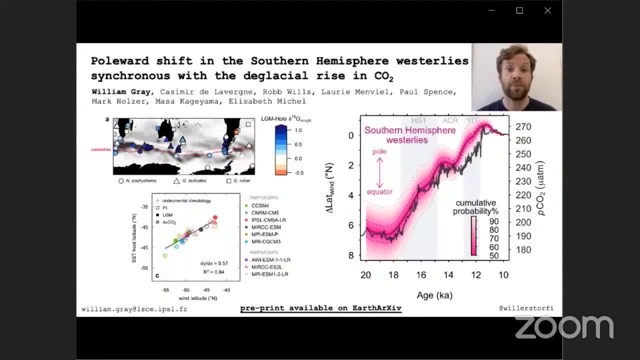 delta-18-0, an ensemble of climate models. delta-18-0, an ensemble of climate models. we reconstruct shifts in the winds over. we reconstruct shifts in the winds over. we reconstruct shifts in the winds over the last deglaciation, the last deglaciation. 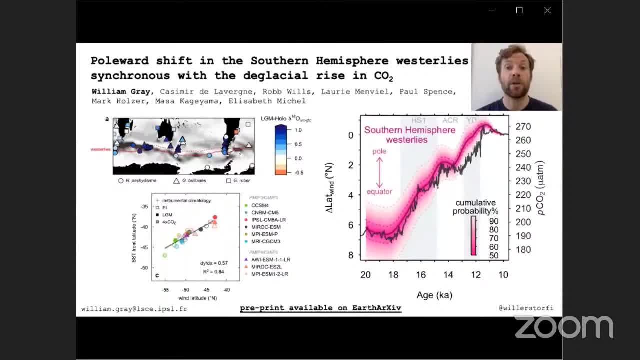 the last deglaciation. we find the westerly winds were five. we find the westerly winds were five. we find the westerly winds were five degrees equator with during the lgm degrees, equator with during the lgm degrees, equator with during the lgm compared to the mid-holocene, and about 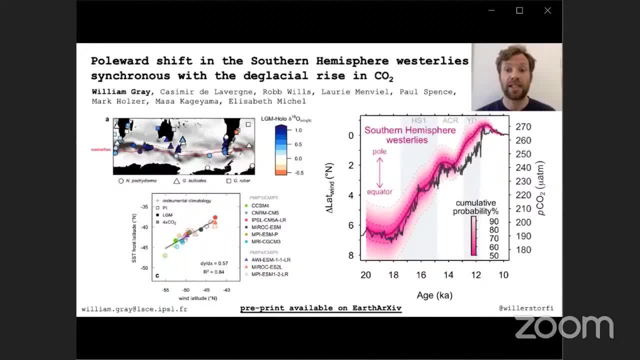 compared to the mid-holocene and about compared to the mid-holocene and about 25 weaker. we show the pole would shift 25 weaker. we show the pole would shift 25 weaker. we show the pole would shift in the westerly winds over deglaciation. 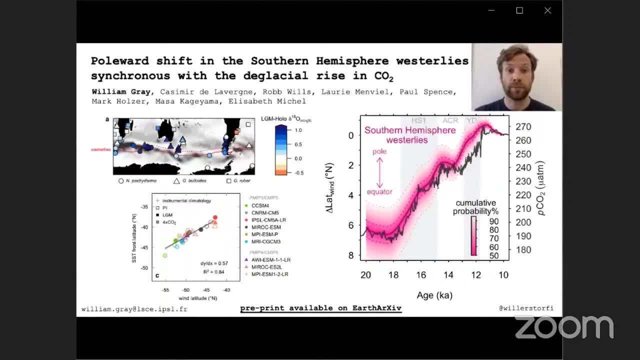 in the westerly winds over deglaciation. in the westerly winds over deglaciation: closely mirrors the rise in atmospheric. closely mirrors the rise in atmospheric. closely mirrors the rise in atmospheric co2- co2- co2 using a quarter degree resolution. ocean. using a quarter degree resolution ocean. 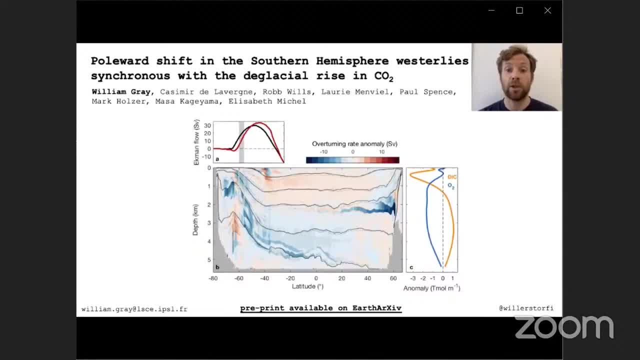 using a quarter degree resolution ocean carbon cycle model. we show that shifting carbon cycle model. we show that shifting carbon cycle model. we show that shifting the westerly's equator wood slows the. the westerly's equator wood slows the. the westerly's equator wood slows the circulation of the abyssal ocean. 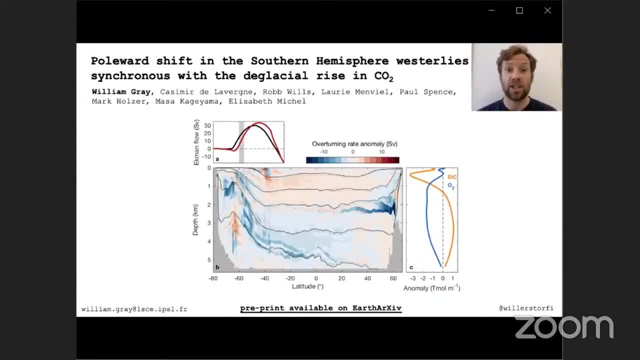 circulation of the abyssal ocean. circulation of the abyssal ocean increasing oceanic carbon storage. our increasing oceanic carbon storage. our finding suggests a central role for. the finding suggests a central role for. the finding suggests a central role for the westerlies in driving the deglacial rise. 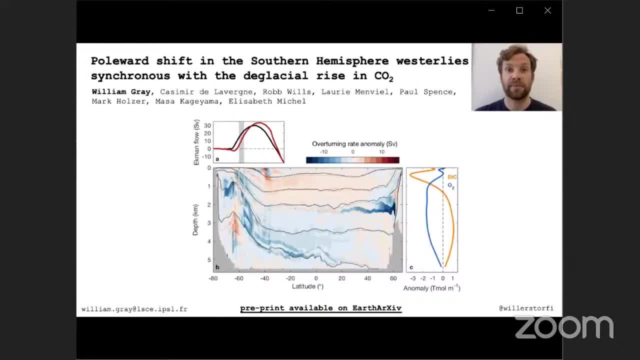 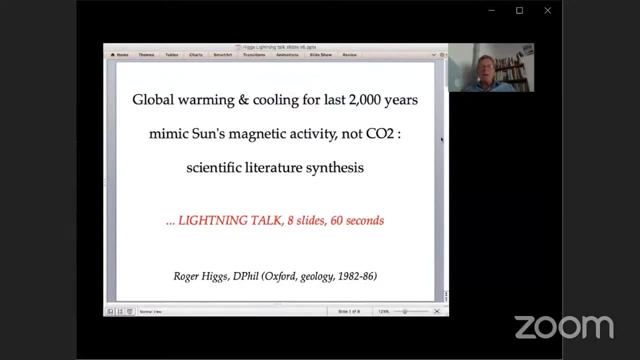 westerlies in driving the deglacial rise. westerlies in driving the deglacial rise in co2. ipcc says the sun plays almost no role. ipcc says the sun plays almost no role. ipcc says the sun plays almost no role in climate change. 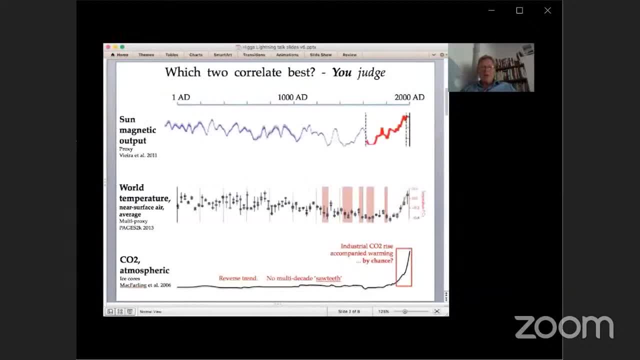 in climate change. in climate change, let's see if we agree. let's see if we agree, let's see if we agree, which two curves correlate best. which two curves correlate best? which two curves correlate best? yes, the first two: the sun's magnetic. yes, the first two: the sun's magnetic. 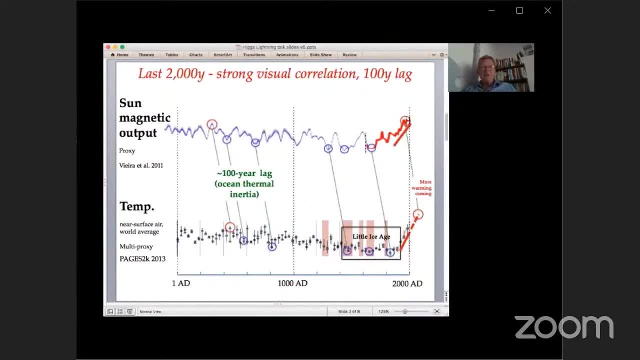 yes, the first two: the sun's magnetic output and global temperature strongly output and global temperature strongly output and global temperature strongly correlate visually for the last two. correlate visually for the last two. correlate visually for the last two thousand years with a 100 year, thousand years with a 100 year. 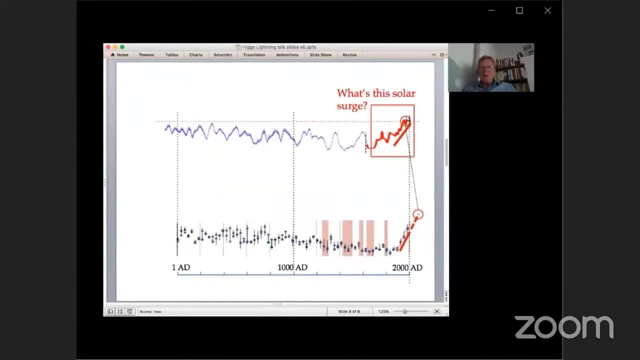 thousand years with a 100 year temperature lag, temperature lag, temperature lag. and what's this solar surge from 1700? and what's this solar surge from 1700? and what's this solar surge from 1700? ad ad ad. it's the largest rise and the strongest. 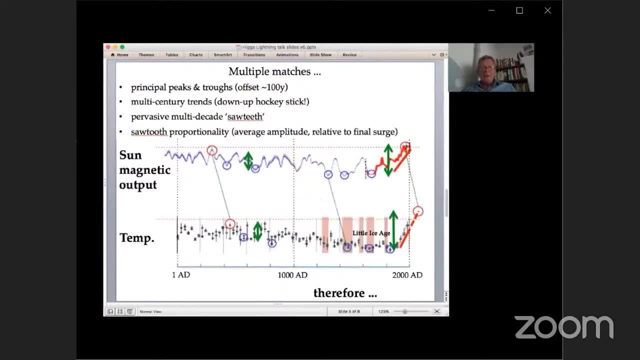 it's the largest rise and the strongest. it's the largest rise and the strongest. grand maximum in more than 10 000 years. grand maximum in more than 10 000 years. grand maximum in more than 10 000 years. look at the multiple matches between the. 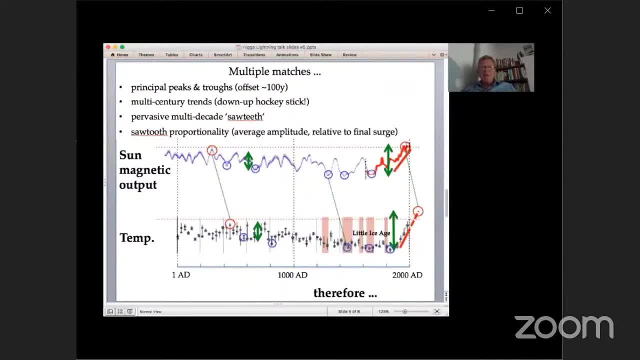 look at the multiple matches between the. look at the multiple matches between the sun's magnetic output and global sun's magnetic output, and global sun's magnetic output and global temperature since two thousand years ago. temperature since two thousand years ago. temperature since two thousand years ago. i conclude that the sun's modern magnetic 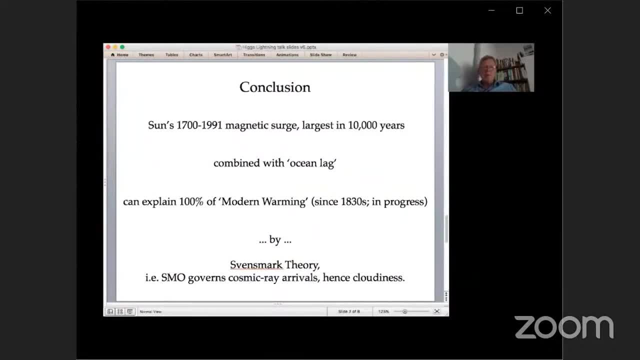 temperature since two thousand years ago. i conclude that the sun's modern magnetic temperature since two thousand years ago. i conclude that the sun's modern magnetic surge, surge, surge combined with ocean lag can explain 100. combined with ocean lag can explain 100. combined with ocean lag can explain 100 percent. 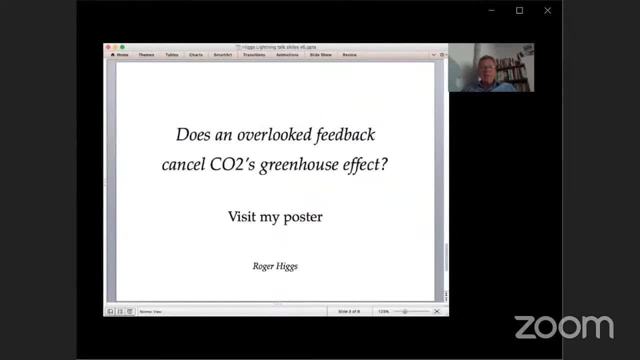 percent. percent of modern warming by sven's mark's theory of modern warming by sven's mark's theory of modern warming by sven's mark's theory. has an overlooked feedback cancelled co2's. has an overlooked feedback canceled co2's. has an overlooked feedback: canceled co2's greenhouse effect. 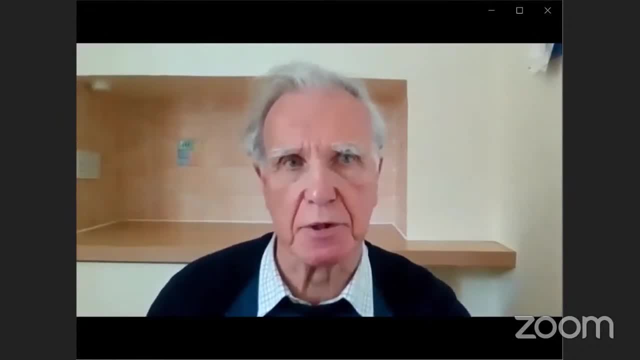 greenhouse effect. greenhouse effect: the polar ice cores show cyclical the polar ice cores show cyclical the polar ice cores show cyclical temperature changes dominated by the temperature changes, dominated by the temperature changes dominated by the earth's, earth's, earth's three orbital cycles, three orbital cycles. 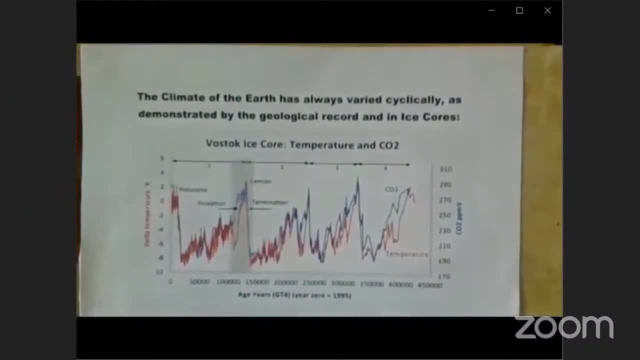 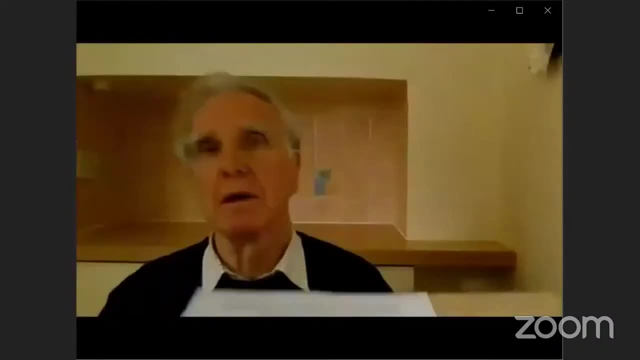 three orbital cycles: the carbon dioxide cycles, the carbon dioxide cycles. the carbon dioxide cycles show a lag behind temperatures. show a lag behind temperatures. show a lag behind temperatures, particularly in the cooling phase, particularly in the cooling phase, particularly in the cooling phase. the influence of seven solar cycles has 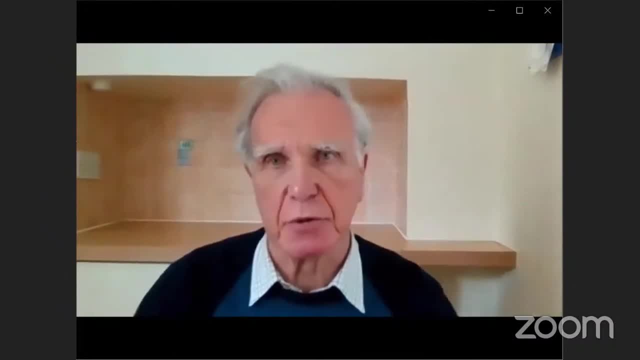 the influence of seven solar cycles has. the influence of seven solar cycles has long been recognized by scientists. long been recognized by scientists. long been recognized by scientists. the seven major ones were also identified. the seven major ones were also identified. the seven major ones were also identified on a 700. 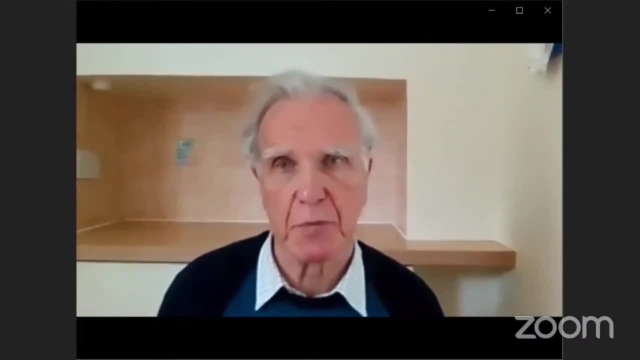 on a 700 on a 700 thousand year long section of piercing. thousand year long section of piercing. thousand year long section of piercing. sediments in lake messel. sediments in lake messel. sediments in lake messel: a synthesis of these seven cycles. a synthesis of these seven cycles. 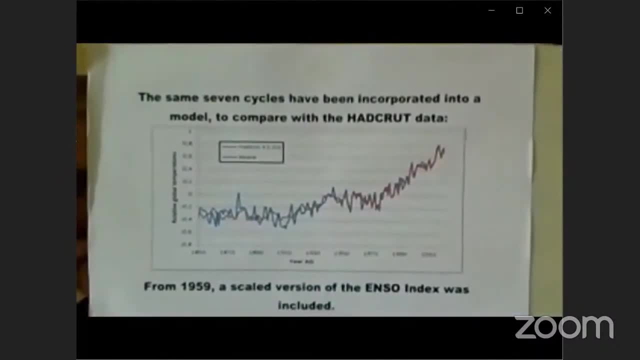 a synthesis of these seven cycles. shows a close correlation with the. shows a close correlation with the shows a close correlation with the measured values: measured values, measured values. it is clear, therefore, that global. it is clear, therefore, that global. it is clear, therefore, that global temperature changes can be related to 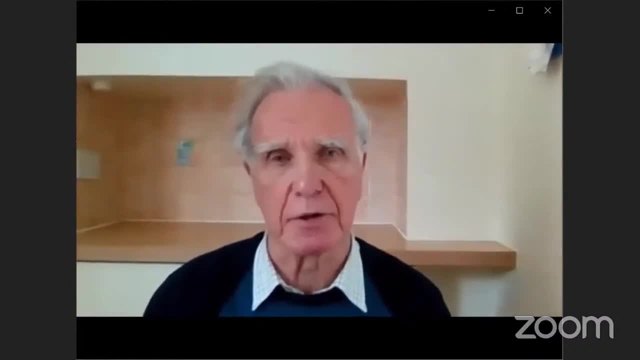 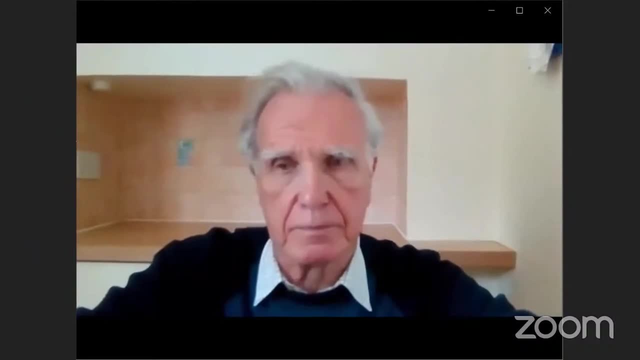 temperature changes can be related to. temperature changes can be related to persistent changes in energy arriving. persistent changes in energy arriving. persistent changes in energy arriving from the sun, from the sun, from the sun, and the carbon dioxide has little effect and the carbon dioxide has little effect and the carbon dioxide has little effect on climate. 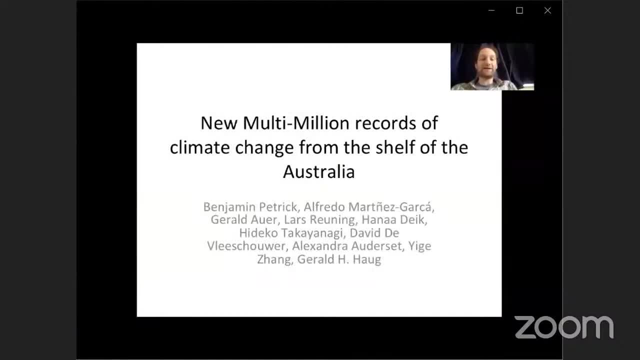 hello, my name is benton petrick. i'm hello, my name is benton petrick. i'm hello, my name is benton petrick. i'm here, here, here. uh, you see the title of my poster and. uh, you see the title of my poster and. 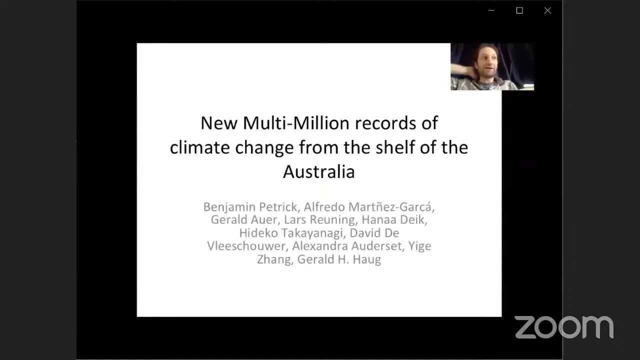 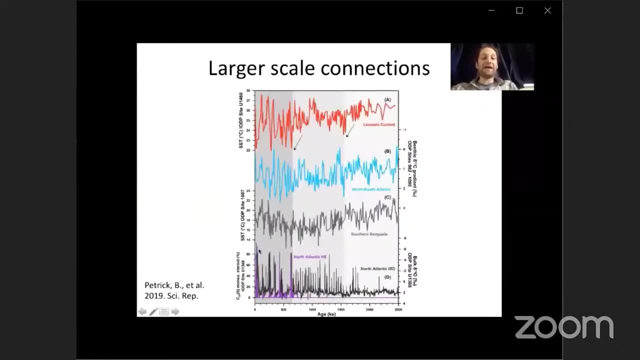 uh, you see the title of my poster and my co-authors, my co-authors, my co-authors: i'm today going to talk to you about new. i'm today going to talk to you about new. i'm today going to talk to you about new technologies. developed is here in red and. 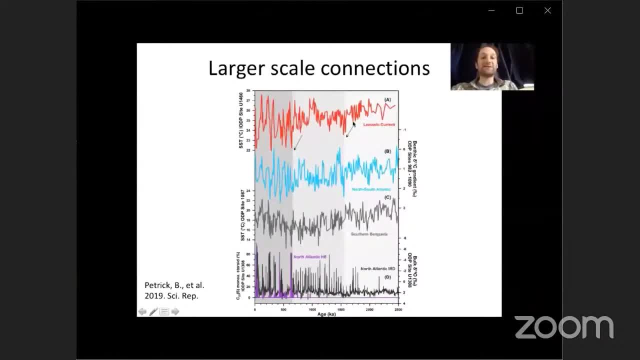 technologies developed is here in red and technologies developed is here in red and i'll talk more to you if you come to my. i'll talk more to you if you come to my. i'll talk more to you if you come to my poster about projection. but essentially, 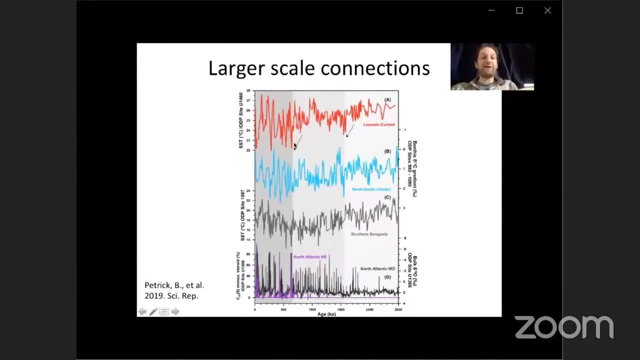 poster about projection, but essentially poster about projection, but essentially we found one cooling around 1.6 million. we found one cooling around 1.6 million. we found one cooling around 1.6 million years and one cooling at 600 000 years years and one cooling at 600 000 years. 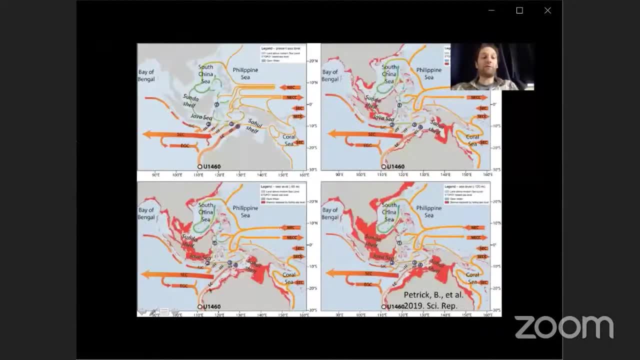 years and one cooling at 600 000 years. we think these coolings are a result of. we think these coolings are a result of. we think these coolings are a result of uh changes in, uh changes in, uh changes in wire level due to sea level changes in. 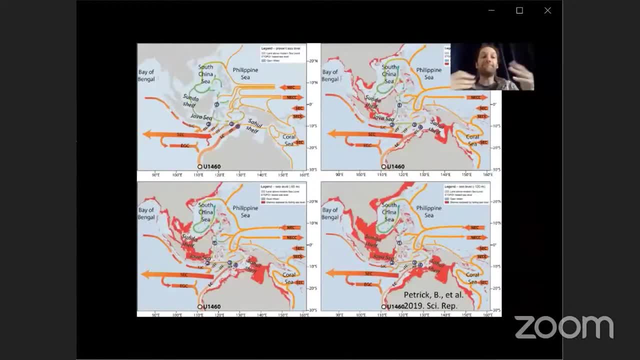 wire level due to sea level changes in wire level due to sea level changes in the indonesian through flow and that the indonesian through flow and that the indonesian through flow, and that these changes had impacts on circulate. these changes had impacts on circulate. 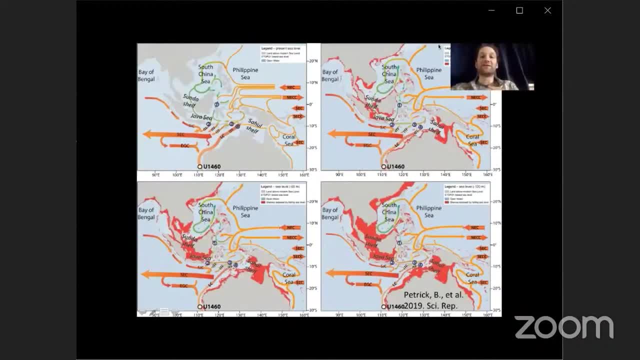 these changes had impacts on circulate, on the climate, the local area and global. on the climate, the local area and global. on the climate, the local area and global circulation. so come to my poster and circulation. so come to my poster and circulation. so come to my poster and i'll say: hello, i'm brian katt, as a 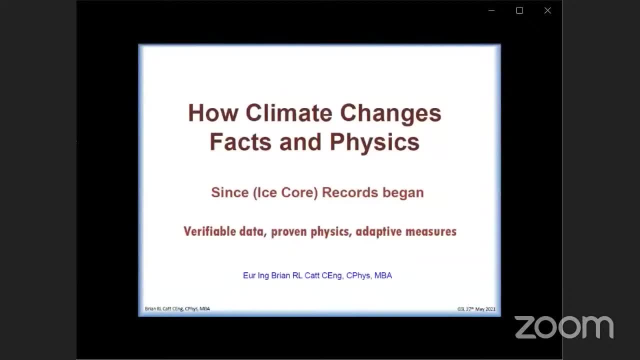 i'll say hello, i'm brian katt as a. i'll say hello, i'm brian katt, as a practical physicist. my approach practical physicist, my approach practical physicist. my approach contrasts the observable physics of contrasts, the observable physics of contrasts the observable physics of climate, with the predictions of models. 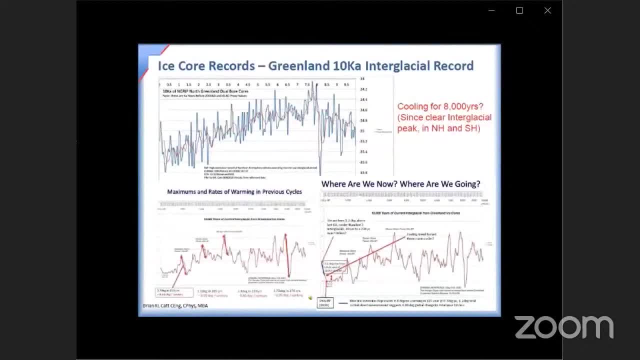 climate with the predictions of models. climate with the predictions of models in three ways. climate with the predictions of models in three ways. climate with the predictions of models in three ways. climate is very stable, strongly. climate is very stable, strongly. climate is very stable, strongly controlled within a narrow range by 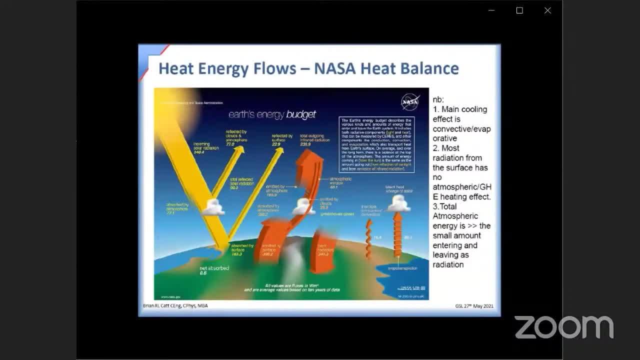 controlled within a narrow range by: controlled within a narrow range by: evaporative and cloud albedo. response to evaporative and cloud albedo. response to evaporative and cloud albedo. response to ocean warming: with no catastrophic ocean warming. with no catastrophic ocean warming. with no catastrophic tipping points. 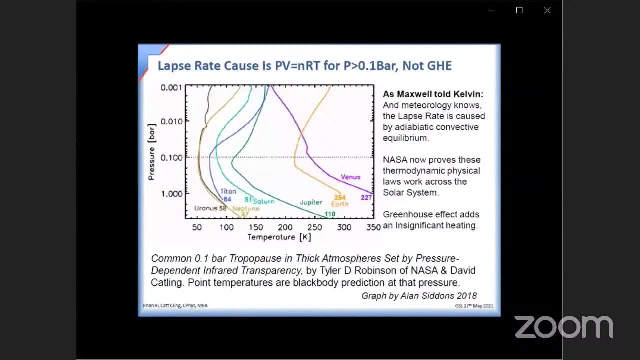 tipping points. tipping points: the atmospheric lapse rate, hence surface. the atmospheric lapse rate, hence surface. the atmospheric lapse rate, hence surface. temperature is primarily controlled by temperature, is primarily controlled by temperature is primarily controlled by solar surface heating. plus solar surface heating, plus solar surface heating, plus gravitational pressure in maxwell's. 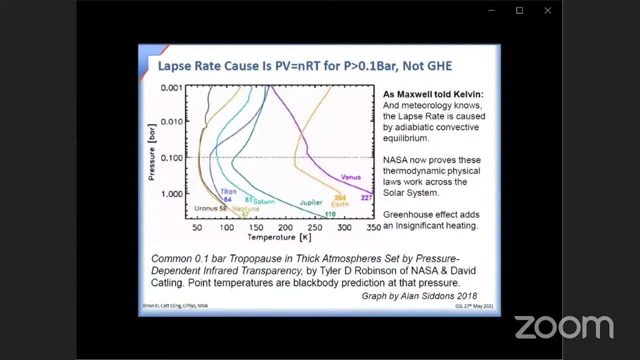 gravitational pressure in maxwell's gravitational pressure in maxwell's convective equilibrium. convective equilibrium, convective equilibrium. the radiative greenhouse effect on this. the radiative greenhouse effect on this. the radiative greenhouse effect on this, but co2 is not significant within it. the 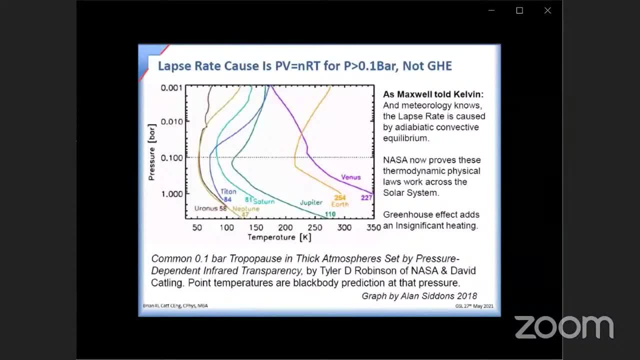 but co2 is not significant within it. the but co2 is not significant within it. the sun heats, the oceans control the cycles. sun heats, the oceans control the cycles. sun heats, the oceans control the cycles. repeat, repeat, repeat. civilization is hugely successful in. civilization is hugely successful in. 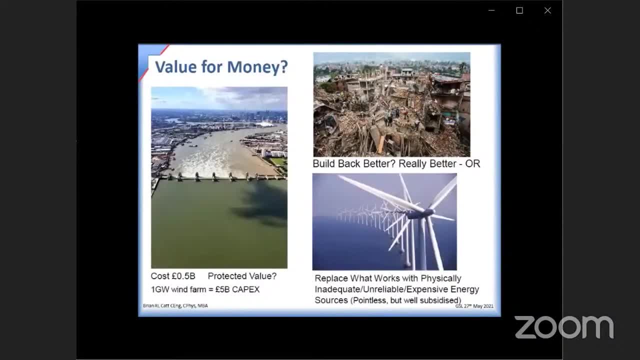 civilization is hugely successful in using its economic progress to protect, using its economic progress to protect, using its economic progress to protect itself against nature itself, against nature itself, against nature. but the un plan to restrict western energy, but the un plan to restrict western energy, but the un plan to restrict western energy use. hence progress. they employ models. 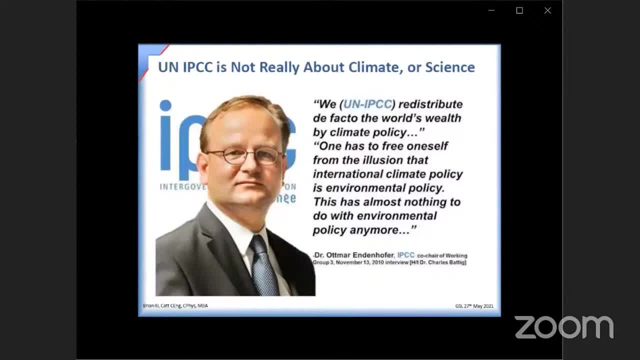 use, hence progress. they employ models, use, hence progress. they employ models that attribute natural change to co2, that attribute natural change to co2, that attribute natural change to co2, then predict on this presumption, as if, then predict on this presumption, as if. then predict on this presumption as if proven. 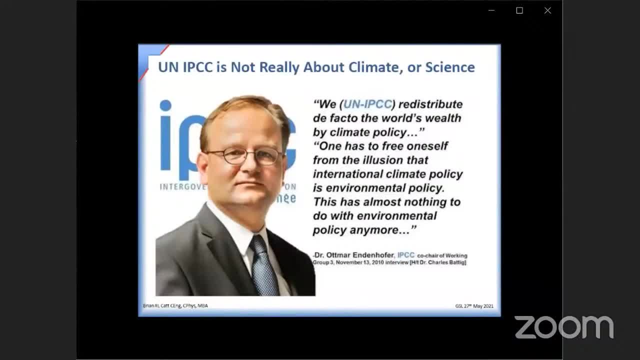 proven proven direct and proxy observations since 2000. direct and proxy observations since 2000. direct and proxy observations since 2000 have serially disproven this causal, have serially disproven this causal, have serially disproven this causal relationship, relationship relationship. so i suggest truly scientific bodies. 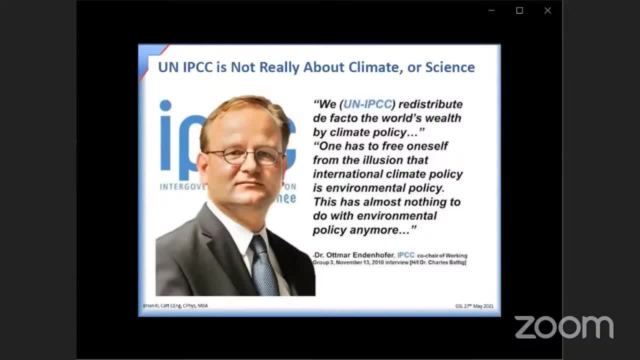 so i suggest truly scientific bodies. so i suggest truly scientific bodies should prepare the evidence of nature, should prepare the evidence of nature, should prepare the evidence of nature to the presumptions and models in this, to the presumptions and models in this, to the presumptions and models in this matter. 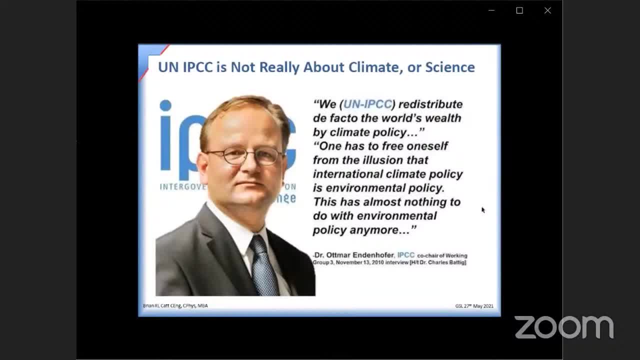 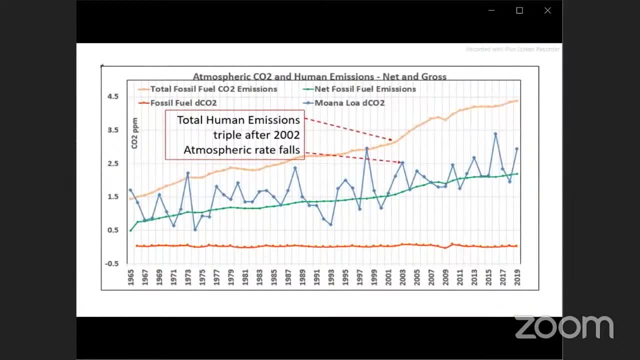 matter matter. thank you, how do you host i present observations? how do you host i present observations? how do you host i present observations that contradict the basic tenors, that contradict the basic tenors, that contradict the basic tenors, the agw conjecture, and will explain why. 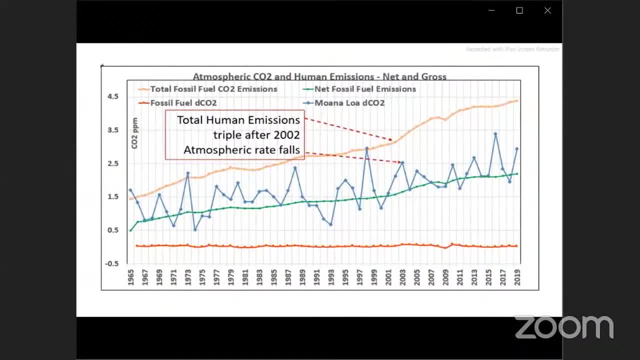 the agw conjecture and will explain why the agw conjecture and will explain why human emissions do not drive climate. human emissions do not drive climate. human emissions do not drive climate change, change, change. the increase in atmospheric co2 of 94. the increase in atmospheric co2 of 94. 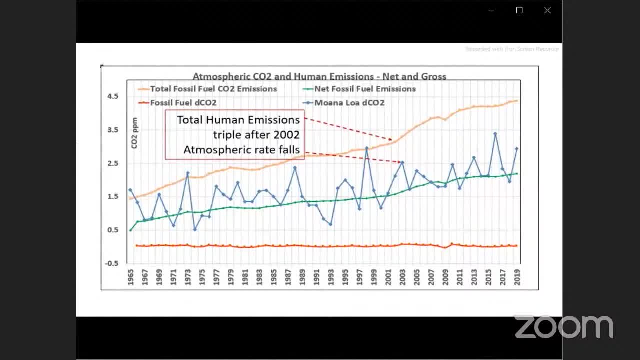 the increase in atmospheric co2 of 94 parts per million since 1965 is only parts per million since 1965 is only parts per million since 1965 is only partly due to the 185 parts per million. partly due to the 185 parts per million. 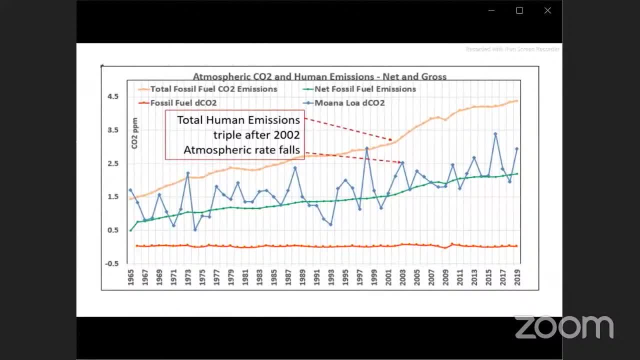 partly due to the 185 parts per million added by humanity, added by humanity, added by humanity. the year-on-year changes in atmospheric, the year-on-year changes in atmospheric, the year-on-year changes in atmospheric co2 are up to two orders of magnitude. co2 are up to two orders of magnitude. 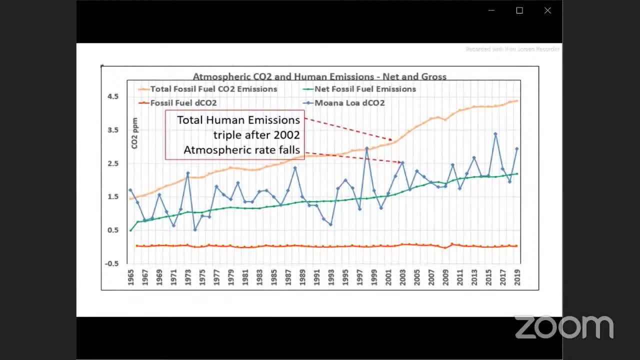 co2 are up to two orders of magnitude, larger than emissions. cutting them will larger than emissions. cutting them will larger than emissions. cutting them will not remove natural variability, not remove natural variability, not remove natural variability. the correlation of global sea surface. the correlation of global sea surface. 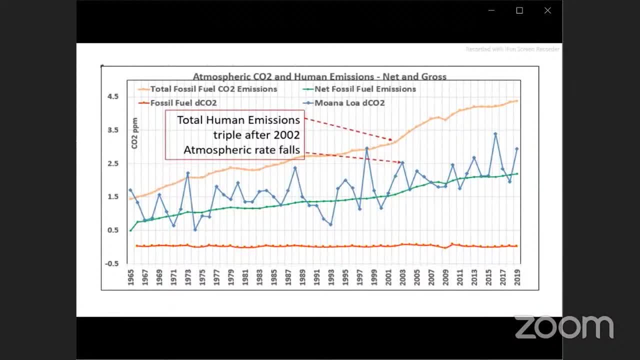 the correlation of global sea surface temperatures and lagged atmospheric co2 temperatures and lagged atmospheric co2 temperatures and lagged atmospheric co2 indicates that global temperatures and indicates that global temperatures. and indicates that global temperatures and not human emissions drive atmospheric. not human emissions drive atmospheric. 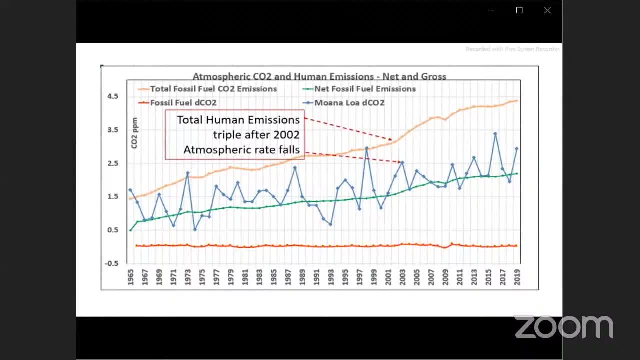 not human emissions drive atmospheric co2. the claim that the global carbon co2, the claim that the global carbon co2, the claim that the global carbon budget was balanced budget was balanced. budget was balanced- balanced before human emissions began. balanced before human emissions began. balanced before human emissions began. it's an unsupported assumption, not a. 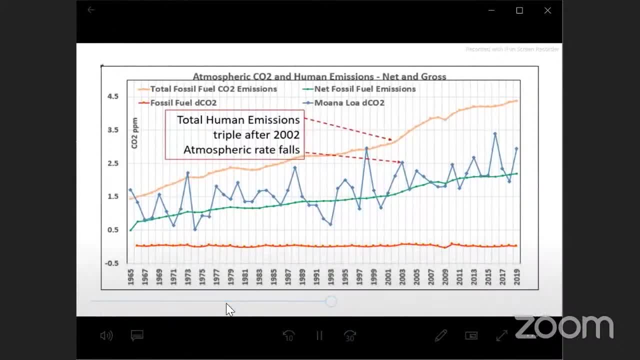 it's an unsupported assumption, not a. it's an unsupported assumption, not a fact. this does not mean that emissions fact. this does not mean that emissions fact. this does not mean that emissions have no effect, but it does mean that have no effect. but it does mean that. 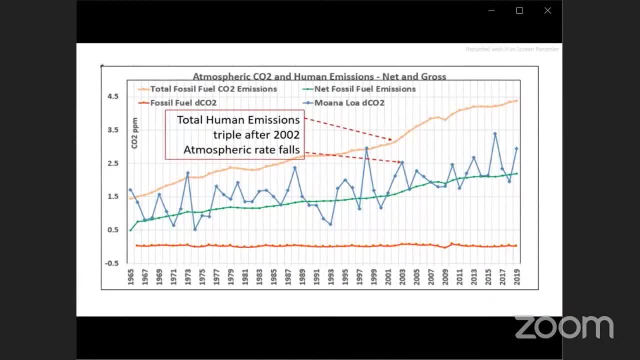 have no effect, but it does mean that they control now the global warming a. they control now the global warming a. they control now the global warming a measurable quantity, not climate change. measurable quantity, not climate change. measurable quantity, not climate change, which has no units, which has no units. 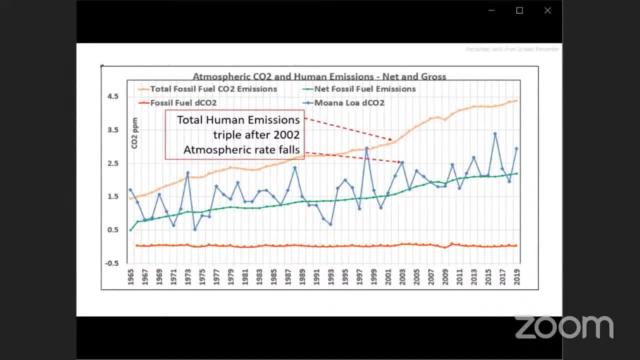 which has no units. both are symptoms of climate change, not both are symptoms of climate change- not both are symptoms of climate change, not causes. a conjecture supported by recent causes. a conjecture supported by recent causes. a conjecture supported by recent lab experiment that found that an 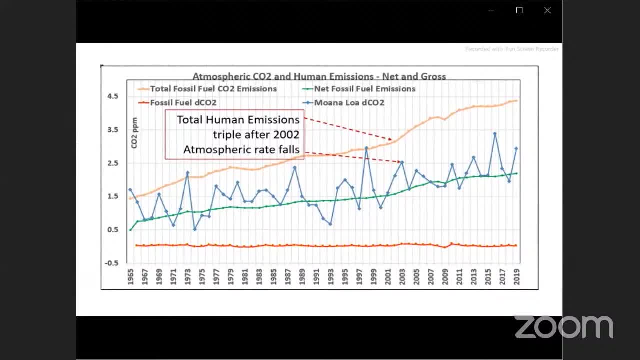 lab experiment that found that. an lab experiment that found that an atmosphere of 100 co2 caused no more atmosphere of 100 co2 caused no more atmosphere of 100 co2 caused no more warming than one with 0.04 percent warming than one with 0.04 percent. 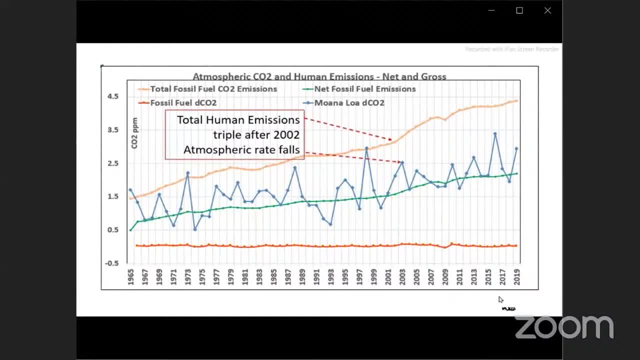 warming than one with 0.04 percent. this experiment will not be the last word, this experiment will not be the last word. this experiment will not be the last word, however, because the science is never, however, because the science is never, however, because the science is never settled. 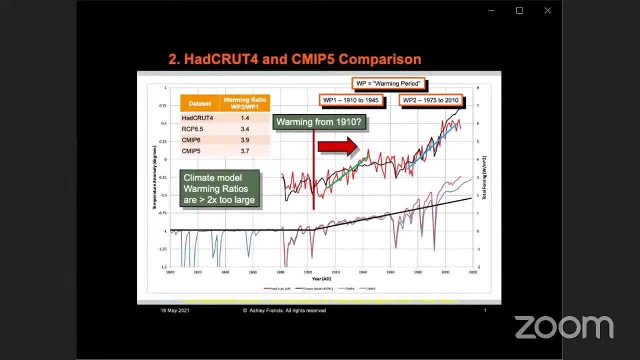 settled, settled. this paper investigates inconsistencies. this paper investigates inconsistencies. this paper investigates inconsistencies post-lia between physical observations, post-lia, between physical observations, post-lia, between physical observations and climate models, and forcings surface and climate models. and forcings surface and climate models. and forcings surface temperatures and models agree warming. 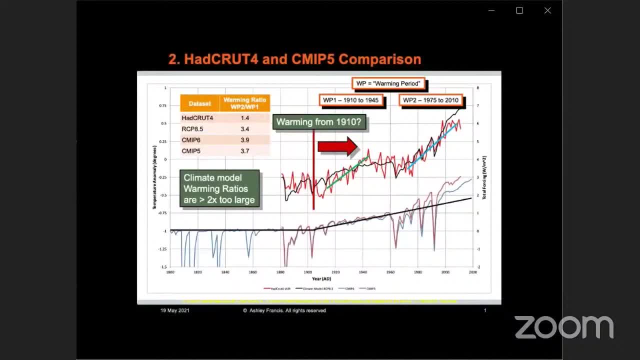 temperatures and models agree. warming temperatures and models agree warming commences around 1910 and that two commences around 1910 and that two commences around 1910, and that two periods of warming are evident early and periods of warming are evident early and. 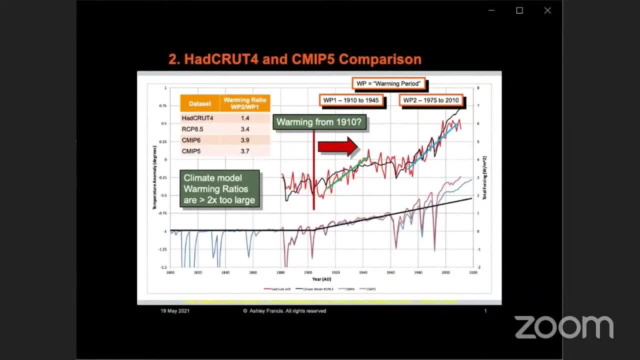 periods of warming are evident early and late 20th century, late 20th century. late 20th century. the observed temperature, glacier and sea. the observed temperature, glacier and sea. the observed temperature, glacier and sea level data agree the ratio of these two. level data agree the ratio of these two. 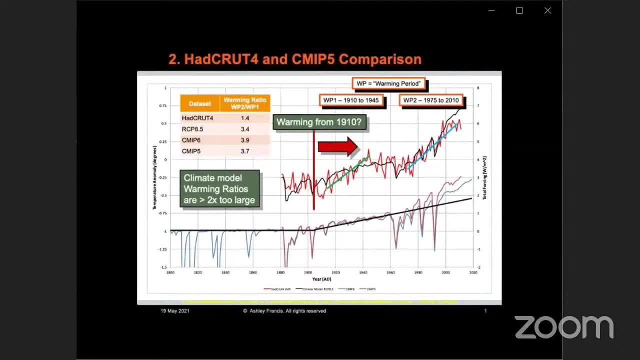 level data agree. the ratio of these two warming rates is about 1.4 times, however. warming rates is about 1.4 times, however. warming rates is about 1.4 times. however. climate model input, forcings and output. climate model, input, forcings and output. 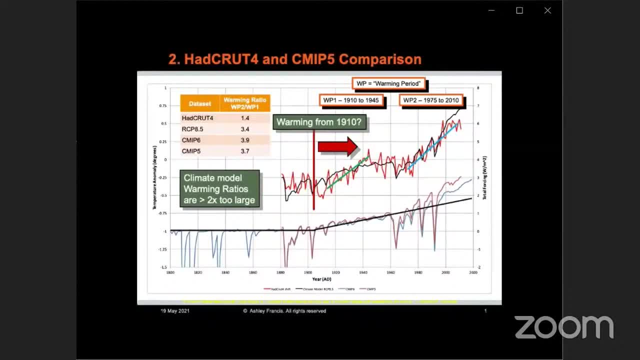 climate model: input forcings and output temperatures have ratios that are more temperatures have ratios that are more temperatures. have ratios that are more than two times larger than two times larger than two times larger. sea level and glacier retreat data show. sea level and glacier retreat data show. 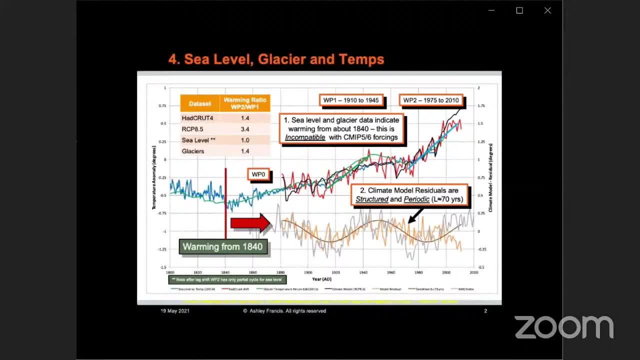 sea level and glacier retreat data show the onset of warming post lai commences. the onset of warming post lai commences. the onset of warming post lai commences much earlier, around 1840, with a third. much earlier, around 1840, with a third. 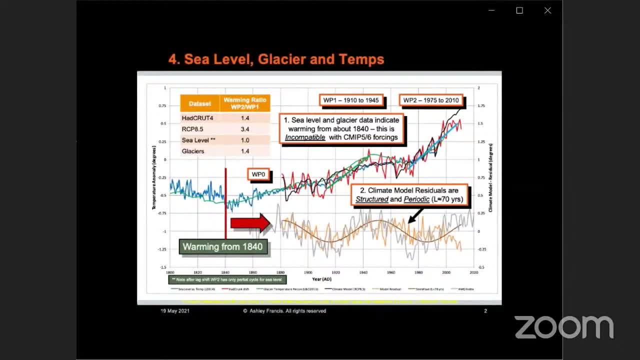 much earlier, around 1840, with a third warming period, evident in the 19th warming period. evident in the 19th warming period, evident in the 19th century. here we also note climate model century. here we also note climate model century. here we also note climate model residuals are structured and periodic. 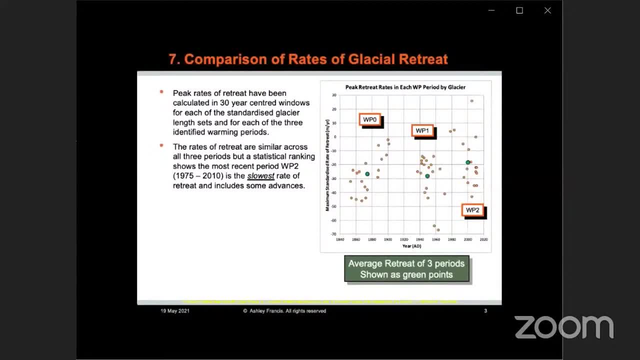 residuals are structured and periodic. residuals are structured and periodic. comparing the three warming periods: we comparing the three warming periods. we comparing the three warming periods, we note the rate of glacier retreat is: note. the rate of glacier retreat is: note. the rate of glacier retreat is similar for all three, with the most. 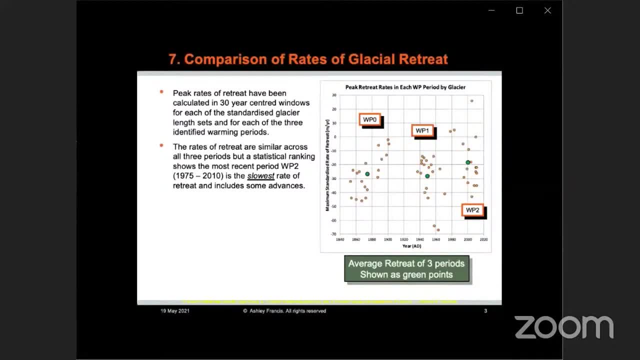 similar for all three, with the most similar for all three, with the most recent warming period statistically. the recent warming period statistically. the recent warming period. statistically. the slowest rate of retreat. slowest rate of retreat, slowest rate of retreat. the geological community should be. the geological community should be. 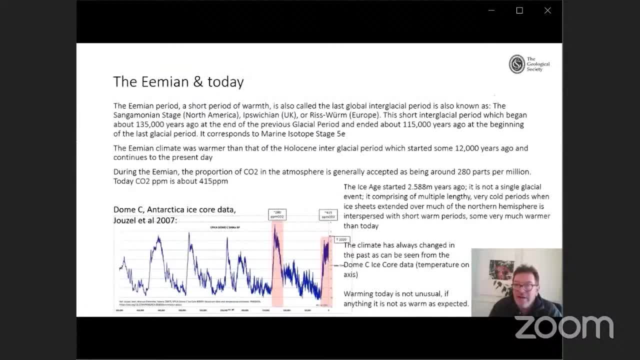 the geological community should be included in the climate debate. included in the climate debate. included in the climate debate. the last interglacial, the ermine, which, the last interglacial, the ermine, which, the last interglacial, the ermine which started 135 000 years ago, was far warmer. 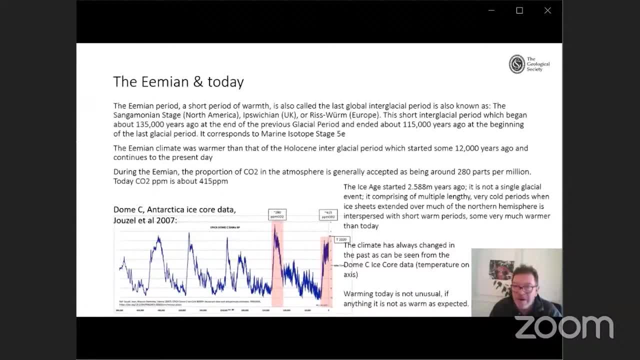 started 135 000 years ago was far warmer. started 135 000 years ago was far warmer than today's. yet co2 parts per million than today's, yet co2 parts per million than today's. yet co2 parts per million were far lower, were far lower. 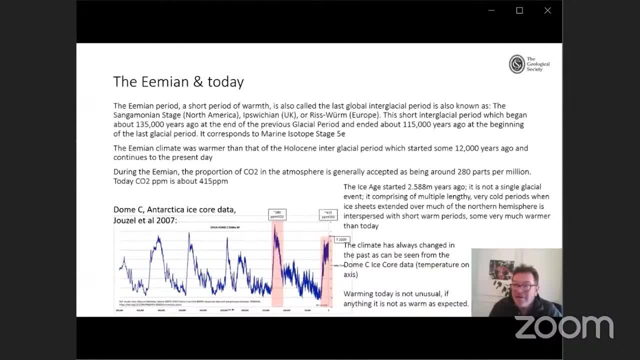 were far lower in the intervening years. ice sheets in the intervening years, ice sheets in the intervening years. ice sheets reached the silly oils. montreal was reached the silly oils. montreal was reached the silly oils. montreal was under three kilometers of ice, it all. under three kilometers of ice, it all. 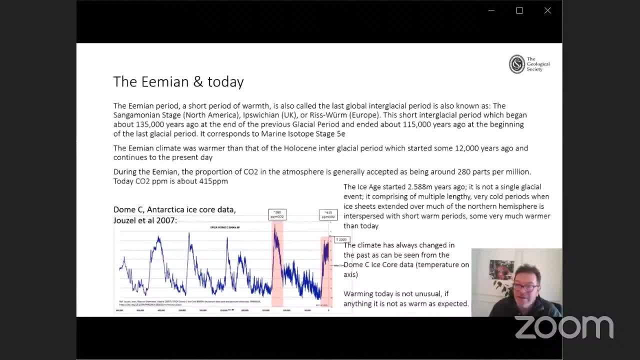 under three kilometers of ice. it all melted at far lower co2 ppm levels than melted at far lower co2 ppm levels than melted at far lower co2 ppm levels than we experienced today. we experienced today. we experienced today. we know it was warmer from ice. core data: 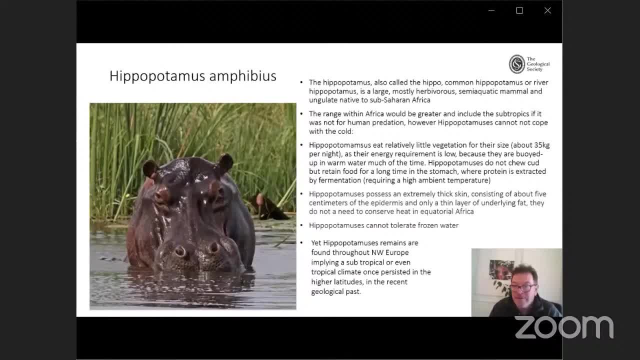 we know it was warmer from ice core data. we know it was warmer from ice core data from floral and faunal records. from floral and faunal records. from floral and faunal records- hippopotamuses, for instance, and other hippopotamuses, for instance, and other. 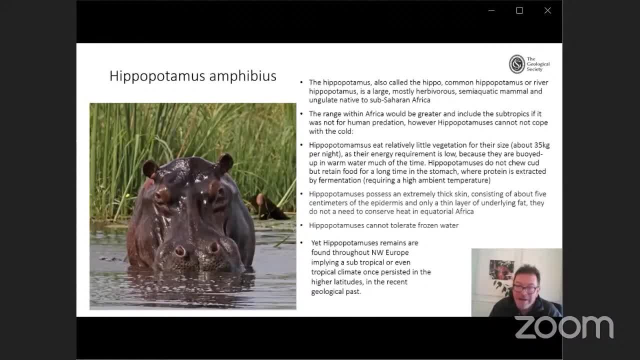 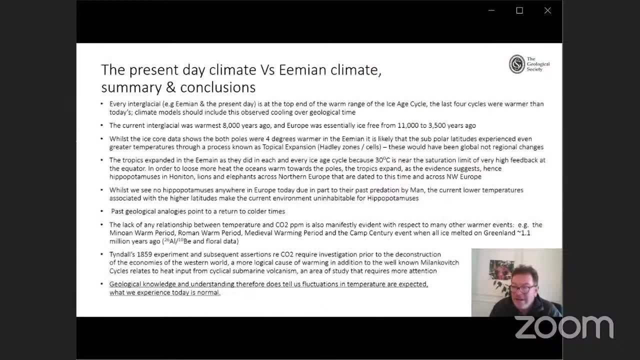 hippopotamuses, for instance, and other tropical and subtropical creatures roam. tropical and subtropical creatures roam. tropical and subtropical creatures roam the higher latitudes, the higher latitudes, the higher latitudes. before taking down western society, before taking down western society, before taking down western society, we need to re-examine tyndall's 1859. 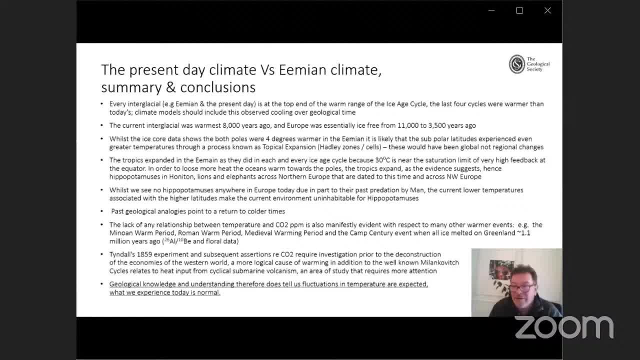 we need to re-examine tyndall's 1859. we need to re-examine tyndall's 1859 experiment and assertions. experiment and assertions. experiment and assertions as the relationship between co2 and as the relationship between co2 and as the relationship between co2 and temperature is logarithmic and not linear. 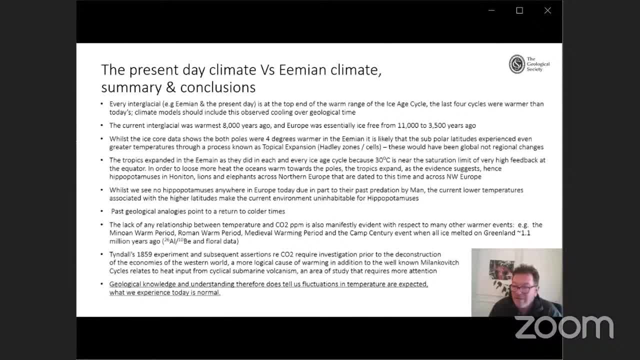 temperature is logarithmic and not linear. temperature is logarithmic and not linear. the modest temperature rise- we are the modest temperature rise. we are the modest temperature rise we are experiencing right now is normal. experiencing right now is normal. experiencing right now is normal. thank you for my minute and yours. 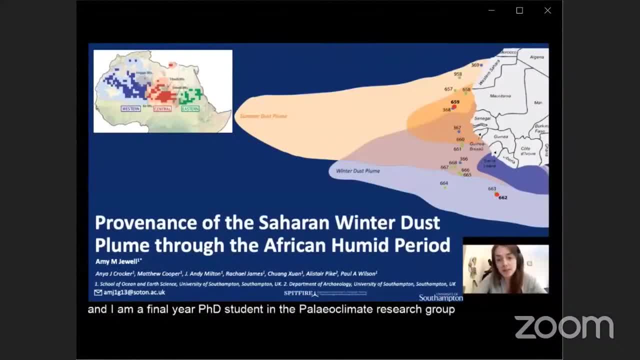 thank you for my minute and yours. thank you for my minute and yours. hi everyone. my name is amy jewel and hi everyone. my name is amy jewel and hi everyone. my name is amy jewel and i'm a final year phd student in the. i'm a final year phd student in the. 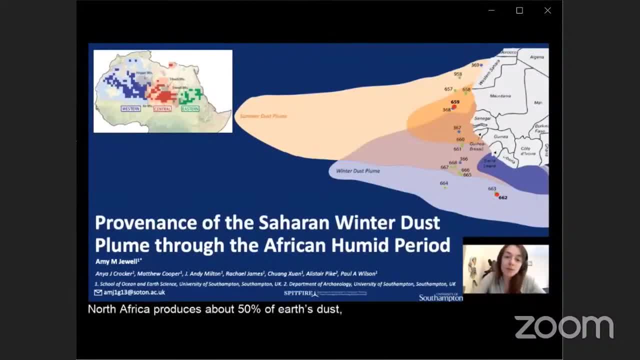 i'm a final year phd student in the paleoclimate research group here at paleoclimate research group. here at paleoclimate research group here at southampton, southampton, southampton. so north africa produces about 50% of, so north africa produces about 50% of. 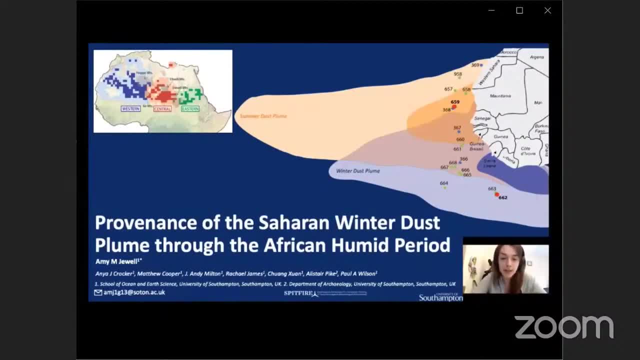 so north africa produces about 50% of earth's dust and this does accumulate earth's dust and this does accumulate earth's dust and this does accumulate in marine sediments in the north, in marine sediments in the north, in marine sediments in the north atlantic, providing us with a continuous 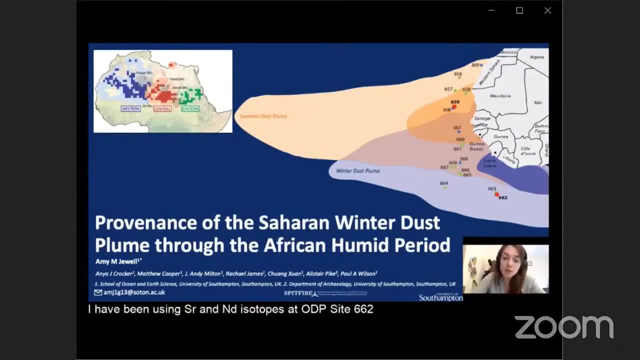 atlantic, providing us with a continuous atlantic, providing us with a continuous archive of continental aridity: archive of continental aridity. archive of continental aridity. i've been using strontium and neodymium. i've been using strontium and neodymium. 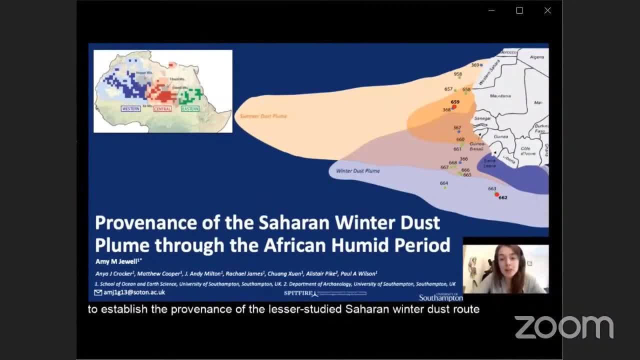 i've been using: strontium and neodymium isotopes at odp site 662. isotopes at odp site 662. isotopes at odp site 662 to establish the provenance of the lesser. to establish the provenance of the lesser. to establish the provenance of the lesser: studied winter dust route and how this. 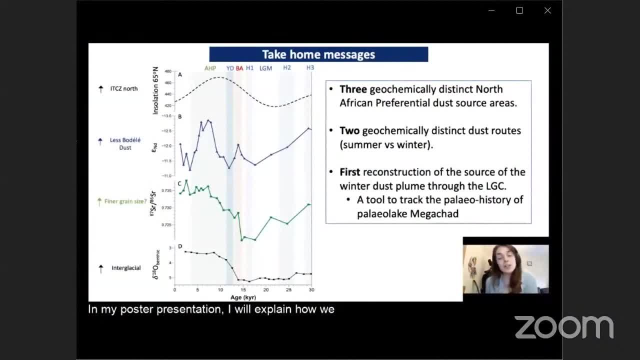 studied winter dust route and how this studied winter dust route and how this has changed through the quaternary, has changed through the quaternary, has changed through the quaternary. so in my post presentation, i will so in my post presentation i will so in my post presentation i will explain how we, geochemically, 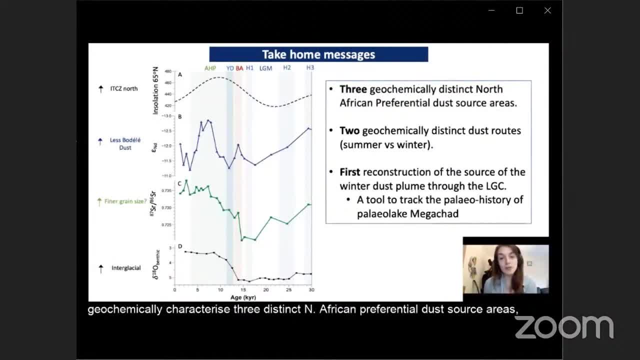 explain how we geochemically explain how we geochemically characterize three distinct north, characterize three distinct north, characterize three distinct north. african preferential dust source areas. african preferential dust source areas. african preferential dust source areas. and then we use this to establish that and then we use this to establish that. 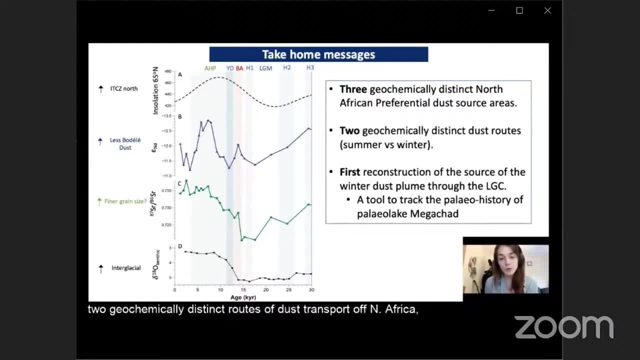 and then we use this to establish that there are two geochemically distinct. there are two geochemically distinct. there are two geochemically distinct routes of dust transport off north. routes of dust transport off north. routes of dust transport off north africa, enabling us to study regional. 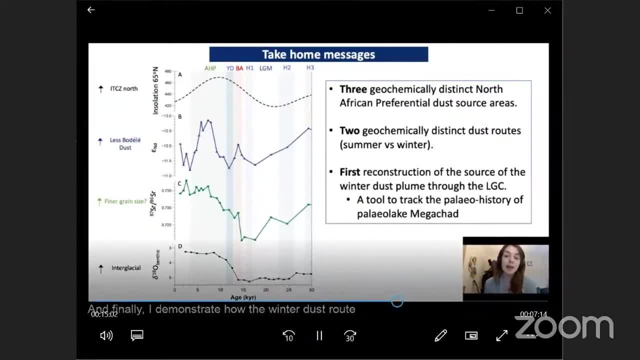 africa, enabling us to study regional africa, enabling us to study regional climate change, climate change, climate change. and then, finally, i demonstrate how the and then, finally, i demonstrate how the and then, finally, i demonstrate how the winter dust route can be used to track. winter dust route can be used to track. 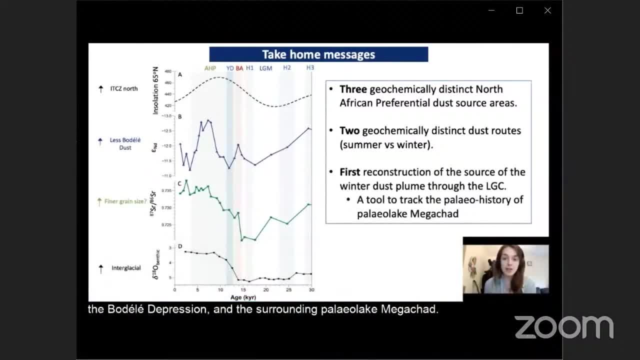 winter dust route can be used to track the paleo history of the dustiest place. the paleo history of the dustiest place, the paleo history of the dustiest place on earth, the bedelia depression and the on earth. the bedelia depression and the. 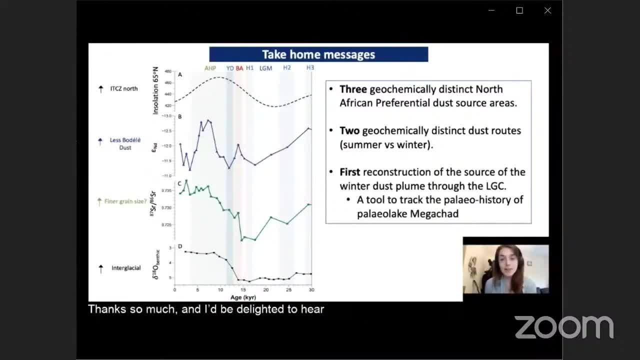 on earth: the bedelia depression and the surrounding paleo lake megachat. thanks. surrounding paleo lake megachat. thanks. surrounding paleo lake megachat. thanks so much and i'd be delighted to hear so much. and i'd be delighted to hear so much and i'd be delighted to hear any comments or questions in the poster. 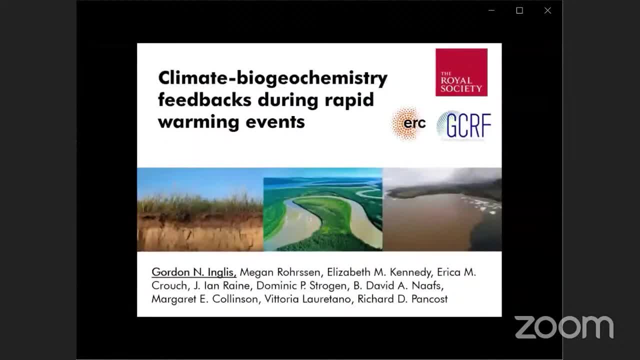 any comments or questions in the poster. any comments or questions in the poster session session session. hi everyone, my name is gordon ingalls. hi everyone, my name is gordon ingalls. hi everyone, my name is gordon ingalls, from the university of southampton i. 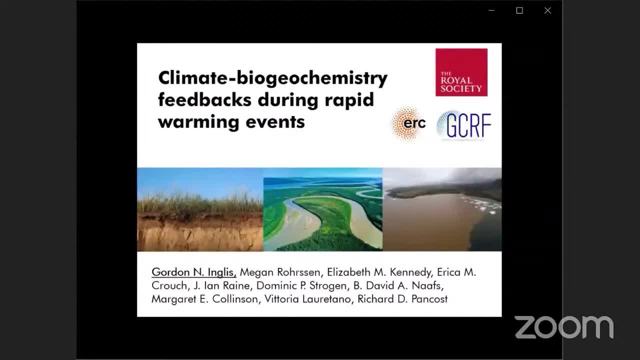 from the university of southampton. i from the university of southampton i will be presenting, will be presenting, will be presenting a recent study looking at the operation, a recent study looking at the operation, a recent study looking at the operation of the terrestrial methane cycle, of the terrestrial methane cycle. 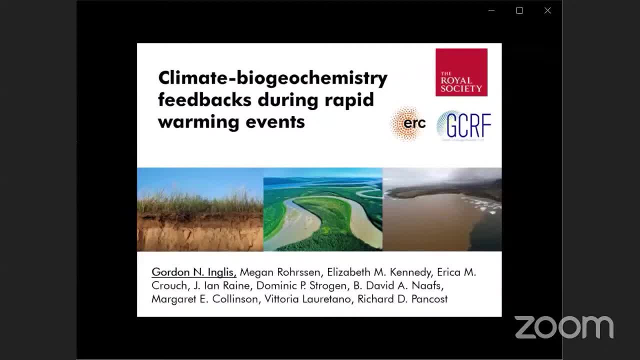 of the terrestrial methane cycle during the paleocene eocene thermal. during the paleocene eocene thermal during the paleocene eocene thermal: maximum maximum maximum 56 million years ago. in this study, we 56 million years ago. in this study, we 56 million years ago. in this study, we use a novel biomarker based approach. 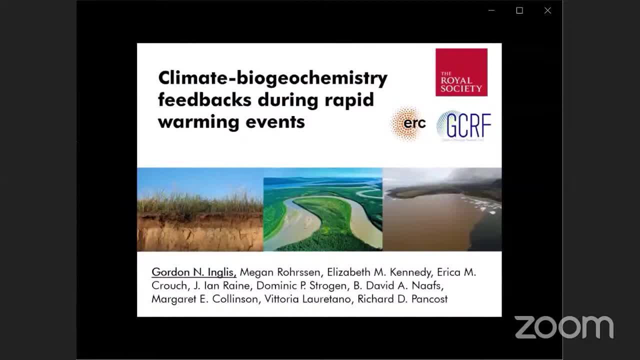 use a novel biomarker based approach. use a novel biomarker based approach to reconstruct methane cycling within a. to reconstruct methane cycling within a. to reconstruct methane cycling within a high latitude wetland- high latitude wetland. high latitude wetland. we show that the methane cycle was. 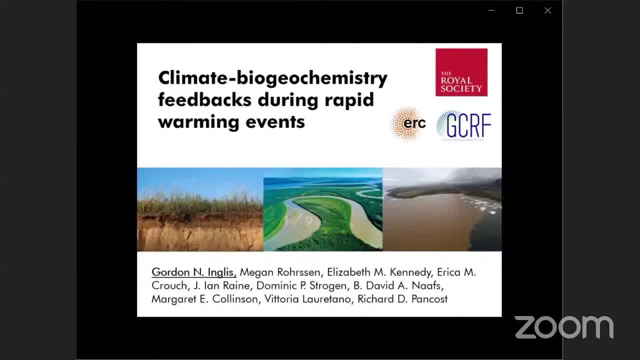 we show that the methane cycle was. we show that the methane cycle was intensified relative to the modern, intensified relative to the modern, intensified relative to the modern. and for the first time, we show that the and for the first time, we show that the and for the first time, we show that the onset of rapid warming during the ptm is. 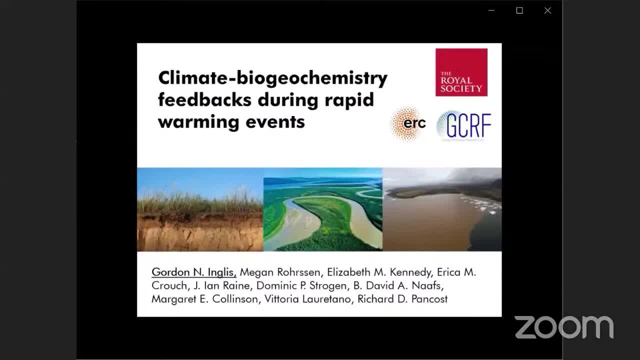 onset of rapid warming during the ptm is. onset of rapid warming during the ptm is particularly crucial, particularly crucial, particularly crucial for modifying wetland biogeochemical. for modifying wetland biogeochemical. for modifying wetland biogeochemical feedbacks, feedbacks. 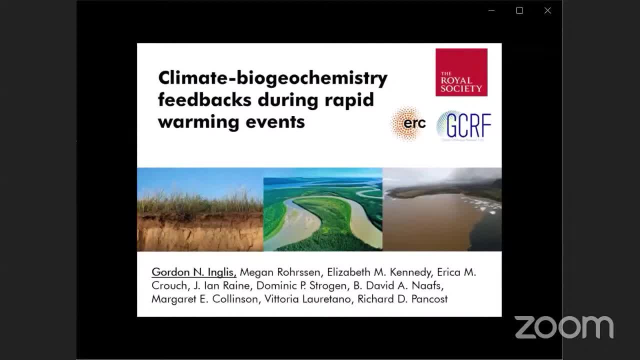 feedbacks in earth's history. so if you want to in earth's history, so if you want to in earth's history, so if you want to find out more, find out more, find out more, you can come find me in the poster. you can come find me in the poster. 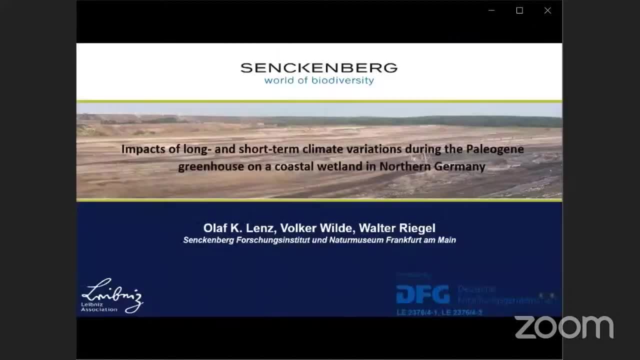 you can come find me in the poster session session session soon, soon, soon. the sedimentary succession of the. the sedimentary succession of the. the sedimentary succession of the hemshed lignite mining district in hemshed lignite mining district in hemshed lignite mining district in northern germany covers the entire. 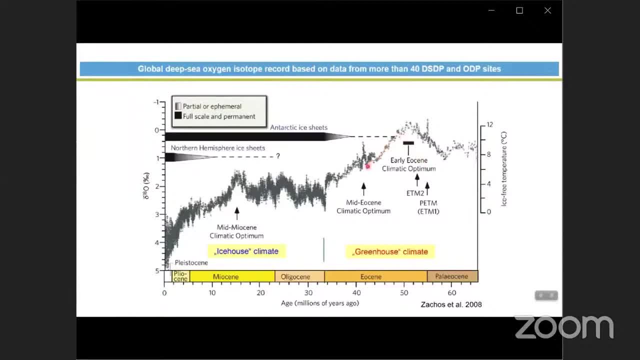 northern germany covers the entire northern germany, covers the entire paleogene greenhouse phase and its paleogene greenhouse phase and its paleogene greenhouse phase and its gentle demise almost continuously from gentle demise almost continuously from gentle demise almost continuously from the latest paleogene to the middle, the latest paleogene to the middle. 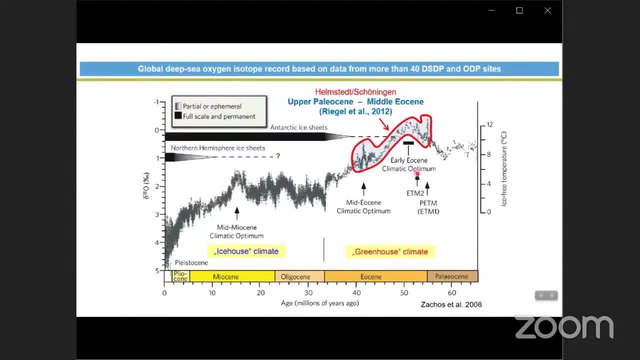 the latest paleogene to the middle eocene, including the early eocene eocene, including the early eocene eocene, including the early eocene climatic optimum, and some short-term climatic optimum and some short-term climatic optimum and some short-term warming events such as the paleogene. 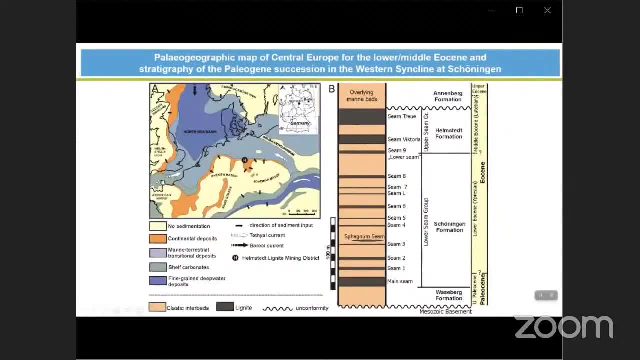 warming events, such as the paleogene warming events, such as the paleogene eocene thermal maximum and the more than 200 meter succession. and the more than 200 meter succession and the more than 200 meter succession has been deposited in an estuarine. has been deposited in an estuarine. 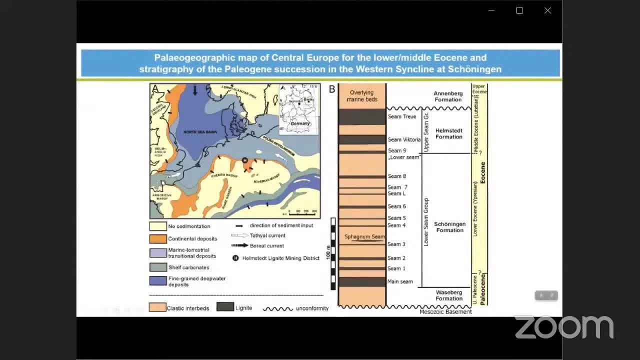 has been deposited in an estuarine setting, at the southern margin of the setting, at the southern margin of the setting, at the southern margin of the proto-northy, proto-northy, proto-northy. the aim of an ongoing project is to study. the aim of an ongoing project is to study. 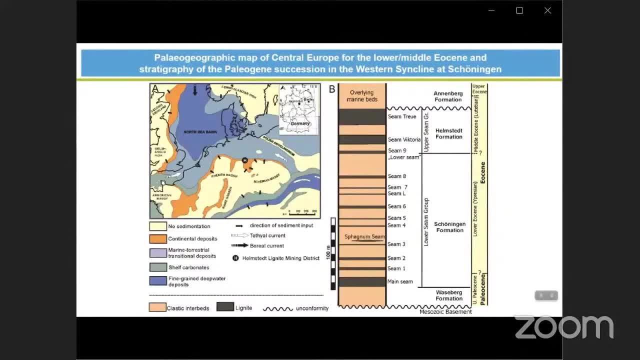 the aim of an ongoing project is to study the response of the vegetation and this, the response of the vegetation, and this, the response of the vegetation and this paralic environment to the long and paralic environment, to the long and paralic environment to the long and short-term thermal events, by making use 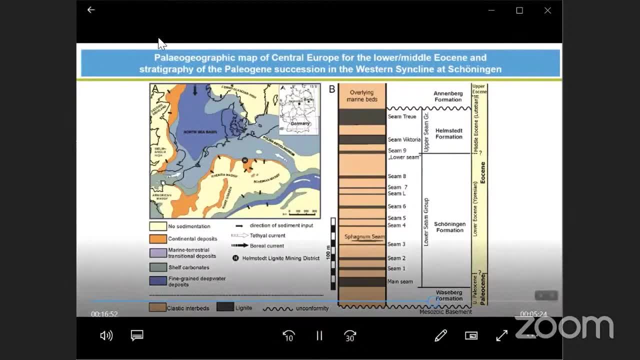 short-term thermal events by making use short-term thermal events by making use of pollen and spores as proxies of pollen and spores as proxies of pollen and spores as proxies. and here we present a new stratigraphic. and here we present a new stratigraphic. 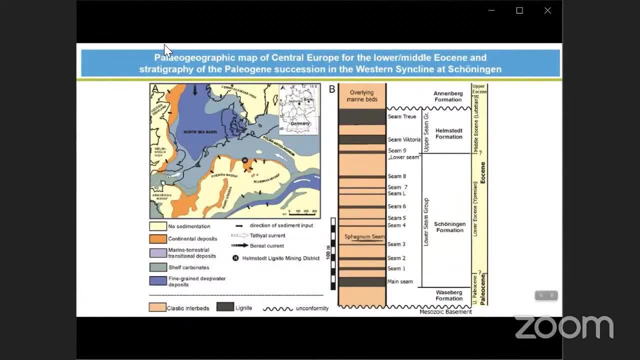 and here we present a new stratigraphic framework for the succession framework, for the succession framework for the succession, which allows for an exact identification, which allows for an exact identification, which allows for an exact identification of individual paleogene thermal events, of individual paleogene thermal events. 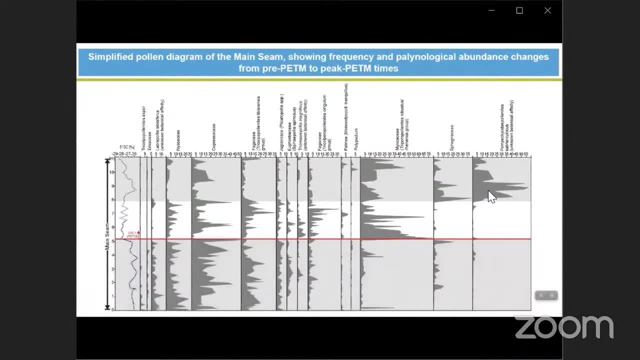 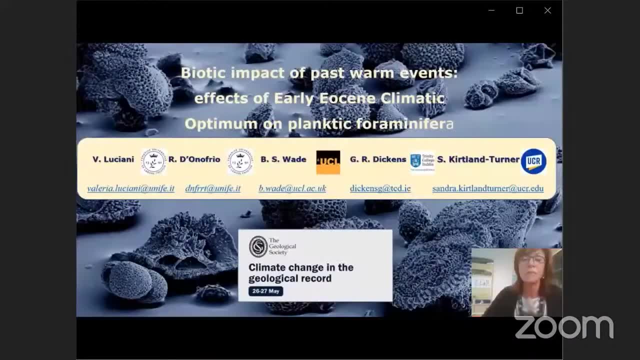 of individual paleogene thermal events. now it is possible to reconstruct the. now it is possible to reconstruct the. now it is possible to reconstruct the vegetation vegetation: vegetation for times before, during, for times before during, for times before, during and after specific thermal events. and after specific thermal events. 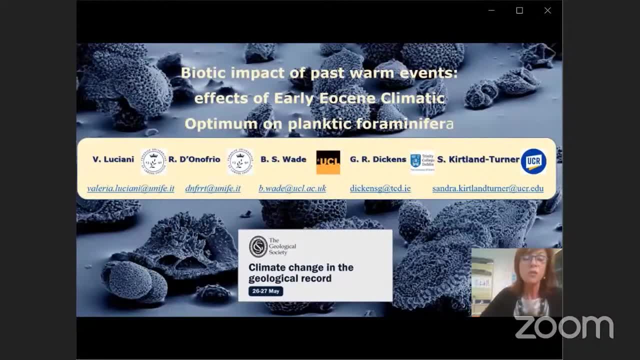 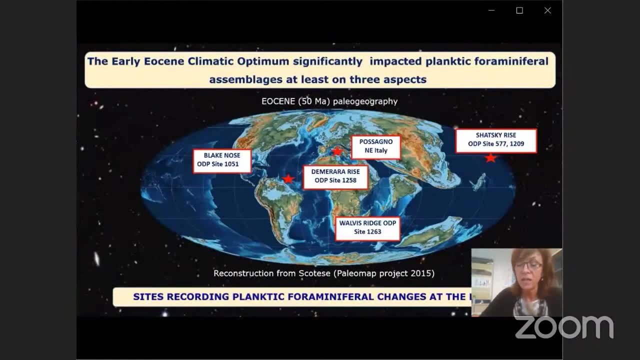 and after specific thermal events. hello, this is valerio gianni speaking. hello, this is valerio gianni speaking. hello, this is valerio gianni speaking at the poster session. now we talk about at the poster session. now we talk about at the poster session. now we talk about: on planting for a miniferal assemblages. 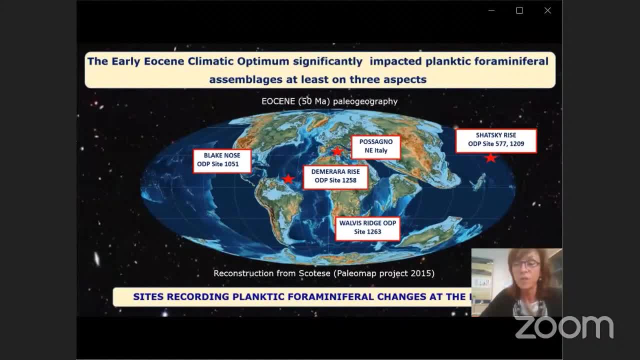 on planting for a miniferal assemblages. on planting for a miniferal assemblages. these are the size investigated from the. these are the size investigated from the. these are the size investigated from the atlantic to the pacific ocean. atlantic to the pacific ocean. 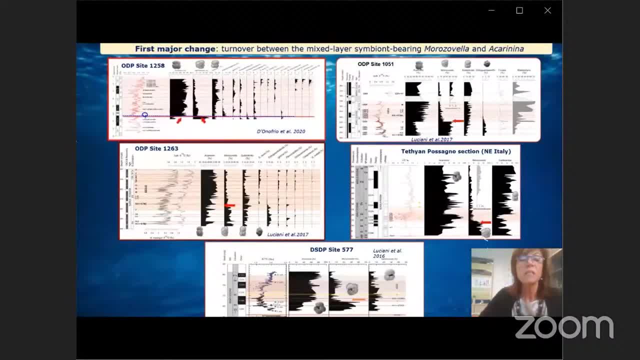 atlantic to the pacific ocean and a first major change. and a first major change. and a first major change is a turnover between the general, is a turnover between the general, is a turnover between the general morozovella and the carinina, and morozovella and the carinina, and 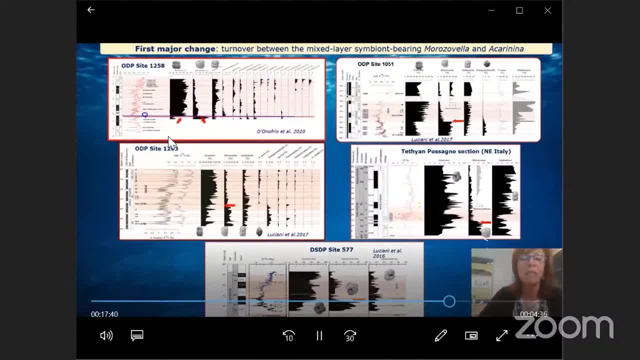 morozovella and the carinina, and precisely the genus morozovella, precisely the genus morozovella, precisely the genus morozovella permanently and markedly declined at, permanently and markedly declined at, permanently and markedly declined at the beginning of the eco close to the j. 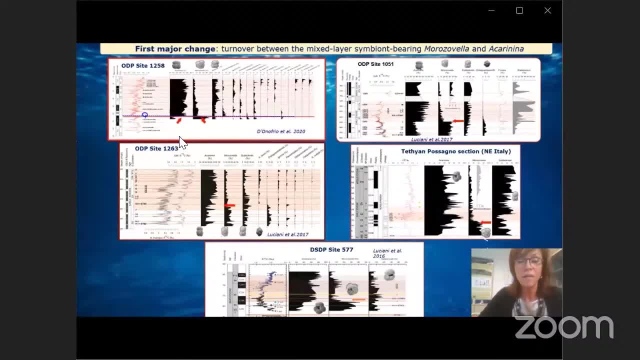 the beginning of the eco close to the j. the beginning of the eco close to the j event event event and the genus carinina increase in and the genus carinina increase in and the genus carinina increase in. abundance and diversity. abundance and diversity. 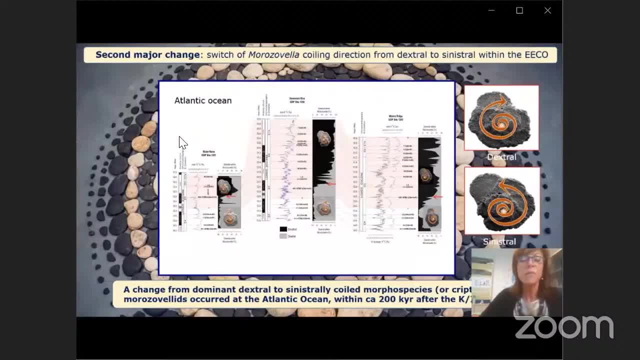 abundance and diversity. a second major change is a switch. a second major change is a switch. a second major change is a switch in the morozovella coiling direction, in the morozovella coiling direction, in the morozovella coiling direction from. 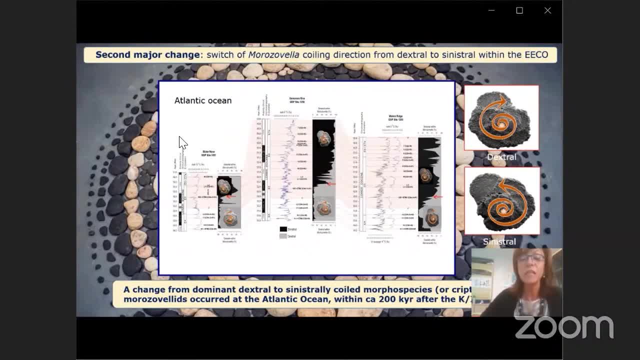 from from from predominantly dextral to sinistral, from predominantly dextral to sinistral, from predominantly dextral to sinistral, within the eco, close to the within the eco, close to the within the eco. close to the key x event. and finally, a third major. 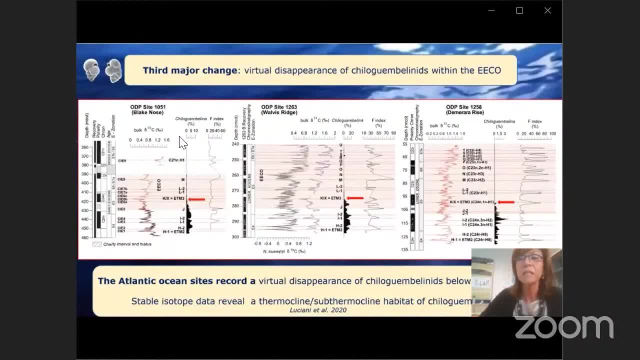 key x event. and finally, a third major key x event. and finally, a third major change involved. change involved, change involved: the genus kilogumbelina that is known, the genus kilogumbelina that is known, the genus kilogumbelina that is known to live within the. 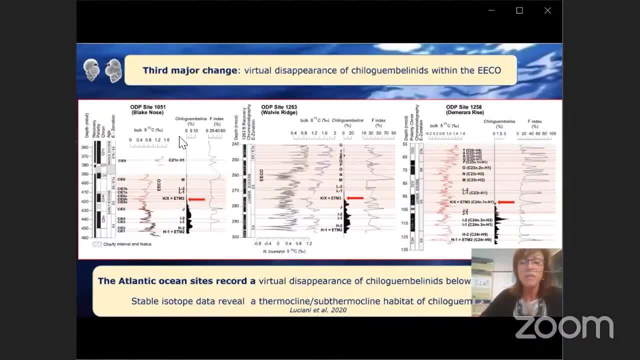 to live within the, to live within the oxygen minimum zone and this genus oxygen minimum zone and this genus oxygen minimum zone and this genus disappear, disappear, disappear, close to the key x event. of course we close to the key x event. of course we close to the key x event. of course we will talk about. 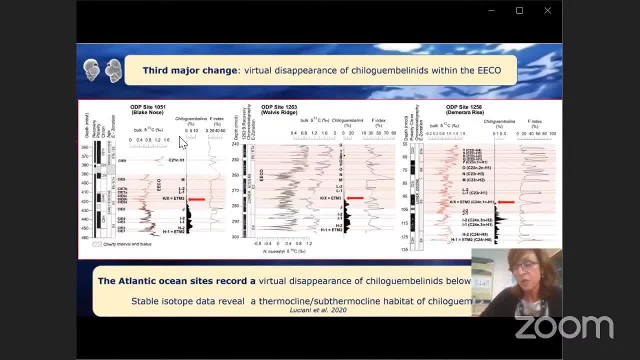 will talk about. will talk about the causes and the scenario related to the causes, and the scenario related to the causes and the scenario related to these themselves changes. these themselves changes. hi everybody, i'm alan mancini from the. hi everybody, i'm alan mancini from the. 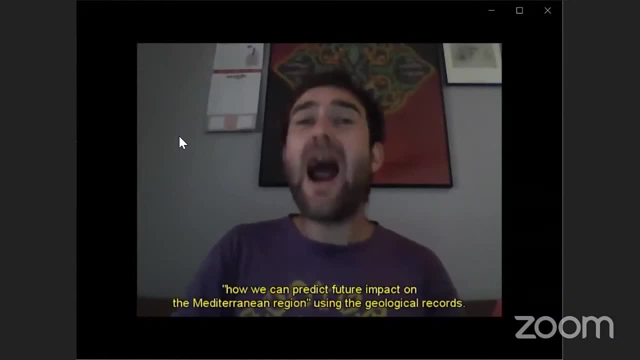 hi everybody, i'm alan mancini from the university of turin university of turin, university of turin, and here i present some ideas regarding: and here i present some ideas regarding, and here i present some ideas regarding how we can predict future impact on the. 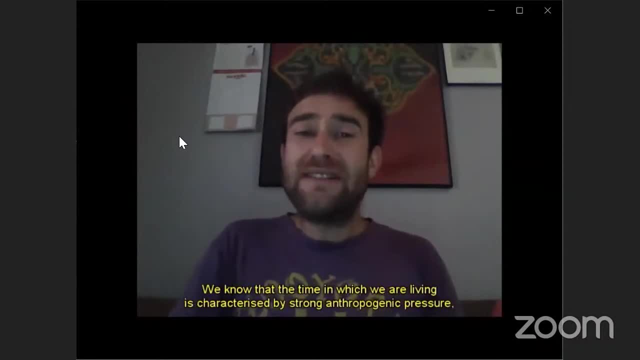 how we can predict future impact on the. how we can predict future impact on the mediterranean region- mediterranean region, mediterranean region- using the geological records. we know that using the geological records, we know that, using the geological records, we know that the time which we are living is. 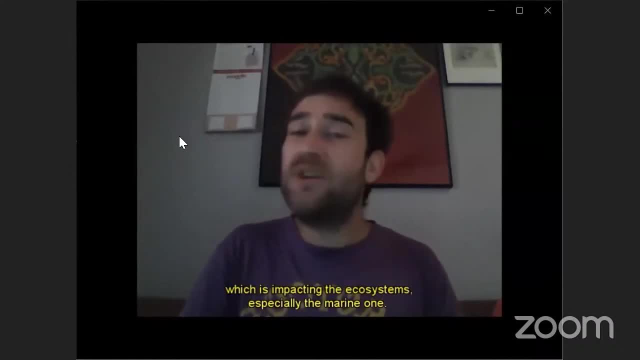 the time which we are living is the time which we are living is characterized by strong anthropogenic, characterized by strong anthropogenic, characterized by strong anthropogenic pressure which is impacting the pressure which is impacting the pressure which is impacting the ecosystem, especially the marine one. ecosystem, especially the marine one. 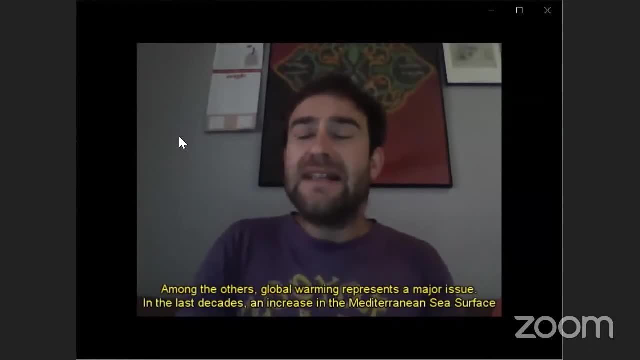 ecosystem, especially the marine one, among the others. global warming, among the others. global warming, among the others. global warming represent a major issue. represent a major issue. represent a major issue. in the last decades, an increase in the in the last decades, an increase in the. in the last decades, an increase in the mediterranean sea surface temperatures. 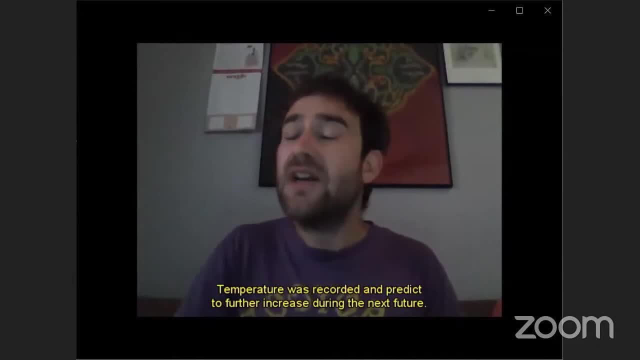 mediterranean sea surface temperatures. mediterranean sea surface temperatures was recorded and predict to further. was recorded and predict to further. was recorded and predict to further increase during the next future. increase during the next future. increase during the next future. this is happening along with the. 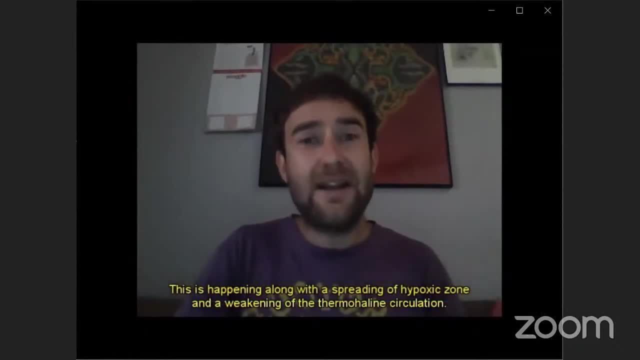 this is happening along with the. this is happening along with the spreading of the hypoxic zone and spreading of the hypoxic zone and spreading of the hypoxic zone and weakening of the thermal line. weakening of the thermal line, weakening of the thermal line. circulation, circulation, circulation: the evolution of these processes and their 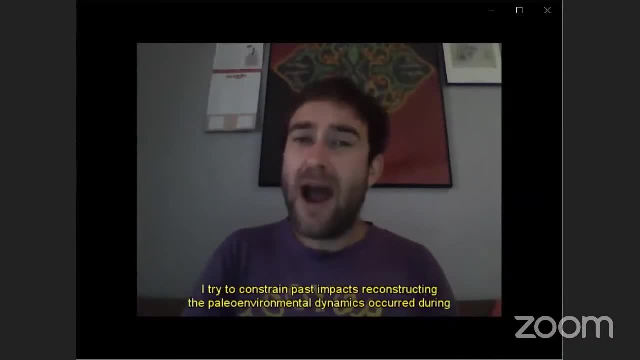 the evolution of these processes and their the evolution of these processes and their impacts are hard to predict. this is the impacts are hard to predict. this is the impacts are hard to predict. this is the reason why i try to constrain past. reason why i try to constrain past. 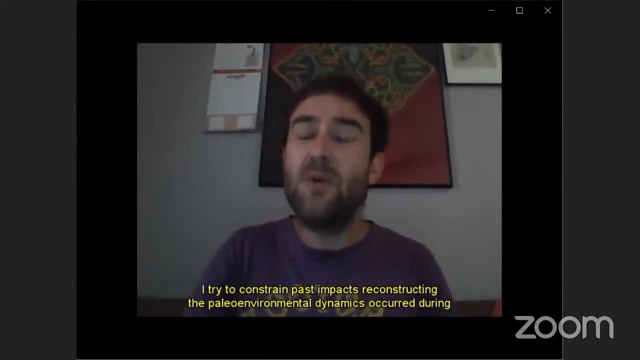 reason why i try to constrain past impacts: reconstructing the impacts. reconstructing the impacts. reconstructing the environmental dynamics occurring during. environmental dynamics occurring during. environmental dynamics occurring during the cyclical messinian warming phases: the cyclical messinian warming phases. the cyclical messinian warming phases, with the aim to indicate possible future. 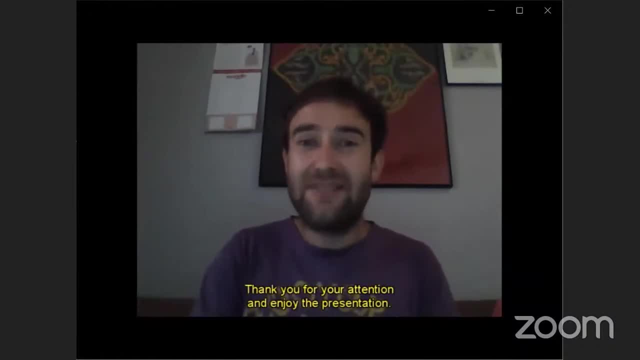 with the aim to indicate possible future. with the aim to indicate possible future impact on the mediterranean region. impact on the mediterranean region. impact on the mediterranean region. thank you for your attention and enjoy. thank you for your attention and enjoy. thank you for your attention and enjoy the presentation. 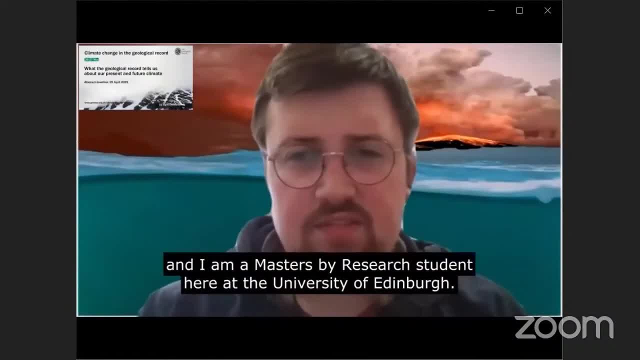 my name is matthew status and i am a. my name is matthew status and i am a. my name is matthew status and i am a master's by research student here at the master's by research student here at the master's by research student here at the university of edinburgh. 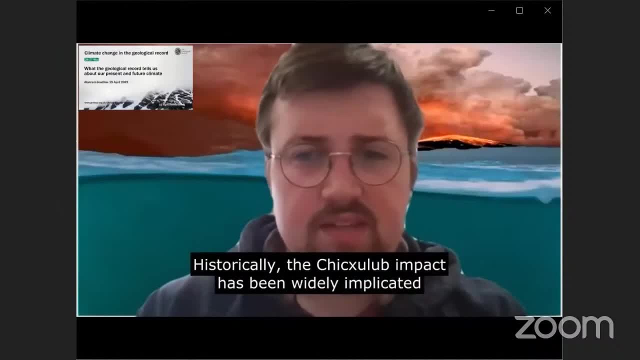 university of edinburgh university of edinburgh. historically, the chixula impact has been. historically, the chixula impact has been. historically, the chixula impact has been widely implicated as the main driver of widely implicated as the main driver of widely implicated as the main driver of the cretaceous paleogene mass extinction. 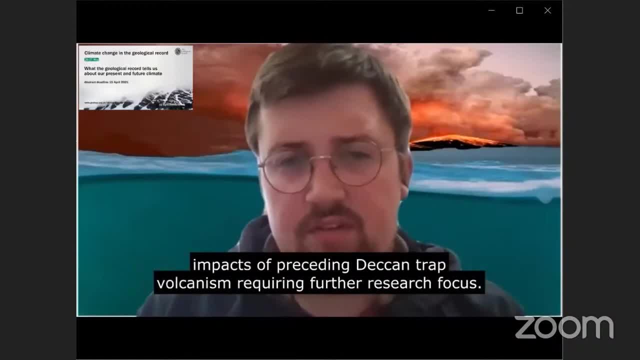 the cretaceous paleogene mass extinction. the cretaceous paleogene mass extinction with the exact environmental impacts of. with the exact environmental impacts of. with the exact environmental impacts of preceding decantrap volcanism requiring preceding decantrap volcanism. requiring preceding decantrap volcanism. requiring further research focus. 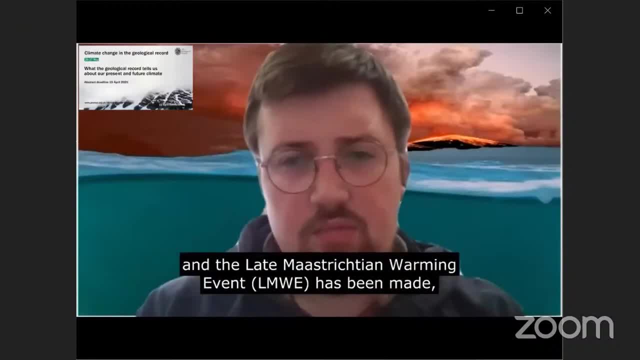 further research focus. further research focus, although a casual link between decant, although a casual link between decant, although a casual link between decant volcanism and the late mastriptine volcanism and the late mastriptine volcanism and the late mastriptine warming event has been made, 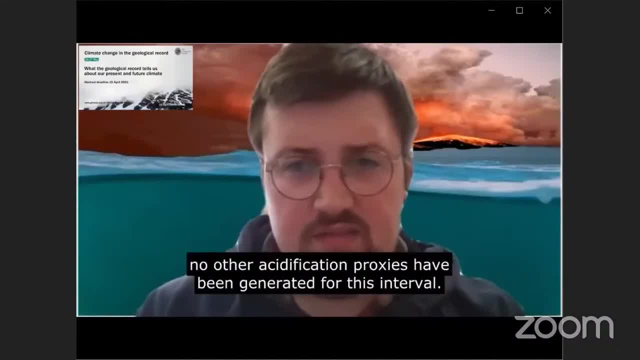 warming event has been made. warming event has been made. no other acidification proxies has been. no other acidification proxies has been. no other acidification proxies has been generated for this interval. generated for this interval. generated for this interval: we have generated novel benthic boron. 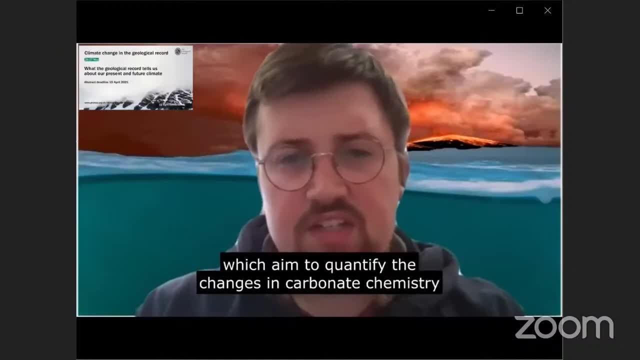 we have generated novel benthic boron. we have generated novel benthic boron. calcium trace element analyses: calcium trace element analyses: calcium trace element analyses which aim to quantify the changes, in which aim to quantify the changes, in which aim to quantify the changes in carbonic chemistry. 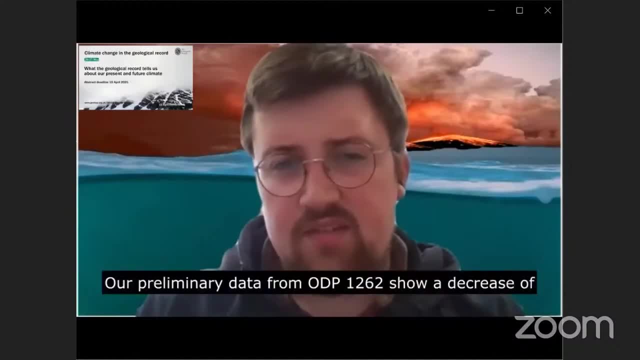 carbonic chemistry. carbonic chemistry at the peak of this event, suggesting at the peak of this event, suggesting at the peak of this event, suggesting potential ocean acidification caused by potential ocean acidification caused by potential ocean acidification caused by decant outgassing. if you're interested, 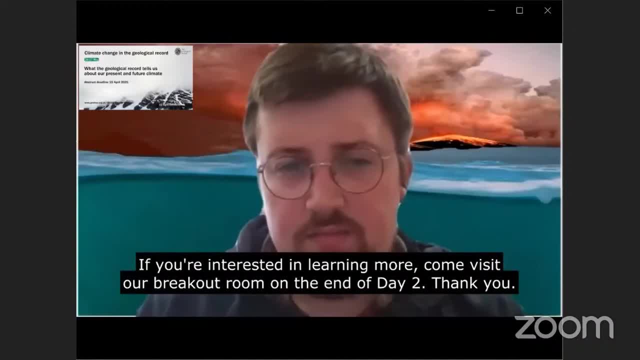 decant outgassing. if you're interested, decant outgassing. if you're interested in learning more, come visit our break in learning more. come visit our break in learning more. come visit our break up room on the end of day two. thank you up room on the end of day two, thank you. 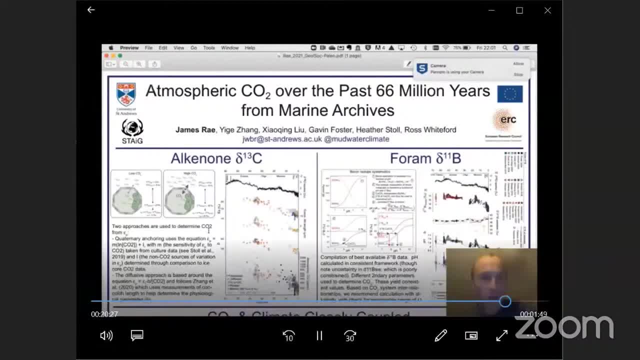 up room on the end of day two. thank you. hi everyone in this poster we compile. hi everyone in this poster we compile. hi everyone in this poster we compile and re-evaluate the best possible co2 and re-evaluate the best possible co2 and re-evaluate the best possible co2 reconstructions. 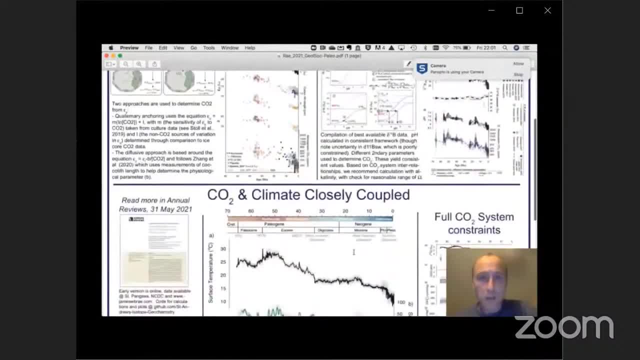 reconstructions: reconstructions from alkanones and boron isotopes. the from alkanones and boron isotopes. the from alkanones and boron isotopes. the results of this are discussed in more. results of this are discussed in more. results of this are discussed in more detail in a paper that's just out in. 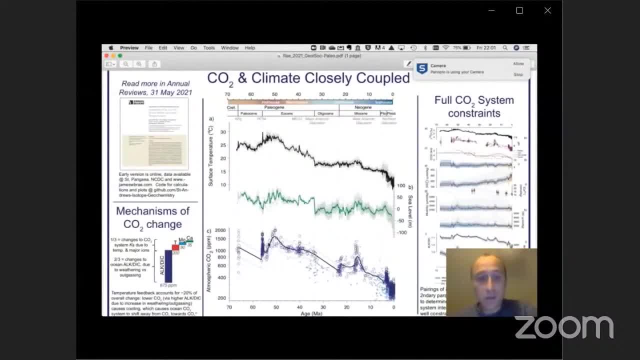 detail in a paper that's just out in detail, in a paper that's just out in annual reviews, annual reviews, annual reviews, and the key result that comes out is: and the key result that comes out is: and the key result that comes out is that our best available reconstructions. 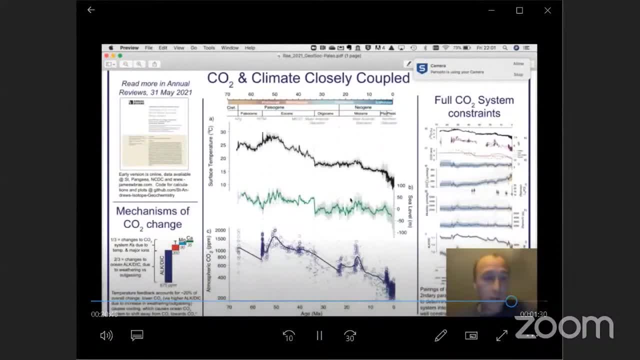 that our best available reconstructions, that our best available reconstructions of co2 are closely coupled with climate of co2 are closely coupled with climate of co2 are closely coupled with climate. we investigate some of the mechanisms of. we investigate some of the mechanisms of. we investigate some of the mechanisms of co2 change- about two-thirds of. 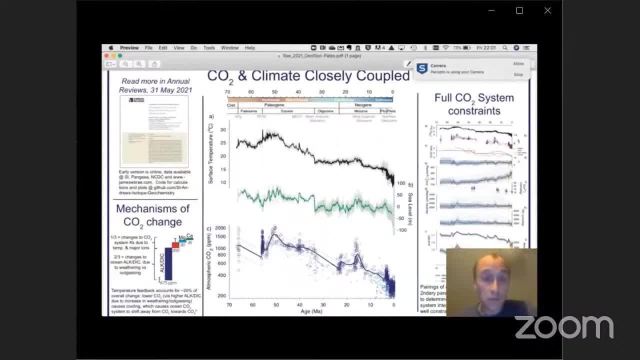 co2 change about two-thirds of co2 change about two-thirds of cenozoic co2 change is explained by cenozoic co2 change is explained by cenozoic co2 change is explained by changes in ocean chemistry. changes in ocean chemistry: changes in ocean chemistry- chemistry via outgassing and weathering. 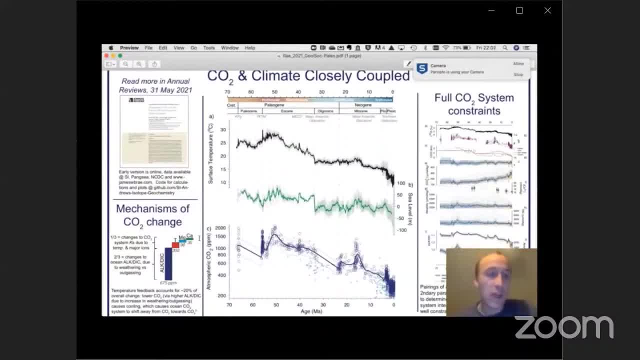 chemistry via outgassing and weathering. chemistry via outgassing and weathering with the remaining thirds, due to changes with the remaining thirds due to changes with the remaining thirds due to changes in the equilibrium constants in the equilibrium constants in the equilibrium constants due to temperature feedback and major. 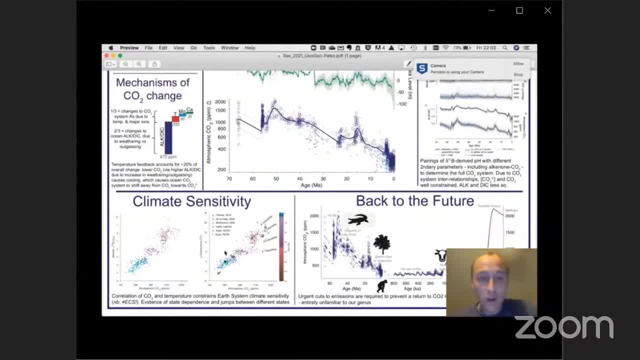 due to temperature feedback and major due to temperature feedback and major iron composition: iron composition, iron composition. we place broad constraints on earth. we place broad constraints on earth. we place broad constraints on earth. system climate sensitivity: noting system climate sensitivity. noting system, climate sensitivity, noting the potential, the potential. 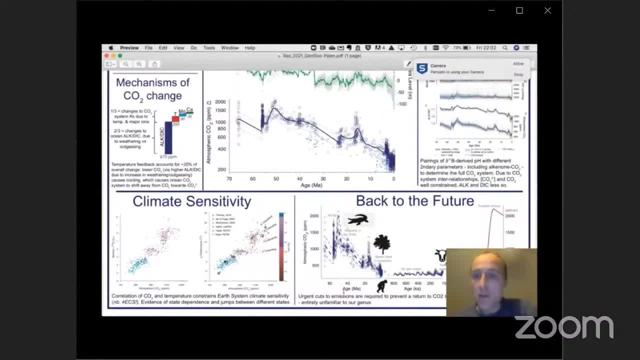 the potential for state dependence in climate, for state dependence in climate, for state dependence in climate, sensitivity, sensitivity, sensitivity, and we highlight that future energy and we highlight that future energy and we highlight that future energy choices have the potential to send co2. choices have the potential to send co2. 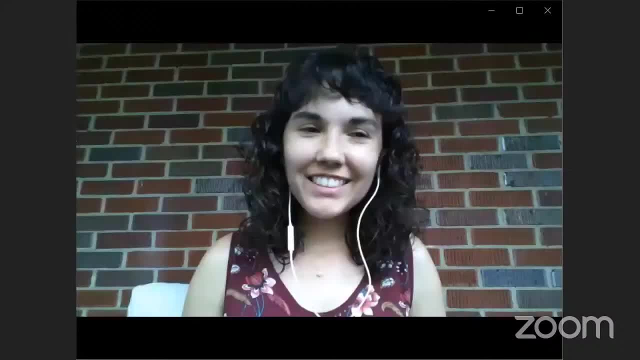 choices have the potential to send co2 levels back to those associated with the levels, back to those associated with the levels, back to those associated with the distant past. distant past, distant past. hi everyone, my name is asia watkins and. hi everyone, my name is asia watkins, and. 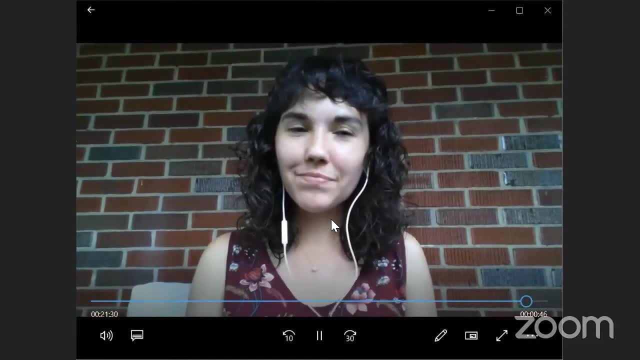 hi everyone, my name is asia watkins and i'm a phd student studying philosophy of. i'm a phd student studying philosophy of. i'm a phd student studying philosophy of science at boston university. my poster: science at boston university. my poster- science at boston university. my poster today is about how to use a process. 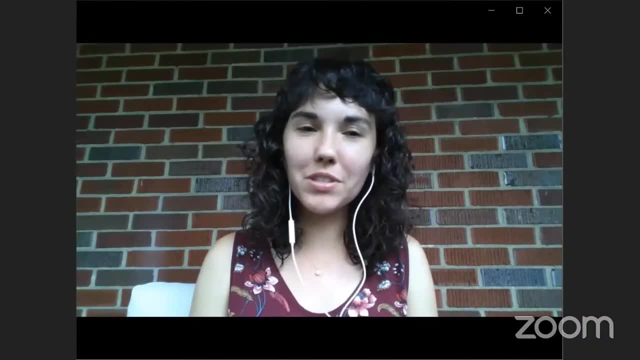 today is about how to use a process. today is about how to use a process called temporal scaling to compare past, called temporal scaling, to compare past, called temporal scaling. to compare past and present climate change episodes with, and present climate change episodes with, and present climate change episodes, with the goal of establishing paleo climate. 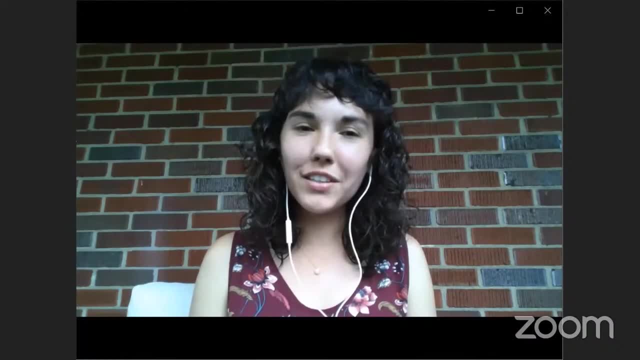 the goal of establishing paleo climate. the goal of establishing paleo climate. analogues: temporal scaling is predicated. analogues: temporal scaling is predicated. analogues: temporal scaling is predicated on the observation that rates are not in. on the observation that rates are not in. 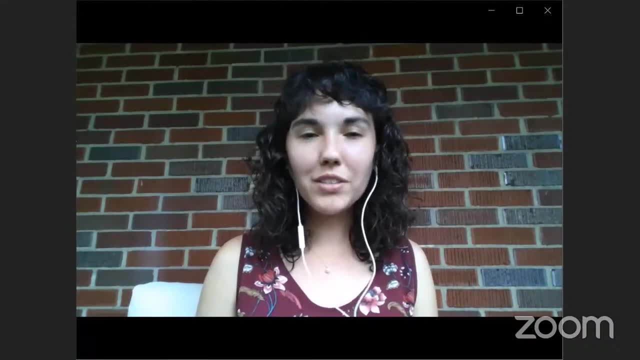 on the observation that rates are not, in general, independent of the durations general, independent of the durations general, independent of the durations over which they are measured. measuring over which they are measured, measuring over which they are measured, measuring processes over shorter durations, processes over shorter durations, processes over shorter durations, produces systematically higher rates than 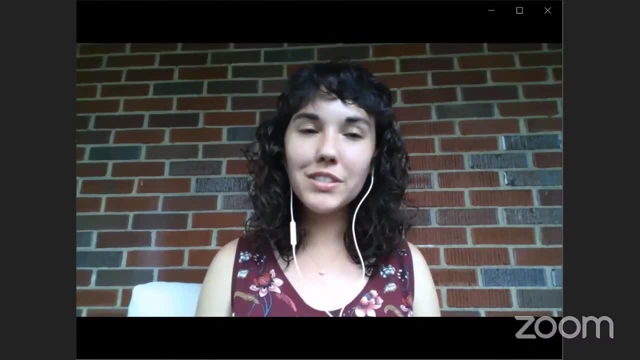 produces systematically higher rates than produces systematically higher rates than if these same processes are measured over. if these same processes are measured over. if these same processes are measured over longer durations, temporal scaling is longer durations. temporal scaling is longer durations. temporal scaling is often useful in the historical sciences. 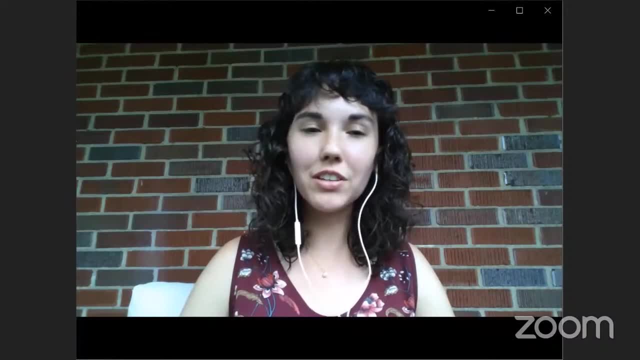 often useful in the historical sciences. often useful in the historical sciences, including paleoclimatology, but also including paleoclimatology, but also including paleoclimatology, but also paleontology, geology and archaeology, paleontology, geology and archaeology, paleontology, geology and archaeology, because we tend to have data of a lower. 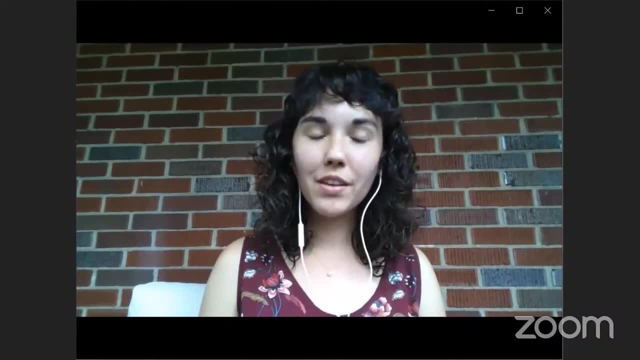 because we tend to have data of a lower, because we tend to have data of a lower temporal resolution for processes. that temporal resolution for processes, that temporal resolution for processes that happen further back in time, happen further back in time, happen further back in time. so i look forward to having you join my 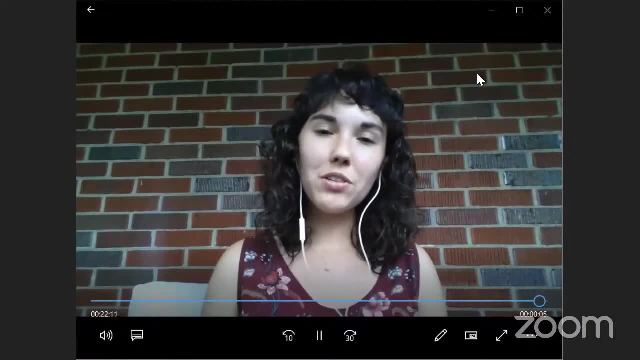 so i look forward to having you join my. so i look forward to having you join my breakout room to hear more about how breakout room, to hear more about how breakout room, to hear more about how temporal scaling works and how we can temporal scaling works and how we can. 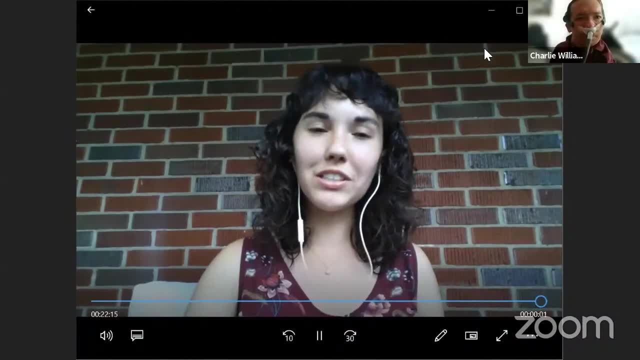 temporal scaling works and how we can use it to compare cases of climate. use it to compare cases of climate. use it to compare cases of climate change in the geological record, to change in the geological record, to change in the geological record. to climate change today. climate change today. 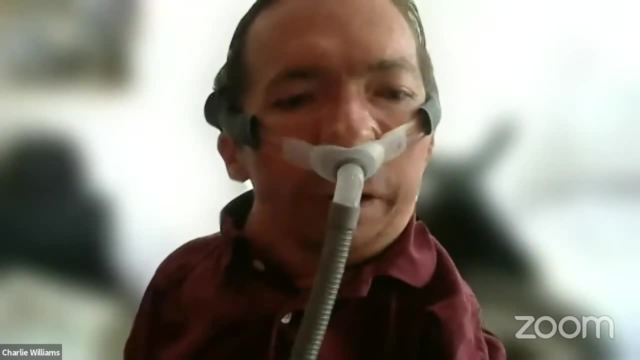 climate change today. okay, brilliant, thank you ever so much. okay, brilliant. thank you ever so much, okay, brilliant. thank you ever so much for all of those, for all of those, for all of those. talks for those of you that are listening. talks for those of you that are listening. 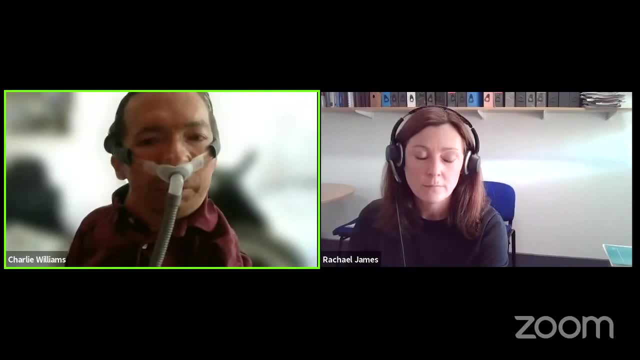 talks for those of you that are listening, and and and that will be in the uh breakout rooms. that will be in the uh breakout rooms. that will be in the uh breakout rooms later. i look forward to uh to meeting later. i look forward to uh to meeting. 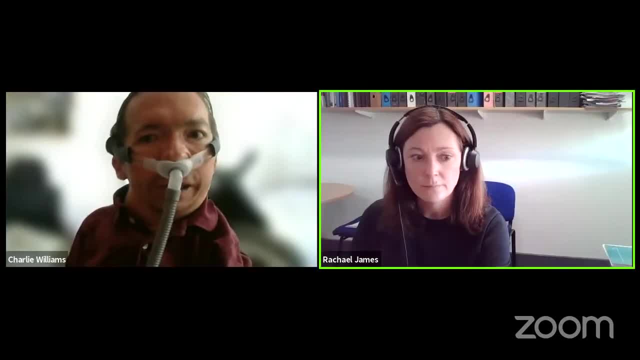 later. i look forward to, uh, to meeting you and talking to you, you and talking to you, you and talking to you. so our final invited speaker is rachel. so our final invited speaker is rachel. so our final invited speaker is rachel james, who is a professor of geochemistry. 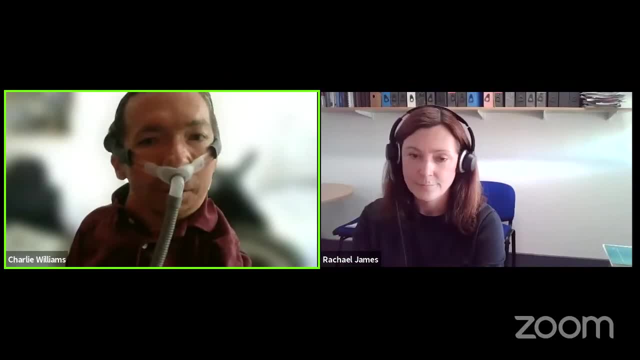 james, who is a professor of geochemistry. james, who is a professor of geochemistry at the university of southampton, here in at the university of southampton, here in at the university of southampton, here in the uk, the uk. the uk, rachel is interested in developing novel. 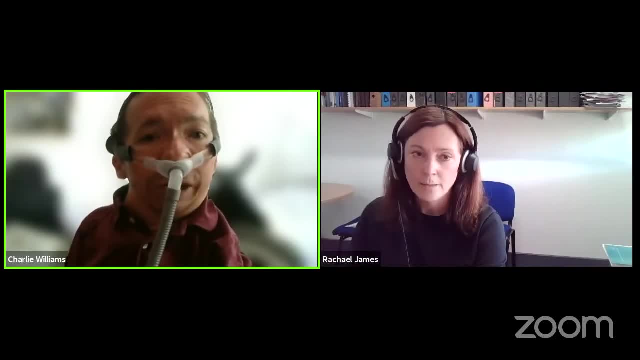 rachel is interested in developing novel rachel is interested in developing novel chemical and isotopic techniques to chemical and isotopic techniques. to chemical and isotopic techniques to improve our understanding of ocean, improve our understanding of ocean, improve our understanding of ocean and societal challenges today. 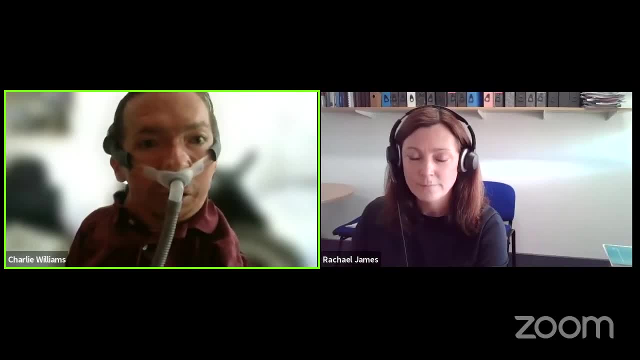 and societal challenges today. and societal challenges today uh rachel is going to be talking about. uh rachel is going to be talking about. uh rachel is going to be talking about question nine of our statement. question nine of our statement. question nine of our statement: what is the role of geology in dealing 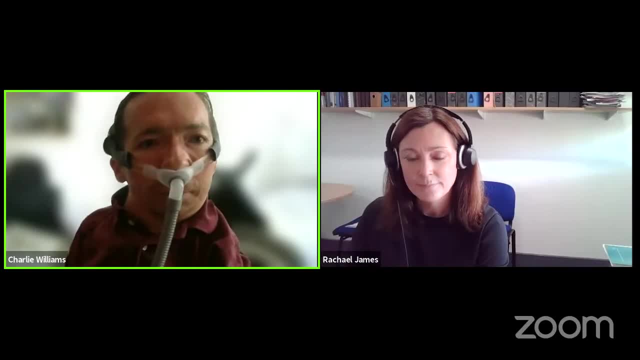 what is the role of geology in dealing, what is the role of geology in dealing with the climate emergency, with the climate emergency, with the climate emergency for a sustainable future. so everything for a sustainable future, so everything for a sustainable future. so everything, grateful as before. 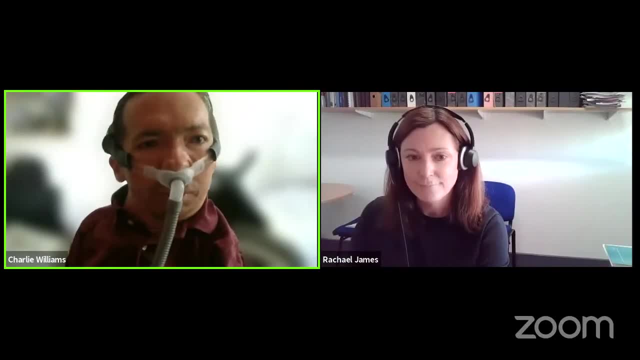 grateful as before. grateful as before. i will turn my video on to give you a. i will turn my video on to give you a. i will turn my video on to give you a two-minute warning. two-minute warning. two-minute warning at the end, over to you. 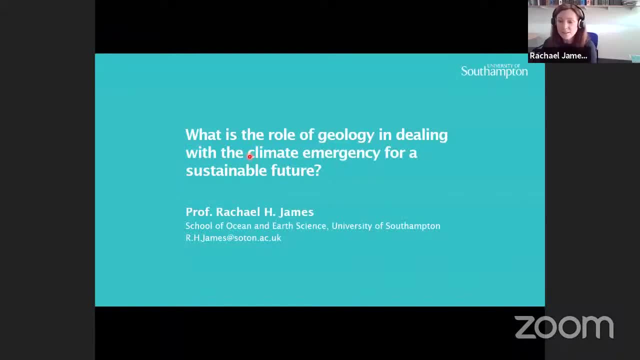 at the end over to you. at the end, over to you. thanks very much for that introduction. thanks very much for that introduction. thanks very much for that introduction, charlie and i'm delighted to be here, charlie and i'm delighted to be here, charlie and i'm delighted to be here today. uh, i'm presenting something a. 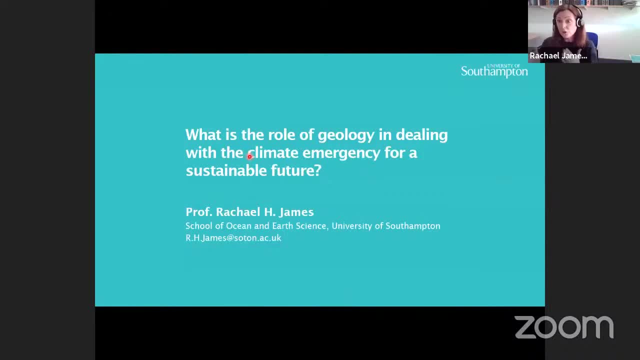 today, uh, i'm presenting something a today. uh, i'm presenting something a little bit different now, little bit different now, little bit different now. so, thinking about uh, not not so many. so thinking about uh, not not so many. so thinking about uh, not not so many wiggly lines, but thinking about how. 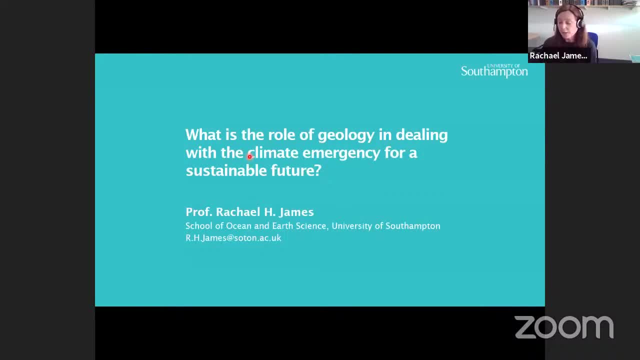 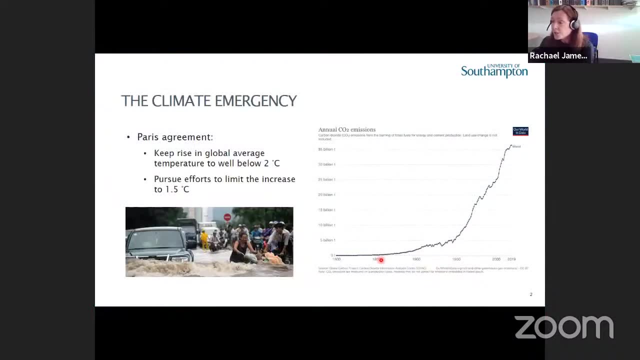 wiggly lines, but thinking about how wiggly lines? but thinking about how geologists can contribute. geologists can contribute. geologists can contribute to solving the climate emergency. uh. so so this is a plot here of uh. uh. so so this is a plot here of uh. 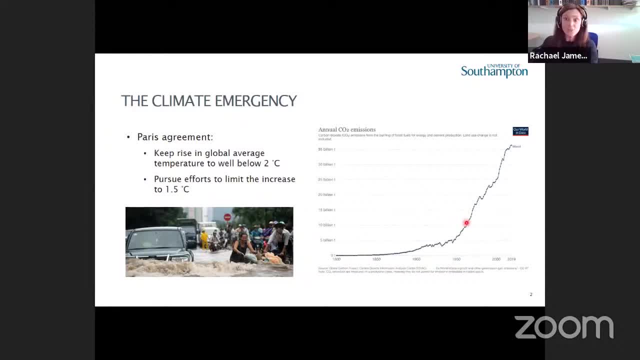 uh, so so this is a plot here of uh- anthropogenic carbon dioxide emissions, anthropogenic carbon dioxide emissions, anthropogenic carbon dioxide emissions, and, as you're well and truly um well, and as you're well and truly um well, and as you're well and truly um well, versed in now. 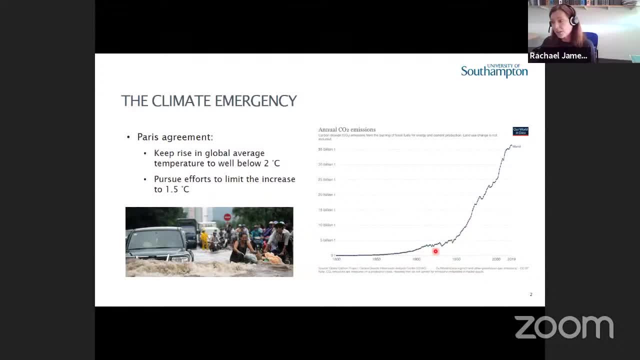 versed in now. versed in now. we can see that uh- anthropogenic carbon. we can see that uh- anthropogenic carbon. we can see that uh- anthropogenic carbon. dioxide emissions have continued to dioxide emissions have continued to dioxide emissions have continued to increase on a sharply upward trajectory. 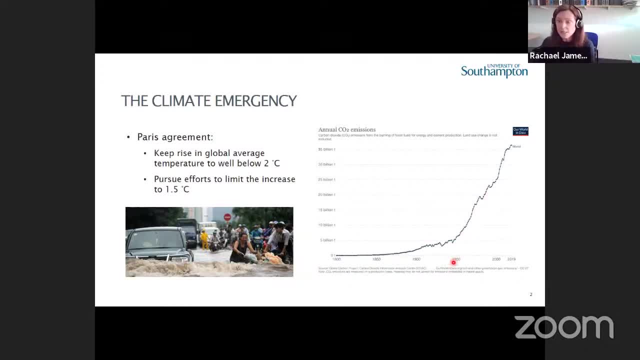 increase on a sharply upward trajectory, increase on a sharply upward trajectory since the industrial revolution, since the industrial revolution, since the industrial revolution. and there's now extremely strong and there's now extremely strong and there's now extremely strong evidence that this is causing uh, evidence that this is causing uh. 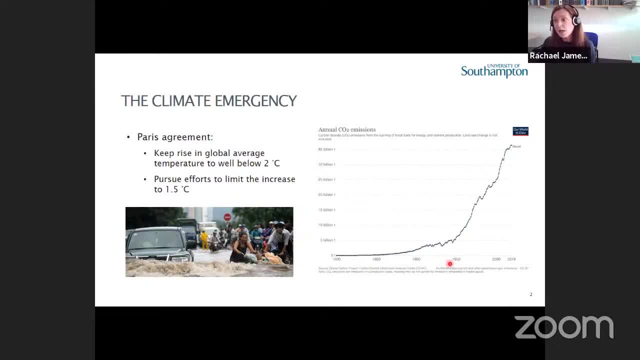 evidence that this is causing, uh, global warming. it's causing warming of global warming. it's causing warming of global warming. it's causing warming of the surface oceans, the surface oceans, the surface oceans. uh, it's changing our weather patterns. uh, it's changing our weather patterns. uh, it's changing our weather patterns and it's causing melting at the poles. 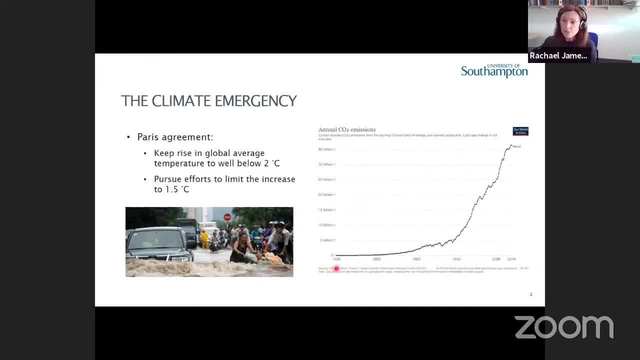 and it's causing melting at the poles, and it's causing melting at the poles, and hence sea level rise, and hence sea level rise, and hence sea level rise. so, in recognition of this groups of so, in recognition of this groups of so, in recognition of this, groups of countries have come together. 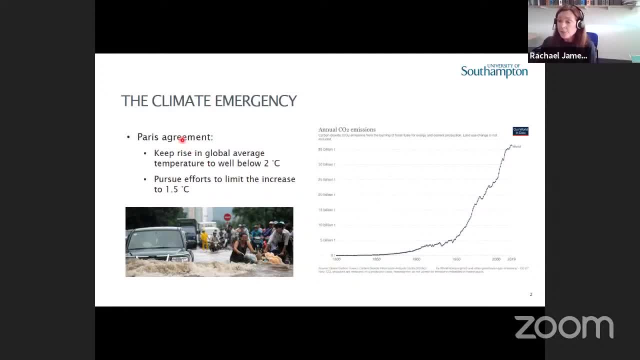 countries have come together. countries have come together to figure out what we can do and to figure out what we can do and to figure out what we can do. and in the 2016 paris agreement, it was in the 2016 paris agreement. it was in the 2016 paris agreement. it was decided. 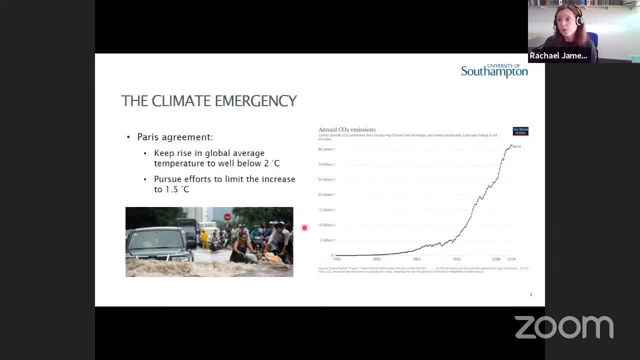 decided, decided by the global nations, that the ambition by the global nations, that the ambition by the global nations, that the ambition was to was to, was to keep the rise in global average, keep the rise in global average, keep the rise in global average temperature to well below. 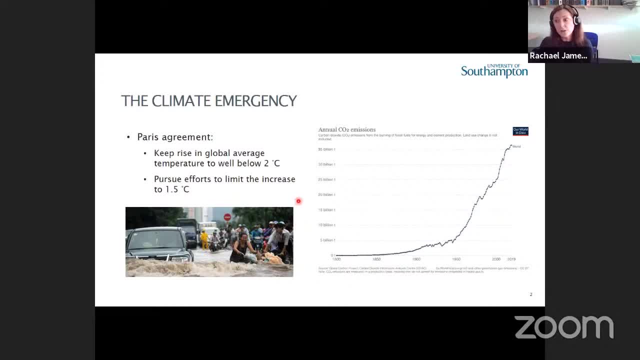 temperature to well below temperature, to well below two degrees centigrade and to pursue two degrees centigrade and to pursue two degrees centigrade and to pursue efforts to limit the increase to one and efforts to limit the increase to one and efforts to limit the increase to one and a half degrees. 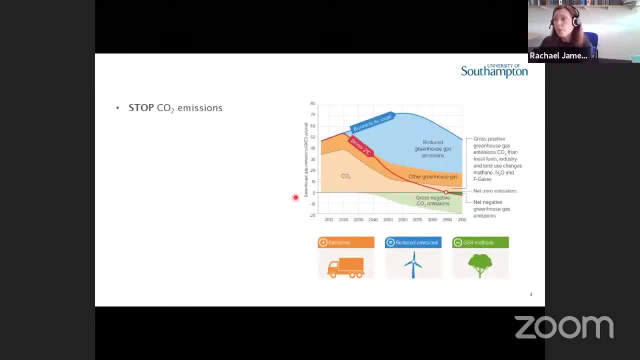 a half degrees, a half degrees. so the question is then: how? how are we so? the question is then: how? how are we so? the question is then: how? how are we going to do this, going to do this, going to do this? well, the most obvious thing we can do is 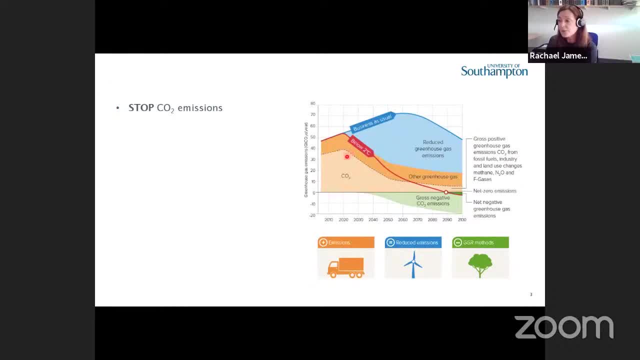 well, the most obvious thing we can do is, well, the most obvious thing we can do is to stop, to stop, to stop. emissions of greenhouse gases and carbon, emissions of greenhouse gases and carbon, emissions of greenhouse gases and carbon dioxide, dioxide dioxide. and if we, if we look at this plot here, we, 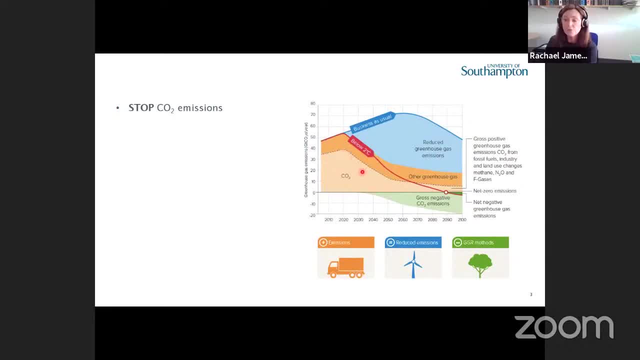 and if we, if we look at this plot here, we, and if we, if we look at this plot here, we can see that we can do this pretty, can see that we can do this pretty, can see that we can do this pretty quickly if we transition from an 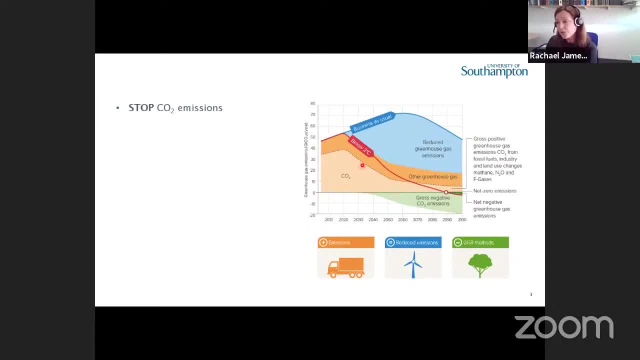 quickly if we transition from an quickly, if we transition from an economy based on fossil fuels economy, based on fossil fuels economy, based on fossil fuels, to renewable energy sources, to renewable energy sources, to renewable energy sources. there's good capacity there to bring. there's good capacity there to bring. 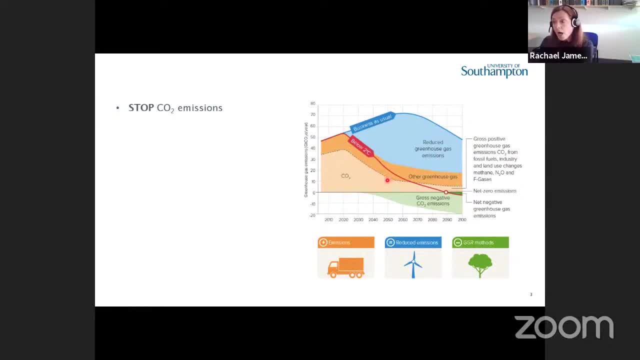 there's good capacity there to bring down levels of atmospheric carbon down levels of atmospheric carbon down levels of atmospheric carbon dioxide, dioxide, dioxide. but you can see that this curve then. but you can see that this curve then. but you can see that this curve then starts to tail off and the reason for 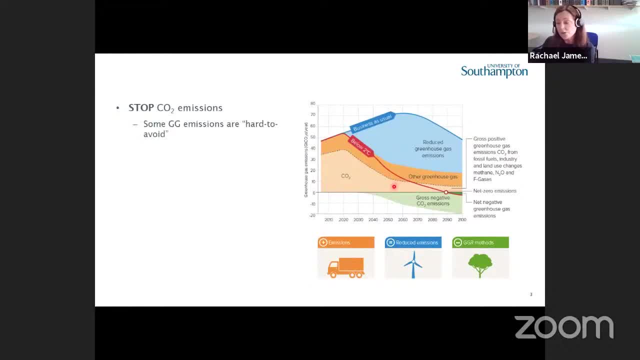 starts to tail off, and the reason for starts to tail off and the reason for that is it's going to take some time to that. is it's going to take some time to that? is it's going to take some time to reduce its reliance on fossil fuels? 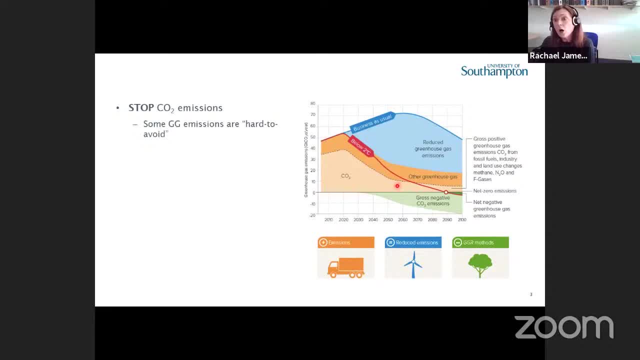 reduce its reliance on fossil fuels. reduce its reliance on fossil fuels and other industries such as agriculture, and other industries such as agriculture and other industries such as agriculture are always basically going to be, are always basically going to be, are always basically going to be emitting carbon dioxide. 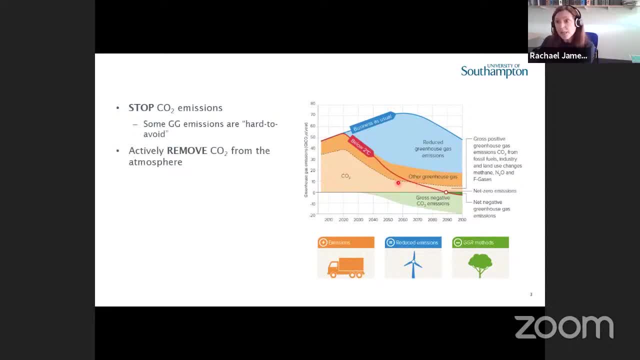 so what we can see is by about 2050. we, so what we can see is by about 2050. we, so what we can see is by about 2050. we actually need to start, actually need to start, actually need to start, not only reducing carbon dioxide. 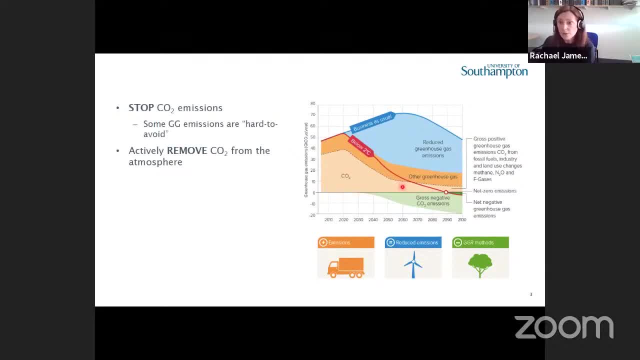 not only reducing carbon dioxide, not only reducing carbon dioxide emissions, but we need to start actively emissions, but we need to start actively emissions, but we need to start actively removing carbon dioxide from the removing carbon dioxide from the removing carbon dioxide from the atmosphere, atmosphere, atmosphere. if we're going to keep to that one and a. 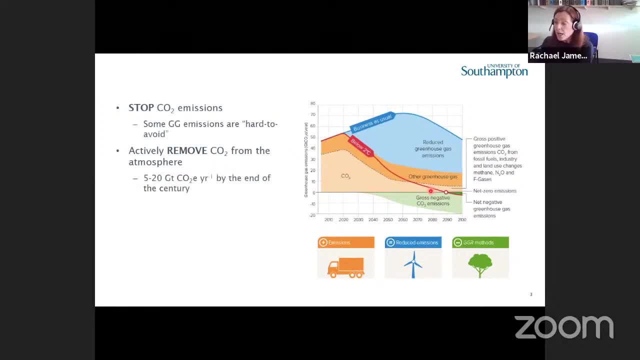 if we're going to keep to that one and a, if we're going to keep to that one and a half or two degree, half or two degree, half or two degree target, and if we look at projections of target and if we look at projections of target and if we look at projections of what's required. 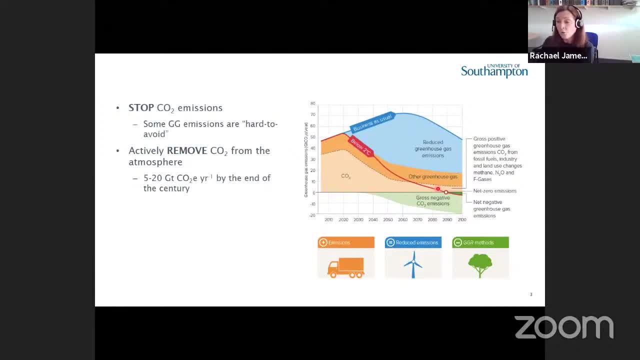 what's required. what's required we're going to need, on the order of to: we're going to need, on the order of to: we're going to need, on the order of to: remove on the order of 5 to 20. remove on the order of 5 to 20. 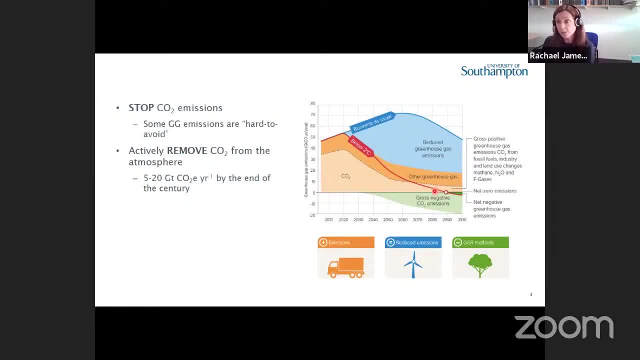 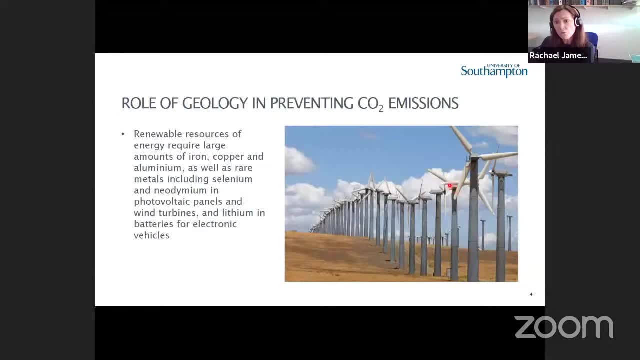 remove on the order of 5 to 20 gigatons, so that's billion tons of gigatons. so that's billion tons of gigatons. so that's billion tons of carbon dioxide equivalents per year. carbon dioxide equivalents per year. carbon dioxide equivalents per year: uh. reducing carbon dioxide emissions. 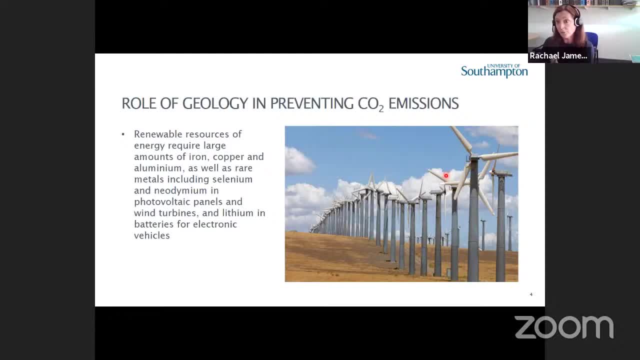 uh reducing carbon dioxide emissions- uh reducing carbon dioxide emissions, and secondly, in removing carbon dioxide, and secondly in removing carbon dioxide and secondly in removing carbon dioxide from the atmosphere, and that's really from the atmosphere, and that's really from the atmosphere, and that's really going to be the focus. 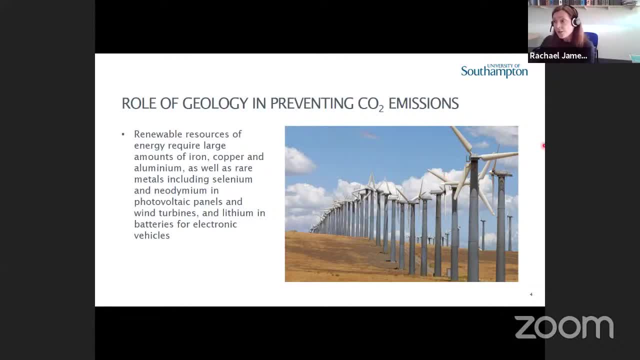 going to be the focus, going to be the focus of my talk today. so starting with the of my talk today, so starting with the of my talk today, so starting with the first of these: the role of geology in. first of these, the role of geology in. 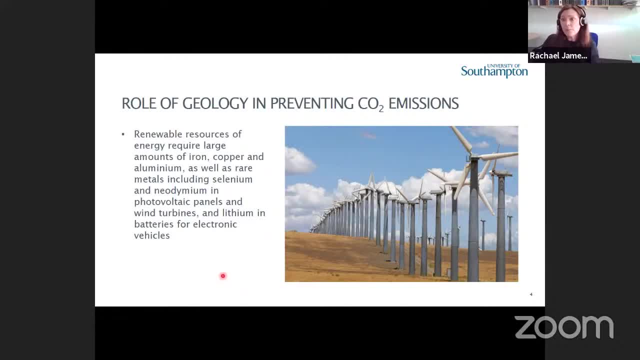 first of these, the role of geology in preventing carbon dioxide emissions. preventing carbon dioxide emissions. preventing carbon dioxide emissions. what we've got to remember is that. what we've got to remember is that what we've got to remember is that renewable sources of energy. renewable sources of energy. 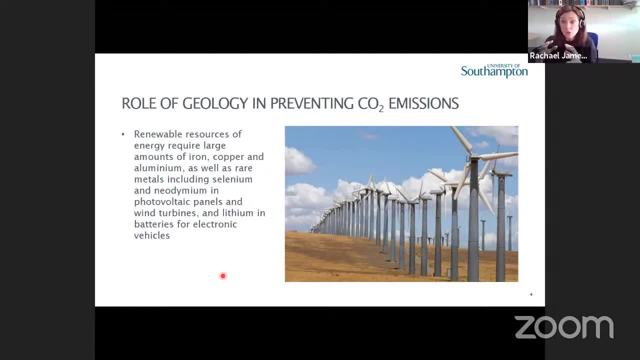 renewable sources of energy require huge quantities of metals. that require huge quantities of metals that geologists actually are really good at. geologists actually are really good at. geologists actually are really good at finding and extracting. so they're things. finding and extracting, so they're things. 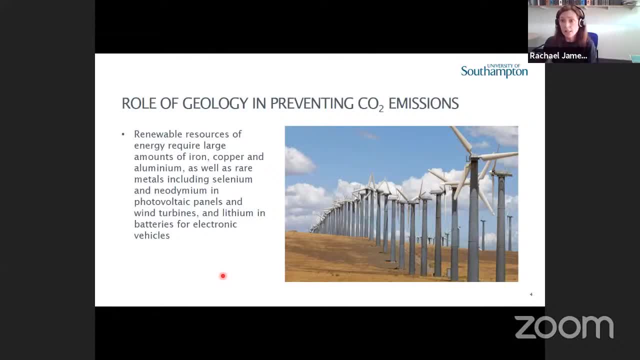 finding and extracting. so they're things like iron, copper and aluminium, which, like iron copper and aluminium, which, like iron, copper and aluminium, which we've been utilizing for for many, we've been utilizing for for many, we've been utilizing for for many thousands, uh, of years already. 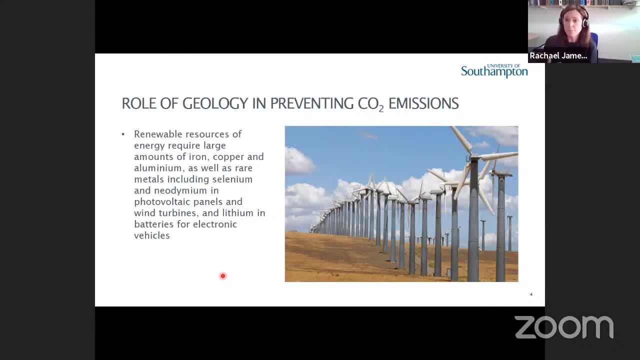 thousands uh of years already, thousands uh of years already. but renewable sources of energy also. but renewable sources of energy also. but renewable sources of energy also require other metal resources that may require other metal resources, that may require other metal resources that may be much, much harder to find. 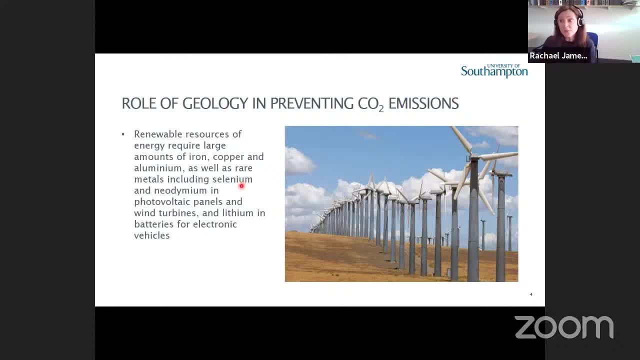 be much, much harder to find, be much, much harder to find, and they include things like rare earth and they include things like rare earth and they include things like rare earth elements, rare metals, elements rare metals, including selenium and neodymium, and we, including selenium and neodymium and we. 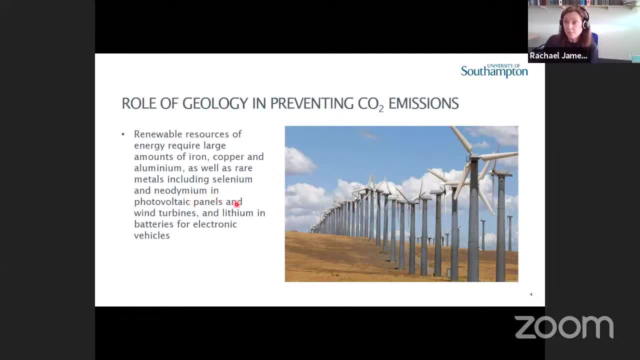 including selenium and neodymium, and we need those for photovoltaic panels and need those for photovoltaic panels and need those for photovoltaic panels, and we need them in wind turbines, we need them in wind turbines, we need them in wind turbines and we also need the element lithium and 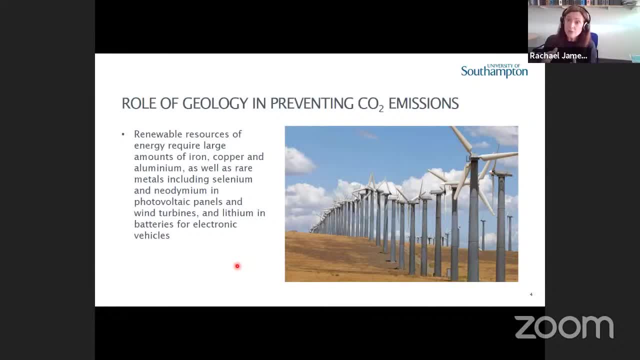 and we also need the element lithium, and, and we also need the element lithium, and many of you are aware that that's a key. many of you are aware that that's a key. many of you are aware that that's a key component of the batteries for electronic. 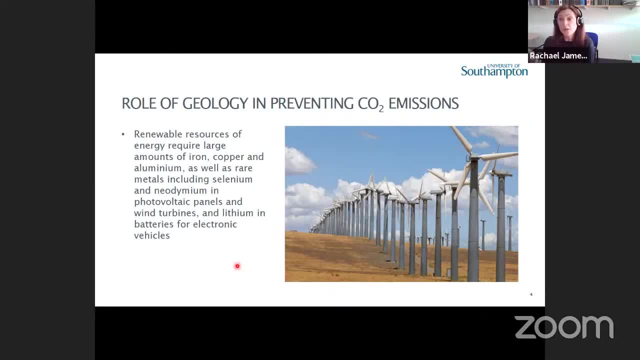 component of the batteries for electronic, component of the batteries for electronic vehicles, but it's also required for vehicles. but it's also required for vehicles. but it's also required for batteries for other types of energy, batteries for other types of energy, batteries for other types of energy storage as well. 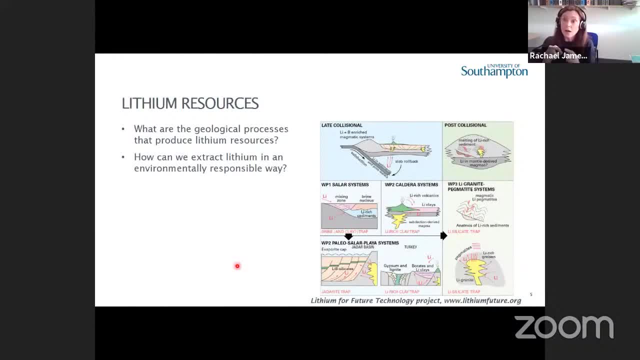 so lithium is is a key topic. uh of so lithium is is a key topic. uh of so, lithium is is a key topic. uh of research at the moment for finding new research at the moment, for finding new research at the moment for finding new resources, and it's been known for some. 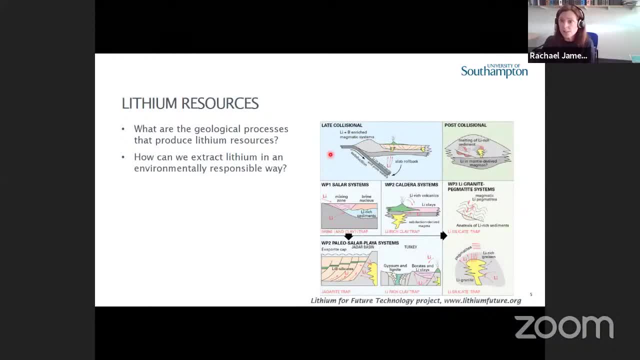 resources and it's been known for some resources and it's been known for some time now. geologists have known that many time now. geologists have known that many time now. geologists have known that many lithium deposits are associated with lithium deposits are associated with. lithium deposits are associated with subduction zone processes. so that's when 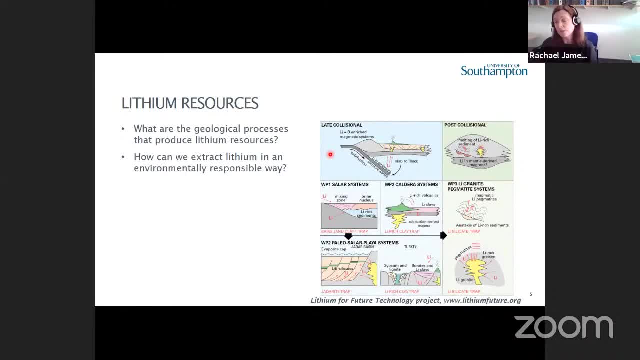 subduction zone processes. so that's when. subduction zone processes, so that's when the uh, the uh, the uh. plates come together, plates come together, plates come together and subducted by underneath one another. and subducted by underneath one another and subducted by underneath one another. and we also know that lithium is quite 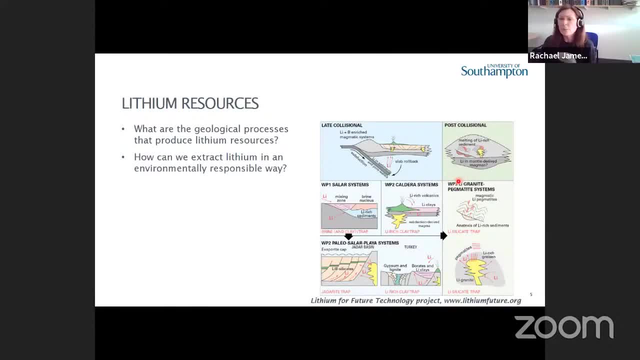 and we also know that lithium is quite and we also know that lithium is quite often found in what we call post, often found in what we call post, often found in what we call post collisional settings as well. but we collisional settings as well, but we 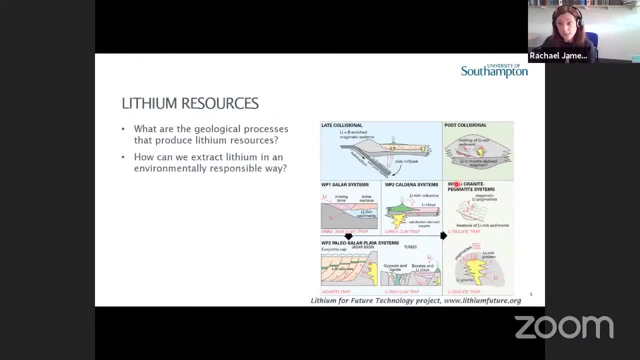 collisional settings as well, but we still don't really know, still don't really know, still don't really know, uh, what the source of lithium in those, uh, what the source of lithium in those, uh, what the source of lithium in those post-collisional settings is. 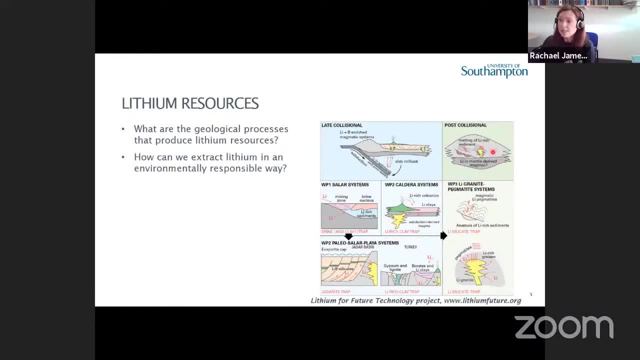 post-collisional settings is. post-collisional settings is: is it from lithium in mantle derived? is it from lithium in mantle derived? is it from lithium in mantle derived magmas, or is it melting of lithium from magmas, or is it melting of lithium from? 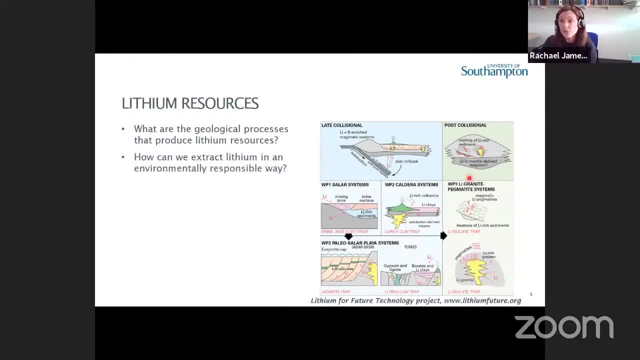 magmas or is it melting of lithium from lithium rich sediments? lithium rich sediments- lithium rich sediments. the other key issue is: how do geologists? the other key issue is: how do geologists? the other key issue is: how do geologists can contribute to is how we extract. 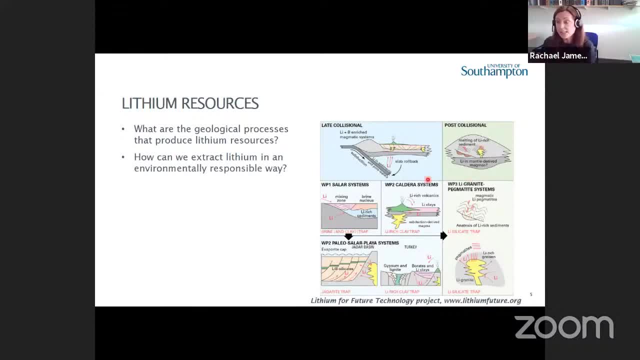 can contribute to is how we extract, can contribute to is how we extract those resources including lithium in an, those resources including lithium in an, those resources including lithium in an environmentally sustainable way, environmentally sustainable way, environmentally sustainable way. and for those of you who think that, and for those of you who think that, 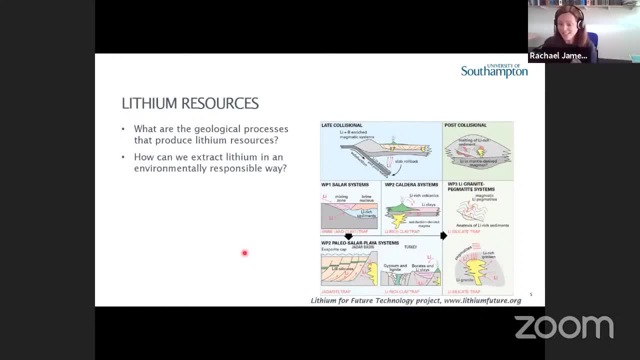 and for those of you who think that geology is kind of an old topic and we, geology is kind of an old topic and we geology is kind of an old topic and we, we never find anything new. i just want we never find anything new, i just want. 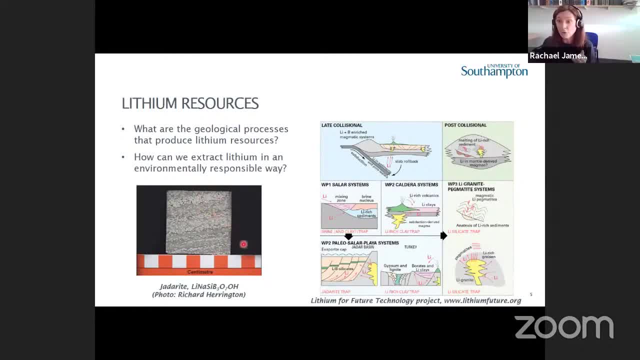 we never find anything new. i just want to point out that this rather uh, to point out that this rather uh, to point out that this rather uh beautiful mineral here, jade right. beautiful mineral here, jade right. beautiful mineral here, jade right. that's the light parts that we can see. 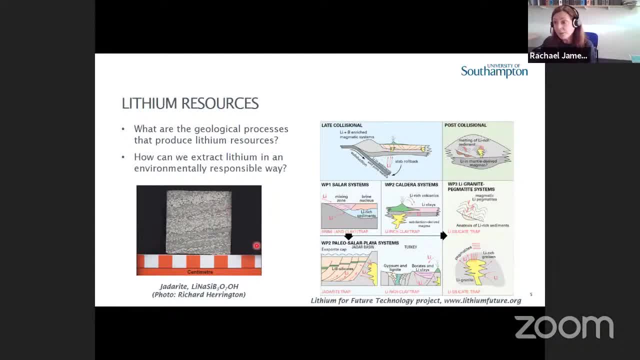 that's the light parts that we can see. that's the light parts that we can see here, here, here it's a lithium sodium borate mineral. it's a lithium sodium borate mineral. it's a lithium sodium borate mineral, and that was actually only discovered. 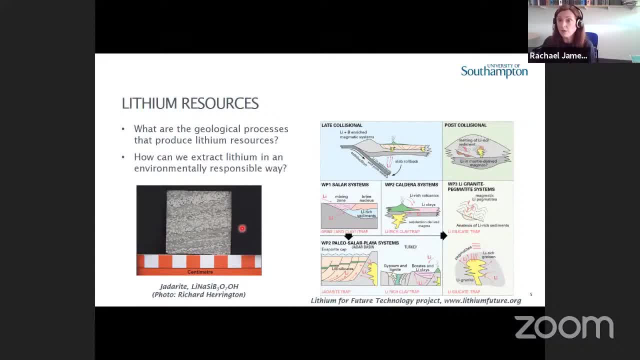 and that was actually only discovered. and that was actually only discovered in 2004. so those resources are out there in 2004. so those resources are out there in 2004. so those resources are out there. we just need to to find more of them. 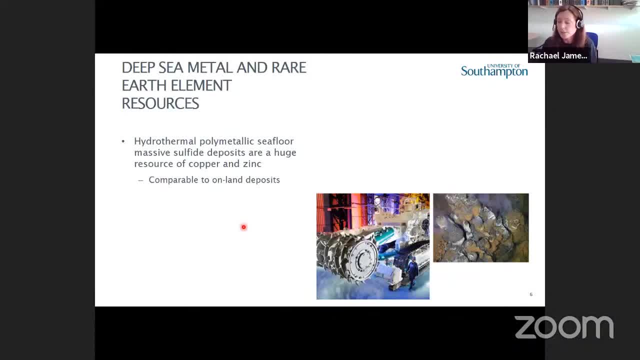 we just need to to find more of them. we just need to to find more of them, and as geologists as well, we're also, and as geologists as well, we're also, and as geologists as well, we're also increasingly looking to the deep oceans. 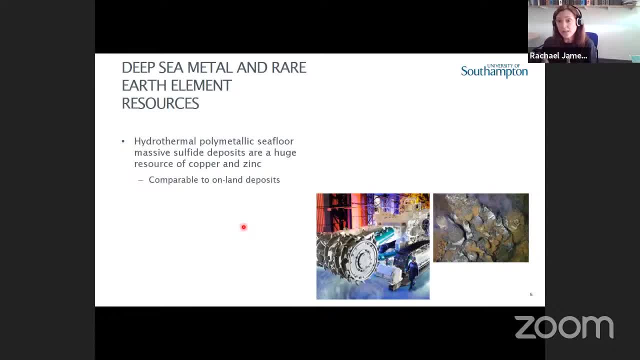 increasingly looking to the deep oceans, increasingly looking to the deep oceans to find new sources of these rare earth, to find new sources of these rare earth, to find new sources of these rare earth: elements, elements, elements and other rare metals and for example, and other rare metals and for example. 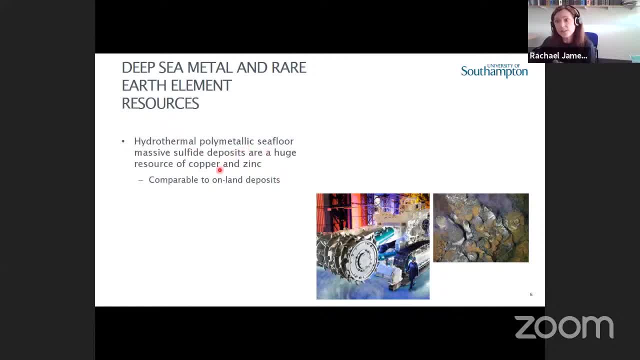 and other rare metals and, for example, uh, uh uh hydrothermal deposits that we find at sea. hydrothermal deposits that we find at sea. hydrothermal deposits that we find at sea, floor, floor, floor. we get these massive sulfide deposits. we get these massive sulfide deposits. 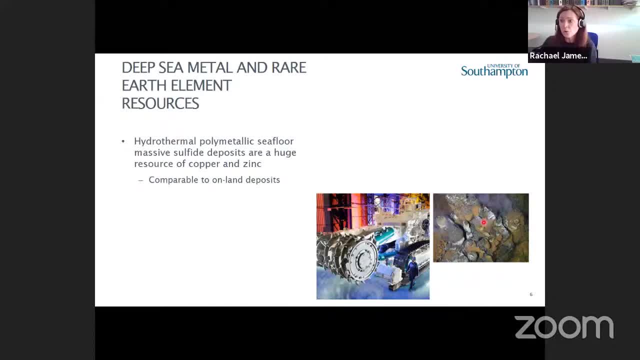 we get these massive sulfide deposits forming in these hydrothermal settings, forming in these hydrothermal settings, forming in these hydrothermal settings, and they're a huge resource of copper and they're a huge resource of copper and they're a huge resource of copper and zinc. we still don't even really. 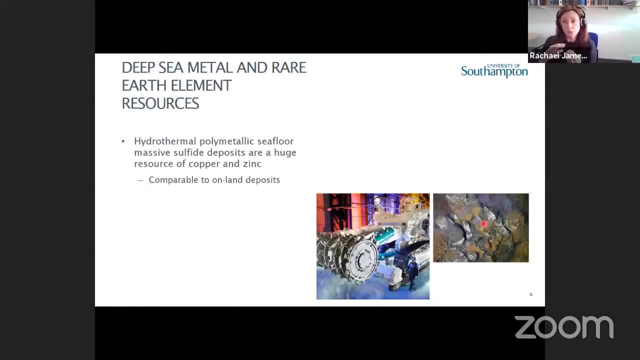 and zinc, we still don't even really. and zinc we still don't even really know how much. because a lot of know how much, because a lot of know how much, because a lot of hydrothermal deposits are in fact hydrothermal deposits, are in fact hydrothermal deposits, are in fact extinct now and deeply buried under. 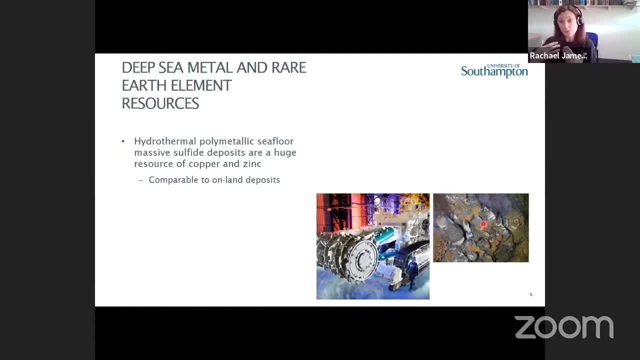 extinct now and deeply buried under extinct now and deeply buried under ocean sediments, and we're finding new ocean sediments, and we're finding new ocean sediments and we're finding new ways, ways, ways, uh to seismically image those, and hence uh to seismically image those, and hence. 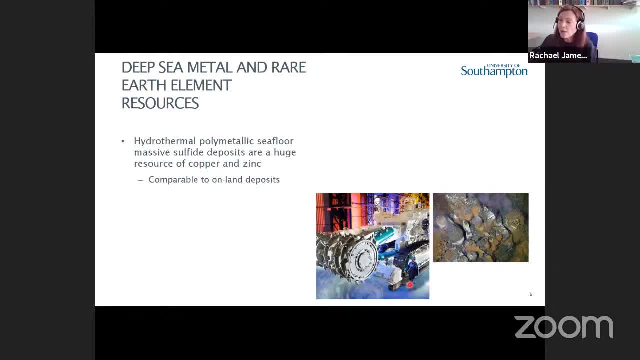 uh, to seismically image those and hence discover them, discover them, discover them, and some of you may be aware that that, and some of you may be aware that that, and some of you may be aware that that some companies, for example nautilus, some companies, for example nautilus. 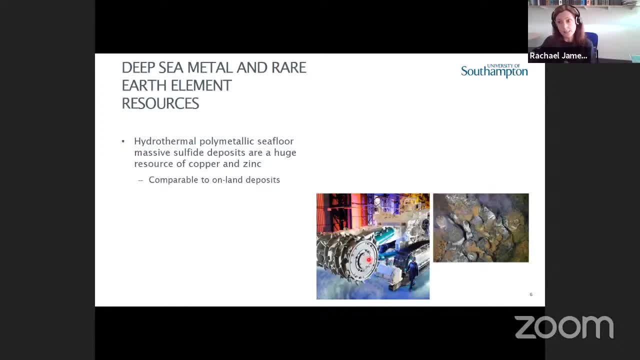 some companies, for example, nautilus minerals, minerals minerals uh have been developing techniques to uh have been developing techniques to? uh have been developing techniques to mine these um sulfides in in the deep mine, these um sulfides in in the deep mine, these um sulfides in in the deep ocean. so thousands of meters of water. 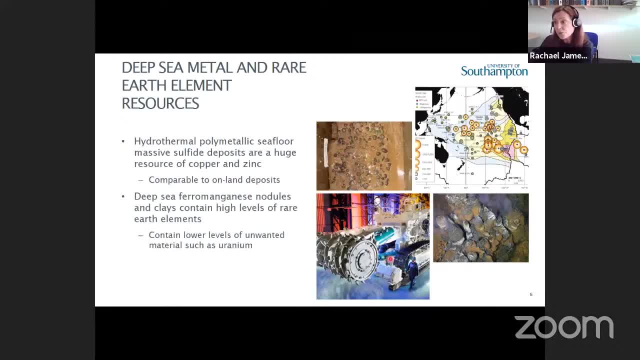 ocean. so thousands of meters of water ocean. so thousands of meters of water depth, depth, depth in a deep ocean as well. we also have in a deep ocean as well. we also have in a deep ocean as well. we also have other metal resources, other metal resources, other metal resources. uh, here i've got some manganese nodules. 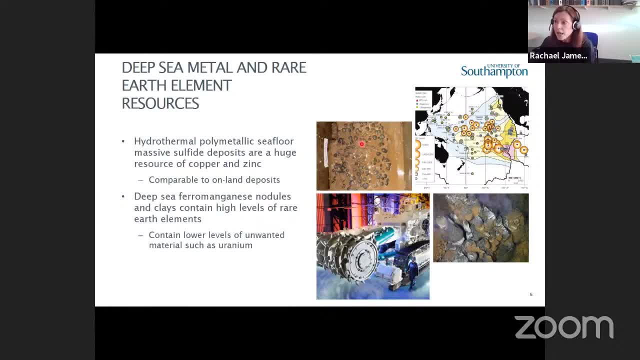 uh, here i've got some manganese nodules. uh, here i've got some manganese nodules which are found in the very, very deepest, which are found in the very, very deepest, which are found in the very, very deepest parts of the ocean basins. parts of the ocean basins. 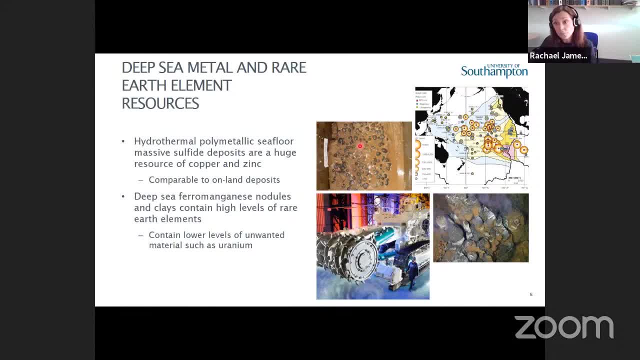 parts of the ocean basins and they're a big resource of uh uh and they're a big resource of uh uh and they're a big resource of uh uh. metals such as cobalt as well as iron, metals such as cobalt as well as iron. 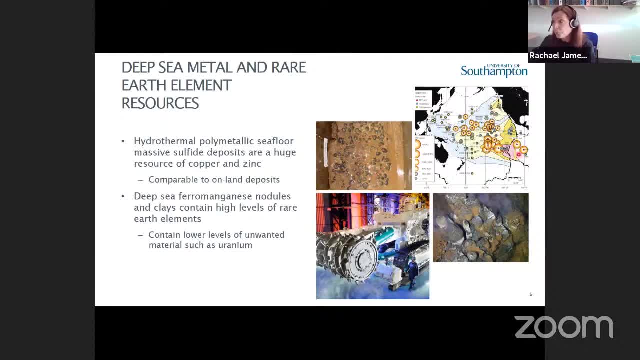 metals such as cobalt, as well as iron and manganese and manganese and manganese and the rare earth elements too, and the rare earth elements too, and the rare earth elements too, and also clay-rich sediments again in, and also clay-rich sediments again in, and also clay-rich sediments again in those deep ocean basins. they turn it. 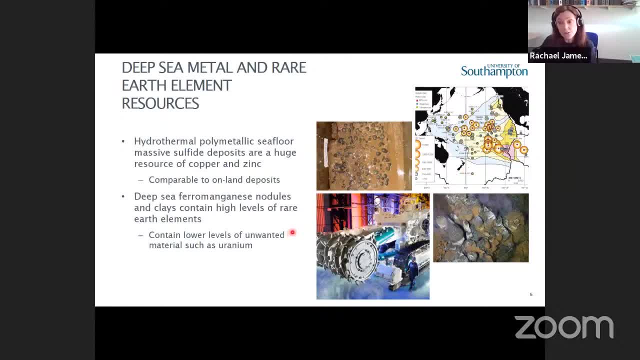 those deep ocean basins, they turn it. those deep ocean basins, they turn it. turns out that they have extremely high. turns out that they have extremely high. turns out that they have extremely high levels of the rare earth elements. that levels of the rare earth elements that. 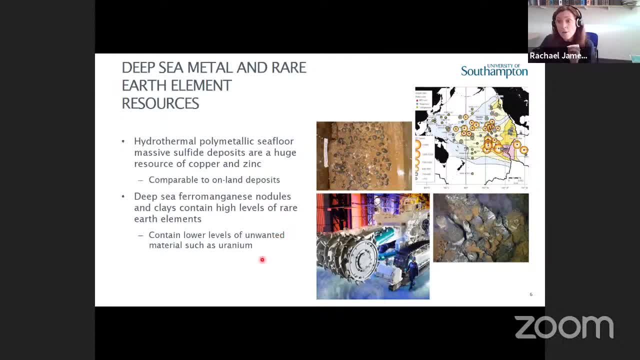 levels of the rare earth elements that are needed for those for, are needed for those for, are needed for those for voltaic cells, voltaic cells, voltaic cells- and the good thing about those is they, and the good thing about those is they, and the good thing about those is they actually contain much. 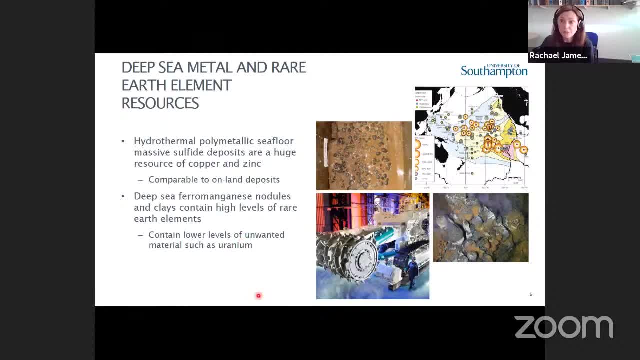 actually contain much, actually contain much lower levels of unwanted materials, such lower levels of unwanted materials, such lower levels of unwanted materials such as uranium, for example, as uranium, for example, as uranium, for example, that most rare earth element deposits on that most rare earth element deposits on that most rare earth element deposits on land. 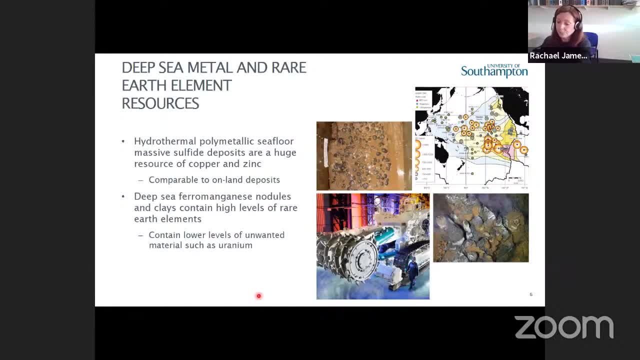 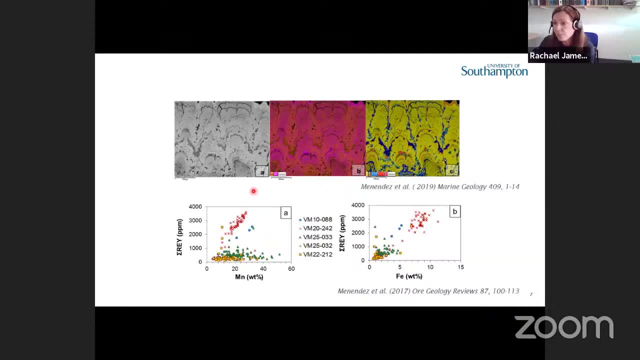 land, land also have high quantities of, also have high quantities of, also have high quantities of. of course, not all um mineral deposits. of course not all um mineral deposits. of course not all um mineral deposits are created equally, are created equally, are created equally. and this is some work that was done by a 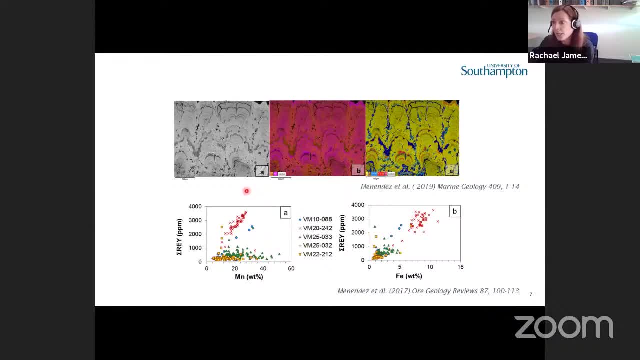 and this is some work that was done by a. and this is some work that was done by a phd student of mine, amaya. phd student of mine, amaya. phd student of mine, amaya menendez, a few years ago now, and this menendez a few years ago now, and this 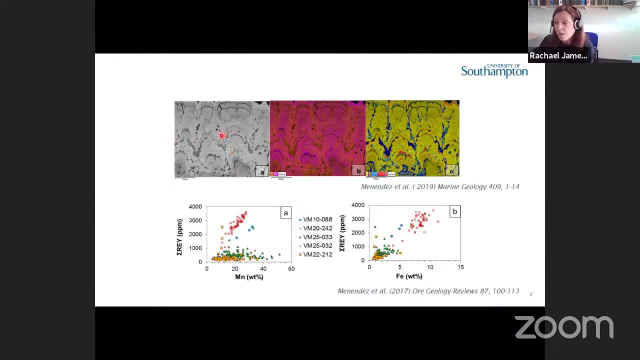 menendez, a few years ago now, and this shows a cross section, shows a cross section. shows a cross section through a manganese nodule, this back through a manganese nodule, this back through a manganese nodule, this back. scatter image here. scatter image here. scatter image here. shows regions of high reflectivity. 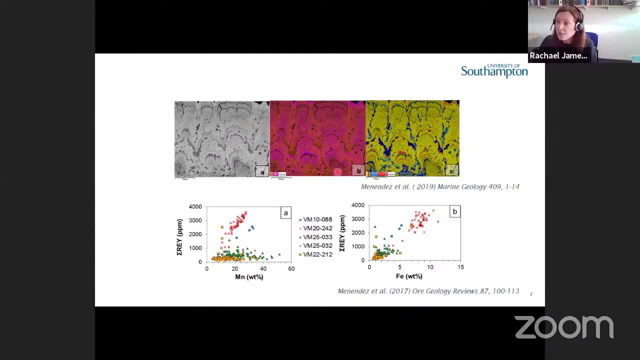 shows regions of high reflectivity, shows regions of high reflectivity, regions of low reflectivity, and if we do regions of low reflectivity and if we do regions of low reflectivity and if we do some elemental mapping, some elemental mapping, some elemental mapping, uh, of this manganese nodule, the orange. 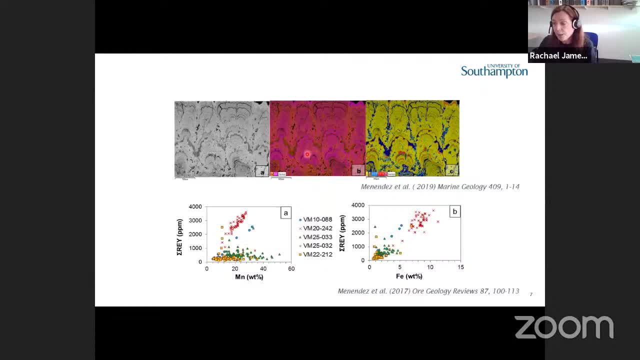 uh of this manganese nodule, the orange uh of this manganese nodule, the orange areas: here are areas that are high in areas. here are areas that are high in areas. here are areas that are high in iron, whereas the purple areas the pinky iron. whereas the purple areas, the pinky. 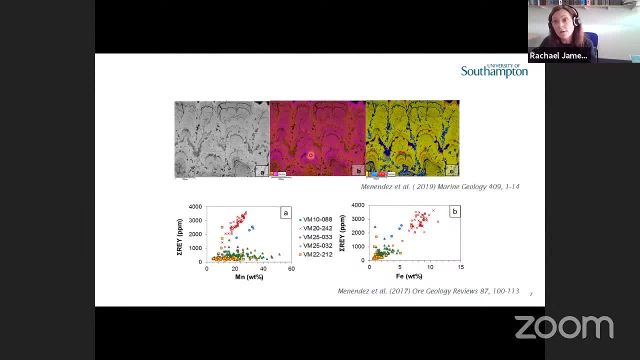 iron, whereas the purple areas, the pinky purple areas, purple areas are areas of the nodule that are high, are areas of the nodule that are high, are areas of the nodule that are high in manganese, in manganese, in manganese and if we look at the rare earth element, 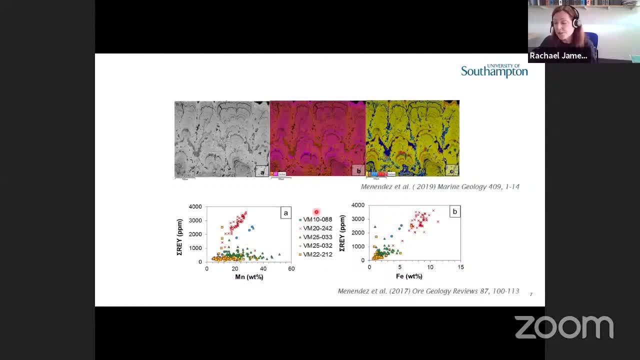 and if we look at the rare earth element, and if we look at the rare earth element, content, content, content of those different iron and manganese rich, of those different iron and manganese rich of those different iron and manganese rich, regions of the knot, regions of the knot, regions of the knot, of the nodules, what we can see is there's 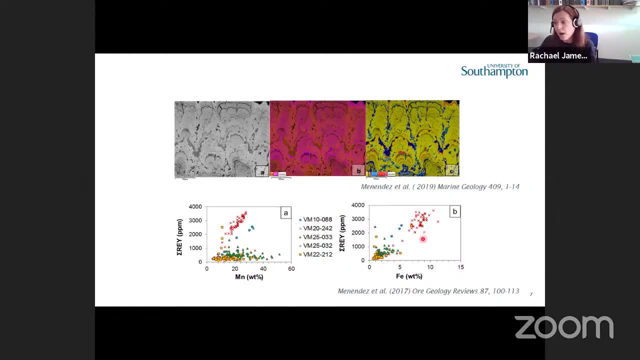 of the nodules. what we can see is there's of the nodules. what we can see is there's a very high con, a very high con, a very high con correlation between the iron contents of correlation between the iron contents of correlation between the iron contents of those layers within that nodule. 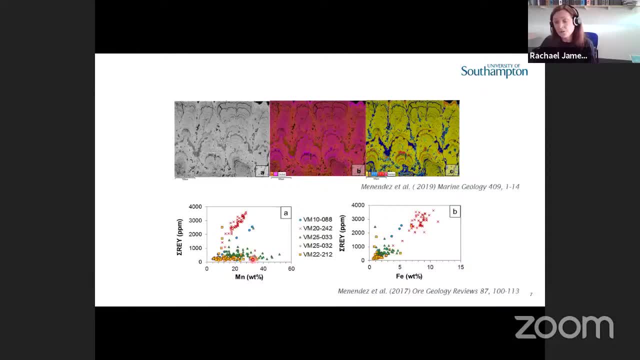 those layers within that nodule, those layers within that nodule, and the rare earth element content, but and the rare earth element content, but and the rare earth element content, but not so much of a relationship with, not so much of a relationship with, not so much of a relationship with manganese. 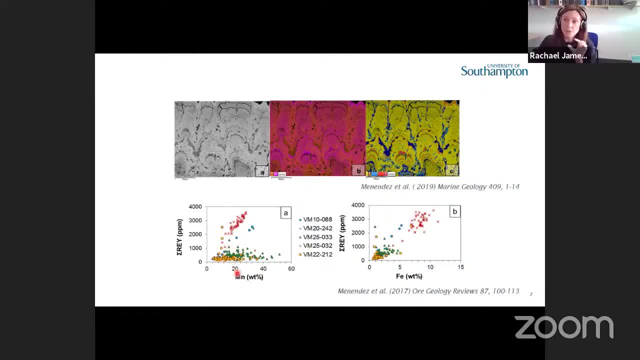 manganese, manganese. so again, our geological knowledge allows. so again, our geological knowledge allows. so again, our geological knowledge allows us to really us, to really us, to really target the areas that are going to target, the areas that are going to target the areas that are going to contain the the highest quantities of 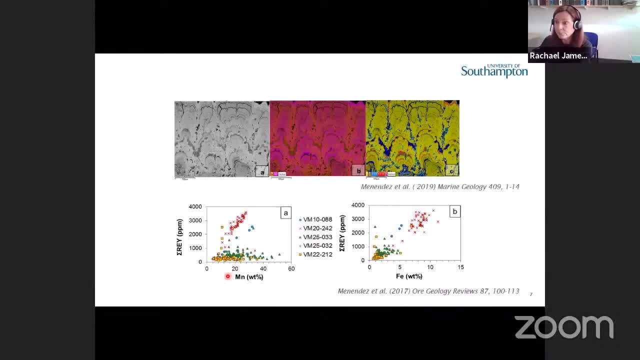 contain the, the highest quantities of. contain the: the highest quantities of the elements that we're most, the elements that we're most, the elements that we're most interested in. another area that geologists can, another area that geologists can, another area that geologists can contribute. 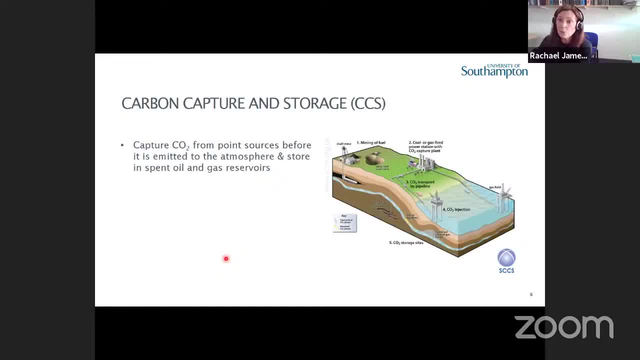 contribute. contribute to reducing carbon dioxide emissions is to reducing carbon dioxide emissions, is to reducing carbon dioxide emissions is through what we call carbon capture and through what we call carbon capture and through what we call carbon capture and storage, storage, storage. so this is where carbon dioxide is. 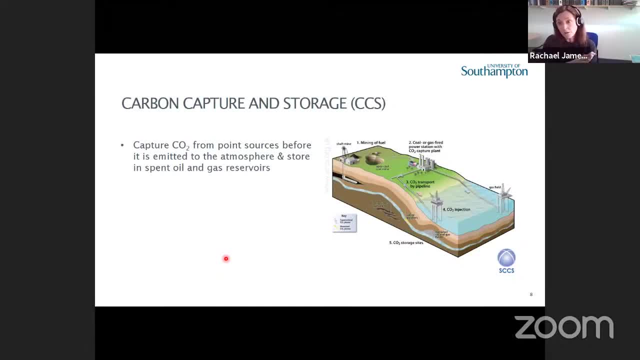 so this is where carbon dioxide is. so this is where carbon dioxide is captured from point sources. captured from point sources, captured from point sources. so power plants um cement manufacturing, so power plants um cement manufacturing, so power plants um cement manufacturing, that kind of thing, that kind of thing. 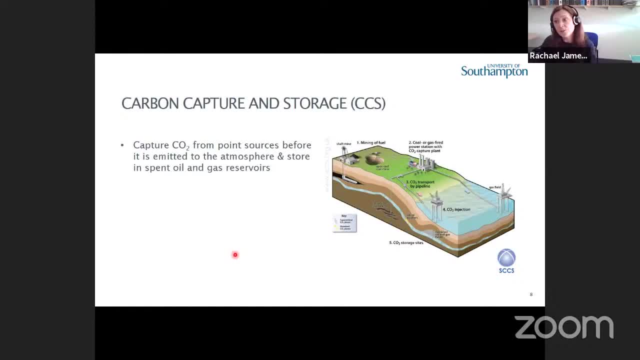 that kind of thing before it's emitted to the atmosphere, before it's emitted to the atmosphere, before it's emitted to the atmosphere, and then is stored in a variety of, and then is stored in a variety of, and then is stored in a variety of geological sequences. 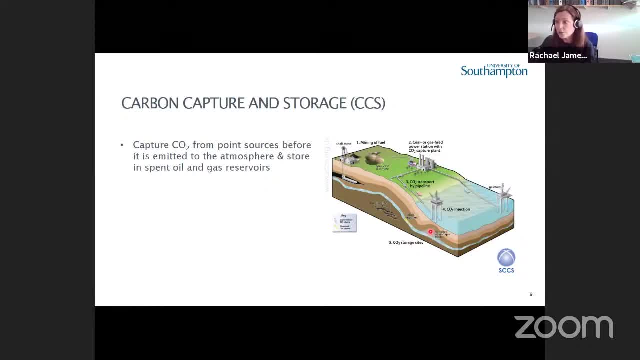 geological sequences. geological sequences including spent oil and gas fields. including spent oil and gas fields. including spent oil and gas fields under the oceans. unmineable coal seams under the oceans. unmineable coal seams under the oceans. unmineable coal seams. and also other projects too. 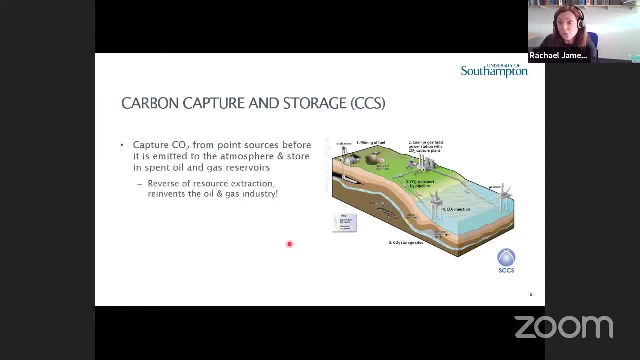 and so, really, this is sort of the and so, really, this is sort of the and so, really, this is sort of the reverse of the reverse of the reverse of the- uh, resource extraction industry- really, uh, resource extraction industry. really, uh, resource extraction industry. really, we're reinventing the oil and gas. 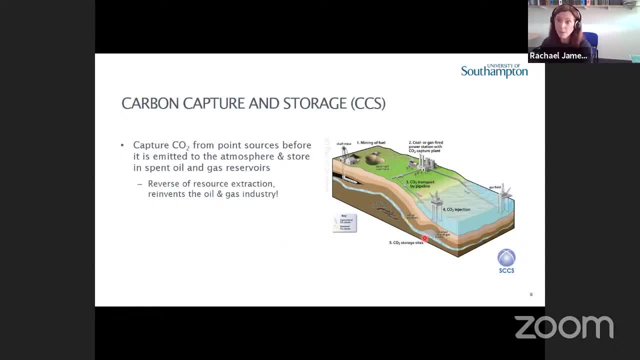 we're reinventing the oil and gas. we're reinventing the oil and gas industry instead of pulling things out industry. instead of pulling things out industry. instead of pulling things out of reservoirs, of reservoirs, of reservoirs, we're pumping carbon dioxide into them. we're pumping carbon dioxide into them. 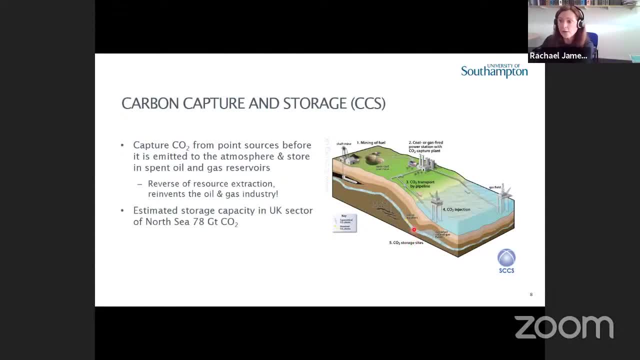 we're pumping carbon dioxide into them and the estimated storage capacity in and the estimated storage capacity in and the estimated storage capacity in the uk sector of the north sea is around the uk sector of the north sea is around. the uk sector of the north sea is around 78 gigatons of carbon dioxide. 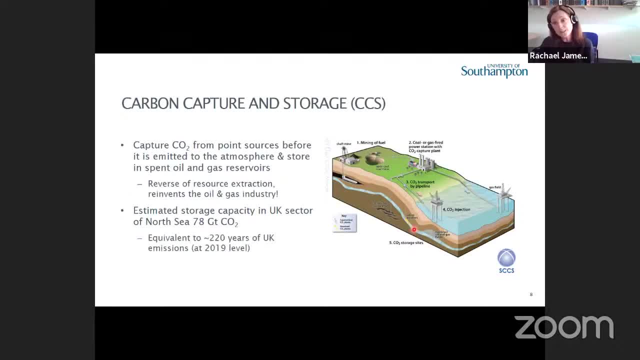 78 gigatons of carbon dioxide. 78 gigatons of carbon dioxide and to put that in context and to put that in context and to put that in context at the 2019 levels of co2 emissions, at the 2019 levels of co2 emissions. 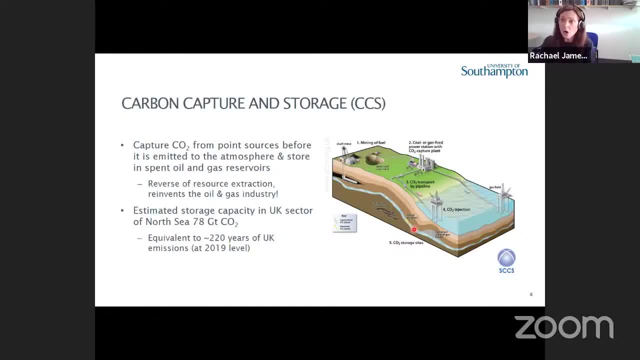 at the 2019 levels of co2 emissions from the uk. that's about 220 years from the uk. that's about 220 years from the uk. that's about 220 years worth of uk emissions and obviously as worth of uk emissions and obviously as. 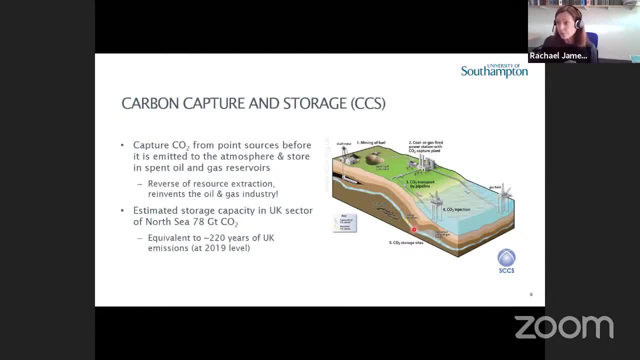 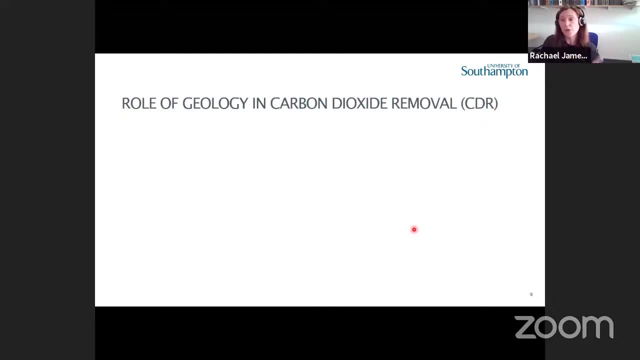 worth of uk emissions and, obviously, as emissions go down, emissions go down, emissions go down, that period is going to increase. so what, then, is the role of geology in? so what, then, is the role of geology in? so what, then, is the role of geology in the other part of my story, which is 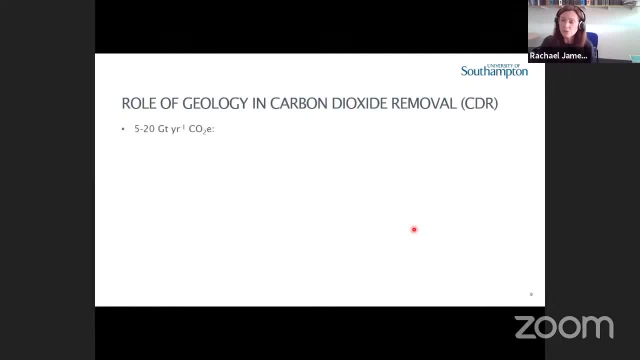 the other part of my story, which is the other part of my story, which is carbon dioxide removal, carbon dioxide removal, carbon dioxide removal. and i just want to remind you again, if, and i just want to remind you again, if, and i just want to remind you again, if we go back to those paris agreement. 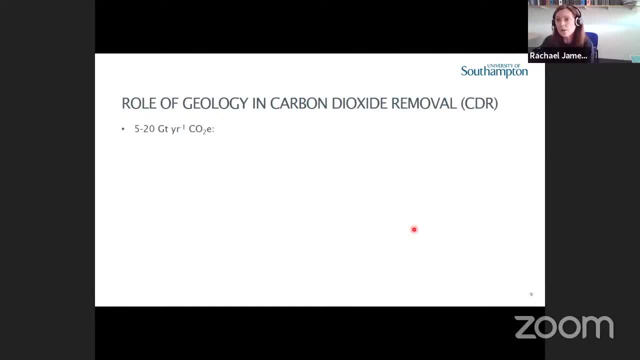 we go back to those paris agreement. we go back to those paris agreement targets that i discussed in the first targets, that i discussed in the first targets, that i discussed in the first slides. slides, slides. we're looking. what do we need to remove? we're looking, what do we need to remove? 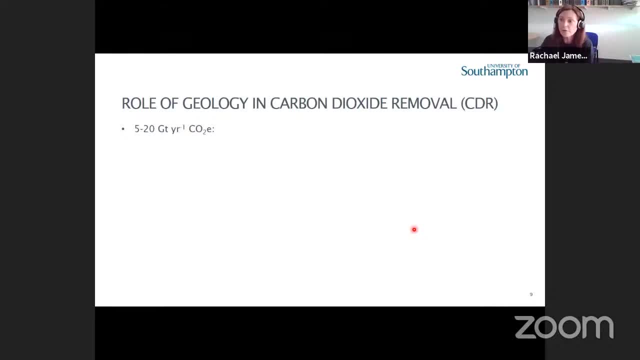 we're looking. what do we need to remove? we need to remove about. we need to remove about. we need to remove about five to 20 gigatons of carbon dioxide. five to 20 gigatons of carbon dioxide- five to 20 gigatons of carbon dioxide equivalent- per year. 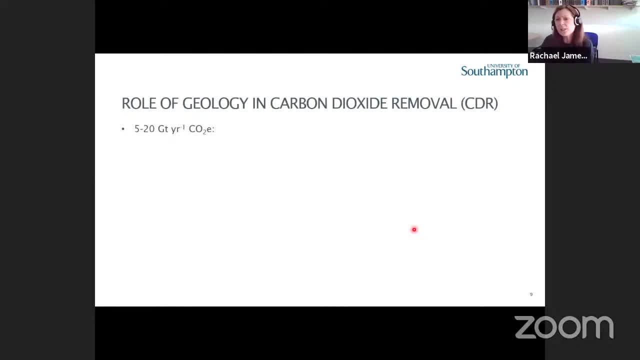 equivalent per year. equivalent per year in order to meet those paris agreement, in order to meet those paris agreement, in order to meet those paris agreement: targets, targets, targets. so what does this mean? this is a very us. so what does this mean? this is a very us. so what does this mean? this is a very us. uh, centered image. uh, because it comes. 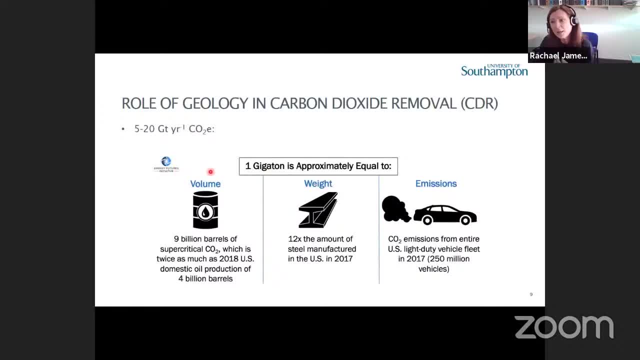 uh centered image. uh, because it comes. uh centered image? uh, because it comes from a us-based um, from a us-based um, from a us-based um think tank, but it's a gigaton of carbon think tank. but it's a gigaton of carbon think tank, but it's a gigaton of carbon dioxide. 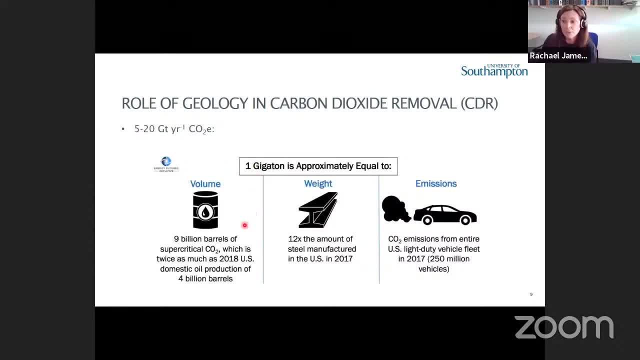 dioxide. dioxide is approximately equal to about nine. is approximately equal to about nine. is approximately equal to about nine billion barrels of supercritical carbon, billion barrels of supercritical carbon. billion barrels of supercritical carbon dioxide, or dioxide, or dioxide, or twice as much as the us. 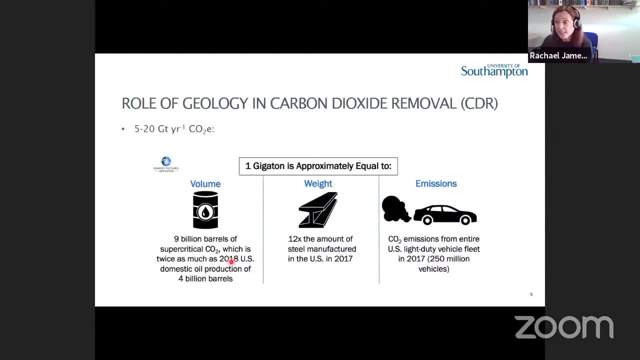 twice as much as the us. twice as much as the us production domestic production of oil production. domestic production of oil production: domestic production of oil. in 2018, it's equivalent to about 12. in 2018, it's equivalent to about 12. 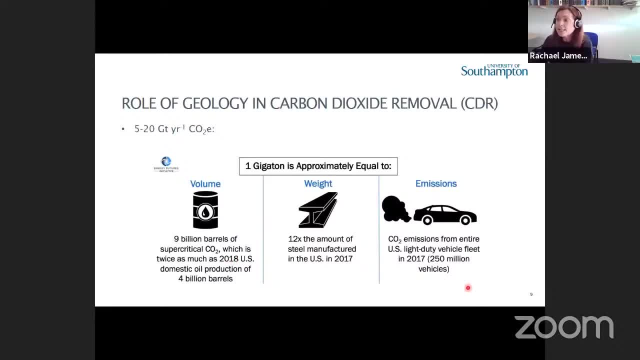 in 2018. it's equivalent to about 12 times the amount of steel manufactured in times the amount of steel manufactured in times the amount of steel manufactured in the us, the us, the us, and it's also the equivalent of removing, and it's also the equivalent of removing. 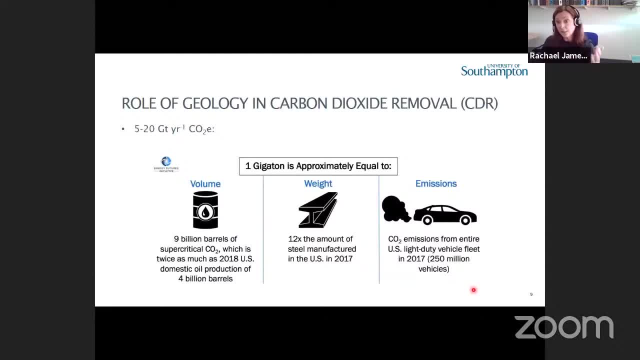 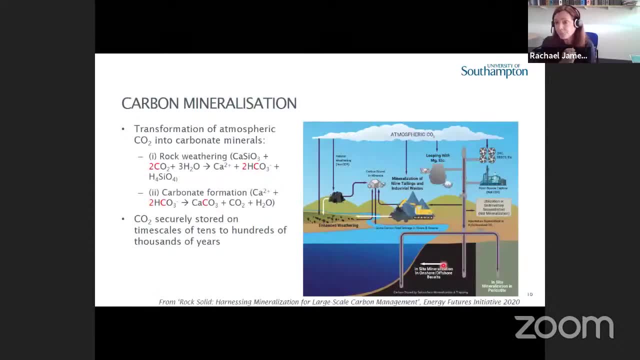 and it's also the equivalent of removing the entire, the entire, the entire uh light vehicle fleet from from the us uh light vehicle fleet from from the us uh light vehicle fleet from from the us. so this is a big challenge. so how can geologists contribute to this? 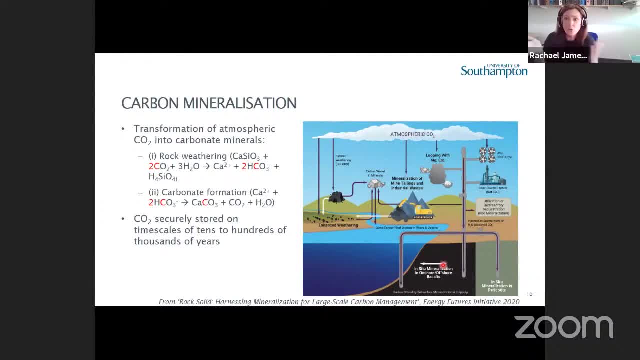 so how can geologists contribute to this? so, how can geologists contribute to this? well, i'm sure many of you will know. and well, i'm sure many of you will know. and well, i'm sure many of you will know, and you've discussed it, you've all looked. 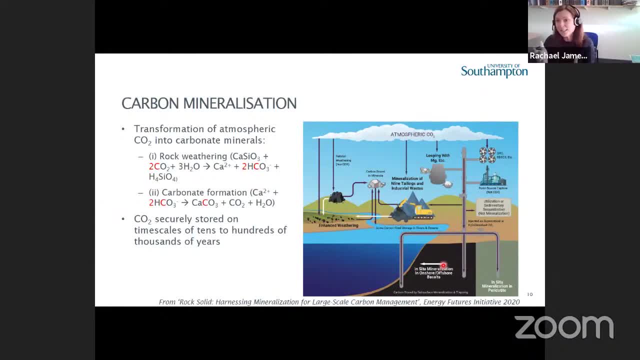 you've discussed it. you've all looked. you've discussed it, you've all looked at your foreign periphery. you've all at your foreign periphery. you've all at your foreign periphery. you've all looked at your carbonate rich, looked at your carbonate rich. looked at your carbonate rich, sediments, um. 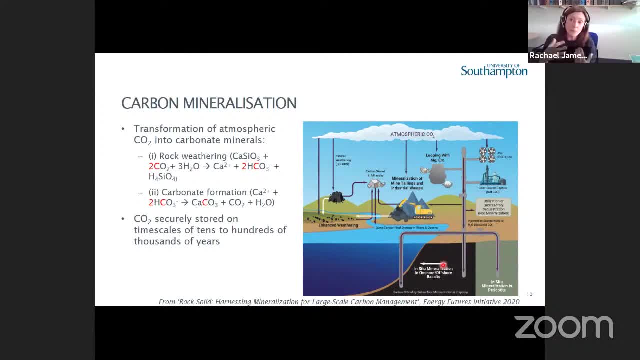 sediments um sediments, um but carbonates that we see in those but carbonates, that we see in those but carbonates that we see in those sediments and that we see in veins in sediments and that we see in veins in sediments and that we see in veins in rocks. 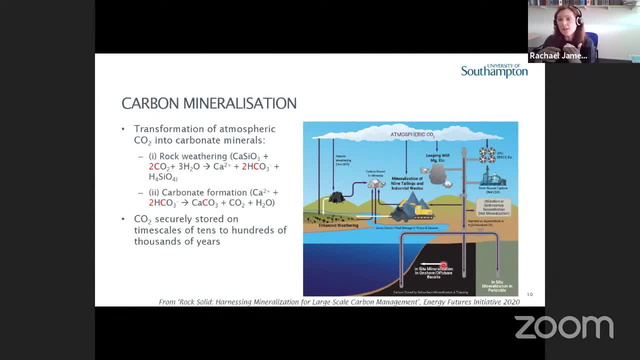 rocks. rocks actually comes from the atmosphere, actually comes from the atmosphere, actually comes from the atmosphere. and so this carbon mineralization, the, and so this carbon mineralization, the, and so this carbon mineralization, the conversion of carbon dioxide, conversion of carbon dioxide, conversion of carbon dioxide into carbonate rocks, is a natural process. 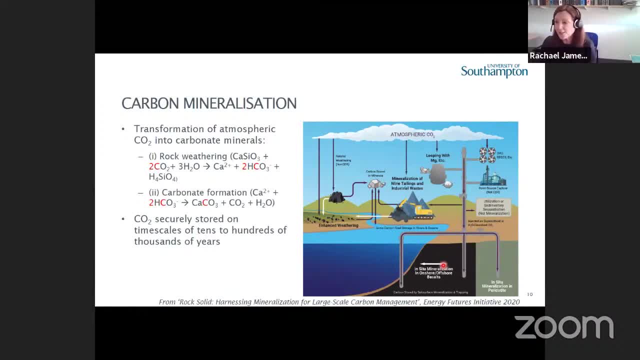 into carbonate rocks is a natural process. into carbonate rocks is a natural process. that's been going on for, for that's been going on for, for that's been going on for, for you know, since time immemorial and it's. you know, since time immemorial and it's. 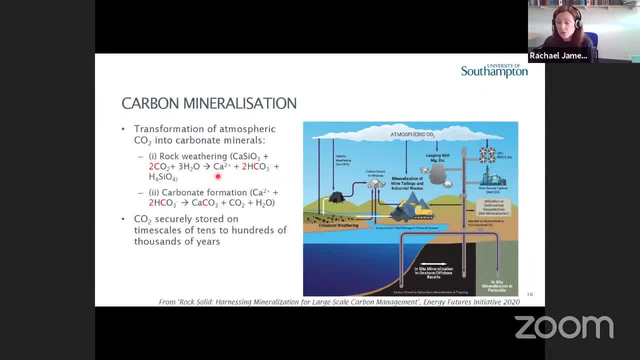 you know, since time immemorial, and it's carbonic acid, carbonic acid, carbonic acid, and the conversion of those rocks into, and the conversion of those rocks into, and the conversion of those rocks into divalent cations, so calcium ions and divalent cations, so calcium ions and 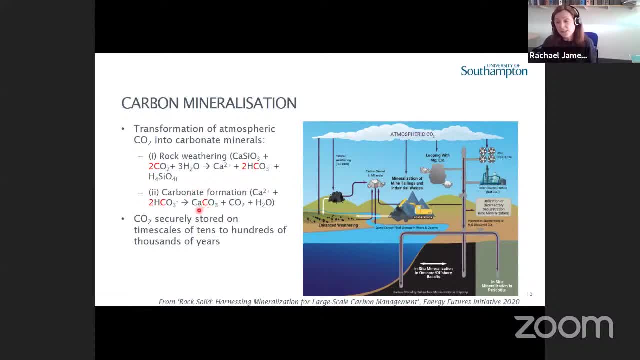 divalent cations, so calcium ions and magnesium ions, magnesium ions that are subsequently, that are subsequently, that are subsequently precipitate as carbonate minerals, precipitate as carbonate minerals, precipitate as carbonate minerals, and those carbonate minerals and those carbonate minerals and those carbonate minerals securely store that carbon dioxide on. 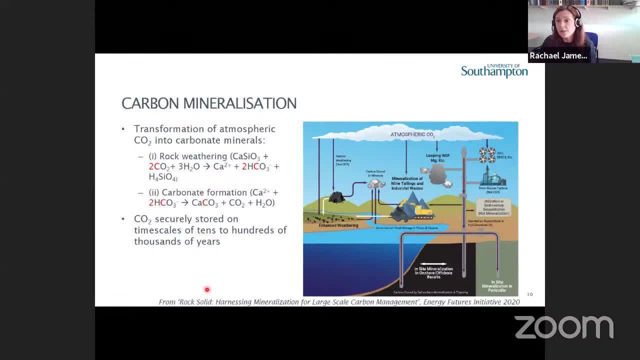 securely store that carbon dioxide on. securely store that carbon dioxide on time scales of tens to hundreds of time. scales of tens to hundreds of time. scales of tens to hundreds of thousands of years. so those carbonate thousands of years. so those carbonate thousands of years. so those carbonate minerals are very stable. 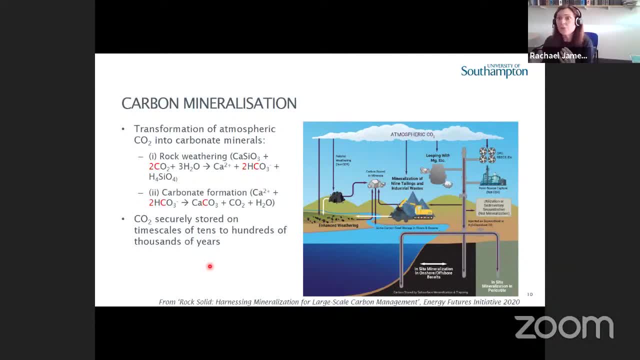 minerals are very stable. minerals are very stable, and uh an effective mechanism for, and uh an effective mechanism for, and uh an effective mechanism for removing carbon dioxide from the, removing carbon dioxide from the removing carbon dioxide from the atmosphere, atmosphere, atmosphere. the only issue is this overall process of 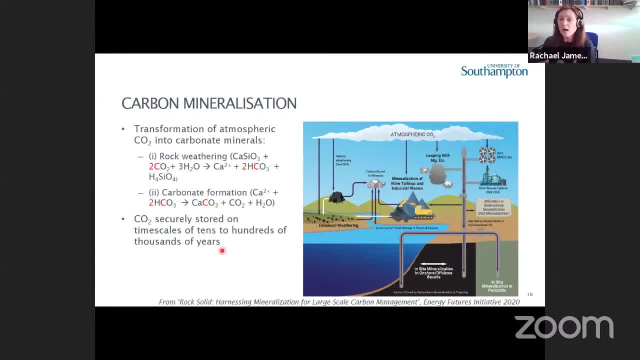 the only issue is this overall process, of. the only issue is this overall process of rock weathering a carbonate formation. rock weathering a carbonate formation. rock weathering a carbonate formation generally, um takes time, generally, um takes time, generally, um takes time. and remember that we need to uh start. 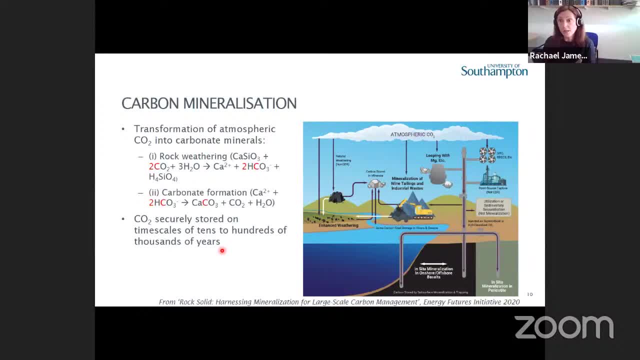 and remember that we need to uh start, and remember that we need to uh start removing significant quantities, of removing significant quantities, of removing significant quantities of atmospheric carbon dioxide by atmospheric carbon dioxide, by atmospheric carbon dioxide, by the end of the millennium. so, geologists, the end of the millennium, so geologists. 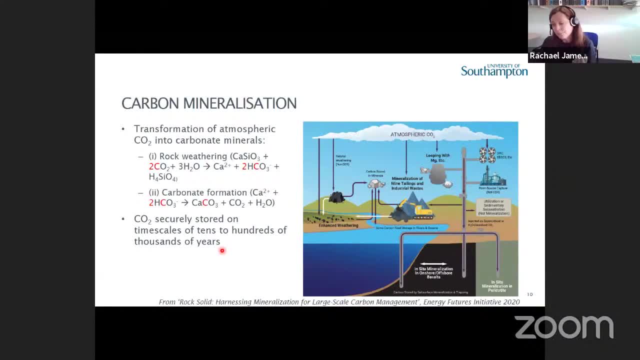 the end of the millennium. so geologists now are looking at ways in which we can now are looking at ways in which we can now are looking at ways in which we can speed this up, speed this up, speed this up. there are various different ways of doing. 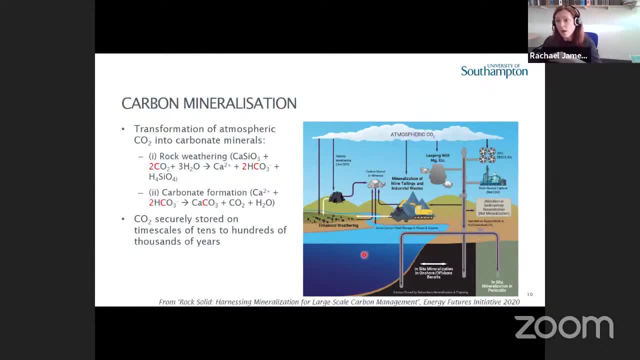 there are various different ways of doing. there are various different ways of doing this, which are this, which are this, which are summarized on this diagram here. i'm not summarized on this diagram here. i'm not summarized on this diagram here. i'm not going to go through all of these today. 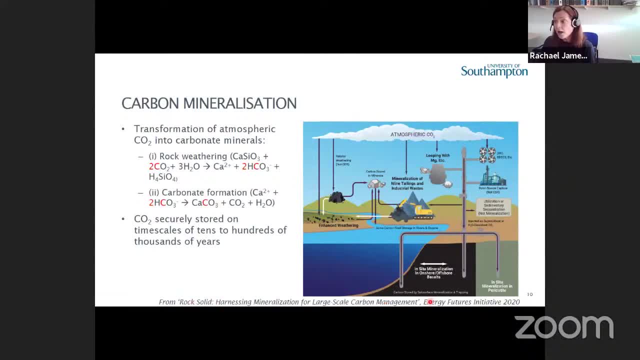 going to go through all of these today. going to go through all of these today. if you're interested, you can look at. if you're interested, you can look at. if you're interested, you can look at this recent, this recent, this recent report, uh, published by the energy. 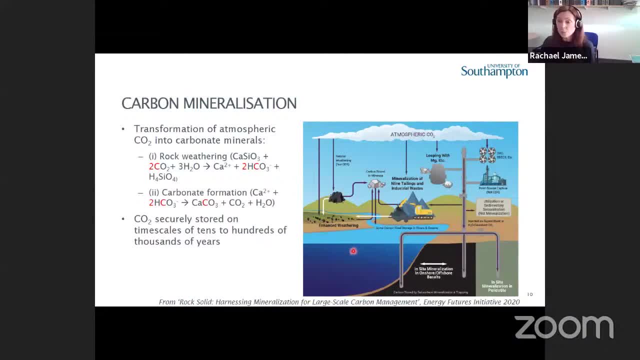 report: uh published by the energy report. uh published by the energy futures initiative: futures initiative, futures initiative. but there are different ways that we can, but there are different ways that we can, but there are different ways that we can try to speed that process. try to speed that process. 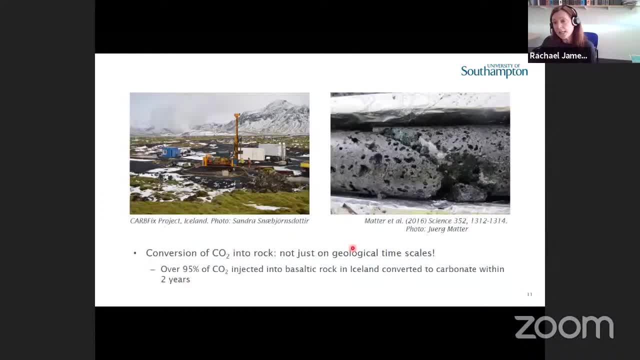 try to speed that process up. so one of these then up, so one of these then up. so one of these, then, is to take carbon dioxide and inject. it is to take carbon dioxide and inject. it is to take carbon dioxide and inject it into reactive, into reactive. 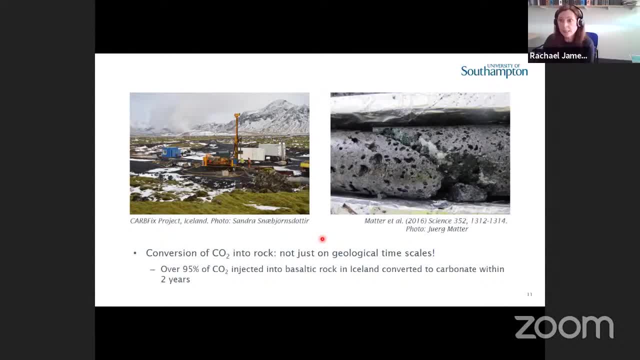 into reactive rocks that contain high quantities of rocks, that contain high quantities of rocks that contain high quantities of calcium and magnesium. calcium and magnesium, calcium and magnesium, ions- and this is uh a project called ions and this is uh a project called ions and this is uh a project called carb fix. that has been going on for a 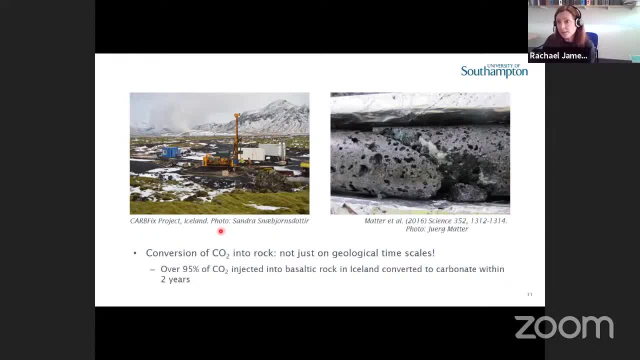 carb fix. that has been going on for a carb fix. that has been going on for a few years now, few years now, few years now in iceland that my colleague jörg matter in iceland, that my colleague jörg matter in iceland, that my colleague jörg matter at the university of southampton is. 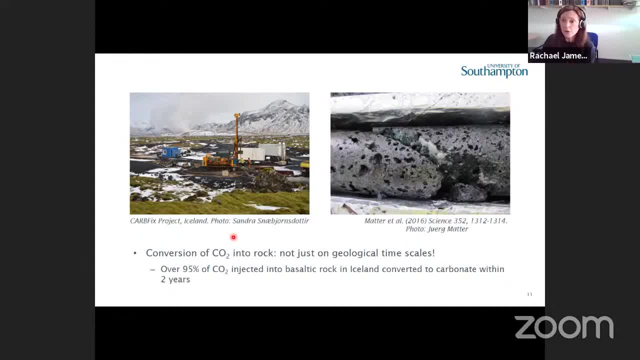 at the university of southampton is at the university of southampton, is involved in, involved in, involved in, and what they've done is they've taken and what they've done is they've taken and what they've done is they've taken carbon dioxide, carbon dioxide. 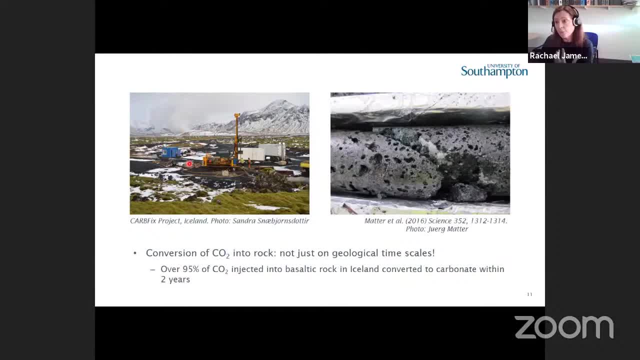 carbon dioxide. that would normally be released to the, that would normally be released to the, that would normally be released to the atmosphere as part of atmosphere, as part of atmosphere, as part of geothermal processing, and they've geothermal processing and they've geothermal processing and they've injected it. 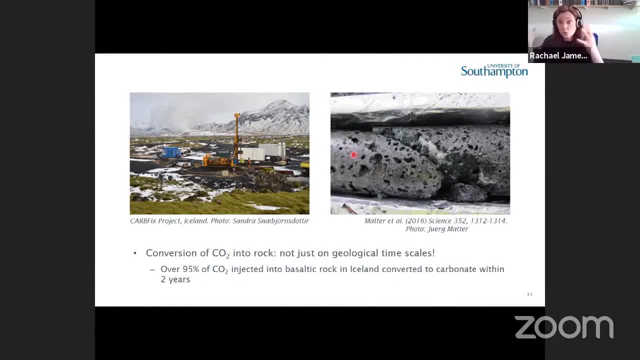 injected it. injected it into the basaltic rocks. that, of course, into the basaltic rocks. that, of course, into the basaltic rocks that, of course, form the island of iceland, form the island of iceland, form the island of iceland. and the surprising uh part of the story. 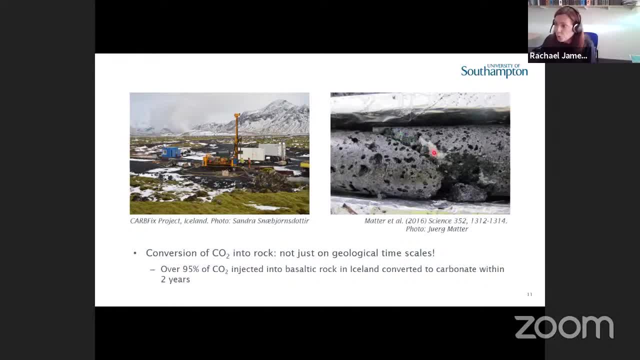 and the surprising uh part of the story. and the surprising uh part of the story here here. here you can see that these carbonate minerals, you can see that these carbonate minerals, you can see that these carbonate minerals are forming, are forming, are forming in the voids and fugs within those um. 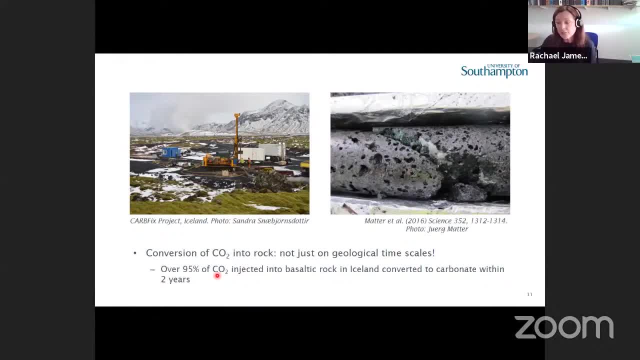 in the voids and fugs within those um. in the voids and fugs within those um basalts. is that over 95 percent basalts? is that over 95 percent basalts? is that over 95 percent of the carbon dioxide that was injected? 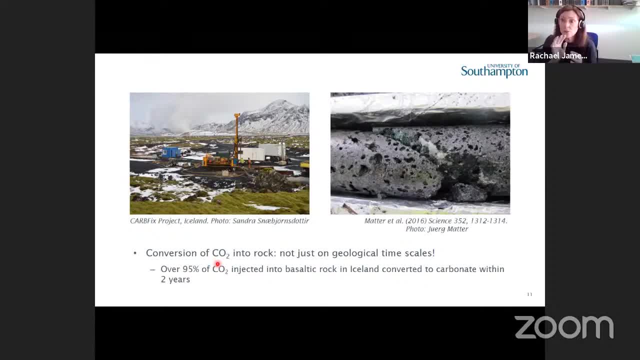 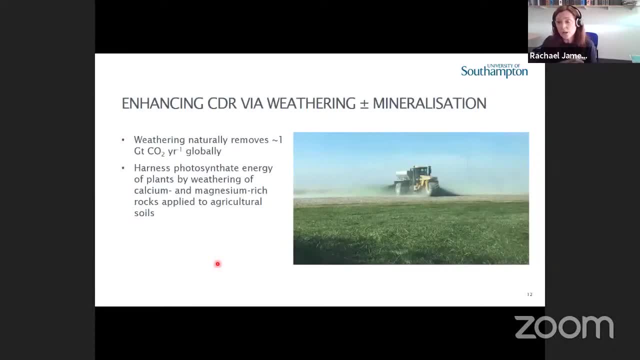 of the carbon dioxide that was injected, of the carbon dioxide that was injected into those basaltic rocks were converted into those basaltic rocks were converted into those basaltic rocks were converted to carbonate- to carbonate within two years, so extremely quickly. and the other um aspect that i wanted of 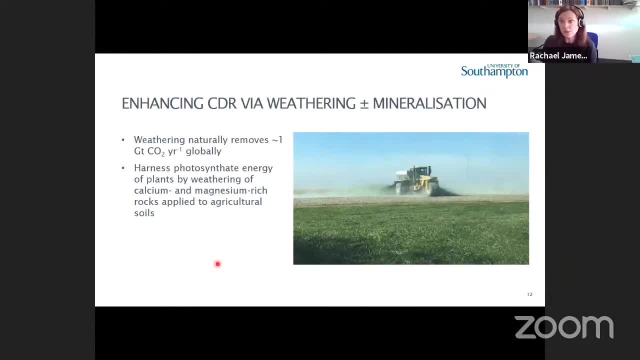 and the other um aspect that i wanted of, and the other um aspect that i wanted of, ways to speed up mineralization process, ways to speed up mineralization process, ways to speed up mineralization process and the weathering process too, that i, and the weathering process too, that i. 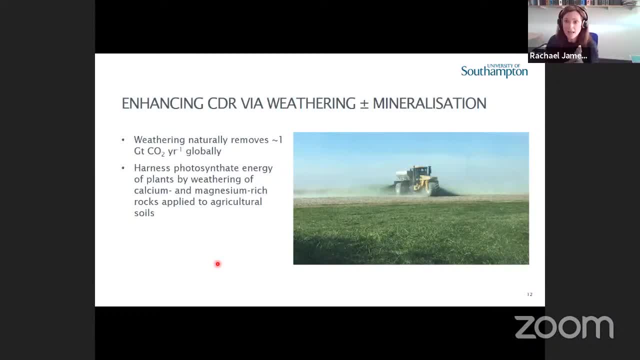 and the weathering process too, that i wanted to talk to you about today. uh wanted to talk to you about today. uh wanted to talk to you about today, uh, principally because it's an area of principally, because it's an area of principally because it's an area of active research of mine and my team. 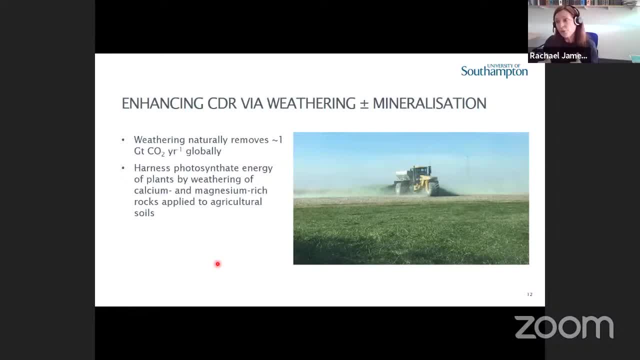 active research of mine and my team- active research of mine and my team- in southampton is carbon dioxide in southampton is carbon dioxide in southampton is carbon dioxide removal via removal via removal via enhanced weathering and mineralization. enhanced weathering and mineralization. so remember that that weathering process. 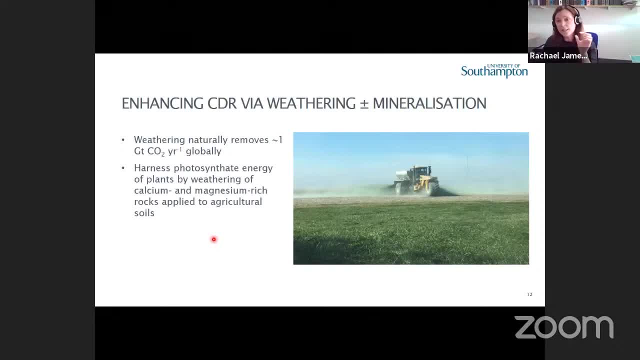 so remember that, that weathering process, so remember that, that weathering process. so the conversion, so the conversion, so the conversion of atmospheric carbon dioxide into of atmospheric carbon dioxide, into of atmospheric carbon dioxide, into carbonic acid, and then that carbonic carbonic acid, and then that carbonic. 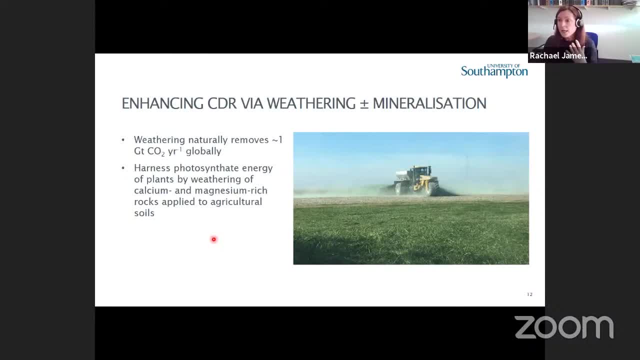 carbonic acid and then that carbonic acid acid acid attacks rocks at the earth's surface, attacks rocks at the earth's surface, attacks rocks at the earth's surface. that naturally removes about a gigaton. that naturally removes about a gigaton. that naturally removes about a gigaton of carbon dioxide. 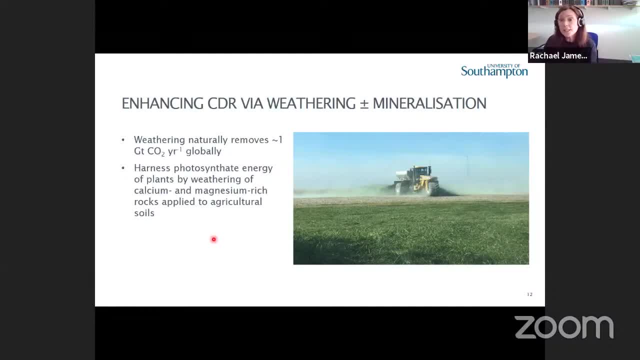 of carbon dioxide, of carbon dioxide per year globally. so the idea per year globally so, the idea per year globally. so the idea to speed this process up, to speed this process up, to speed this process up, is to apply crushed up calcium and is to apply crushed up calcium and 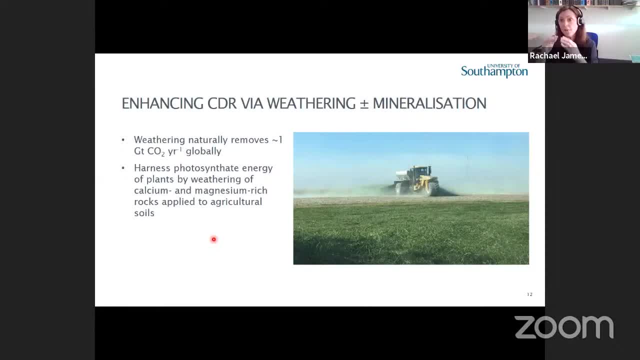 is to apply crushed up calcium and magnesium rich rocks to agricultural magnesium rich rocks to agricultural magnesium rich rocks to agricultural soils and then to harness the soils, and then to harness the soils and then to harness the photosynthate energy of plants to do the photosynthate energy of plants, to do the. 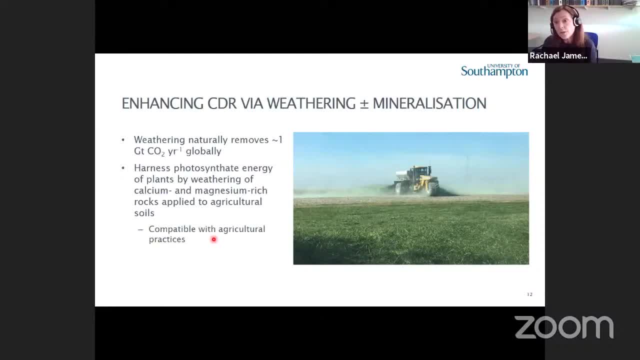 photosynthate energy of plants to do the weathering reaction for us. weathering reaction for us. weathering reaction for us. good thing about this is it's good thing about this is it's good thing about this is it's compatible with agricultural practices- compatible with agricultural practices. 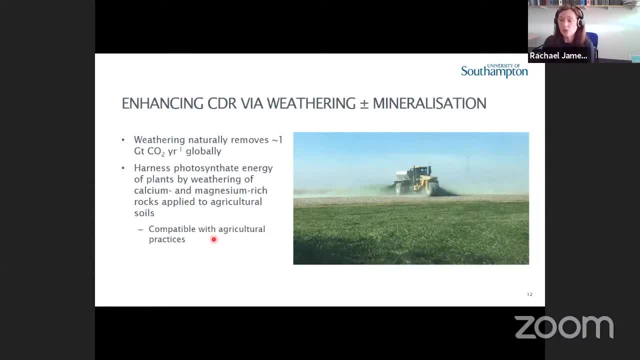 compatible with agricultural practices. farmers are well used to spreading. farmers are well used to spreading. farmers are well used to spreading fertilizers and lime etc all over their fertilizers and lime etc all over their fertilizers and lime etc all over their soils, soils, soils, and there are also potential co-benefits. 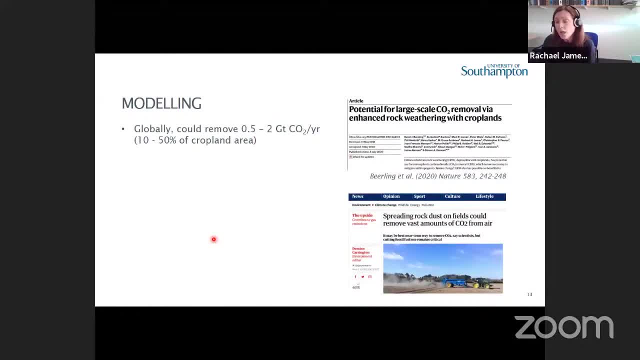 and there are also potential co-benefits, and there are also potential co-benefits for agriculture as well, for agriculture as well, for agriculture as well. so early work on this. uh has mainly so early work on this. uh has mainly so early work on this. uh has mainly focused on modeling. 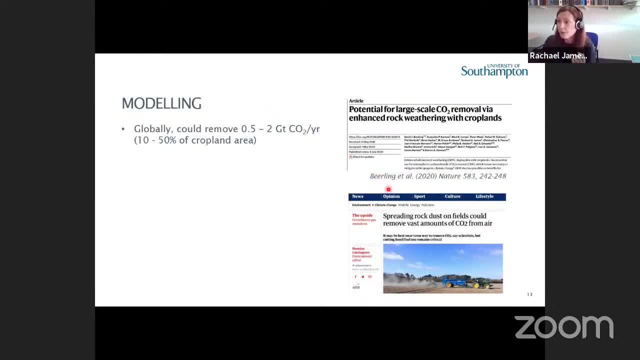 focused on modeling, focused on modeling, uh, and there was a modeling study that i, uh, and there was a modeling study that i, uh, and there was a modeling study that i was involved in, was involved in, was involved in published um last year that you can you published um last year that you can you. 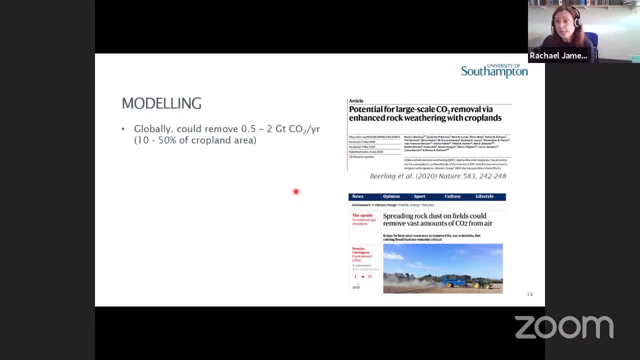 published um last year that you can, you can see here, can see here, can see here. that suggests that on a global basis, that suggests that on a global basis, that suggests that, on a global basis, um, um, um. rock weathering in this way could remove, rock weathering in this way could remove. 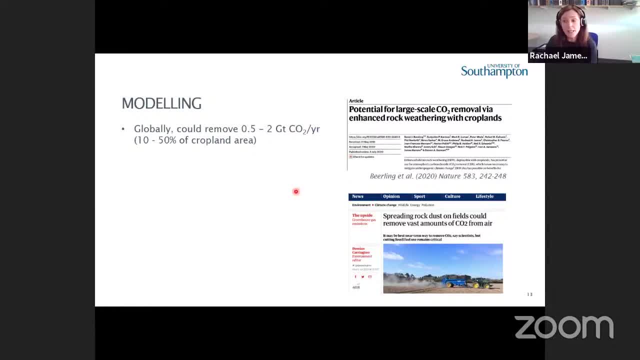 rock weathering in this way could remove about 0.5 to 2 gigatons of carbon. about 0.5 to 2 gigatons of carbon. about 0.5 to 2 gigatons of carbon dioxide per year. dioxide per year. 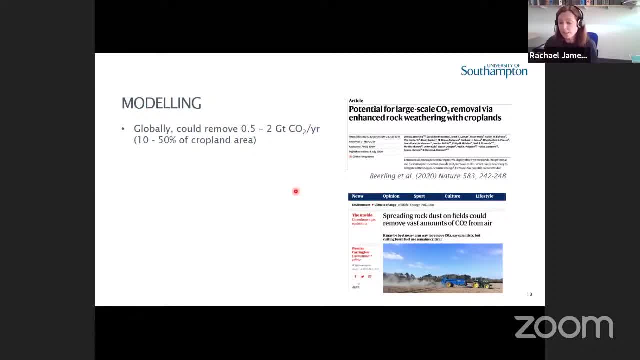 dioxide per year. if if the crushed up rock was applied to. if if the crushed up rock was applied to, if if the crushed up rock was applied to 20 to 50 percent, 20 to 50 percent, 20 to 50 percent of the cropland area. so they're pretty. 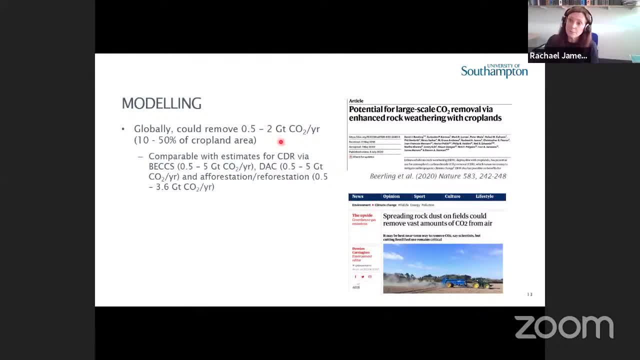 of the cropland area, so they're pretty of the cropland area, so they're pretty significant quantities of carbon dioxide, significant quantities of carbon dioxide, significant quantities of carbon dioxide, and they're and they're and they're comparable uh with estimates for carbon, comparable uh with estimates for carbon. 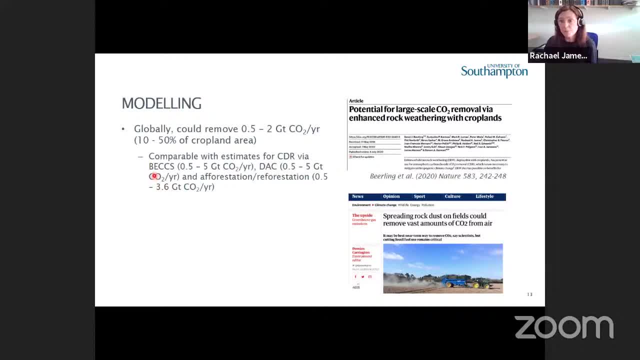 comparable uh with estimates for carbon dioxide removal via other techniques. that dioxide removal via other techniques, that dioxide removal via other techniques that you may have heard of, such as beck. so you may have heard of such as beck. so you may have heard of. such as beck. so that's bioenergy with carbon capture and 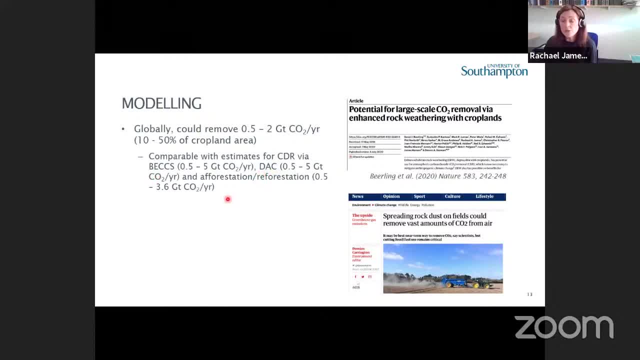 that's bioenergy with carbon capture and that's bioenergy with carbon capture and storage, storage, storage with direct air capture and also with with direct air capture and also with with direct air capture, and also with nature-based solutions or natural nature-based solutions or natural nature-based solutions or natural techniques, such as afforestation, and. 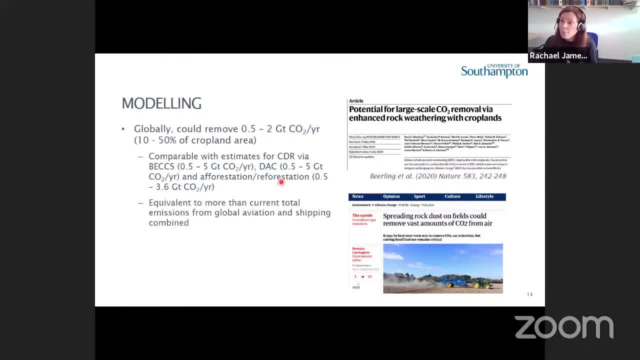 techniques such as afforestation, and techniques such as afforestation and reforestation. the quantities of carbon dioxide that i'm, the quantities of carbon dioxide that i'm, the quantities of carbon dioxide that i'm talking about here, talking about here, talking about here- are equivalent to more than uh the. 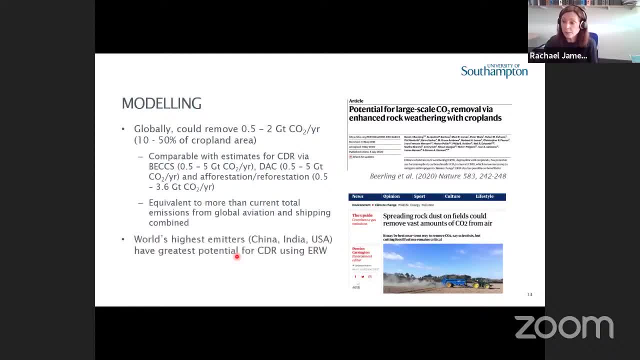 are equivalent to more than uh. the are equivalent to more than uh. the current total emissions from global. current total emissions from global. current total emissions from global aviation and shipping combined aviation and shipping combined aviation and shipping combined. and the other thing about this: this and the other thing about this: this 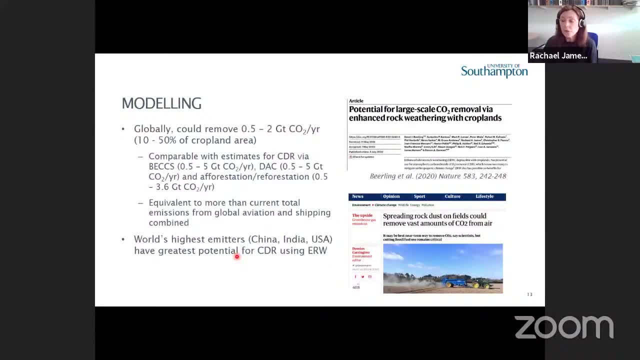 and the other thing about this, this technique is that the world's highest technique is that the world's highest technique is that the world's highest emitters- so china, india and the usa- also emitters. so china, india and the usa also emitters. so china, india and the usa also have the highest potential for carbon. 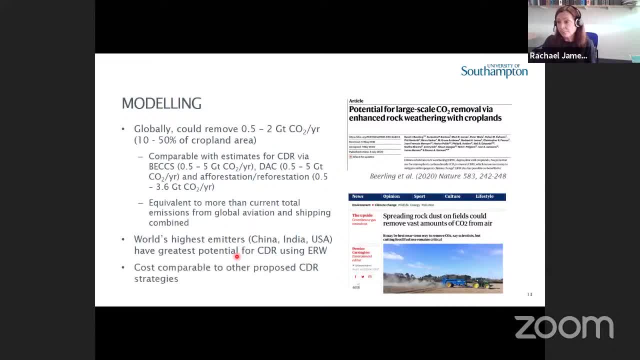 have the highest potential for carbon. have the highest potential for carbon dioxide removal. dioxide removal, dioxide removal using enhanced rock weathering and the using enhanced rock weathering and the using enhanced rock weathering and the cost as well is comparable to other. cost as well is comparable to other. 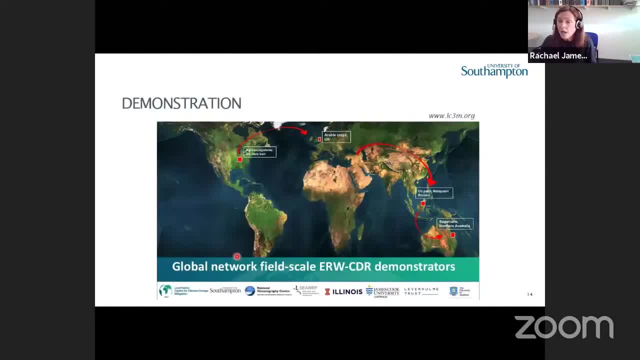 cost as well, is comparable to other proposed carbon dioxide removal. proposed carbon dioxide removal. proposed carbon dioxide removal strategies, strategies, strategies, so their modeling studies. the key is, so their modeling studies. the key is, so their modeling studies. the key is: does this work in practice? does this work in practice? 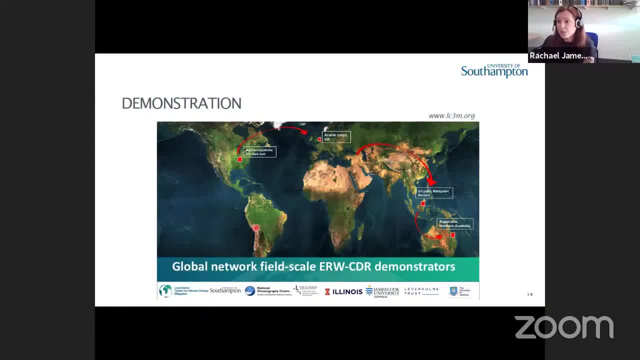 does this work in practice? so as part of the labor home center for. so as part of the labor home center for. so as part of the labor home center for climate change mitigation, i'm involved climate change mitigation. i'm involved climate change mitigation. i'm involved in a series of large-scale field trials. 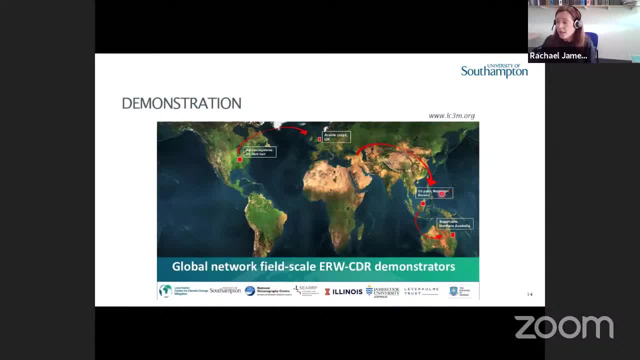 in a series of large-scale field trials, in a series of large-scale field trials in the us, in the uk, in the us, in the uk, in the us, in the uk, in in the us, in the uk, in malaysia and also in australia, in malaysia and also in australia. 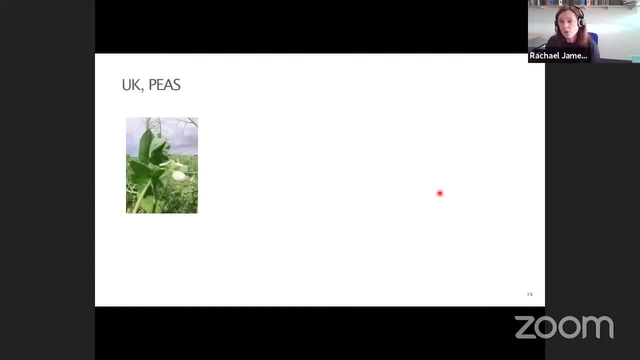 in malaysia and also in australia. and today i just wanted to highlight to, and today i just wanted to highlight to, and today i just wanted to highlight to you some of the results from our trial, you some of the results from our trial, you some of the results from our trial in the uk. 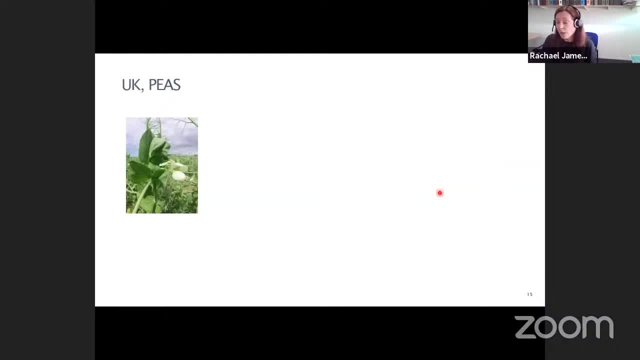 in the uk. in the uk, where we have been applying crushed up, where we have been applying crushed up, where we have been applying crushed up basaltic rock to peas, basaltic rock to peas, basaltic rock to peas. this is just an overview of our 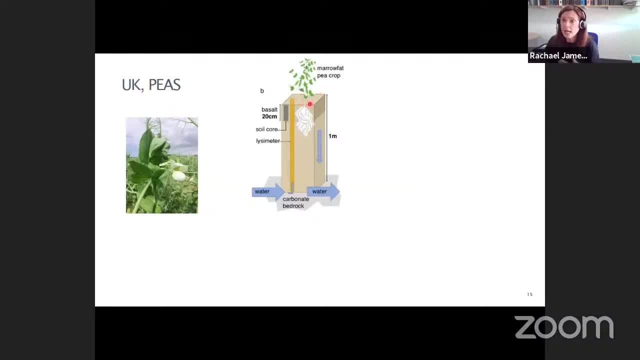 this is just an overview of our. this is just an overview of our experimental setup here. so the the experimental setup here. so the, the experimental setup here. so the the basalt is applied, basalt is applied. basalt is applied and plowed in as usual practice to the. 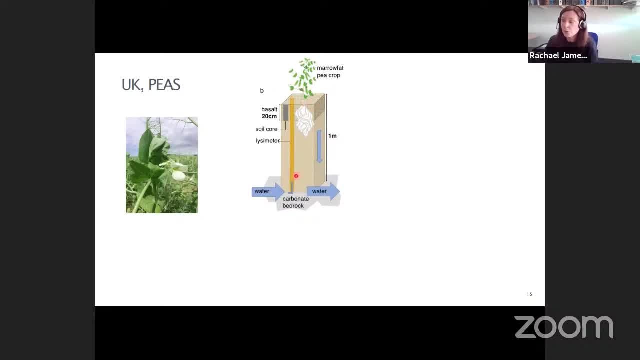 and plowed in, as usual practice, to the and plowed in, as usual practice, to the surface of the soil, surface of the soil, surface of the soil, and then we've been sampling the soil, and then we've been sampling the soil, and then we've been sampling the soil. pore waters. 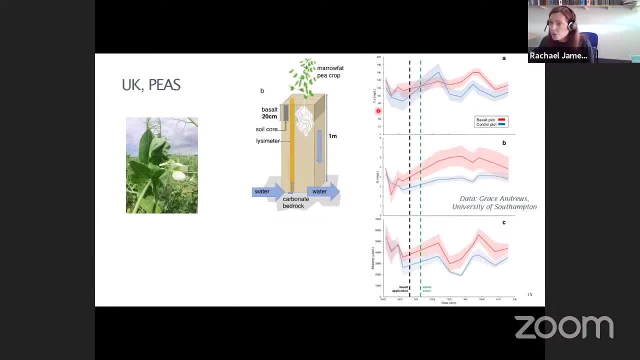 pore waters: pore waters using lysimeters. okay, these plots are a using lysimeters. okay, these plots are a using lysimeters. okay, these plots are a little bit difficult to see, little bit difficult to see, little bit difficult to see. but along here we have uh date. but along here we have uh date. 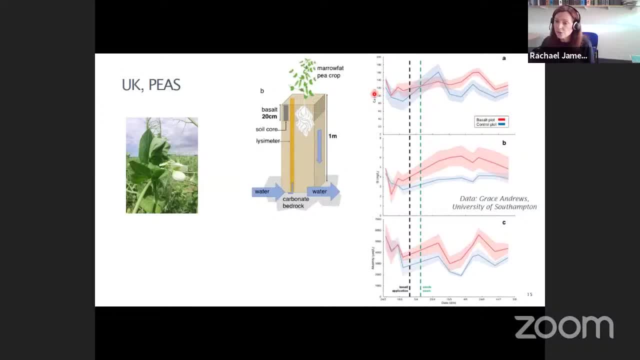 but along here we have uh date and on the top plot here i'm showing, and on the top plot here i'm showing, and on the top plot here i'm showing calcium concentrations in those uh calcium concentrations in those uh calcium concentrations in those uh soil, pore waters. 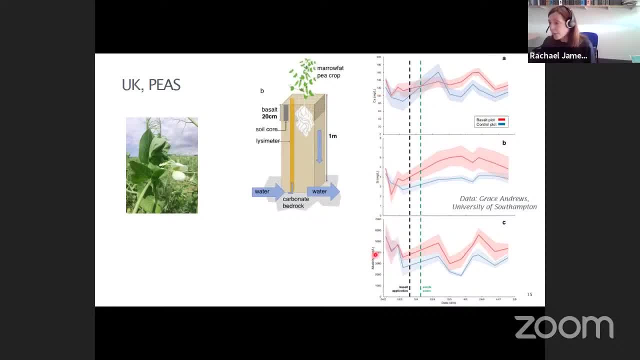 soil pore waters. soil pore waters. silicon concentrations and alkalinity. silicon concentrations and alkalinity. silicon concentrations and alkalinity. and what we can see is that in our plot, and what we can see is that in our plot, and what we can see is that in our plot, where we apply the basalt, compared to 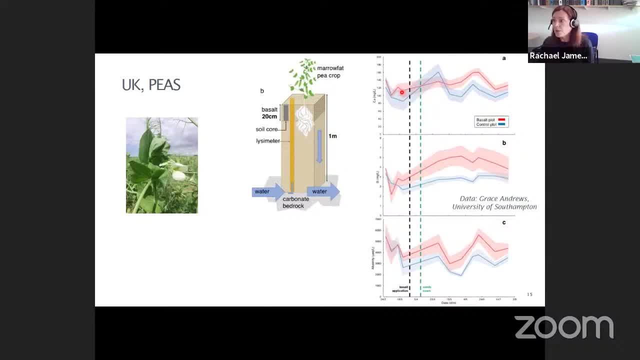 where we apply the basalt, compared to where we apply the basalt, compared to our plot. where which is a control? where our plot? where which is a control? where our plot? where which is a control? where we don't apply the basalt, we don't apply the basalt. 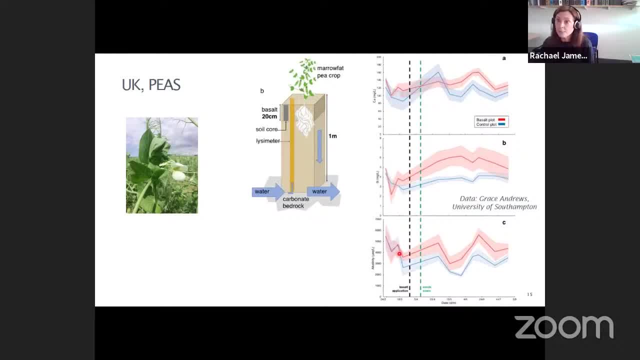 we don't apply the basalt concentrations of calcium silicon and concentrations of calcium silicon and concentrations of calcium silicon and alkalinity are pretty similar before we. alkalinity are pretty similar before we. alkalinity are pretty similar before we stick the basalt in the field. stick the basalt in the field. 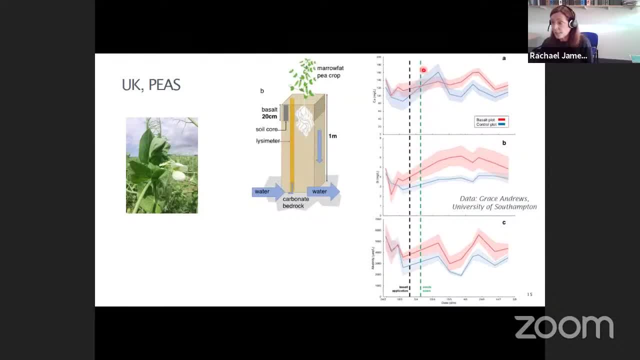 stick the basalt in the field. the green line here shows where the. the. the green line here shows where the the. the green line here shows where the. the peas were, seeds were sown. peas were, seeds were sown. peas were, seeds were sown, and the growing period extends to here. 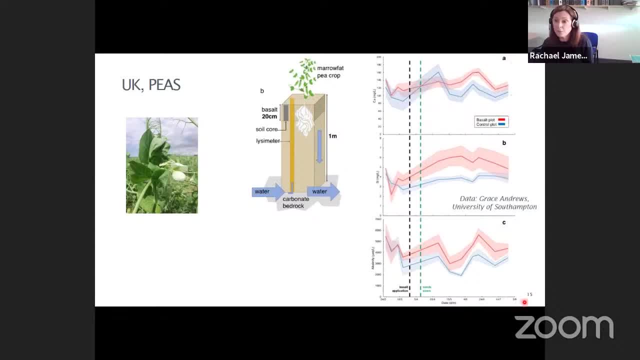 and the growing period extends to here, and the growing period extends to here, and then the peas are harvest at this, and then the peas are harvest at this, and then the peas are harvest at this point here, which is five months later. point here, which is five months later. 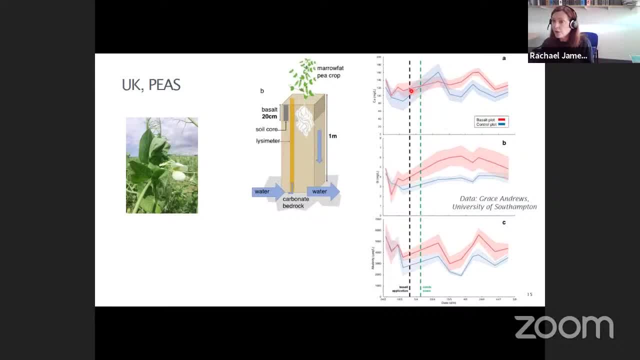 point here, which is five months later, and what we can see is that um after, and what we can see is that um after, and what we can see is that um after we've applied, we've applied, we've applied the basalt, and particularly after the the basalt, and particularly after the 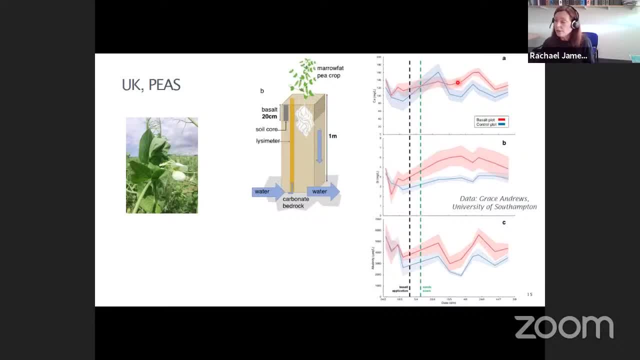 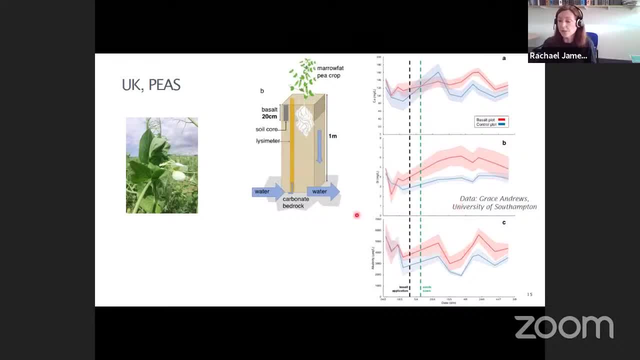 soil waters, higher concentrations of soil waters, higher concentrations of silica, silica, silica and higher alkalinity concentrations, and higher alkalinity concentrations and higher alkalinity concentrations, too, too, too, and all of this is evidence for, and all of this is evidence for, and all of this is evidence for enhanced weathering of the basalt that 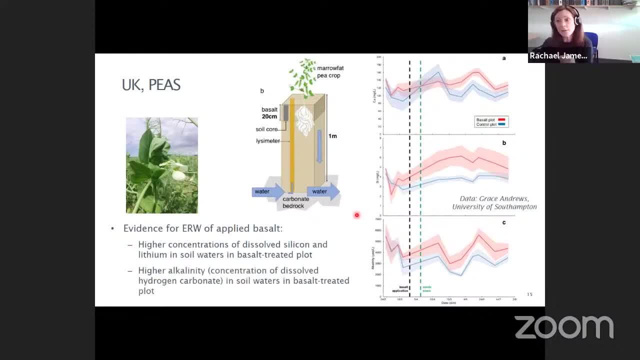 enhanced weathering of the basalt. that enhanced weathering of the basalt that we apply, we apply, we apply to those soils and the higher to those soils and the higher to those soils and the higher alkalinity concentrations that we see, alkalinity concentrations that we see. 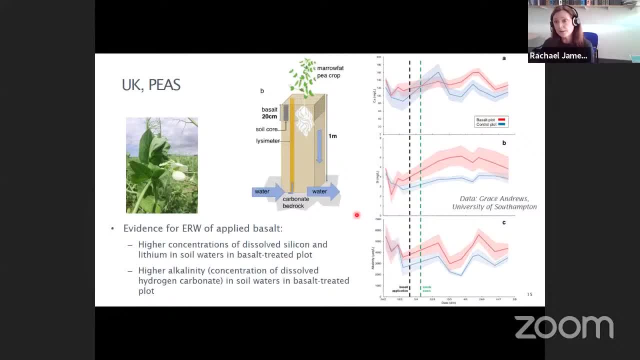 alkalinity concentrations that we see in these soils equate to draw down of in these soils, equate to draw down of in these soils, equate to draw down of atmospheric carbon dioxide, atmospheric carbon dioxide, atmospheric carbon dioxide. and so if we convert those alkalinity and so if we convert those alkalinity, 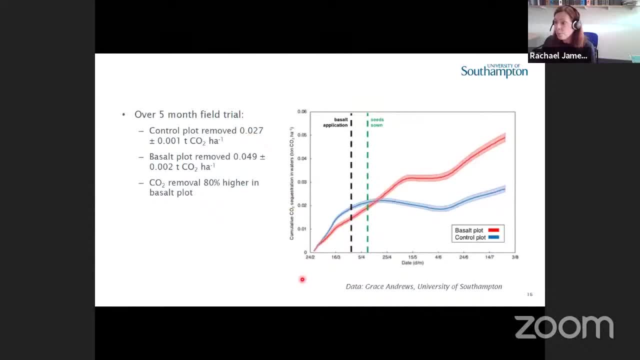 and so if we convert those alkalinity concentrations, concentrations, concentrations, into carbon dioxide removal, i've got cumulative carbon dioxide. i've got cumulative carbon dioxide. i've got cumulative carbon dioxide. removal on the the vertical axes here. removal on the the vertical axes here. removal on the the vertical axes- here. control plot is shown with the red line. 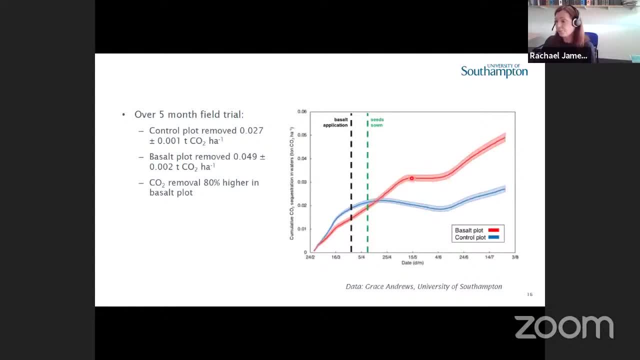 control plot is shown with the red line. control plot is shown with the red line and the blue line. uh, and the blue line. uh and the blue line, uh, sorry. the red line shows the basalt plot. sorry. the red line shows the basalt plot, sorry. the red line shows the basalt plot and the blue line shows the control plot. 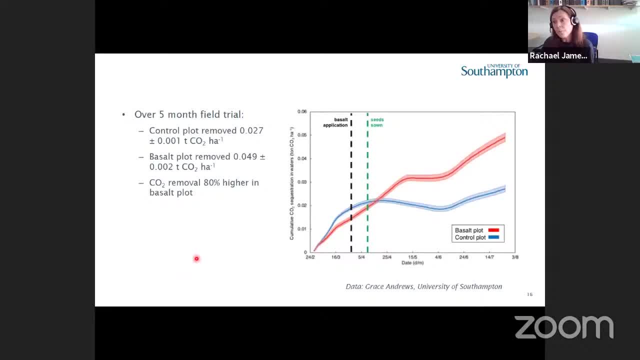 and the blue line shows the control plot. and the blue line shows the control plot and what you can see is over that five. and what you can see is over that five. and what you can see is over that five. month field trial, month field trial, month, field trial. uh, the plot where we added the basalt. 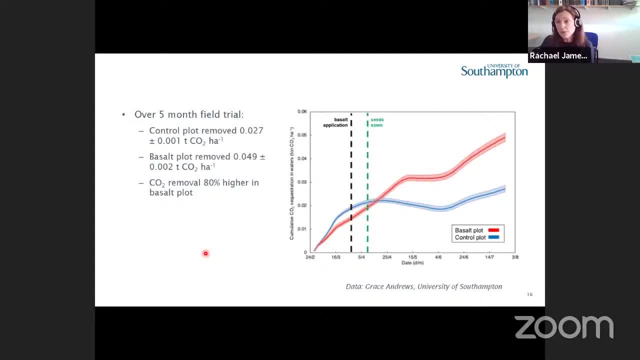 uh, the plot where we added the basalt. uh, the plot where we added the basalt removed, approximately 80 percent more removed, approximately 80 percent more removed, approximately 80 percent more carbon dioxide than the plot where we carbon dioxide, than the plot where we carbon dioxide than the plot where we didn't apply the basalt. 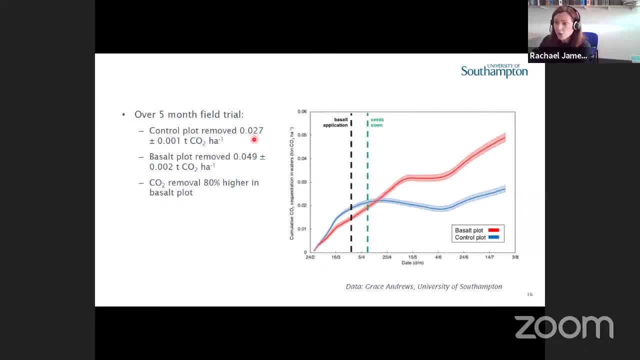 didn't apply the basalt, didn't apply the basalt. so that's that's quite an important, so that's that's quite an important, so that's that's quite an important result. but actually, if we look at the result, but actually if we look at the 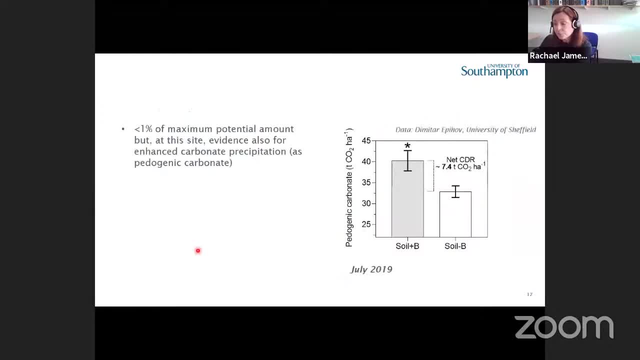 result. but actually, if we look at the quantities of carbon dioxide, quantities of carbon dioxide, quantities of carbon dioxide that are removed- um they're, they're that are removed, um they're, they're that are removed, um they're, they're quite, they're pretty small and, in fact, 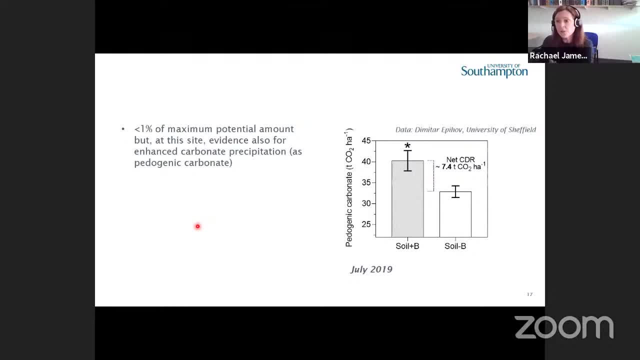 quite, they're pretty small and in fact, quite they're pretty small and in fact they're less than one percent of the. they're less than one percent of the. they're less than one percent of the maximum potential amount, maximum potential amount, maximum potential amount of carbon dioxide removal that we would 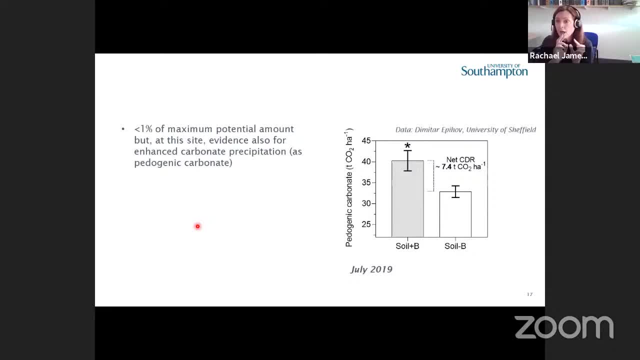 of carbon dioxide removal that we would, of carbon dioxide removal that we would expect, expect, expect, given the amount of rock that we added, given the amount of rock that we added, given the amount of rock that we added. but one thing i should say is at this. but one thing i should say is at this: 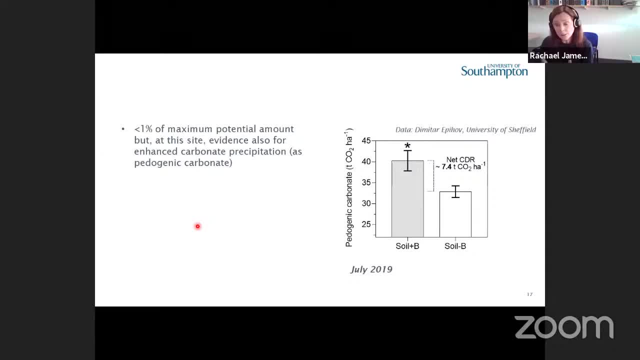 but one thing i should say is: at this site, site, site, uh, uh, it's in east anglia. there are uh, uh, it's in east anglia. there are uh, uh, it's in east anglia. there are carbonate rich soils here, carbonate rich soils here, carbonate rich soils here. we also see evidence for enhanced 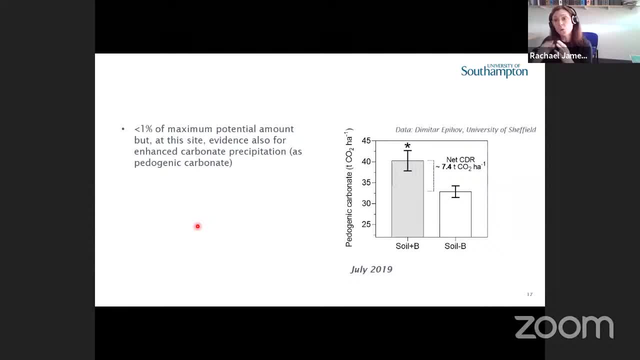 we also see evidence for enhanced, we also see evidence for enhanced carbonate precipitation and that carbonate precipitation and that carbonate precipitation and that carbonate of course also comes from the carbonate, of course also comes from the carbonate, of course also comes from the atmosphere, atmosphere, atmosphere, and that's shown in this plot here. 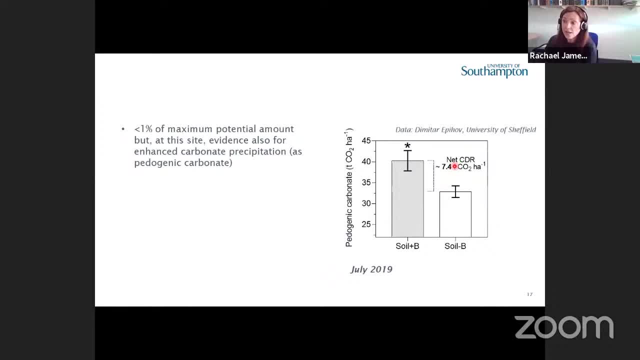 and that's shown in this plot here and that's shown in this plot here and you can see that, the uh quantities and you can see that the uh quantities and you can see that the uh quantities, this change that we see this change that we see this change that we see in the amount of soil carbonate. that's. 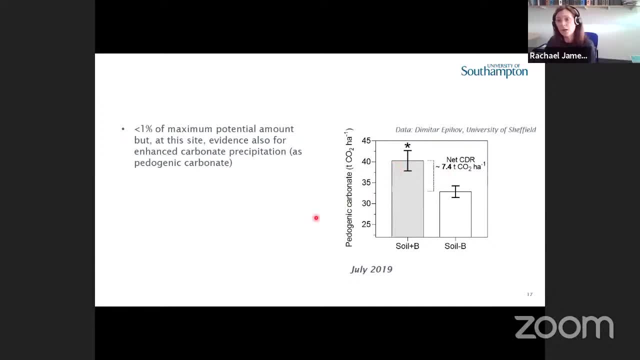 in the amount of soil carbonate, that's in the amount of soil carbonate that's being produced, are really significant. being produced are really significant. being produced are really significant orders of magnitude, higher than the orders of magnitude, higher than the orders of magnitude, higher than the change we see in alkalinity. 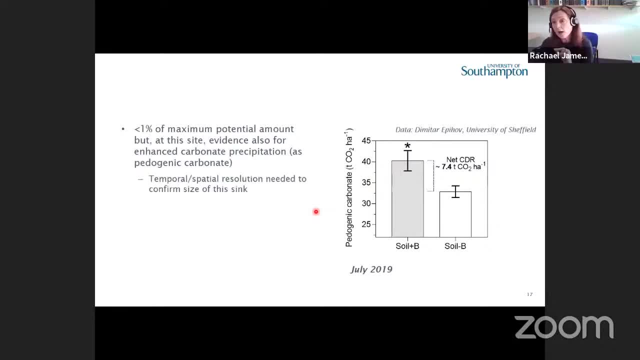 change we see in alkalinity, change we see in alkalinity. caveat to this, i would say: is that caveat to this? i would say, is that caveat to this, i would say, is that measurements of soil carbonate are measurements of soil carbonate are measurements of soil carbonate are incredibly patchy. 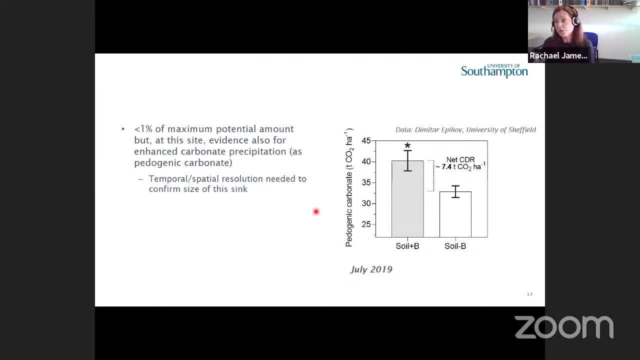 incredibly patchy, incredibly patchy. we need to do a huge amount of sampling. we need to do a huge amount of sampling. we need to do a huge amount of sampling to confirm that this result is, to confirm that this result is to confirm that this result is statistically significant, and we also 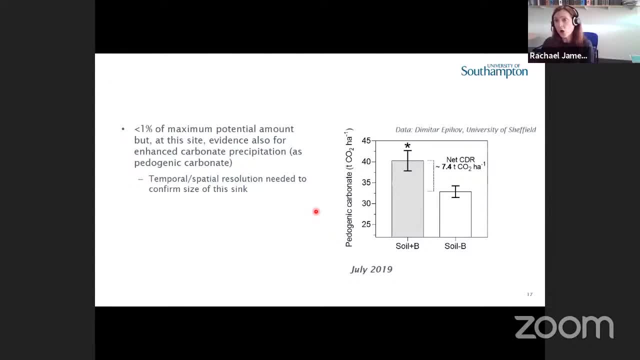 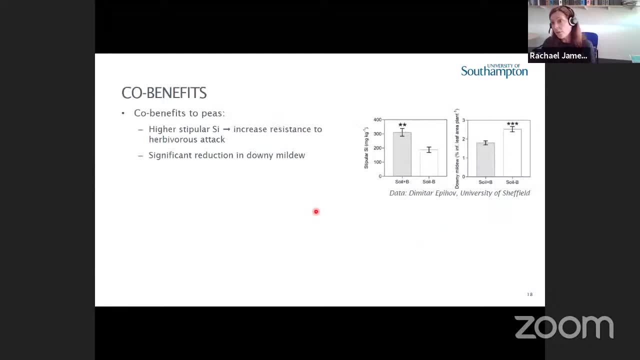 statistically significant and we also statistically significant and we also need to increase the special spatial need, to increase the special spatial need, to increase the special spatial resolution resolution, resolution of that sampling to confirm this, of that sampling to confirm this, of that sampling to confirm this. i also mentioned that 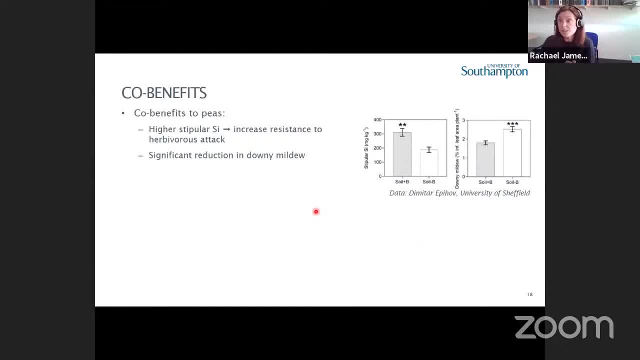 i also mentioned that. i also mentioned that this technique could have potential code. this technique could have potential code. this technique could have potential code benefits for the crops themselves, benefits for the crops themselves, benefits for the crops themselves. and if we look at the silicon, and if we look at the silicon, 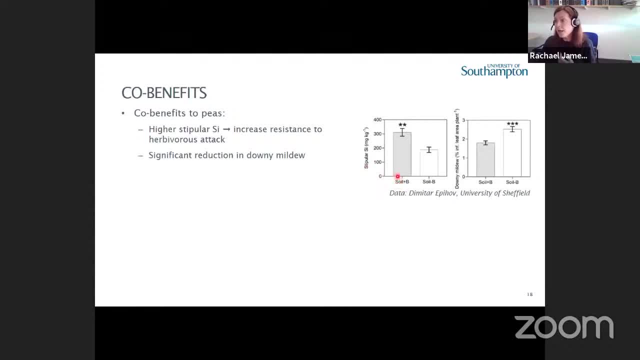 and if we look at the silicon concentrations, concentrations, concentrations in the stipular parts of those, please, we in the stipular parts of those, please, we in the stipular parts of those, please- we can see that they're higher in the plot, can see that they're higher in the plot. 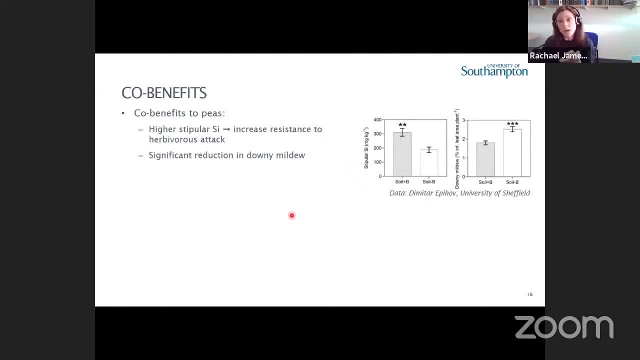 can see that they're higher in the plot where we've added basalt, where we've added basalt, where we've added basalt, and the higher the quantity of silica in and the higher the quantity of silica in and the higher the quantity of silica in those peas, it makes them more resistant. 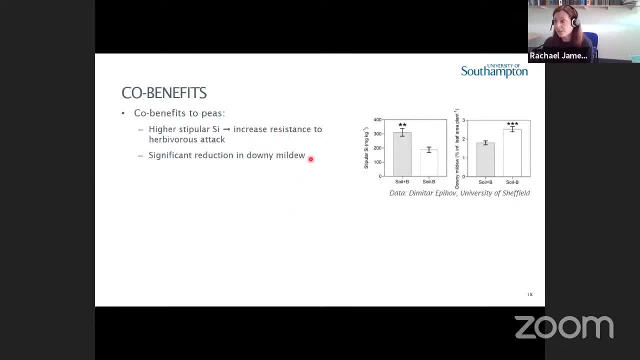 those peas. it makes them more resistant those peas. it makes them more resistant to herbivorous attacks. so farmers are to herbivorous attacks. so farmers are to herbivorous attacks. so farmers are happy about this, happy about this, happy about this: these crushed up rocks, two crops is. 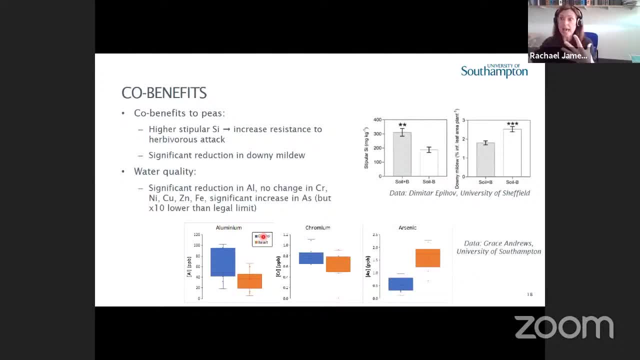 these crushed up rocks two crops? is these crushed up rocks two crops? is what effect does this have on water? what effect does this have on water? what effect does this have on water quality? don't these rocks quality? don't these rocks quality? don't these rocks add heavy metals into the water system? 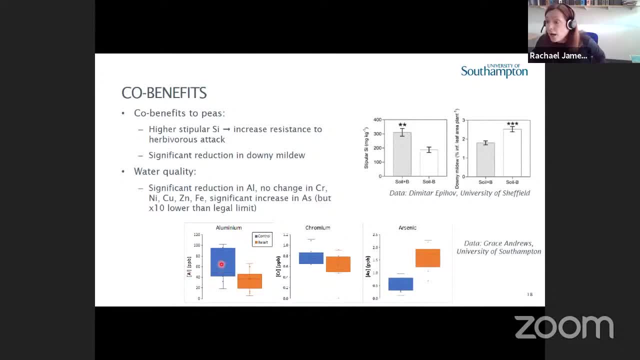 add heavy metals into the water system. add heavy metals into the water system? well, actually, in most cases, no, they well, actually, in most cases, no, they well, actually in most cases, no, they don't, don't, don't. uh, if i, if we look at aluminium here, uh, if i, if we look at aluminium here. 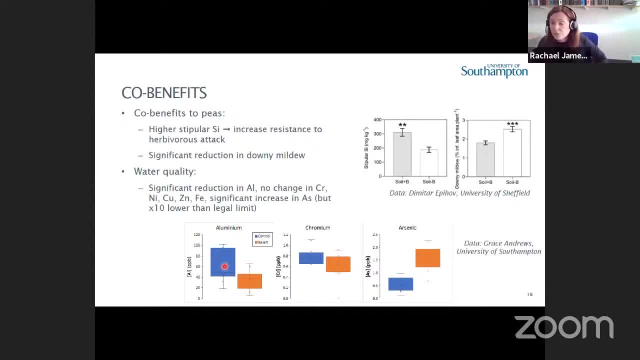 uh, if i if we look at aluminium here in the control plot and the basalt plot, in the control plot and the basalt plot, in the control plot and the basalt plot, actually we see a significant reduction. actually we see a significant reduction. actually we see a significant reduction in the amount of aluminium in the soil. 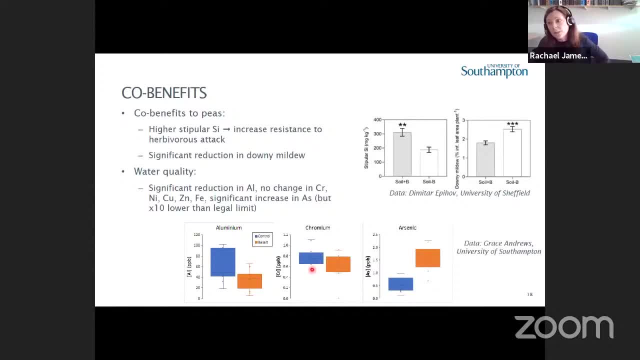 in the amount of aluminium in the soil, in the amount of aluminium in the soil. waters, waters, waters. we see no change in the amount of. we see no change in the amount of. we see no change in the amount of chromium in those soil waters, chromium in those soil waters. 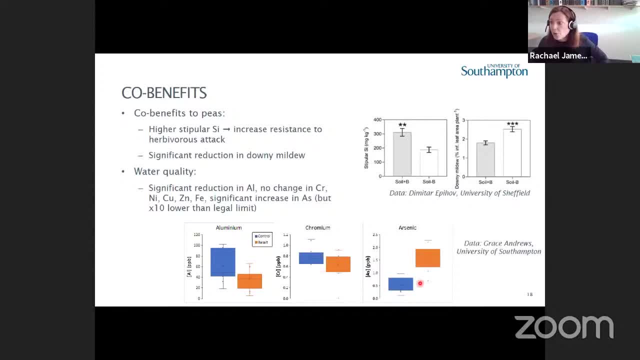 chromium in those soil waters. and, in fact, the only element we do see a, and in fact, the only element we do see a and in fact the only element we do see a change for is the amount of arsenic in change for is the amount of arsenic in. 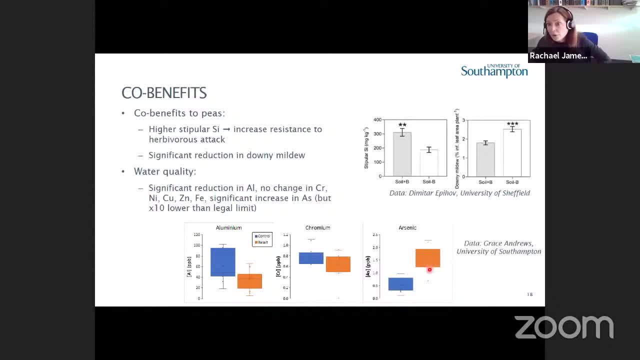 change for is the amount of arsenic in those soil waters, those soil waters, those soil waters, which might shock many of you, but i would, which might shock many of you, but i would, which might shock many of you, but i would point out that the arsenic levels, that 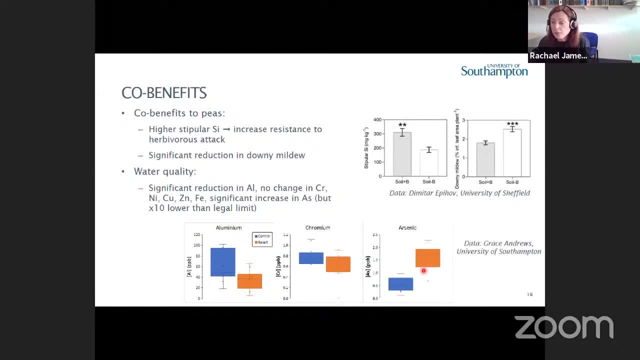 point out that the arsenic levels, that point out that the arsenic levels that we see here are still 10 times lower- we see here- are still 10 times lower. we see here- are still 10 times lower than the legal limit. and we think the 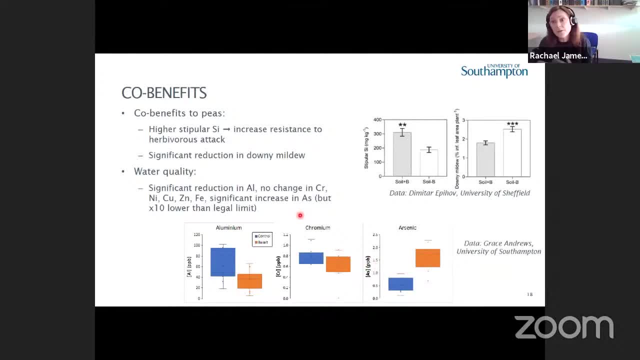 than the legal limit, and we think the than the legal limit, and we think the reason for these, reason for these, reason for these: these changes in metals is, in fact, the. these changes in metals is, in fact, the. these changes in metals is, in fact, the secondary minerals that form. 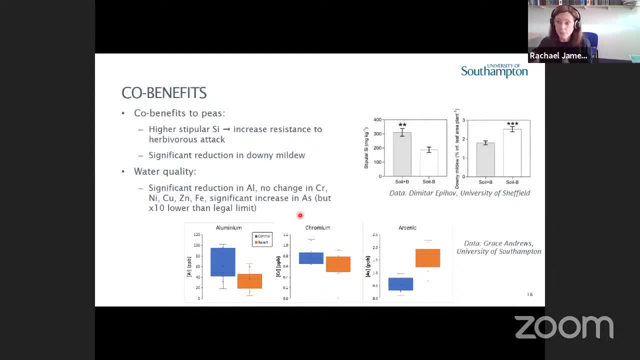 secondary minerals that form, secondary minerals that form as a result of weathering of that basalt. as a result of weathering of that basalt, as a result of weathering of that basalt, are mopping up those heavy metals. and the final thing i just wanted to: 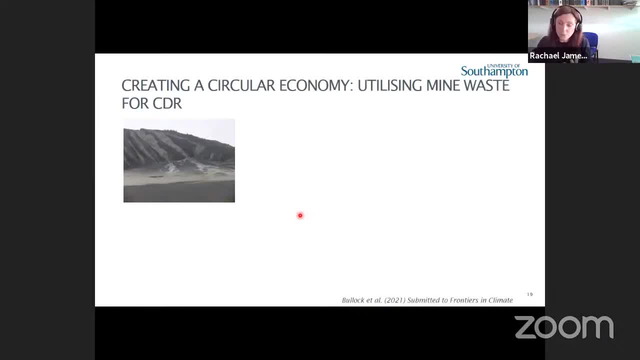 and the final thing i just wanted to, and the final thing i just wanted to point out for you, is that this technique point out for you is that this technique point out for you is that this technique also also also offers the opportunity for creating a, offers the opportunity for creating a. 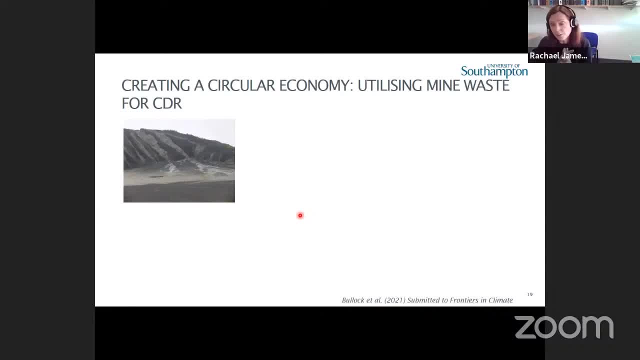 offers the opportunity for creating a circular economy, circular economy, circular economy in all of those field trials. i'm involved in all of those field trials. i'm involved in all of those field trials i'm involved in. we're actually using waste products in. we're actually using waste products. 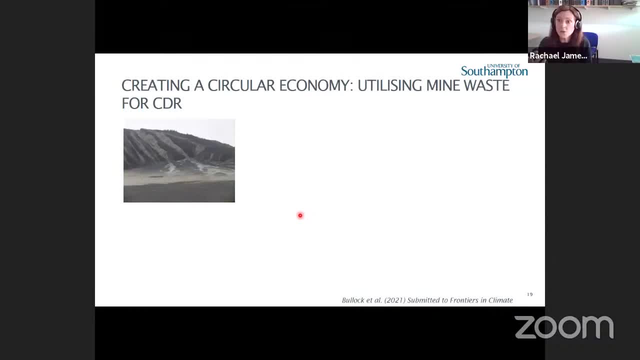 in. we're actually using waste products from the mining industry and applying from the mining industry and applying from the mining industry and applying those to those to those, to the soils potential for creating a the soils potential for creating a, the soils potential for creating a circular economy here, and one of my 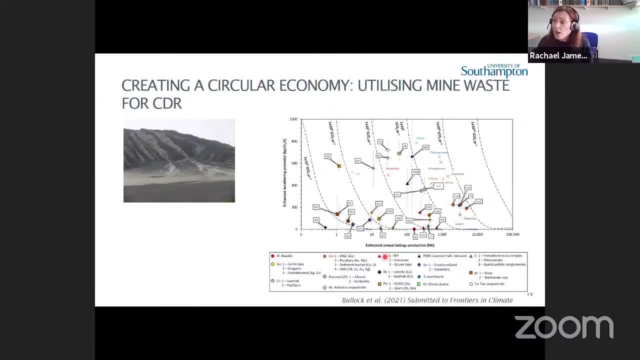 circular economy here and one of my circular economy here and one of my postdocs, liam bullock, has done some work. postdocs: liam bullock has done some work. postdocs: liam bullock has done some work on this, on this, on this where he's looked at the amount of mine. 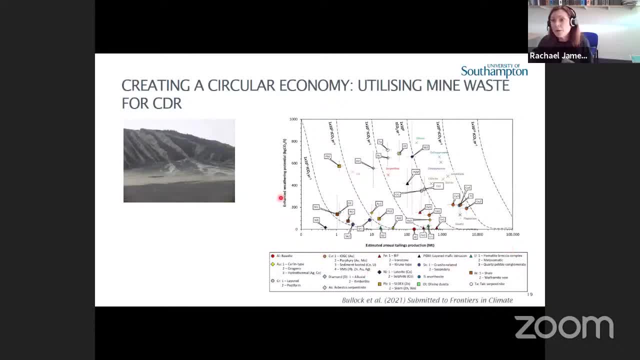 where he's looked at the amount of mine, where he's looked at the amount of mine tailings being produced on an annual tailings being produced on an annual tailings being produced on an annual basis, basis basis, and then looked at the chemical and then looked at the chemical. 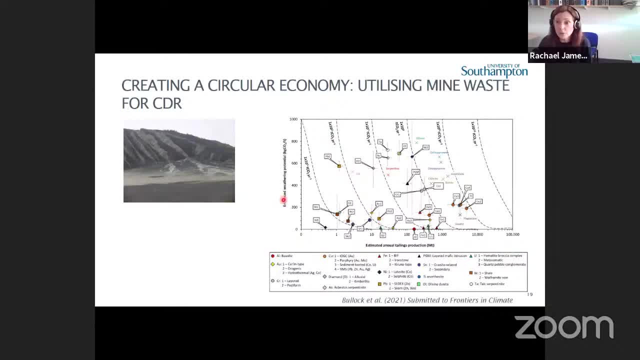 and then looked at the chemical composition of those mine tailings, to composition of those mine tailings, to composition of those mine tailings to figure out what their carbon dioxide figure out, what their carbon dioxide figure out, what their carbon dioxide removal potential, removal potential, removal potential is, uh, this here, this would be 10. 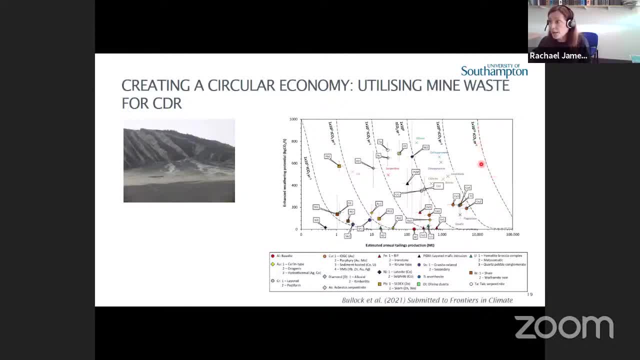 is uh this here? this would be 10 is uh this here? this would be 10 billion tons. 10 gigatons of carbon billion tons. 10 gigatons of carbon billion tons. 10 gigatons of carbon dioxide removal per year. dioxide removal per year. 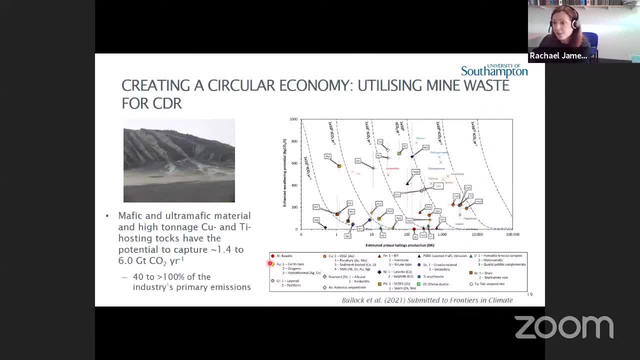 dioxide removal per year, and this would be a gigaton here and this would be a gigaton here, and this would be a gigaton here and on the basis of his work, and on the basis of his work, and on the basis of his work, the types of rocks that are most. 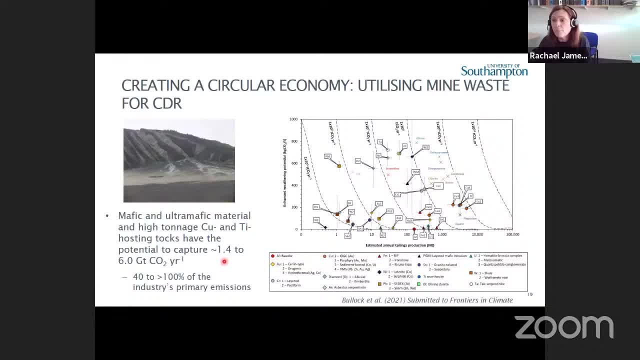 the types of rocks that are most the types of rocks that are most conducive to carbon dioxide conducive to carbon dioxide. conducive to carbon dioxide removal and mafic and ultra mafic removal and mafic and ultra mafic removal and mafic and ultra mafic materials. 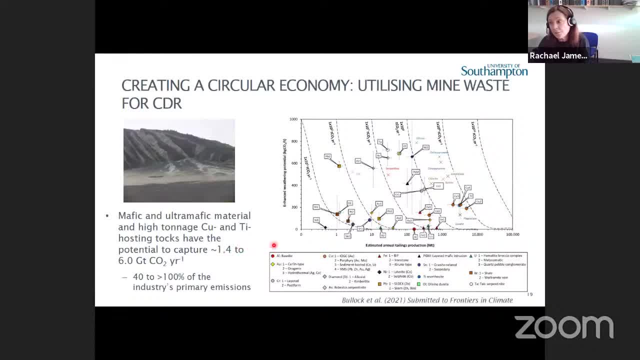 materials, materials and those that are produced in high and those that are produced in high and those that are produced in high quantities by the mining industry, quantities by the mining industry, quantities by the mining industry. and if we sum that up, those rocks have. and if we sum that up, those rocks have. 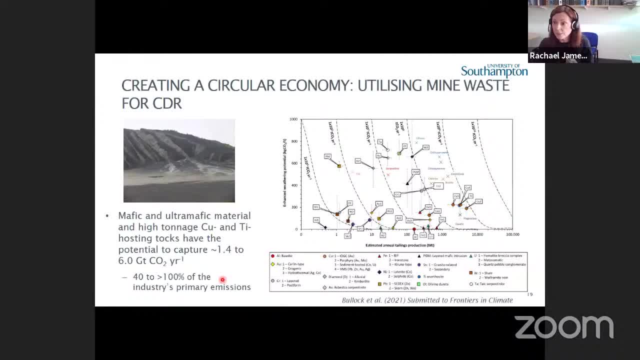 and if we sum that up, those rocks have all of that mining industry's primary, all of that mining industry's primary, all of that mining industry's primary: emissions, emissions, emissions. okay, i can see i need to wrap up. uh, okay, i can see i need to wrap up, uh. 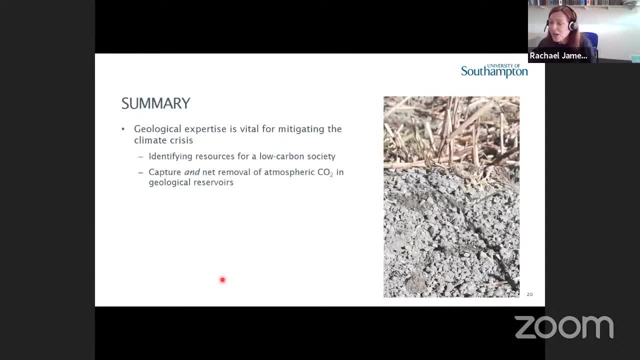 okay, i can see i need to wrap up. uh, it's been a long day. uh, thank you for it's been a long day. uh, thank you for it's been a long day. uh, thank you for staying with us, staying with us, staying with us. uh, points i wanted to make is that. 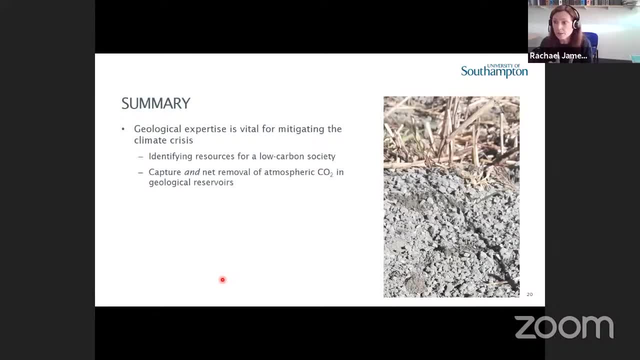 uh points i wanted to make. is that? uh, points i wanted to make is that geological expertise, geological expertise, geological expertise are vital for mitigating the climate, are vital for mitigating the climate, are vital for mitigating the climate crisis, crisis, crisis. uh, what geologists can do is identify. 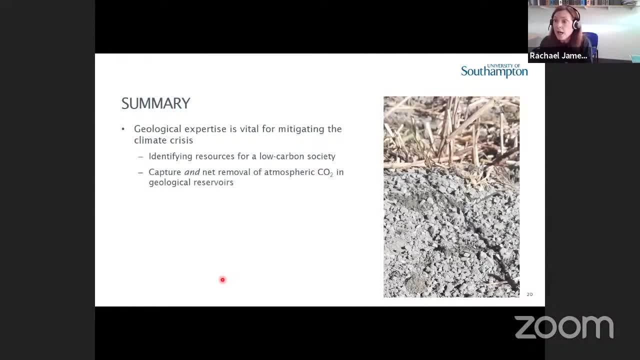 uh, what geologists can do is identify- uh, what geologists can do is identify resources needed for a low carbon resources needed for a low carbon resources needed for a low carbon society, society, society, and they're also, and they're also, and they're also hugely important for verifying. 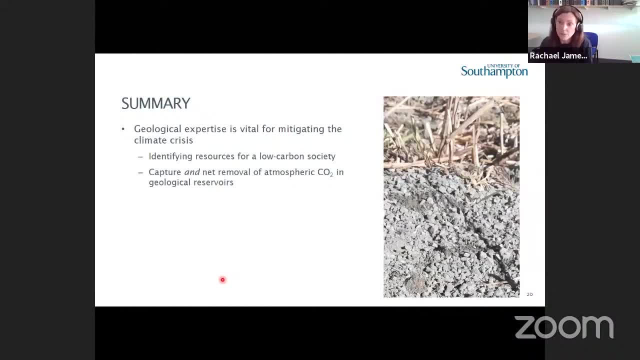 hugely important for verifying, hugely important for verifying, quantifying, quantifying, quantifying removal of atmospheric carbon dioxide. in removal of atmospheric carbon dioxide, in removal of atmospheric carbon dioxide in geological reservoirs, geological reservoirs, geological reservoirs and those traditional geology and those traditional geology. 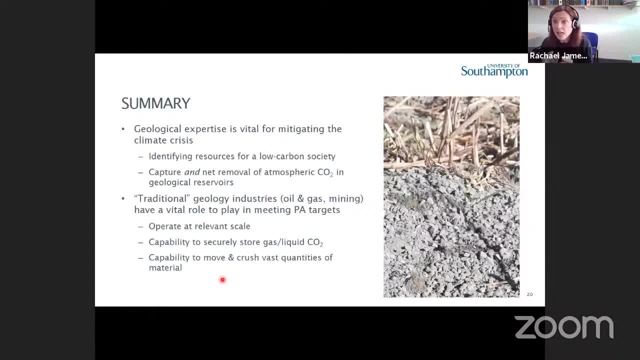 and those traditional geology industries as well, the oil and gas and industries as well, the oil and gas and industries as well, the oil and gas and the mining industries, the mining industries, the mining industries can have a really vital role to play in, can have a really vital role to play in. 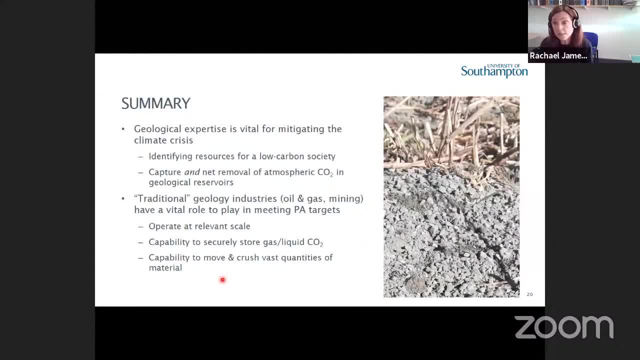 can have a really vital role to play in meeting paris agreement targets. meeting paris agreement targets: meeting paris agreement targets- secure- securely storing gas or liquid. secure securely storing gas or liquid. secure securely storing gas or liquid forms of forms of forms of carbon dioxide. and they have the 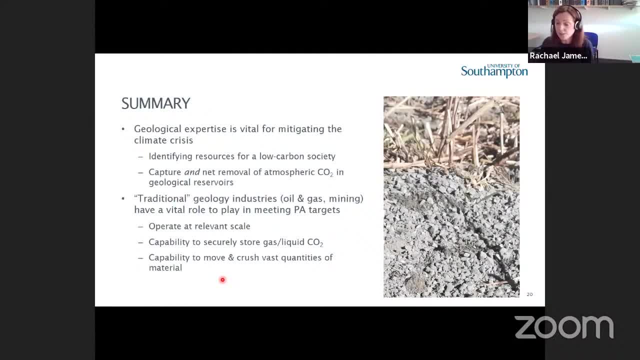 carbon dioxide. and they have the carbon dioxide and they have the capability to move and crush- vast capability to move and crush, vast capability to move and crush vast quantities of material, quantities of material, quantities of material. so i want to wrap up first of all by: so i want to wrap up first of all by: 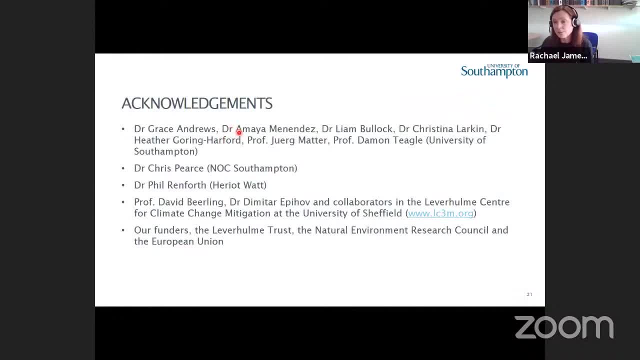 so i want to wrap up, first of all, by acknowledging, acknowledging, acknowledging all of my colleagues in southampton, my all of my colleagues in southampton, my all of my colleagues in southampton, my postdocs, phd students and collaborators. postdocs, phd students and collaborators. 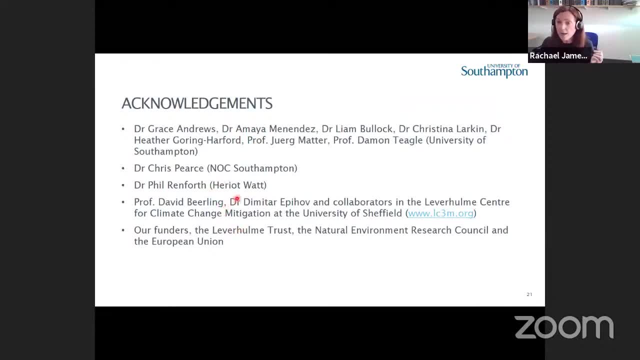 postdocs, phd students and collaborators, teams outside of southampton, that i work. teams outside of southampton, that i work teams outside of southampton that i work with and our funders as well, and i will with and our funders as well, and i will. 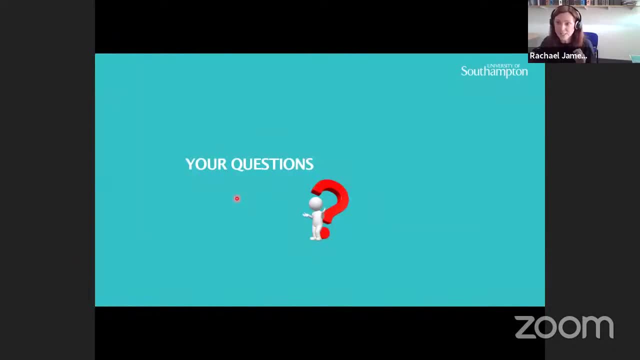 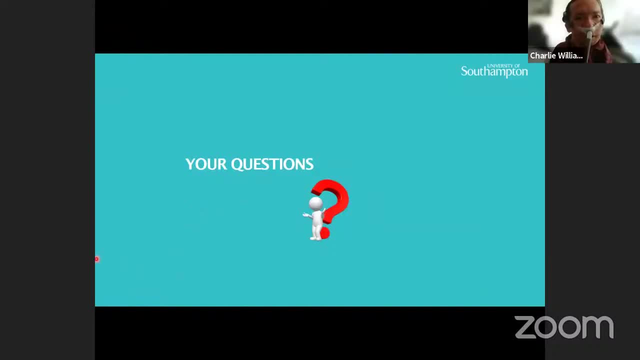 thank you ever so much, rachel. that was absolutely fascinating, sort of really absolutely fascinating, sort of really absolutely fascinating, sort of really really interesting, really interesting, really interesting. so we have a couple of very good, so we have a couple of very good, so we have a couple of very good questions from the 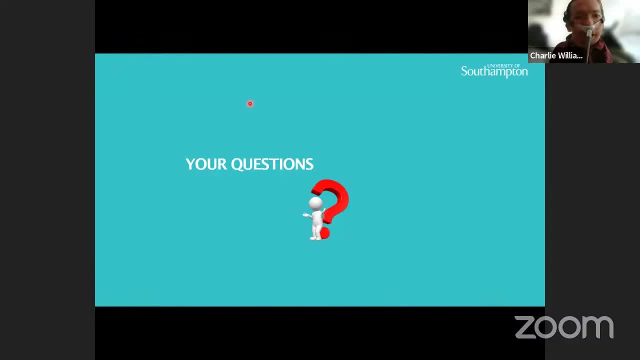 questions. from the questions from the. uh from the attendees. uh from the attendees. uh from the attendees. first up is: is there a model to how first up is? is there a model to how first up is? is there a model to how much energy will be required to extract? 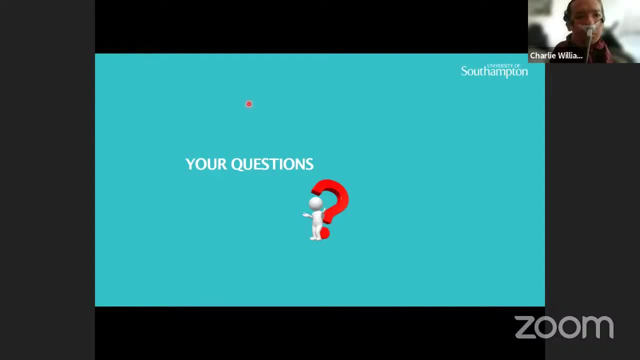 much energy will be required to extract, much energy will be required to extract all the additional resources for these, all the additional resources for these, all the additional resources for these. new technologies, new technologies, new technologies, and what is the co2 impact of these, and what is the co2 impact of these. 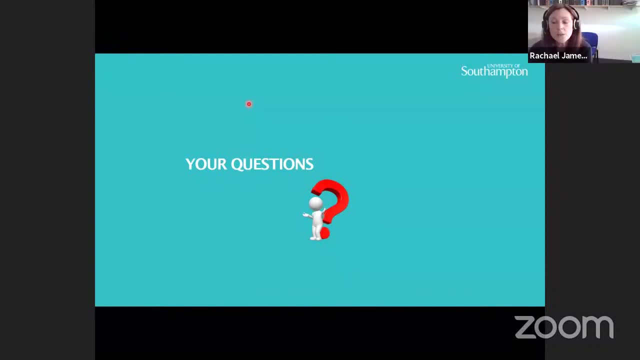 and what is the co2 impact of these energy requirements? energy requirements: energy requirements: yeah, absolutely so. so the the modeling: yeah, absolutely so. so the the modeling- yeah, absolutely so. so the the modeling study that i refer to, uh, in the middle study that i refer to, uh, in the middle. 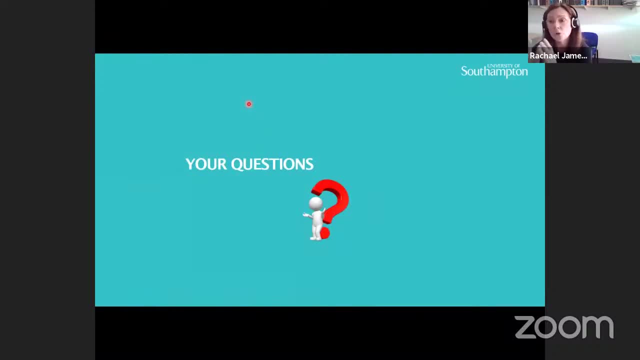 study that i refer to, uh, in the middle, part of my talk takes that into account. part of my talk takes that into account. part of my talk takes that into account. so it's not just looking at carbon. so it's not just looking at carbon. so it's not just looking at carbon dioxide drawdown. 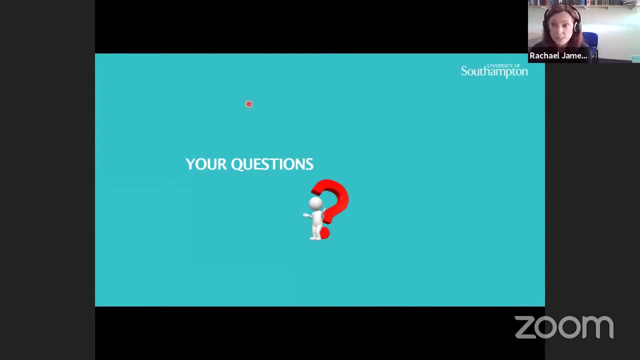 dioxide drawdown. dioxide drawdown um as a result of applying the the um. as a result of applying the the um. as a result of applying the the crushed up silicate rock. it also takes crushed up silicate rock. it also takes crushed up silicate rock. it also takes into account the energy required. 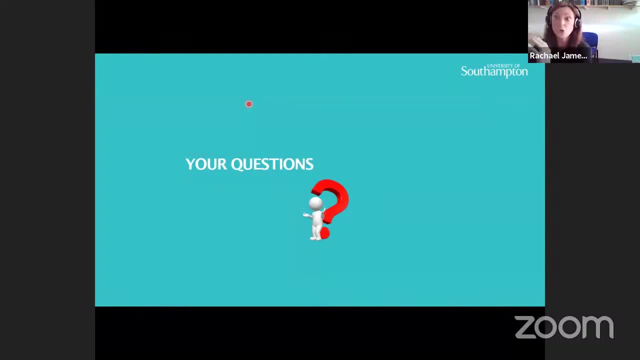 into account the energy required, into account the energy required um to crush that rock up in the first, um to crush that rock up in the first, um to crush that rock up in the first place, place, place. should it not be a? a waste product? should it not be a? a waste product? 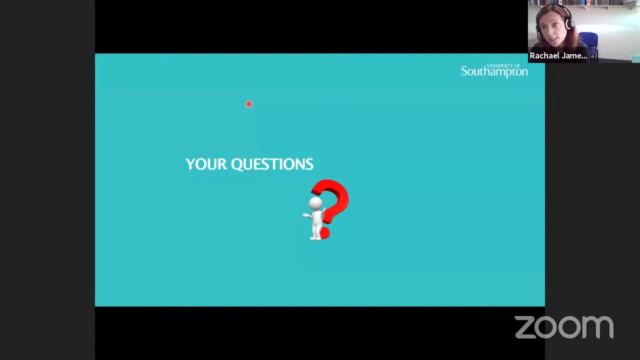 should it not be a a waste product? transportation of that material, transportation of that material, transportation of that material to the site and all of the knock-on to the site and all of the knock-on to the site, and all of the knock-on emissions as well, and it still comes. 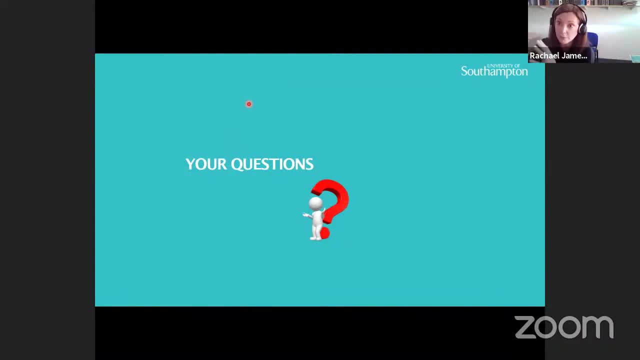 to the site and all of the knock-on emissions as well. and it still comes to the site and all of the knock-on emissions as well, and it still comes out. so so the the quantities of out, so so the the quantities of out, so so the the quantities of carbon dioxide that i refer to are net. 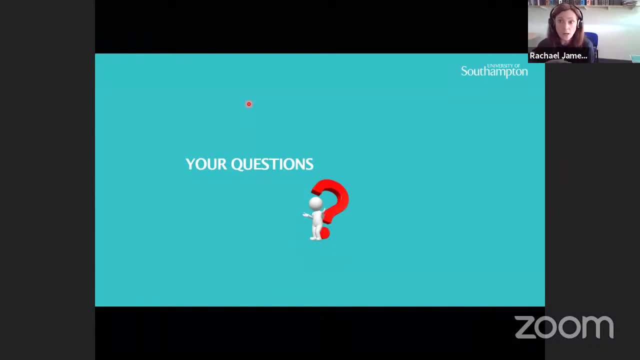 carbon dioxide that i refer to are net carbon dioxide that i refer to are net quantities of carbon dioxide, that take quantities of carbon dioxide, that take quantities of carbon dioxide that take those um uh processes into account, those um uh processes into account, those um uh processes into account. and the other thing i would say is: i'm 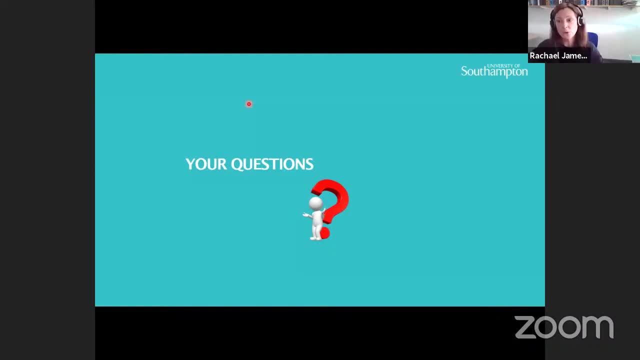 and the other thing i would say is i'm. and the other thing i would say is i'm not in any way advocating that we open, not in any way advocating that we open, not in any way advocating that we open up new mines and start crushing up. 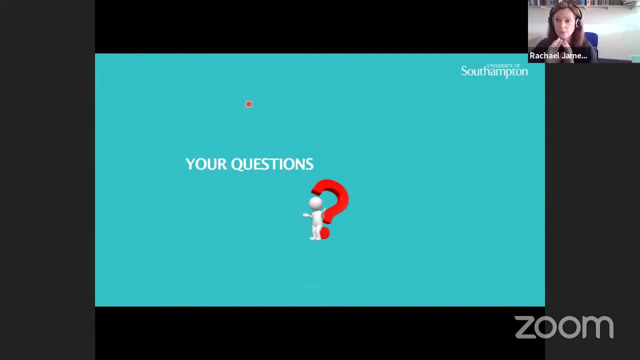 up new mines and start crushing up up new mines and start crushing up material purely for this reason, that material purely for this reason, that material purely for this reason. that that would be, that would be. that would be crazy, okay, so the next question. crazy okay, so the next question. 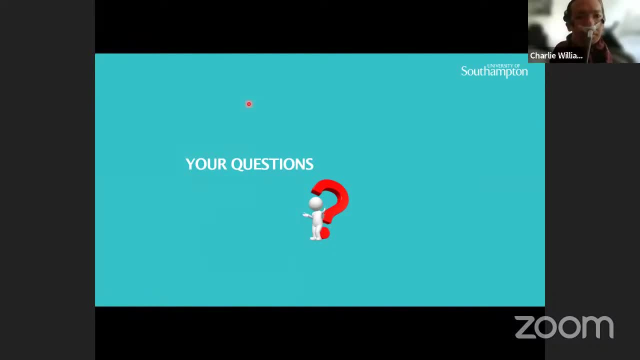 crazy. okay. so the next question is more about deep sea mining, is more about deep sea mining, is more about deep sea mining and it basically asks: could some of the? and it basically asks: could some of the? and it basically asks: could some of the by-products of deep sea mining? by-products of deep sea mining. by-products of deep sea mining, such as the triangle carbonates, be used. such as the triangle carbonates be used. such as the triangle carbonates be used to offset ocean acidification. uh for deep sea mining generally. uh for deep sea mining generally. 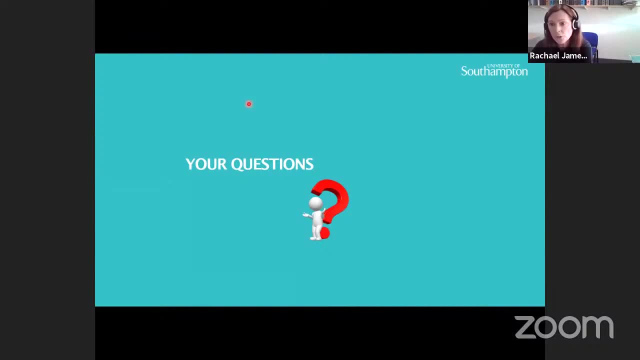 uh, for deep sea mining. generally speaking, we wouldn't. we wouldn't be speaking, we wouldn't, we wouldn't be speaking, we wouldn't, we wouldn't be mining carbonates because they don't mining carbonates, because they don't mining carbonates, because they don't contain sufficient quantities. 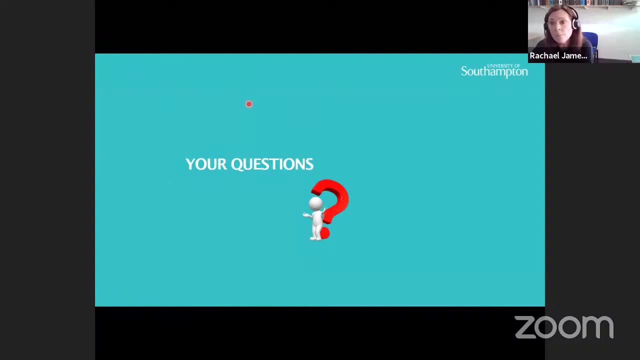 contain sufficient quantities, contain sufficient quantities of the resources that we need, of the resources that we need, of the resources that we need, um uh. we principally be looking at um uh. we principally be looking at um uh. we principally be looking at uh. hydrothermal sulfides, manganese. 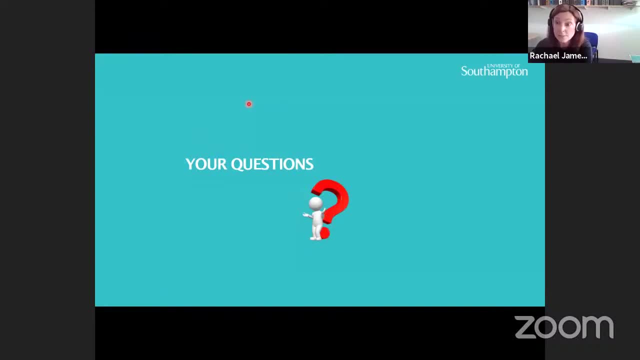 uh hydrothermal sulfides- manganese. uh. hydrothermal sulfides- manganese. nodules um, nodules um, nodules um and the and the deep sea clays as well, and the. and the deep sea clays as well, and the and the deep sea clays as well. so we're 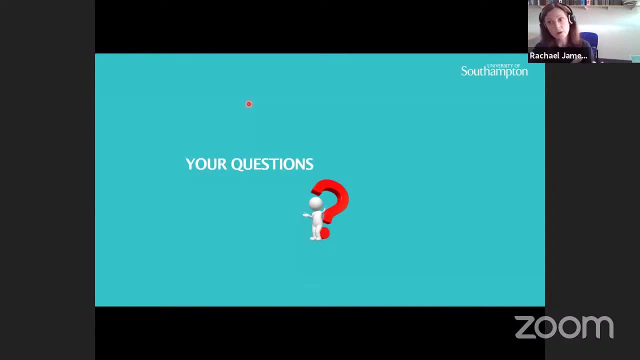 so we're, so we're, generally speaking, the resources that we generally speaking, the resources that we generally speaking, the resources that we need are not going to be found in the need, are not going to be found in the need, are not going to be found in the carbonate rich. 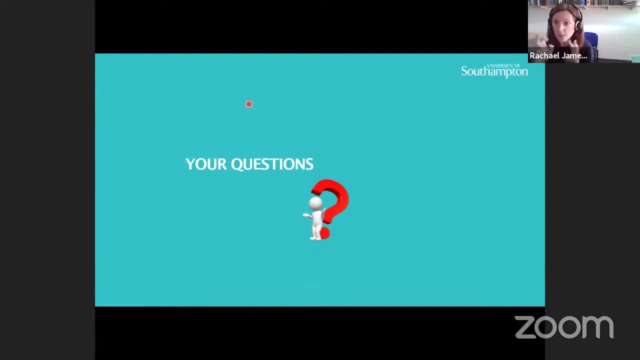 carbonate rich carbonate rich- parts of the ocean, but it is an parts of the ocean. but it is an parts of the ocean. but it is an interesting question that actually has a interesting question, that actually has a interesting question that actually has a bearing, bearing, bearing on um uh. 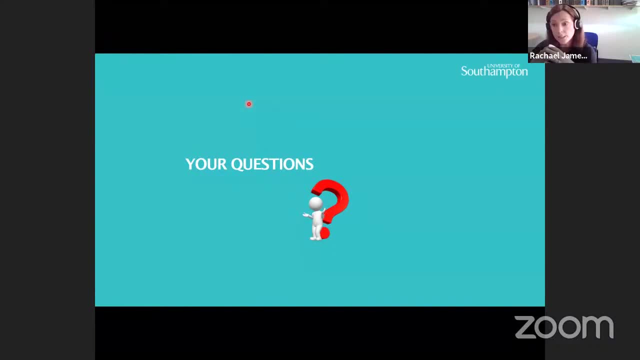 on um uh, on um uh. the the other part of my talk where i the the other part of my talk where i the the other part of my talk where i where i was looking, where i was looking, where i was looking at um carbon dioxide removal on land. 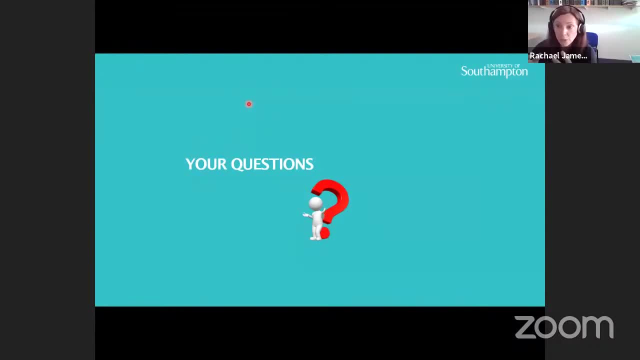 at um carbon dioxide removal on land, at um carbon dioxide removal on land, because, because, because, because actually the weathering part of that, because actually the weathering part of that, because actually the weathering part of that process- process creates alkalinity, and so if those sites 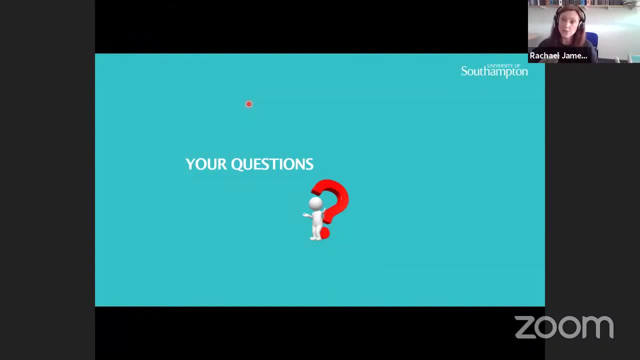 creates alkalinity, and so if those sites creates alkalinity, and so if those sites are close to the ocean, are close to the ocean, are close to the ocean, and that alkalinity is transferred to the, and that alkalinity is transferred to the, and that alkalinity is transferred to the ocean without, 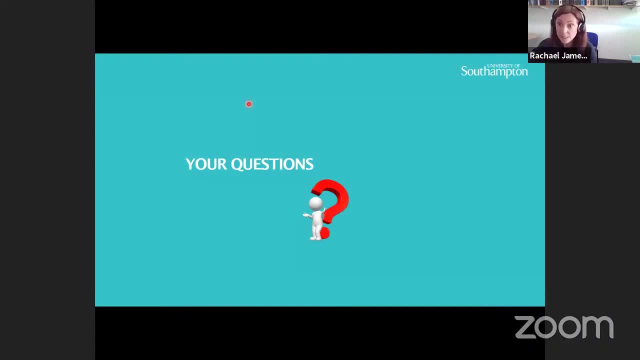 ocean without ocean, without the carbonate precipitation process, the carbonate precipitation process, the carbonate precipitation process happening, happening, happening, uh. then then actually that could partly uh, then then actually that could partly uh, then then actually that could partly combat um ocean acidification, combat um ocean acidification, combat um ocean acidification. so alkalinity enhancement as a result of 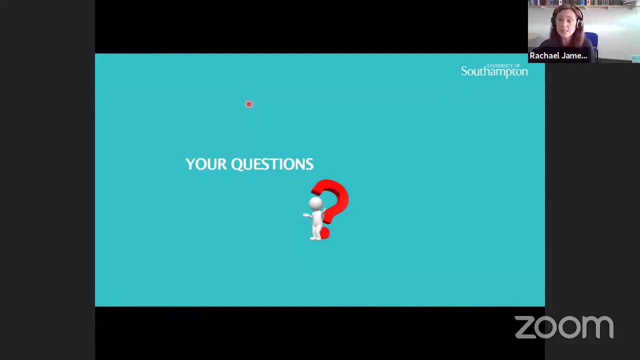 so alkalinity enhancement as a result of so alkalinity enhancement as a result of that enhanced weathering process. that enhanced weathering process, that enhanced weathering process, could uh help to mitigate ocean, could uh help to mitigate ocean, could uh help to mitigate ocean acidification. 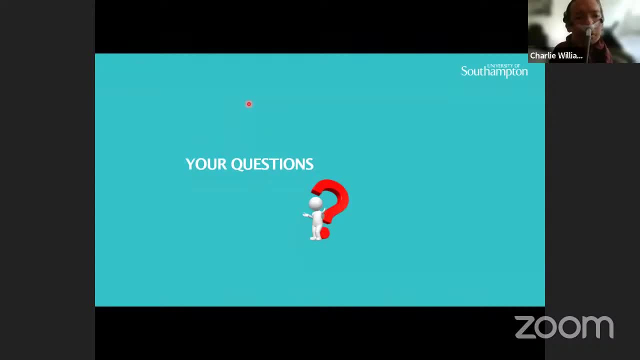 acidification, acidification, okay, and i think we've got time for okay, and i think we've got time for okay, and i think we've got time for one more question, which is one more question, which is one more question, which is hopefully a, uh, hopeful way to edge. 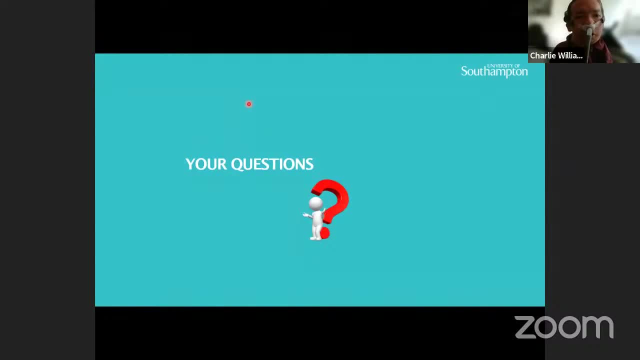 hopefully a uh hopeful way to edge- hopefully a uh hopeful way to edge the question from one of the attendees. the question from one of the attendees. the question from one of the attendees is: do you think it's possible? is: do you think it's possible is: do you think it's possible to reverse many of the negative effects? 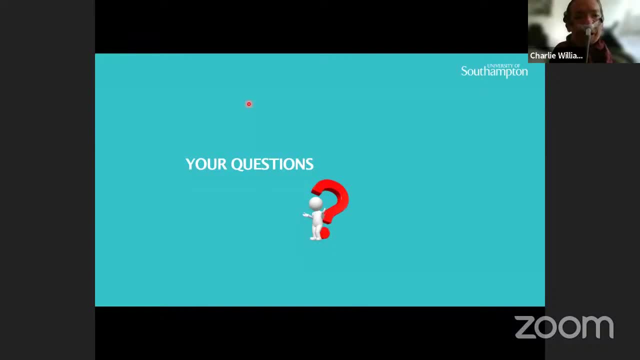 to reverse many of the negative effects, to reverse many of the negative effects of, of of anthropogenic warming, using these large anthropogenic warming, using these large anthropogenic warming, using these large scale, scale, scale geoengineering projects, geoengineering projects, geoengineering projects. so, if they're applied at sufficient, 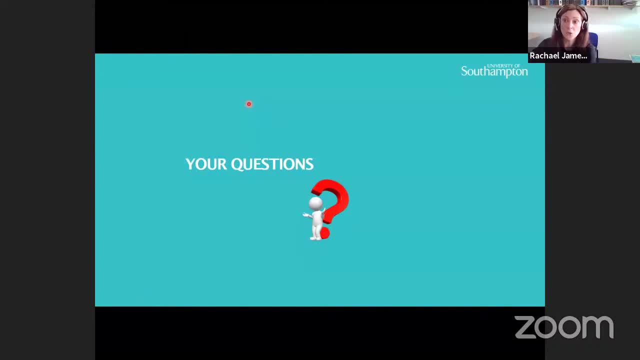 so if they're applied at sufficient. so if they're applied at sufficient scale, scale scale. there is the potential to um uh. there is the potential to um uh. there is the potential to um uh. yeah, lower levels of atmospheric carbon. yeah, lower levels of atmospheric carbon. yeah, lower levels of atmospheric carbon dioxide. 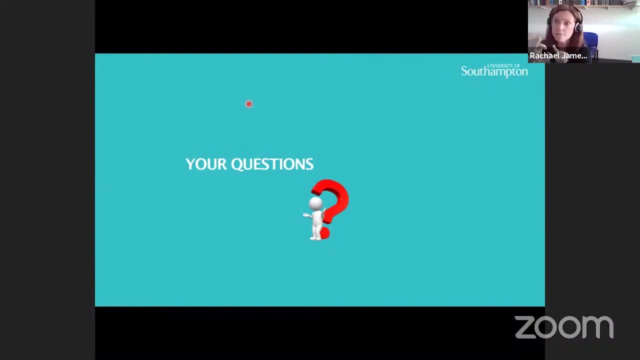 dioxide, dioxide. i think the the only thing there is. no, i think the the only thing there is. no, i think the the only thing there is no. magic bullet here, magic bullet here, magic bullet here. okay, none of the techniques i i talked. okay, none of the techniques i i talked. 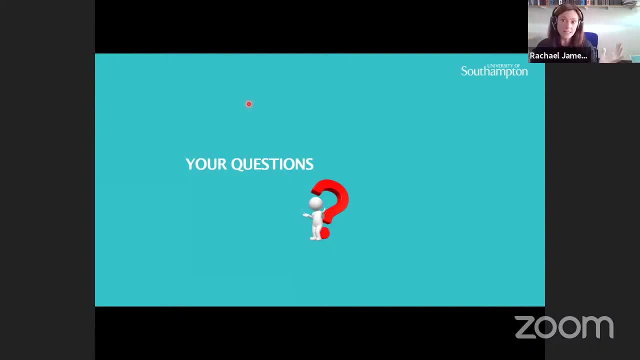 okay, none of the techniques i i talked about today are magic bullets and it's about today are magic bullets and it's about today are magic bullets and it's going to take a blend of natural, going to take a blend of natural, going to take a blend of natural techniques, such as afforestation. 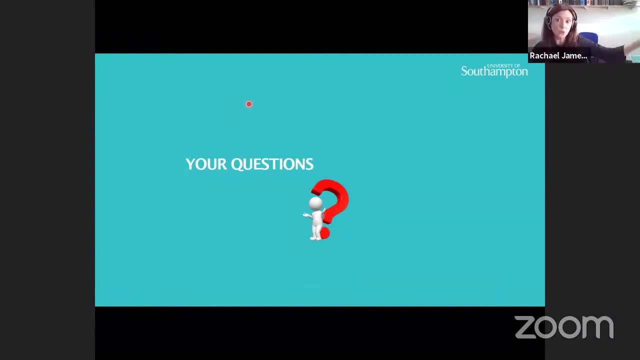 techniques such as afforestation. techniques such as afforestation, reforestation, reforestation, reforestation, uh blue carbon, so so replacing um i'm uh blue carbon, so so replacing um. i'm uh blue carbon, so so replacing um. i'm pointing out here because i'm 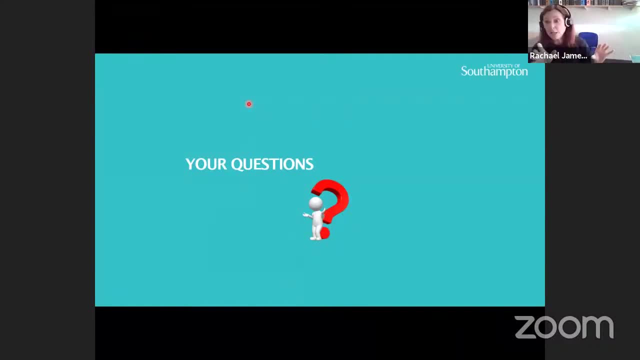 pointing out here, because i'm pointing out here because i'm in southampton, i could see the ocean in southampton. i could see the ocean in southampton. i could see the ocean today, uh, today, uh, today, uh, mangroves um, mangroves um, mangroves, um, and that kind of thing it's going to take. 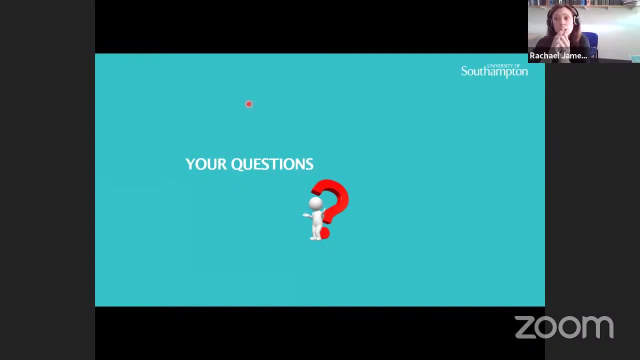 and that kind of thing it's going to take. and that kind of thing it's going to take, a blend of all those different, a blend of all those different, a blend of all those different technologies, technologies, technologies, but of course, the massive thing that we, but of course the massive thing that we. 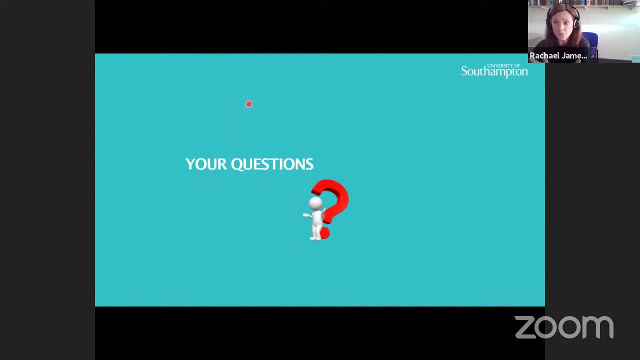 but, of course, the massive thing that we need to do is to stop carbon dioxide need to do is to stop carbon dioxide. need to do is to stop carbon dioxide emissions in the first place. uh, there's emissions in the first place. uh, there's emissions in the first place. uh, there's absolutely no way that a geoengine 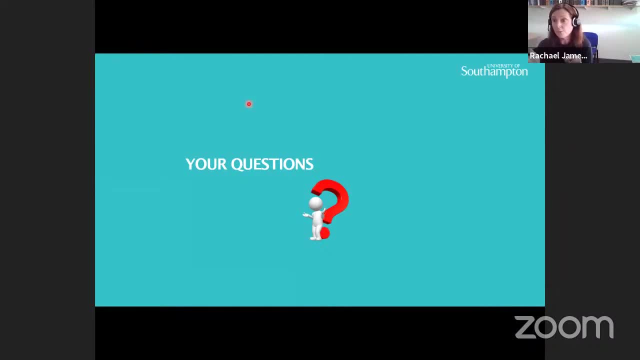 absolutely no way that a geoengine, absolutely no way that a geoengine and geoengineering techniques, either by and geoengineering techniques, either by and geoengineering techniques, either by themselves or combined themselves, or combined themselves or combined are going to be any substitute for doing are going to be any substitute for doing. 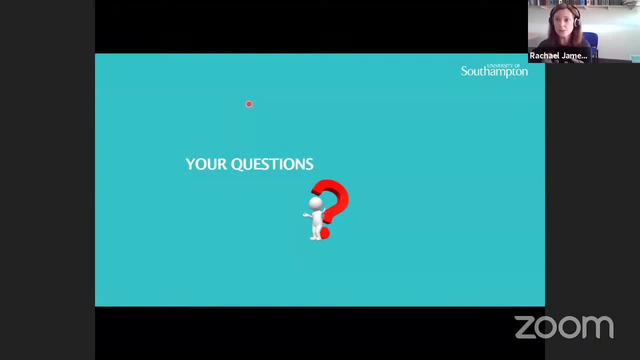 are going to be any substitute for doing that. that's the most important thing, is that that's the most important thing, is that that's the most important thing is reducing emissions, reducing emissions, reducing emissions, and then and then and then, from those industries that are difficult, from those industries that are difficult. 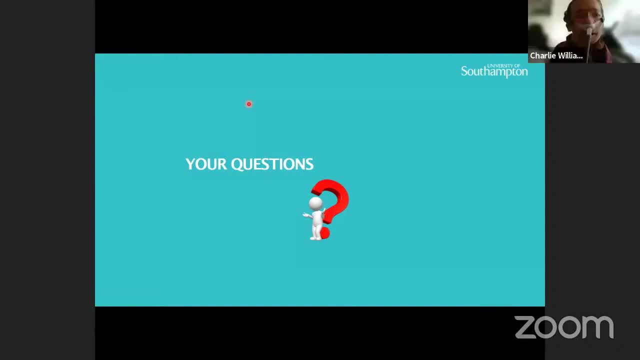 from those industries that are difficult to decarbonize, to decarbonize, to decarbonize. okay well, thank you very much again. okay well, thank you very much again. okay well, thank you very much again. um. so this is the end of um. so this is the end of. 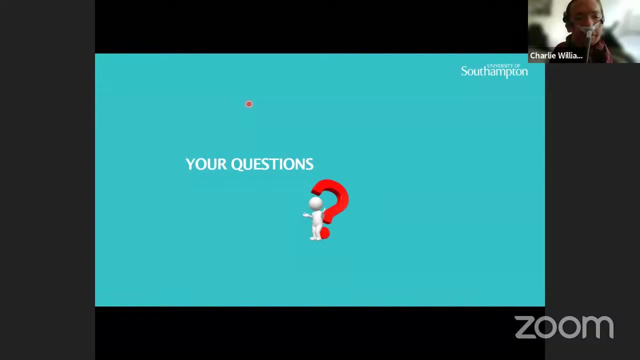 um, so this is the end of this uh session, um, or rather the end of this uh session, um, or rather the end of this uh session, um, or rather the end of the invited speakers part. thank you, the invited speakers part. thank you, the invited speakers part. thank you again to. 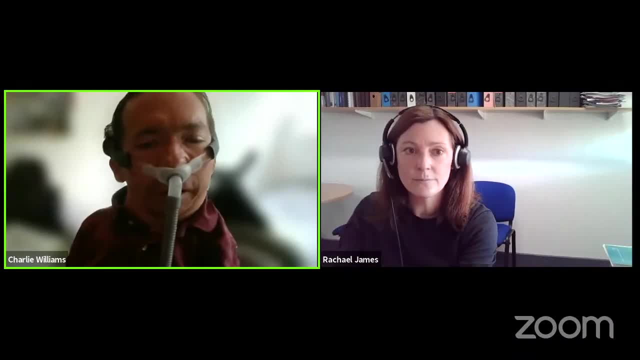 again to again to carl and rachel. and thank you also to carl and rachel. and thank you also to carl and rachel. and thank you also to the other speakers earlier the other speakers earlier the other speakers earlier earlier on this afternoon, earlier on this afternoon. 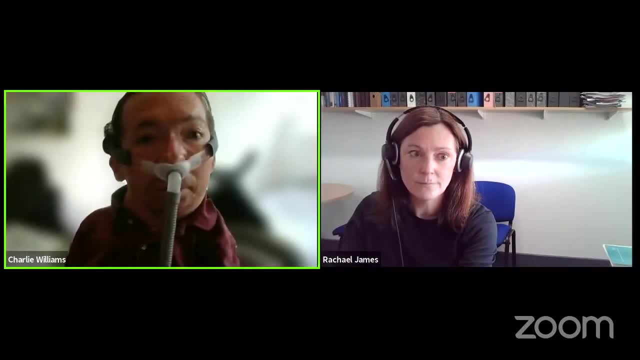 on this afternoon. so we now have our breakout rooms um i. so we now have our breakout rooms um i. so we now have our breakout rooms um i believe that all the techniques believe that all the techniques believe that all the techniques would have been sent an email with a. 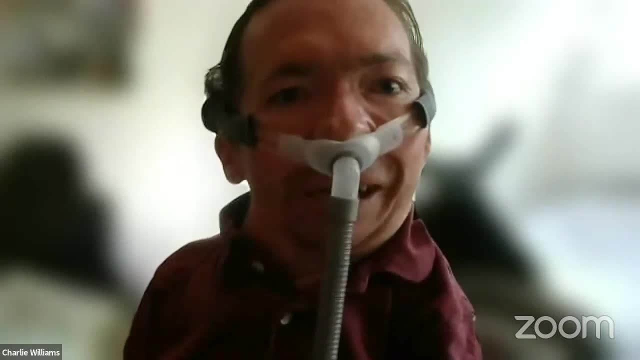 would have been sent an email with a would have been sent an email with a link to this. it is a link to this. it is a link to this. it is a separate zoom meeting, so it's not this separate zoom meeting, so it's not this separate zoom meeting, so it's not this room. 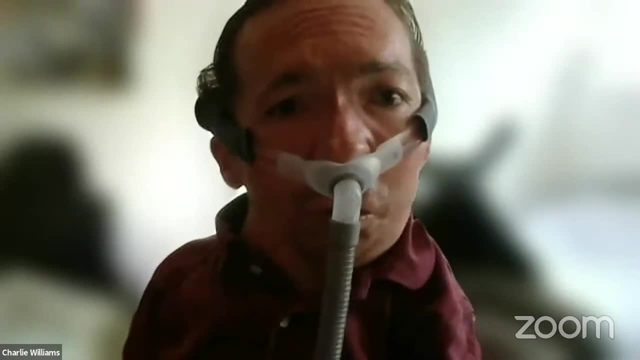 room, room um, and basically the idea is that all um, and basically the idea is that all um, and basically the idea is that all these short talks that you heard earlier, these short talks that you heard earlier, these short talks that you heard earlier, they will be there. 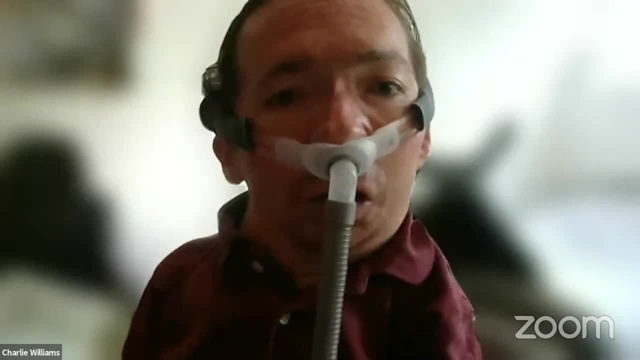 they will be there. they will be there in their own individual breakout room, in their own individual breakout room, where you can go and chat to them you, where you can go and chat to them you, where you can go and chat to them, you can ask questions about their posters. 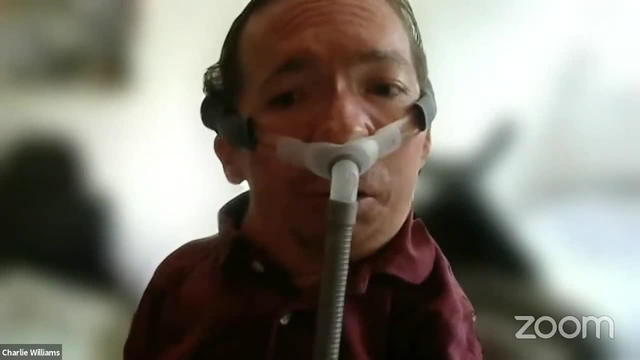 can ask questions about their posters, can ask questions about their posters and they can talk to you and they can talk to you and they can talk to you. the chat room is going to be open- any. the chat room is going to be open- any. the chat room is going to be open any minute and will be open. 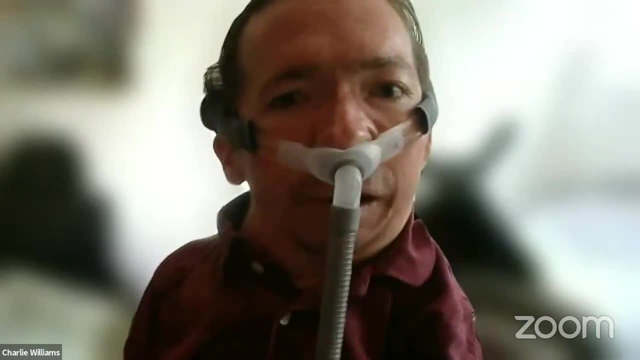 minute and will be open minute and will be open until 7 pm. then we will have a very until 7 pm. then we will have a very.